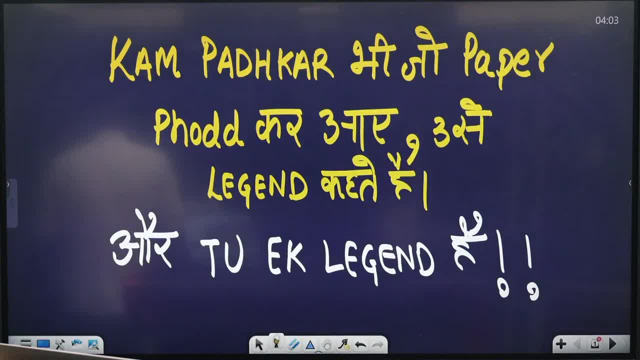 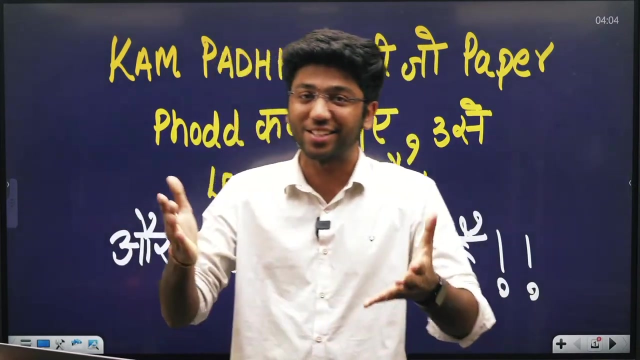 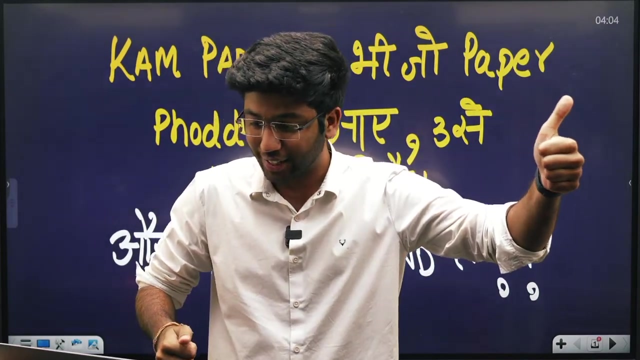 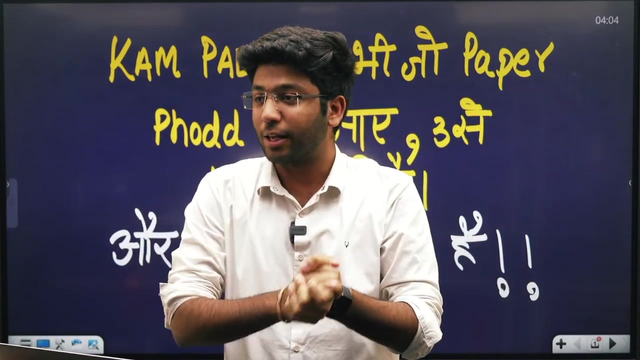 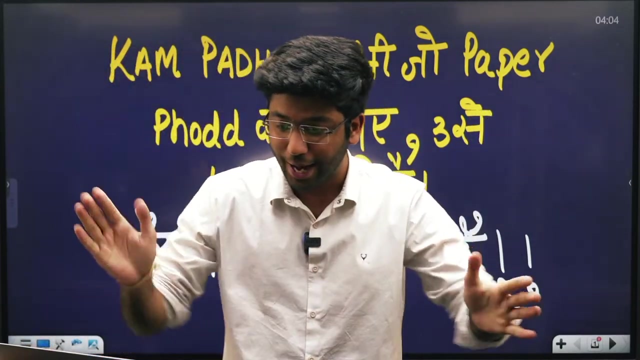 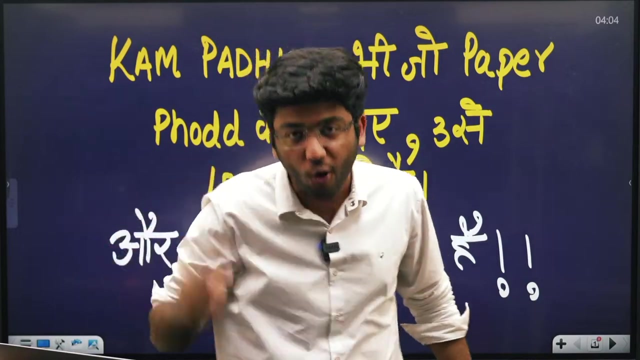 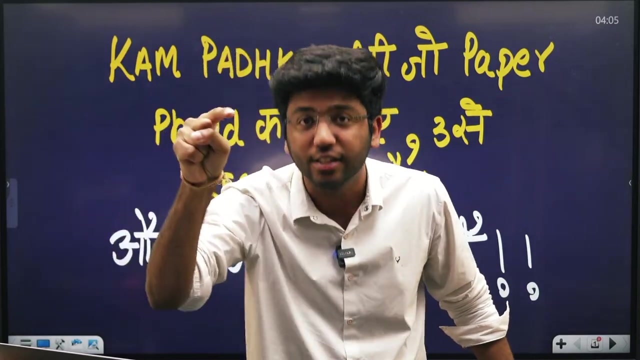 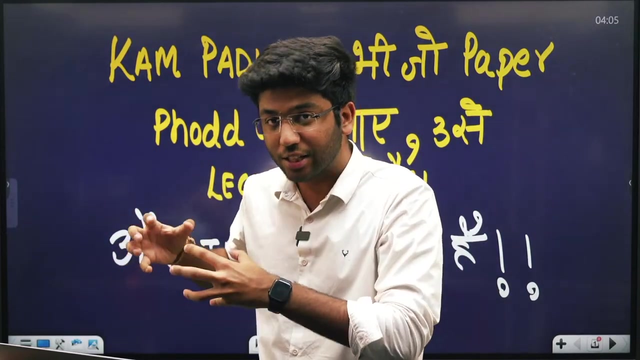 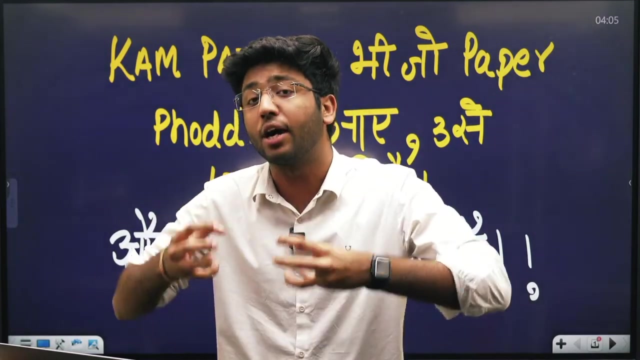 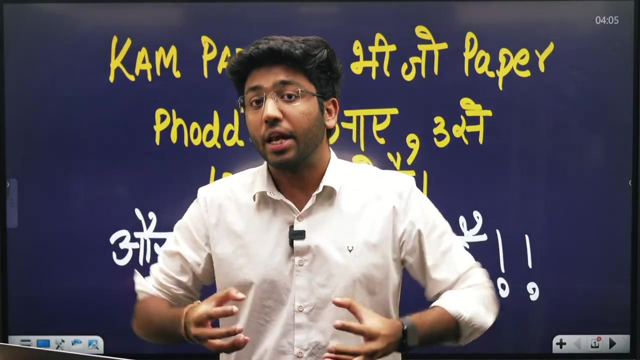 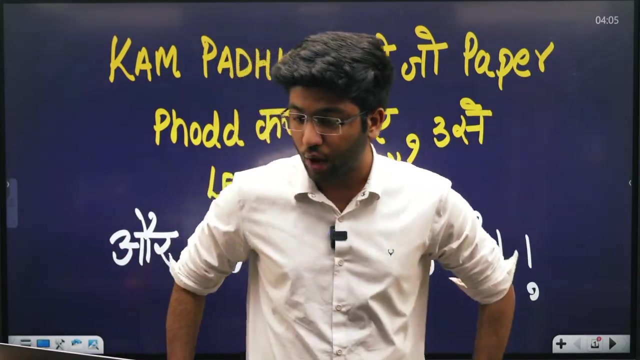 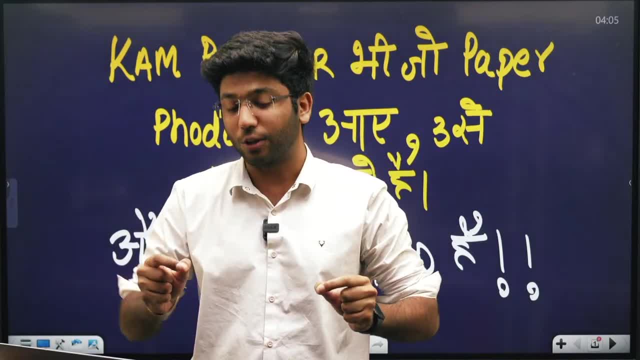 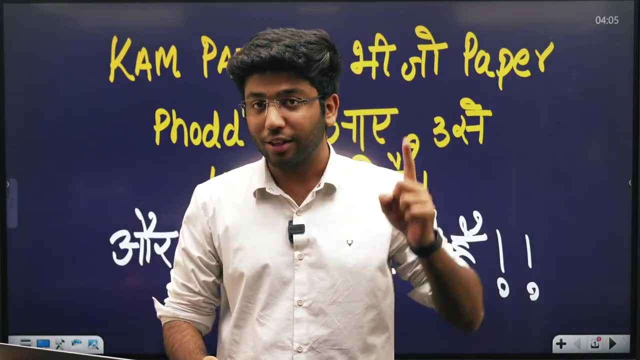 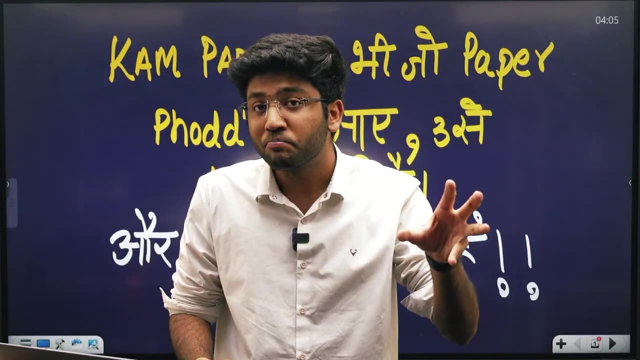 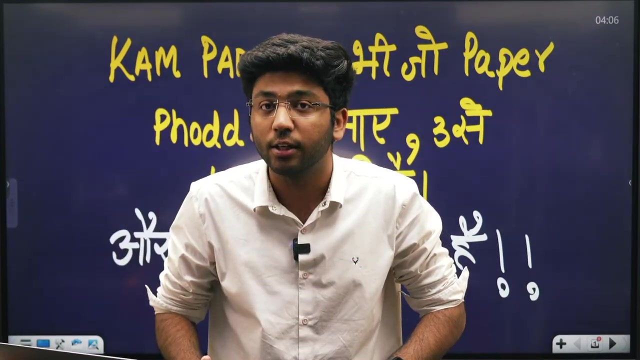 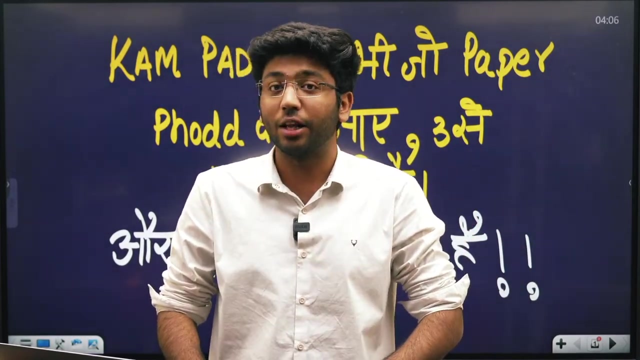 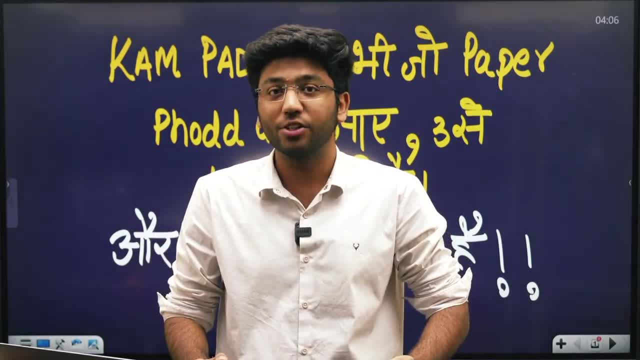 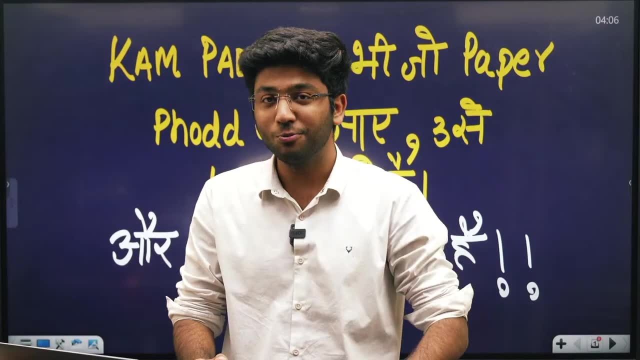 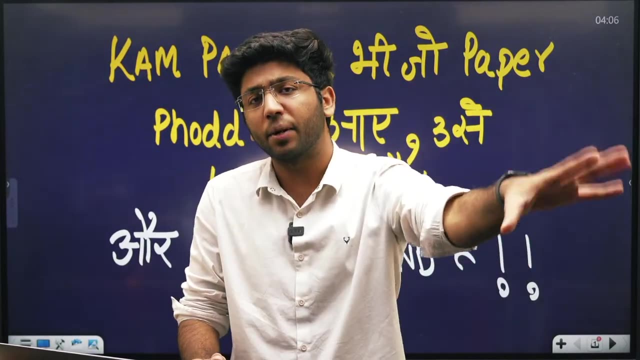 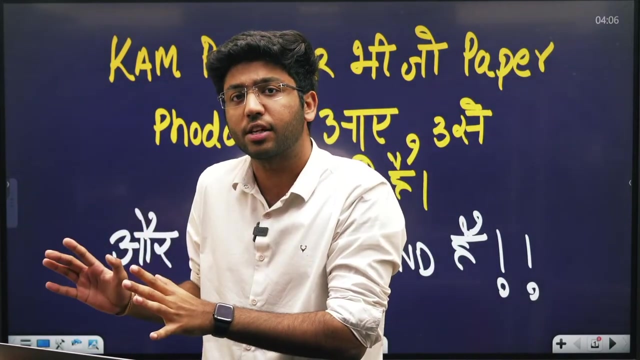 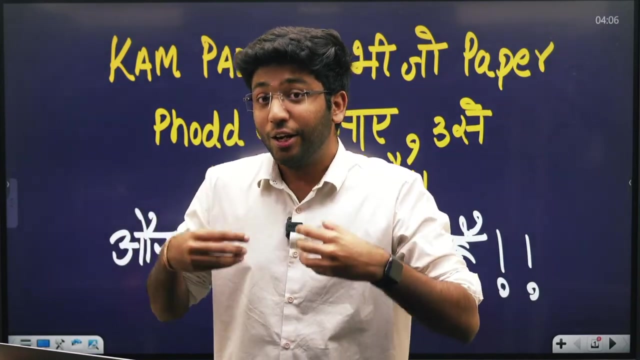 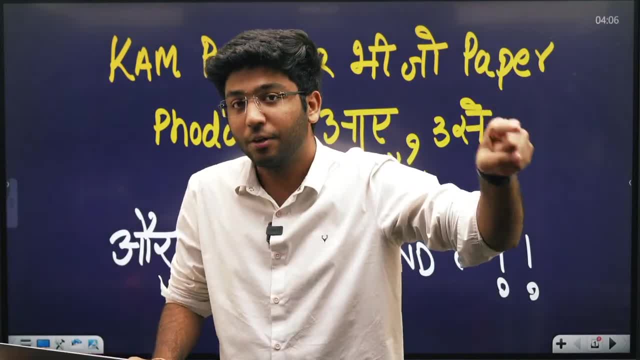 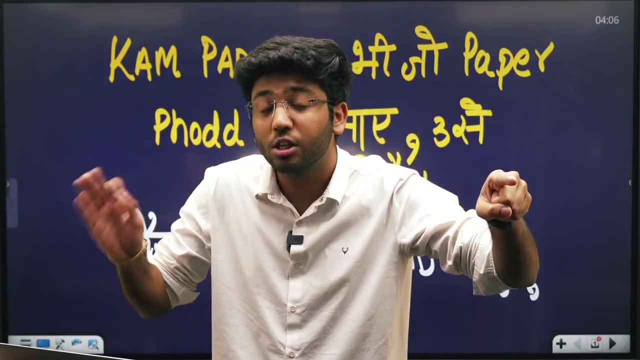 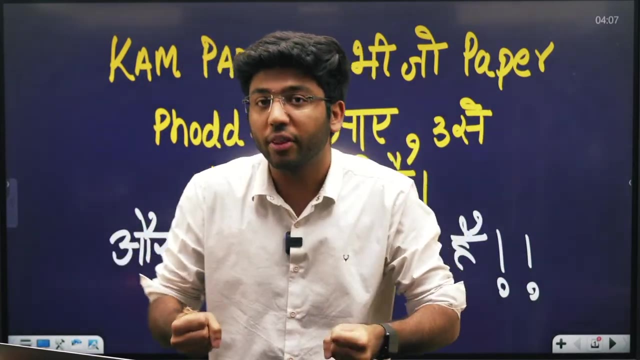 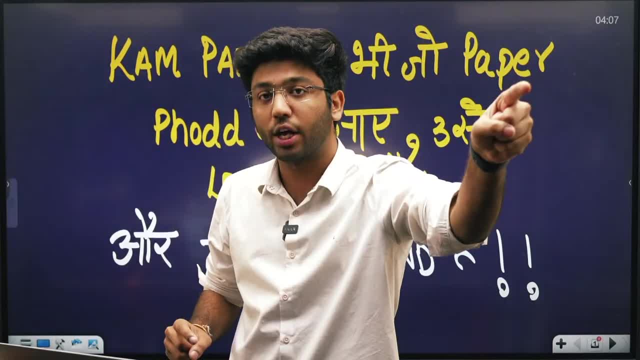 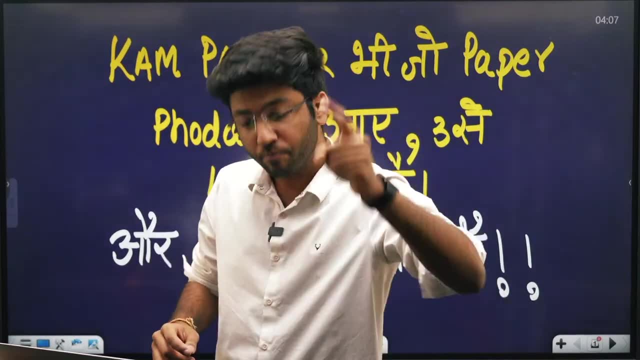 Both of us together. now we will go and break the paper, Even if we have studied less, no problem. Now read the things that I am going to tell you properly. Understand it carefully. You will come after breaking it. Did you understand what I said? 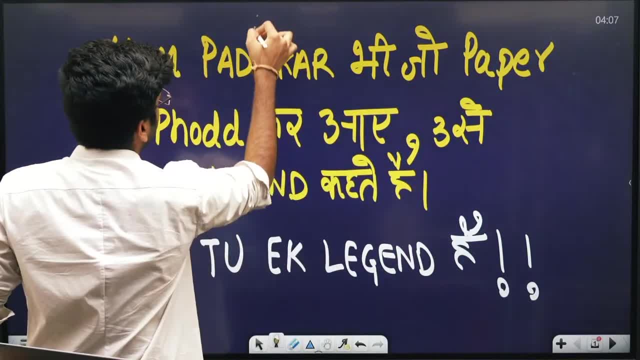 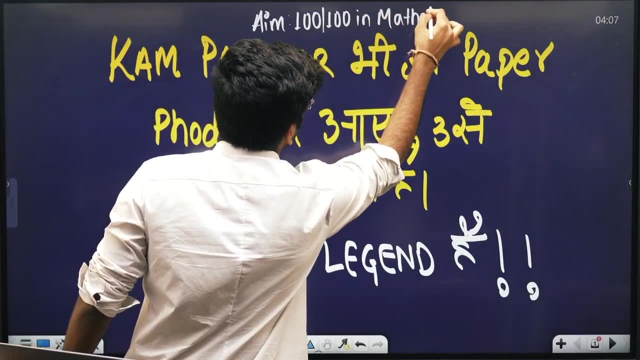 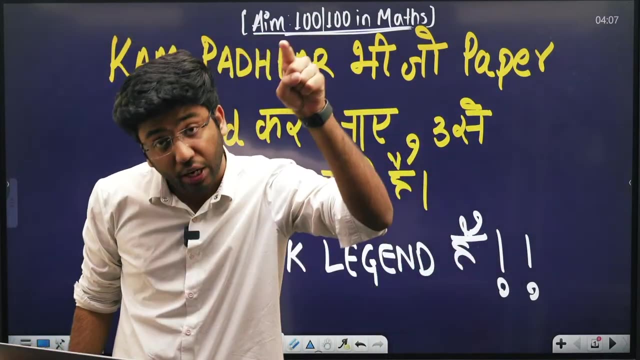 Our aim is that we have to bring 100 out of 100 maths exams. Our aim is that we have to bring 100 out of 100 maths exams. We will complete that aim today. We will complete that aim today. Write it on your copy for the last time. 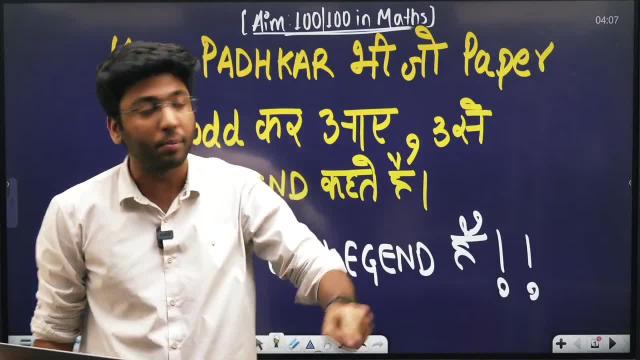 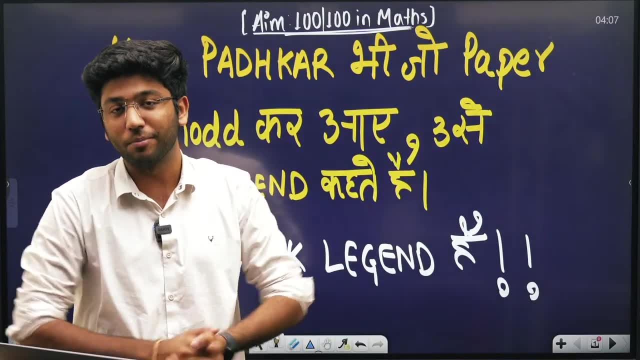 For the last time, because today is our exam. Write 100 out of 100 maths on your copy for the last time, And then we will start today's class, not today's class. We will start today's class. Okay, Okay, Okay. 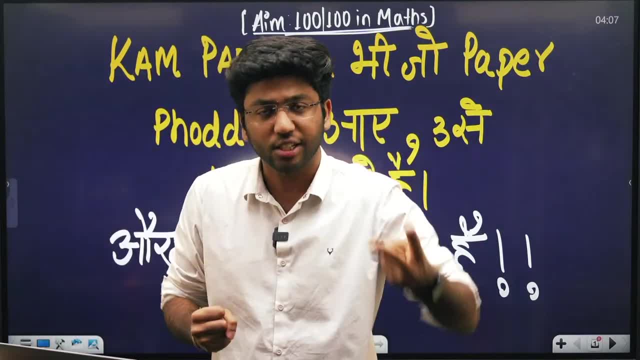 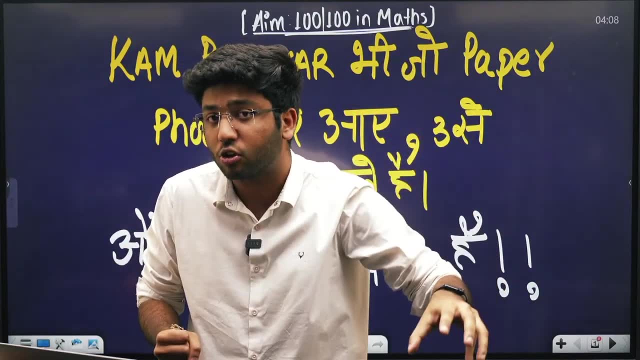 With full enthusiasm. You don't have to worry at all. You don't have to worry at all. In 1.5 to 2 hours we will complete this whole session. What are the possible questions from each chapter? What are the possible concepts? 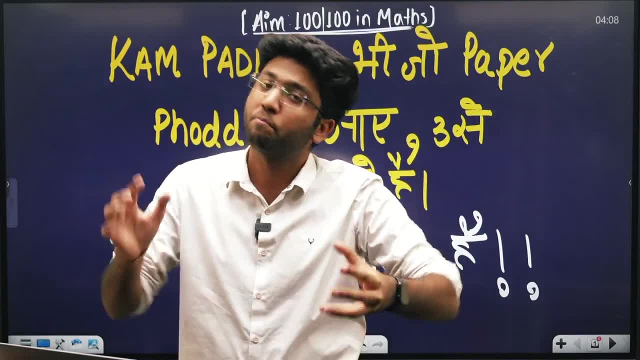 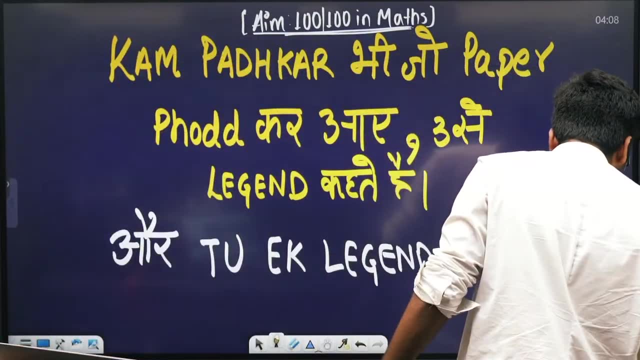 We will revise it quickly And by the end of today's session I will bid you farewell And you will come. after breaking the paper. Did you understand what I said? Let's start. Let's start. See, See, Your first chapter comes. 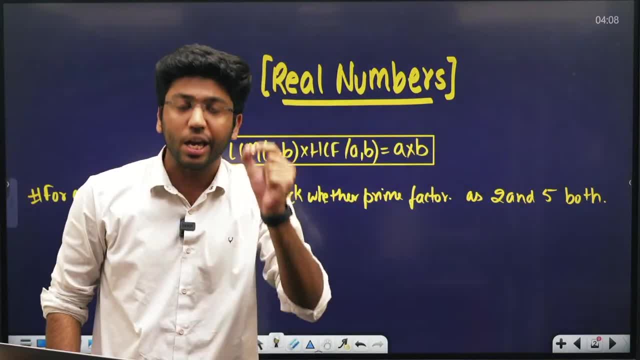 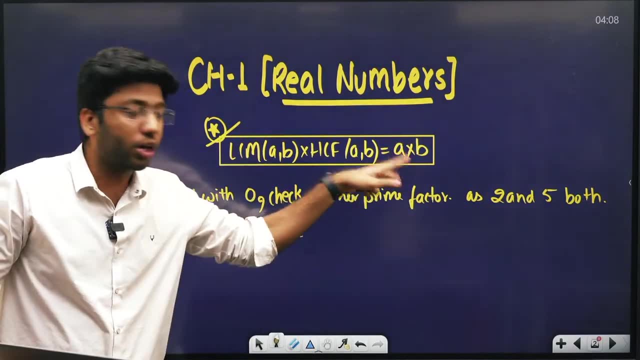 Your first chapter comes Your real numbers. The most important formula in real numbers is that if we make HCF of 2 numbers into LCM of 2 numbers, then it is a product of 2 numbers, LCM of 2 numbers. 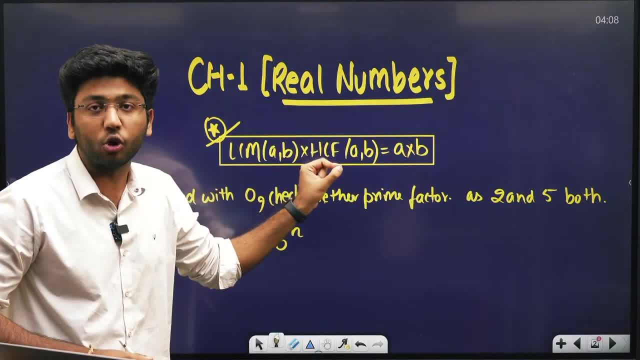 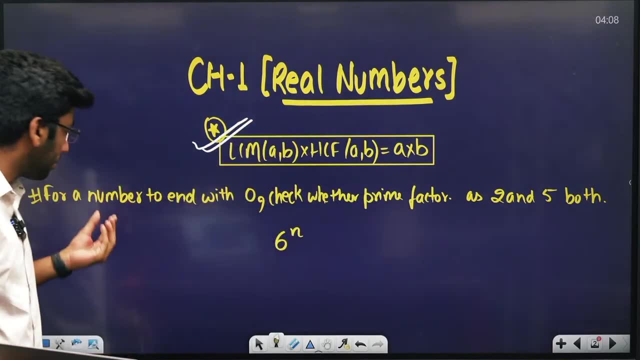 LCM into HCF is equal to product of 2 numbers. It is a very important formula. You can get to see the question from here. Did you understand what I said? This is the first important formula from this chapter. Now, if I talk, 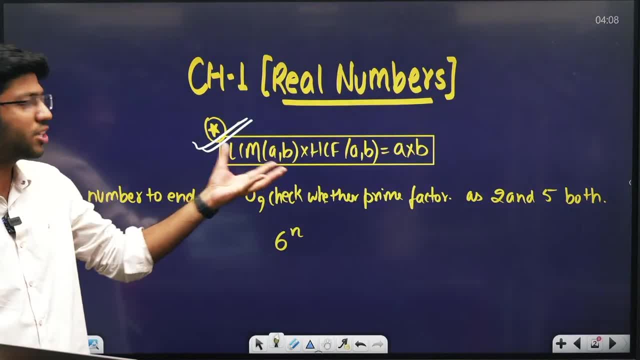 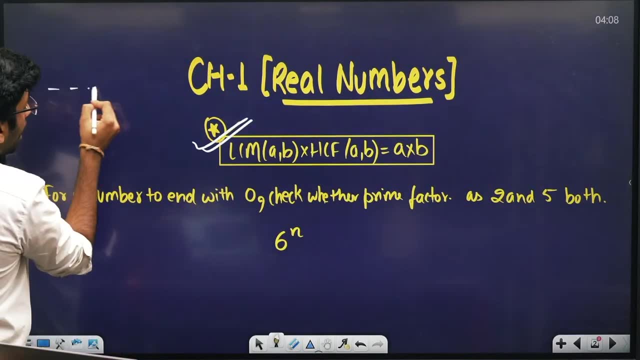 there is a very famous question which CBSC asks repeatedly. You all have read this chapter many times, So I will read it quickly. For a number to end with 0,. there is a number, If it has to end with 0,. 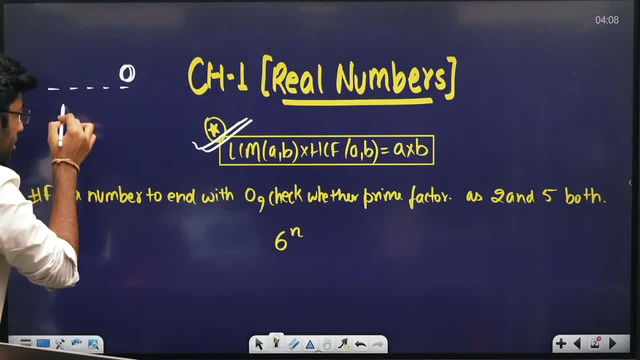 then in its prime factorization. what is prime factorization Like this? So if we do prime factorization of 18,, 2 9s are 18,, 3, 3s are 9, and 3, 1s are 3.. 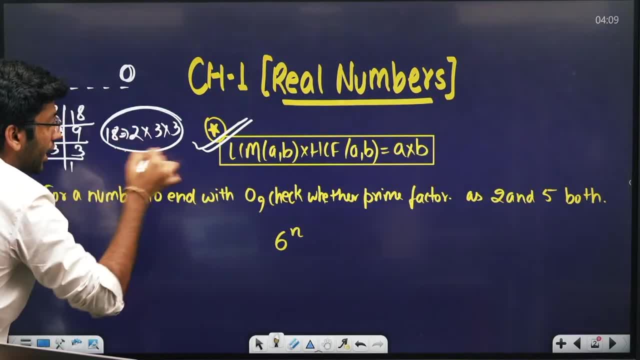 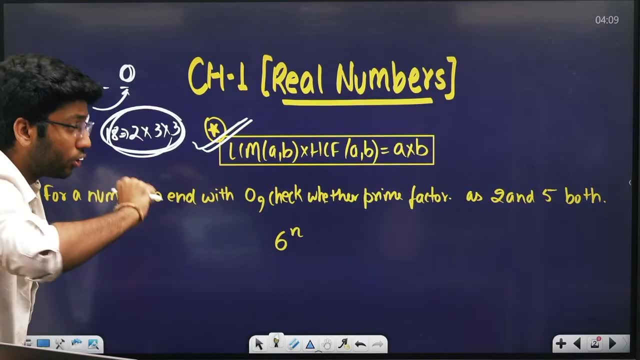 So prime factorization of 18 will be 2 into 3 into 3.. So it is being said that if any number has to end with 0, then in its prime factorization 2 and 5 should be both. What did I say? 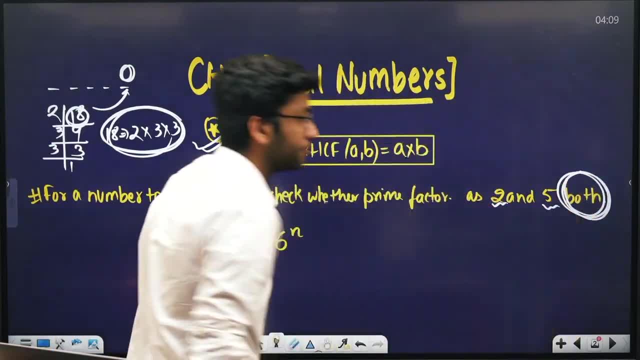 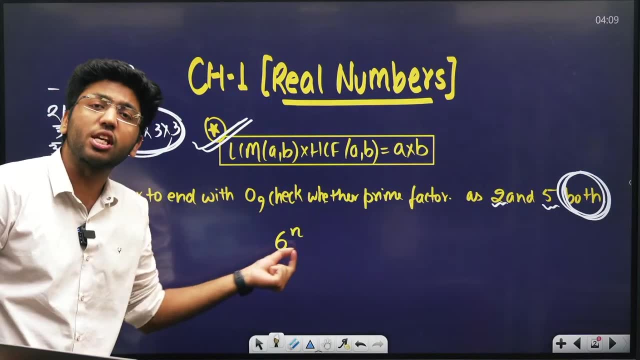 2 and 5 should be both. This is a very important thing which can come to you in the exam Like. it will give you a question that tell me what will end with 6 power n. It will ask you Check whether 6 power n. 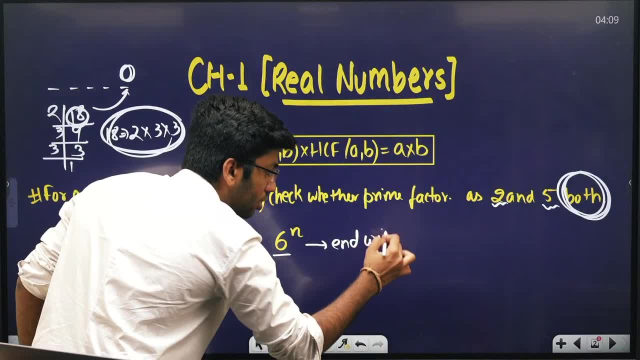 will end with 0. It will ask: you: Tell me, will it end with 0?? So what you have to do, You don't have to do anything. You have to do. prime factorization of 6.. 2, 3s are 6,. 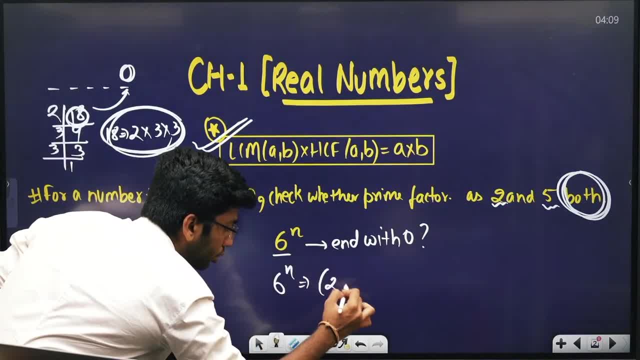 3 1s are 3.. So you can write 6 power n as 2 into 3 power n. Now you will say that in prime factorization 2 is coming, but 5 is not coming. 2 is coming. 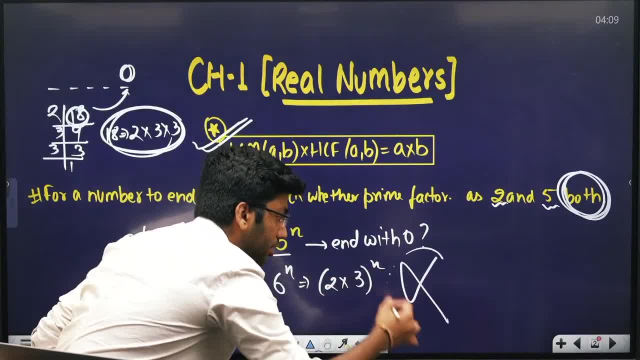 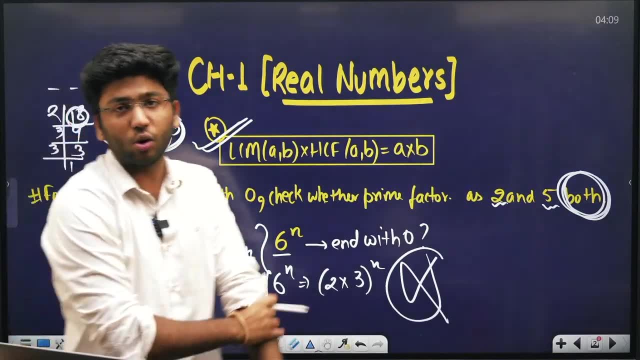 but 5 is not coming. That is why 6 power n cannot end with 0.. So from here, 6 power n, 7 power n, 5 power n will be asked like this and it will ask you: will it end with 0?? 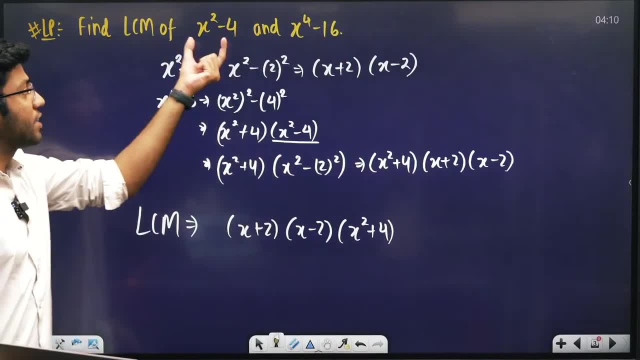 You will say that it will not end. Next, LCM of x square minus 4, x to the power 4 minus 16.. How do we get LCM? We all know that we have to take prime factorization for LCM also. 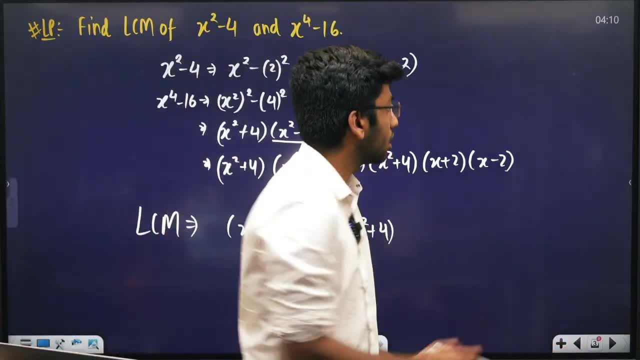 You can ask this kind of question to CBSE. Earlier CBSE used to ask that: tell me what will be the LCM of 18 and 36? Earlier it used to ask like this: Now it doesn't ask like this. Now it doesn't ask like this: 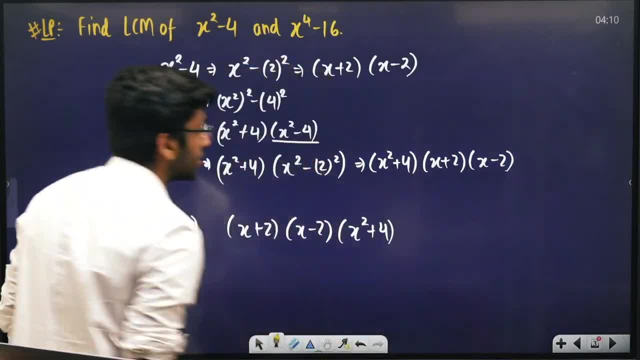 Now it will ask like this: So what will you do? What will you do? See, keep watching carefully. I will tell you the solution step by step, Because if I would have done the solution here, it would have taken a lot of time. 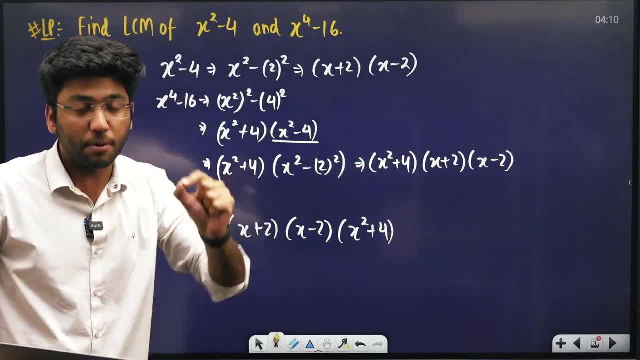 I have written it before In this I will tell you step by step. Okay, You have to stay here with full focus. I am asking you for 1.5 to 2 hours. In that, 1.5 to 2 hours. 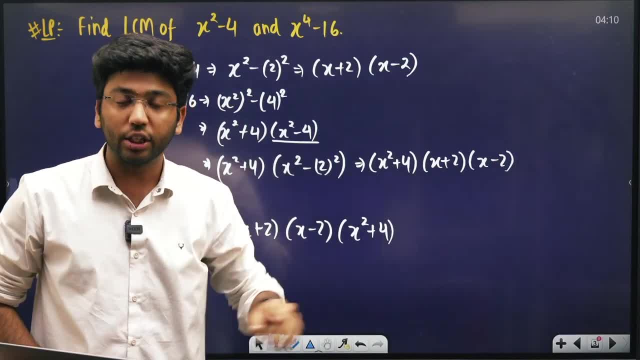 I will pick up the whole paper and put it in front of you In that 1.5 to 2 hours. I will pick up the whole paper and put it in front of you. You should have full focus here. Nothing else should happen. 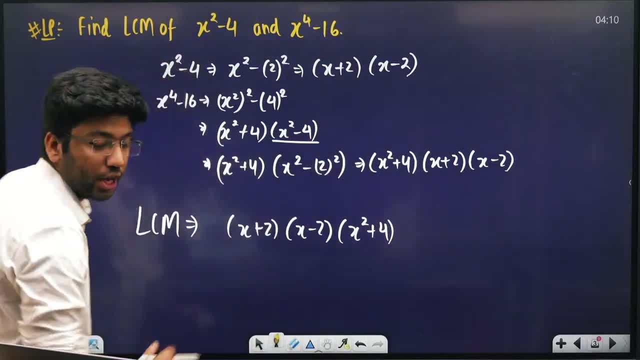 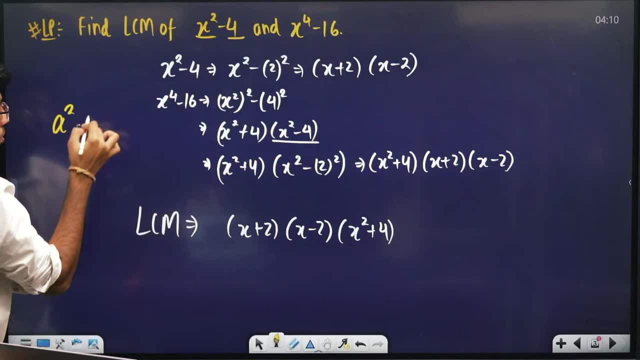 You should have full focus here. Understood, Understood. See x square minus 4.. If I talk about x square minus 4, then see what is a square minus b square. What is this, a plus b into a minus b. 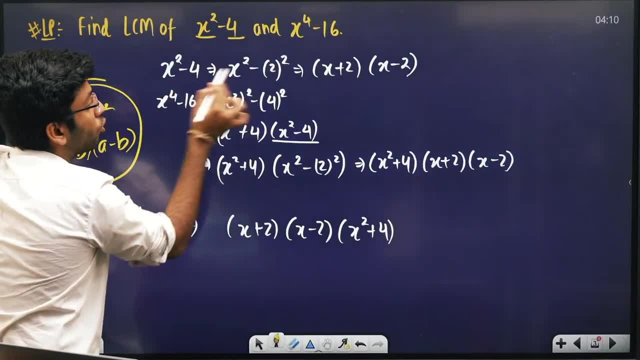 It happens. This is a very important formula. It will keep coming. So I have written 4 as 2 square, So a square minus b, square a plus b into a minus b. So I have made these two factors. 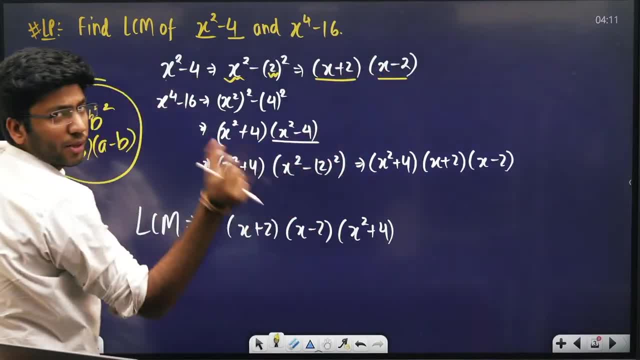 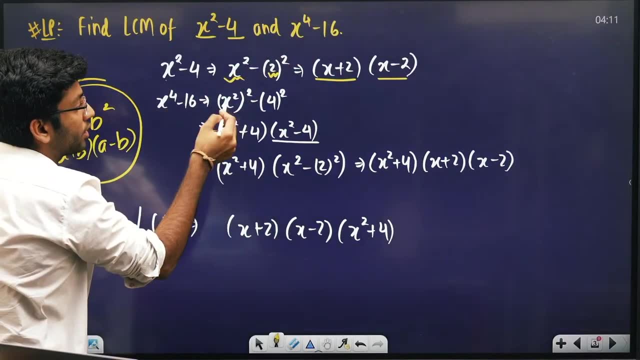 of x square minus 4.. I have made these two factors of this. Factor means what is being multiplied. It is called factor. So these two are factors. If I open x to the power of 4 minus 16, then I can write x to the power of 4. 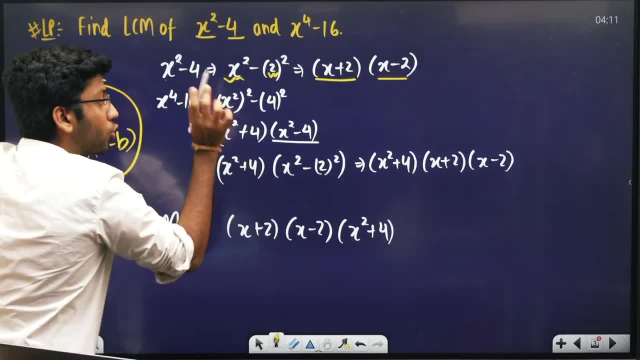 as the square of x square And I can write 16 as the square of 4.. So now, if I open this with a square minus b square, then a is now complete. Earlier a was just x, Now here. 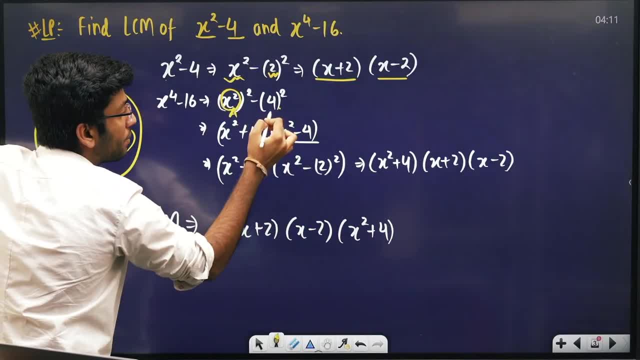 a is the square of x square, So a is complete of this. a minus b, So a square minus b square where a is x square, So a plus b into a minus b becomes like this: Now I have seen: 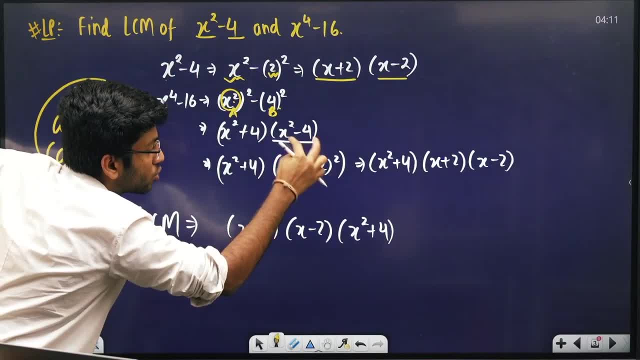 that it is being made exactly like this here, So I can open this also by doing a square minus b square. I have written 4 as 2 square, So it will become a square minus b square. So now this whole equation. 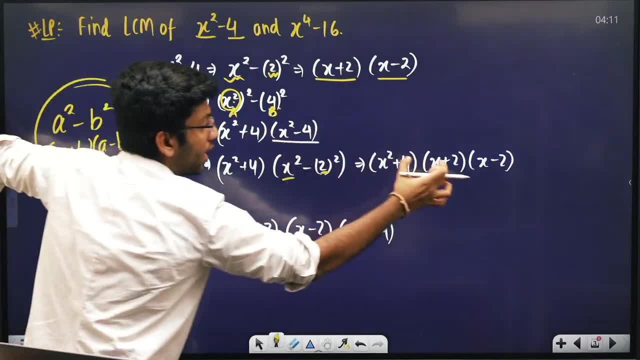 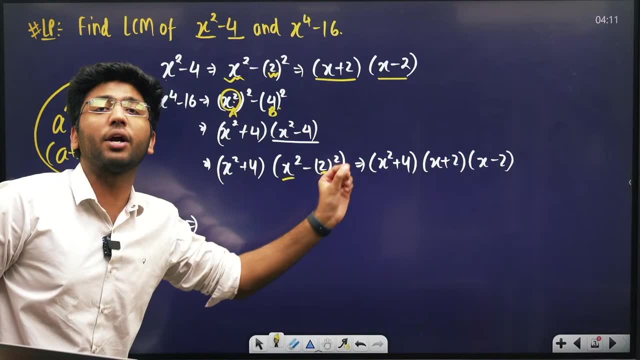 will be made. x square plus 4 is like this, And I have written this x plus 2 into x minus 2.. What is LCM? What is LCM? LCM is, whatever you see, different creatures. So if you see, 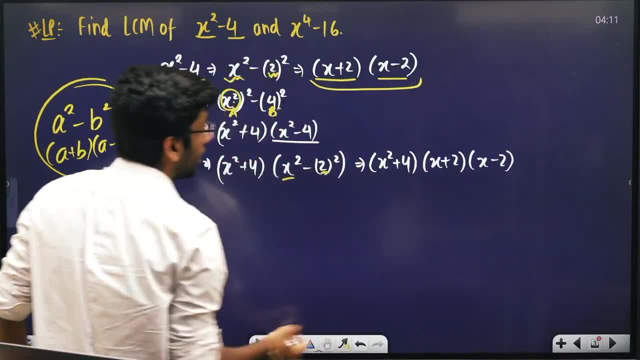 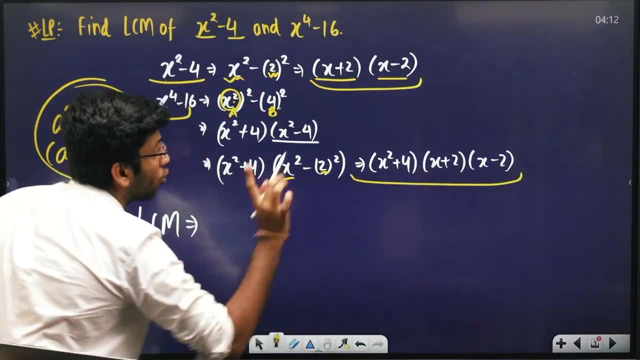 in prime factorization. whatever you see different creatures in prime factorization, first of all write it What all creatures are seen. different creatures: x plus 2 is seen- I have written this. x minus 2 is seen- I have written this. 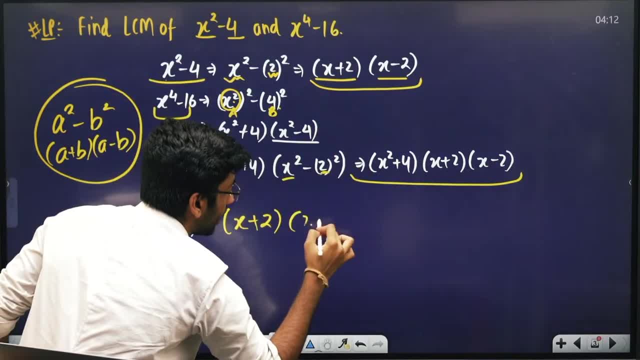 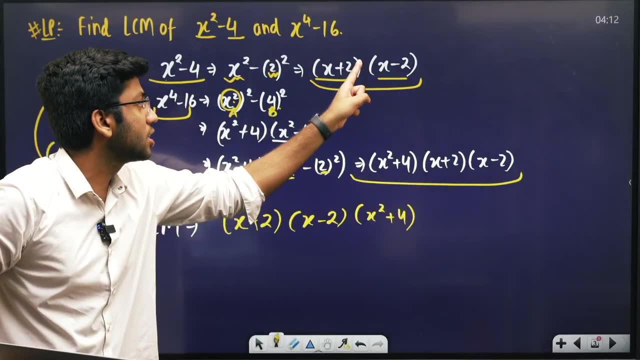 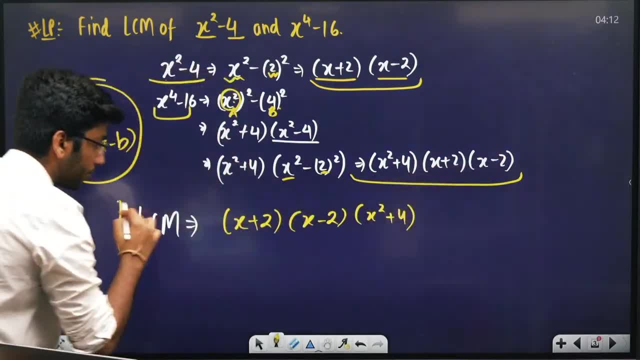 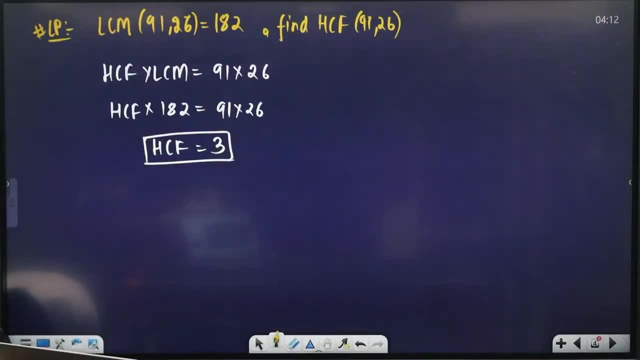 Its power is 1.. Its power is 1.. So this will be its LCM. This will be its LCM Understood. Next question. Next question. I will go fast so that you can understand. See this is. 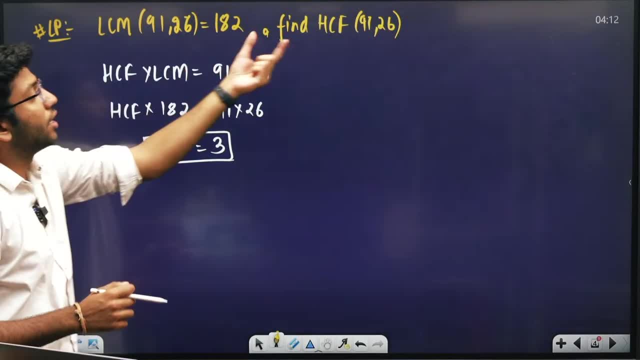 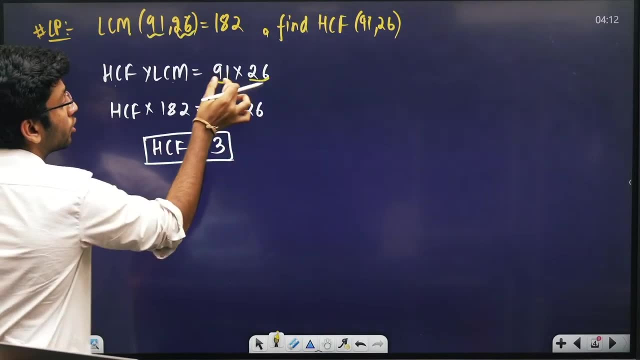 exactly the same question which I have just told, the formula That I have given you LCM. I have asked you what will be HCF. So we know what is LCM into HCF. Product of two numbers. Product of these two numbers. 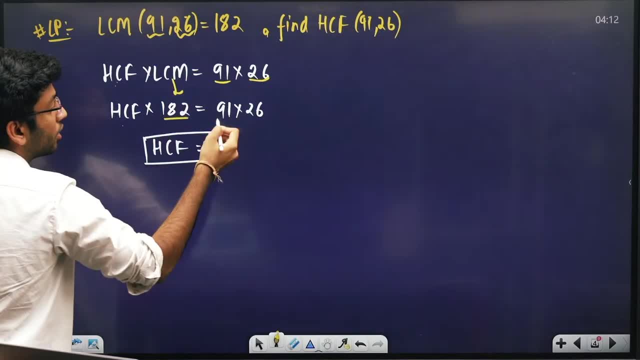 So, product of two numbers, You had to take out HCF. I have given you LCM, So I am doing it from here. So from here, if we do cut-peat, then the value of HCF will be 3.. 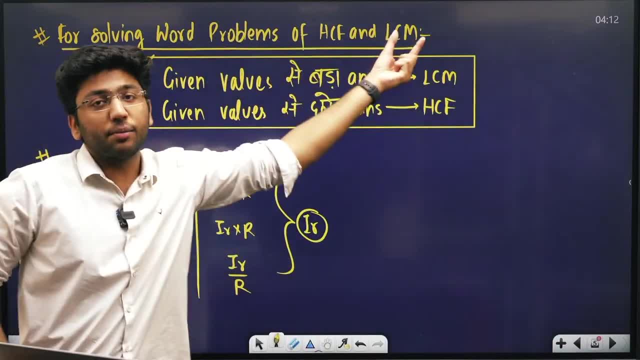 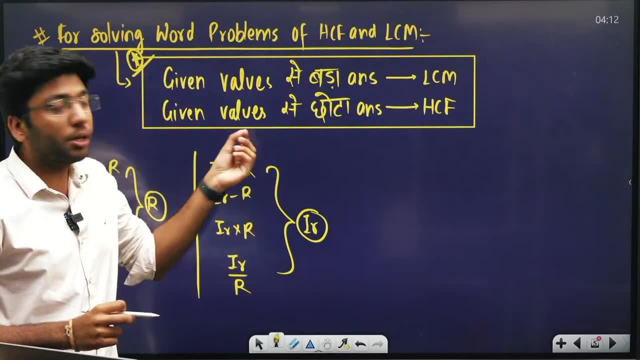 Such a direct question can come in your exam. Now see if we have to solve word problem of HCF and LCM, If we have to solve word problem of LCM. So to solve word problem, the best trick which is there is this: 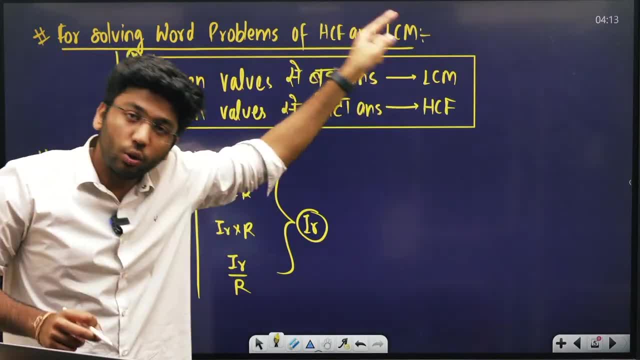 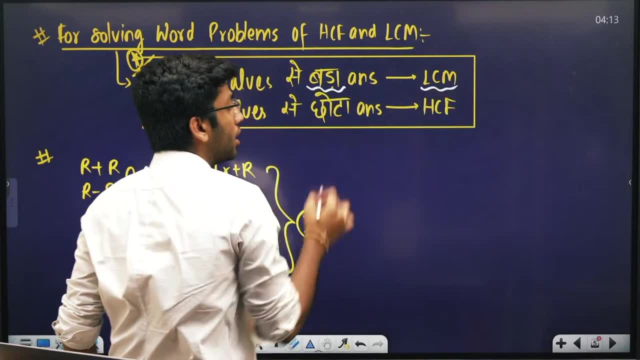 That if you want to get big answer from given value, then LCM See see. In LCM L means low. So if you want to get big answer, then you will take LCM. If you want to get small answer, then you will take. 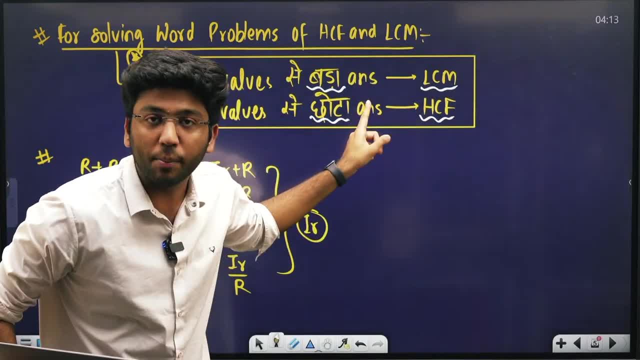 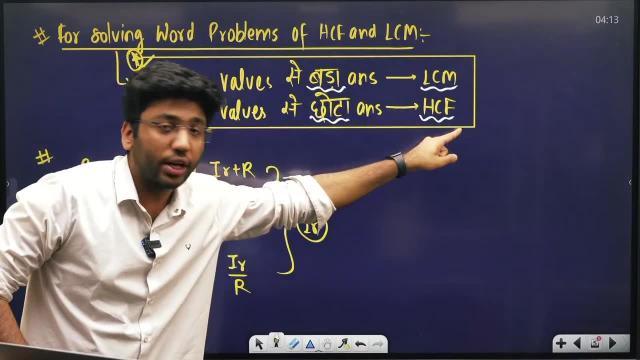 HCF. Just understand this line. Now I will ask you one or two questions, one or two examples, and you will understand. Now I will ask you one or two examples, and you will understand. If you want to get small answer, then you will take. 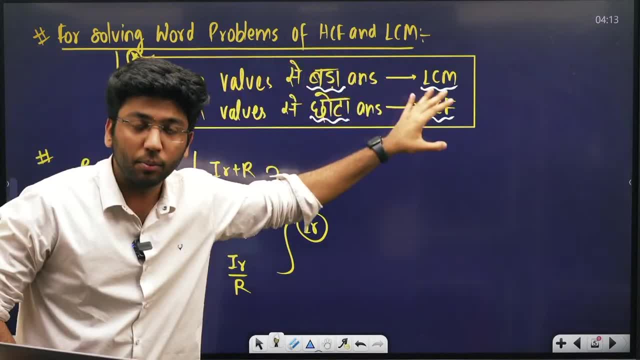 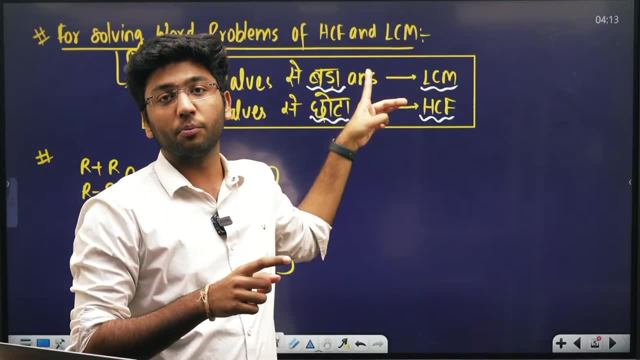 HCF. This is very important. We can get direct questions from this. Word problems. Look, there are three word problems in this whole chapter. One is HCF and LCM. So either the director will ask the question or he will ask. 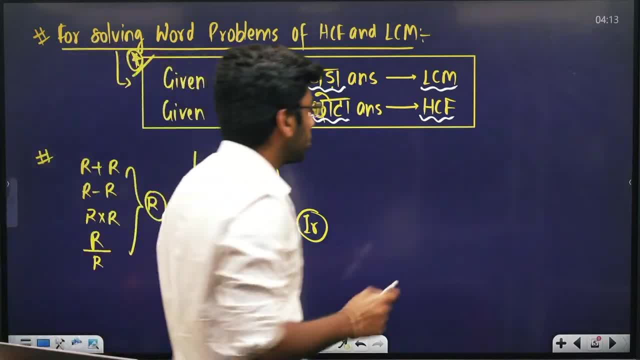 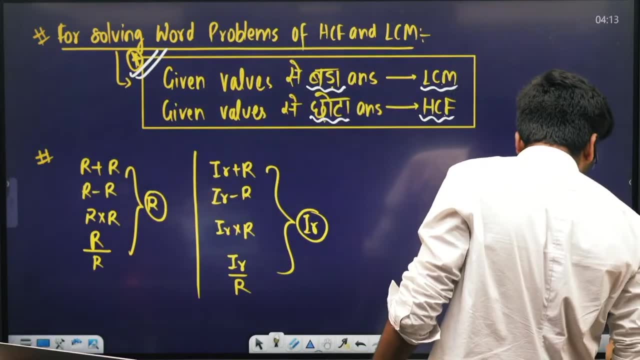 the word problem, or he will ask the one with irrationality. Okay, So remember this one: Bigger answer from given value then LCM, Smaller answer from given value, then HCF. Now I will tell you an example on this. 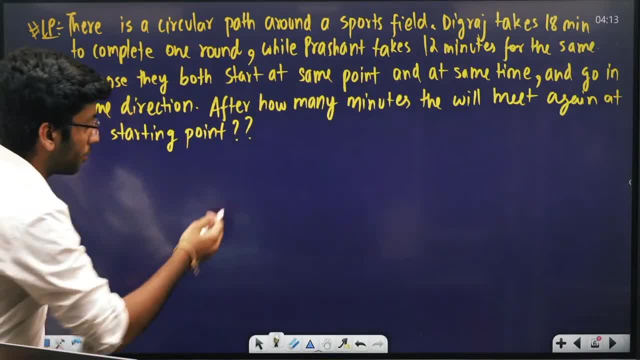 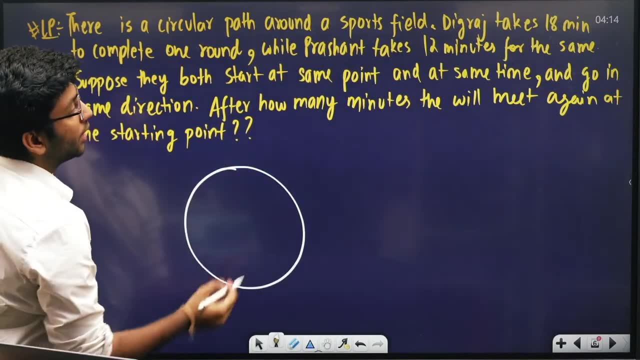 See, like CBC's favorite question, that there is a circular path. There is a circular path like this: There is a circular path around a sports field. Okay, There is a circular path like this. Digraj ji takes 18 minutes to complete. 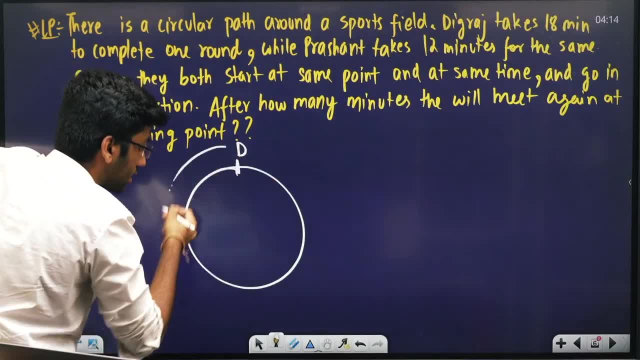 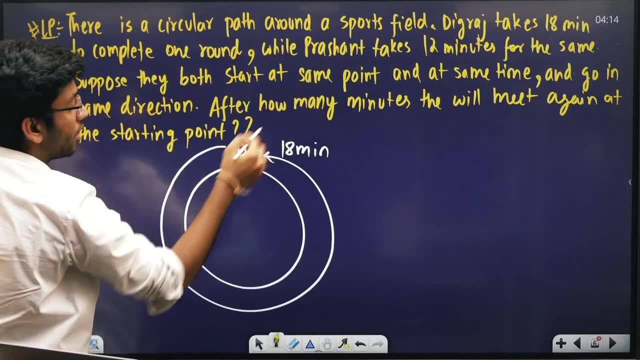 one round. Let's say Digraj ji starts from here, So when Digraj ji reaches here, then how much time is he taking? He is taking 18 minutes And Prashant ji and Prashant ji if Prashant ji. 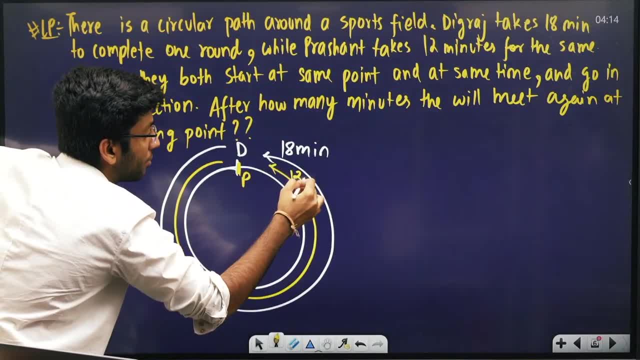 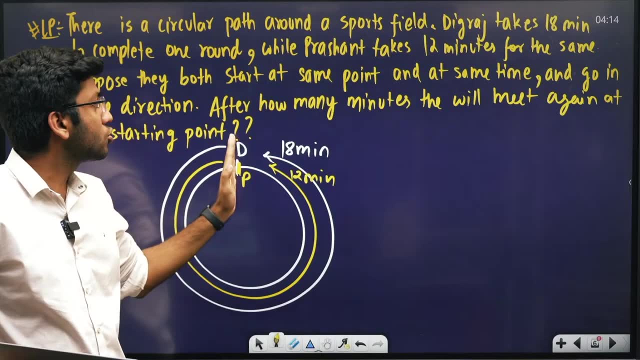 is standing here, then how much time is Prashant ji taking to roam from here? So the question is: suppose they both start at same point. both of them start from here, start at the same time, and what did both of them do? They started to roam. 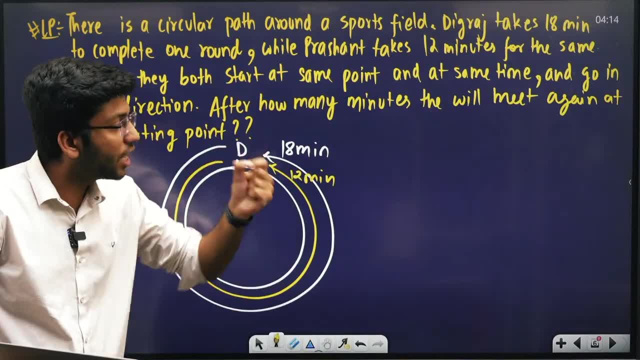 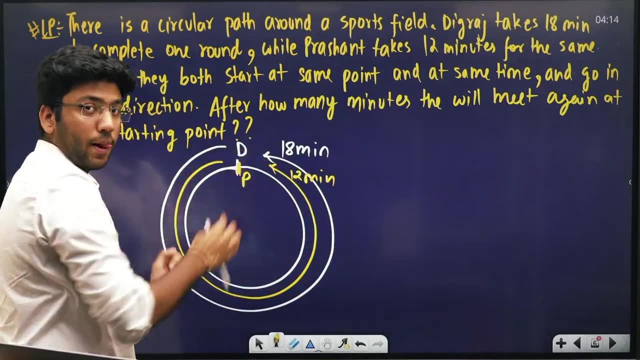 here and go in the same direction. Both of them started to roam here, So we are asked: how much time will they get back from here? Prashant ji is taking 12 minutes and Digraj ji is taking 18 minutes, So he is asking. 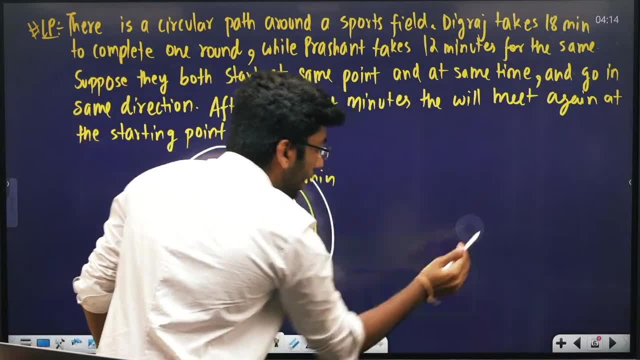 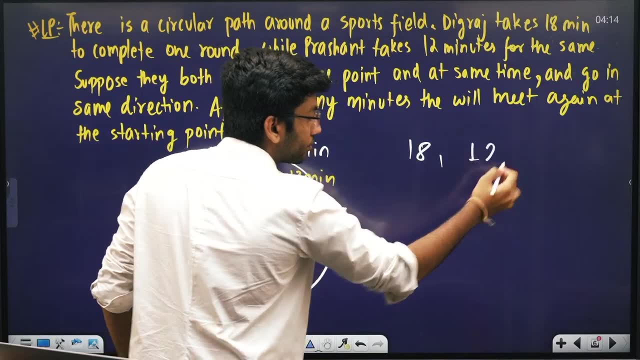 how much time will they get back from here? Think about the answer in your mind. Think about the answer in your mind. These two values: one is 18 and the other is 12.. First of all, think about a very small value from these two. 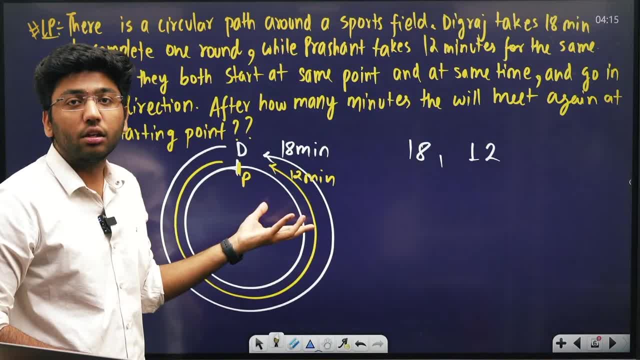 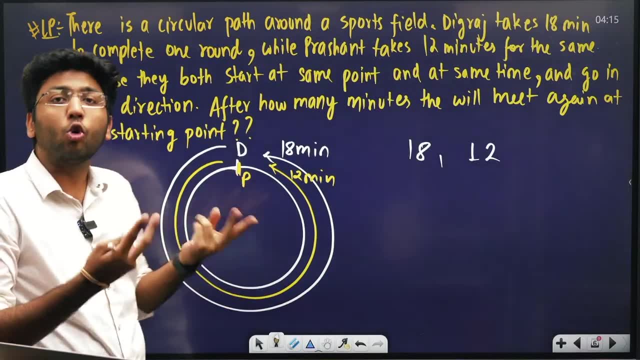 Can two minutes be the answer for both of them to get back from here in two minutes? In two minutes Digraj will go till here and Prashant can also walk a little. They are completing in 12 minutes, so how can two minutes be the answer? 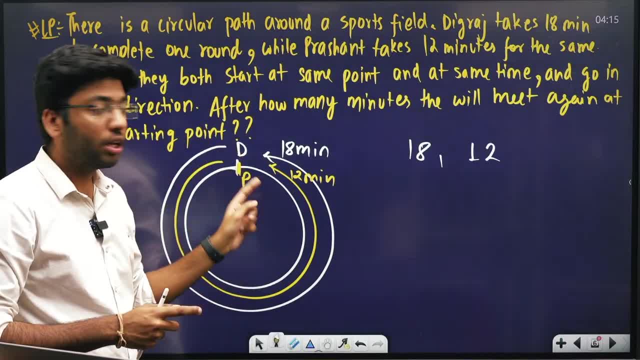 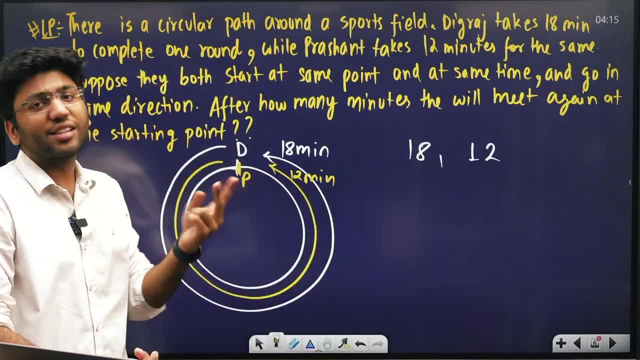 Do you understand? They are completing in 12 minutes and in 18 minutes Digraj sir is completing. So what did I do? first I thought of a small value from both of them in my mind. So two minutes came in my mind. 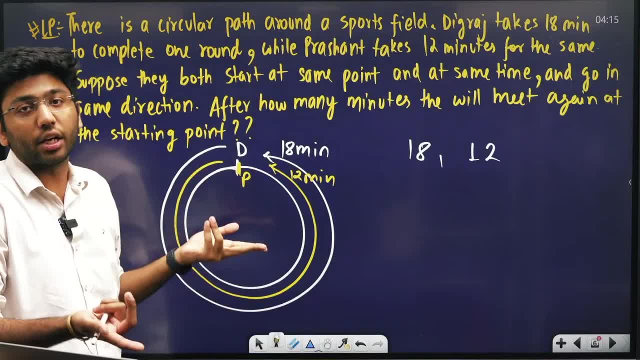 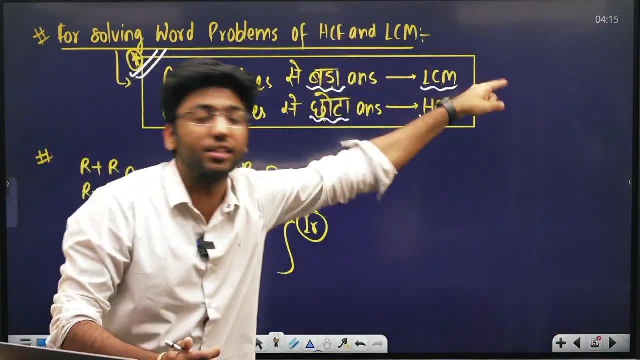 So two minutes can't be the answer. In two minutes we will walk here only. So how will we come back to the starting point? So two answers can't be the answer Means I want a bigger answer than given. 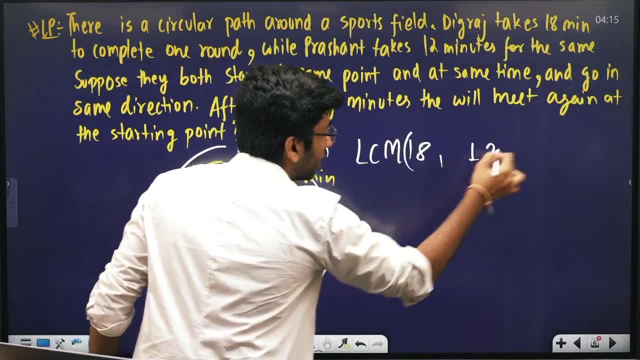 If I want a bigger answer than given, then I will take LCM. So what will I do? I will take LCM. So my answer will be LCM of 18 and 12.. My answer will be LCM of 18 and 12.. 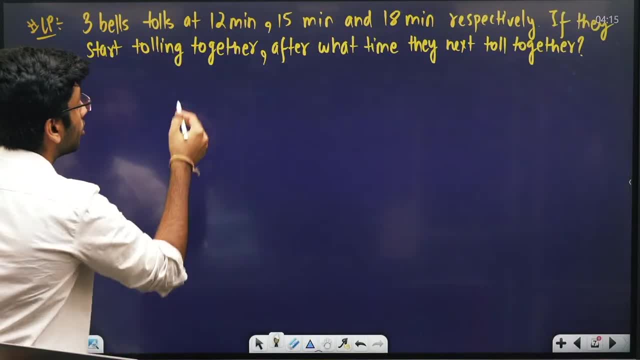 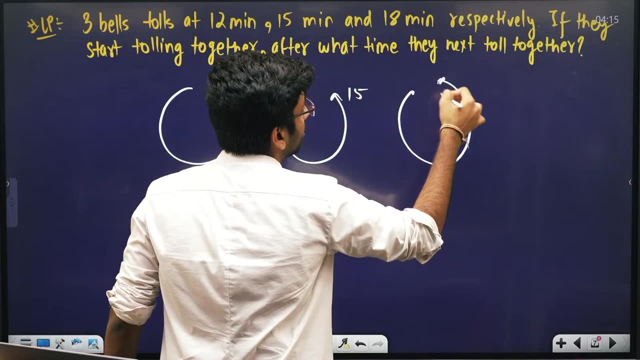 You will get that. This is the answer. I have told you that the first bell rings in 12 minutes, The second bell rings in 15 minutes And the third bell rings in 18 minutes. Okay, This is how I have given you. 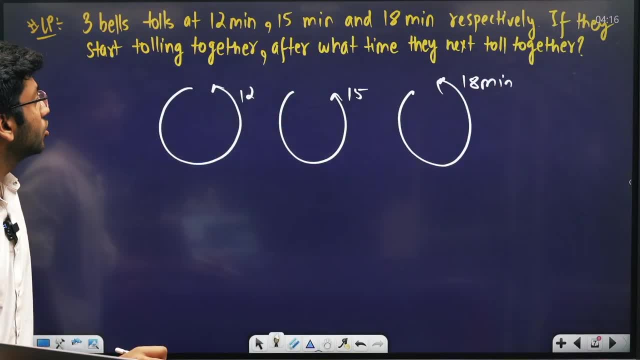 If they start tolling. tolling means to ring. If they are starting at the same time, then after what time they will toll together? So one is 12,, one is 15,, one is 18.. Think of a small value. 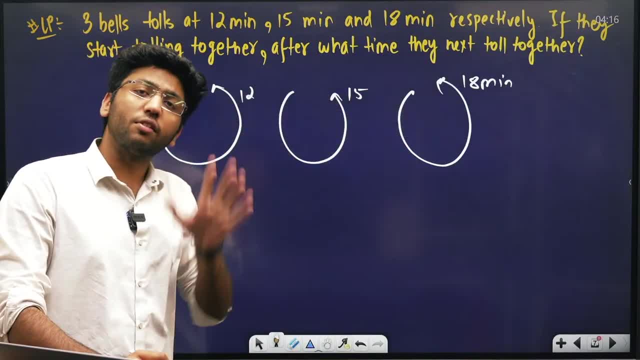 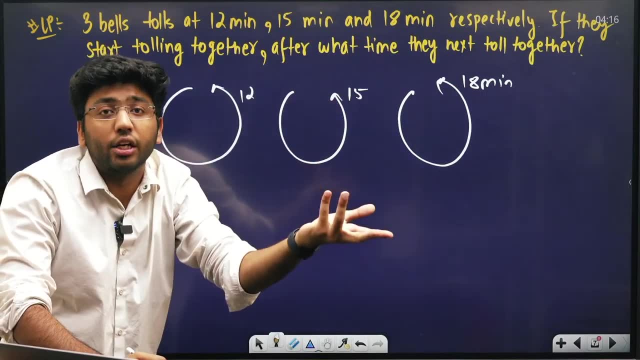 from these three? Can both of them ring together in two minutes? The first bell is ringing in 12 minutes, So in two minutes. what is the answer? So how will it be saved? in two minutes, So two. It won't be a small answer. 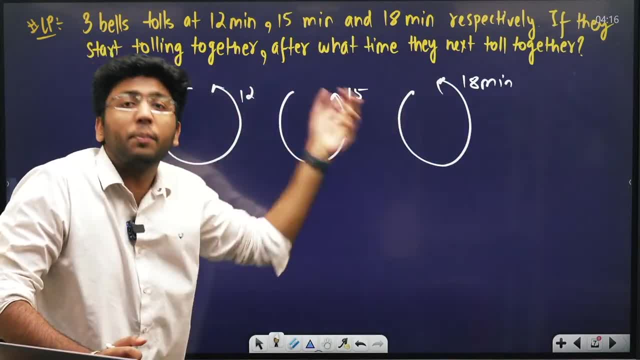 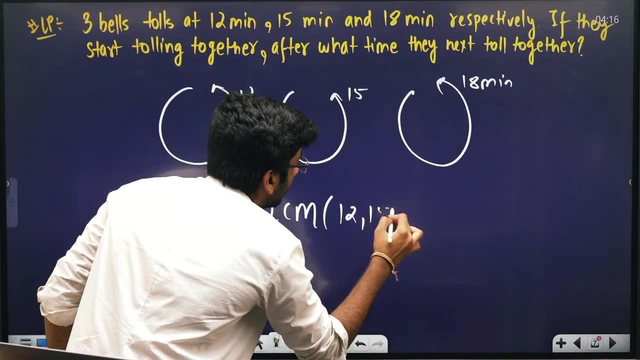 So I want a bigger answer than given. If it is not small, then obviously I want a bigger answer. So I want a bigger answer than given. I want a bigger answer than given. I want a bigger answer than given. So what will I take? 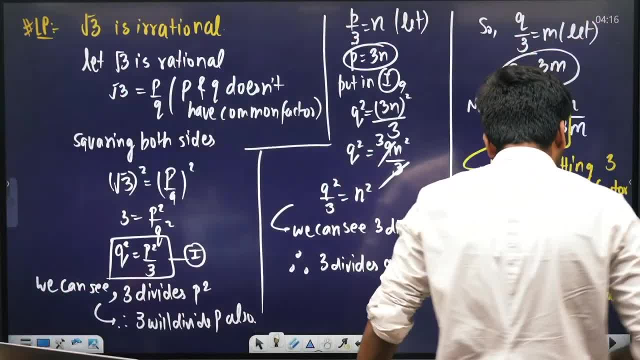 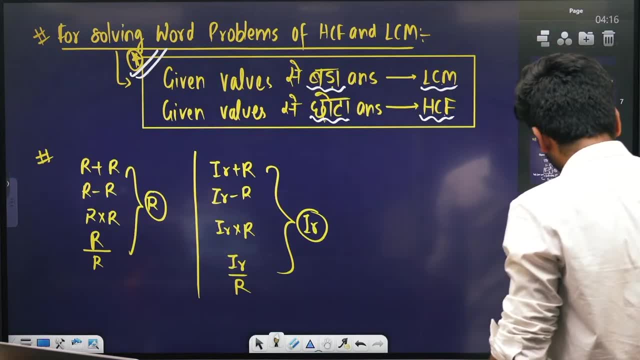 I will take LCM here also LCM of 12,, 15 and 18.. This will be our answer. Okay, Okay, I have understood till here. Now comes our question on irrationality. Question will be asked on irrationality. 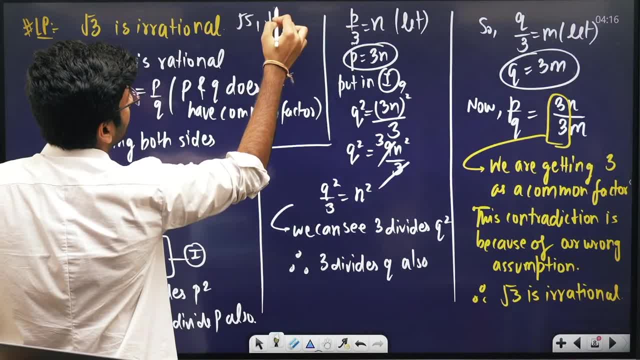 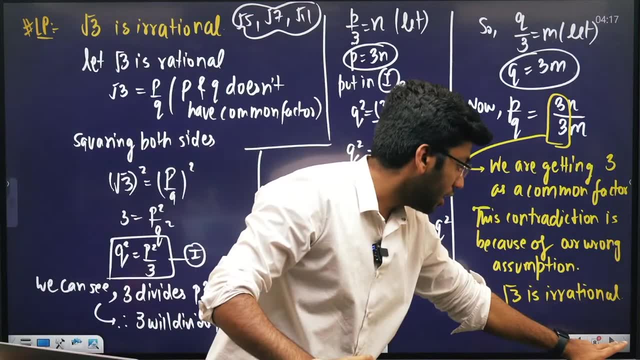 You will be asked root 3, or you will be asked root 5, or you will be asked root 7, or you will be asked root 11.. In this way, any question can be asked. Either you will ask directly, like this: 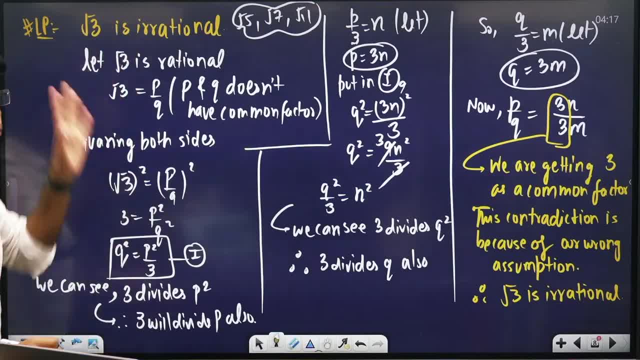 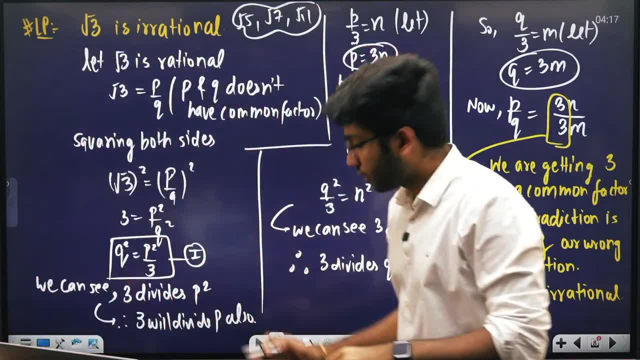 or you will ask like this: in addition, One of the two will be asked for sure. How do we prove? You all know, You all know maximum very well. Many children know very well. See how I will tell you quickly, You will understand. 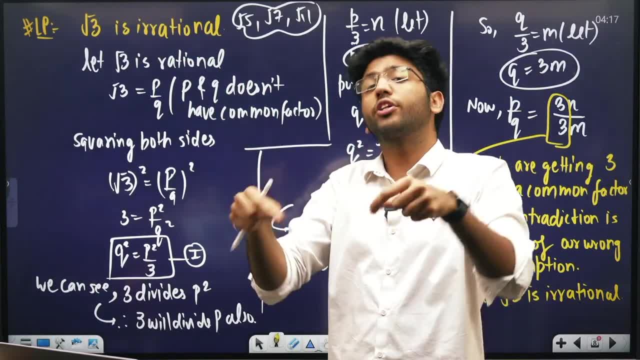 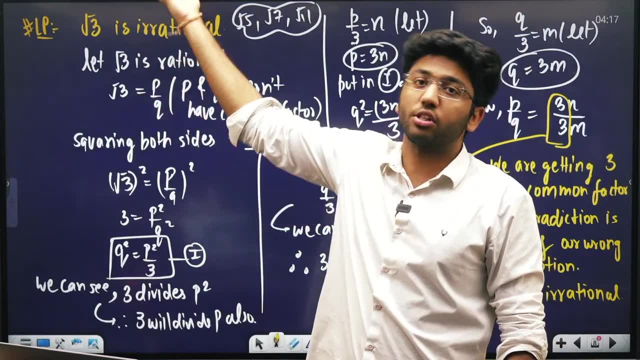 We have to prove root 3 is irrational. This question is always proved by rationality. I will assume that it is rational. What to prove Irrational? I will assume that it is rational. If it is not rational, then it will be irrational. 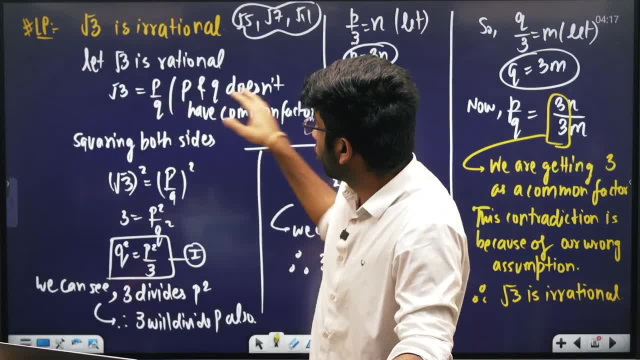 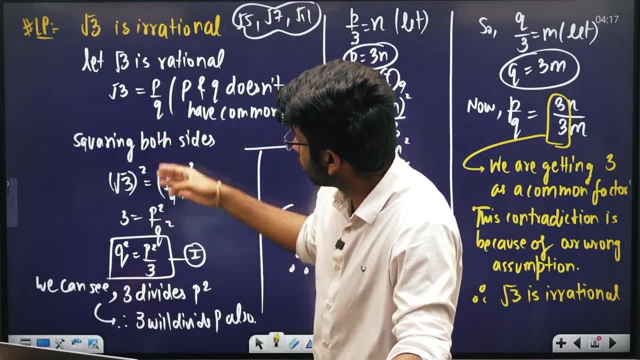 It is obvious. If it is rational, then I can write root 3 in the form of p by q, Where there will be no common factor of p and q Because it is a rational number. So I can write rational number in the form of: 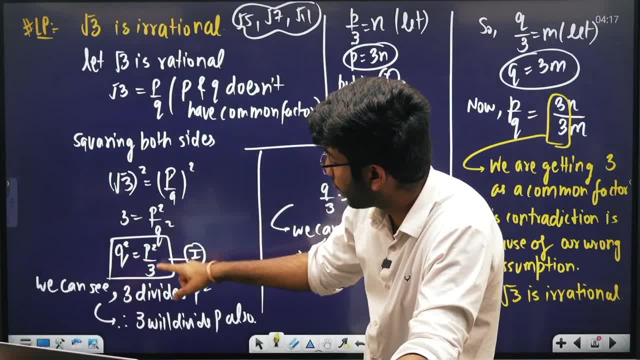 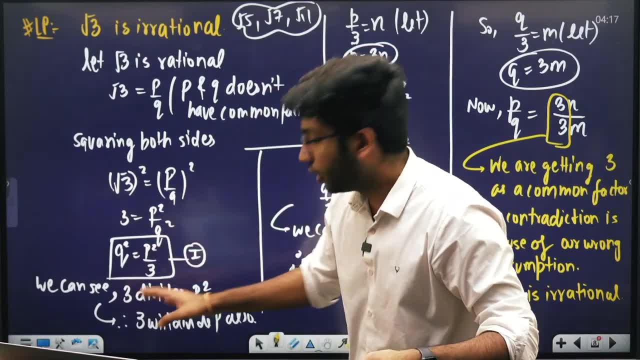 p by q. I did squaring on both sides. After squaring, root went from root p square by q square. This happened From here. 3 goes here and there is a theorem that if 3 is dividing p square then 3 will divide. 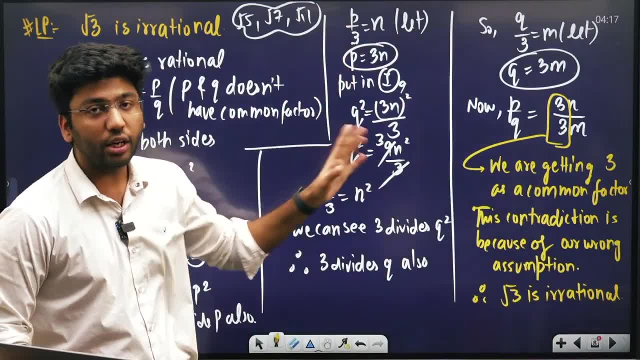 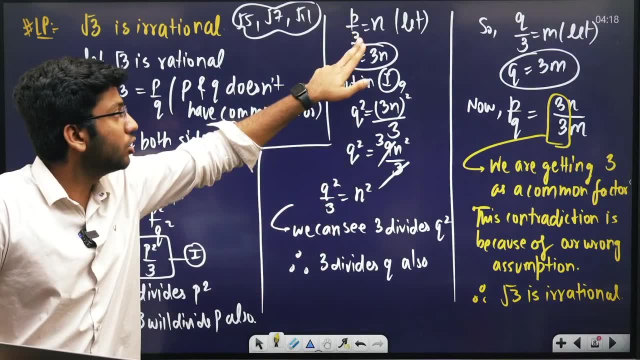 p also, Did you understand? So 3 is dividing p also. p is equal to 3n. If we put p equal to 3n here, then we saw that 3 is dividing q also. 3 is dividing p also. 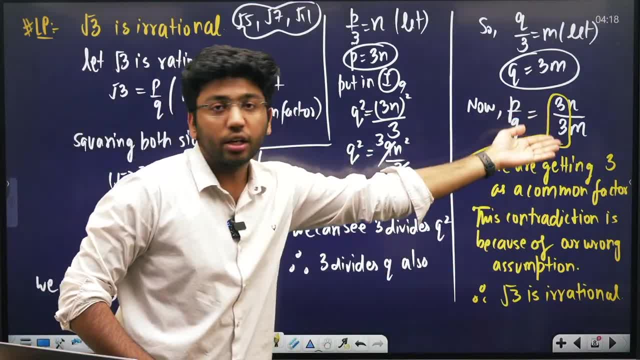 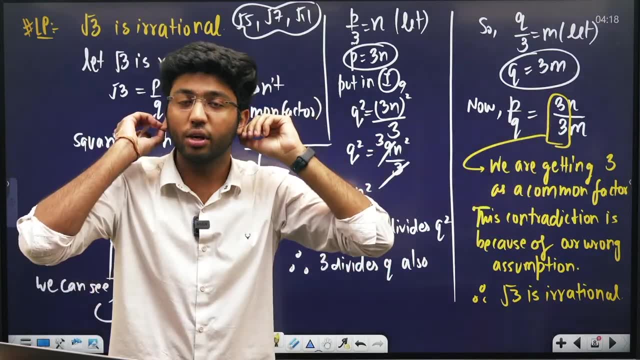 3 is dividing q also, And I had said that there is no common factor of p and q. Here 3 is the common factor. There are contradictions. I said that I made a mistake. Please forgive me. What is wrong? The problem is: 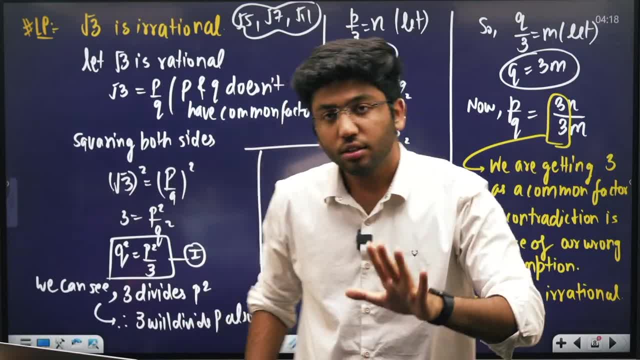 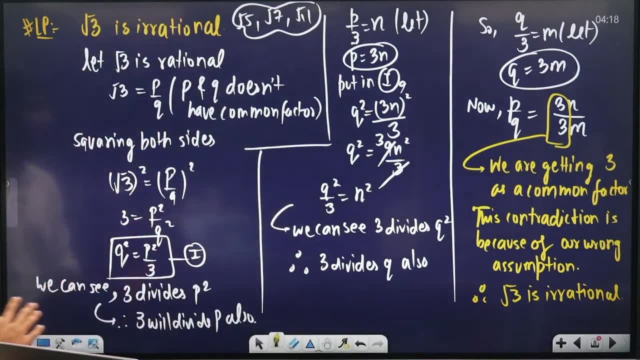 that the root 3 is one irrational number. That is one irrational number, Okay, Okay, We will do it in this way. You take a screen shot of this. You can get a direct question. Who is not understanding? now there is no time. 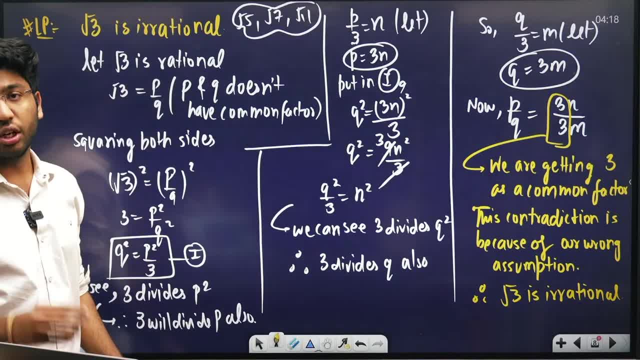 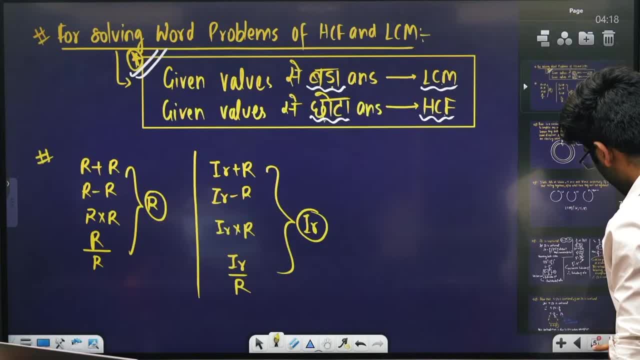 that we can understand this much. So what can you do? You can take a screen shot. Just take a letter. Write steps in this way. Write steps in this way If you want to prove root 3,, root 5,, root 7 irrational. 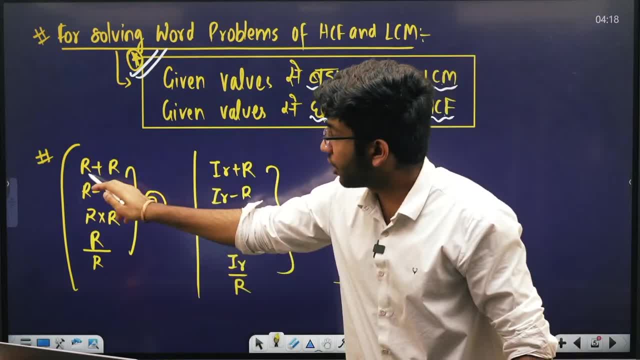 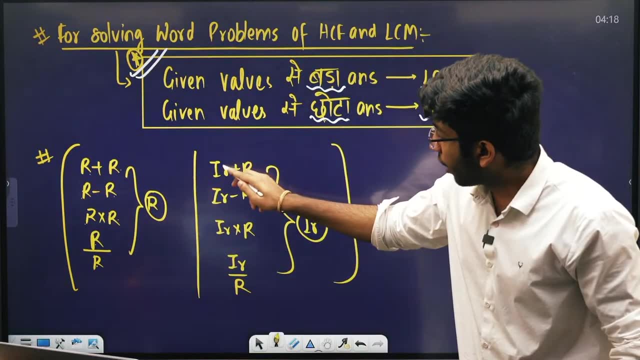 For the second question, you should know that Add rationals in any rational, do a rational minus in any rational, Multiply in any rational, divide in any rational, All will be rational. And add rationals in irrationals, Subtract rationals in irrationals. 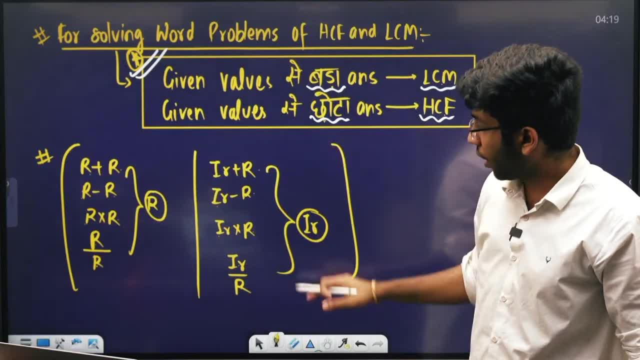 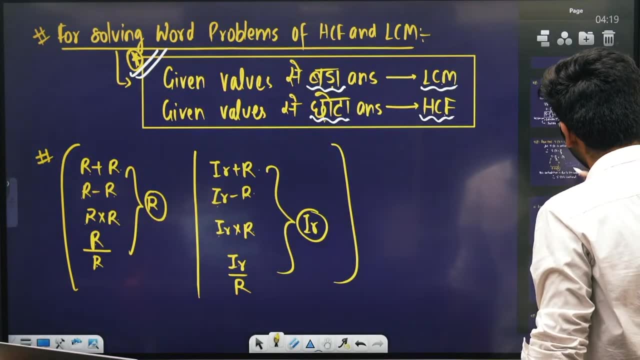 Multiply in irrationals in irrationals, Divide rationals in irrationals, So this will be an irrational. All will be rational. in this case, All will be irrational in this case. You should know this. Okay, For this, only for this, only you can have this question. 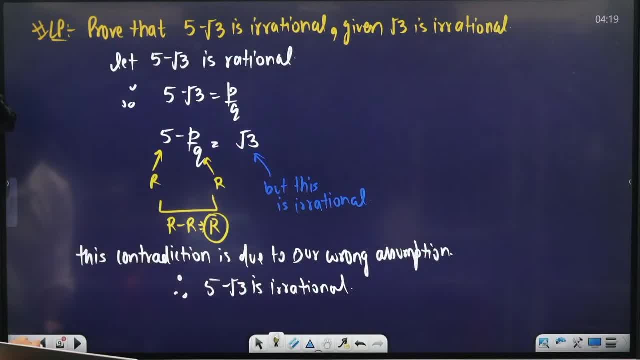 This type of question can come 질문able to you. One of these two questions will definitely be asked. Either tell it blank And there are more chances to ask this kind of questions, So this kind of questions are easier. Suppose you have been told to prove that 5-√3 is irrational. 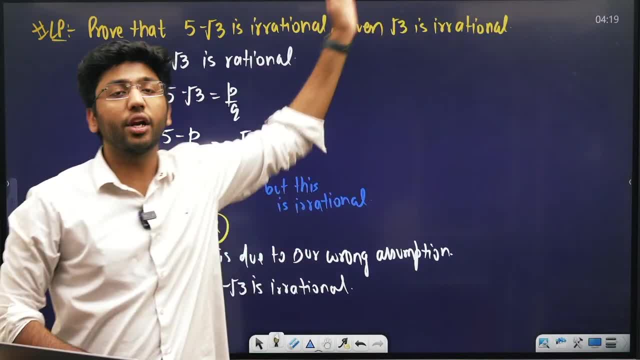 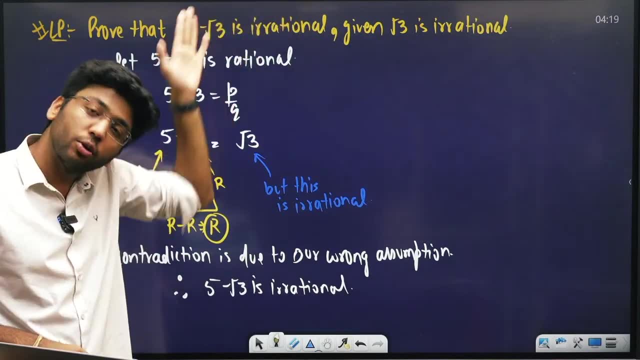 Given that √3 is irrational. √3 is irrational. So he is asking: will 5-√3 also be irrational? So what we have to do is: we will assume that it is rational. We have to prove that it is irrational. so I will assume that it is rational. 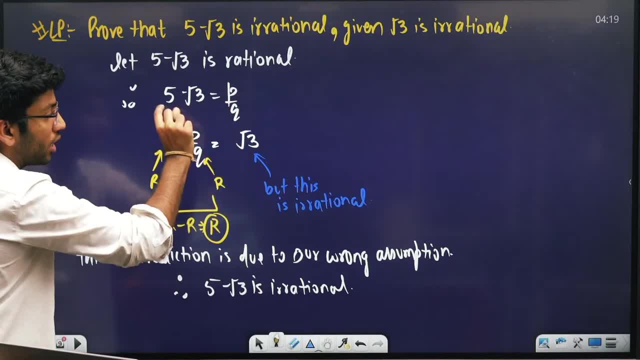 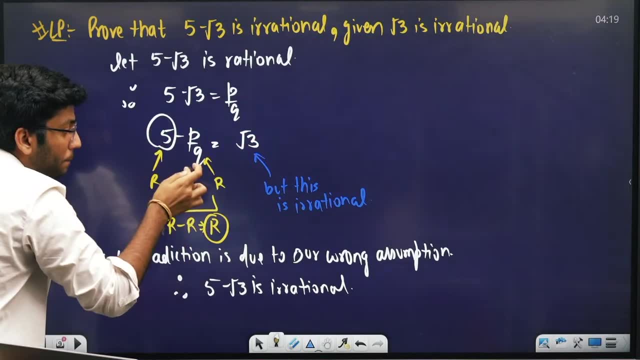 So I will write 5-√3 in the form of p by q. When p by q comes here, then it will be 5-p by q, equal to √3.. p by q here, √3 here. So see here, 5 is a rational. 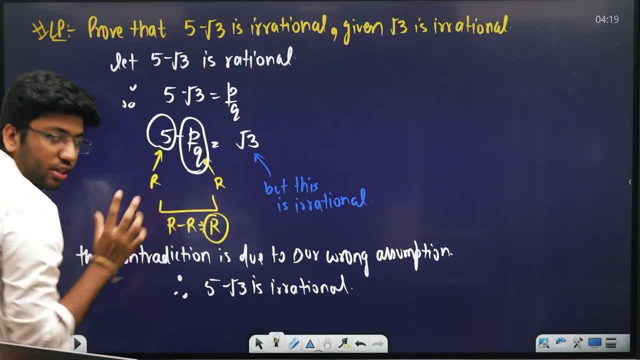 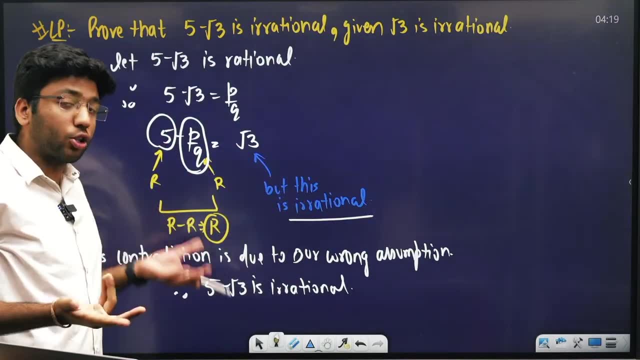 p by q is also a rational, And rational minus rational is a rational, And it is said that √3 is irrational. Given that √3 is irrational, So how can a rational be equal to an irrational? This is a contradiction. 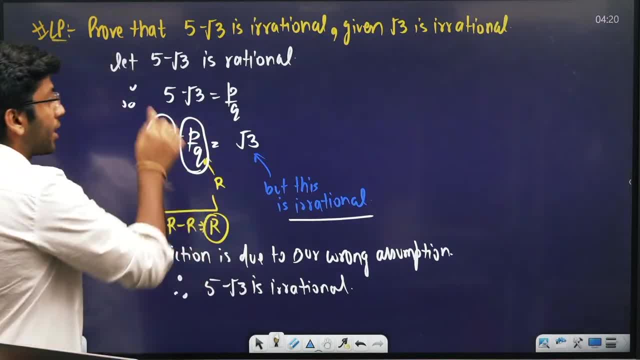 It means that we made a mistake, So we made a mistake, so we apologized. What did we believe? That this is a rational, So it is not a rational. Therefore, this is an irrational number. Okay, we will do it this way. 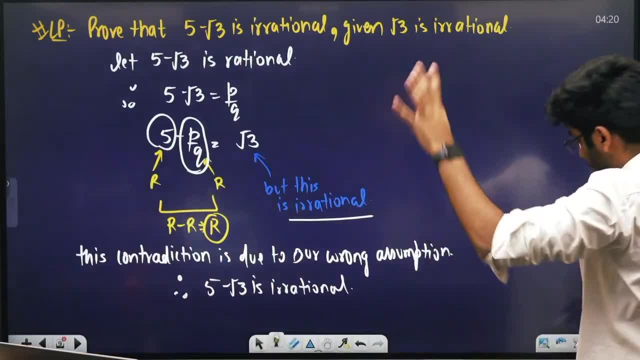 We will finish it this way. Understood, We will finish it this way If you have not been given this, If you have not been given this in the question, Then prove it on the side. How will you prove it? I have told you this. 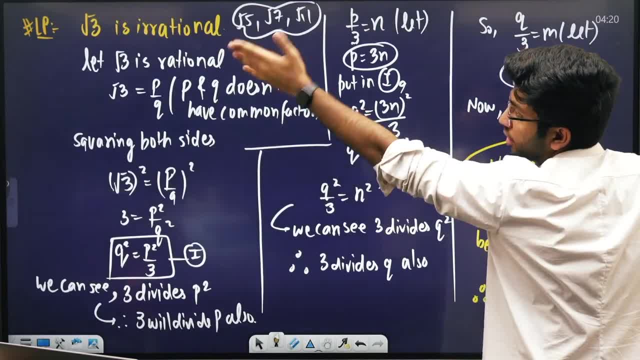 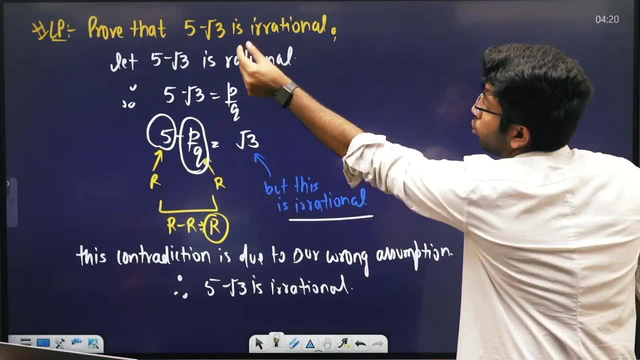 I have told you this here: If you have not been given √3 in the irrational question, Suppose the question of number 5 has come, That prove it as irrational and did not give this. So what will you do first? First, you will prove √3 as irrational. 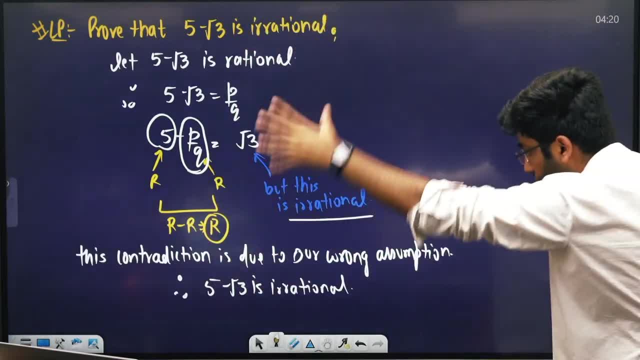 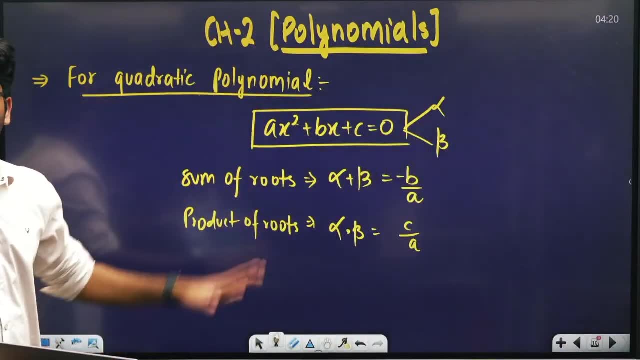 Then after that, you will do this step And to prove √3 as irrational, I have told you this one. Okay. next, If we come to the next chapter, Then the next chapter is your polynomials. Okay, one more question on polynomials, which is very famous, is this: 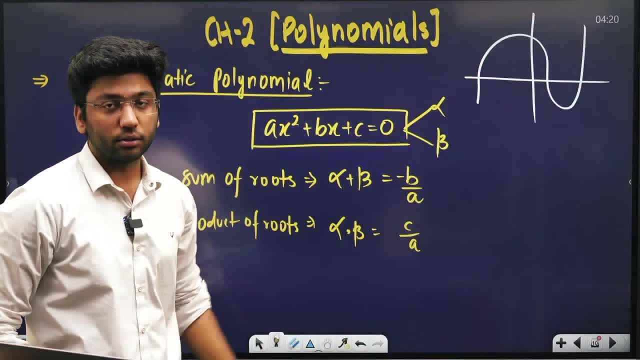 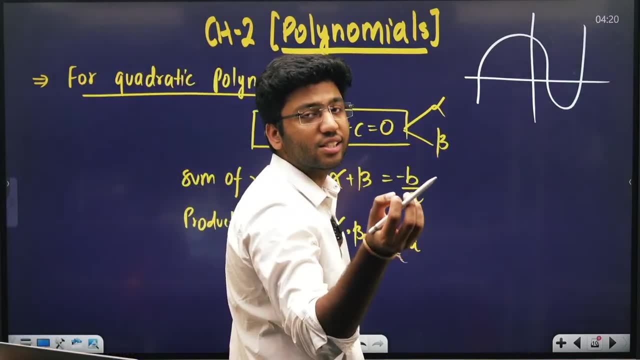 That we will give a graph like this And it will ask you how many roots are there. Leave this now First look at this. It will ask you how many roots are there. So how will you find out Wherever the x-axis is touched or intersected? 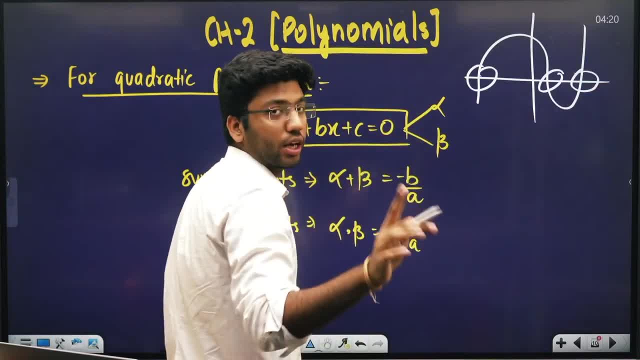 That many roots are there: 1,, 2, 3.. If you want to see only x-axis, Then it has 3 roots. If it is touching, then also we will assume. Assume that it is touching like this. Assume that the graph is touching like this. 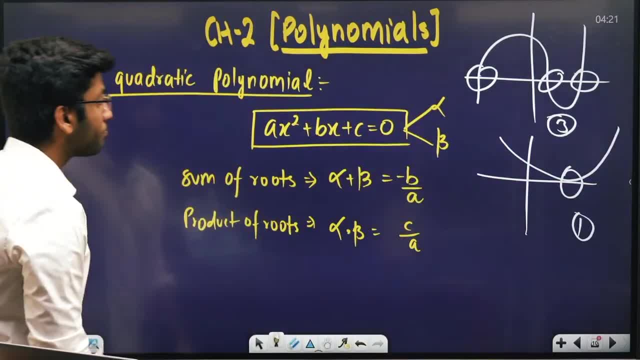 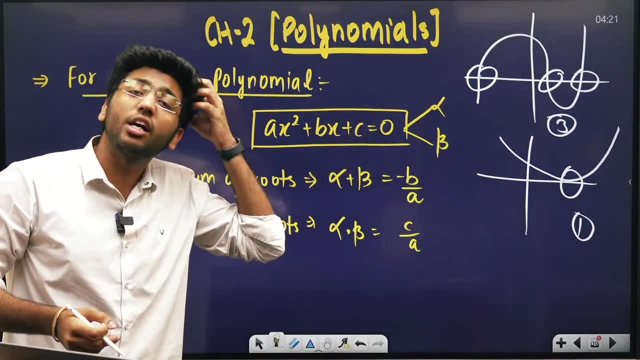 Then it will have one root. Just look at x-axis. Okay, Now let's talk about quadratic polynomial. What is quadratic polynomial Which has degree 2.. What is quadratic Which has degree 2.. Degree means highest power of x. 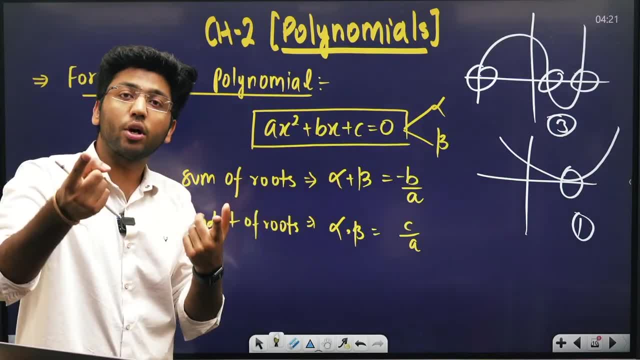 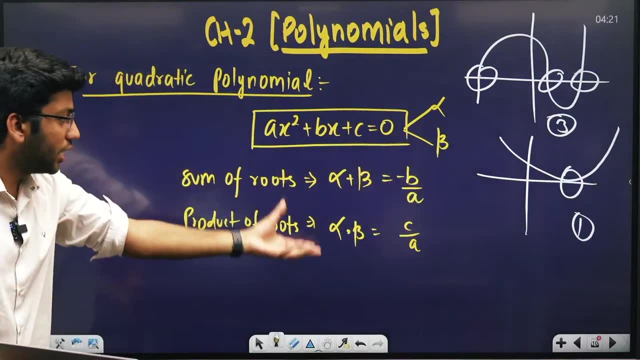 Here the highest power of x is 2.. So it is quadratic. So degree 2 means quadratic, Degree 1 means linear And degree 3 means cubic. So we know this. So it is said that quadratic is polynomial. So for this, these two relations. 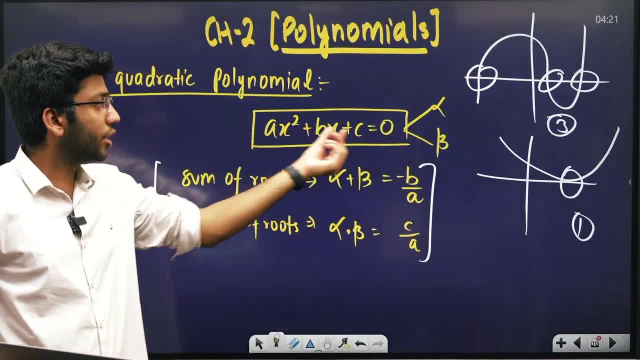 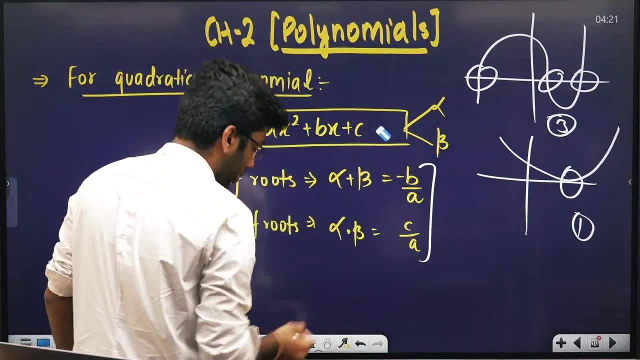 What Sum of roots That if this is polynomial, A quadratic equation or a quadratic polynomial, Its roots are alpha and beta. Its roots are alpha and beta. Okay, It can be equal to zero. It can not be equal to zero. 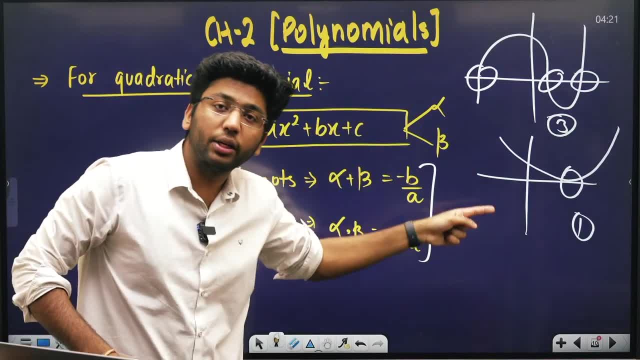 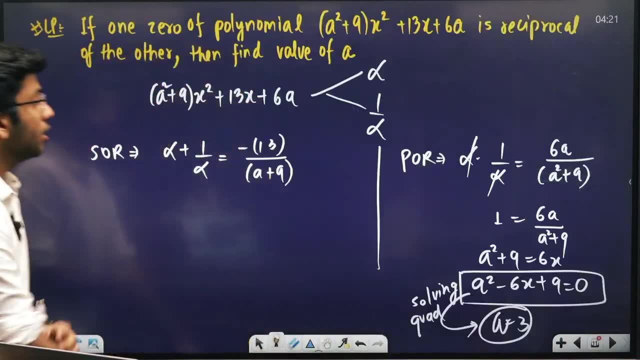 There is no problem. So the roots of a quadratic polynomial are alpha and beta. So if you do sum of roots, Then minus b by a. If you do product of roots, Then c by a. We know this, Okay, Okay. 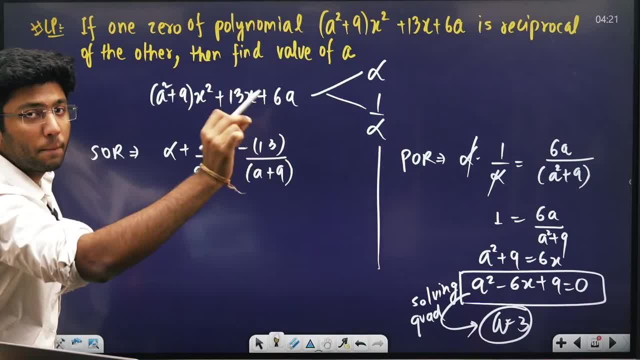 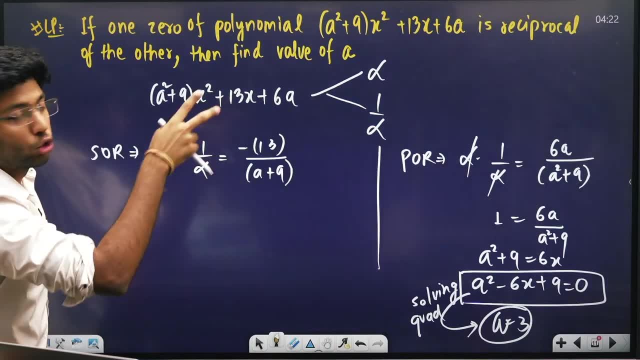 This kind of question can be asked from you for sure, In quadratic polynomial, In quadratic, In the chapter of polynomials. What will it do to you? It will give a relation about both roots. It will say: If one zero of this equation, 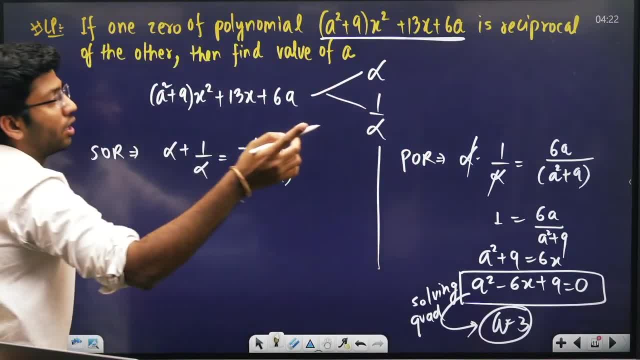 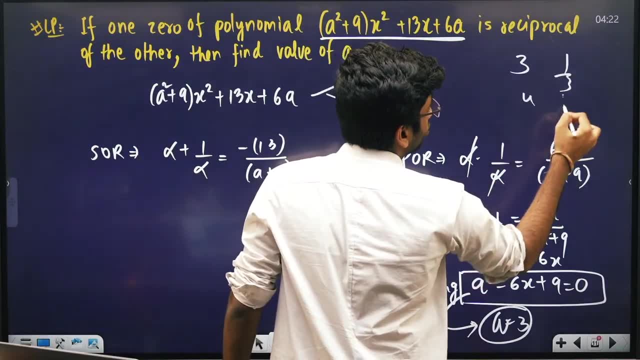 This polynomial given to you, One zero of this polynomial And the other zero. They are reciprocal to each other, Like If one is three, Then the other is one by three, So if it is four, Then the other is one by four. 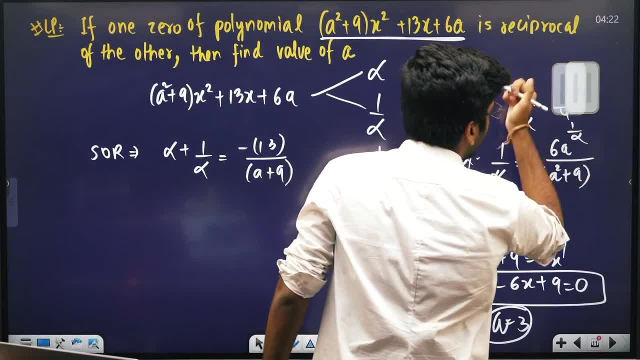 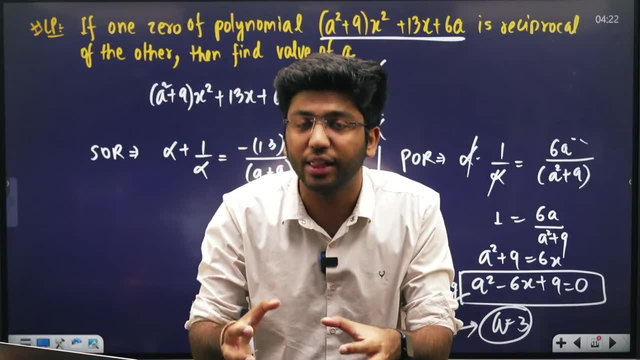 So if it is alpha, Then the other is one upon alpha. So we have accepted. We have accepted that two roots are alpha and one upon alpha, Whenever you, Whenever you are given an equation or polynomial, Whenever you are given a polynomial. 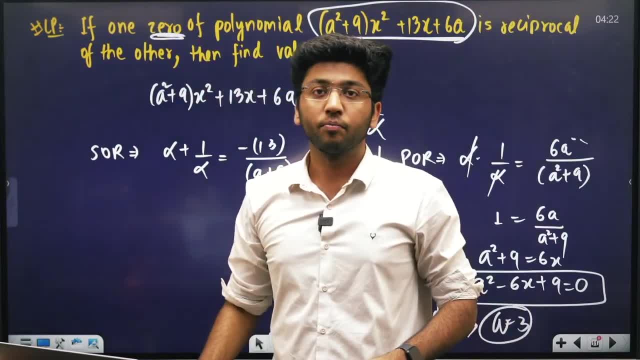 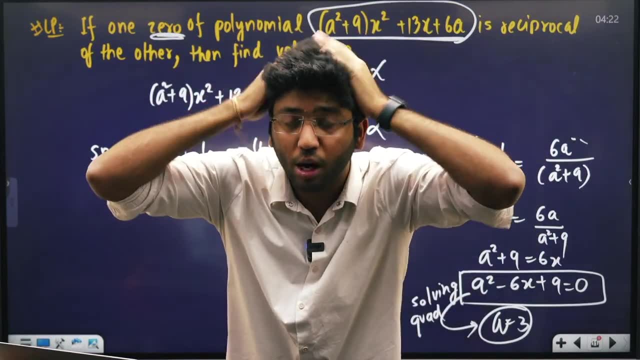 Whenever you are given a polynomial And talk about zeros and roots, Then you will understand. You will understand The question of sum of roots and product of roots. Write it on the roof And put it in your mind. Put it in your mind. 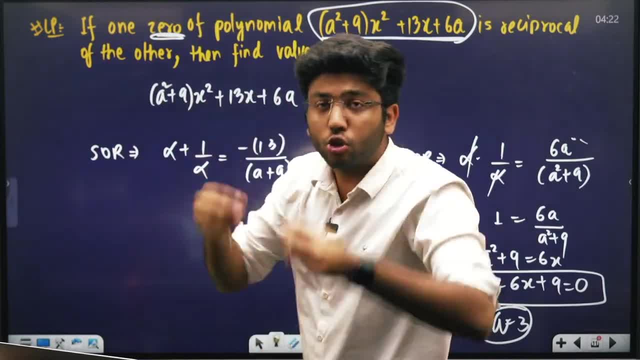 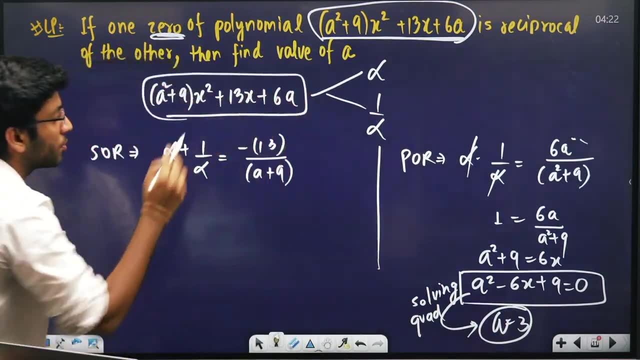 What? Then? you will also talk about polynomial and zeros. Then I will write the sum of roots and the product of roots. That's what I did here. That's what I did here, That you had talked about this. So what I did in this. 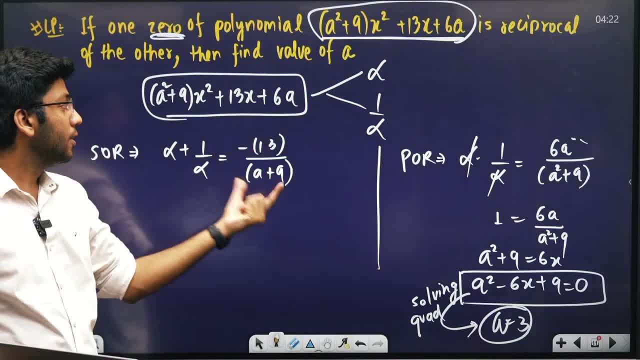 First I wrote the sum of roots. Sum of roots minus B by A. Write it Minus B upon A. Write it: Minus B means the coefficient of X, A means written this. So this will be the sum of roots. 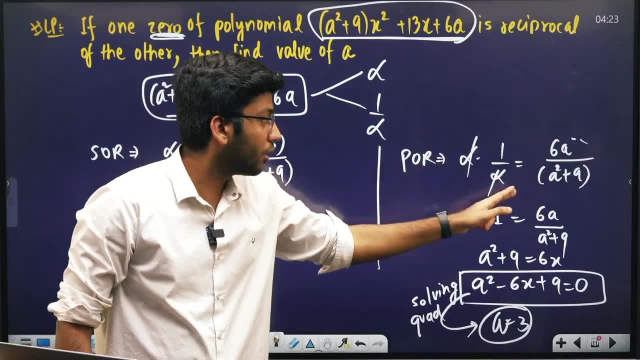 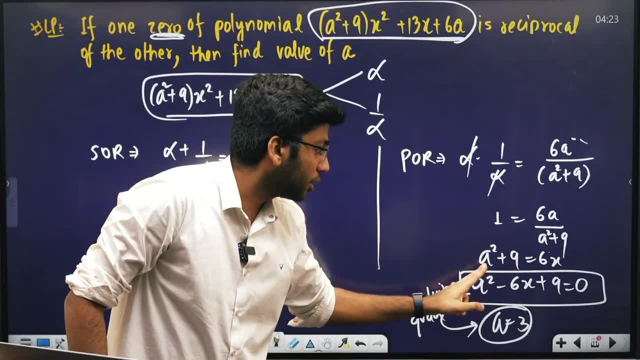 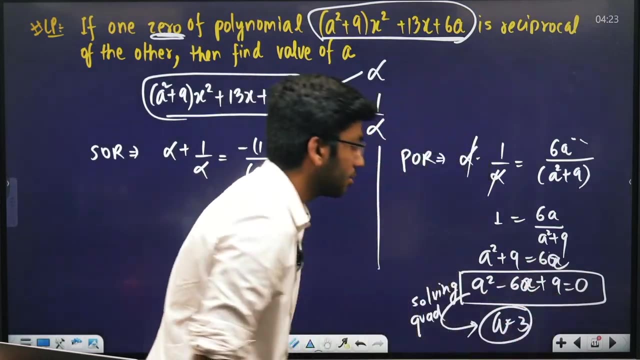 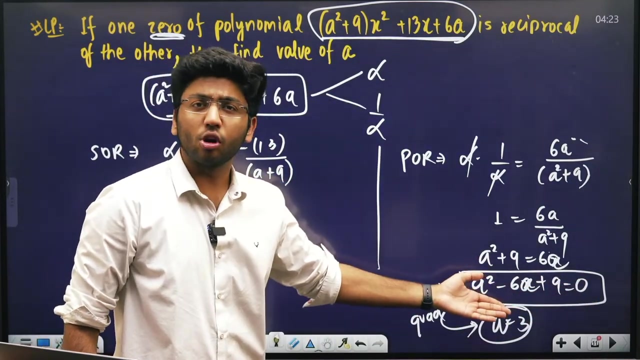 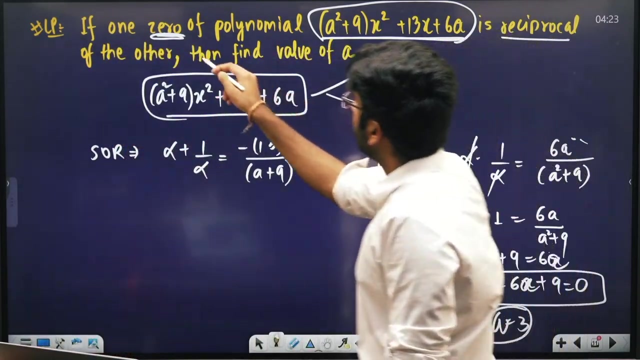 When I did their product of roots, Alpha, into one upon alpha. Then it is C upon A. This cut alpha by alpha, So one equal to six. A upon this, This will be cross multiplied, so a square plus 9 equal to 6x, a square minus 6x plus 6x, not 6a, 6a. so from here I saw a square minus 6a plus 9 equal to 0, some kind of quadratic polynomial has been made. we know to solve this how we will do: splitting the middle term. the value of a will be 3, this is the answer. so this kind of relation between roots, that one root is the reciprocal of the other or one root is the square of the other, we get to see such questions a lot, okay. 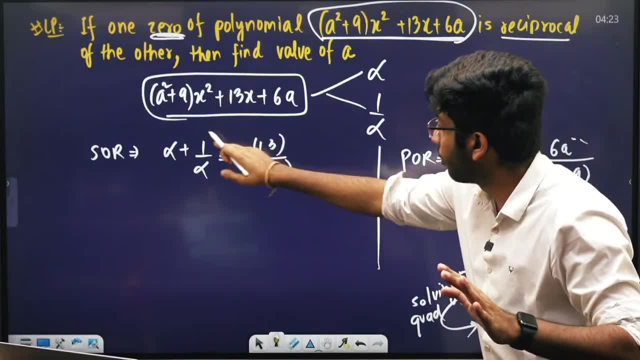 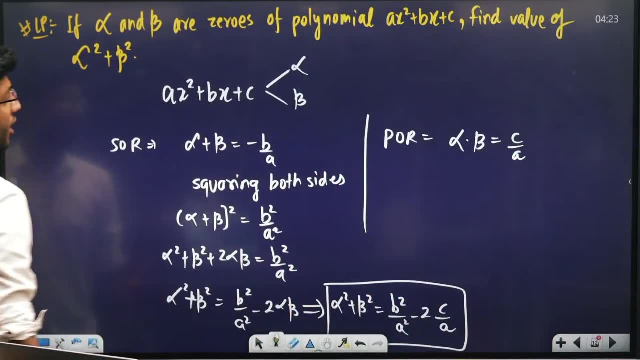 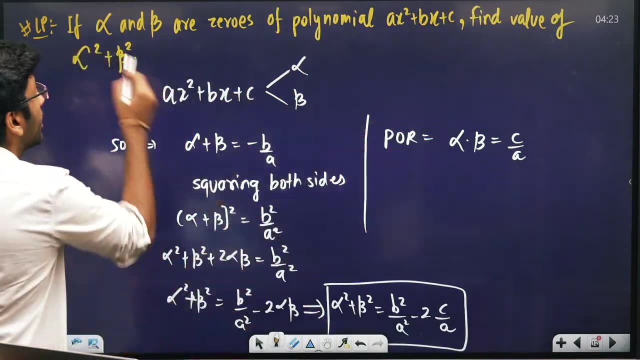 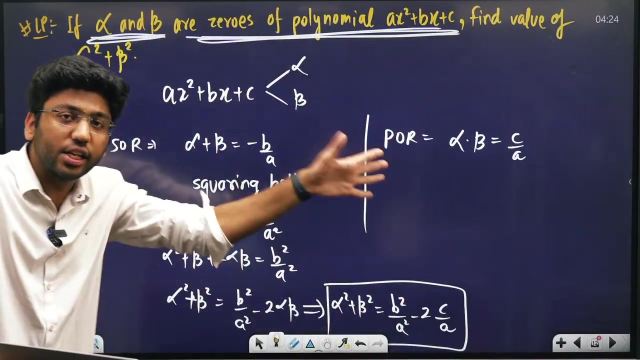 we understood this. nothing is being done. sum of roots, product of roots. sum of roots, product of roots. the answer will definitely come. it will come immediately. if alpha and beta- yes, see, alpha and beta are roots of this. so what did I say? whenever we will read in the question that alpha and beta are zeros of polynomial, whenever we will read in the question that alpha and beta are zeros of polynomial, what will I write immediately? sum of roots and product of roots. 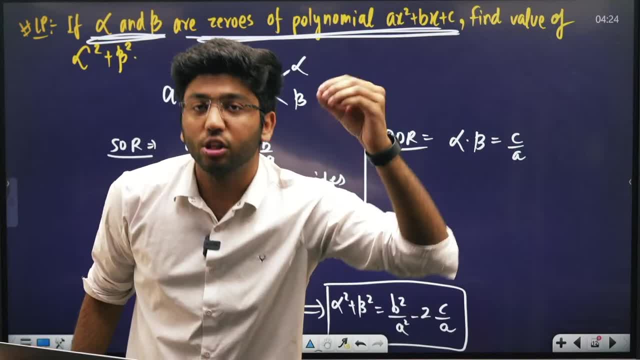 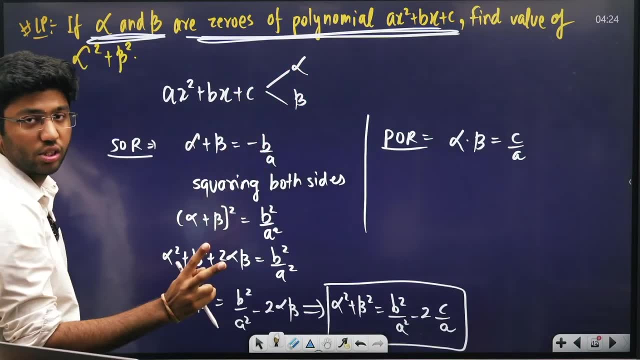 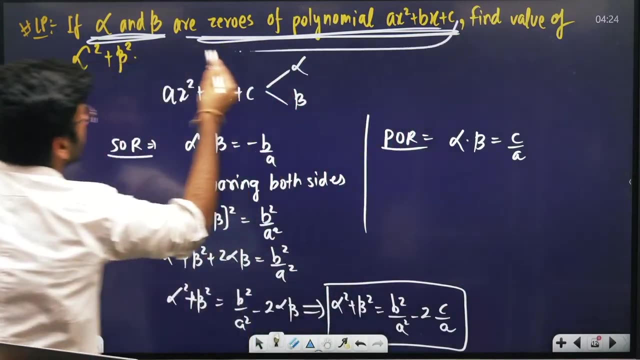 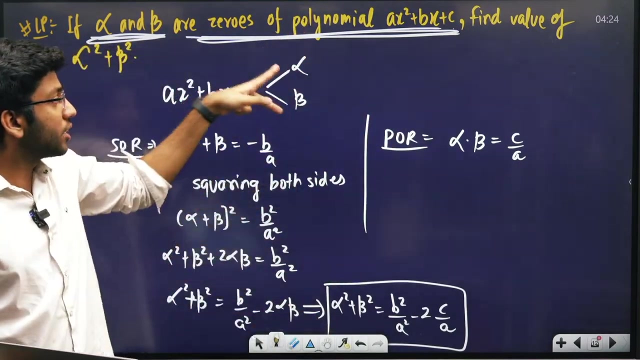 put this in your mind. quadratic question is coming and we are talking about zeros. so I will immediately write sum of roots and product of roots. so what did I do? it was a quadratic question, I have talked about alpha and beta zeros, so I wrote sum of roots and product of roots. now I will read the next question. I just read this line, this comma line. I wrote sum of roots and product of roots. so I was given alpha and beta roots. so sum of roots minus b by a, product of roots, c by a. 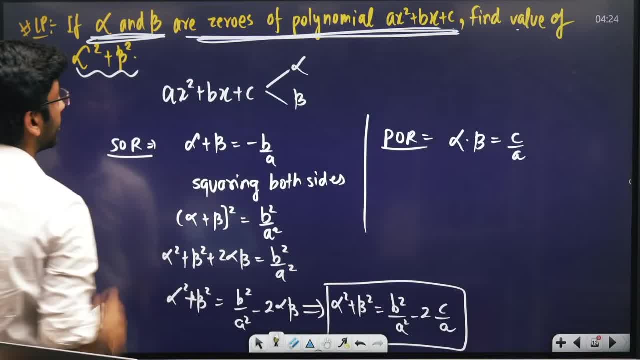 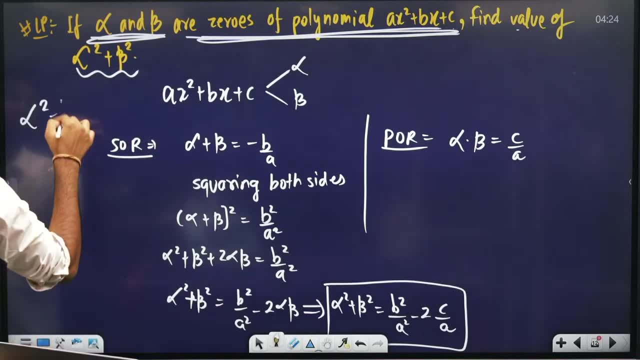 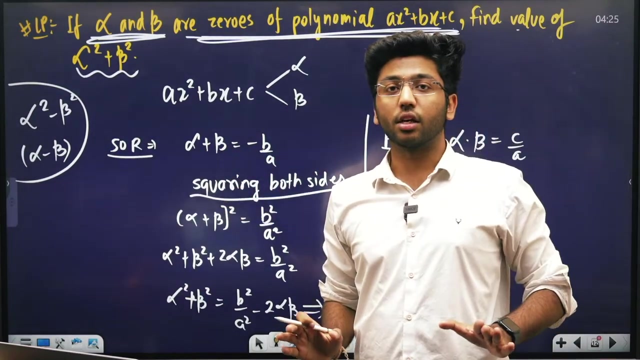 now what has been asked me? find the value of alpha square plus beta square. so see, whenever the integral will ask alpha square plus beta square, or alpha square minus beta square, or alpha plus beta or alpha minus beta, whenever the integral will ask, then do squaring both sides. so what did I do? alpha plus beta equals minus b by a. 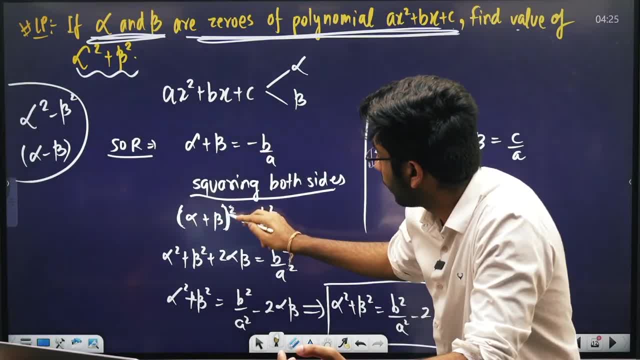 this, I knew, so I did. squaring on both sides. The whole square of a plus beta is equal to the whole square of b by a, which is b square by a square. Open this: How will you open the whole square of a plus b? 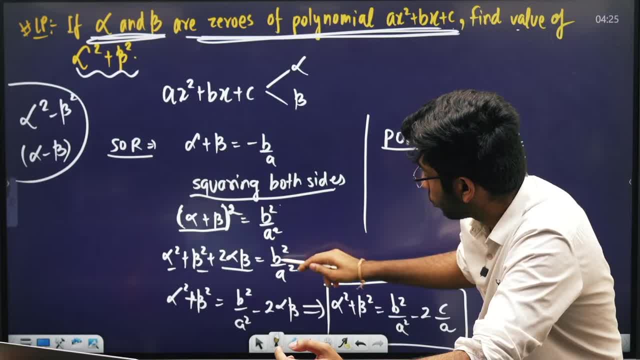 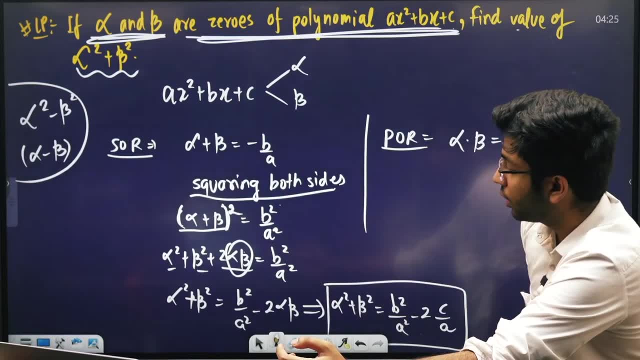 a square plus b square plus 2ab. Will you write b square by a square. equally Okay, The value of alpha beta. I know this Product of root c by a, So I put c by a here. So alpha square plus beta square. 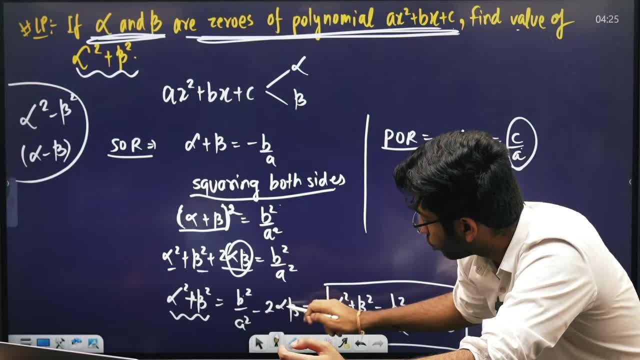 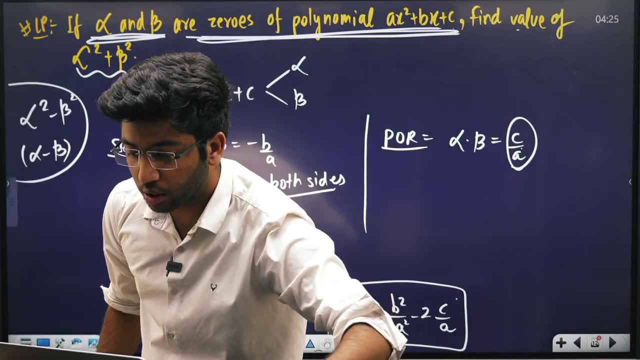 If this goes here, equal to b square by a square minus 2 alpha beta. and if I put alpha beta then it becomes 2 into c by a Easy peasy, Easy peasy, Okay. So we will do this by doing sum of roots and product of roots. 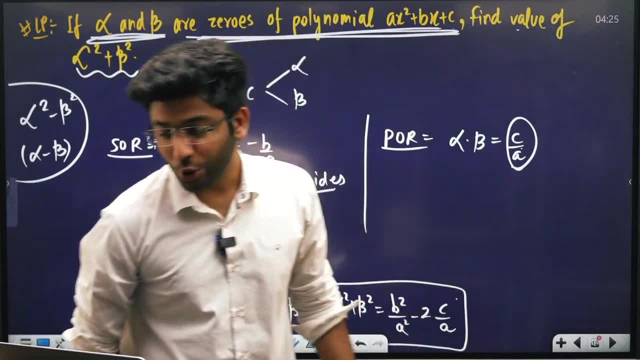 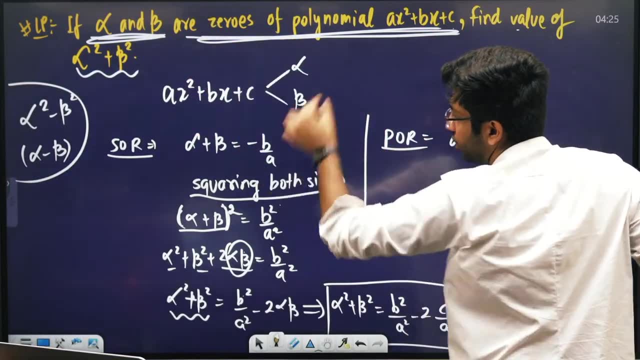 Okay, I didn't sleep, brother. Very good, very good, Brother, let's go a little faster. How can I go faster than this? So look, I gave you the polynomial, I gave you the roots. So, sum of root c by a product, of root c by a. 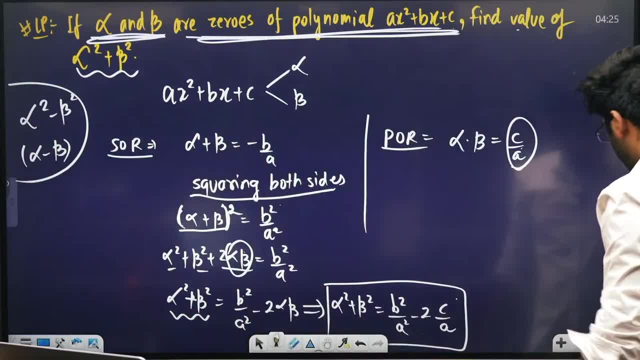 do squaring both sides Whenever you are asked so hard, do squaring both sides like this. I have done one or two questions like this in the marathon when I took out alpha minus beta. For that too, I did squaring both sides. 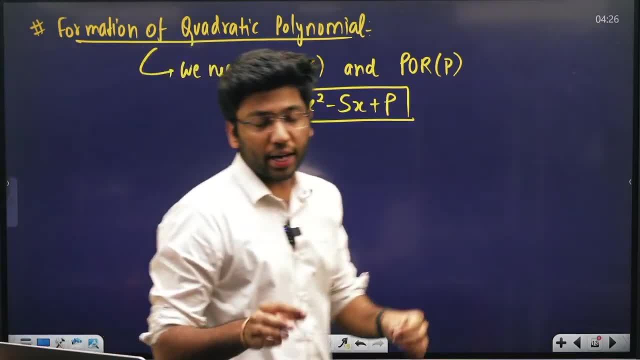 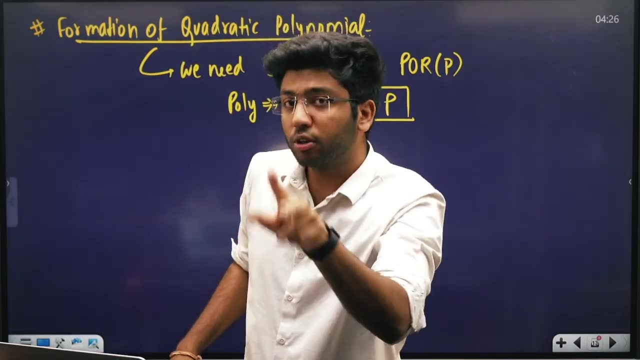 So go and see it once. I am saying this again in maths It won't be necessary that you will see the same ditto question. They will change the values a little. They will change the values a little, But the questions will look like this: 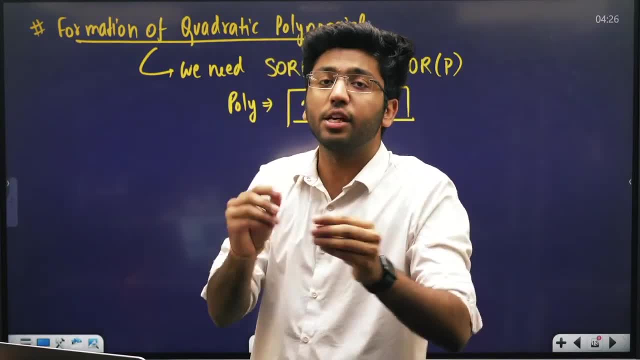 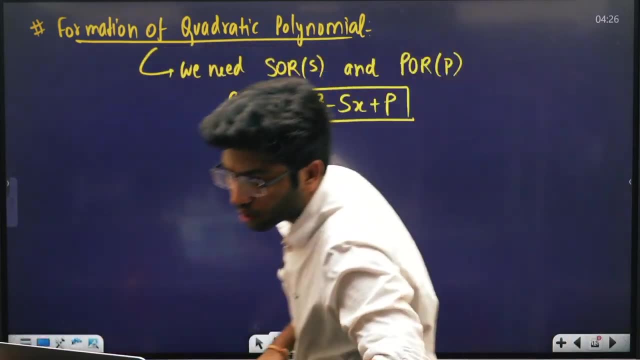 Questions will look like this: Values can be done here and there Rest all the concepts will come up like this: Do you understand what I am saying? Okay, Okay, What happened, Brother? let's go to 15x. Now comes the formation of quadratic polynomial. 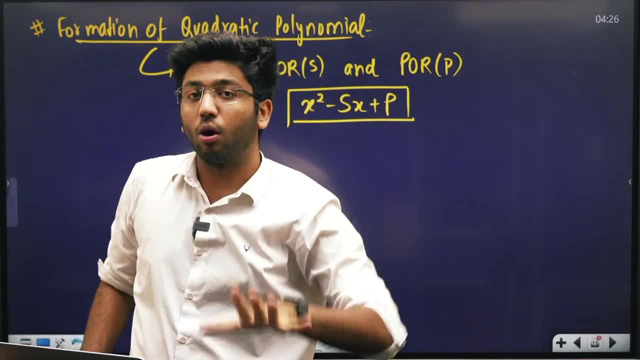 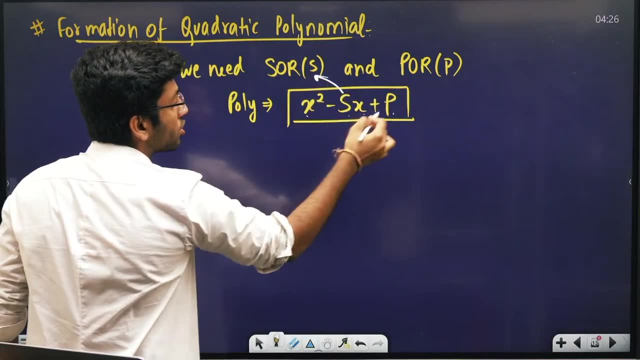 If I tell you that, make a quadratic polynomial and show it, I am telling you to make it and show it. So for that, do x square minus sx plus p, Where s means sum of roots and p means product of roots. So if I tell you that, 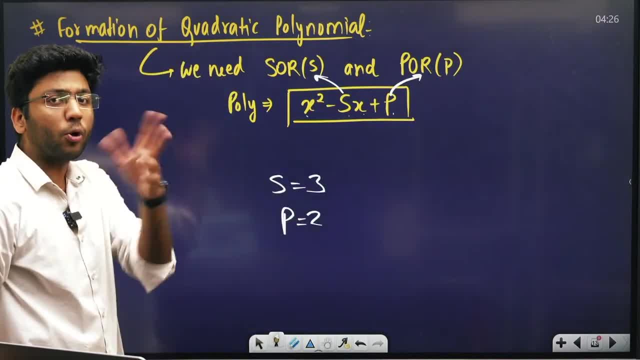 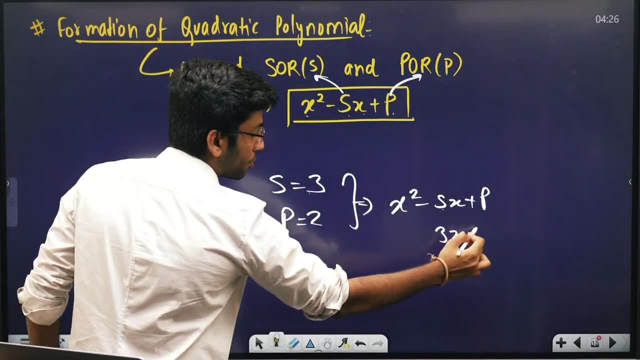 sum of roots is 3 and product of roots is 2.. So tell me what will be the polynomial. So you have to write immediately: x square minus sx plus p, where s means 3.. So 3x plus p means 2.. 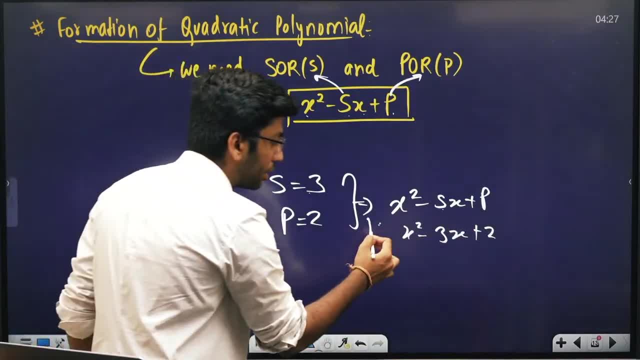 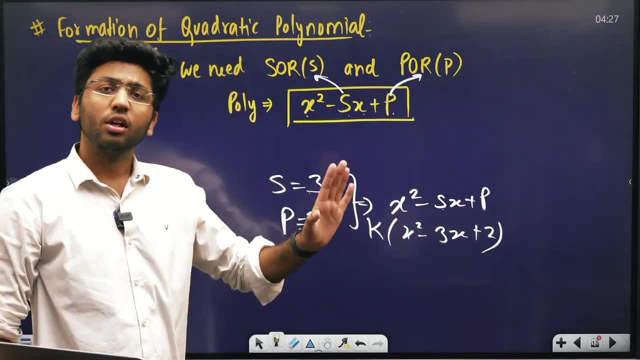 And here x square. Okay, Worldly people also multiply k. here We multiply k because you can keep any number of k: 1,, 2,, 3,, 4.. So if it is written like this, no problem, no problem, no number is cut. 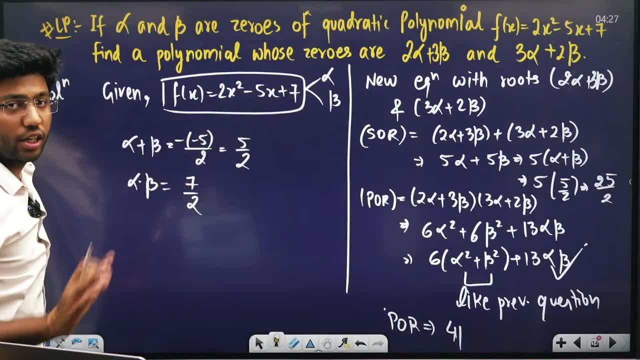 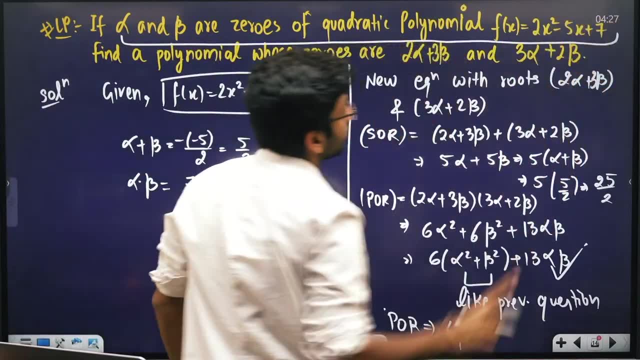 So this is the sum of roots and product of roots. if you want to find out the equation- So the question can be asked directly from you- What It is given to you that alpha and beta are the roots of this quadratic polynomial. Look carefully. 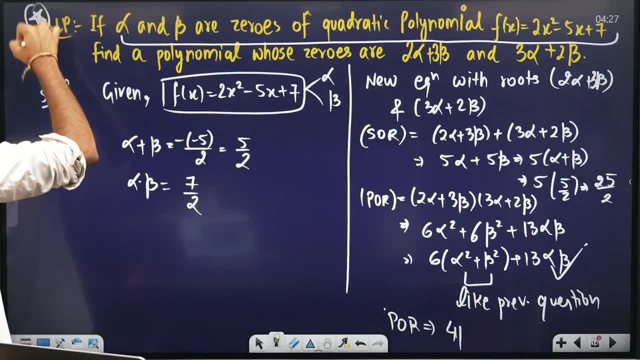 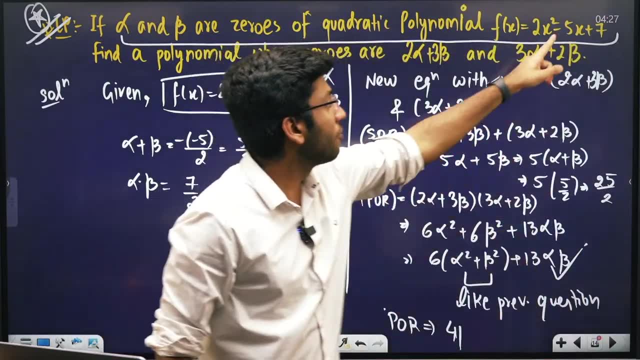 This question is important. The question can come from the formation of quadratic equation: Formation. The question can come from the formation of quadratic equation. It will change the value a little. It will put 7 instead of 5.. It will put 8 instead of 5.. 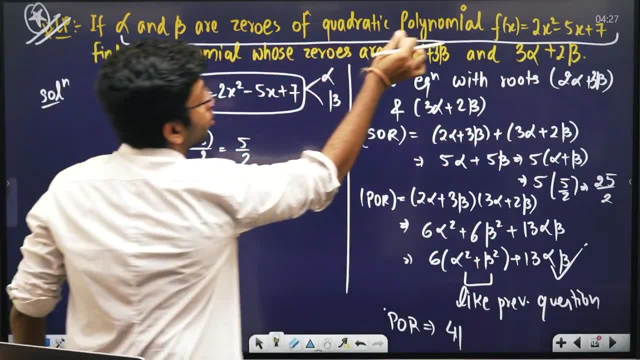 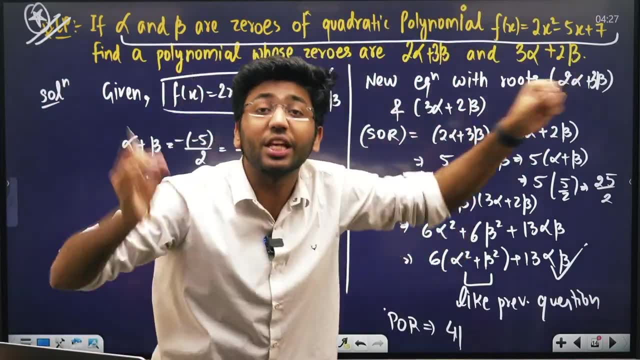 But the question will be like this: If alpha and beta are zeros of this polynomial, If I have alpha and beta zeros of this polynomial, So what did I write when I read the first line? What did I write when I read the first line? 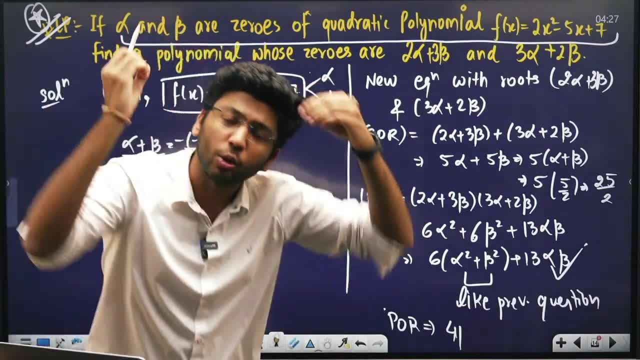 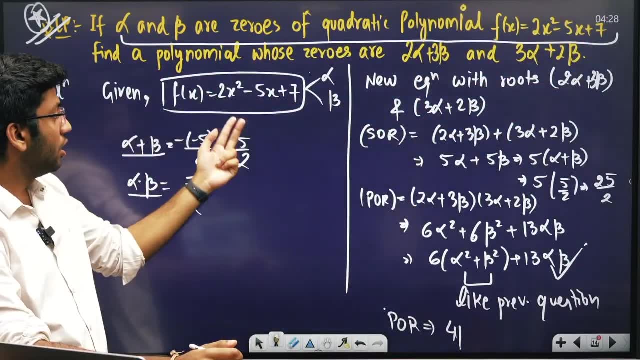 Sum of roots and product of roots. I said I will not write anything. I will read further later. I wrote earlier. I said there are alpha and beta zeros of this equation. So it became: minus b by a Means 5 by 2.. 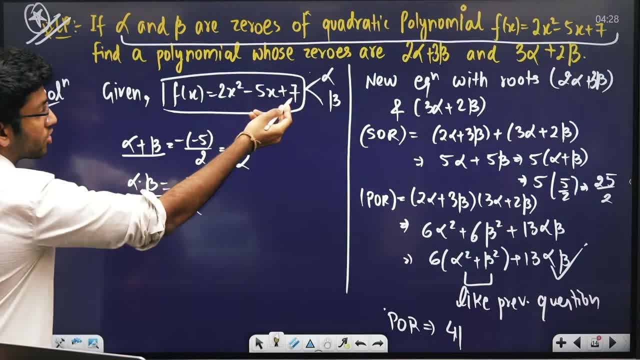 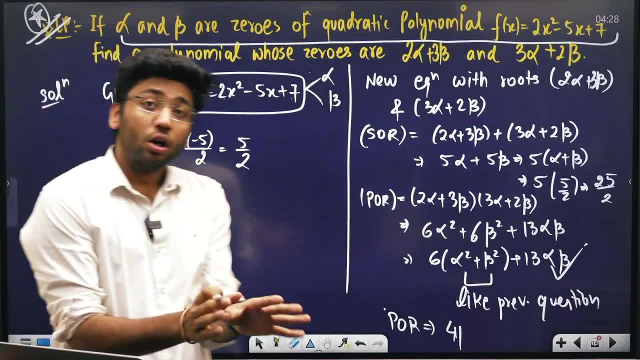 So minus of minus 5 by 2.. And product of roots became c by a, Means 7 by 2.. Now I will read further: Find a polynomial If I want to make a polynomial. Shobit bhaiya said: 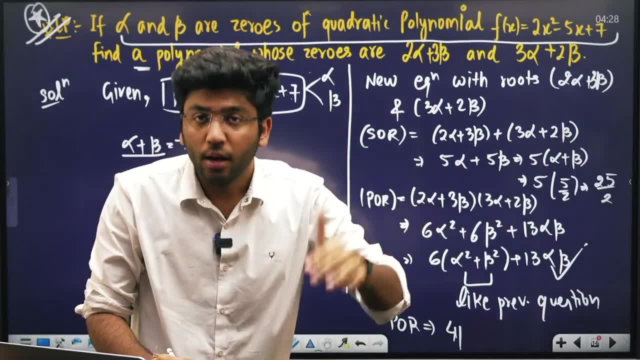 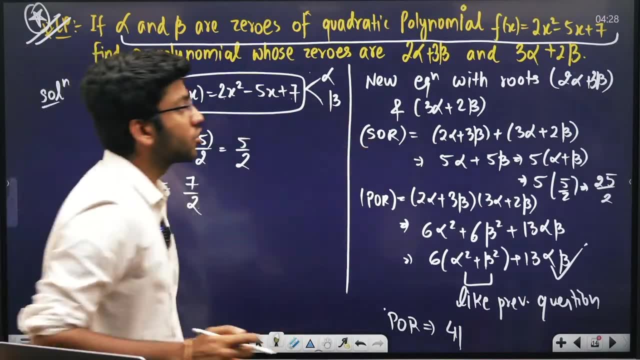 If I want to make a polynomial, then the sum of roots and product of roots is needed. If I want to make a polynomial, then the sum of roots and product of roots is needed. So make a polynomial with roots of this and this. 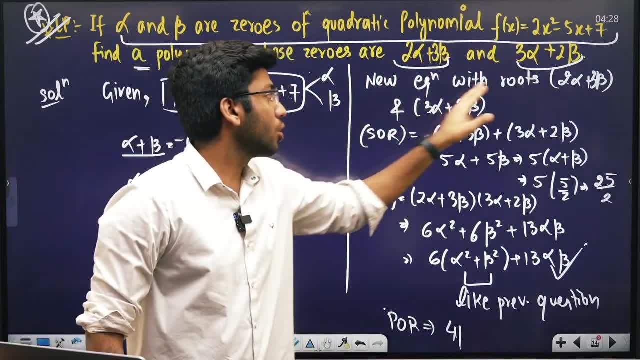 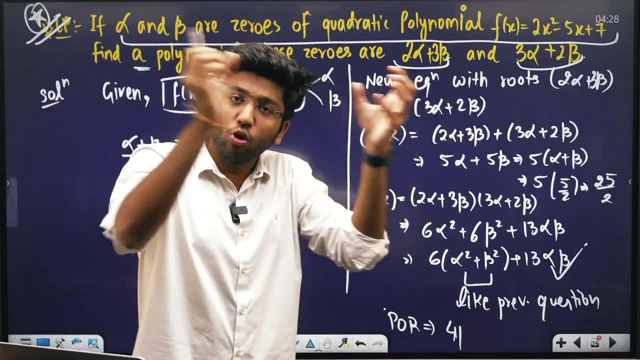 So I said, okay, these two roots are good. so I have to make an equation. whose roots are this and this? So if I know two roots, then how will I know the equation? First I will sum them, then I will know the sum of roots which I got, 25 by 2.. 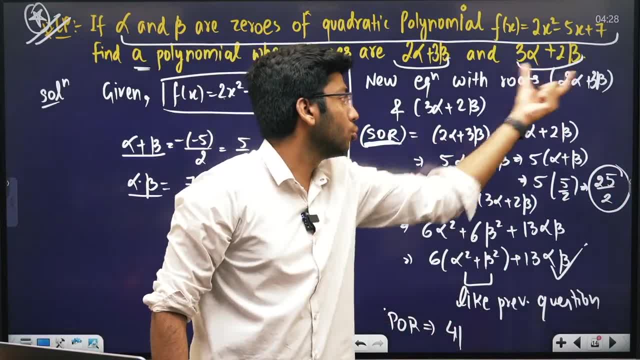 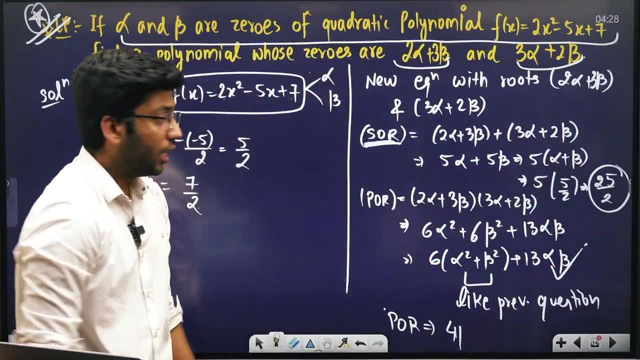 What did I do? I summed this and this. these are two roots. this is a whole big root, This is one root, this is one root. So first I summed, then I got the sum of roots. Okay, I did the product of these two, then I got the product of roots 41.. 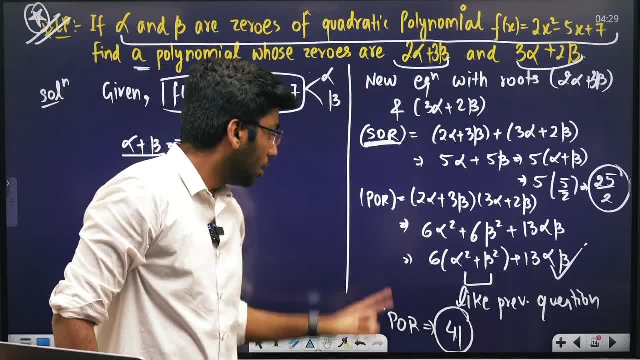 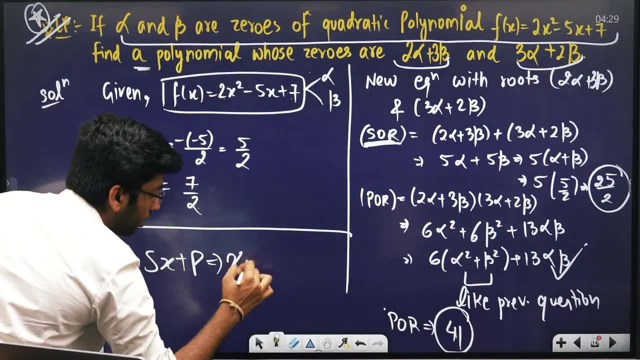 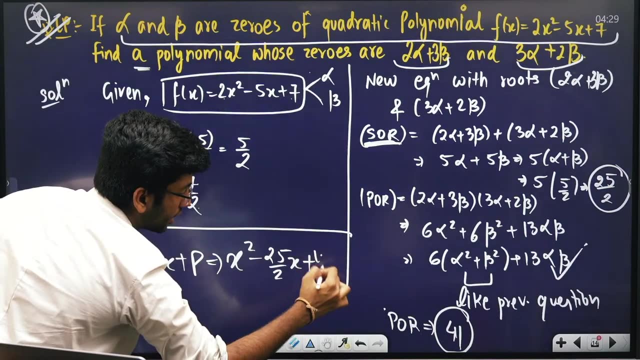 So as soon as I got the sum of roots, 25 by 2, the product of roots is 41.. So now how will I write the equation? I will write x square minus sx plus p. So x square minus the value of s- the value of s is 25 by 2, into x plus the value of p is 41.. 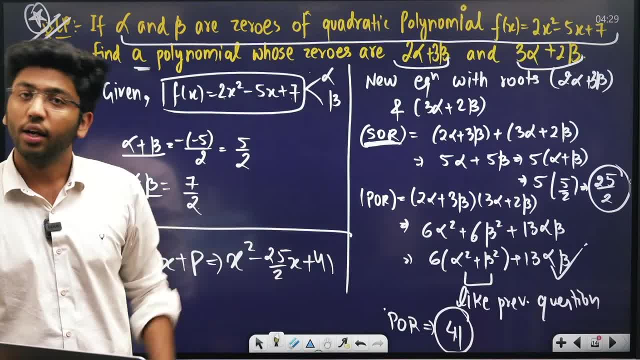 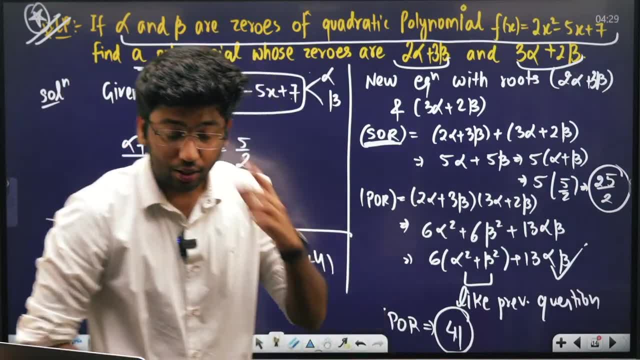 Okay, you can leave it like this, or you can take LCM and leave it. If you take LCM, then also the answer will come: Okay, Okay, what are you writing? Like it? Oh, it will be done. it will be done. 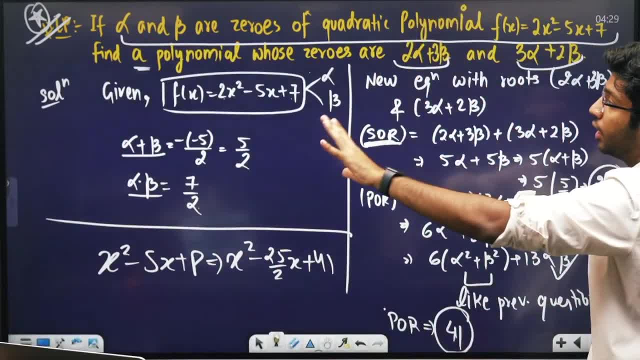 Like, will be done later. Okay, now we will focus on studies. Like it was just for one or two days Now, we will focus on studies. So whenever such a question will come, that tell me. tell me which polynomial has these roots. 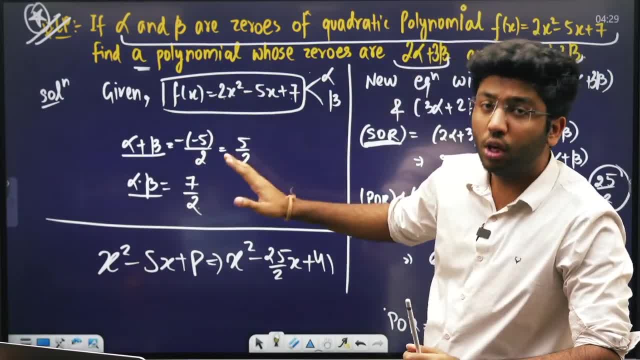 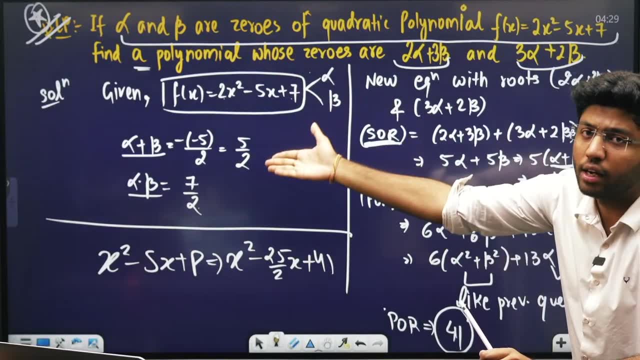 So first write the sum of roots, product of roots of the given. Why? Because alpha plus beta and alpha includes beta. they are useful here. See, instead of alpha plus beta I put 5 by 2 here, So it is useful from here. 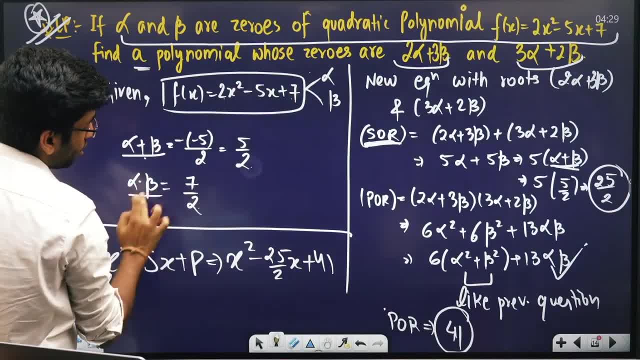 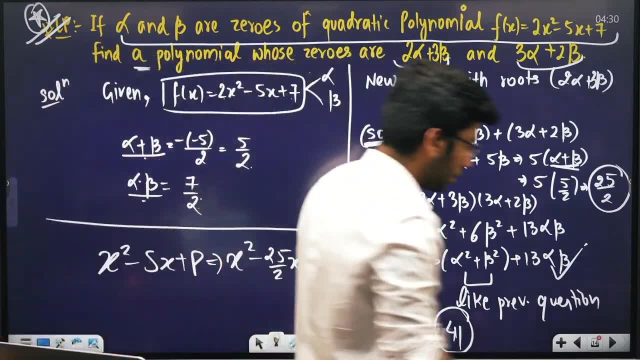 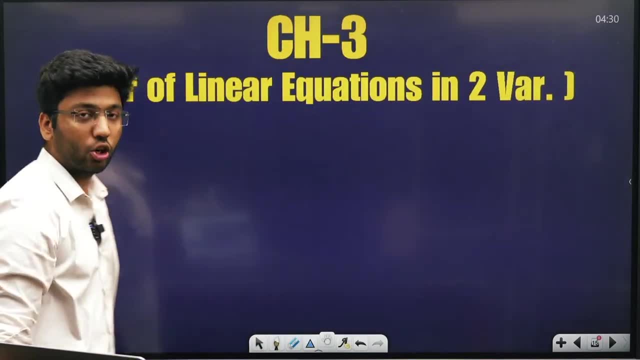 So this equation that was given this was only given for its value. Apart from that, this equation has no use. Okay, okay, let's come to the next question. Next chapter comes your pair of linear equations in two variables. Okay, from the previous chapter, polynomials. from which questions can we come? 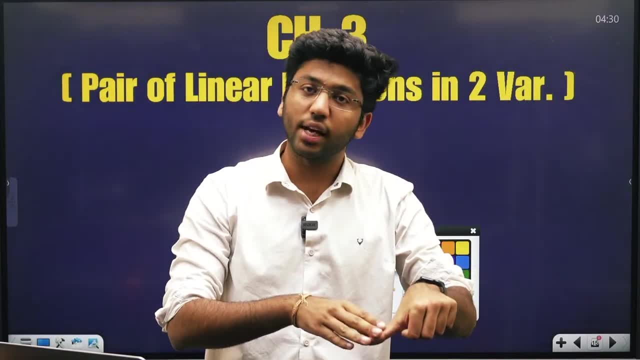 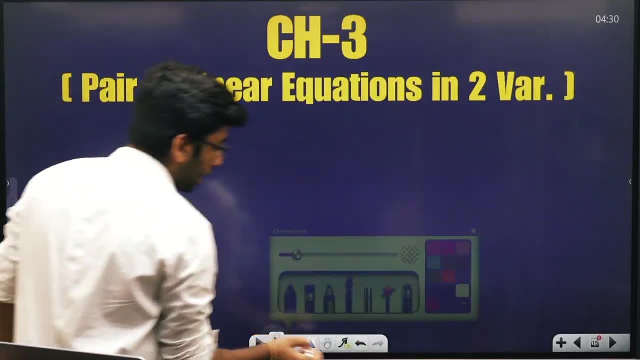 What did I tell you? One sum of roots, product of roots, can come from that And and form a quadratic equation. The question has to come on this. Okay, the question has to come on this. Now let's talk about pair of linear equations in two variables. 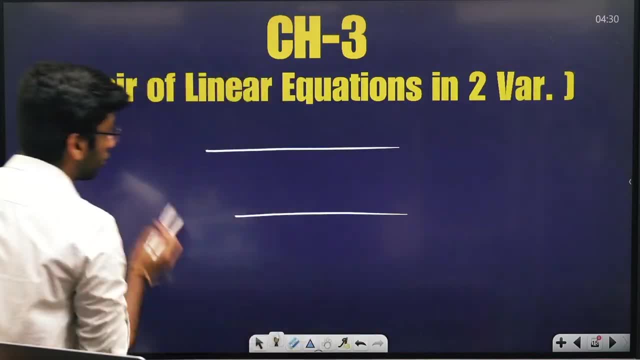 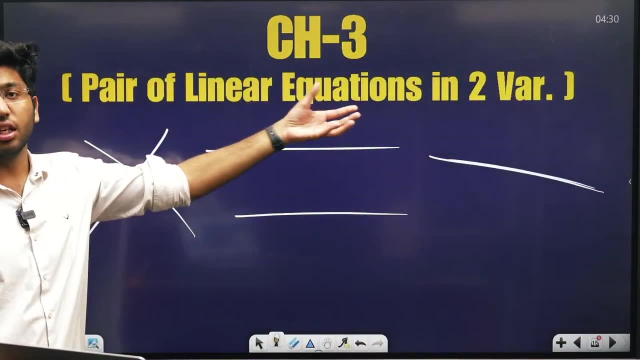 So we have talked about two linear equations, So we have talked about two lines. Either that line will intersect, or it will be parallel, or it will be coincident. Coincident means that one will come on top of the other. So these three, these three can be our conditions of two lines. 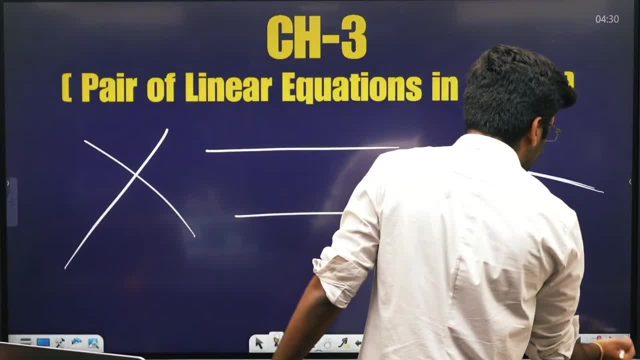 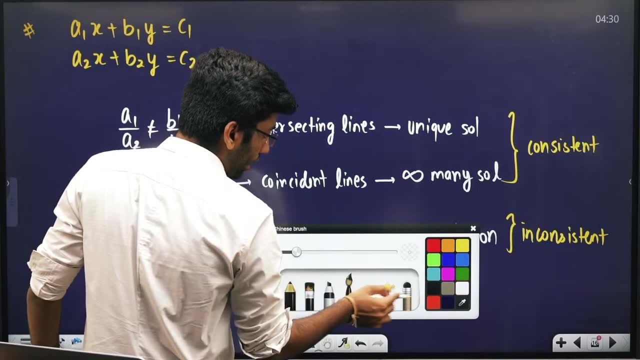 Okay, pair of linear equations means talk about two lines. So how will we know when it is linear, when it is parallel, when it is intersecting? So see, suppose these are two such lines, Suppose these are two lines. do we remember this? 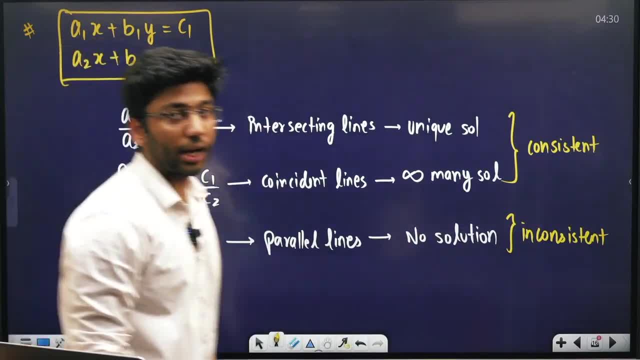 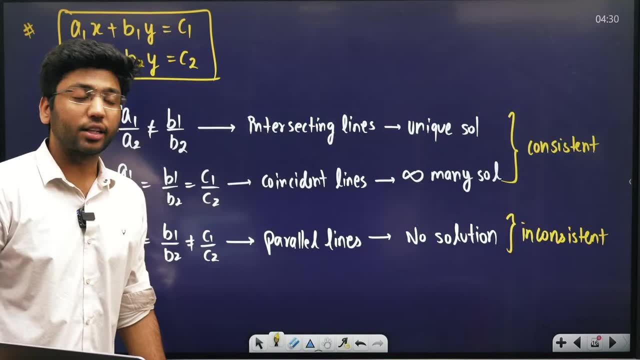 Okay, the question has to come from this. The question has to come from this. absolutely From which? From this It will ask you: tell me what is the condition. When will it be parallel? When will it be intersecting? 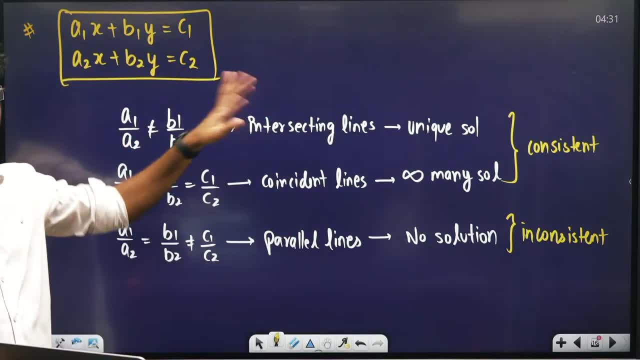 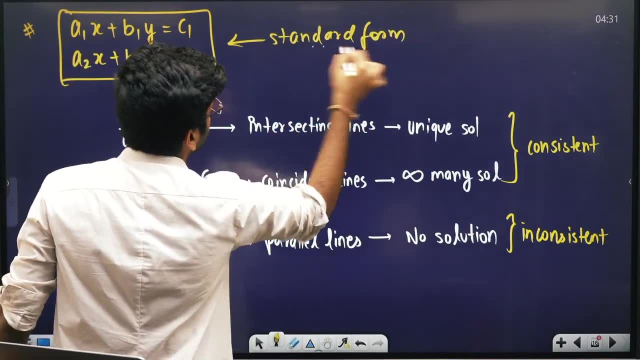 And when? will it be coincident? So first of all, write the equation like this: What is this? This is called the standard form. This is called the standard form. Writing in the standard form is the most important. Remember this. Kids make a mistake here. 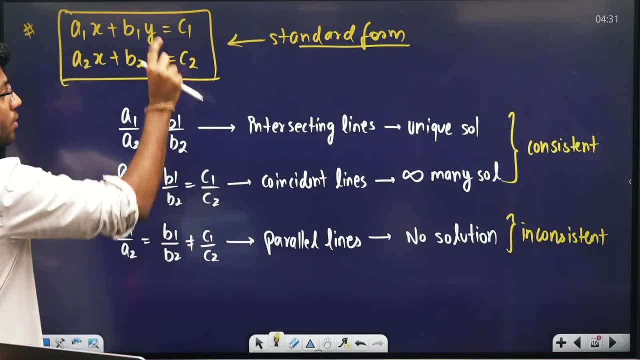 What? That we do not convert it to the standard form. Standard form means the constant term in RHS, The constant term in RHS. So first of all we will convert it to the standard form. So it became like this in the standard form: 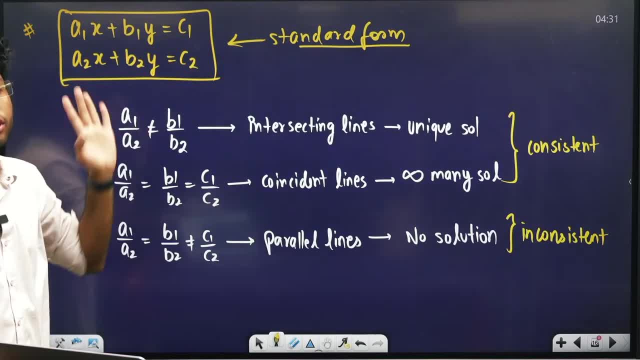 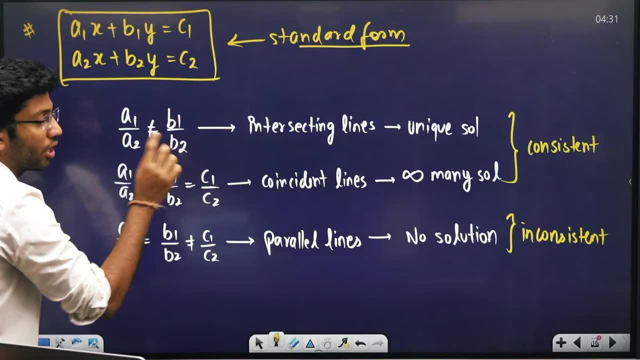 a1x plus b1y equal to c1, first equation: a2x plus b2y equal to c2, second equation: Now compare the coefficients. of this Means if a1 upon a2 is not equal to b1 upon b2.. 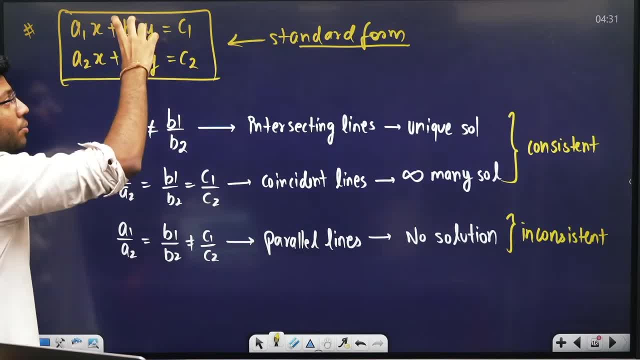 First what I did. I took a1 upon a2 out and kept it aside. B1 upon b2 kept separately, C1 upon c2 kept separately. So if a1 upon b2 is not equal to b1 upon b2,. 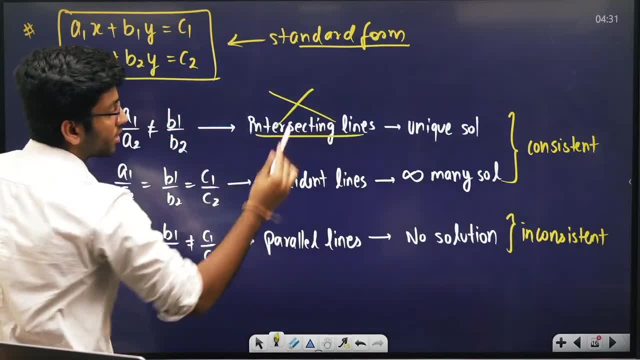 then there are intersecting lines, Means there are intersecting lines. Intersecting means only one solution, So unique solution If a1 upon a2, b1 upon b2 and c1 upon c2, all three came equal. 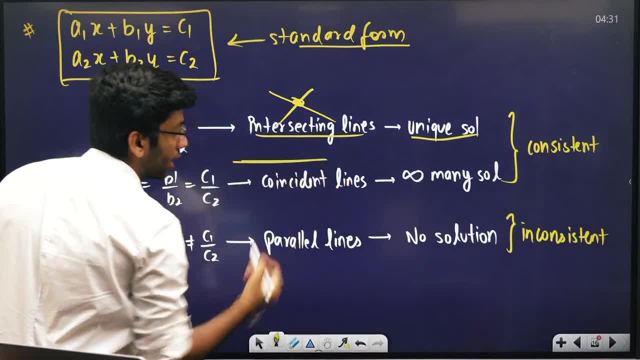 All three ratios came equal, Then it is coincident. Means one is going up and one is going down, Means there are many solutions. And if a1 upon a2 is not equal to b1 upon b2, but c1 upon c2 is not equal, 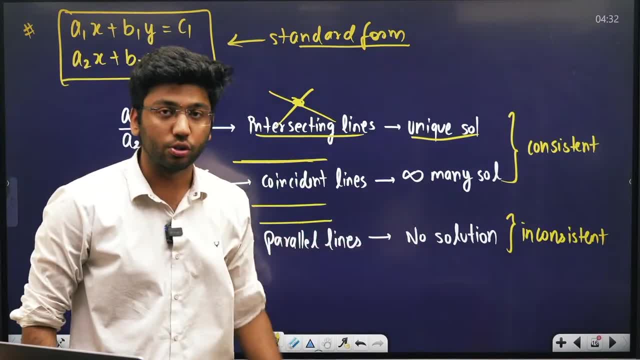 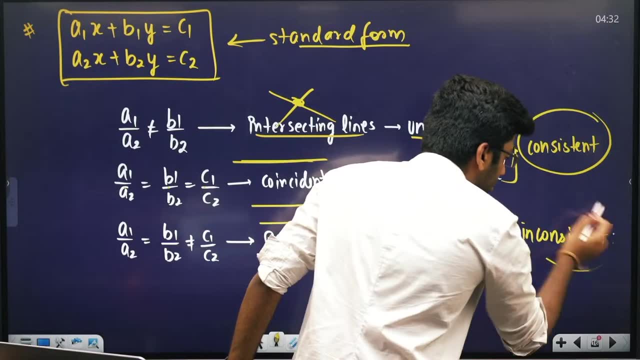 then there will be parallel lines. And what happens in parallel lines? No solution. So the case of even one solution is called as consistent by the world, And when even one solution is not there, then it is called as inconsistent by the world. 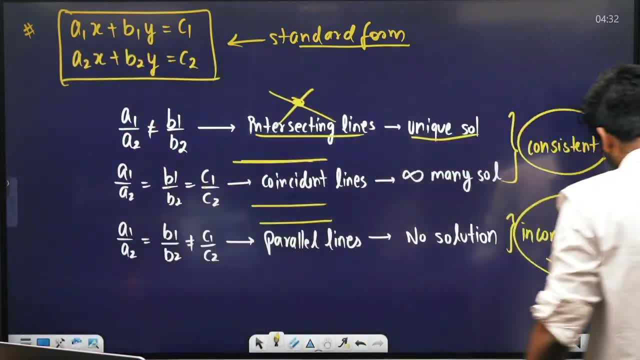 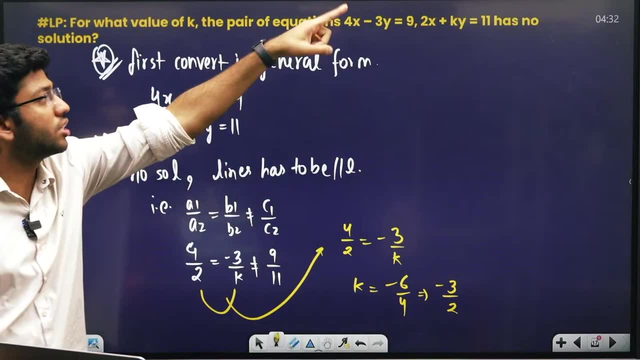 It is just a name. It is just a name, Okay. Okay. So your question can be like this: Find the value of k, for which the pair of equations this and this has no solution. So what we have to do for no solution. 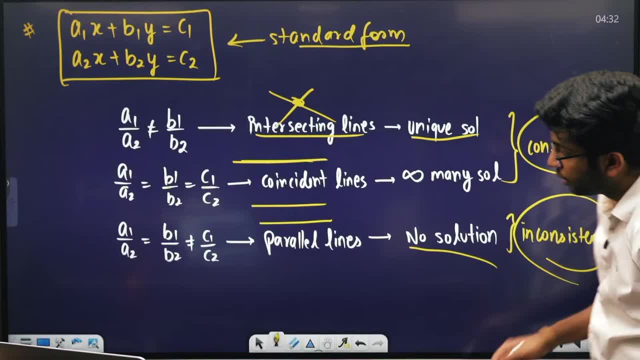 This will come in the table's mind. No solution means no solution means I have to apply this condition. I have to apply this condition: a1 upon a2 is equal to b1 upon a2, but not equal to c1 upon c2.. 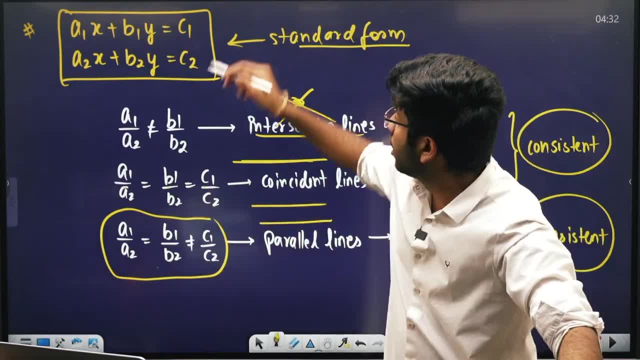 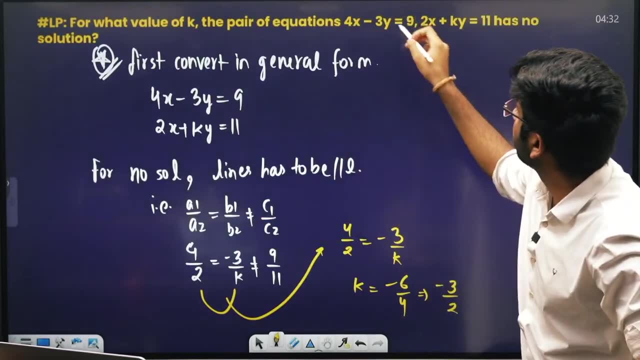 But before applying this condition, keep one thing in mind: What It should be in standard form Means the term of constant is equal to this side. Have I given the term of constant equal to this side? Have I given the term of constant equal to this side? 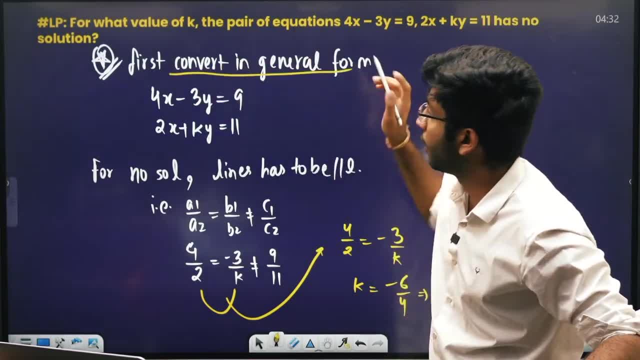 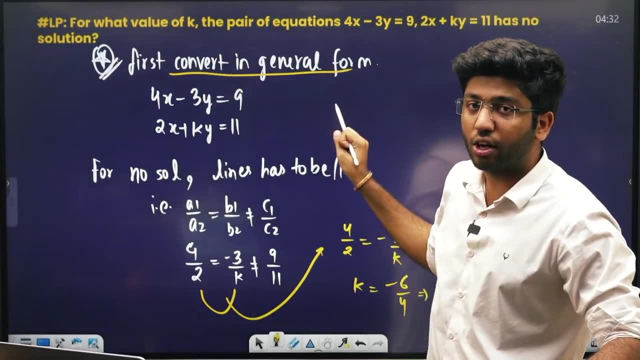 Yes, I have given it Means. it is in standard form. It is converted in general form. It is converted in general form. Here I have applied start. Here only CBS can play with you. So just take the constant term on this side of equal to. 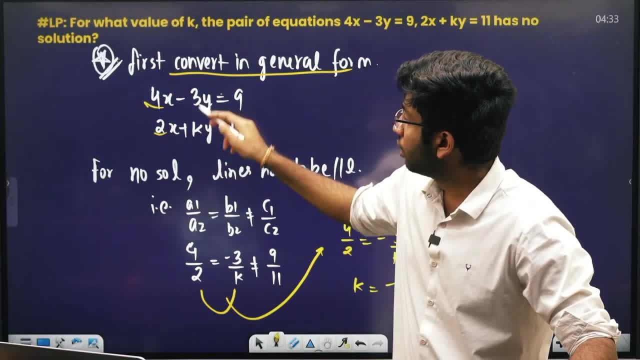 Now these two equations are made So a1 upon a2 is equal to b1 upon b2, but not equal to c1 upon c2.. I have written this, Okay, I have written this. Whenever it will come in this way: 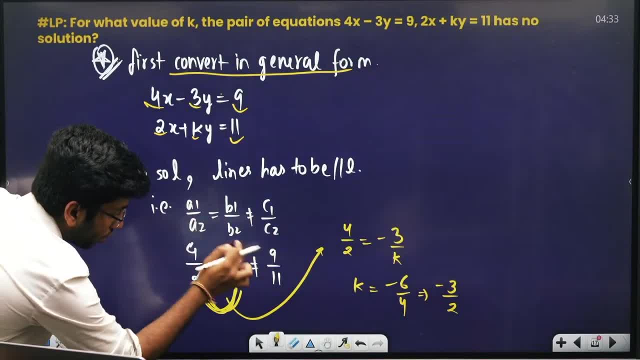 then I said my answer is being made by these two. So I took these two things, I kept it here. So the value of k came from here minus 3 by 2.. The value of k came from here. 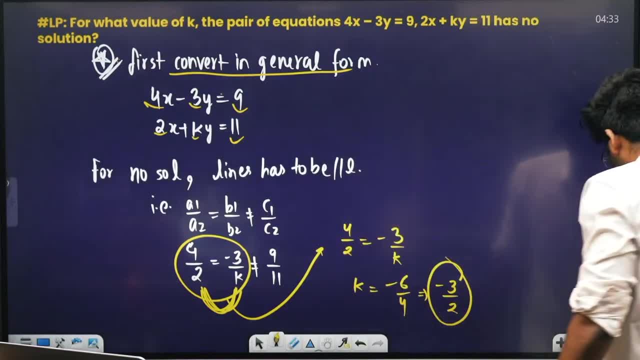 minus 3 by 2.. Okay, Some kids have also taken it out. Well done, So there was a chance to get a question from here. This is a very nice question to CBSC. This is a very nice question to CBSC. 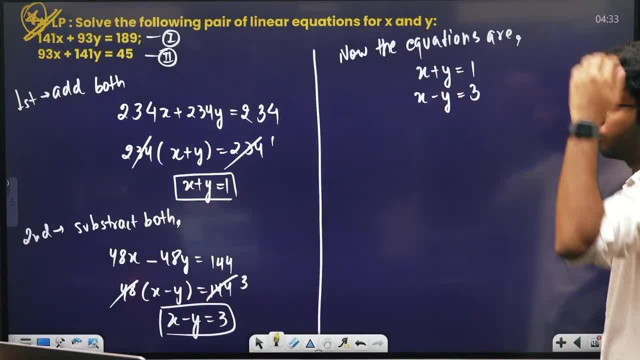 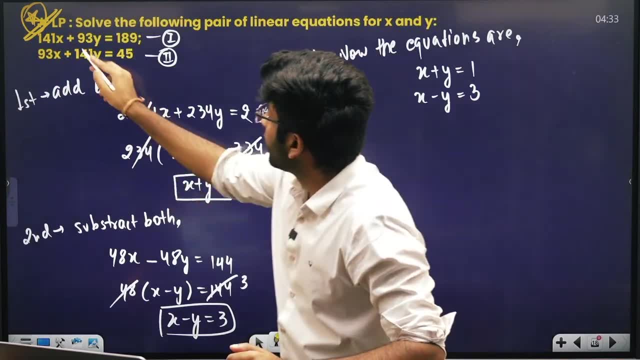 This is a very nice question to CBSC. CBSC can definitely ask such kind of questions. What is it? See, there was 141 with x. here 141 became 141 with y. Here there was 93 with y. 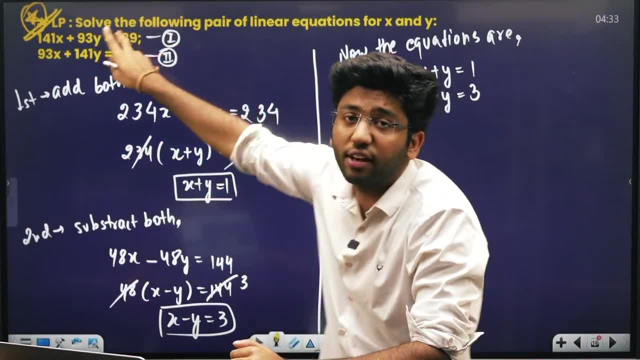 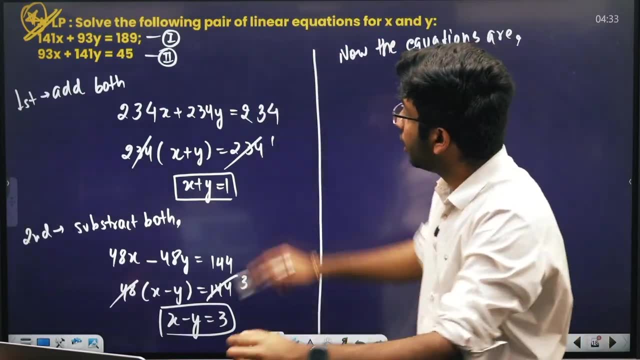 here 93 became with y, So it asks such questions about coefficient interchange. What is the best way to do this? What is the best way to solve this? What is the best way? First, add these two equations. So what will happen if you add? 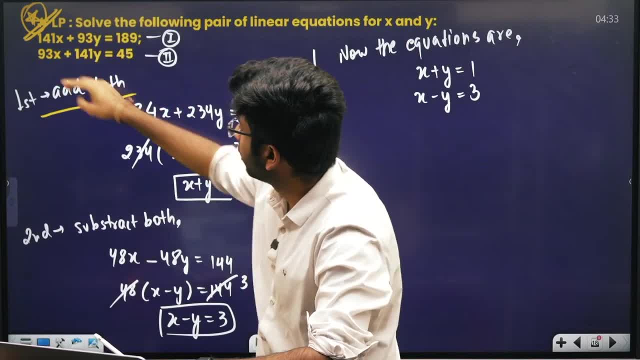 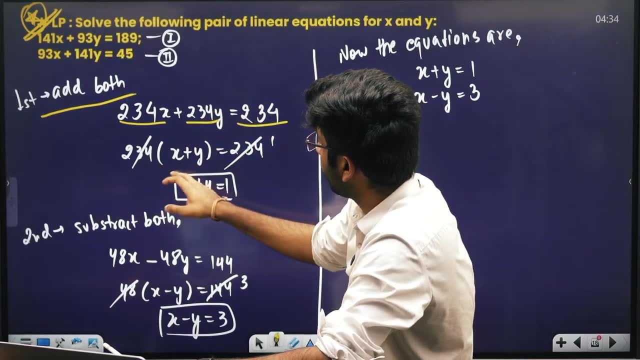 Add LHS to LHS, add RHS to RHS, So 141 plus 93, 234.. 93 plus 141, 234.. If you add these two, then 234.. If you take 234 and subtract, then x plus y equals to 1.. 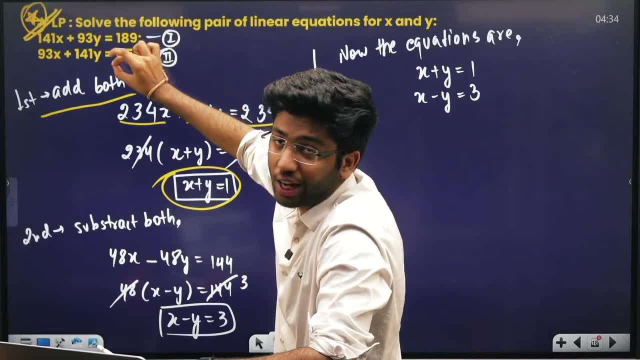 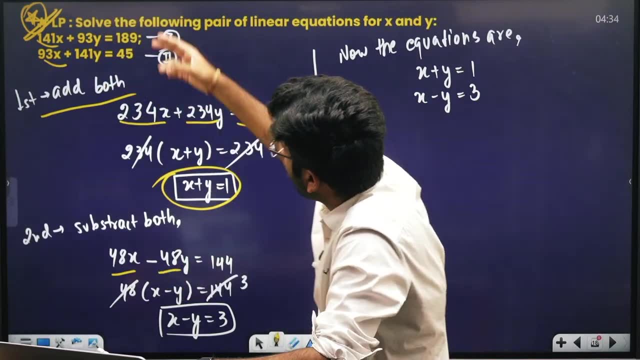 So add these two at least once. Subtract these two at least once. If you subtract, 93 out of 141 becomes 48.. 141 out of 93 becomes minus 48.. And 145 out of 189 becomes 144.. 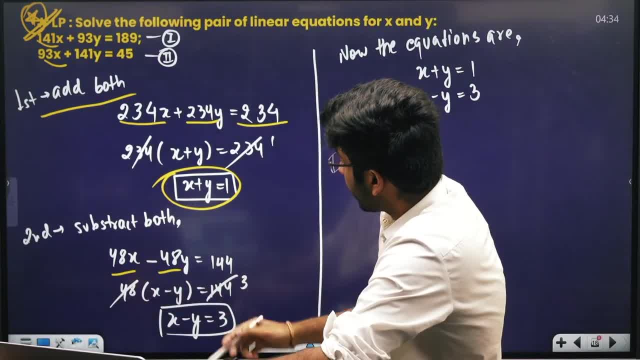 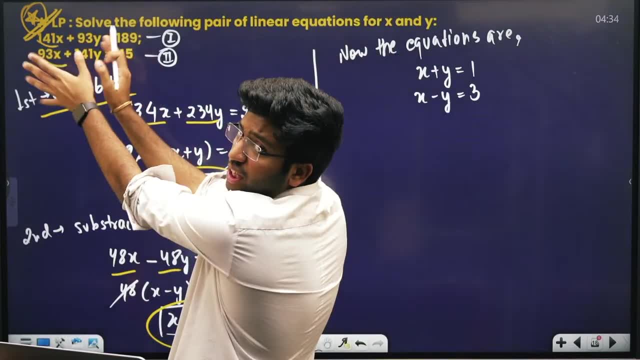 48 is common, 48 plus 3 is 144.. So one equation becomes: x plus y equals to 1.. And one equation becomes: x minus y equals to 3.. So the equation which was so heavy, the equation which was so heavy, 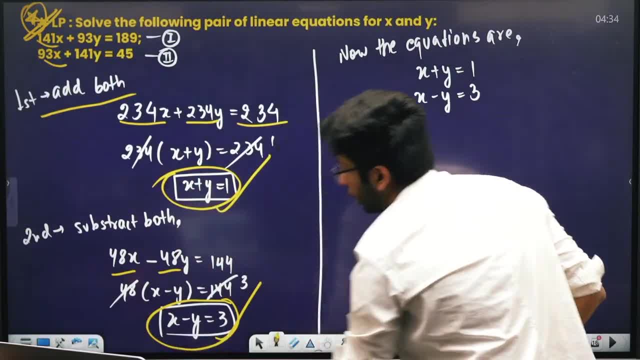 I broke it in such a small equation. I broke it in such a small equation. Now, what to do? Solve these two equations. How will you solve it? Take one of the values and put it in the other. Do substitution Or do elimination? 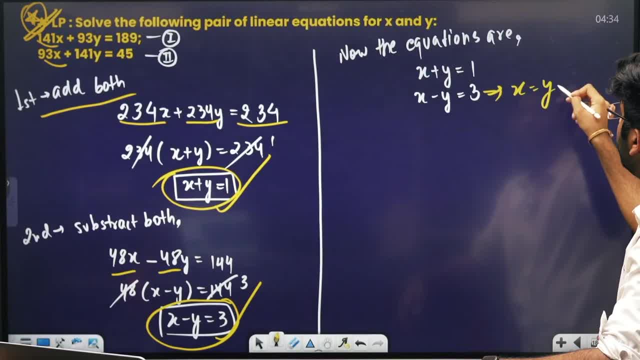 You can do anything. So what did I do? I took x's value y plus 3.. I took x's value y plus 3 and put it in it. So instead of x, I will keep y plus 3.. 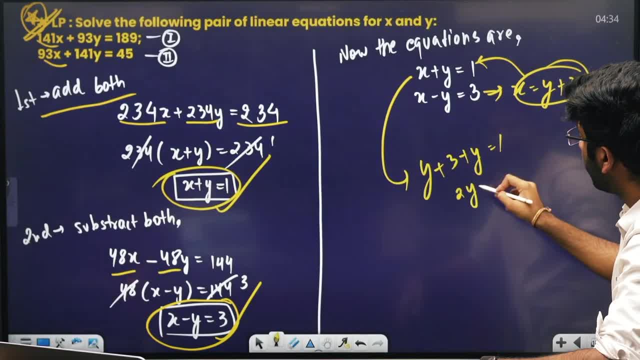 So y plus 3 plus y equals to 1.. So 2y plus 3 equals to 1.. So what is the value of y Minus 2.. If this goes here, then minus 2.. Minus 2 upon 2.. 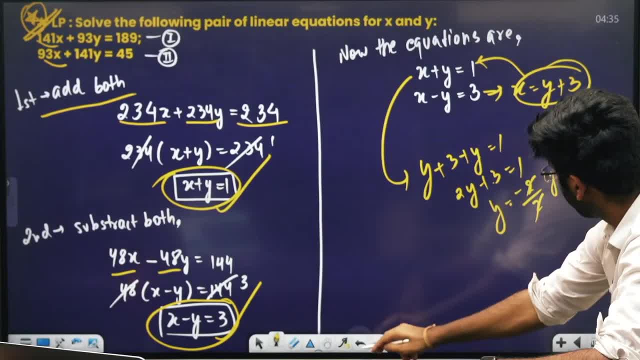 So the value of y is minus 1.. The value of y is minus 1.. The value of y is minus 1.. So what will be? the value of x Minus 1 plus 3 is 2.. The value of x will be 2.. 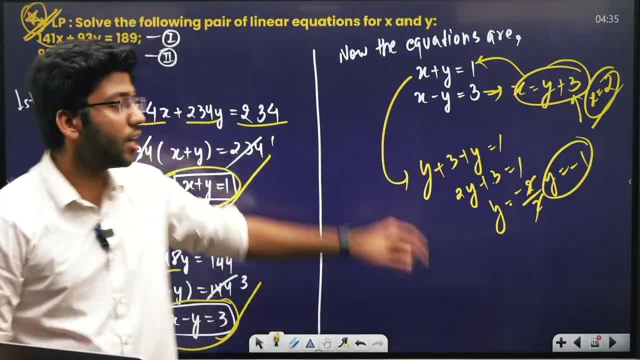 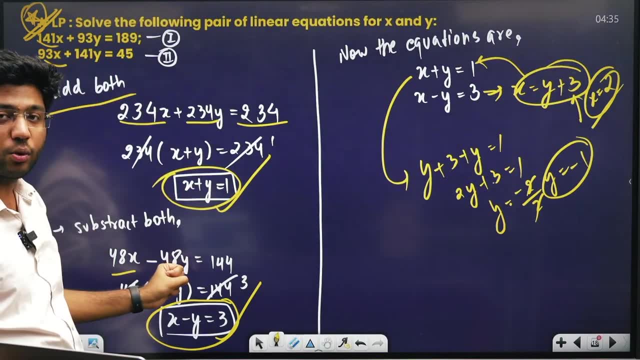 Okay, So we will take out y and x in this way. So this is an important question In this way. whatever question will come whenever you will see such heavy terms, then add it once. Subtract the equation once. You will get a small equation. 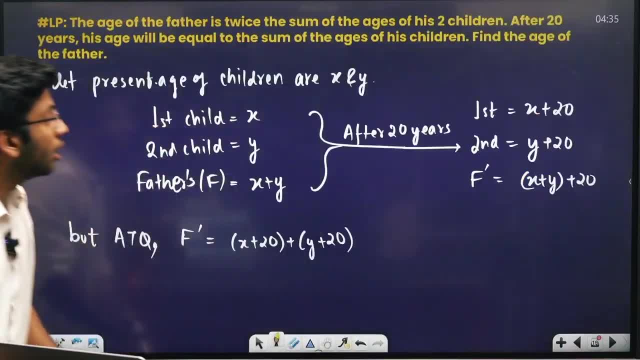 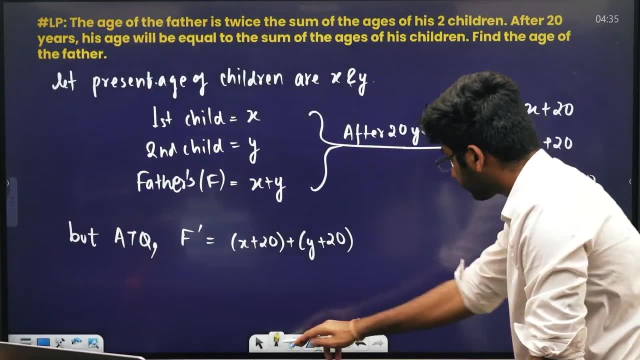 Solve it. Okay, This was very important. Next, The question of father and son. It is very lovely. It is very lovely. CBSC has asked this question many times. How Look, Look, Look carefully, Look carefully at this. 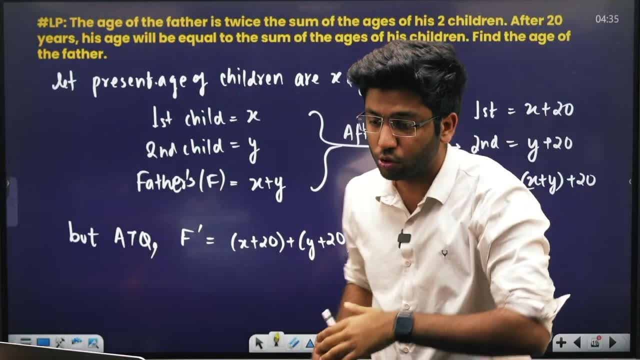 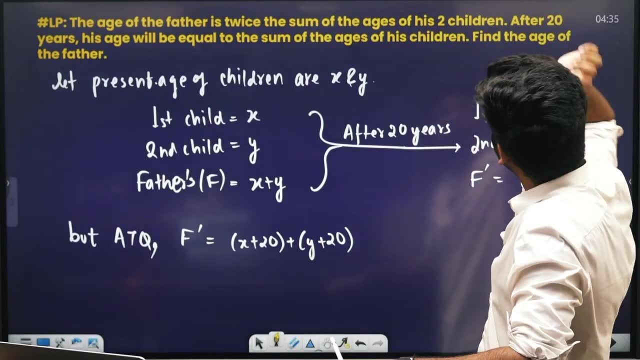 Children get confused in this. Look carefully at this. Children get confused in this. It is said that the age of father is twice the sum of the ages of his two children. After 20 years, his age will be equal to the sum of the ages of the children. 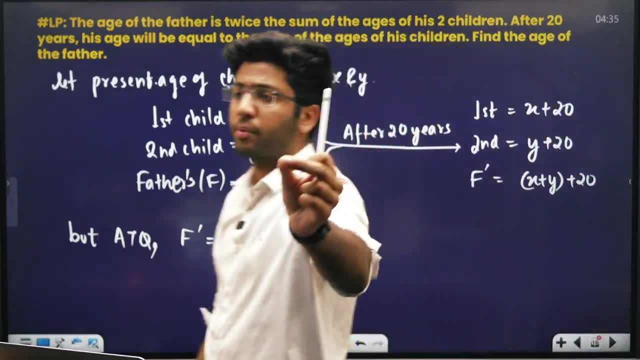 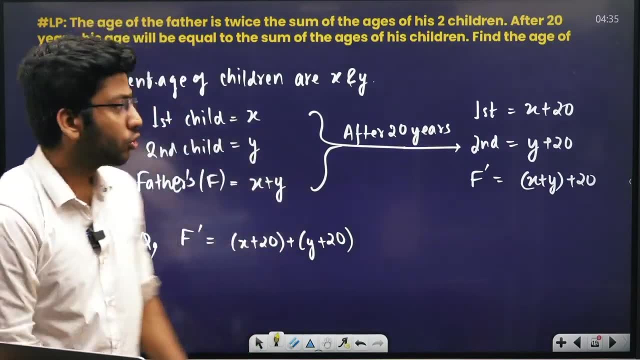 Find the age of the father. So the best way to do this is the present age of the son, The present age of the children. So their present age is X and Y. Look, Present age of children is X and Y. 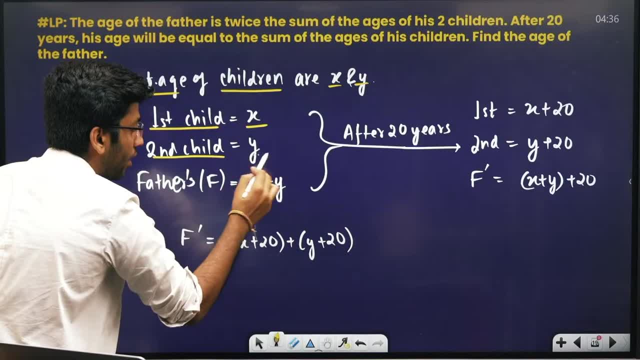 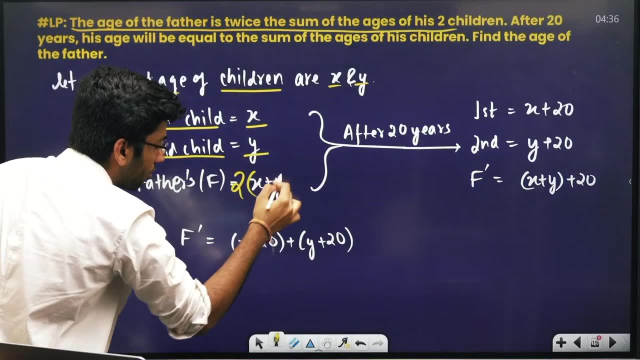 So how do you know the present age of the first child X, and the present age of the second child, Y? And the answer is: the age of the father is twice the sum of the ages of the two children, So the result to be twice the sum of the ages of the two children. 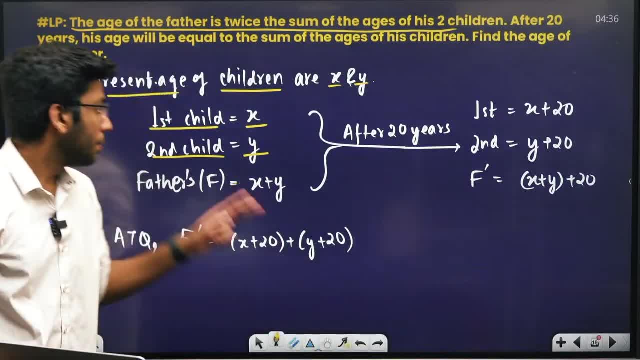 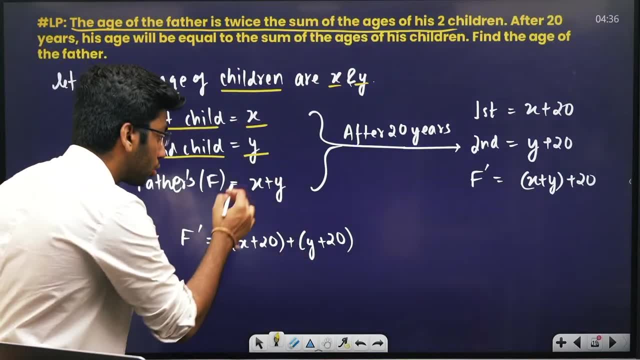 is the father's age. Look again carefully. See Next. referring to father's age does not correspond to the real age of the father and therefore a child's father's present age is the total number of two children ages of two children, so twice the sum of ages. This is the present age. Now he is saying: 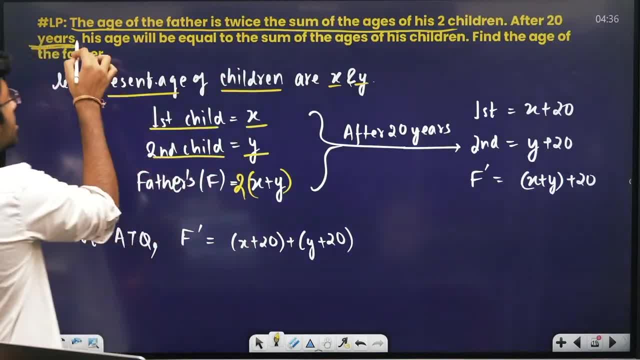 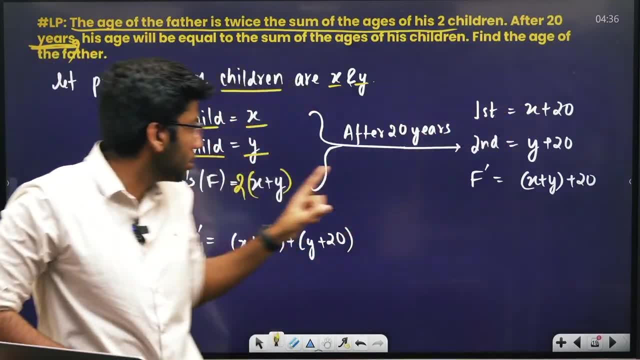 after 20 years. after 20 years. after 20 years there is a coma. after 20 years, stay here. After 20 years. see, according to this, what will happen after 20 years? First child's x plus 20,. second child's y plus 20, and what will happen to the father 2 times x plus y? 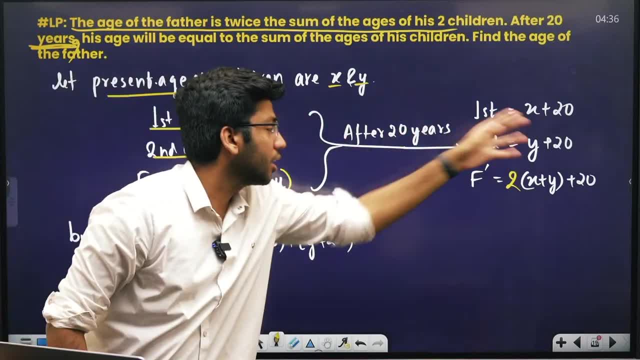 plus 20.. We will add 20 in this. we will add 20 in this. we will add 20 in this. So, after 20 years, this is the father's age. this is the age of the children. Now read the question. 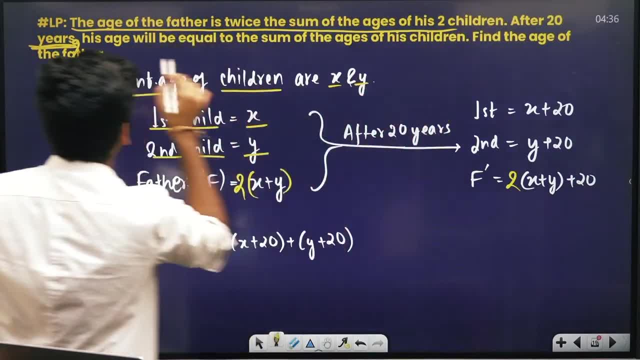 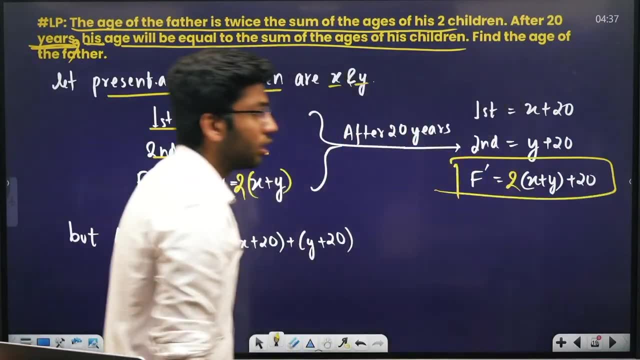 again The father's age after 20 years. his age means the father's age will be equal to sum of ages of his children. Okay, we took this out. we took this out. And the question is: he is saying that the father's age will be equal to the age of both the children. 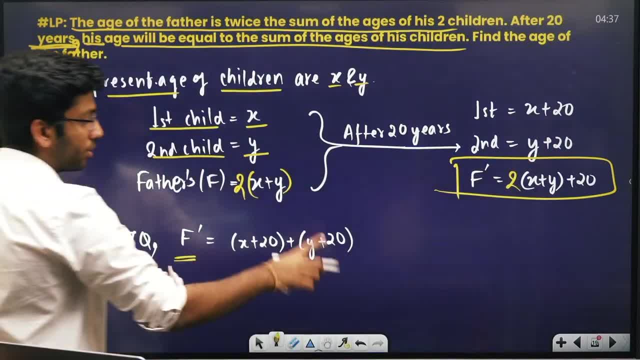 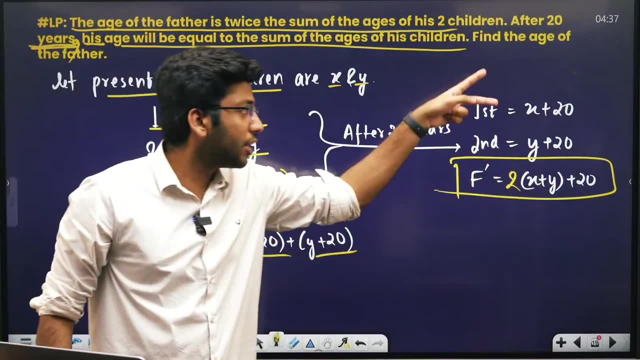 Means the father's age will be. the father's age will be the f? dash. we took out first, f was this, then f? dash came out this, But the question says f? dash will be this. So the question is saying that after 20 years, if you sum up the children's age, then 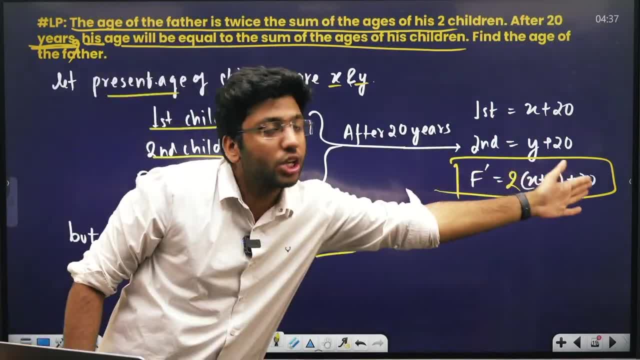 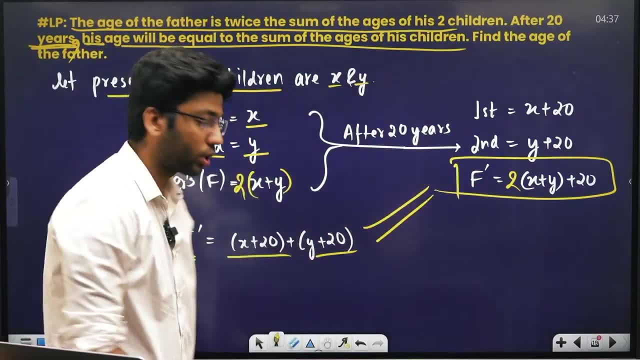 that will be the father's age And, according to us, the father's age is coming, So means he is giving the question we are giving it. So what will happen to these two? They will be equal. Just make this and this equal. What That? x plus 20 plus y plus. 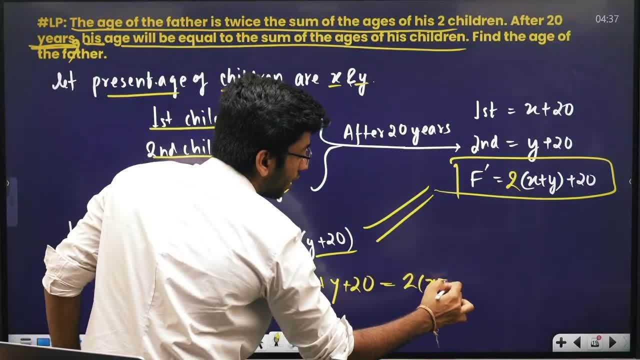 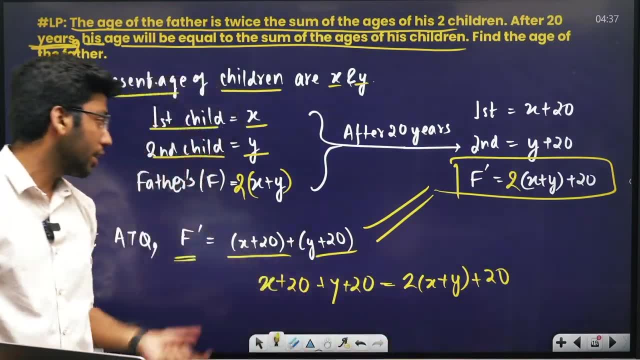 20, equal to 2 times x plus y plus 20.. If you make it equal to this, then x plus y will come out from here. Taking that x plus y and putting it here, the father's age will come out From here. x plus 20 plus y plus 20 will come out from here. So 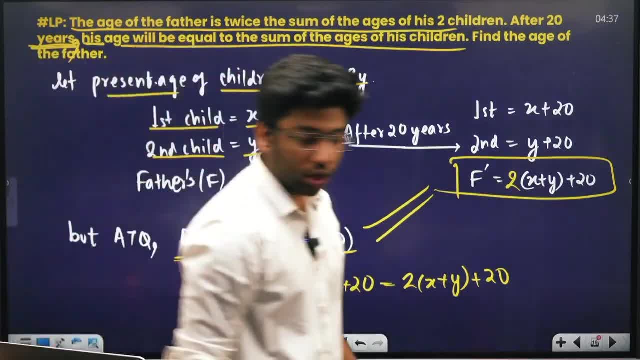 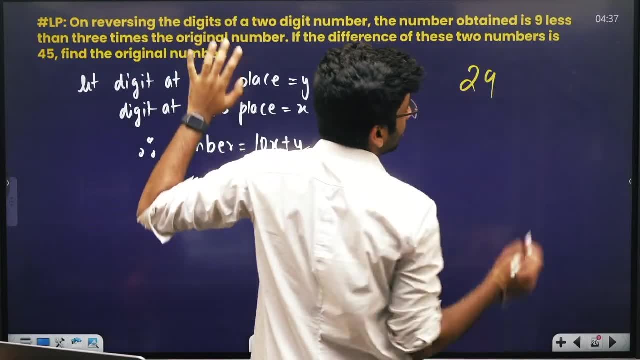 x plus y will speaking, Putting that here, the father's age will come out. Ok, next question on reversing of the two-digit number. Look at the two digit number. Let's say it's 29.. This is a two-digit number In which this is its unit place and this is its 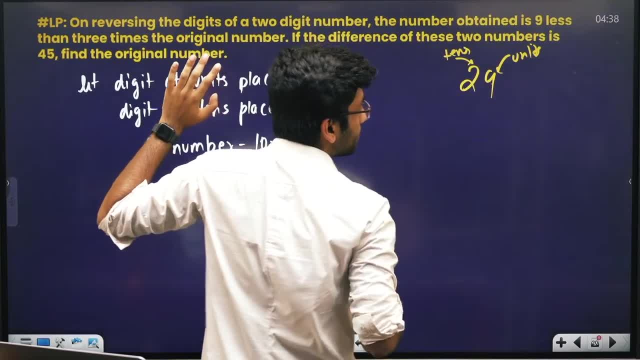 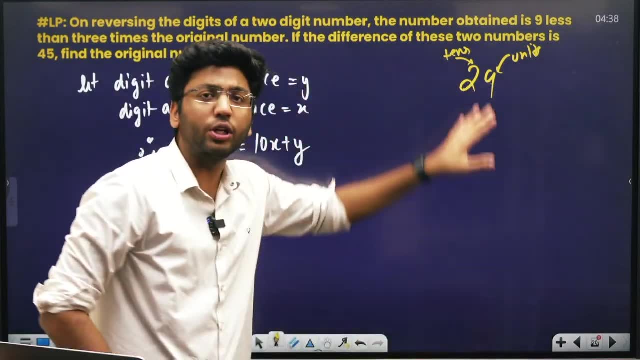 tenth place. This is the unit place and this is the tenth place. Do you understand what I am saying? Do you understand? So this is the unit space and this is the tenth space. If I am taking some two-digit number, then this is the unit place. this is the tenth place. How can I write this, Can I? 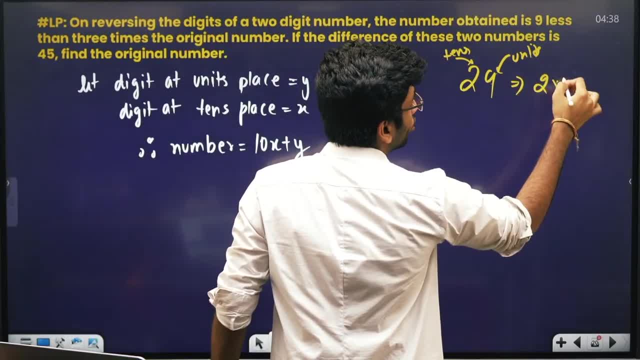 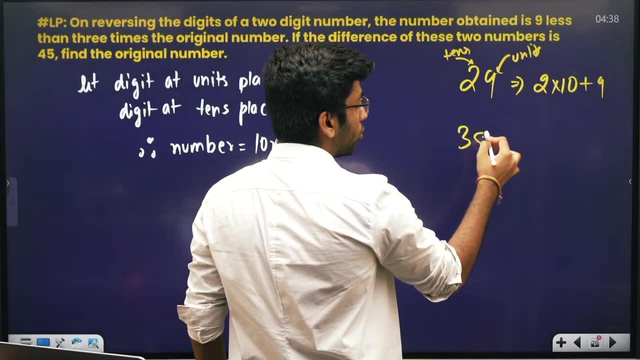 How can I write this? How can I write this: 2 into 10 plus 9 In tens. I multiplied tens In unit. I multiplied units Like: what can I write? 38?. 3 into 10. 3 into 10 plus 8. 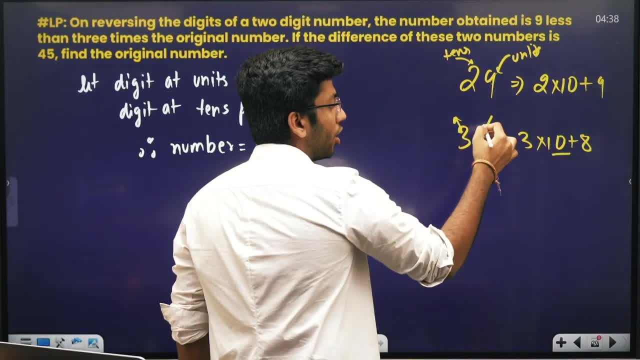 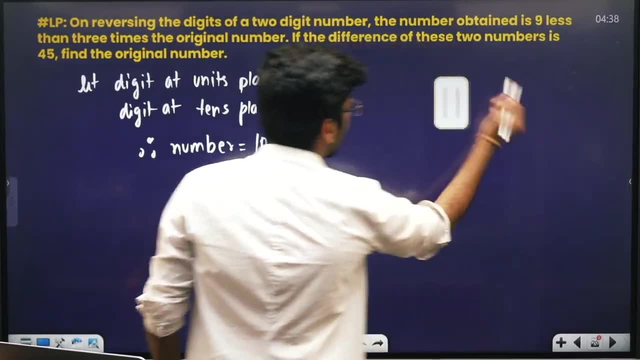 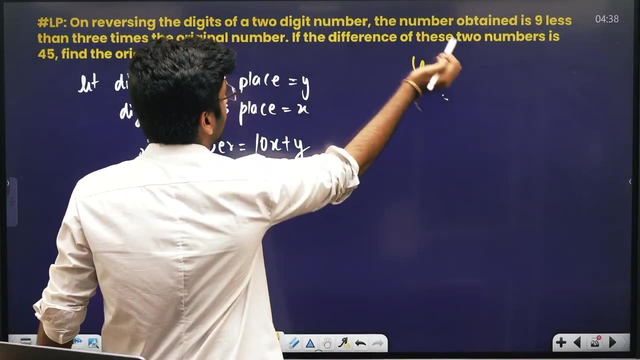 So in tens place 10 multiplied and in unit place 1 multiplied, So we can write 1 multiplied, like this: So similarly Now see my dear Assume, that In unit place there is digit x, In unit place there is digit y. 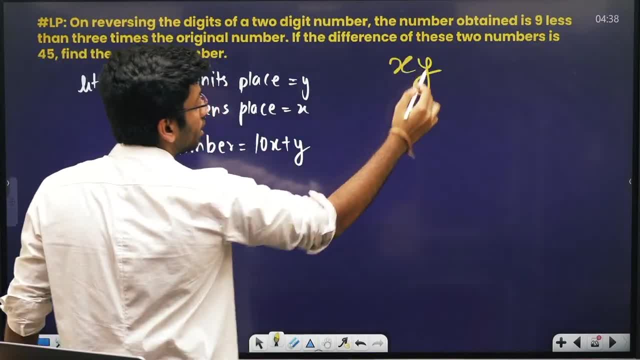 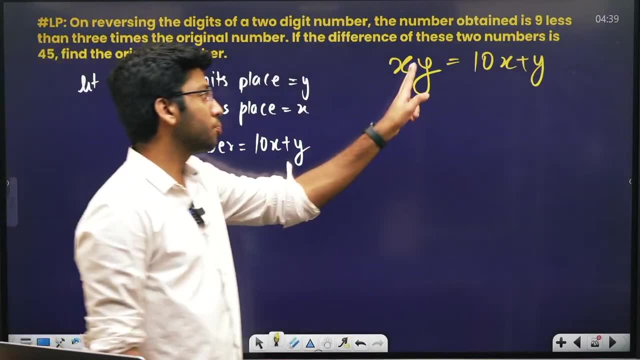 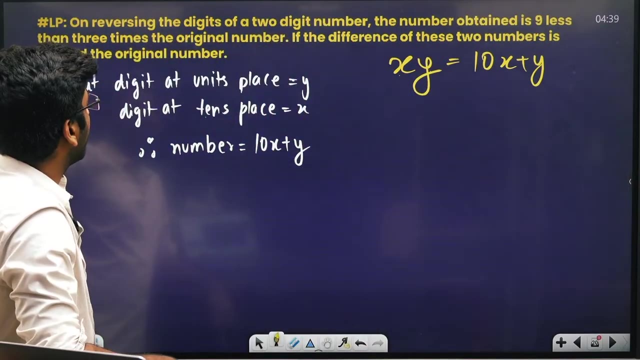 And in tens place There is digit x. So can I write this: 10x plus y Can I write? So in unit place there was digit y And in tens place there was digit y. I have said, I have said On reversing the digits of 2 digit number, 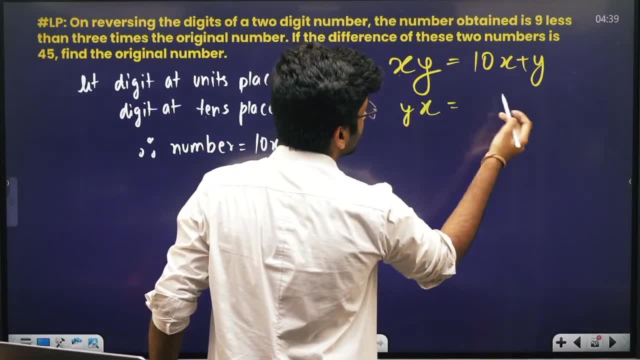 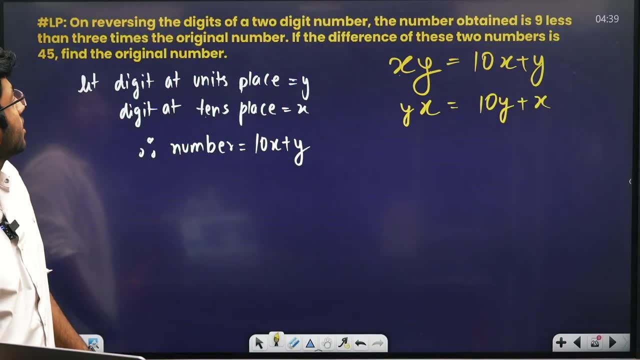 Now we have reversed, So this became yx. So how can I write yx? So I am saying, On reversing the digits of 2 digit number, The number obtained is less Is 9, less than 3 times the original number. So according to question, 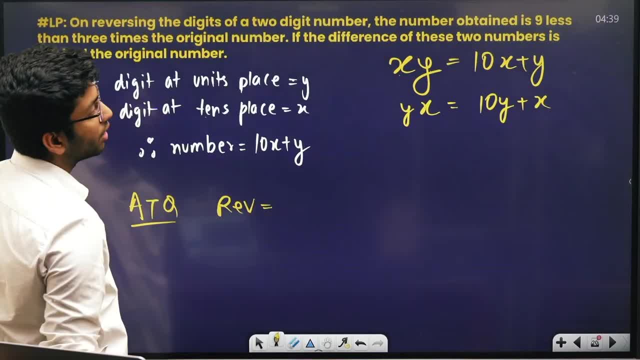 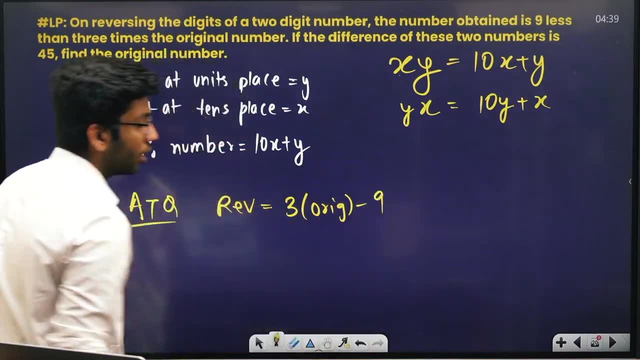 According to question The reverse number. What is that? That is 9 less than 3 times the original number, So 3 times Original minus 9. This is what the question is saying. Listen carefully Whenever you want to take 2 digit number. So you will take this. 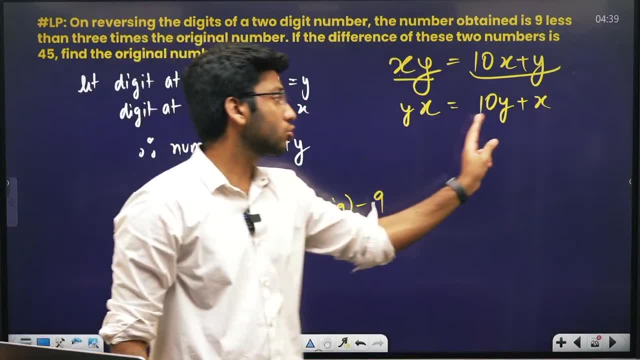 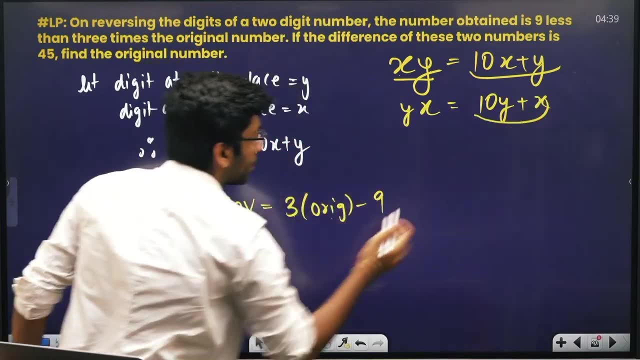 You will take xy, Which we can say like this: We will reverse it, So we can say this: So I am saying Reverse is 3 times original minus 9. This is written. So what is the reverse Reverse is this: 10y plus x. 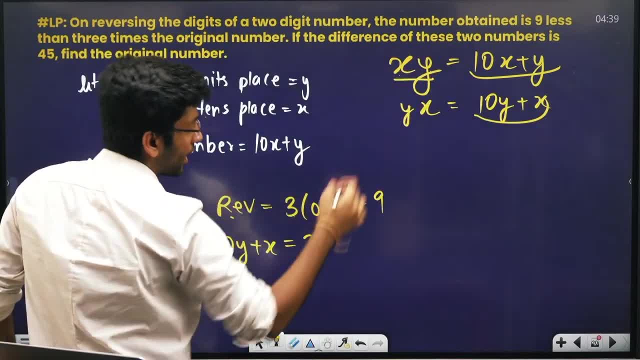 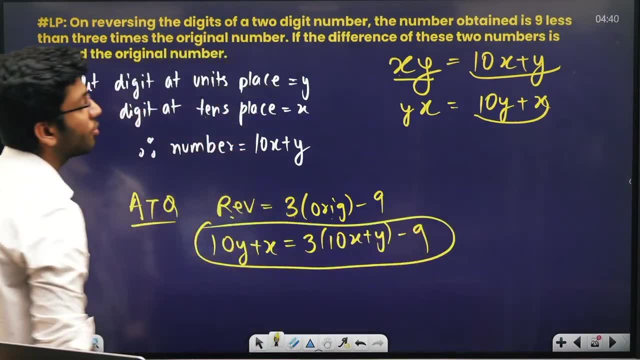 10y plus x. Who is equal to this 3 times? What is the original 10x plus y Minus 9? This is given to us. This is given to us. Okay, What other information is given to us If the difference of these 2 numbers is 45? 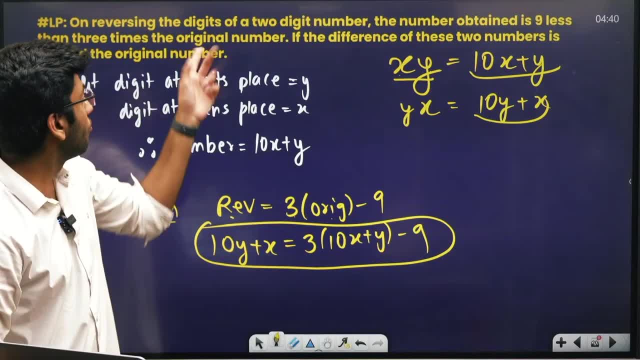 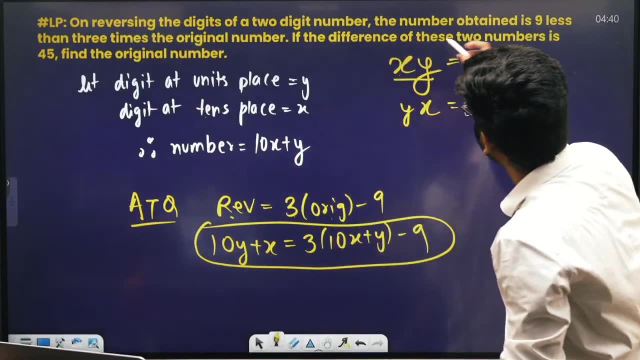 Okay, The difference of these 2 numbers is 45. Then find the original number. Then find the original number. So what is the difference of these 2 digits? Then, what difference has been given If the difference of these 2 numbers, Either the difference of both, 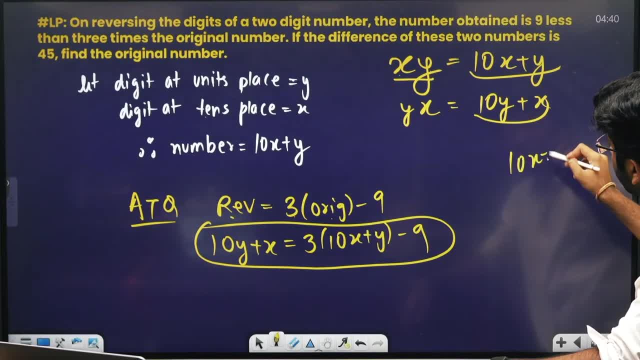 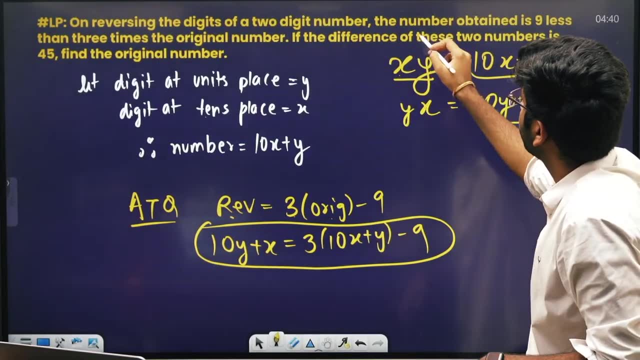 That means What is the difference of these 2 numbers? Then 10x plus y Minus 10y plus x, This I have raised the question a little bit. If the difference between digits, If the difference of digits, If the difference of digits, This is the question. 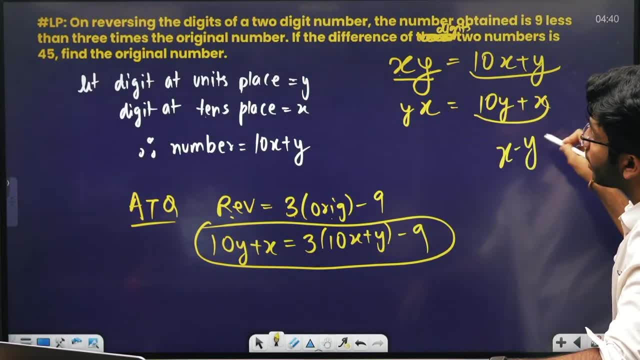 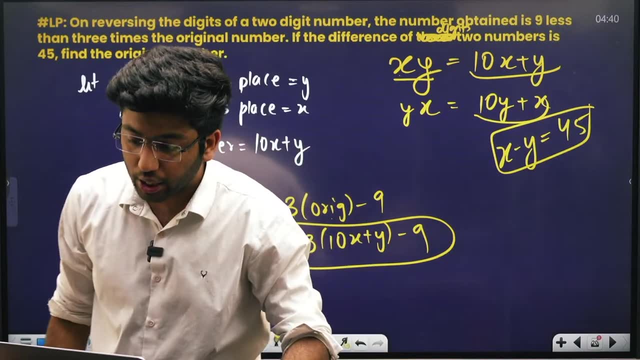 If the difference of digits, That means What is x minus y, What has been given to us, has been given 45, Then find the original number. So one equation will be taken here. One equation will be taken here. One equation will be made here. one equation will be made there, and it will be solved. 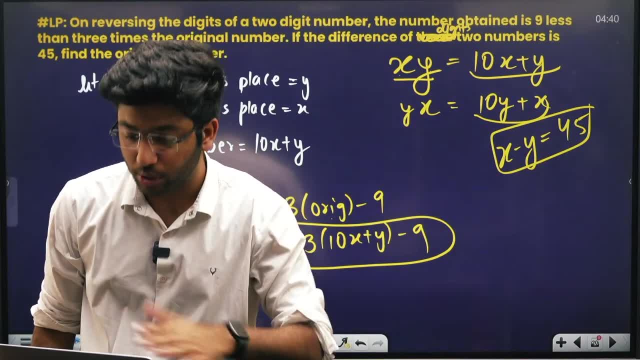 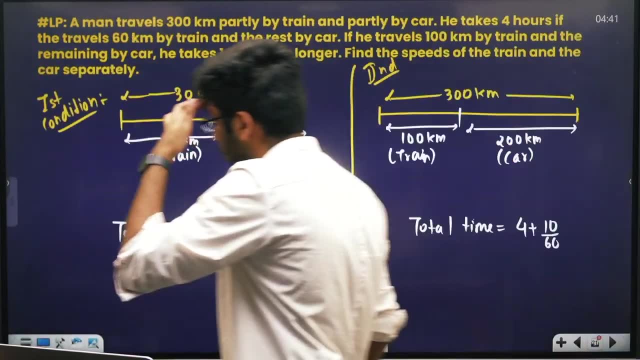 Okay, watching 140k. thank you so much. Did you understand? Did you understand? Did you understand. So we will do this question in this way. Next question: Whenever you have to take 2 digit number, take it Okay. 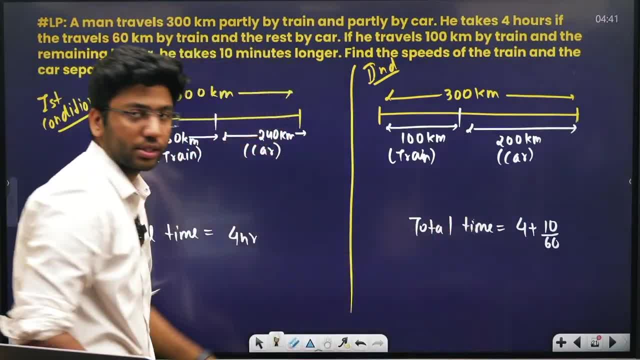 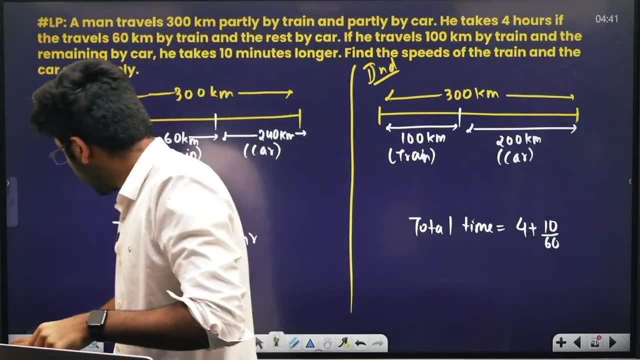 Next question: A man travels. This question is very famous. Two or three questions are very famous. Two or three questions are very famous. One question that I told you about 2 digit is famous. Right Before that, what did I do? 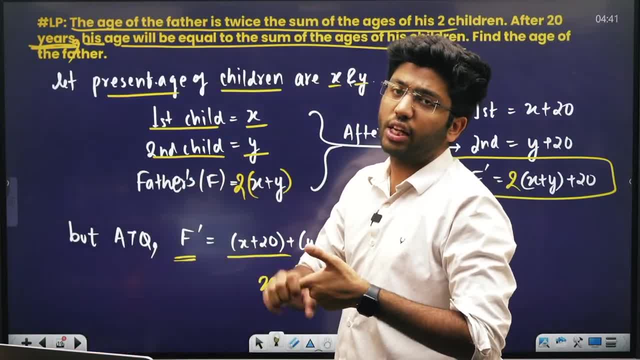 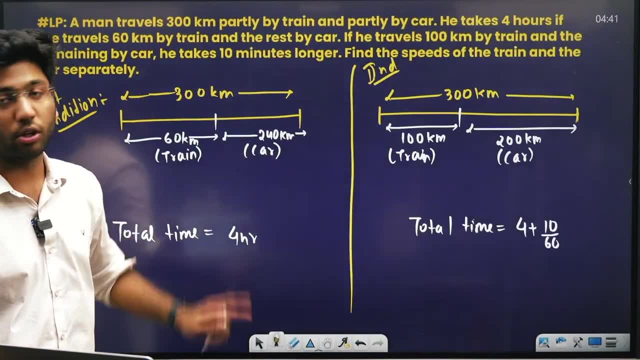 Before that I did this question, This age of father, age of son. this is very famous. And third, I am doing this airplane and train question. And I am doing this airplane and train question. This is very important. You are asked such questions. 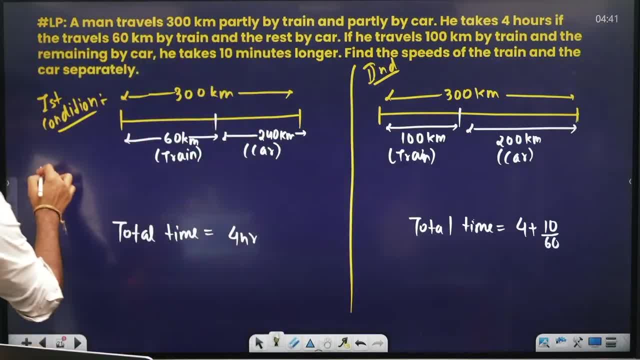 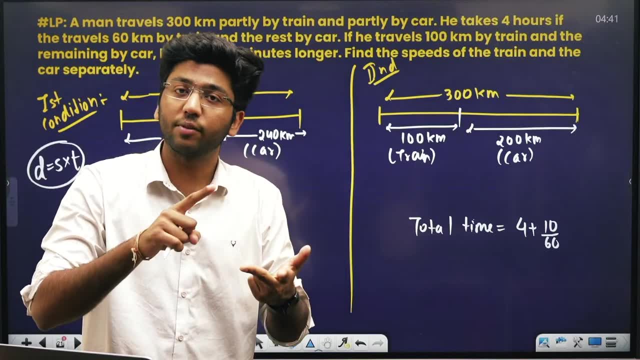 Distance equal to speed times. this is asked. You know this formula: distance equal to speed times. this is asked One. you will be asked this, Or you will be asked the age question, Or you will be asked the number question. 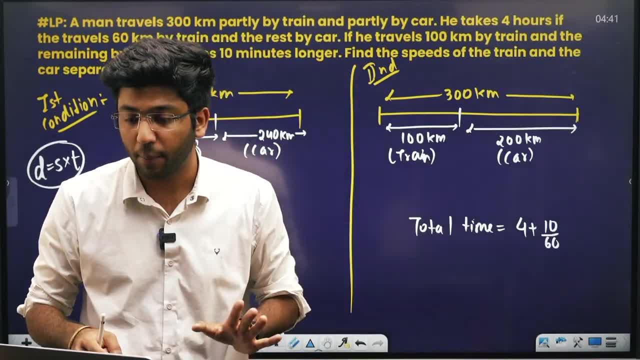 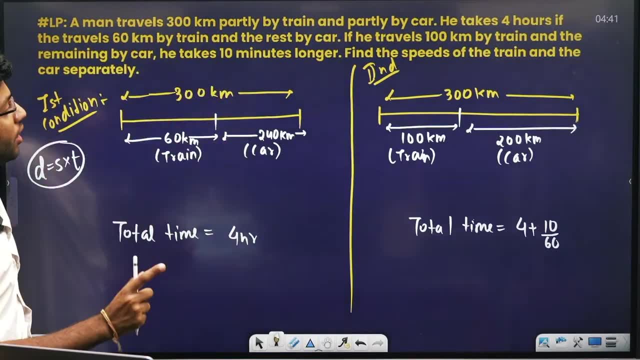 One of these three questions. One question will come for sure. One of these three questions will come for sure, Okay, Okay. So see, A man travels 300 kilometers. He is traveling 300 kilometers, total Some. he is traveling by train. 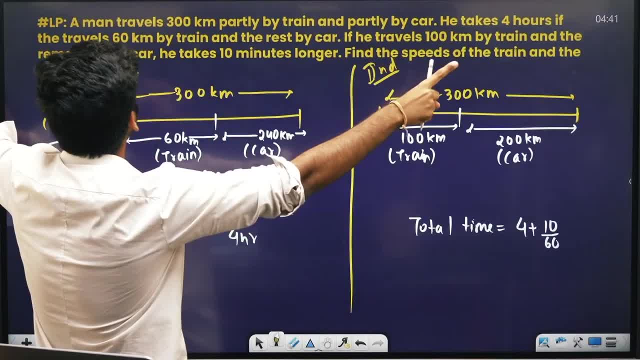 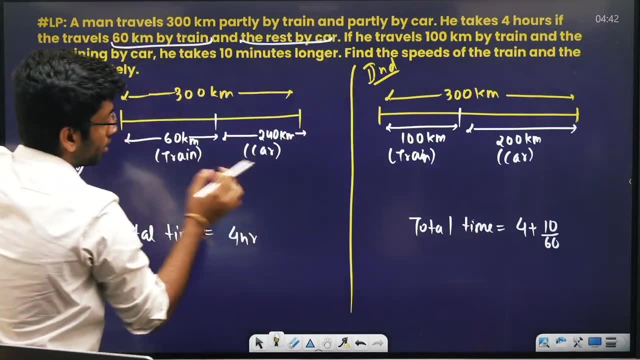 Some. he is traveling by car. He takes 4 hours if he travels 60 kilometers by train, So 60 kilometers by train, And rest by car, So 60 out of 300.. So 60 kilometers by train And 240 he did by car. 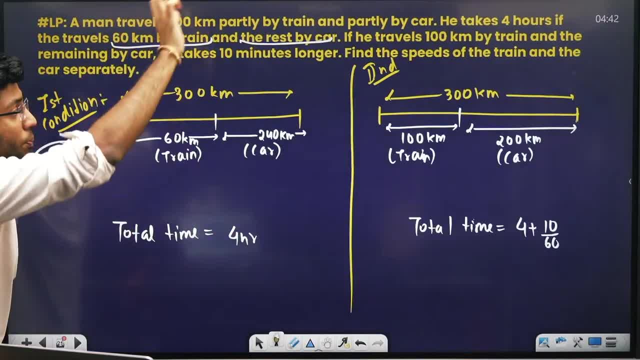 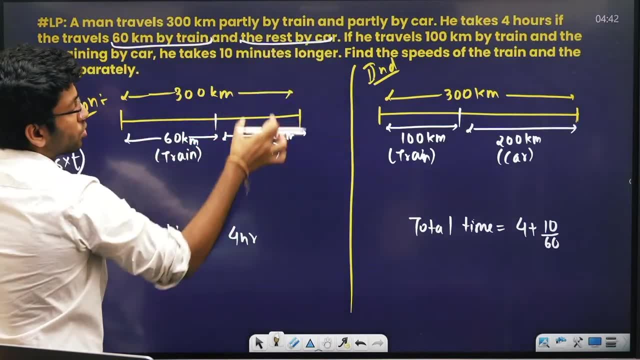 So it took him 4 hours. Listen carefully, Read the first line. What Total is 300 kilometers. Out of that, 60 kilometers he traveled by train And rest he traveled by car. So he takes 4 hours. He takes 4 hours if he is traveling like this. 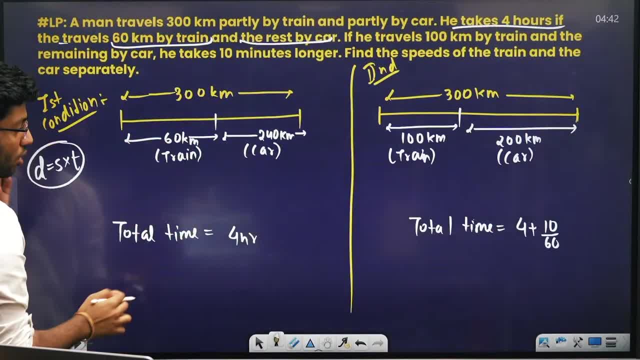 So total time is this much? So what will be the total time? What is equal time? If distance equal to speed is equal to time, So what will be equal time? Distance upon speed. So assume, So assume That train's speed. 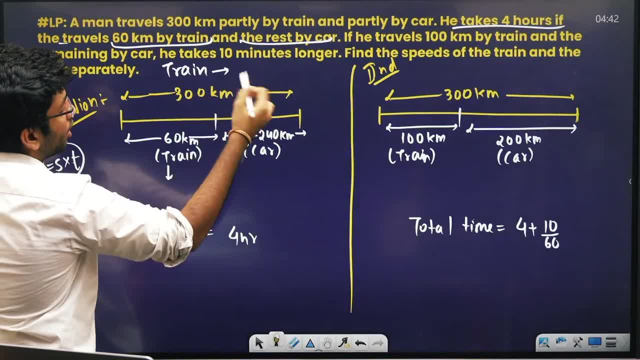 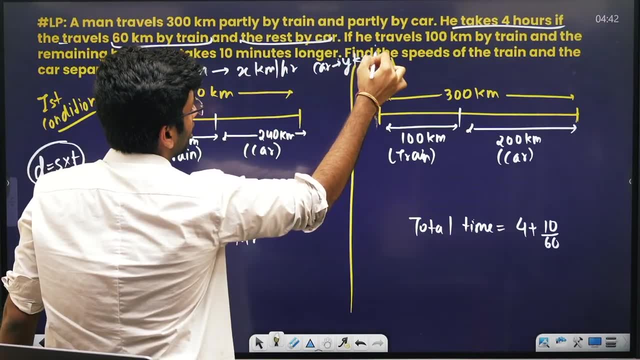 Assume that train's speed is coming at X kilometers per hour And car's speed is coming at Y kilometers per hour. So how much time will it take here? How much time will it take here? Distance upon speed, So 60 by X. 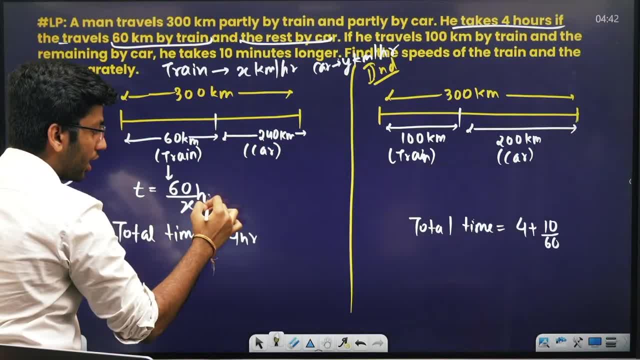 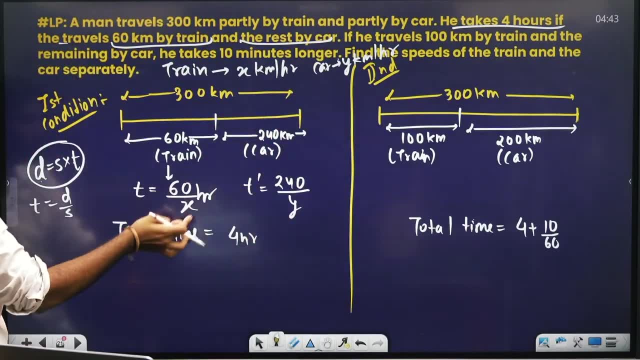 How much time will it take here? How much time will it take here And how much time will it take here? 240 divided by How much speed is there by car? Y So distance upon speed. This time came out Distance upon speed. 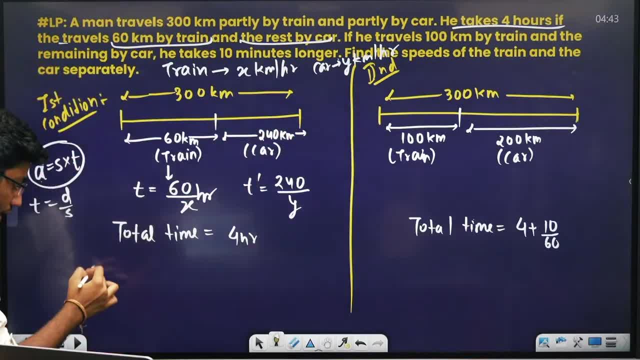 Time came out here, So here's time plus here's time Equal to 4 hours. So 60 by X. So 60 by X plus 240 by Y, This is given to us equal to 4.. This is the first equation. 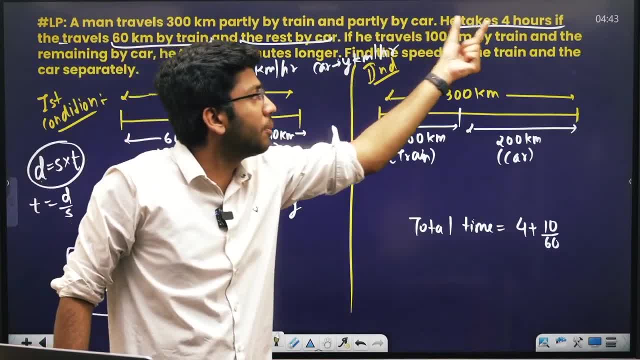 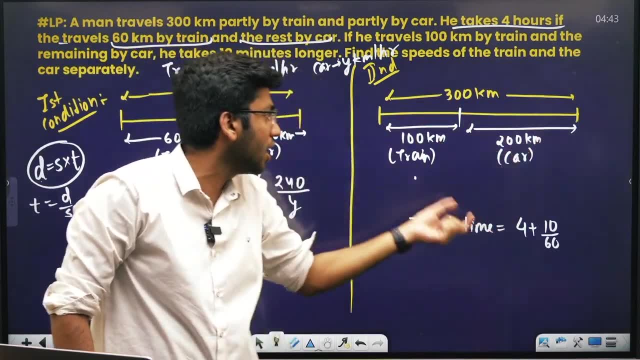 Next question: If he travels 100 kilometers by train, If he travels 100 kilometers by train And the remaining by car, So 100. If he goes from 300 to 100.. If he goes from 200 by car, If he goes from 100 by train, 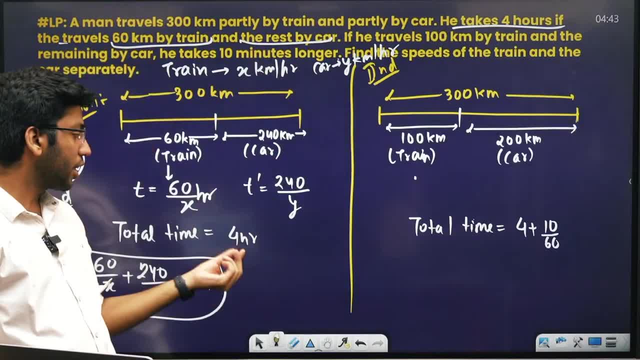 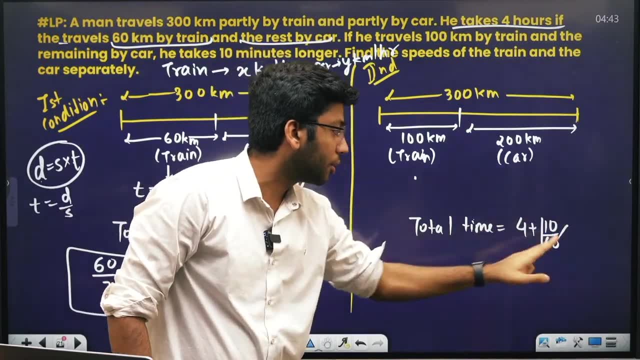 He takes 10 minutes longer, So earlier. if it used to take 4 hours, So now 4 plus 10 by 60.. What did I do? I converted minute into hour, So 10 by 60 is yours. 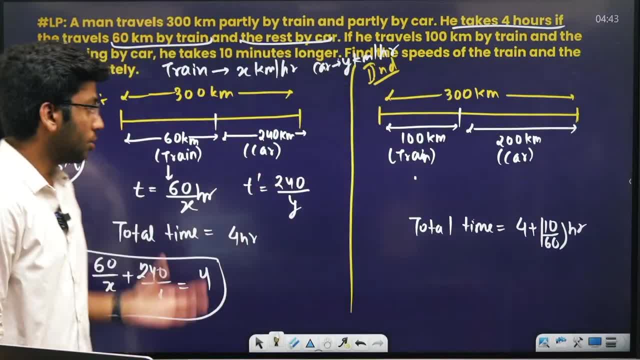 10 by 60. This is mine, So when he used to do this much, So it used to take 4 hours. So here's time, and here's time Equal to 4 hours When he is doing like this. So what will be the time here? 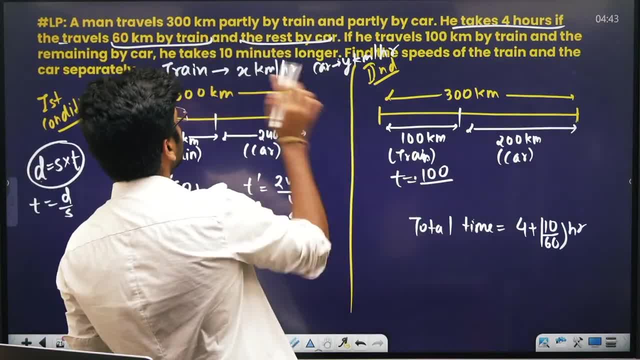 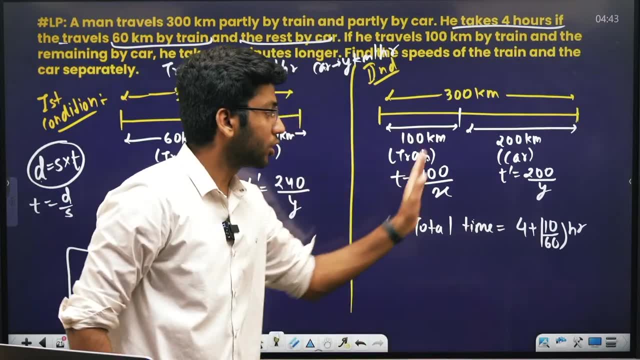 What will be the time here? 100 by What is the speed of the train X, And here's time will be T dash J, That will be 200 by What is the speed of the car Y. So now, what is the total time? 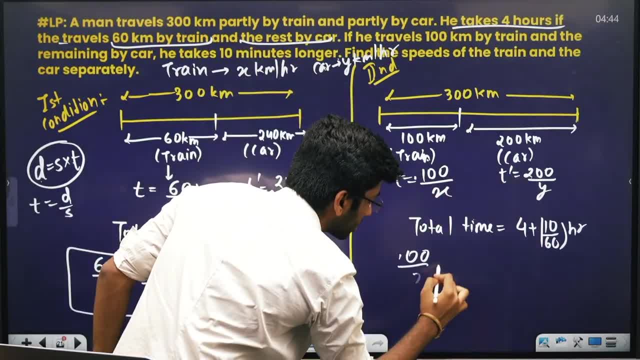 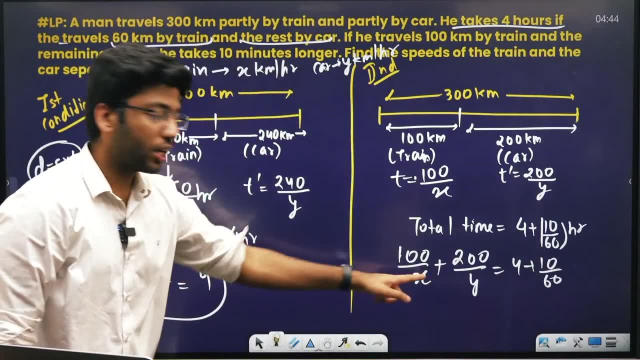 So total time means This plus this. So 100 by X Plus 200 by Y, This will be 4 plus 10 by 60. And 1 minus 2 dash Y. See all these things countries. 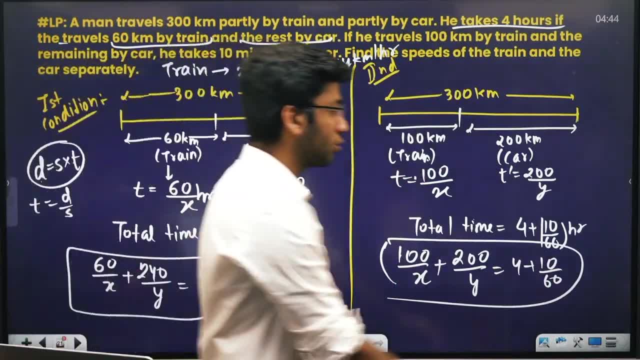 So now you have worked out The same, the 2 term Times that you have drawings In this language, Like this number, You realize exactly It's not easy, right? And then you see the total time here. Let's see what is the time. 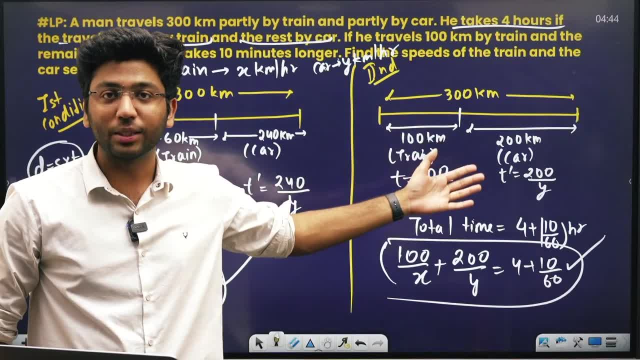 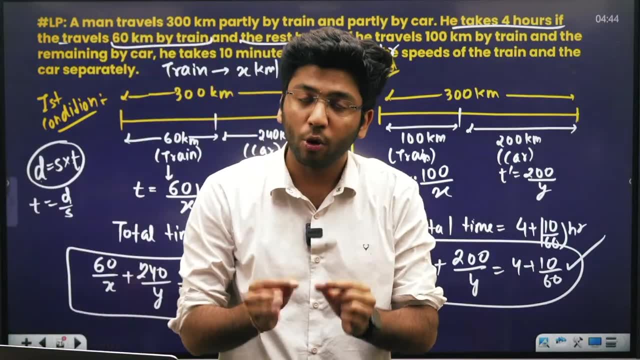 Let me just try this Now. every time I am going to try this, This is how shape work. That means One Time loop go. That means Evolution just fades away. But if I thought that I was just taking一. 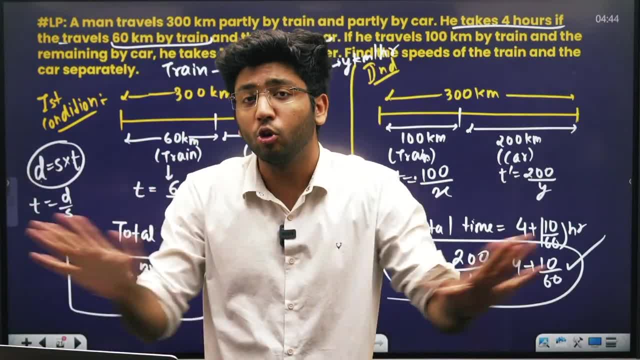 thought that Time loop through these rules. But if I thought that, Then you will see That the time loop in all these systems It was applied to, That it didn't break. Read one line and write. Read one line and make a diagram. 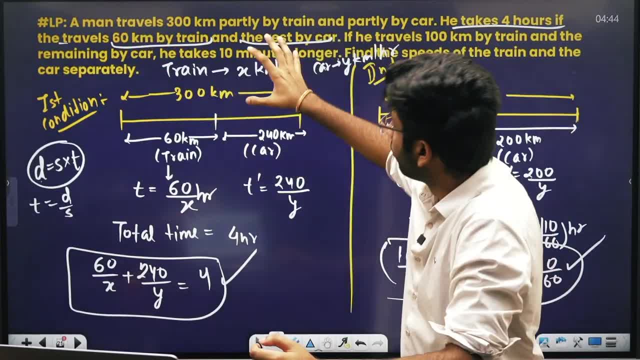 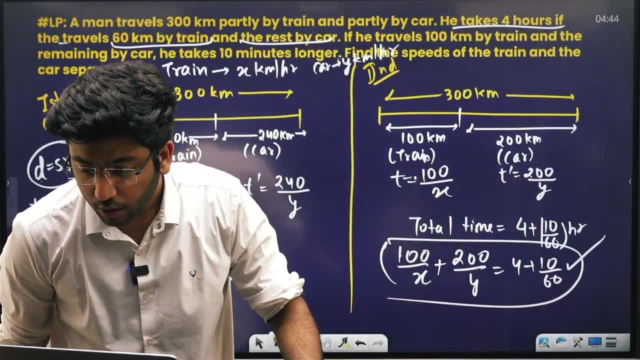 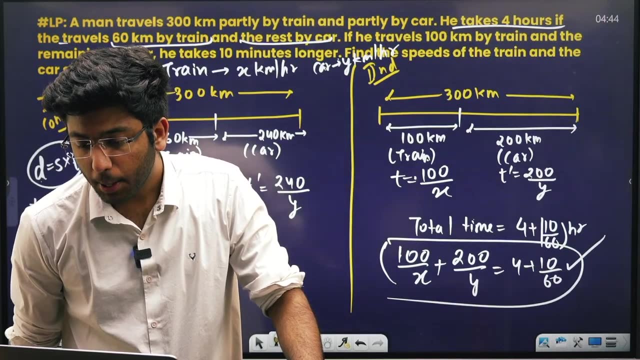 I did the same thing: Read the first line and made a diagram, Then solved it accordingly. Then read the second line and made a diagram and solved it accordingly. The answer is here. Okay, Okay, Did you understand? Did you understand? 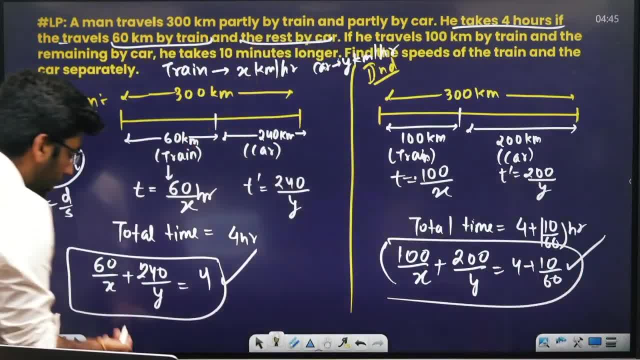 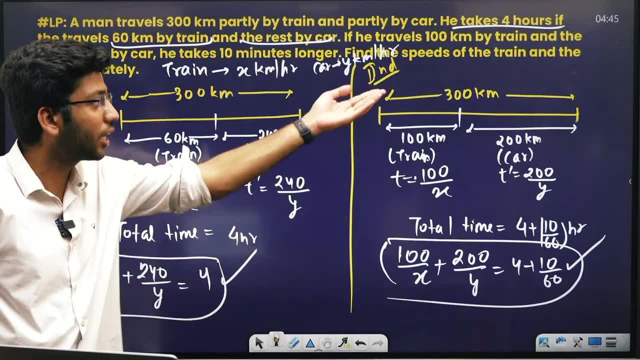 How do we solve? You don't have to do anything to solve From here. the common will be cut. It will be cut from 4.. x plus y. I will teach you to solve by taking LCM. Then the whole time will be spent. 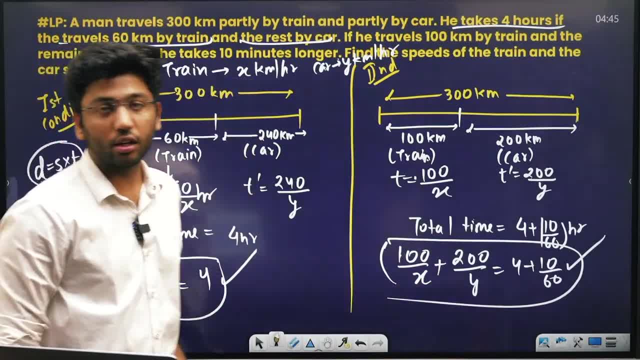 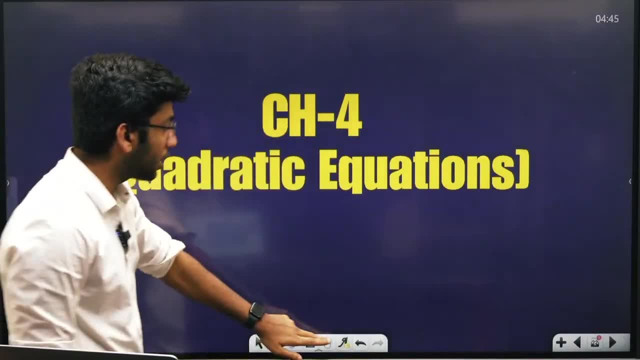 You will solve the question further. One equation is being made, Solving it is very easy. You have to find the value of x and y. These are linear equations. The fourth chapter. The fourth chapter is your quadratic equation. The fourth chapter is your quadratic equation. 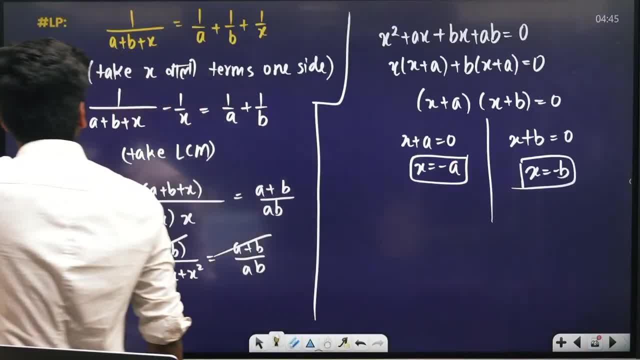 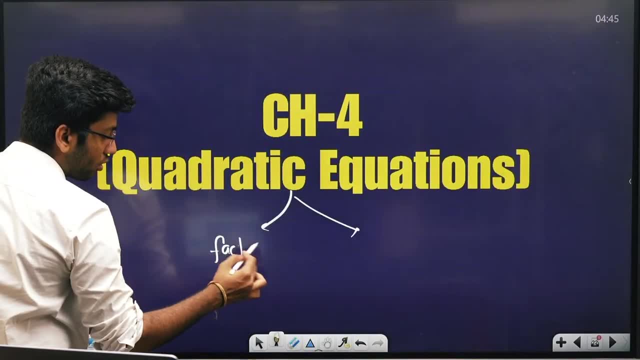 In the quadratic equation. the main thing, the main thing, you should know What Two One, you should know how to solve by factorization, Meaning splitting the middle term. Splitting the middle term, You should know how to do it. You write the middle term. 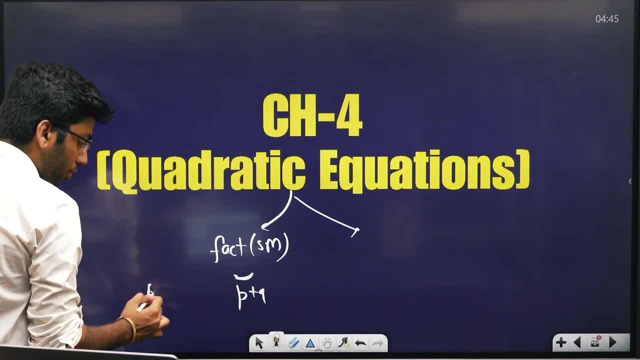 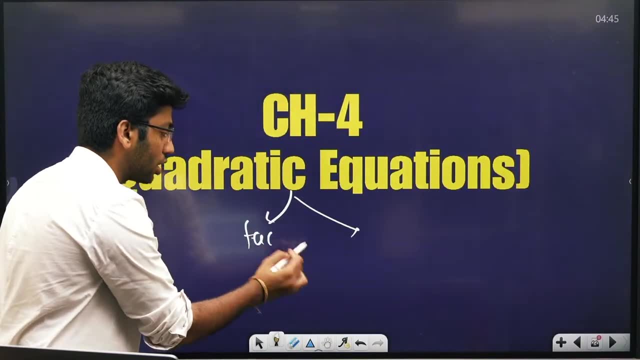 in two such numbers, whose sum will be this And the product will be equal to a into c. I told you this: One is your factorization method And the other is the discriminant method, In that the value of x is minus b plus minus square root of. 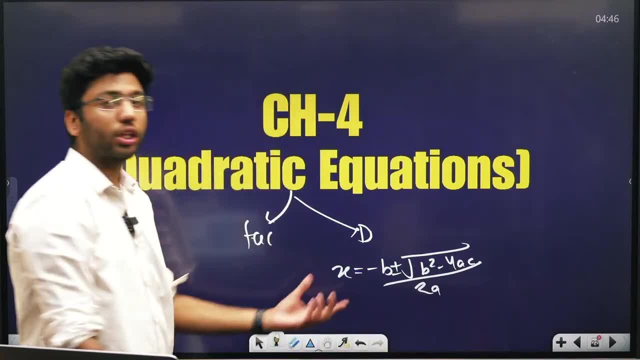 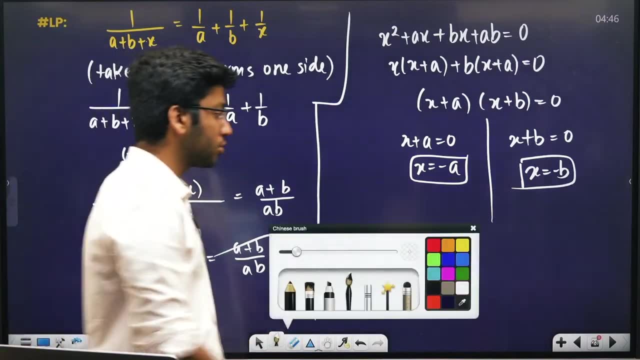 b square minus 4ac by 2a. So in these two ways you can solve the quadratic equation. A CBC asks a very nice question. It is this. A CBC asks a very nice question. It is this: There is a way to solve it. 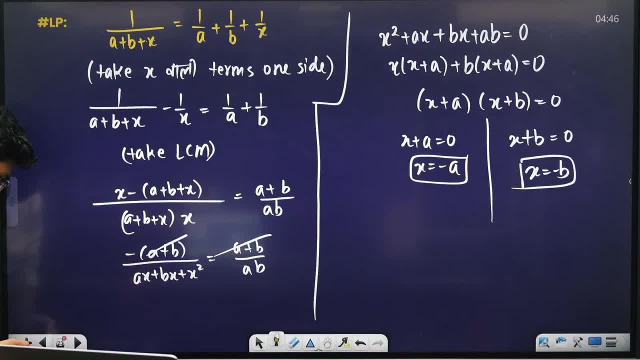 Whenever you see a question like this- I am saying it again- Like this: How will you solve it? You will take the LCM. Whenever you see a question like this, your job will be to take the LCM. Your job will be to take the LCM. 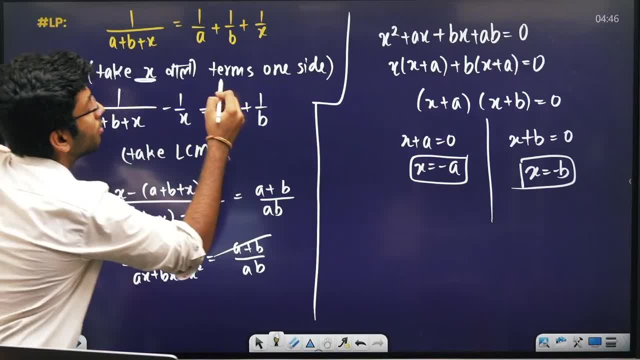 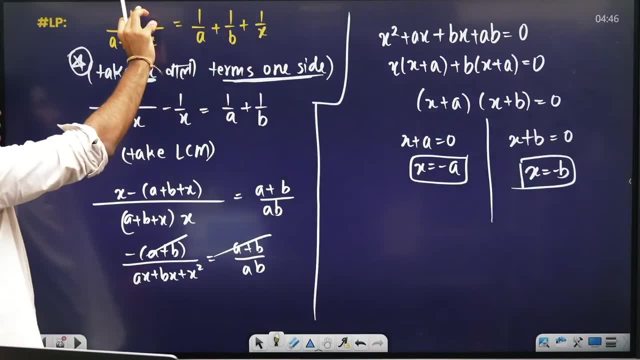 But when you take the LCM, when the term of x is divided- This is the most important thing in this- Here is x and here is x. So first take this x here, First take this x with this, Take it with this and now take the LCM. 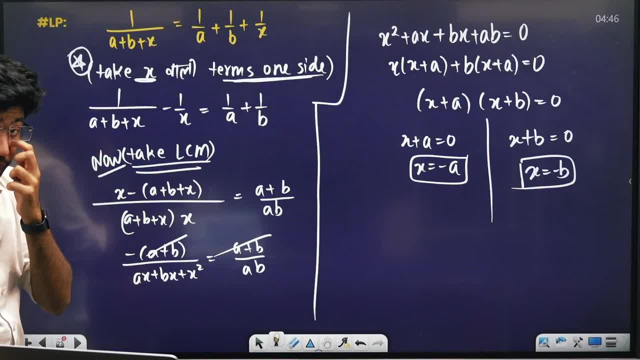 Now take LCM, Did you understand? Take the ones with x together In 1 upon a plus b, plus x was here and this x was here. I said, let's take this x here too. Now I will take the LCM. 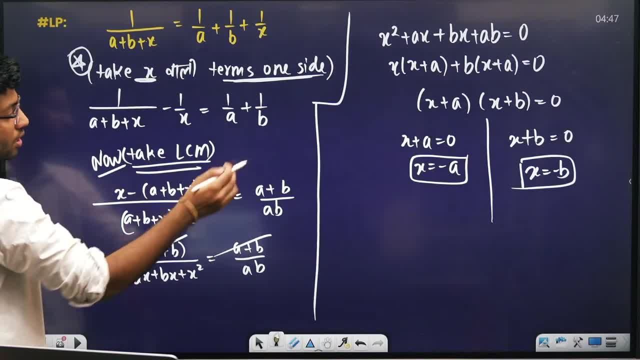 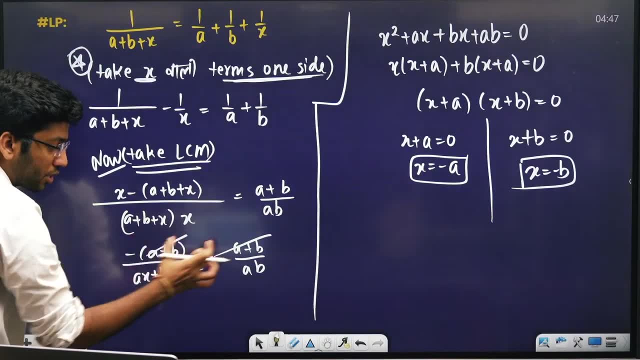 It will be like this And it will be x minus this. If I take the LCM here, then a plus b. When this minus goes inside, it will be cut and a plus b will come out. a plus b will be cut from a plus b. 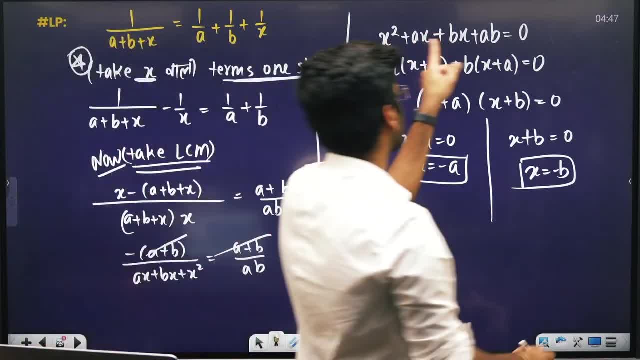 Then what will you do? You will cross, multiply, Cross, multiply and something like this will happen: x square plus ax plus bx plus ab. From here: if you take x, then x plus a. From here, if you take b, then x plus a. 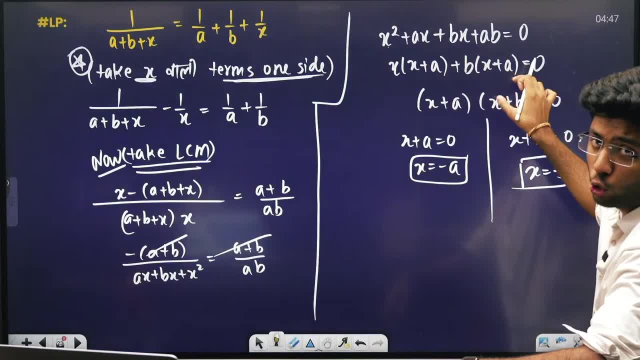 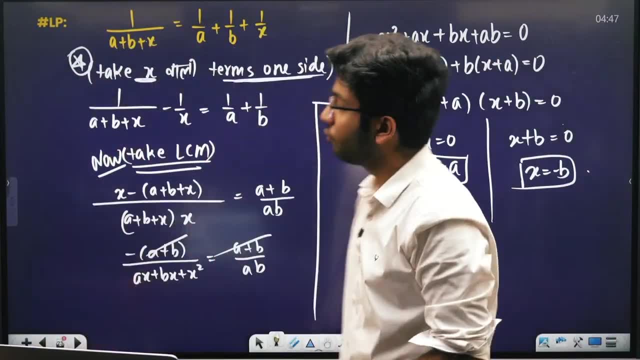 So x plus a came out, x plus a into, x plus b is 0. If the product of two things is 0, then this is also 0 and this is also 0.. The answer is here. Okay, The only thing is this. 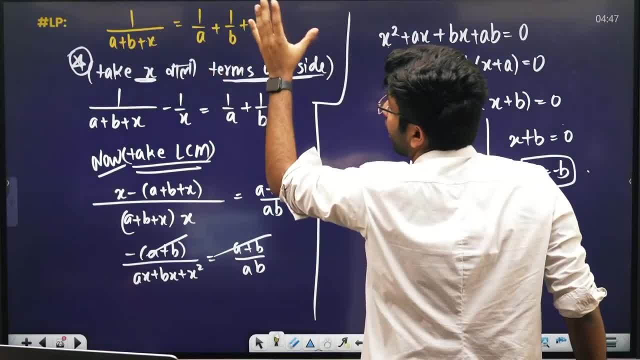 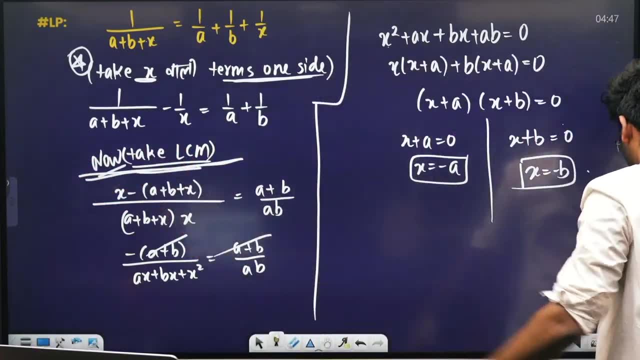 Take the product of x here. Take the product of x together. Whenever x will come out like this, Equal to will be seen on different sides. So take one side and then take LCM. Now take LCM, This is important. After that you have to solve. 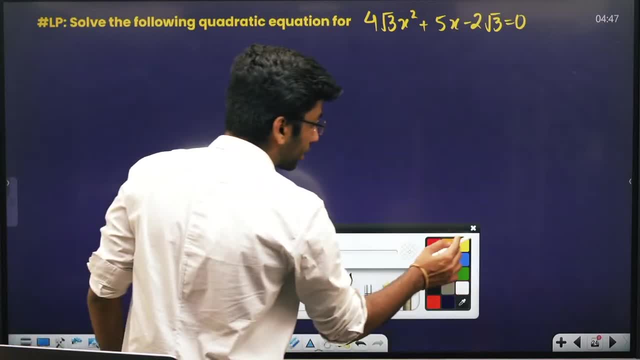 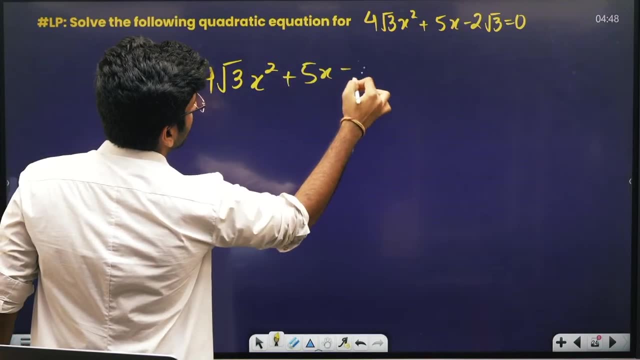 Solve the following quadratic equation. Now I will tell you how to do middle term splitting. Children are scared of the root question, But it is very easy: 4 root 3, x square plus 5x minus 2 root 3 equal to 0.. You have to solve this. 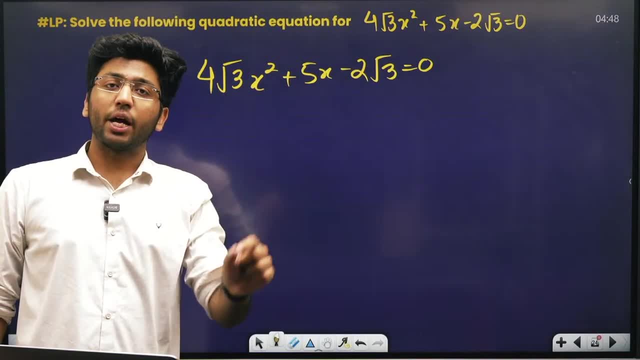 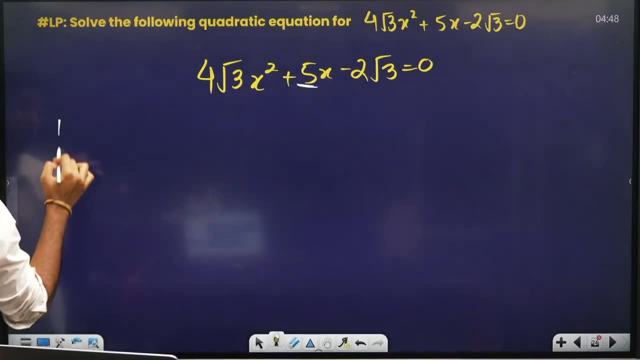 The root question at maximum time will be from splitting the middle term. You will say that it is very difficult. I will say that it is very easy. Why See you have to break 5 in such two numbers? Whose sum is 5.. 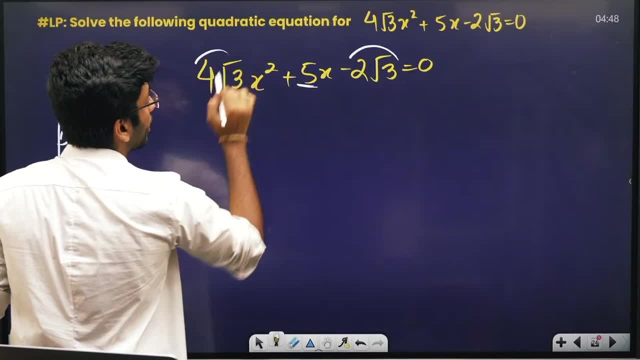 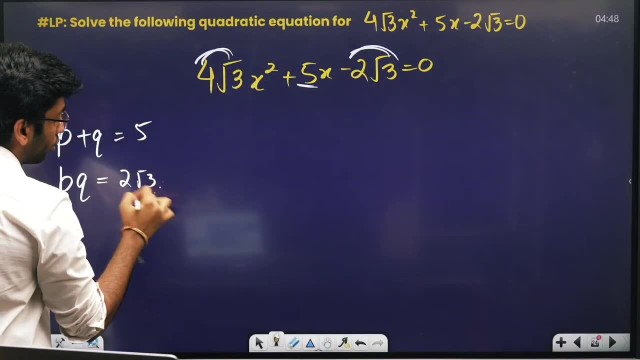 And what comes after product. This x. this Means this x. this Means 2 root, 3 x, 4 root, 3.. 2 root, 3 x, 4 root 3.. What is this? 2 root, 3 x, 4 root, 3.. 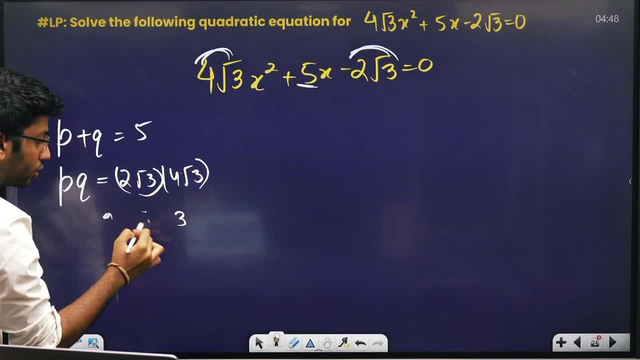 2 root: 3 x 4 root 3.. 3 root: 3 x 4 root. 3 is 8.. 8 x 3 is 24.. I need 24.. How will I do that? Tell me, how will I do that? 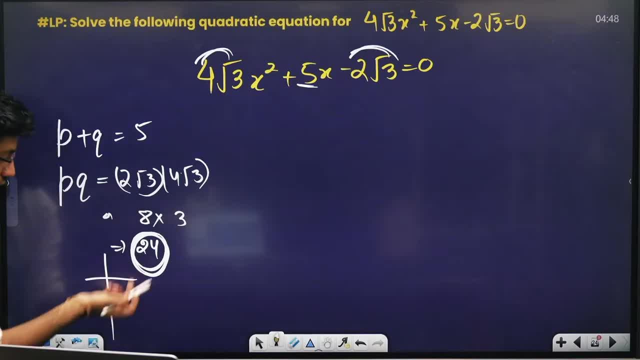 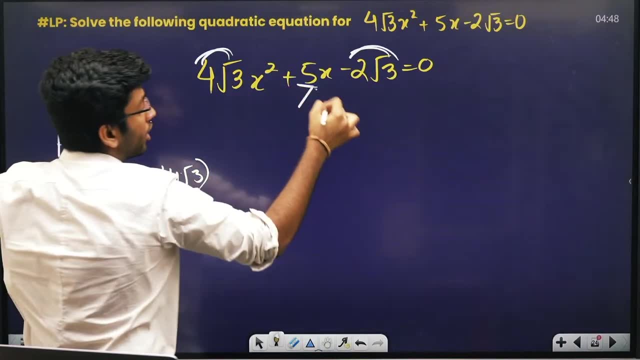 How will I do that? What factors can be of 24? 8 x 3 is 24.. If I subtract 8 x 3 from 3? 8 x 3 and minus 3.. If I write 5 as 8x, 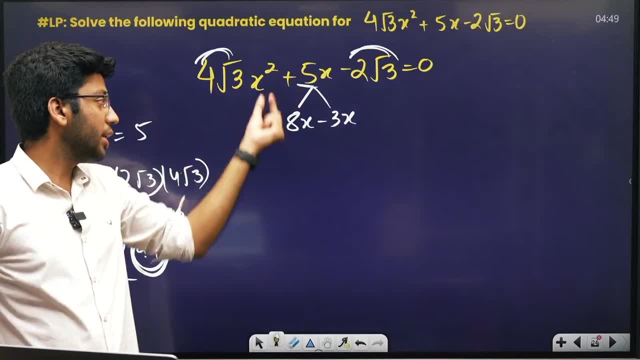 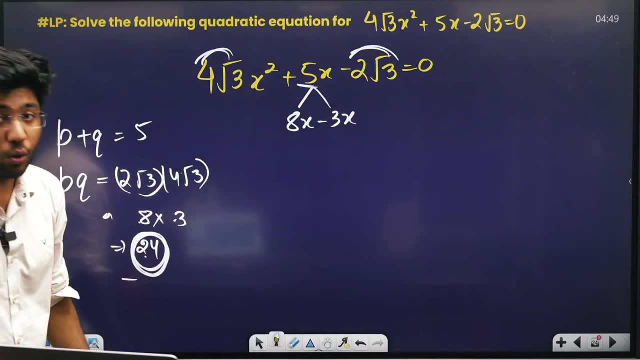 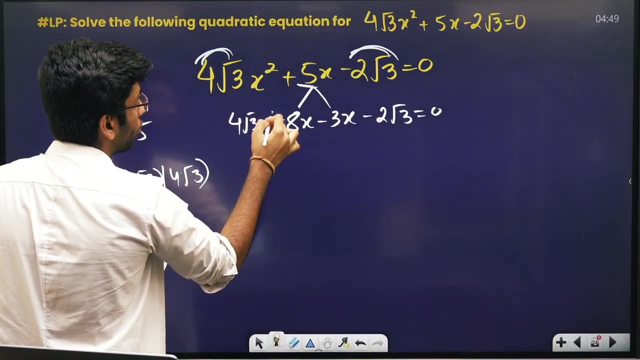 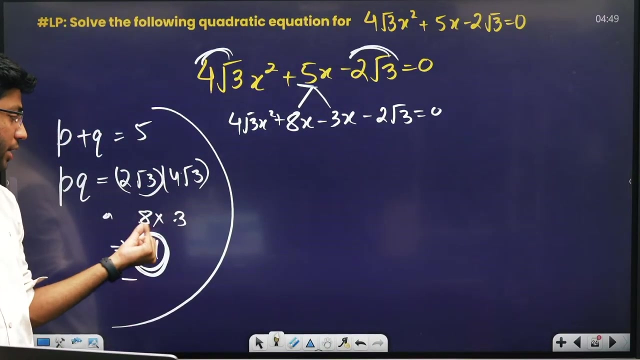 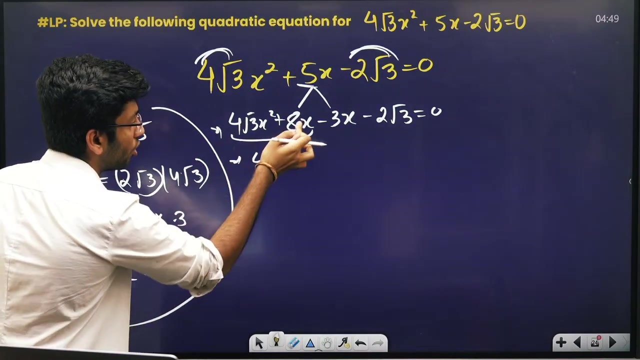 Minus 3x. How can I write that? I have written 5 as 8 x 3.. So I have written 5 as 8 x 3.. As soon as I wrote this, as soon as I wrote this, now what happened now? what happened? now? the question is solved. plus 4 root 3 x square. 4 root 3 x square is like this: minus 2 root 3 is like this: so you don't have to do anything in the root question, just multiply it. multiply it and you will see it yourself. you can see 8 and 3, so I broke it like this. now what will you do? take whatever is common. take common: 4x is common from here. 4 and x is common. take 4x common from here. root 3 plus 4, 2 is 8, root 3 plus 2,. 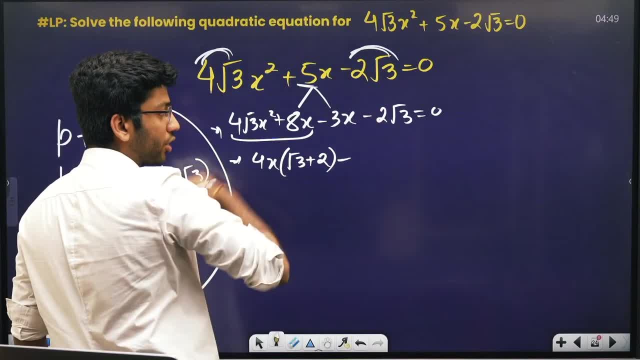 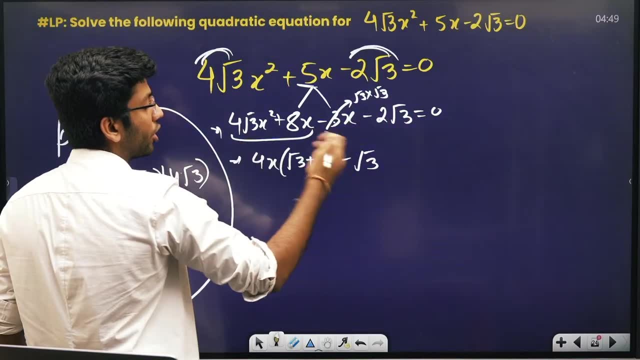 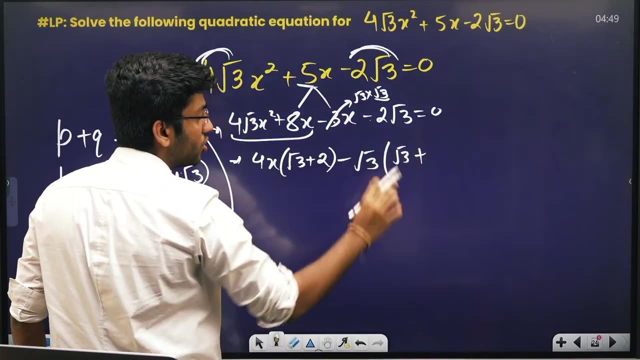 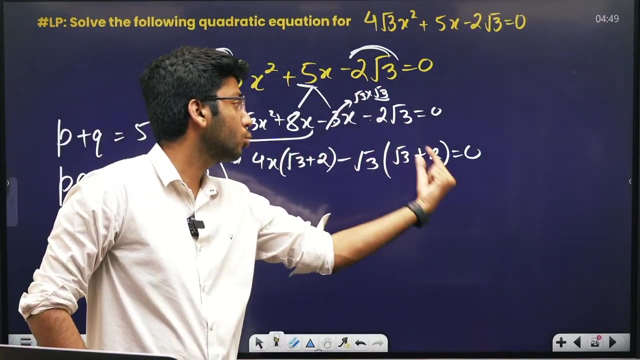 take 0 by 2, take minus common from here and in minus. if I take root 3 common, what can I write? 3, I can write root 3 into root 3, so I took 1 root 3 common. 1 root 3 common. what was left inside? 1 root 3 was left. 1 root 3 came out. 1 root 3 was left and if minus came out, then plus will be sign change and plus 2 equal to 0, so root 3 came out. 1 root 3 came out here, so root 3 came out. 1 root 3 was left here and 2 was left here. this sign change happened because minus is out. 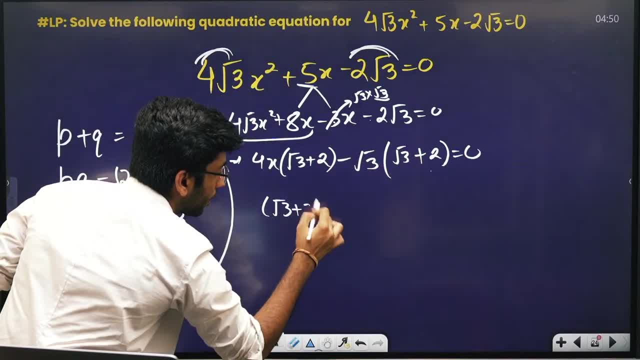 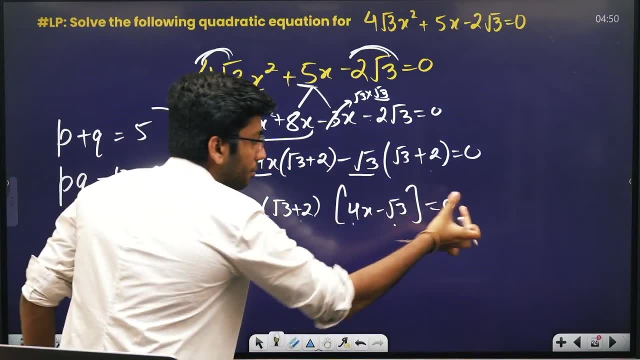 now see: in this whole equation, root 3 plus 2 is common. What's left inside 4x minus root 3, 4x minus root 3 is left. this is equal to 0.. So this into this is equal to 0.. The product of two things is 0. 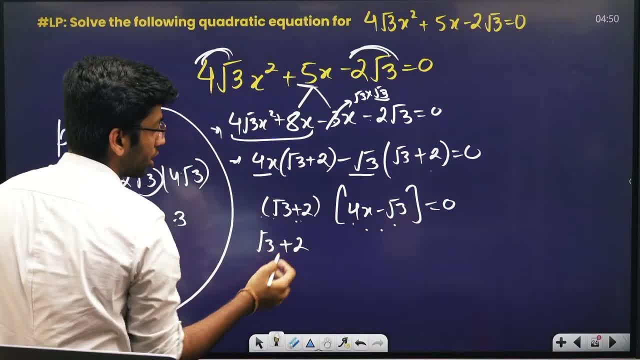 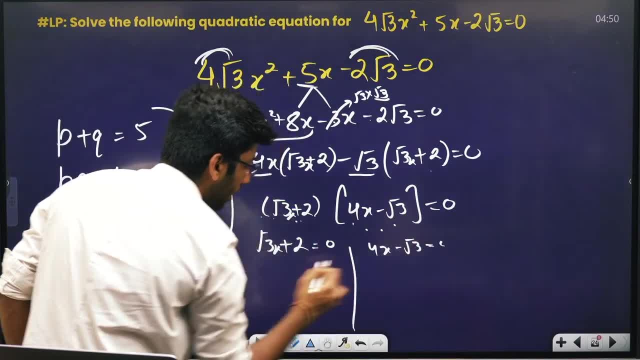 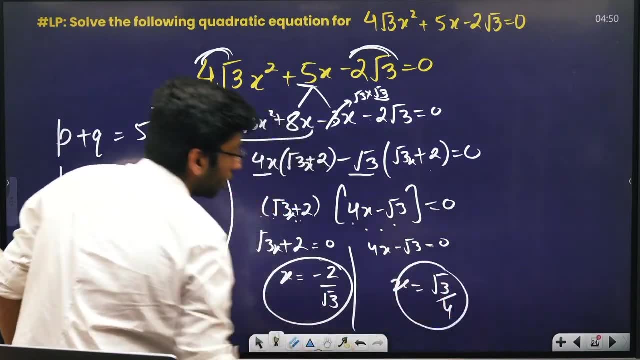 And 4x minus root 3 is equal to 0. So from here the value of x is minus 2 by root 3.. And from here the value of x is root 3 by 4.. So these two values are of x and this is the answer. 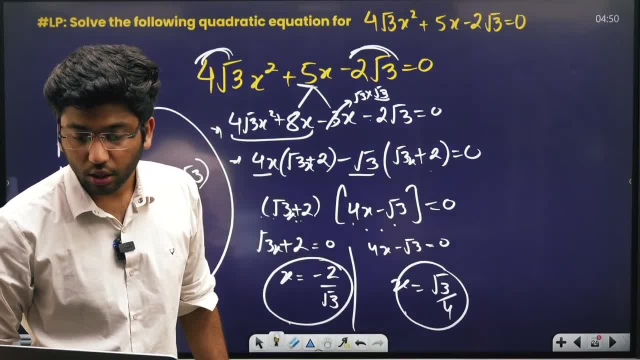 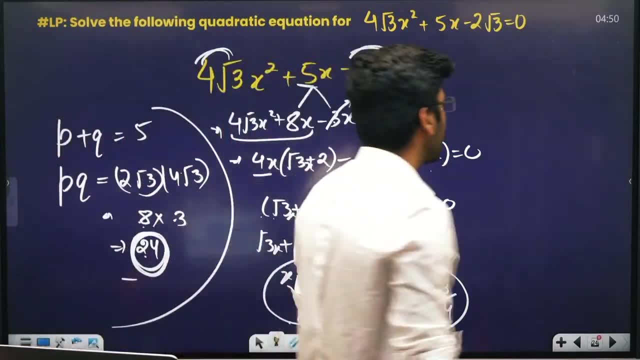 This is the answer, Okay. Okay, Did you understand? It was not wrong. I forgot to write x, so I wrote x. here I wrote x. it's done, Okay. So whenever you get this, then try to do it from splitting the middle term. 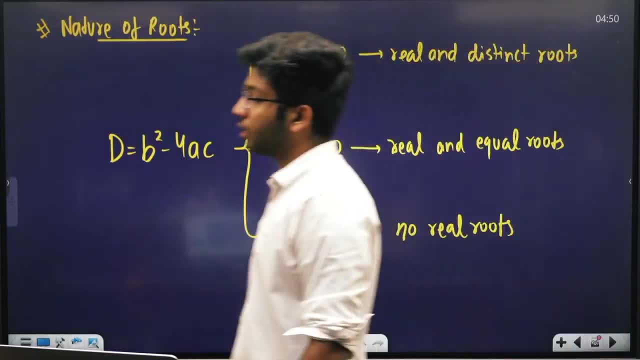 It will be easy. There are many chances of such root ones coming. The second type of question. the second type of question: the nature of roots. there will be a fixed question. Write it down. There is a fixed question from nature of roots. 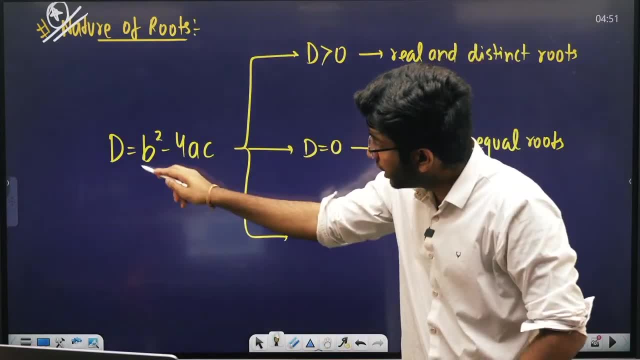 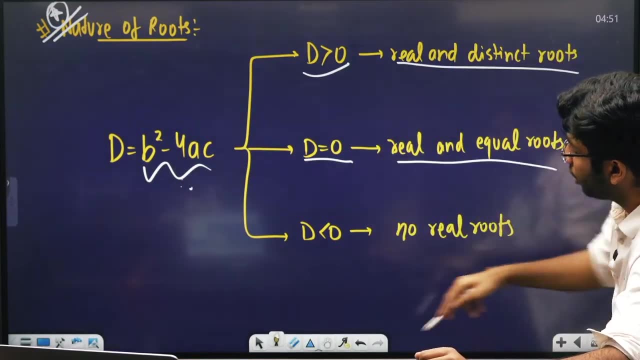 Write it down. How will we find the value of D? If D is positive, then it is real and distinct. If it is equal to 0,, then it is real and equal. If it is less than 0,, then there are no real roots. 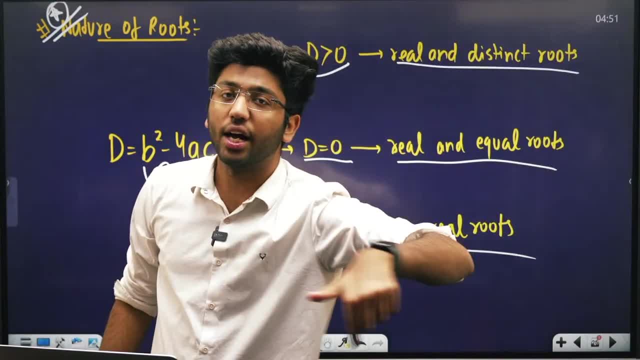 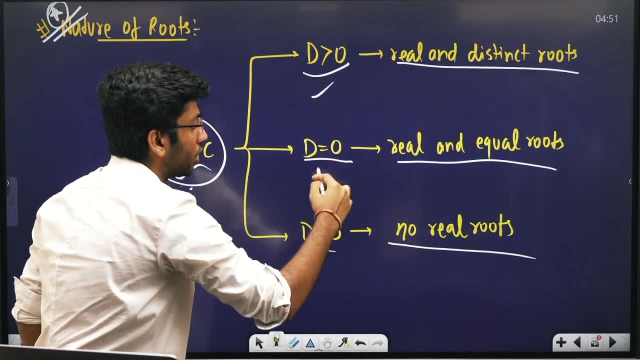 So, whenever you will be asked, tell me, how are the roots? Are they real, non-real or equal? How will you find it? You will find the value of D. If D is positive, then it is a real root. If it is equal to 0, then it is equal roots. 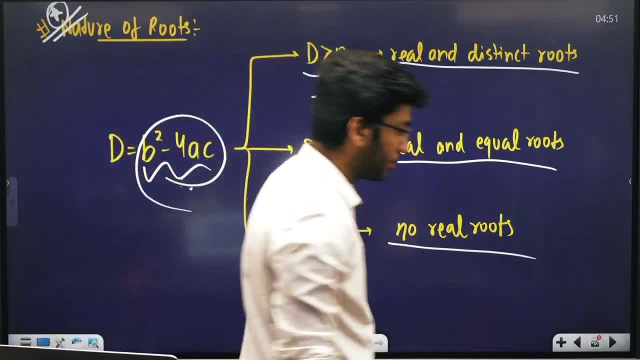 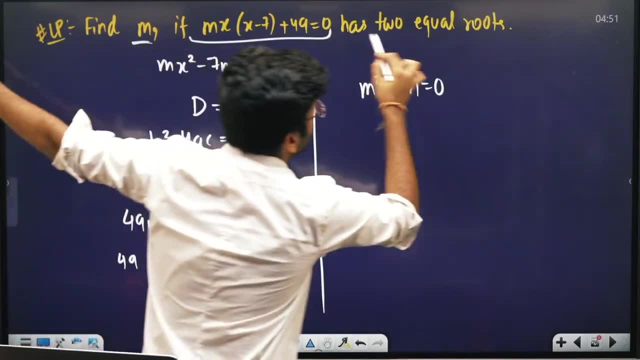 If it is less than 0, then there are no real roots. Did you understand? Did you understand Like I am talking to you? Find the value of M, for which this equation has two equal roots. So equal means: D is equal to 0.. 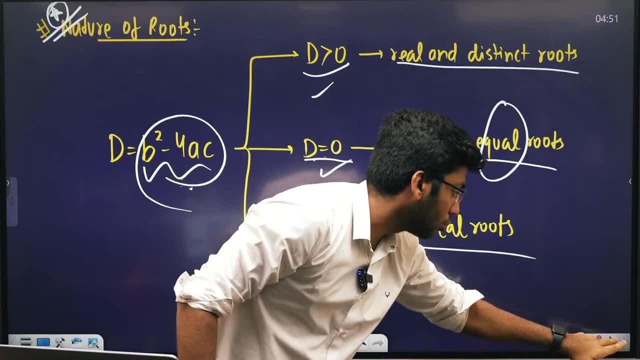 Equal roots means D is equal to 0.. So I will do D is equal to 0 and nothing else I will do. D is equal to 0.. The value of D. first I did it in MX. that is why I got X square. 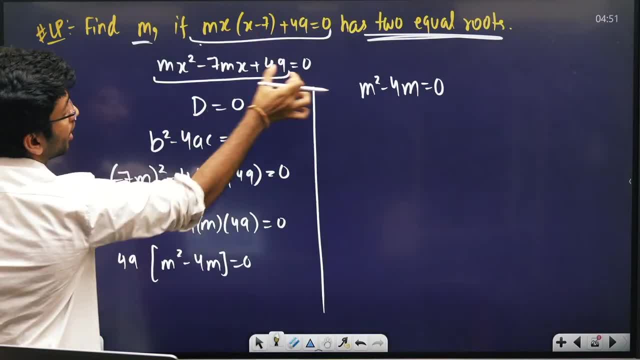 Because I will be able to apply it in the quadratic equation. So I multiplied it in MX and it became this: Now see, D is equal to 0, means B square minus 4 is equal to 0.. What is B square? What is B? 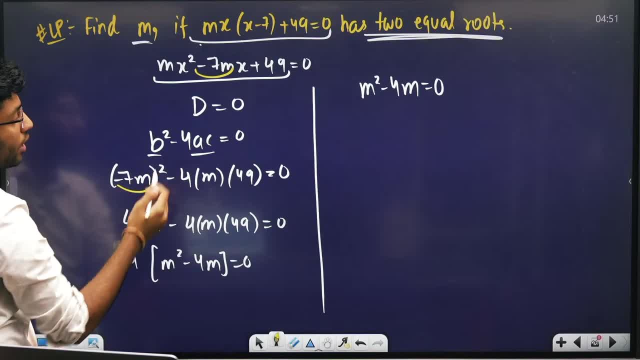 What is B? The coefficient of X is minus 7.. So the whole square is minus 7M Minus 4AC. So what is 4AC? What is A? The coefficient of X square is M. What is C? This is 49.. 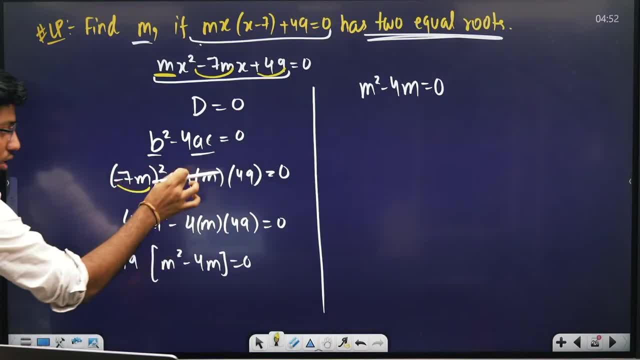 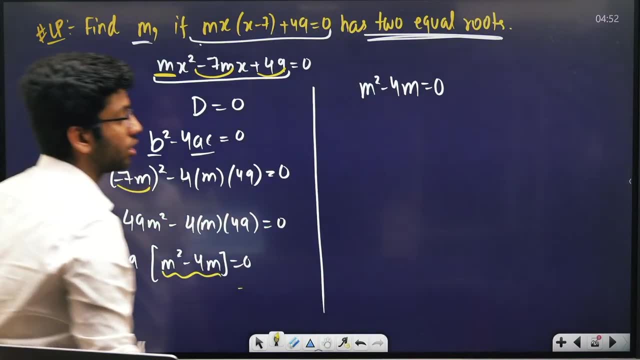 So I did it in this way: 7M square became 49M square. This became 4M into 49.. 49 came out completely. 49 will come out and go to 0.. So it remains M square minus 4M is equal to 0.. 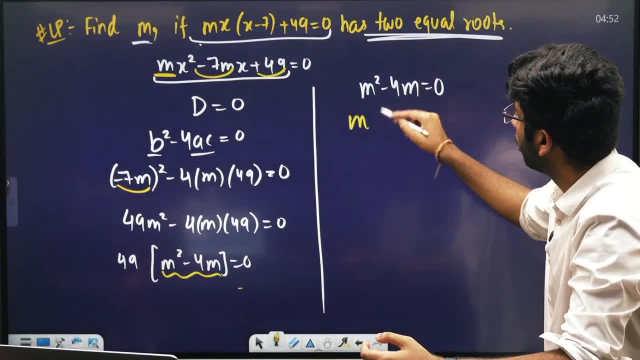 M square minus 4M is equal to 0.. Now take M common from this. What will be left inside? M minus 4 is equal to 0.. So the product of two things is 0.. The product of two things is 0.. 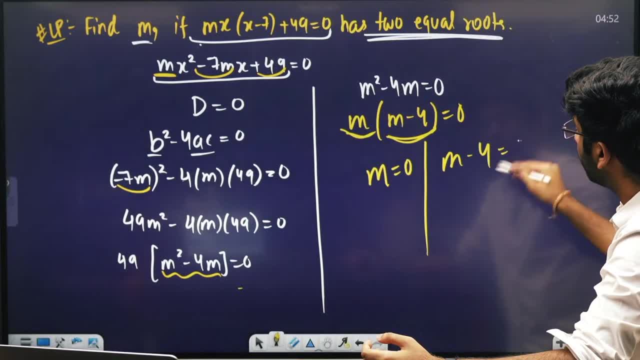 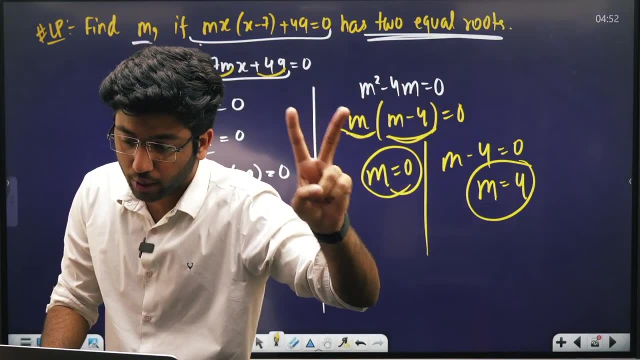 So either M is equal to 0 or M minus 4 is equal to 0.. Now m has two values: 1m equal to 4, 1 M equal to 0. both will be the answer. Both will be the answer of 4 and 0.. 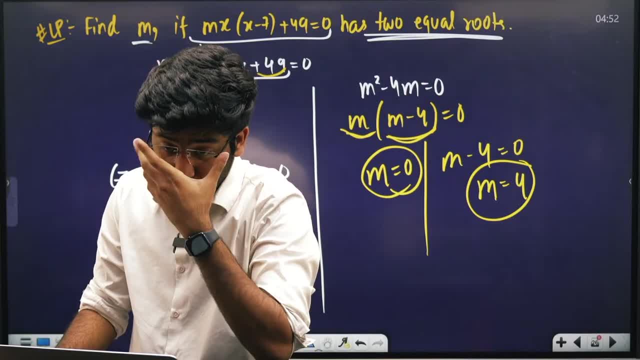 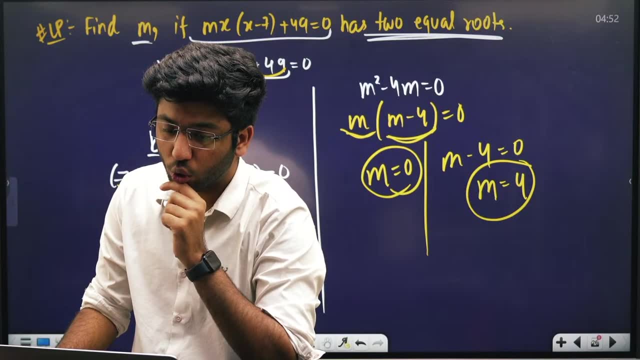 Both will be the answer of 4 and 0.. Both will be the answer of 4 and 0.. Tell me, will they or not? Will both answer be the answer of 4 and 0?? Two answers are coming. M's value is also 0, or is it 4?? 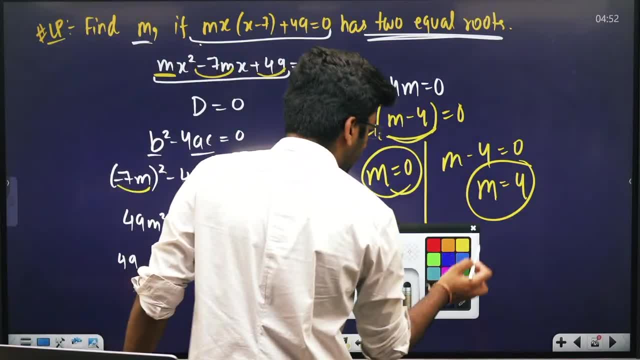 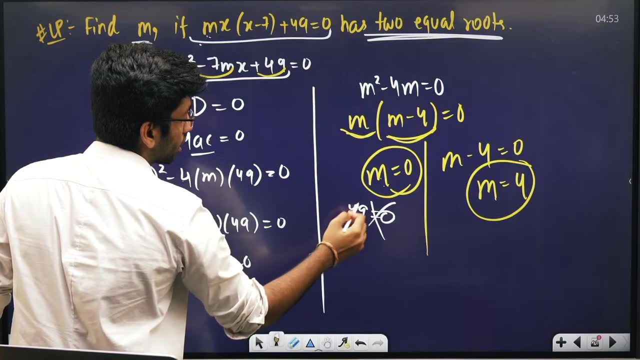 What will be the answer? Let's verify: If I put m equal to 0 in this, then 49 is equal to 0.. Is it possible or not? So the value of m is not 0.. If I put m equal to 0 here, then 49 is equal to 0.. 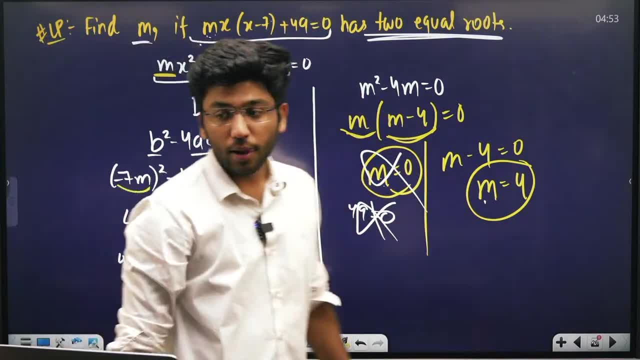 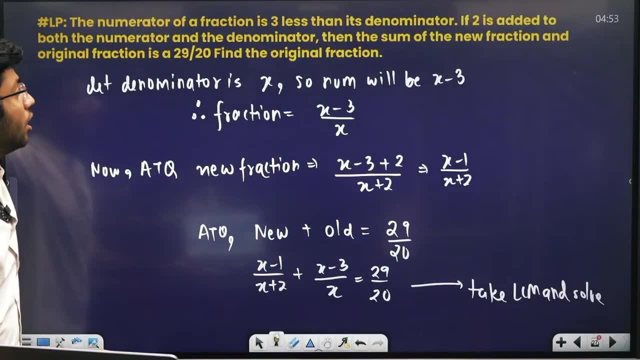 No, it is not possible. If I put m equal to 4, then it will be satisfied. If I put m equal to 4, then it will be satisfied. Next question: Numerator and denominator. Very important question. CBSE likes it a lot. 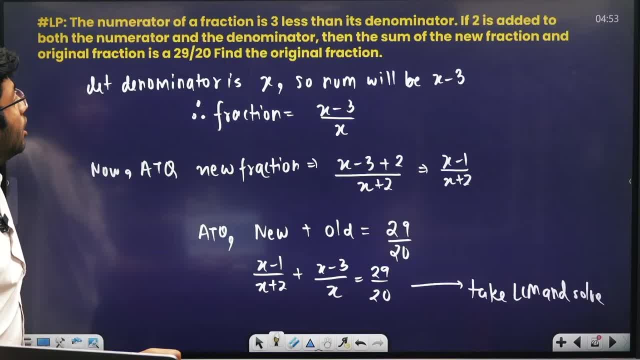 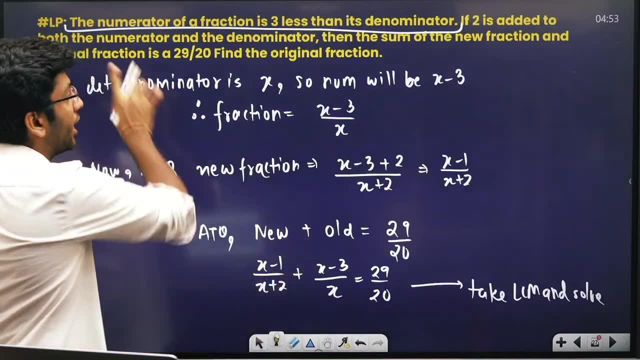 So look at the question of numerator and denominator. So numerator and fraction is 3 less than denominator. Read the first line and answer Whenever there is a big question. don't read the whole line. Read the first line. Numerator and fraction is 3 less than denominator. 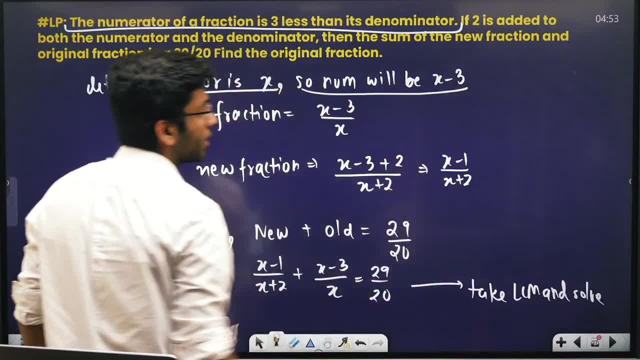 So if I consider denominator as x, then what will be the numerator? It will be x minus 3.. Understood What did I say? Numerator is 3 less than denominator. So if denominator is x, then what will be the numerator? It will be x minus 3.. 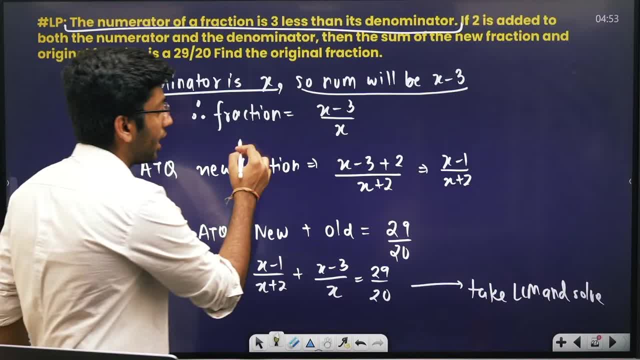 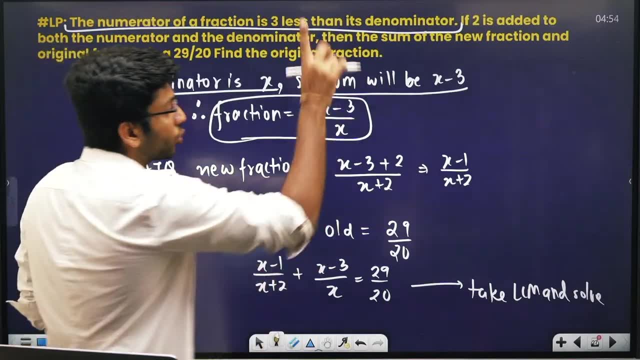 So what will be the fraction? It will be x minus 3 upon x. It will be this: If denominator is x, then numerator is x minus 3.. It will be this fraction If 2 is added to both numerator and denominator. 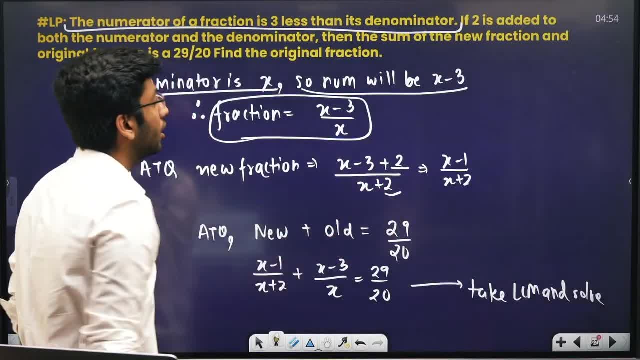 If numerator is 2, then it will be 2.. If denominator is 2,, then it will be 2.. So if you add 2, it will be this. So this is the new fraction and this is the old fraction. 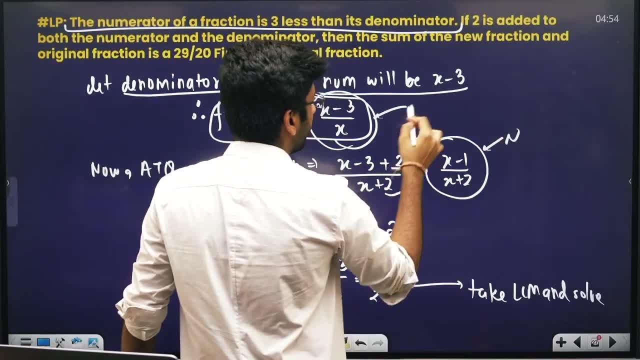 What is this? This is our new fraction and this is our old fraction. Okay, Look, there was a comma, so I read it before the comma. Whenever you read, read in parts. Whenever you read a question, read it in parts. 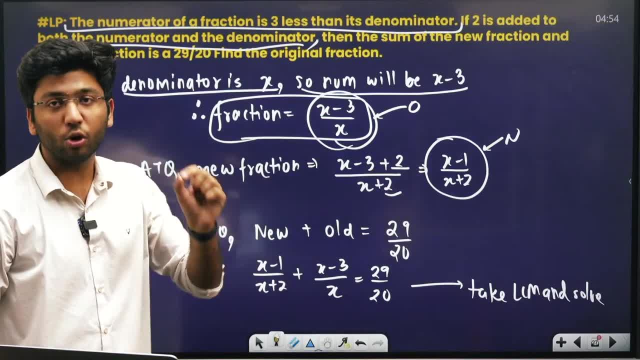 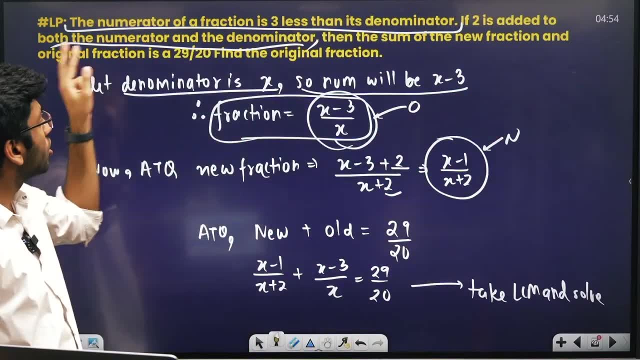 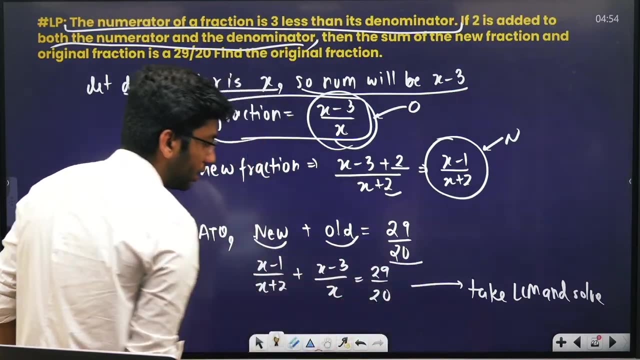 Keep this in your mind: Whenever you read a question, read it in parts. So what did I do? I read the one before the comma. Then the sum of new fraction and the original fraction is 29 by 20.. So the sum of new and original is 29 by 20.. 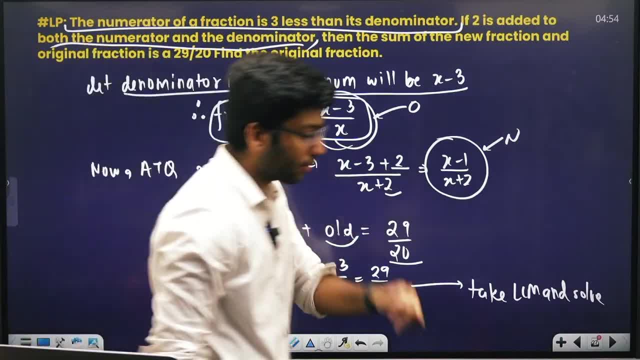 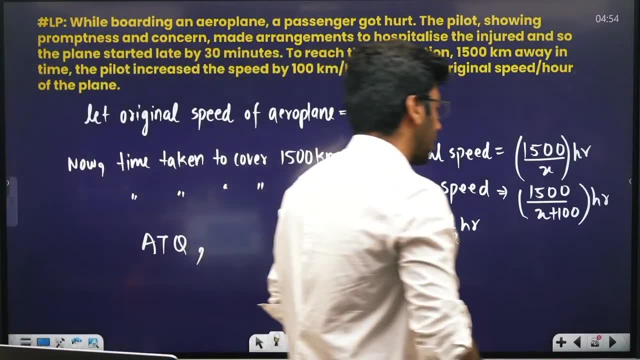 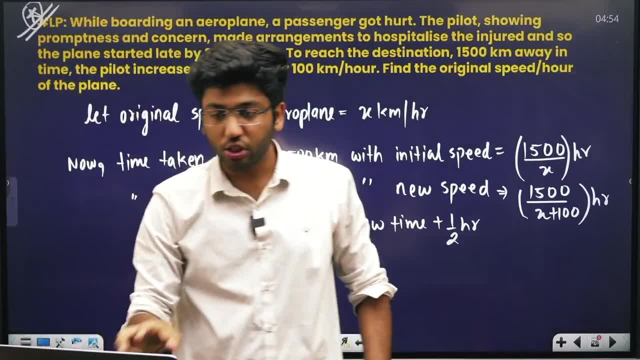 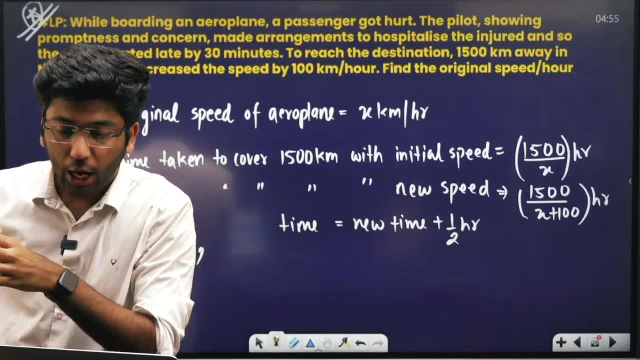 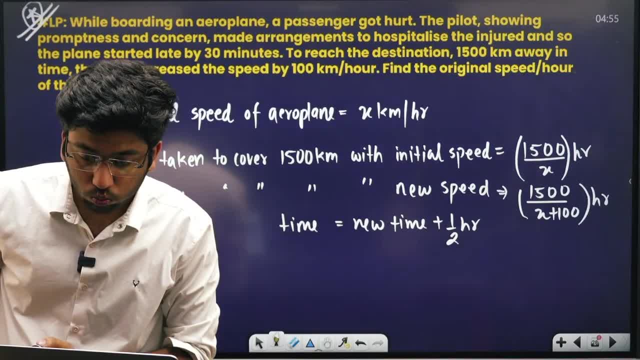 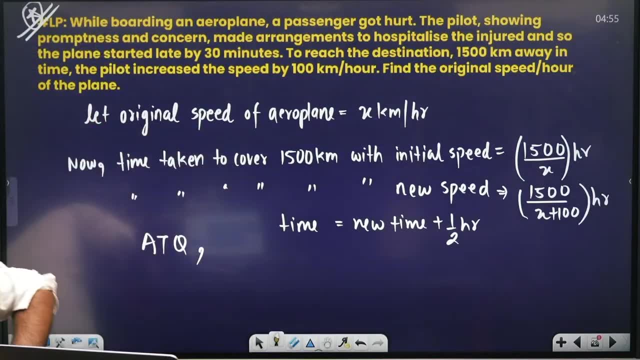 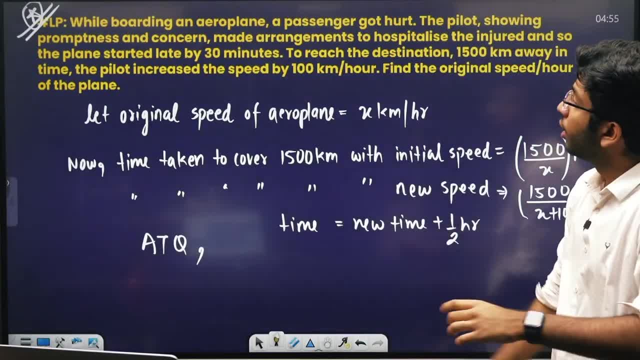 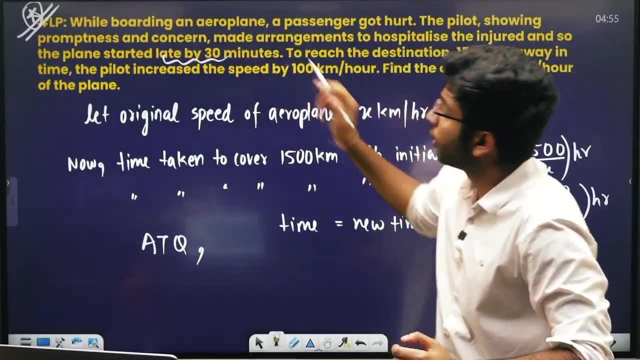 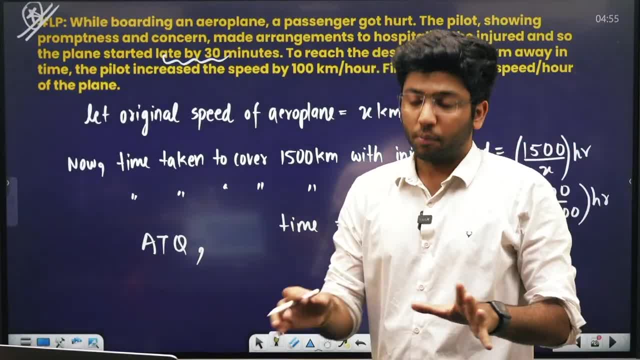 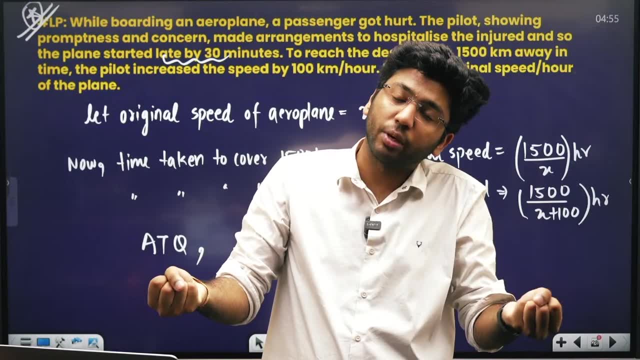 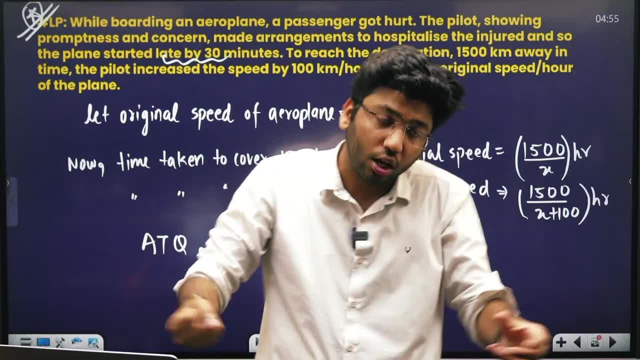 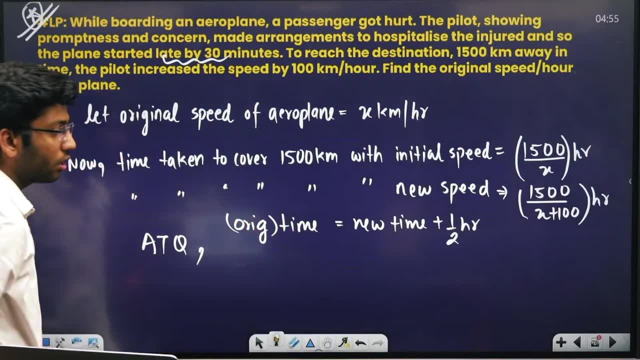 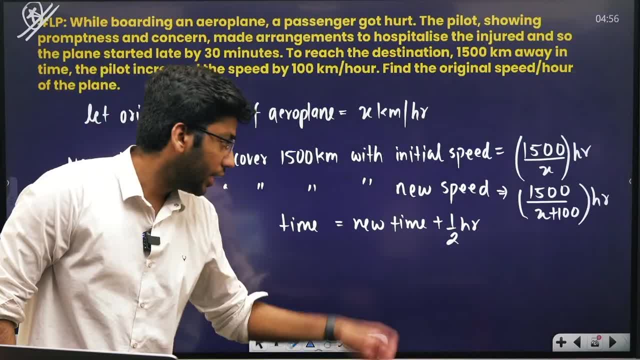 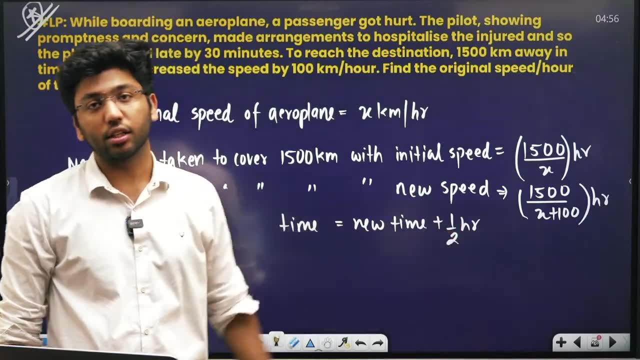 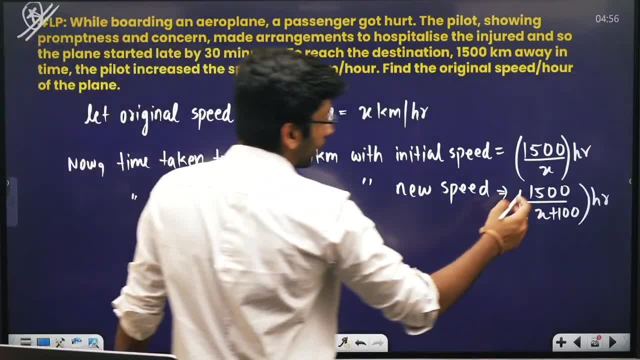 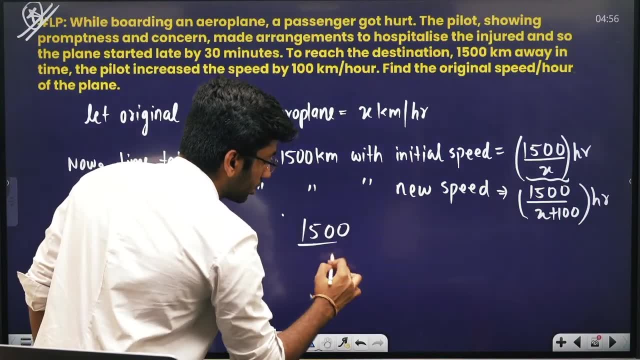 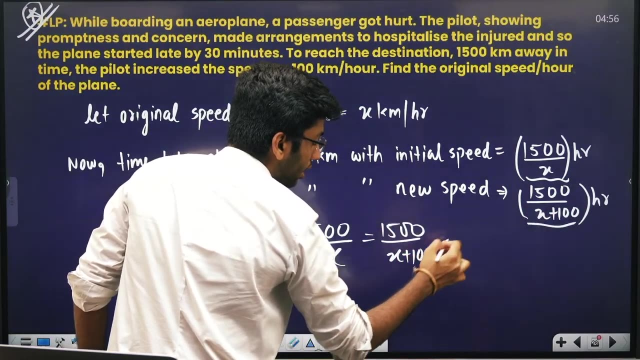 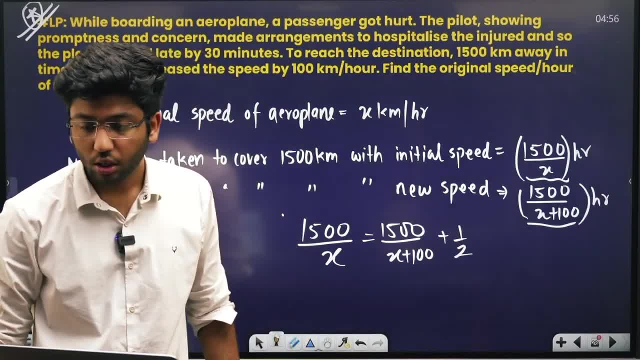 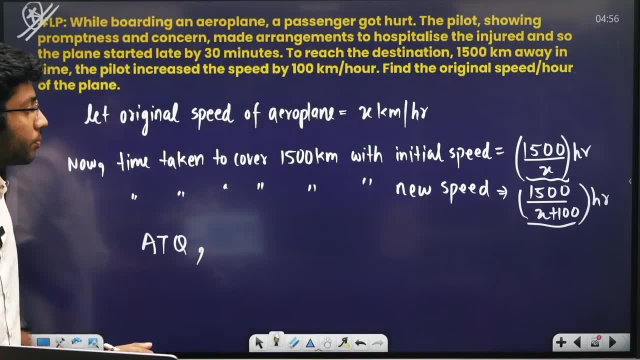 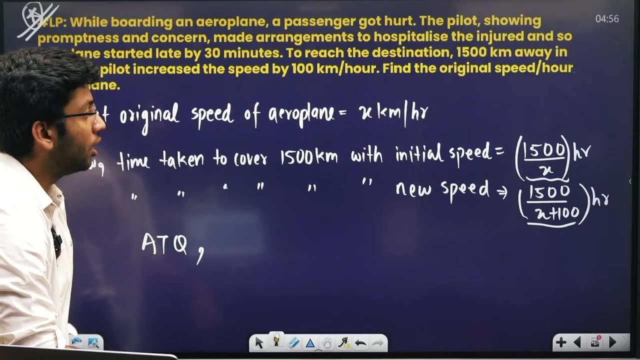 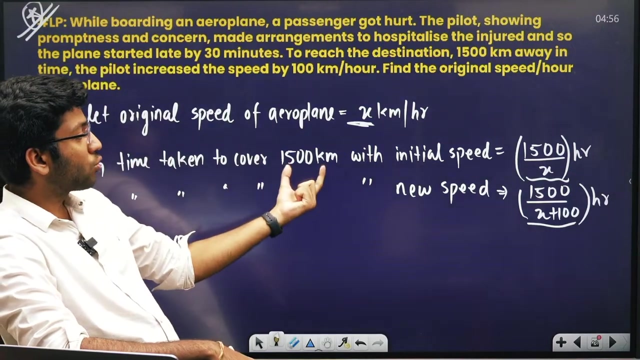 Understood, Understood, Understood, Understood. 500 answers are hanging around. Listen carefully first Look, look, look. The original speed is x. So if it had to go 1500km and suppose it would have reached initial speed. 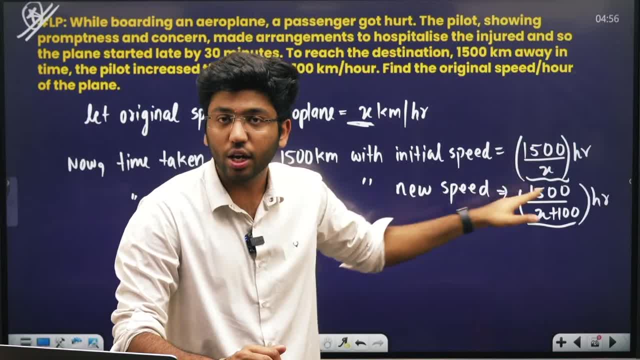 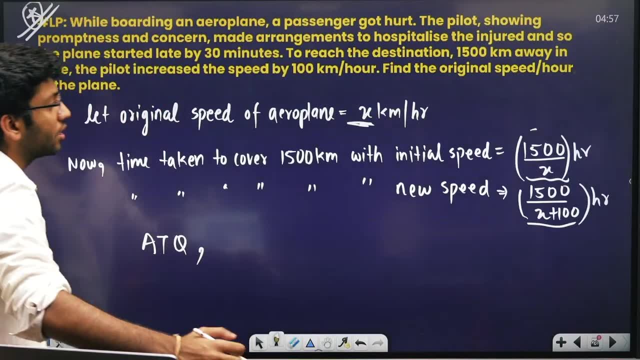 then it would have reached like this: It would have reached like this: If it had reached initial speed, then it would have reached 1500 upon x. Now, what did it do? Now, what did it do? it did that. the pilot increased the speed. 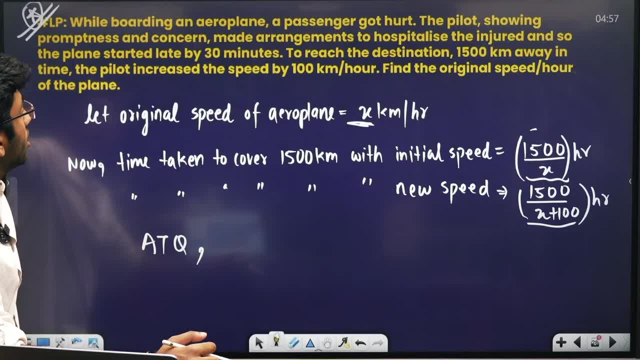 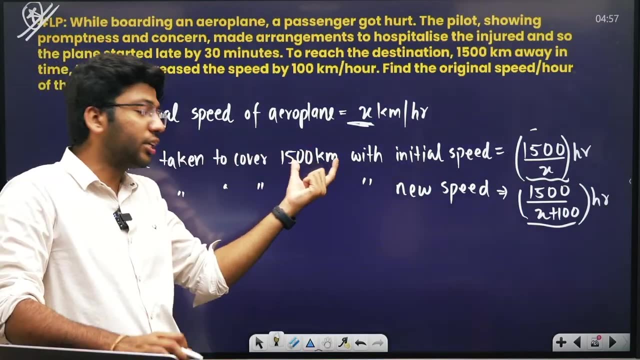 The pilot increased the speed. So the pilot increased the speed by 100 km per hour. So he increased the speed by 100 km per hour. So find the original speed. So if 1500 km would have gone with the original speed, then this would have happened. 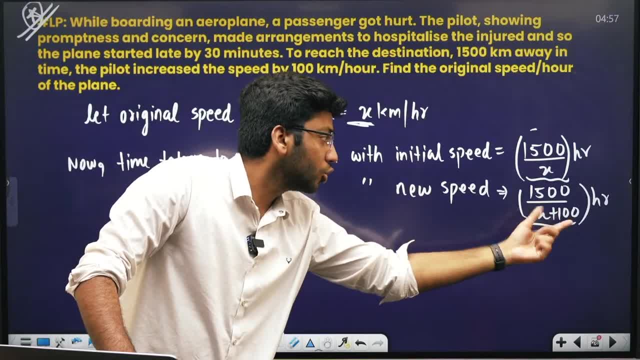 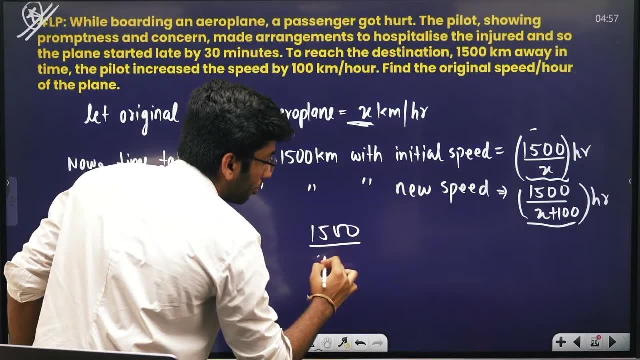 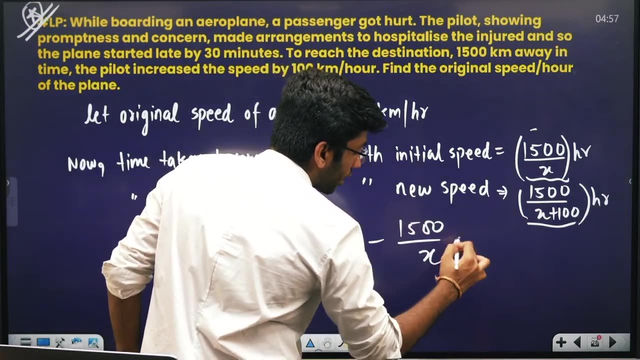 But he increased the speed by x plus 100. So now the time is this much, So this time is 1500 upon x plus 100. If I differentiate this new time with 1500 upon x, then it will be equal to 1 by 2.. 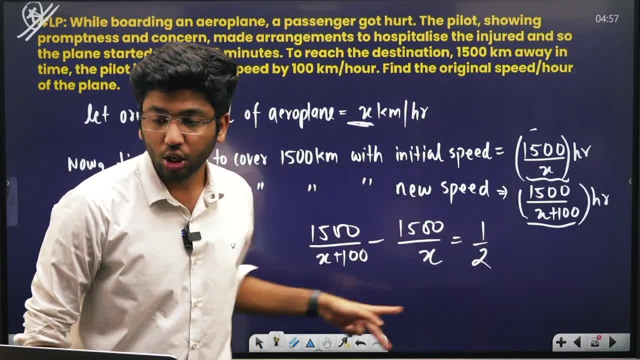 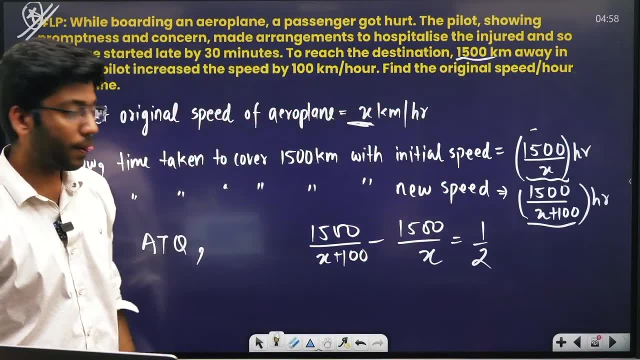 Because it takes more than half an hour. What is the difference between both? Half an hour. What is the difference between both? Half an hour? Is it 1500 or 500?? It is written as 1500.. What is the difference between both? 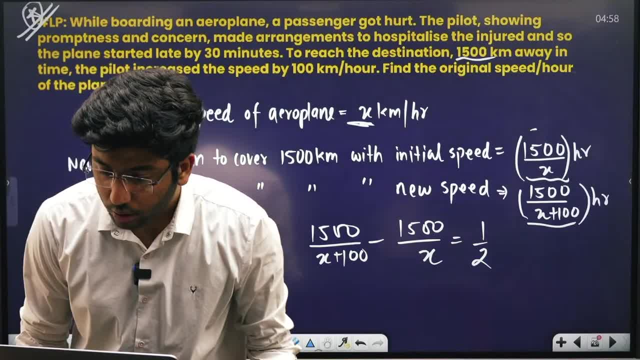 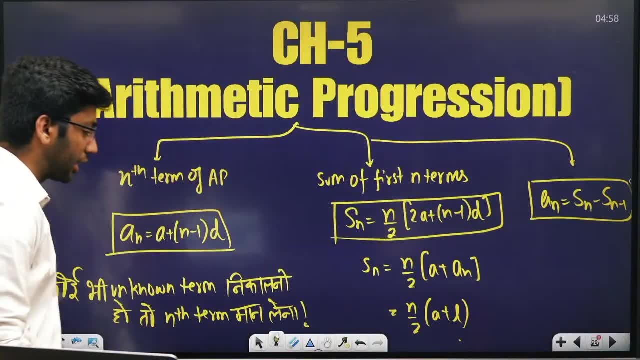 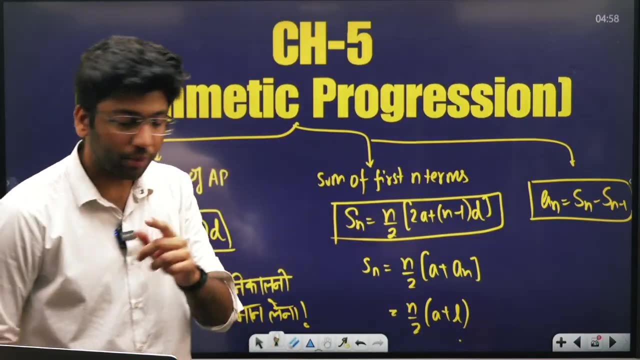 Okay, Did you understand? Did you understand? Is it 500?, Brother, it's 5 o'clock. Okay, let's come to the next question. Come to the next question: Arithmetic progression. I have written the opposite. Yes, I think I have written the opposite. 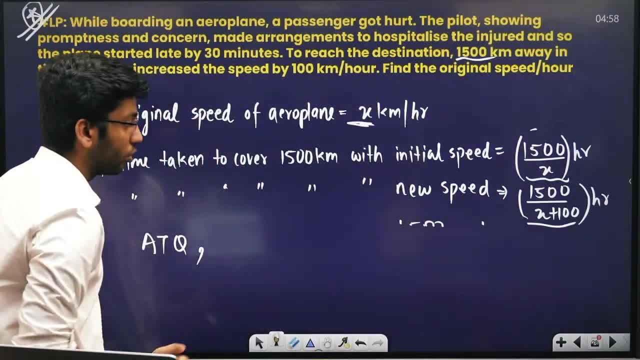 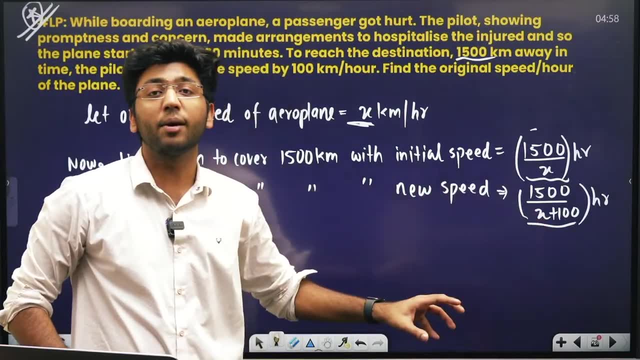 See, wait a second. The new speed, Yes, yes, yes, We're talking about the time. This time is more. This time is more. This is not about speed, We're talking about time, So this time is more. 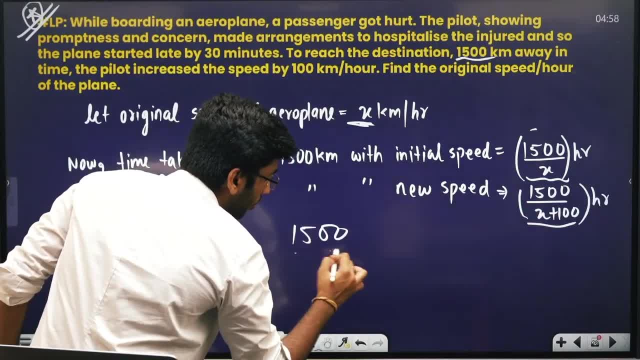 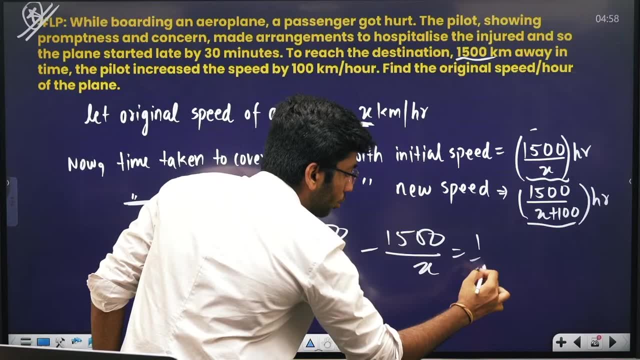 This time is more. This time is more. So 1500 upon x plus 10, x plus 100.. If I remove the original time from this time, then there is a difference of 1 by 2 in both. There is a difference of 1 by 2 in both. 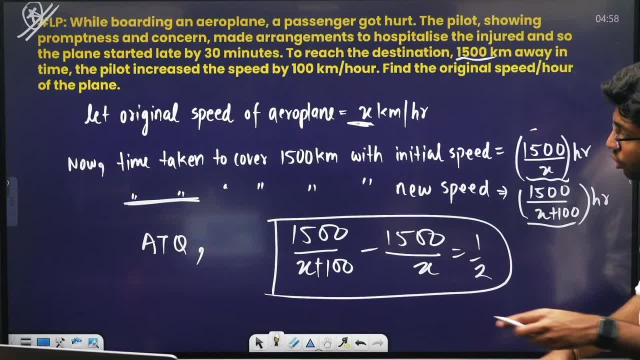 Look, understand it carefully. It seems that this time is more Okay. Someone wrote the opposite. It was written correctly. It was written correctly. Who said it? Who said it? It was written correctly. It was written correctly. Someone said it. 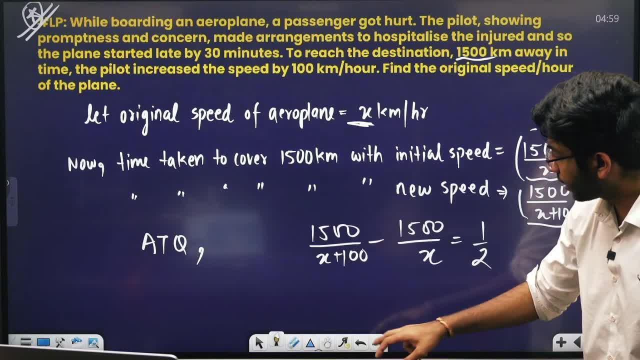 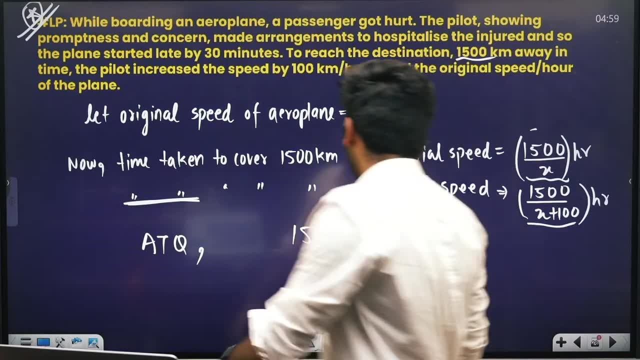 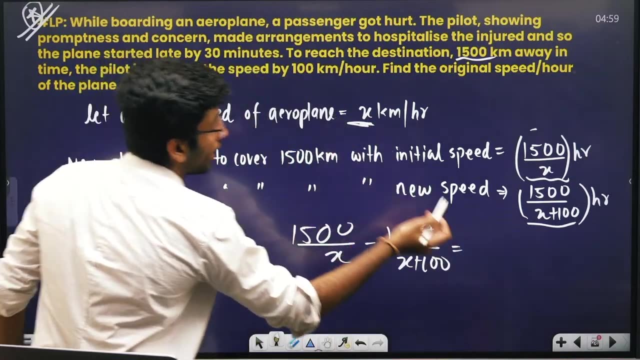 I got confused. It was written correctly. It was written correctly. Where did it go? Where did it go? Look What is 1500 upon x minus 1500 upon x plus 10. equal to What is equal to? It is equal to half. 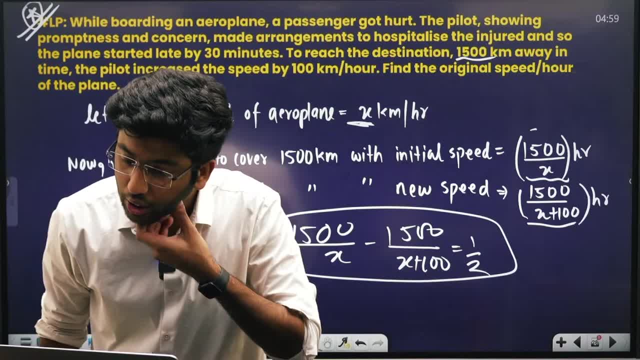 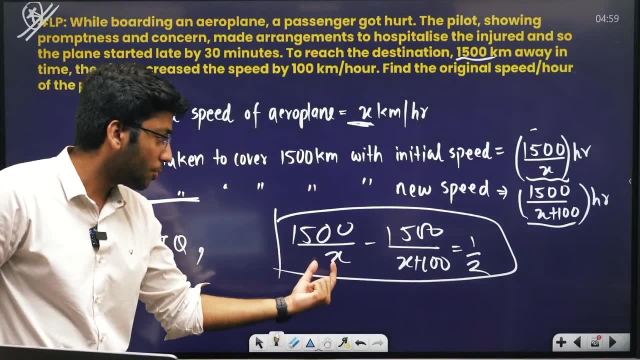 It is equal to equal to half. This equation will be made Okay. Okay, Hey, there was no confusion. I am teaching a little fast, That's why I made a little mistake, But now you understood. What is 1500 upon x minus 1500 upon x plus 10?? 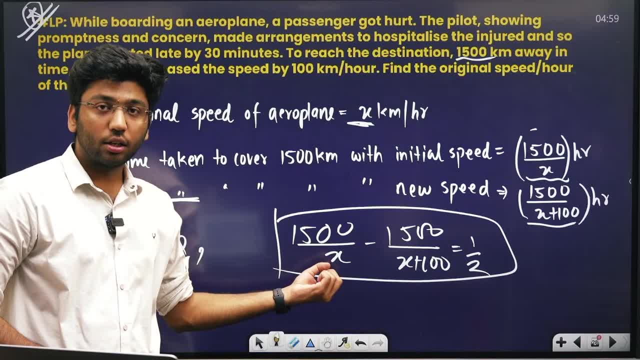 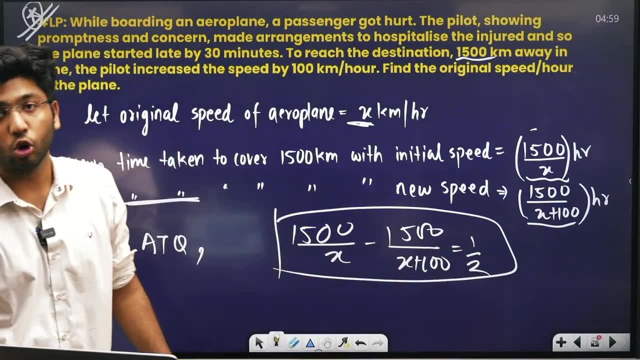 This? Why? The original time was this, But then what happened? Time is less, Time is less, So the original minus time, which is less, is equal to half. What is the difference between both? It is half. What is the difference between the difference between the original time and the time which is? 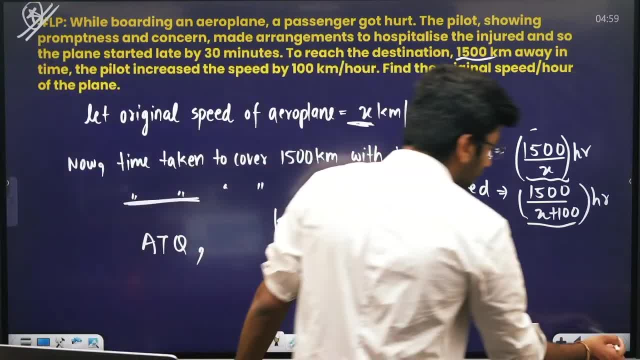 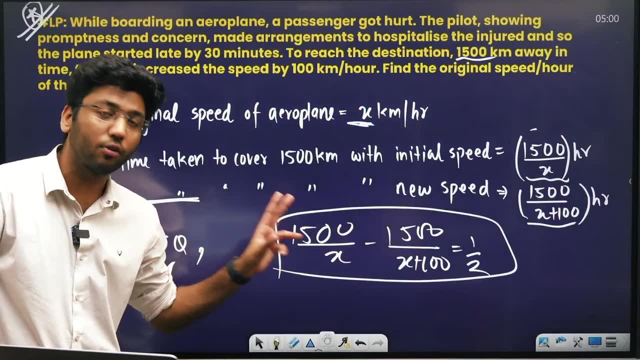 given in the last, It is half. This is written in this equation. Okay, Next, Next, Next, we come to arithmetic. Who doesn't understand this? Look, It takes a lot of time to explain this. Who is not understanding this? 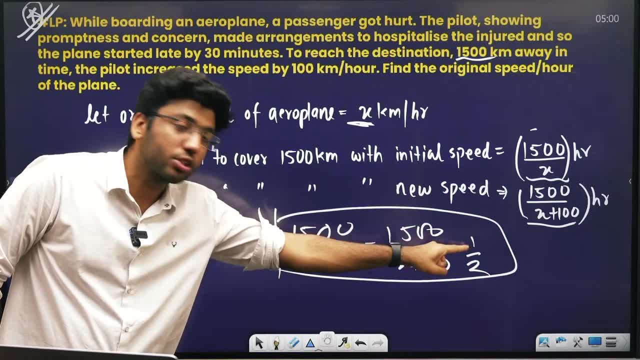 Understand that. Look, This is the big quantity. Smaller is the big, then the positive will come. This is the big quantity. Whose denominator is less? the whole quantity is big. Whose denominator is small? the whole quantity is big. 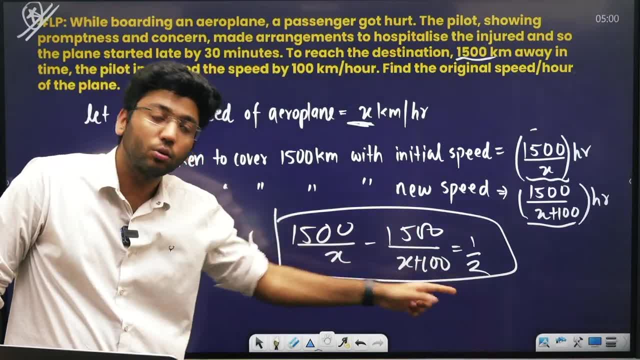 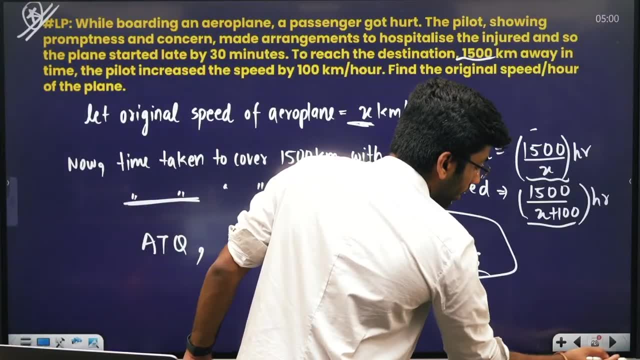 So big minus small quantity will give positive 1 by 2.. So big minus small equal to 1 by 2.. Do this according to question. Those who don't understand can do it this way. Okay, Next, Next, If I talk about arithmetic progression, 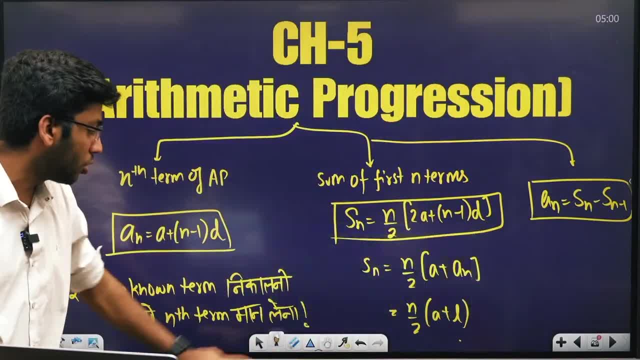 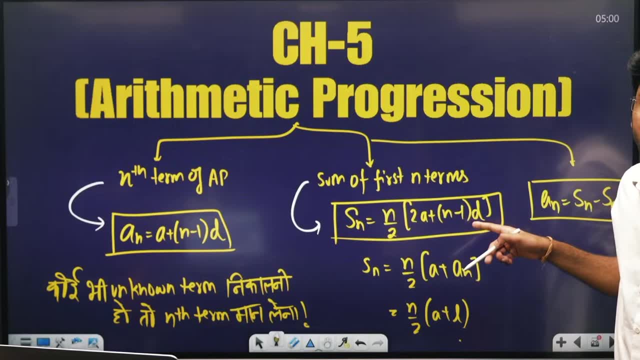 If I talk about arithmetic progression, then two formulas which are very important: Nth term of AP AN equal to A plus N minus 1 D. Sum of N terms of AP N by 2 into 2 A plus N minus 1 D. 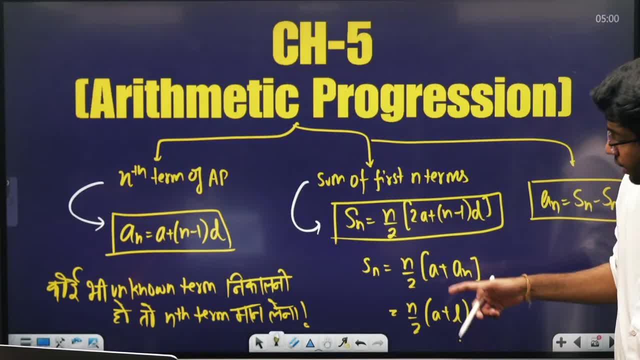 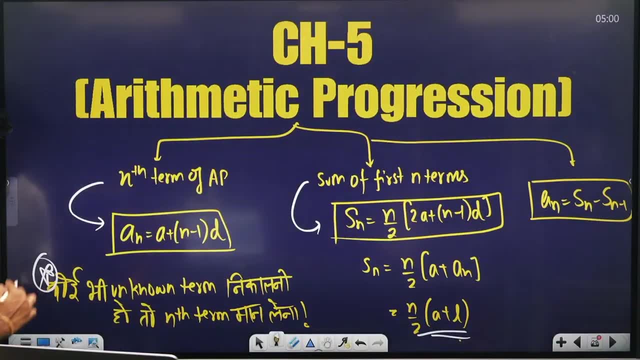 Okay. Sometimes this is written as N by 2 into 2 A plus AN or A plus L. This is also written in this way. We know that these two formulas are very important. If you have to find any unknown term, then consider it as Nth term. 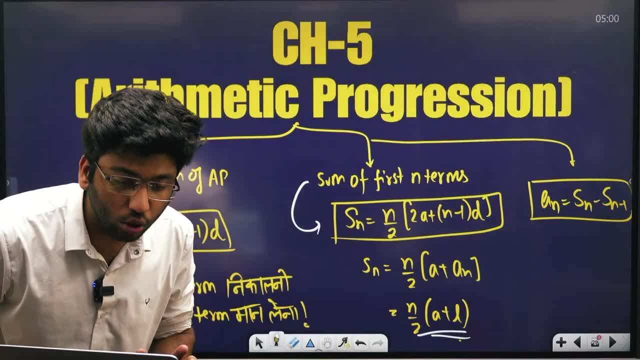 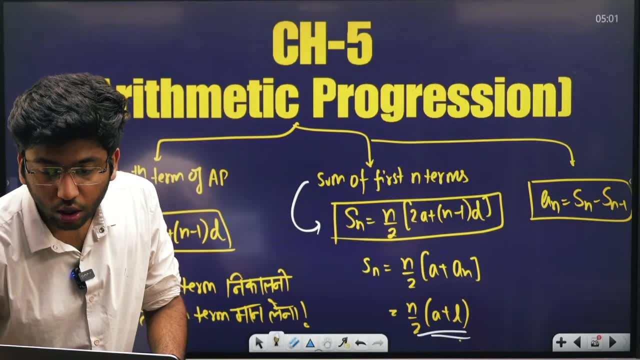 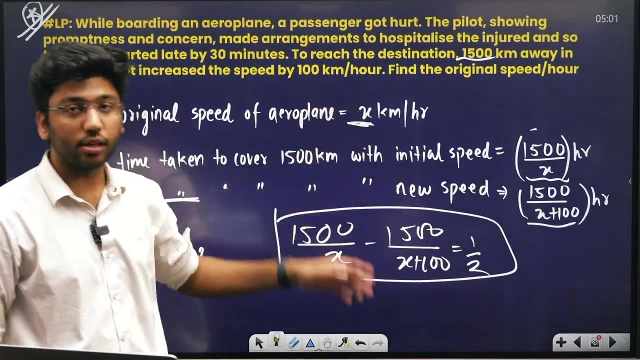 What am I saying? If you have to find any unknown term, Any Brother, was that the answer? I said no, my dear, It was not there. Now I will solve it for you. Take out the value of X. The value of X is the answer. 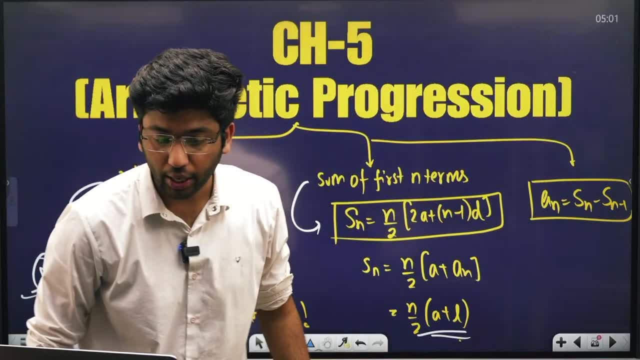 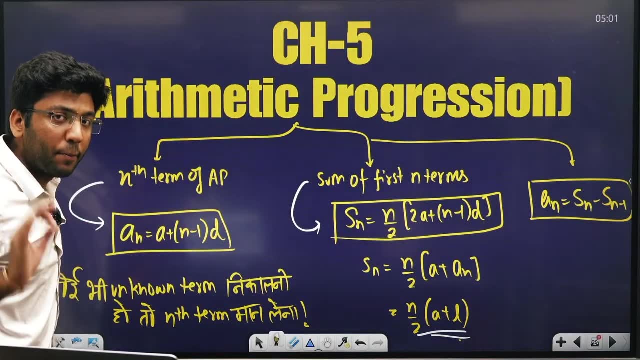 You don't have to do this much. I am giving you that by making you an equation. I am giving you that by making you an equation. Look, Look, Look carefully. Nth term, If you have to find any unknown term in AP. 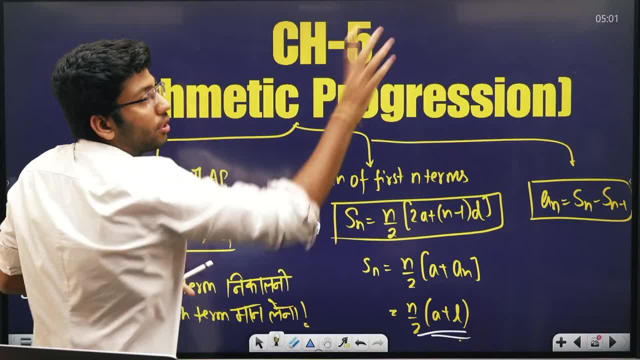 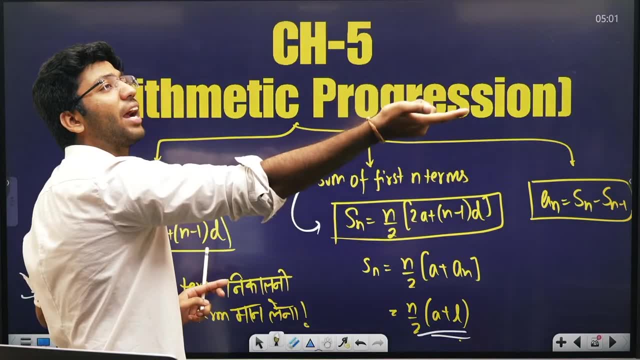 I told you. Tell me which term will be this, Then consider it as Nth term. Tell me which will be the first positive term Nth term. Tell me which number will be 150 in this AP, Then consider it as Nth term. 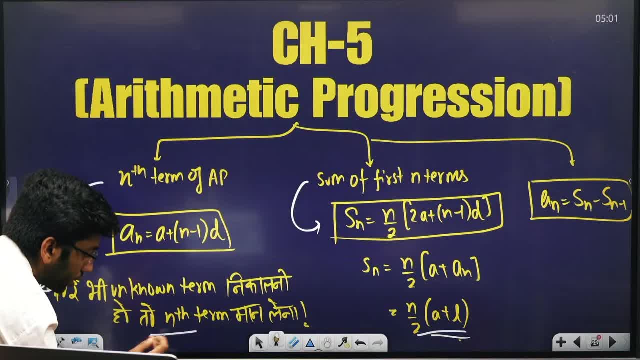 So whenever you talk about unknown term in AP, Consider it as Nth term. Then consider it as Nth term. Now I will do the next question You will understand. Sum of first N terms is this: And there is one formula: 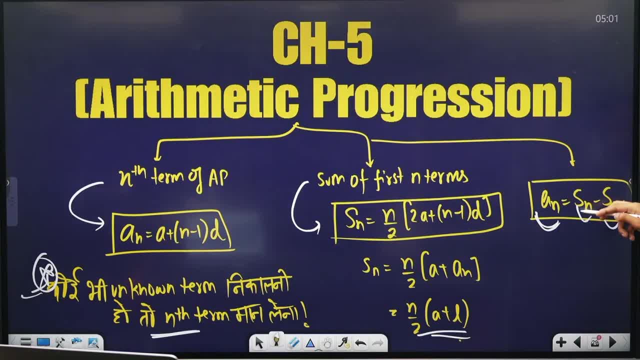 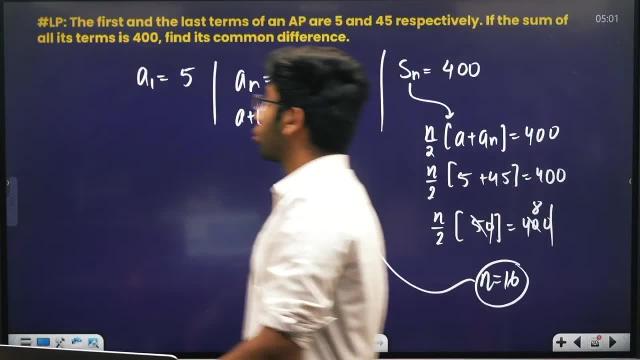 That Nth term is Sn-Sn-1.. Means the sum up to N term And the sum up to N-1 is this. So these three formulas are very useful for you. Some questions which CBSE likes a lot. There are chances of getting such questions. 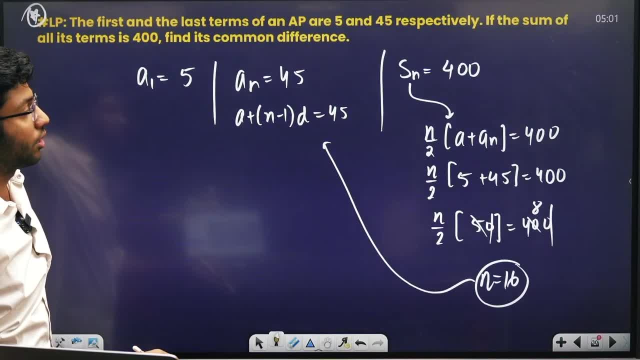 What? First and last term of AP are 4 and 5 respectively. So first term is 5. And last term means Nth term is 45. Okay, So suppose there were N terms in AP. There were N terms in AP. 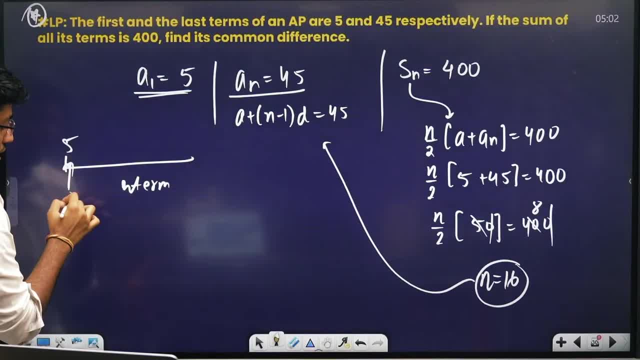 You know the fifth term. You know the first term is A And last term means 45. Means this is Nth term, Last term means Nth term. So you know the Nth term is 45. So first term is 5.. 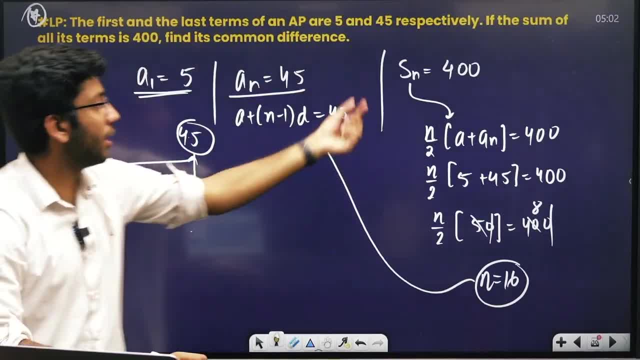 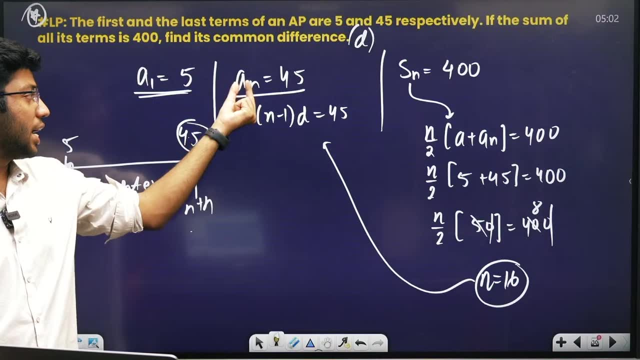 Second term is 45. If the sum of all terms Means Sn is equal to 400.. So find the common difference. Common difference means you have to find the value of D. So you know A, An is equal to this. You know this. 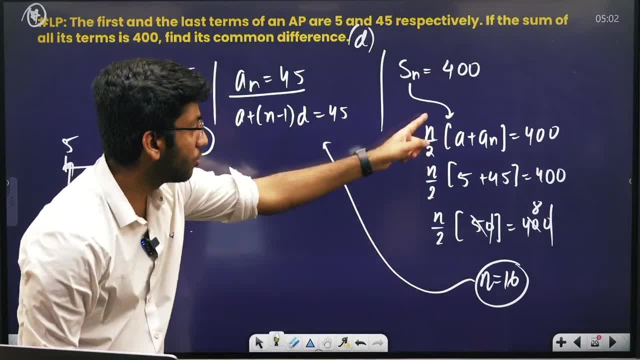 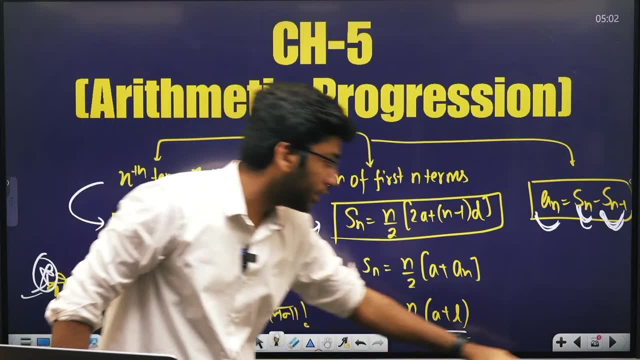 Okay, You need the value of Sn. You need the value of Sn. What is the formula of Sn, n by 2 into A plus An? I know two or three formulas for Sn, So I said I know A and An, So I have put this formula. 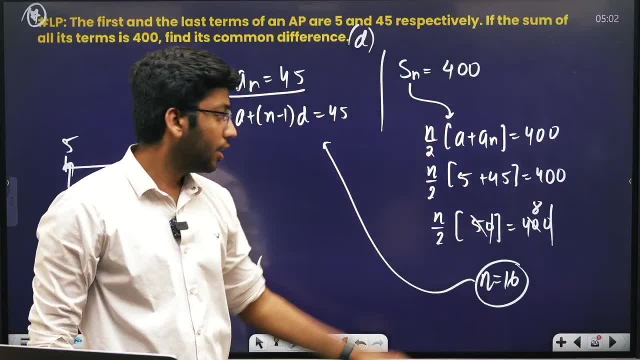 Sn is equal to n by 2- into A plus An. I kept this. I knew A's value, I know An's value. I put it So from here. I know the value of N. I know n's value. I know n's value. 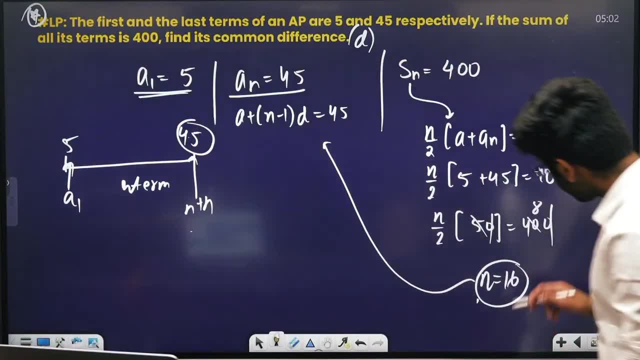 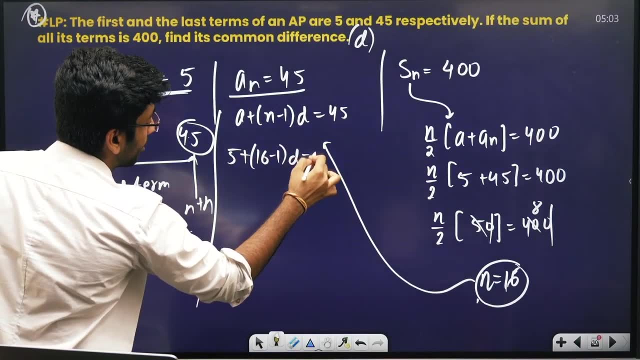 I will put that n's value here. So what is n's value? N's value is 16.. So if I put 16 here, then what will happen? 5 plus 16 minus 1 into D is equal to 45.. 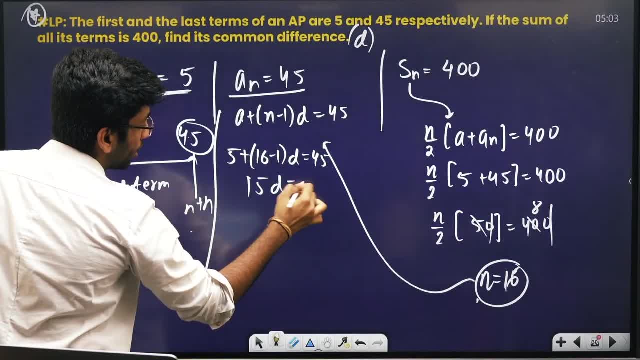 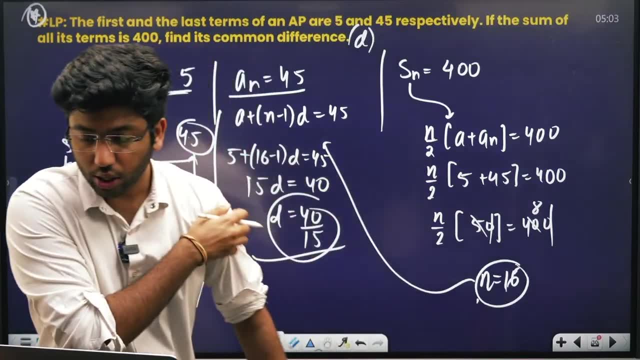 So from here, 16 minus 1 will be 15 into D Equal to 40. So D value will be 40 divided by 15. This will be your D value. This will be your D value. 8 by 3 will be your D value. 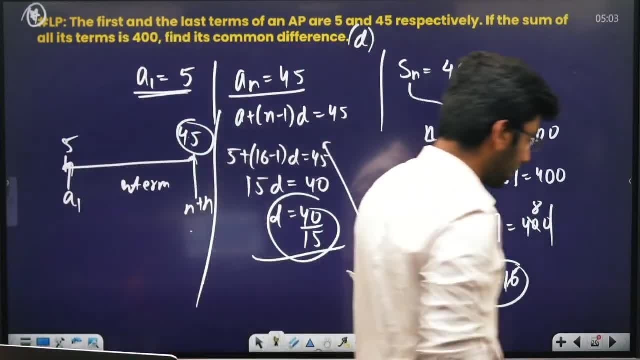 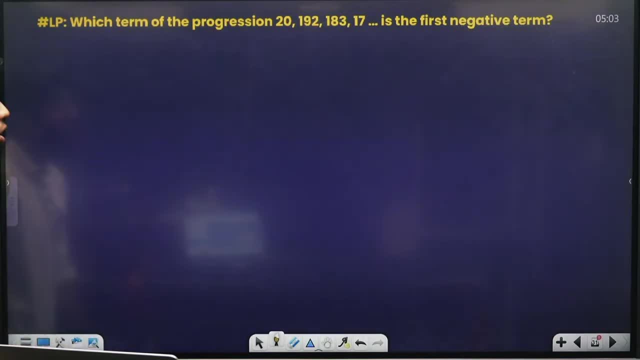 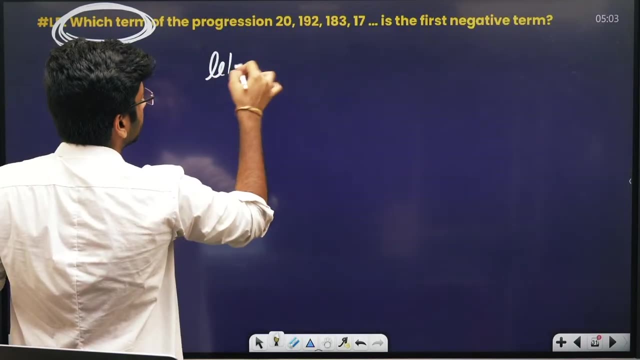 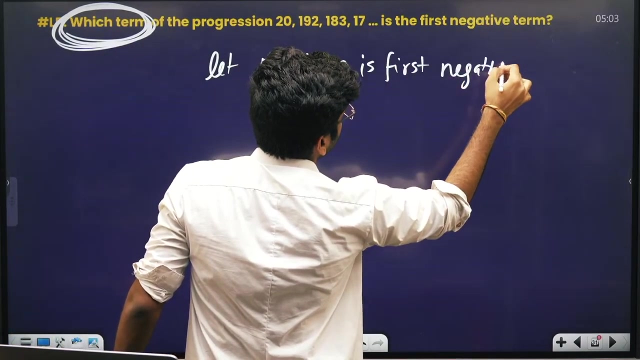 Okay, Okay. Next question: Which term of the progression Is first negative term? See which term I am talking about: unknown term. Which term- Let an ananth term- Let an ananth term- Is first negative term. Which term- An ananth term- Which is first negative term Of this progression? 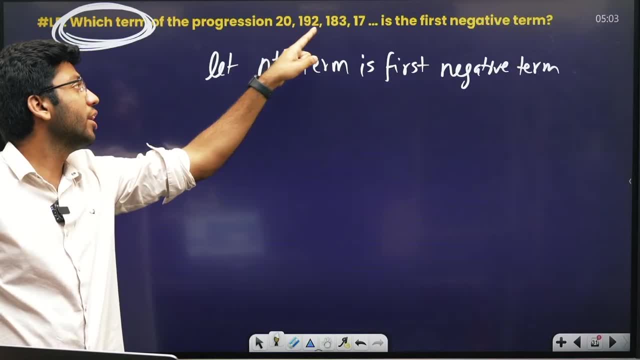 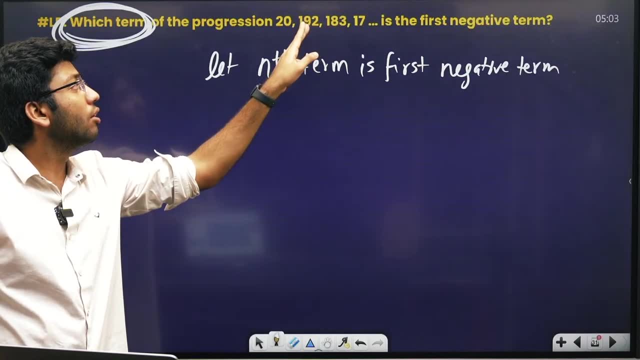 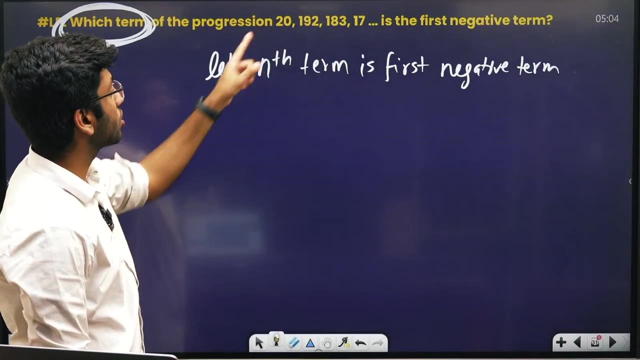 So do 192 minus 20, Do 192 minus 20. Do 20 minus 172 From 183. From 192, This is 120. Yes, This is 220. I have shown this question is wrong. Wait a second. This question is wrong. 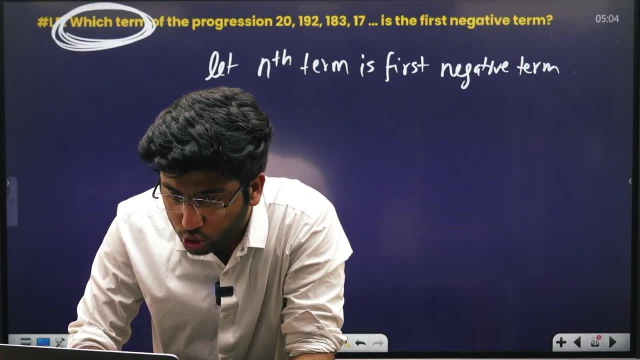 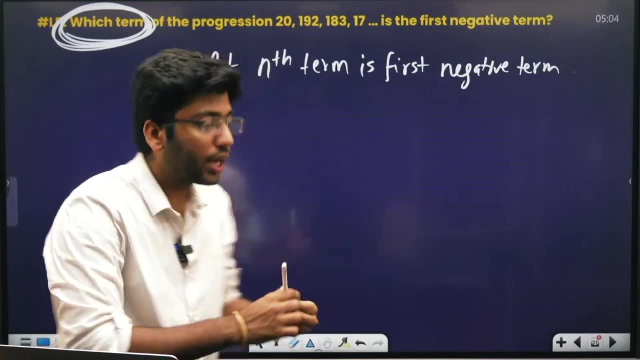 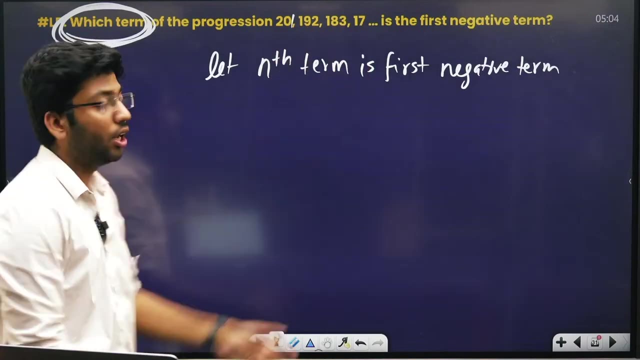 One second. This is 200 or something else. Hold for one second. This is 201.. This is 201.. 201, 192.. This is decreasing. One was 201 and one was 192.. Like this: 192 minus 201.. 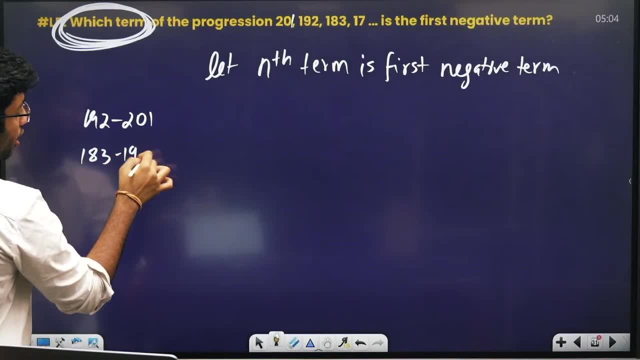 Take out 183 minus 192.. First we have to check if it is AP or not It is AP. How do we check 192 minus 201.. 192 minus 201.. How much Minus of 9.. 183 minus 192.. 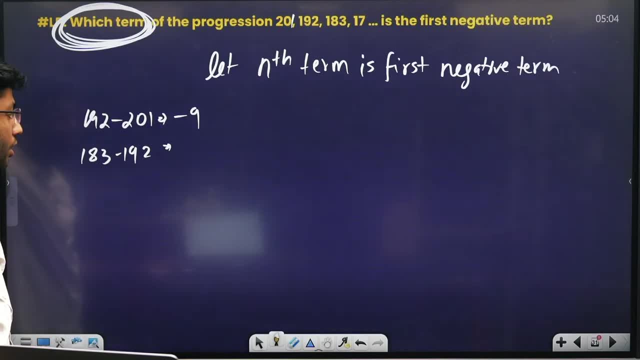 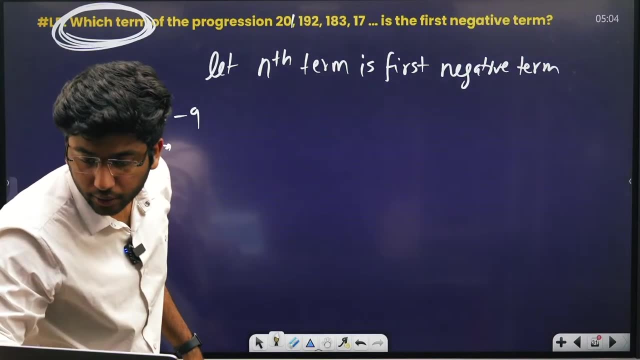 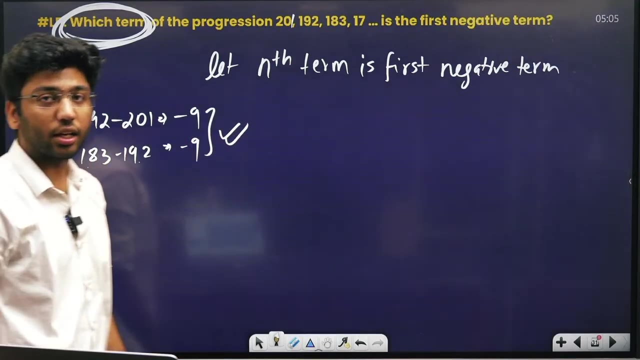 183 minus 192.. 183 minus 192.. So what Minus of? Am I doing something wrong? It is correct. Similarly, 183 minus 192.. So what does this mean? This is one AP. This is one AP. 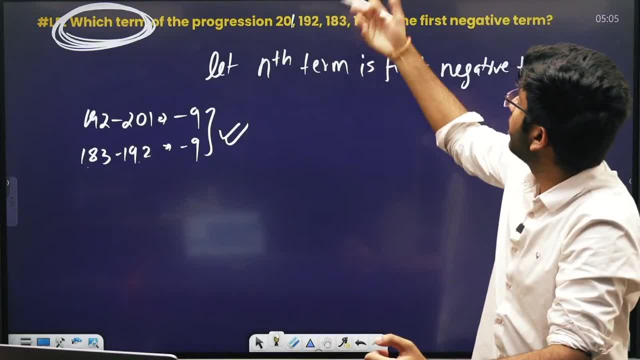 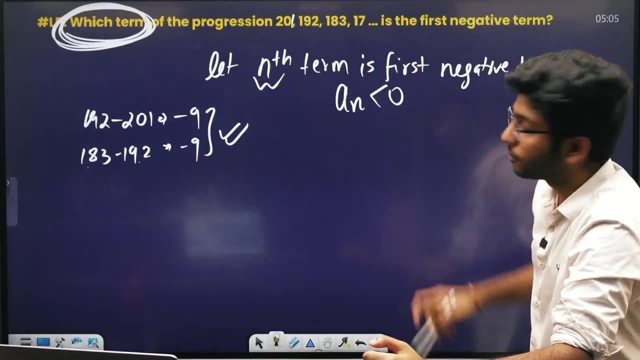 AP is coming Now. what do we have to do? Which term is the first negative term? So I have taken: Nth term is the first negative term, Which means AN will be less than 0.. Nth term means AN. Nth term means AN. 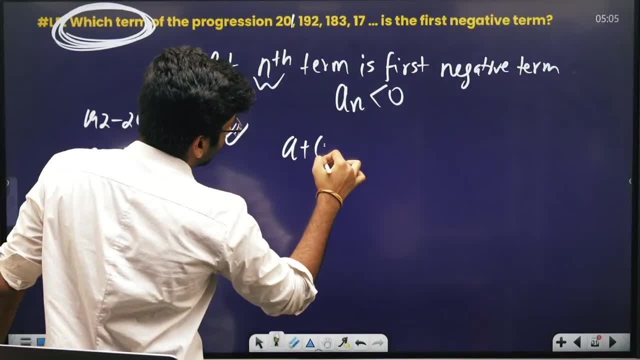 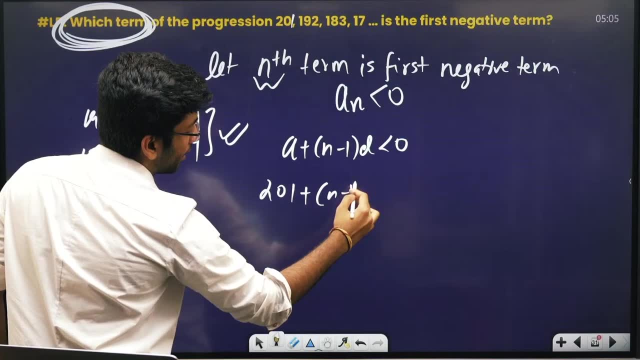 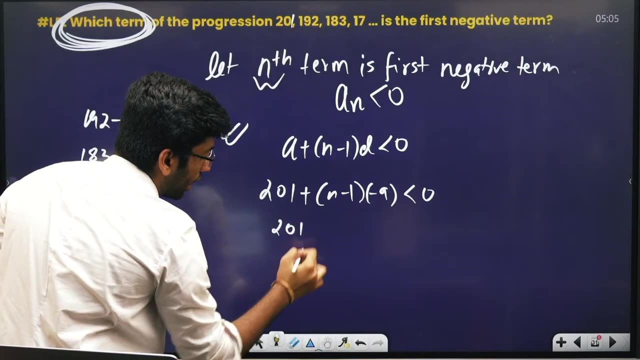 It is negative. So what is AN A plus N minus 1? D is less than 0.. The value of A is 201.. Plus N minus 1.. What is D Minus 9.. Less than 0.. It is coming in this way: 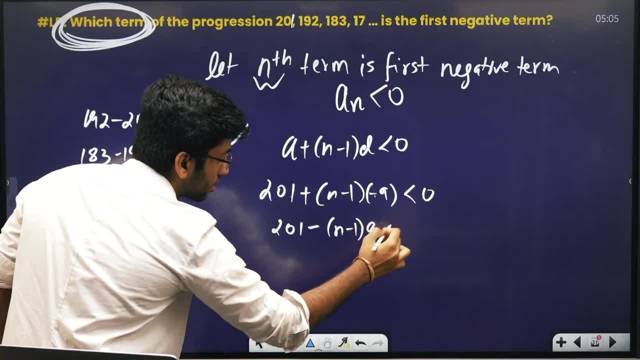 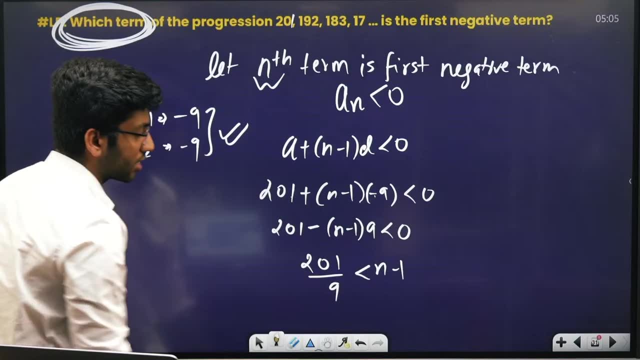 If we take this, 201.. This will be minus, So minus 9.. N minus 1 into 9 is less than 0.. This will go here: 201 upon 9.. Less than N minus 1.. It is coming in this way: 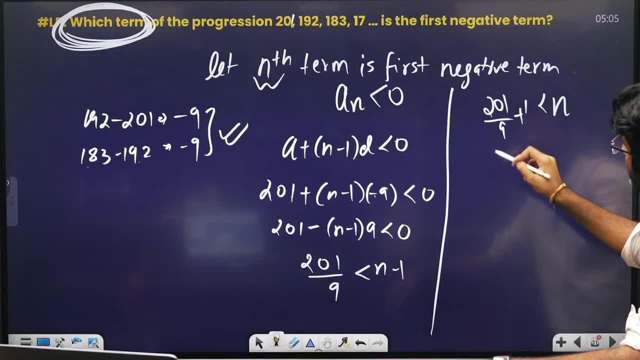 So, if we see from here, N is greater than 201 by 9 plus 1.. 210 by 9.. Less than N, So 9 to the 18.. 9 to the 18.. 9 to the 18.. 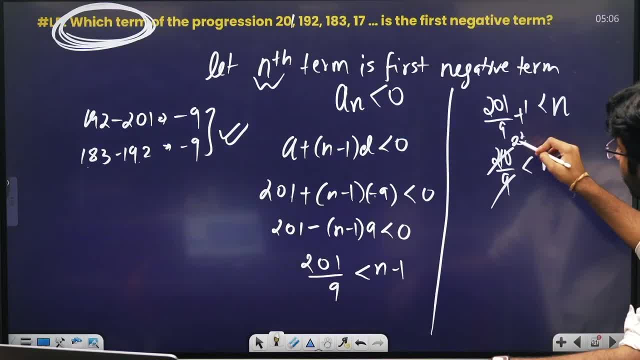 19,, 20,, 21.. 3.. 9,, 3 is 27.. So 23 point, something is coming, 23 point something. So N is greater than 23, point something. Which number is greater than 23?? 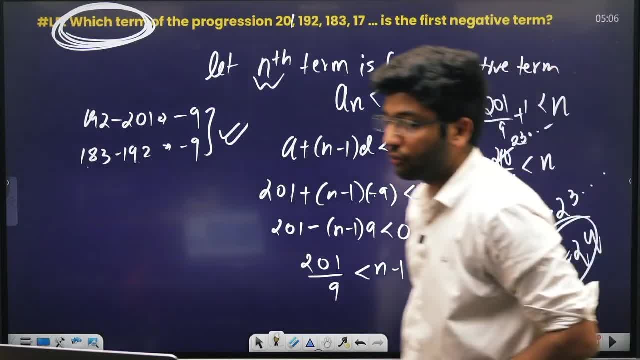 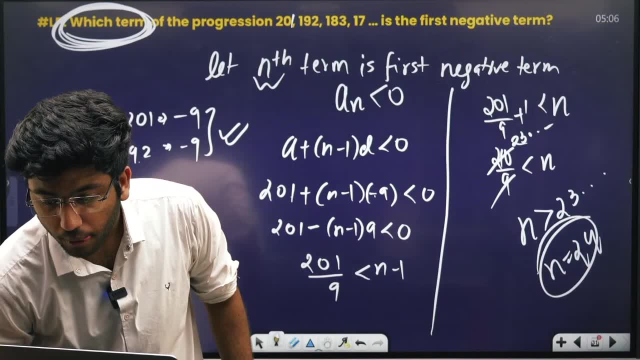 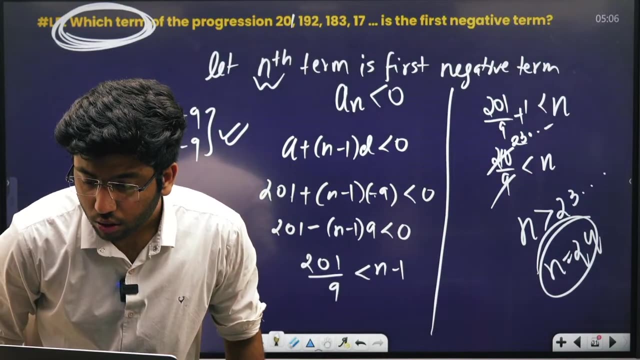 Natural number 24.. So N is equal to 24.. So what will be the 24th term? What will come? What is wrong? I think it is wrong. I think it is wrong, Brother. this is for basic. What is wrong? 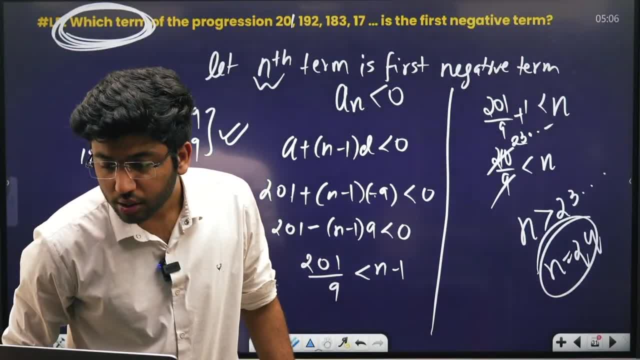 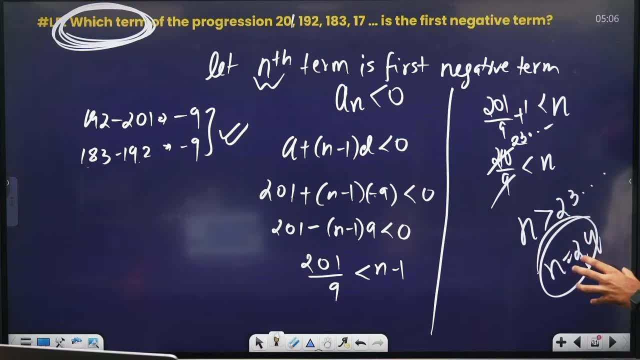 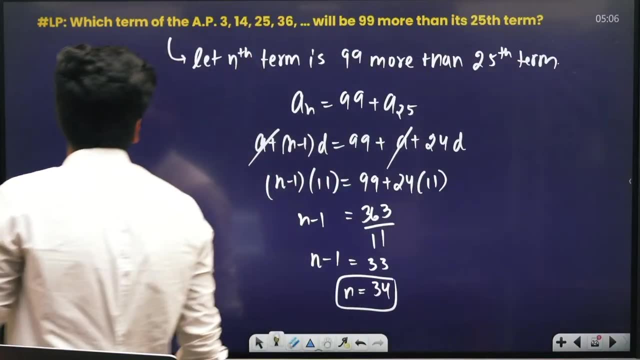 It is correct. It is correct, Brother. will you give this PDF? I will definitely give. So this is yours. N is 24.. This will be your answer. You will get it, Ok. Next question: Which term will be 99 more than Nth term? 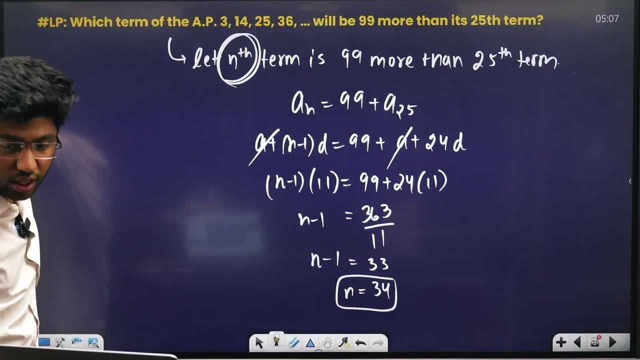 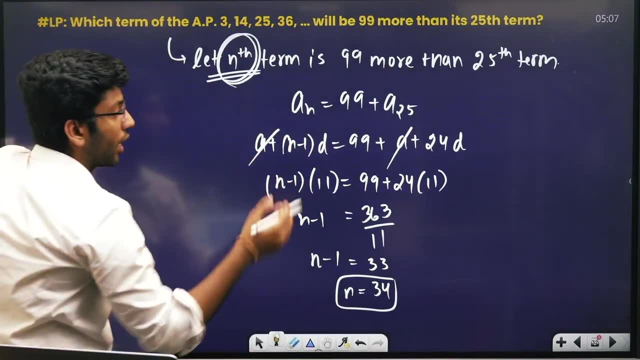 Which term. So what will I assume? Nth term. What is he saying? Which term will be 99 more than 25th term. So I will assume Nth term is 99 more than 25th term, So Nth term. 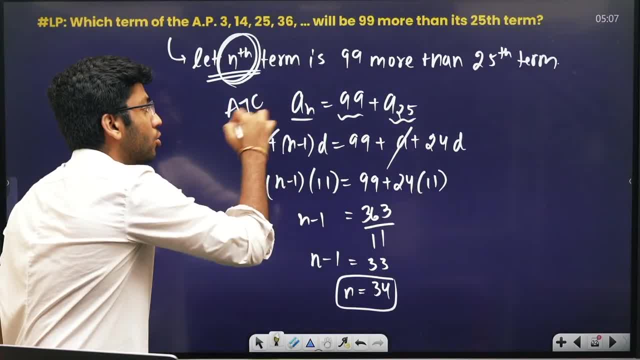 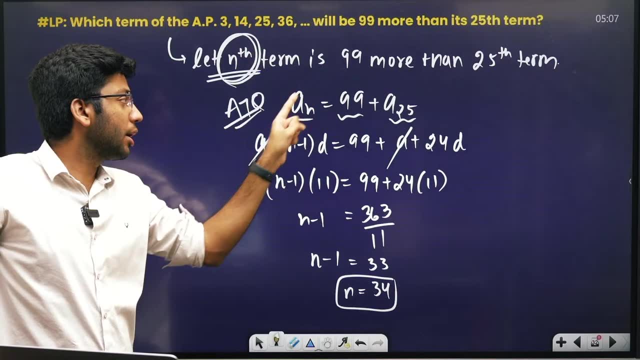 So AN will be 99 plus A25.. According to question he is saying: According to question he is saying: AN is equal to 99 plus A25.. AN is equal to 99 plus A plus A. We will calculate from here. 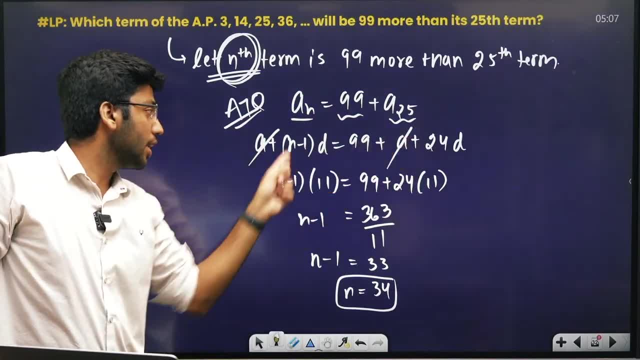 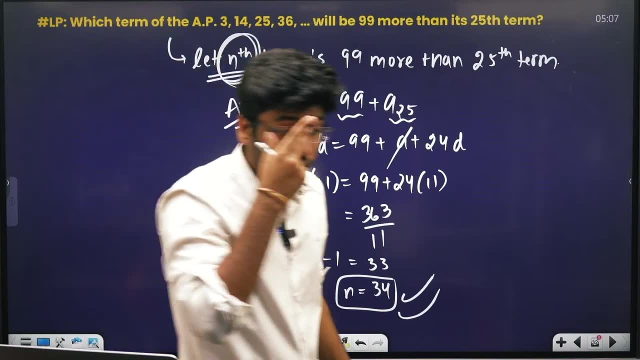 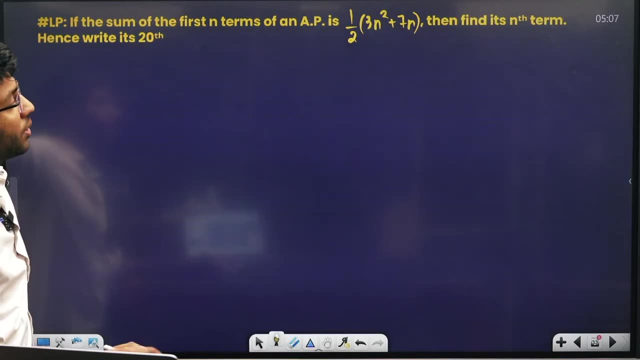 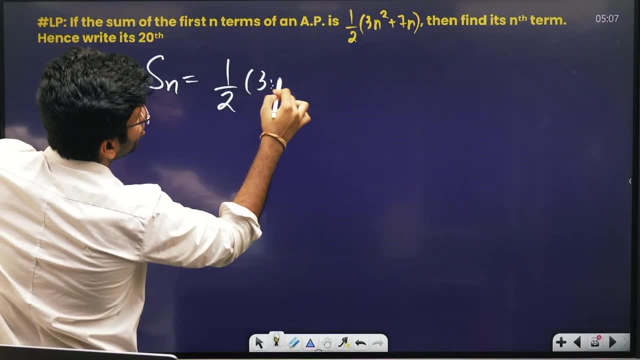 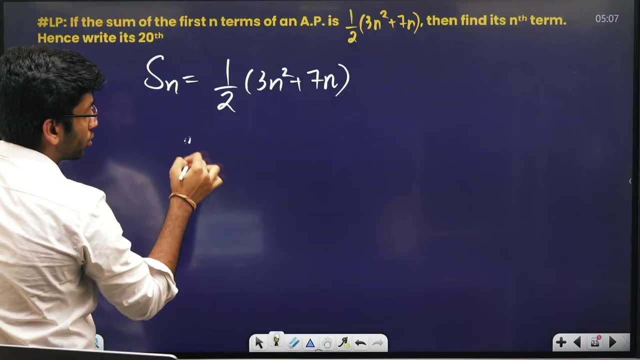 We have been given the sum of first N terms, 1 by 2, 3 N square plus 7, N plus 7n. This is the sum of first n terms of apd. If I put 1 in the place of n in the sum of n terms, then the sum of first term 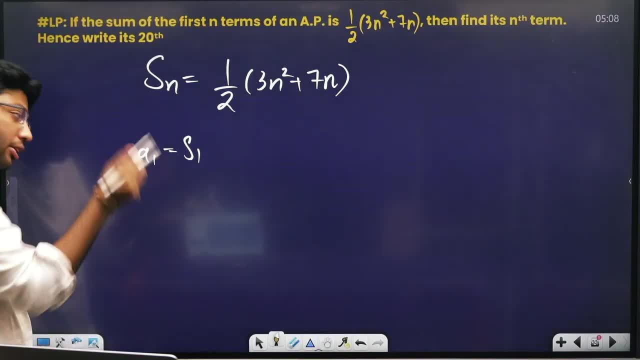 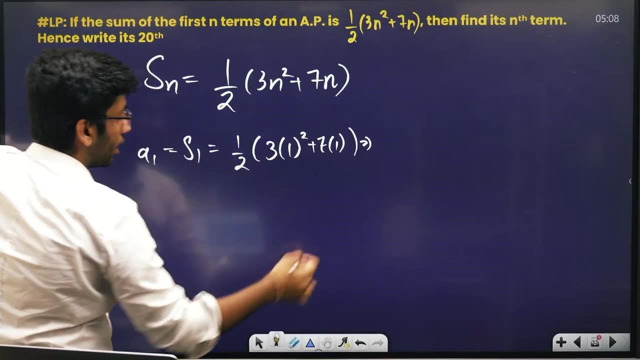 The sum of first term means the first term. The sum of first term means the first term. So what will that be? 1 by 2 into I put 1 in the place of n plus 7 into n 1.. So what will this be? 7 plus 3. 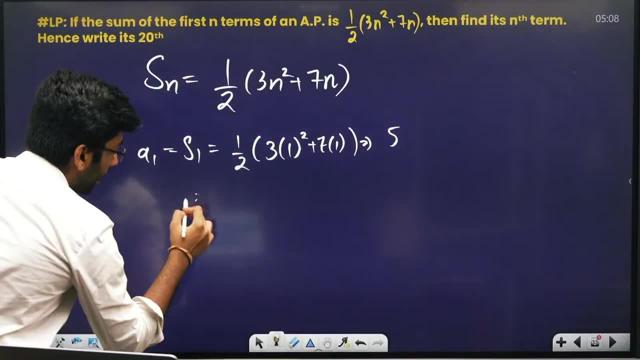 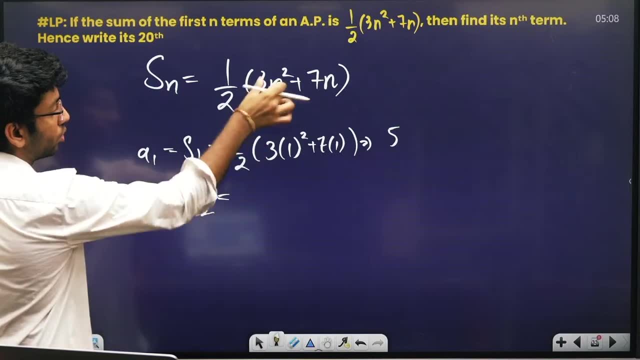 10 by 2 is 5.. This is the first term. If I talk about s2, then s2 means first term plus second term. So I put 2 in the place of n. So if I put 2 in the place of n, then 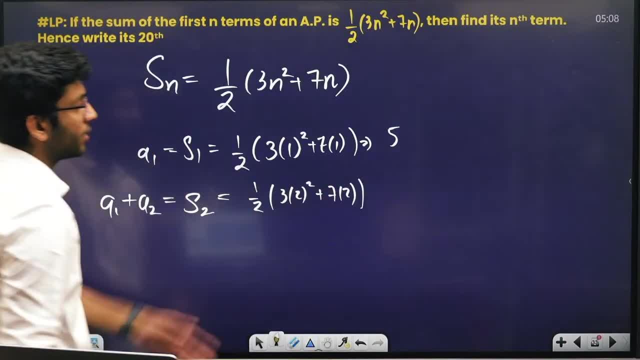 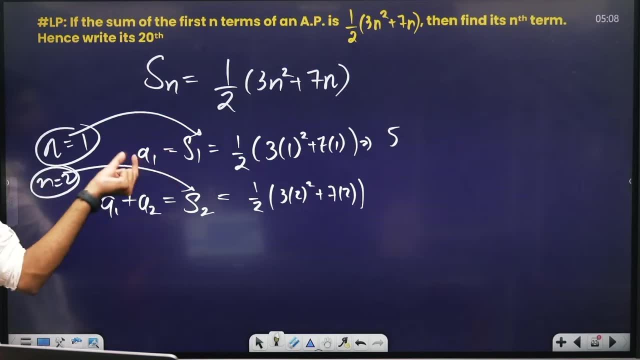 1 by 2 into 3, into 2 square, plus 7 into 2.. Whenever this type of formula will come, then what to do? Put 1 in the place of n and take out s1.. Put 2 in the place of n and take out s2.. s1 will be equal to the first term. 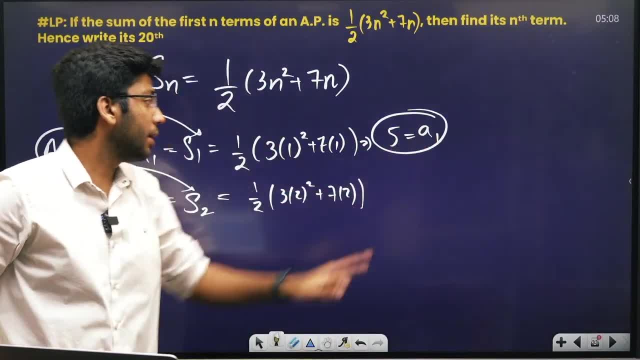 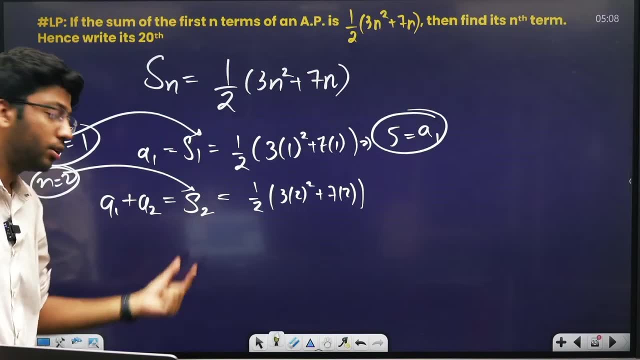 So a is equal to 5.. The first term is a1.. Our first term is 5.. If I put 2 in the place of n in s, then we will know s2.. s2 means the sum of first and second. First is 5. 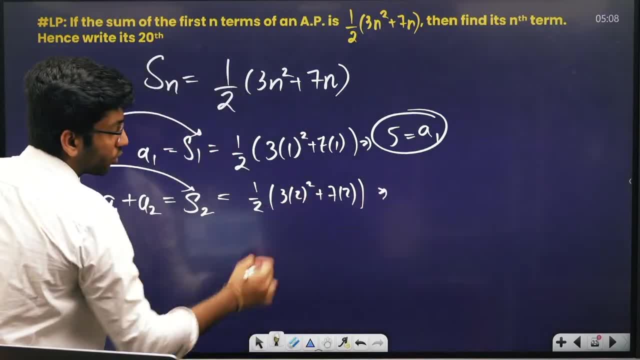 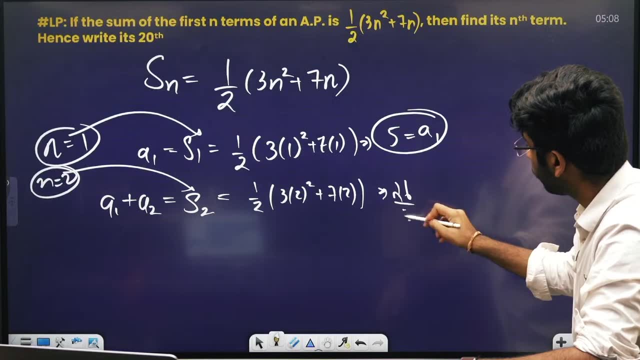 and then we will know the second. So if we put 2 in the place of n, then what will this be? 4 plus 3 is 12.. 12 plus 14.. 12 plus 14 is 26.. 26 by 2 is 13.. 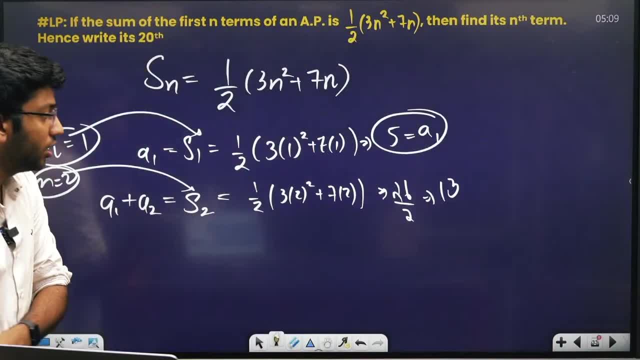 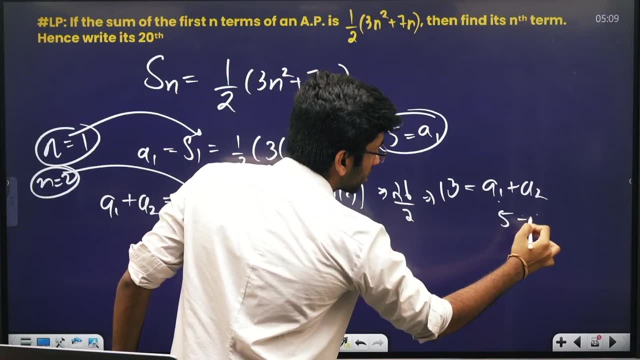 12 plus 14 is 26.. 26 by 2 is 13.. So what is this? This is s2.. s2 means a1 plus a2.. a1 plus a2.. a1 is 5.. So 5 plus a2 is equal to 13.. 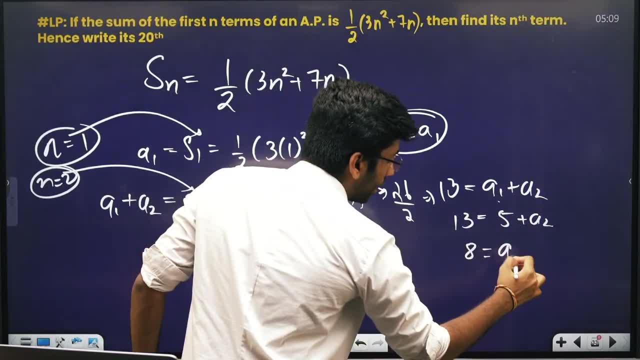 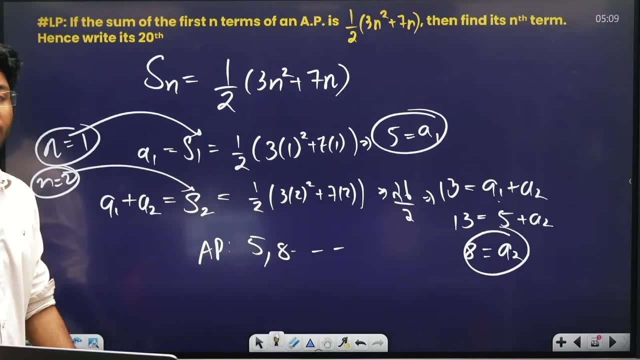 So 5 out of 13 is equal to 8.. 8 is equal to a2.. So the first term is 5 and the second term is 8.. AP is made like this. 5 and 8 are made like this. We know AP. 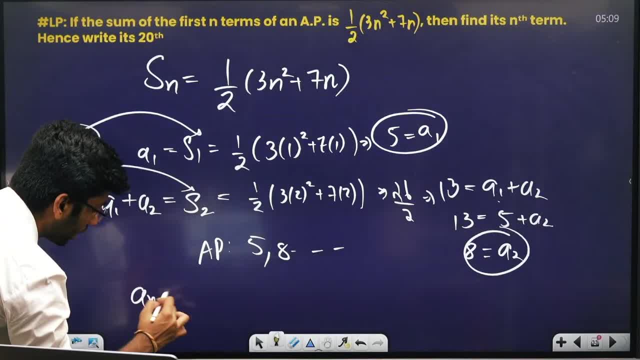 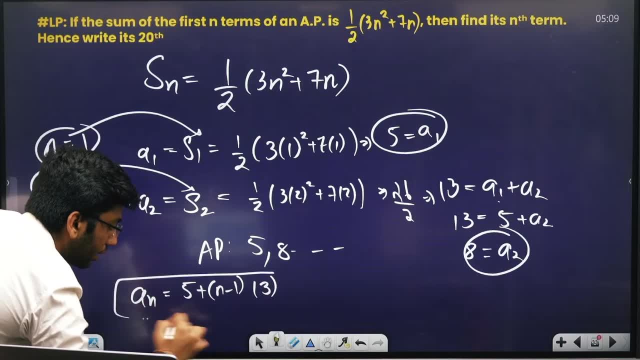 We have been asked to find its nth term. So take out an equal to an. What will an be? a plus n minus 1d? a is 5 plus n minus 1 into d. What is d? 8 minus 5 is 3.. This is an. 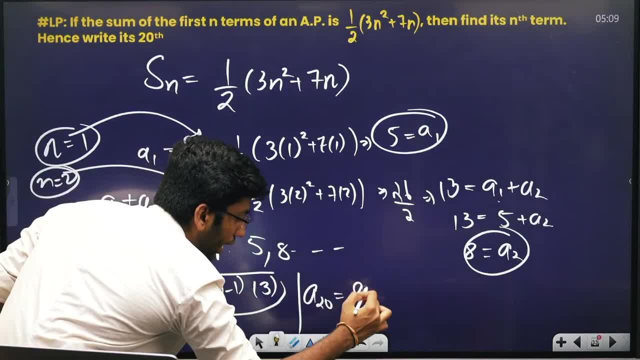 And the 20th term, We have to take out a20.. So what will a20 be? a plus 20 minus 1 into d? So what is a? 5 plus 20 minus 1 is 19.. 19 into d is 3.. 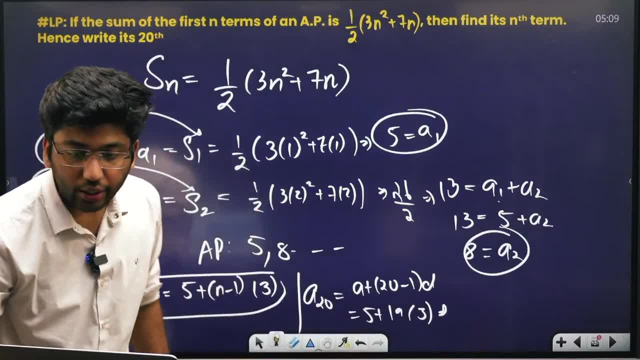 So 19 into 3.. 19 into 3.. 19 into 3 is a. 19 into 3 is a. 9 into 3 is 27.. 3 into 3 is 45.. 57.. 57 plus 5.. 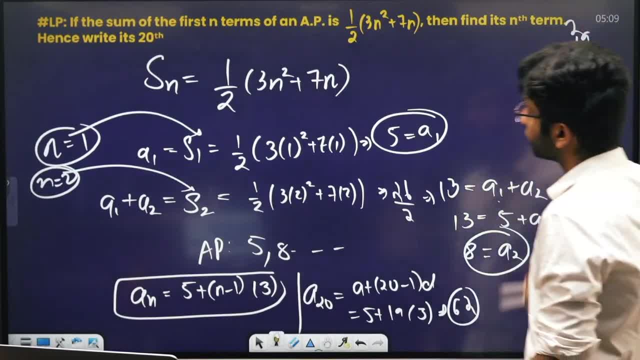 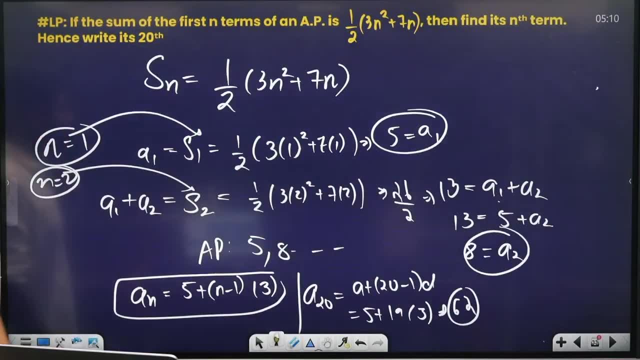 57 plus 5 is 62.. This is your 20th term. 62 is your 20th term, Okay, Okay, Okay. So whenever you get such a question, I am telling you the method of the question, How to do it. Whenever you get such a question. 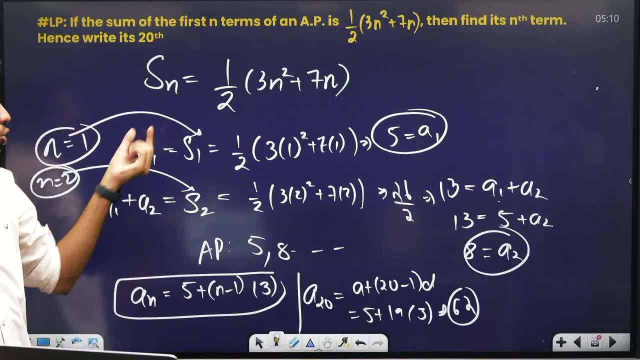 That it is given like this. So if you put n value 1. So a1 plus a2.. So a1 plus a2.. So you will get the answer. S1 will not be a1. Because the sum of the first is a1.. 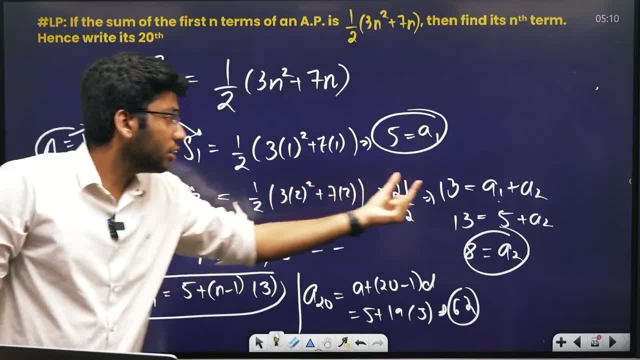 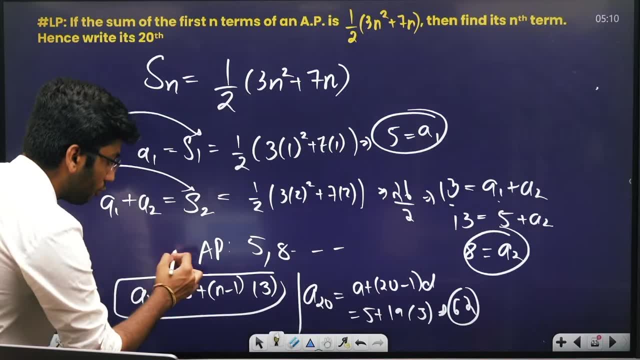 So you will get s1, a1.. If you put n value 2. Then you will get s2.. s2 means The sum of the first and second. So if s2 is 13.. So the sum of the first and second is 13.. 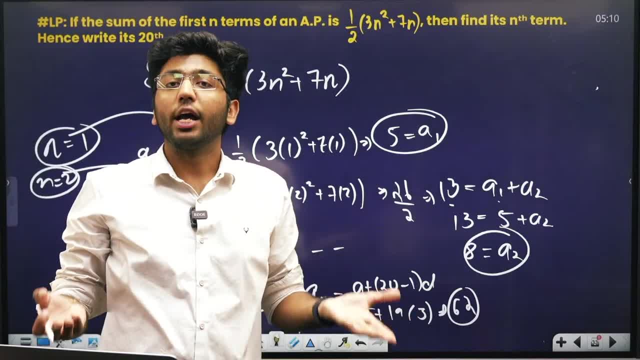 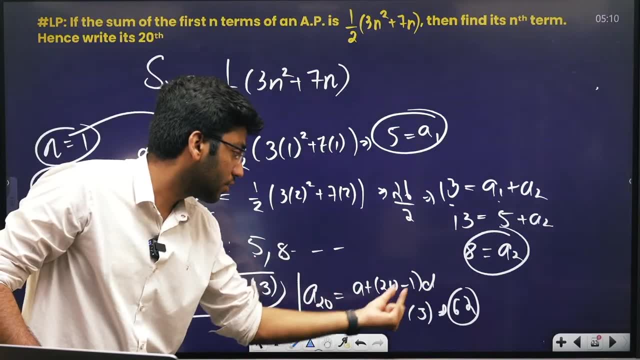 And the first is 5.. So what is the second? 8.? So our ap is 5 and 8.. If you ask 28th term, then A plus 20 minus 1 is D, So A is 5,, 20 minus 1 is 19,, D is 3.. 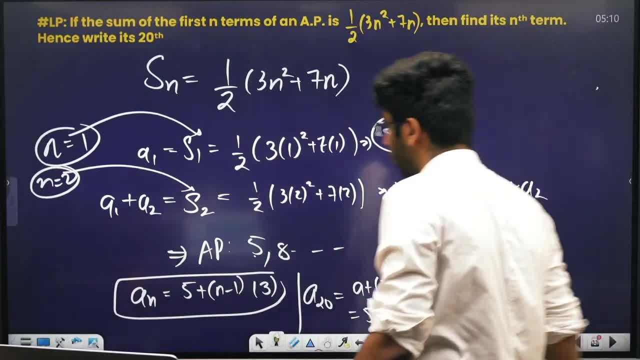 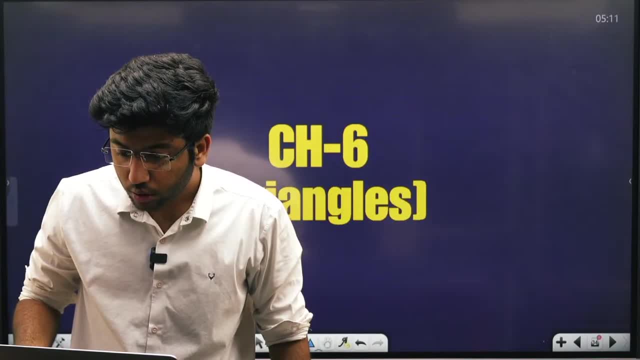 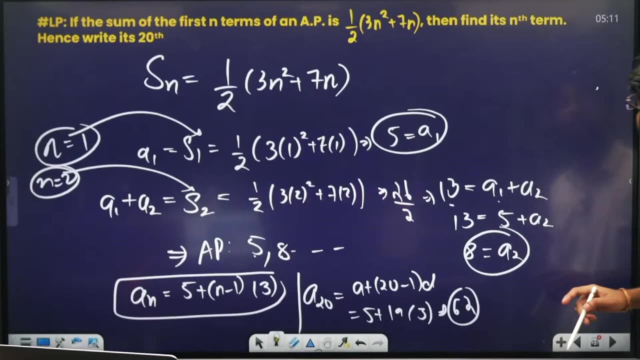 The answer is here: Okay, Okay. Next question: You are writing everything wrong, wrong, wrong, wrong. What table doesn't come? Stop, Stop, Where, Where, Where, Where? 19,, 3000.. 9,, 327,, 3003.. 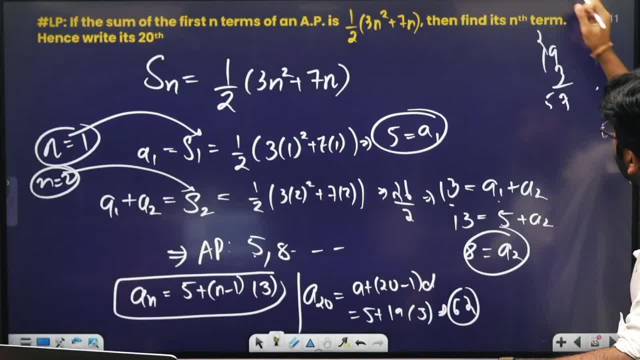 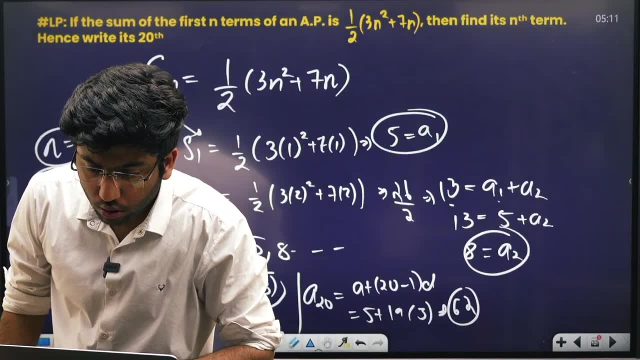 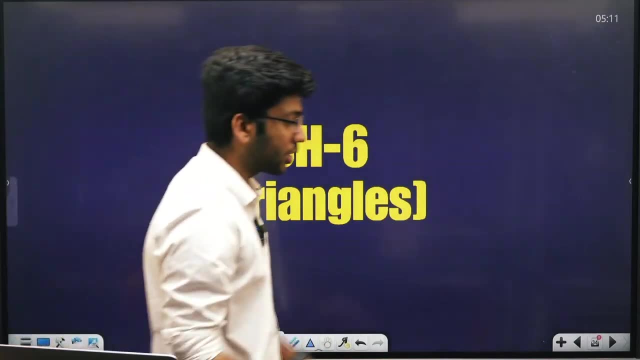 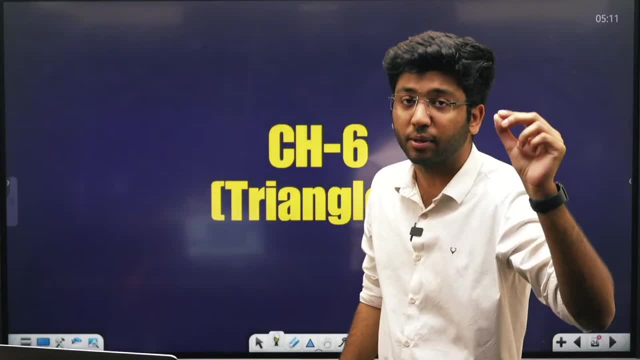 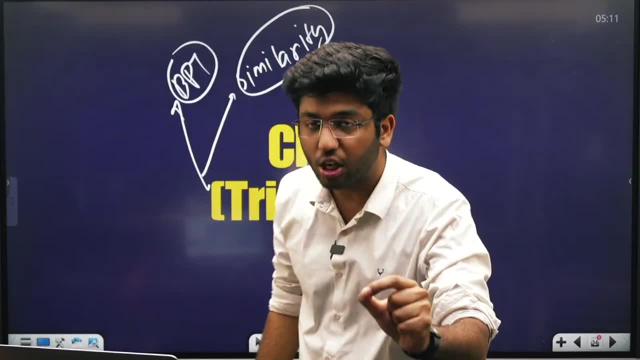 So whenever you get stuck in the question of triangle, whenever you get stuck in the question of triangle, then write either BPT or similarity in the next, Whenever you get stuck in the question of triangle, write in the next either BPT or similarity. 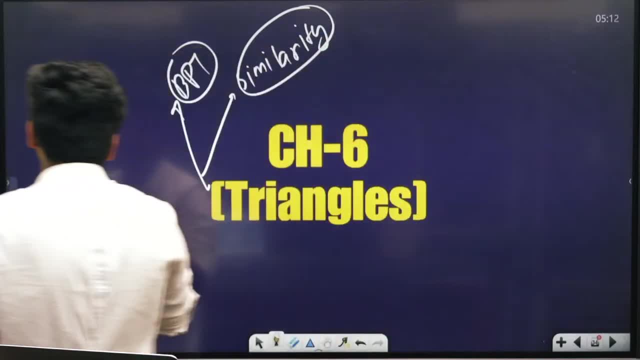 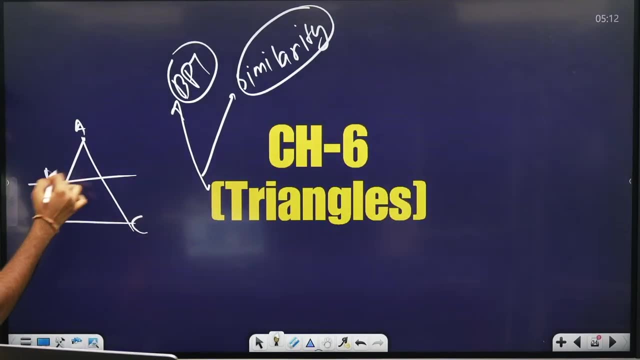 Either it will be solved with BPT or similarity. What does BPT say? BPT says that if there is a triangle and this line is parallel, then in triangle, ABC, which is the DE line, which is DE if it is parallel to BC. 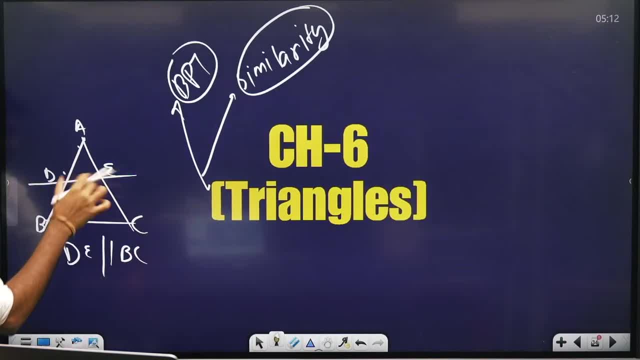 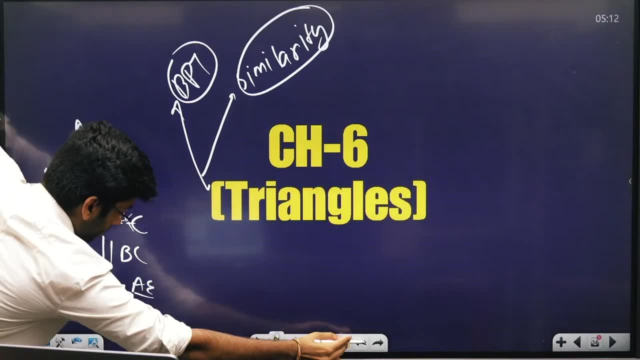 if one line is parallel to any side. So small by small is equal to small by small, means AD by DB is equal to AE by AC, AE by EC. This is BPT. If it is parallel then it will be proportional. 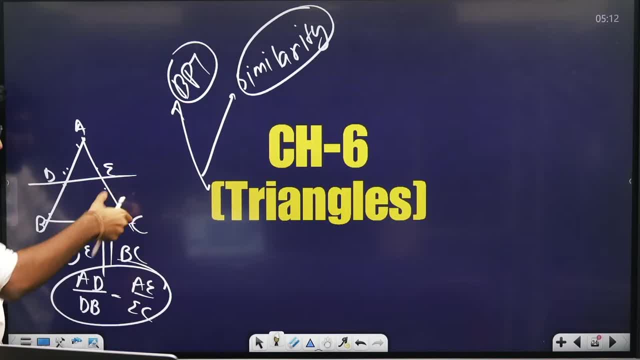 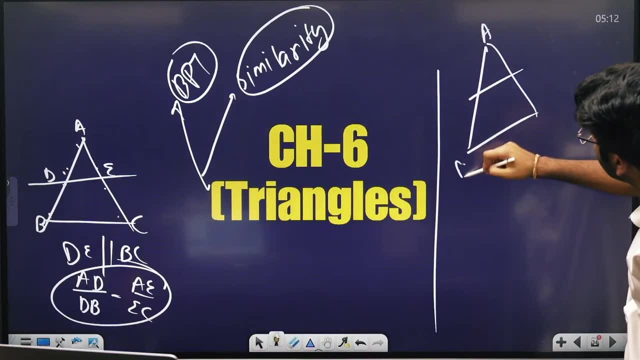 If it is parallel, then AD by DB is equal to AE by EC. This is it, And if proportional is given, what is given to you- A, B, C, D, E- If AD by DB is equal to AE by EC, then it will be parallel. 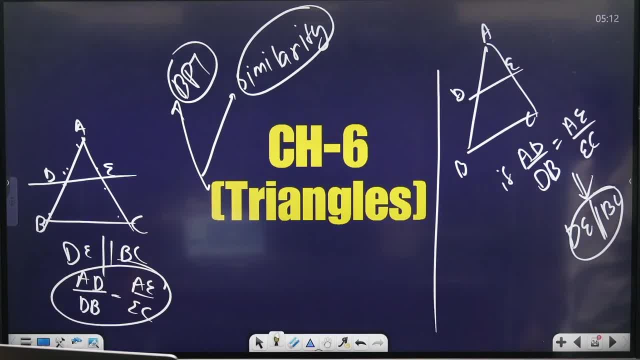 Means DE is equal to BC. This is called Converse of BPT, Converse of Basic Proportionality Theorem. What did I say? If it is parallel DE, parallel BC, then small by small is equal to small by small. 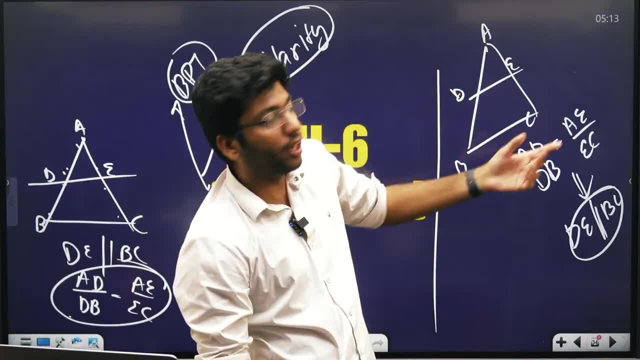 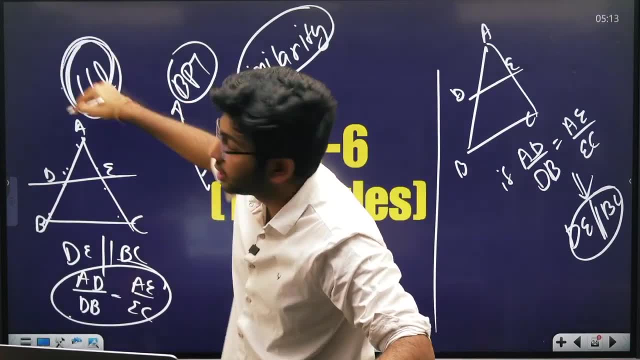 And if small by small is equal to small by small, then DE, parallel, BC. So if you are given parallel, then you will use BPT. Parallel is given. It is very important. Whenever parallel is given in triangle, use BPT. 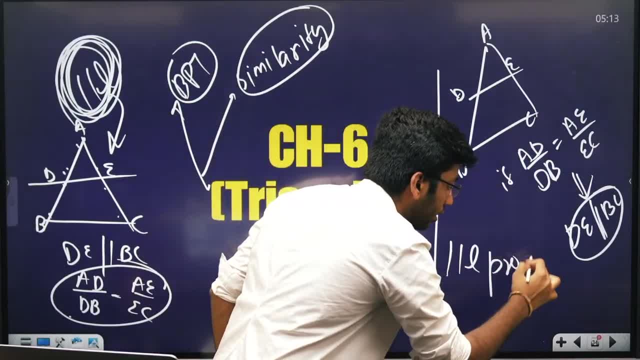 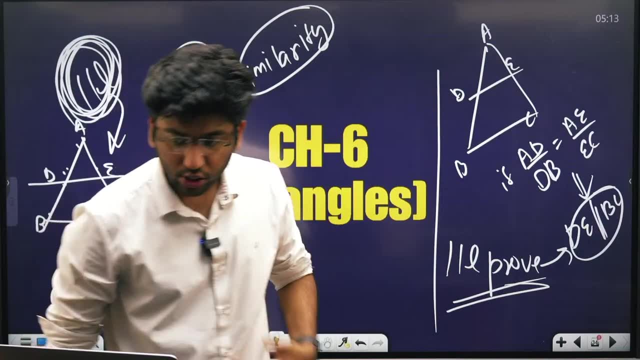 And parallel is to be proved. What Parallel is to be proved? Converse of BPT. So we will use Converse of BPT. So we will use Converse of BPT. Okay, So we will use Converse of BPT. 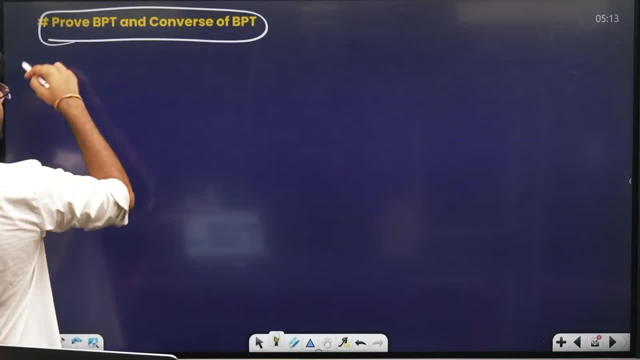 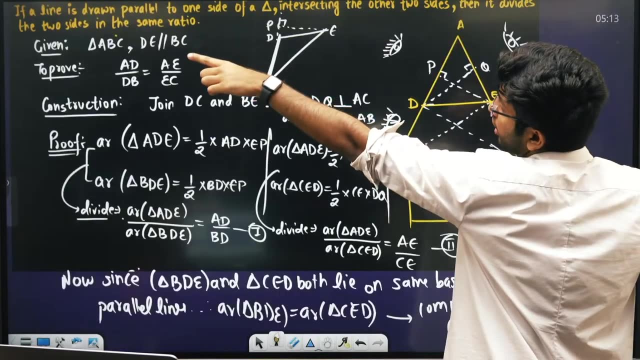 Proof of BPT and Converse of BPT. One of the two will be confirmed. One of the two will be confirmed: Proof of BPT or Converse. We will give you the line of BPT by writing like this: Will write like this: 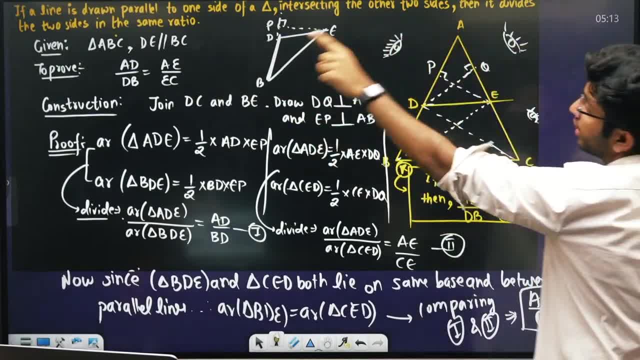 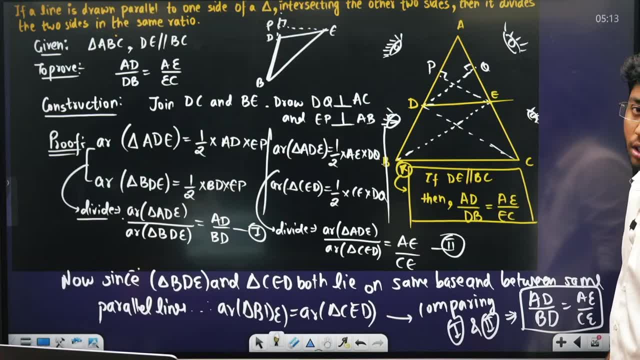 If a line is drawn parallel to one side, intersecting other side, then it divides the two sides in same ratio. It will say from you like this: If this line is parallel to it, if this line is parallel to it, then this ratio will be proportional. 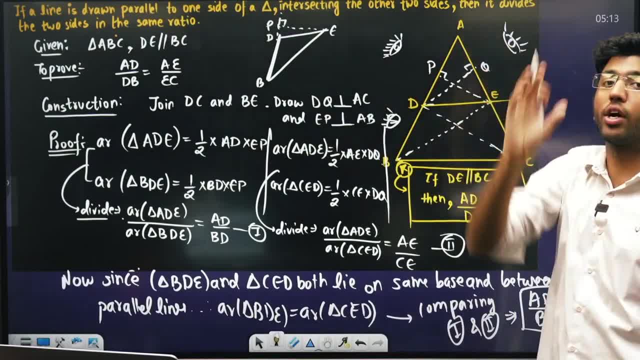 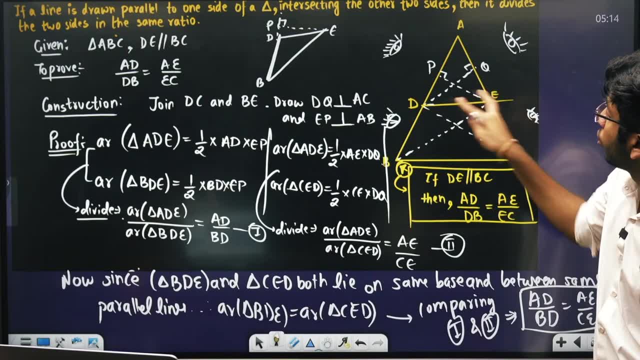 It will write this line like this And it will say: to prove it: If a line is drawn parallel to one side, If this line is parallel to it, which intersects both sides, this line intersects this side and this side and this is its parallel. 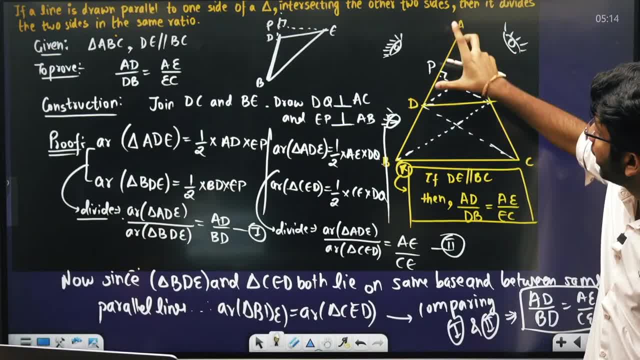 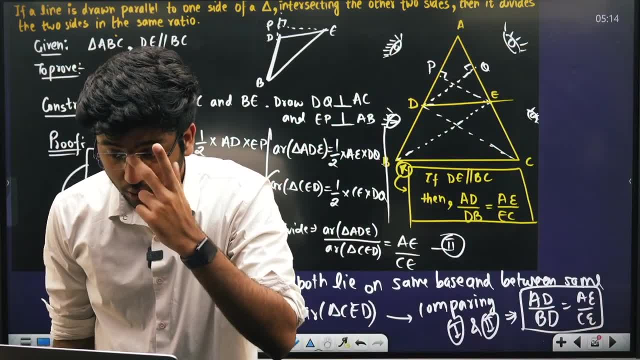 So it divides it in the same ratio. It means AD upon DB, equal to AE upon EC. This has to be proved. I had got its proof done in the marathon yesterday. Okay, Brother, will you give its PDF? I will definitely give it. 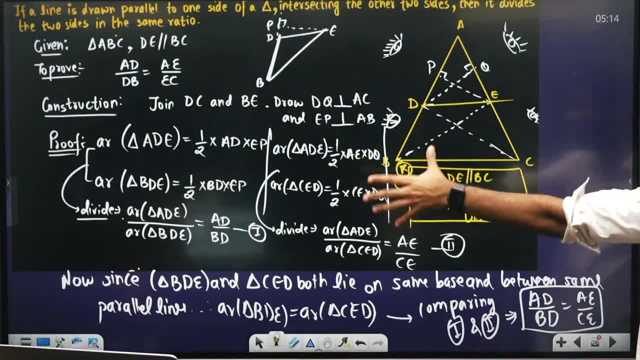 So the proof of this, the proof I had got done in the marathon, I have written that proof here. Okay, I will explain later. It will take a lot of time, So you can see it in the marathon: Maximum children. 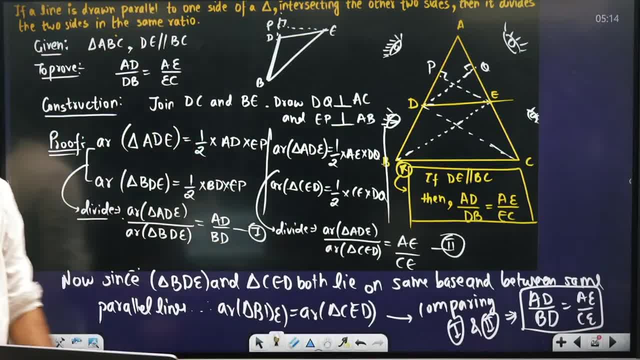 maximum children must have understood. The proof will come Just come after printing this. Just come. after printing this, You can take screenshot. The proof will come Just come after printing this. I will not explain this because it will take a lot of time in this thing. 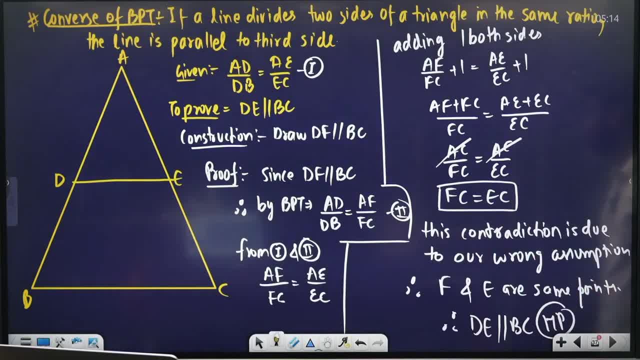 Next question: This is the proof of Converse of PPT. Okay, Proof and Converse of PPT proof: Just come after printing this. If you have time, then see it once from the marathon. Otherwise, just come after printing this. 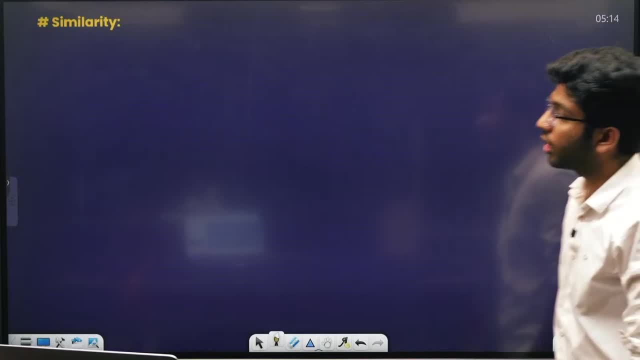 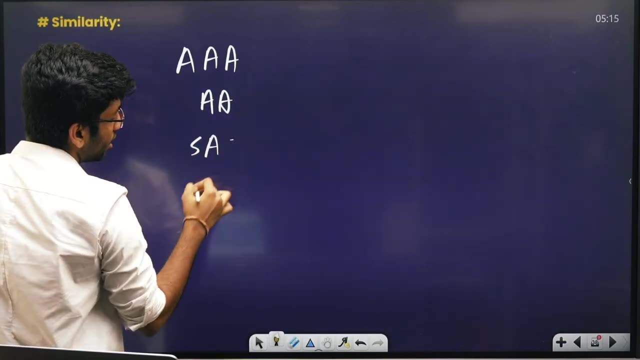 One of the two must come for sure. One of the two must come for sure. Okay, Now let's talk about similarity, Similarity, Four criteria: Angle angle: angle Angle angle Side, angle side, Side side side. 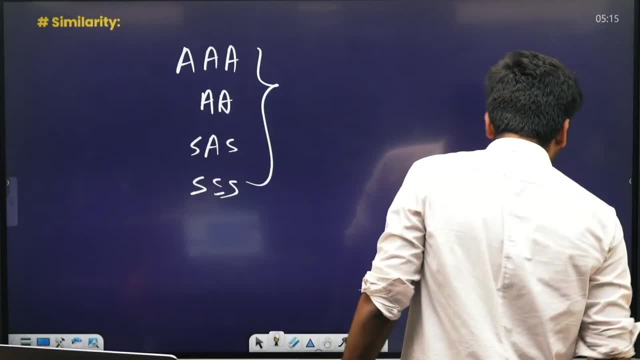 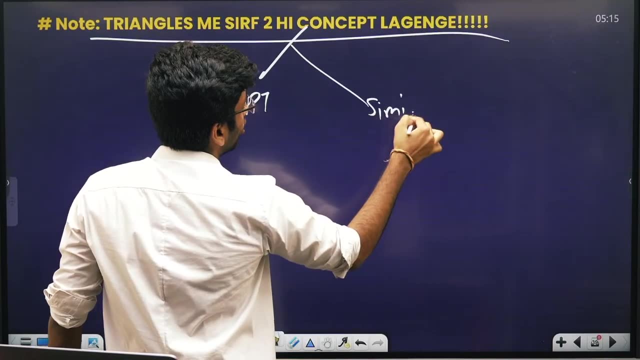 One of these four criteria. you can use one of these criteria. Okay, You know this. Only two concepts will be used in triangle. Either PPT will be used or similarity will be used. Only one concept will be used in triangle out of these two. 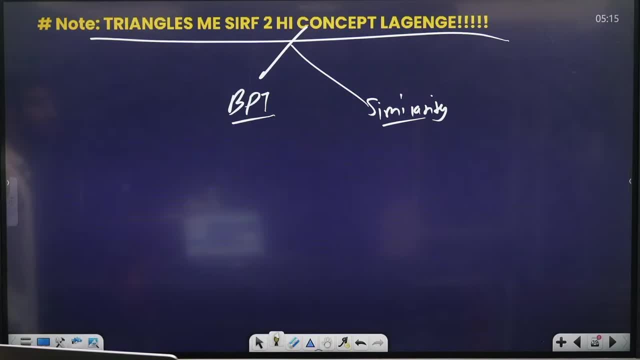 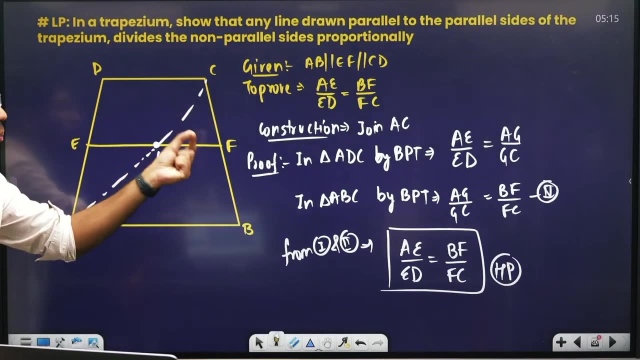 Either PPT or similarity. See See Like a question. Some questions which are very famous questions in this In a trapezium show that any line drawn parallel to the parallel sides of trapezium divide the non-parallel side proportionally. 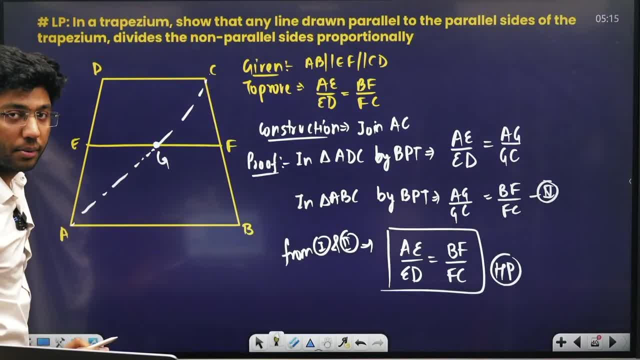 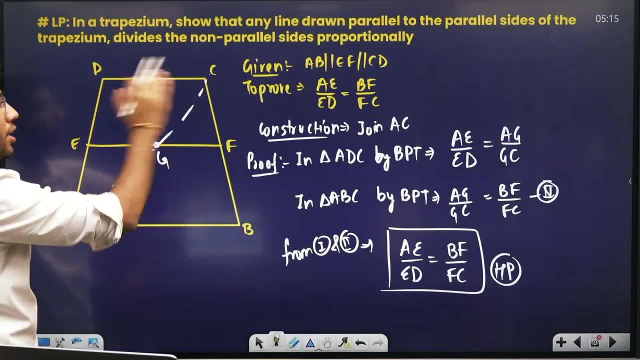 Means this trapezium was ABCD. This trapezium is given to us. This trapezium has told us that this EF is parallel to it. Bro, AB is parallel CD. This is in trapezium. 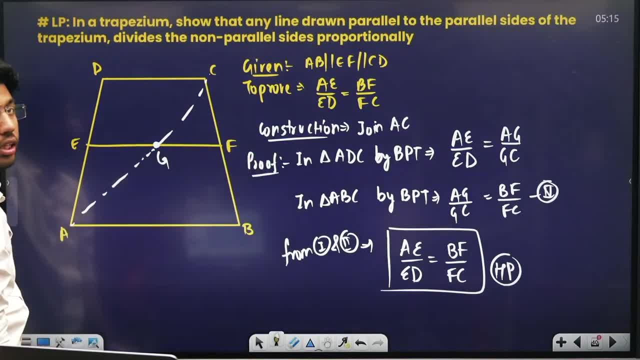 AB is parallel CD. There is one more line which is parallel to it. Means these three lines are parallel to each other. Okay, We have to tell that it will divide non-parallel side proportionally. Means this AE upon ED is equal to BF upon FC. 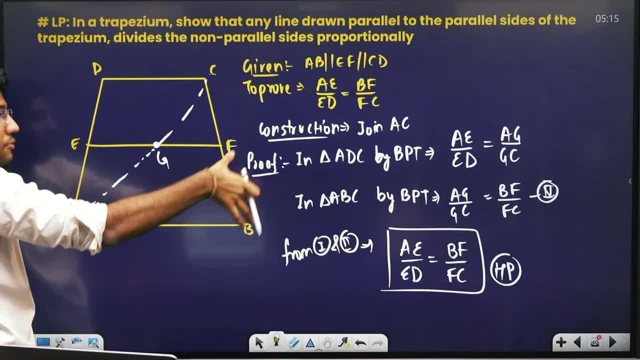 AE upon ED is equal to BF upon FC. AE upon ED is equal to BF upon FC. We have to do this and show Okay. Whenever we have to do ratio proportionally, It will come in my mind that we have to apply BPT. 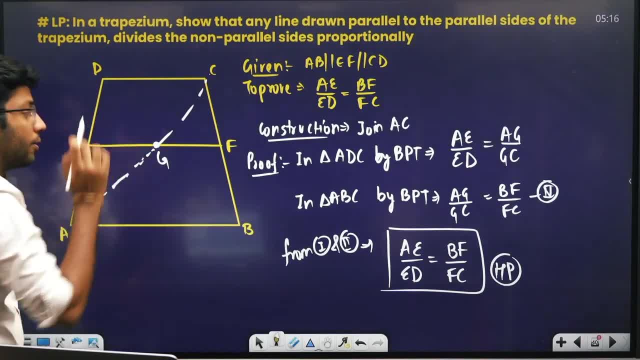 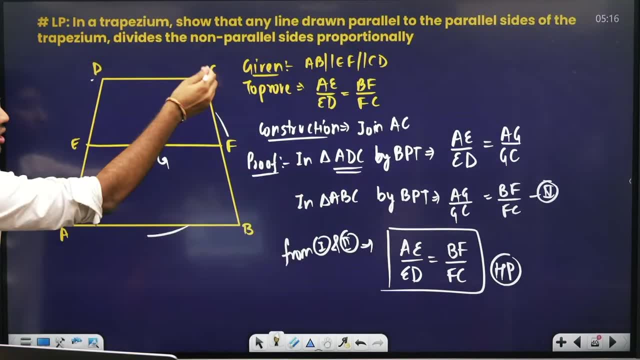 But to apply BPT, I will do construction. So, after doing construction, one triangle is formed. So see In triangle ADC, Which triangle ADC, If we see in this triangle, If we see in this triangle. So this side is parallel to this. 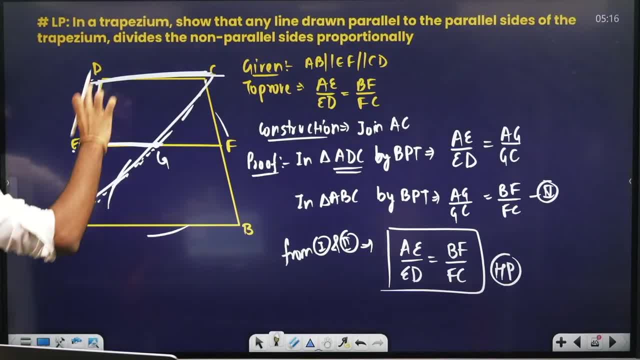 This side is parallel to this. This side is parallel to this. So AE upon ED is equal to AG upon GC. I have written: AE upon ED is equal to AG upon GC. This happened in this triangle, In this triangle. Okay. 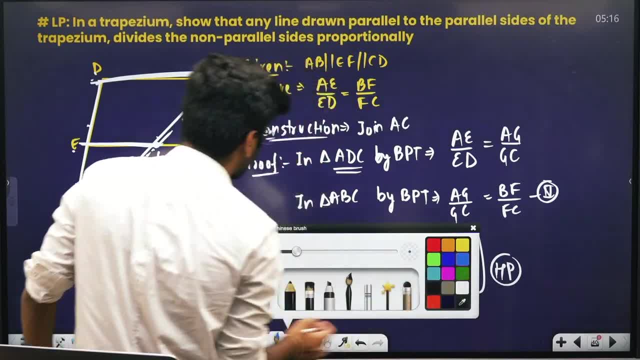 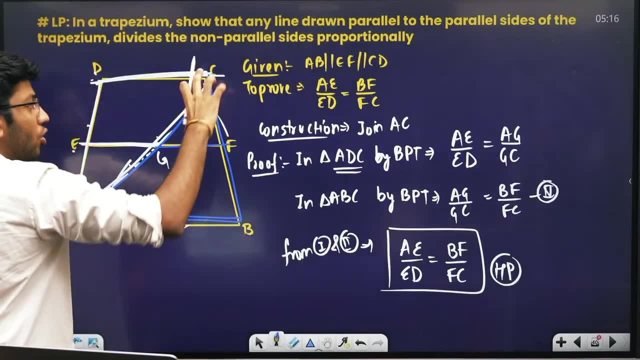 Similarly, if I, Similarly, if I, Similarly, if I talk about this triangle, Which one? ABC, ABC If I talk about this triangle. So this side is parallel to this. So CF upon BF is equal to this upon this. 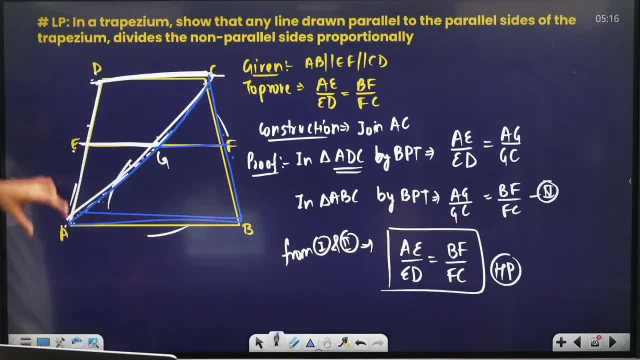 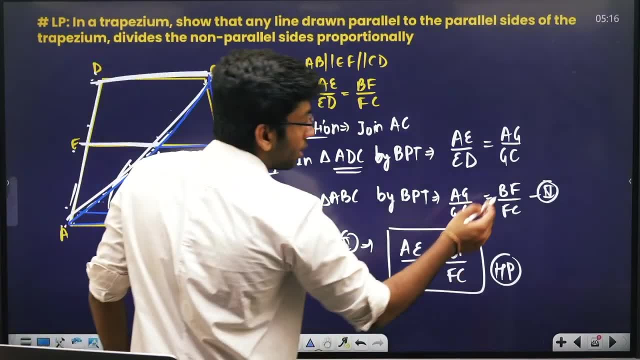 What did I write? AG upon GC Means This: AG upon GC is equal to BF upon FC. I have written this: AG upon GC is equal to BF upon FC. Now see: AG upon GC is equal to this And AG upon GC is equal to this. 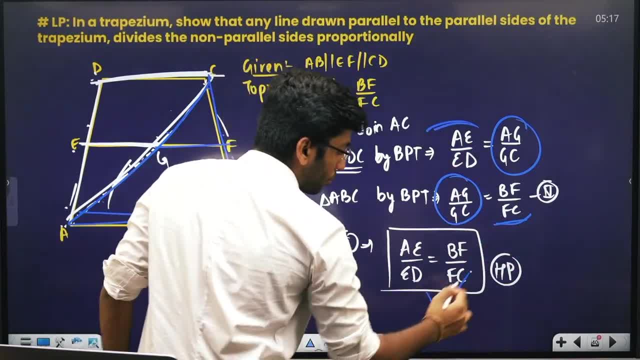 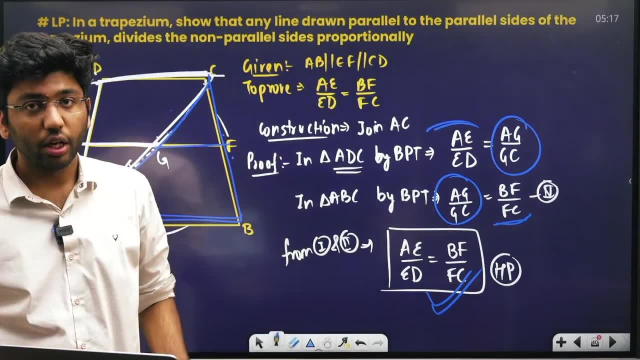 And AG upon GC is equal to this Means This and this are equal to each other. This is what we had to prove. This is what we had to prove, Okay, Okay, Okay Okay. This kind of question will come. 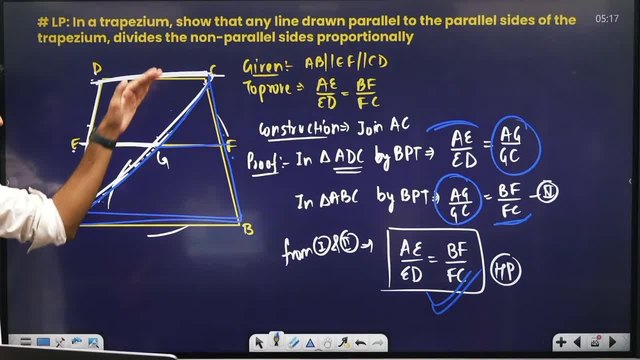 Whenever trapezium question will come: Do construction in between? After construction you will get two triangles. Put BPT in both triangles. The answer will come: Got it? Next question: In the figure There is some kind of figure. 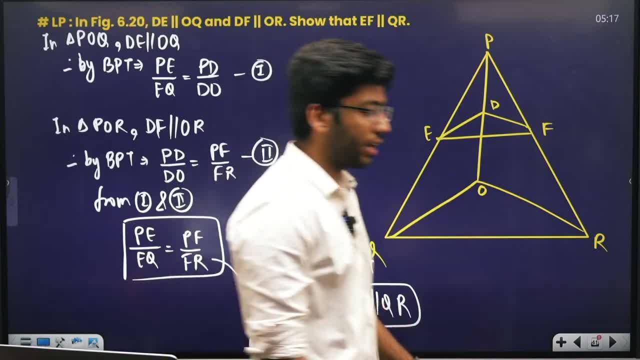 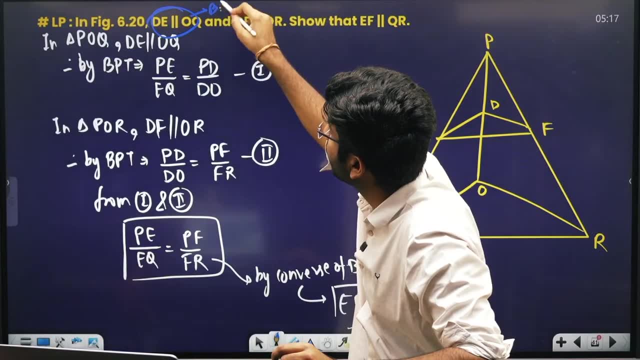 Exactly the same. Look In this figure. I have said DE parallel OQ. So if the parallel is given in the triangle, In my mind I have written DE parallel OQ, DE, parallel OQ, DE. DE is the parallel of OQ. 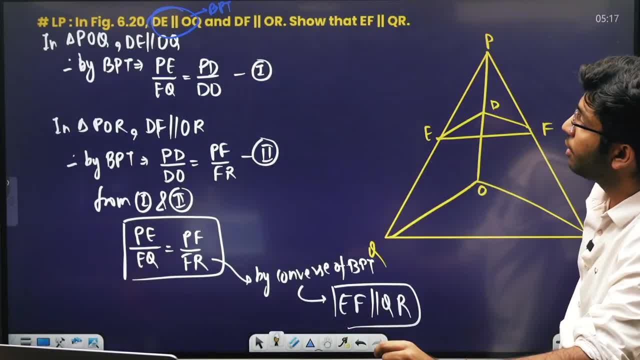 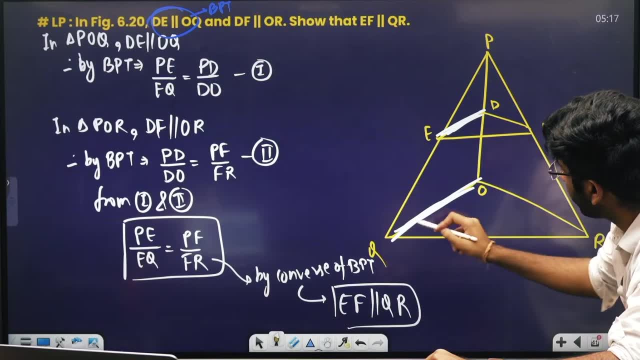 So DE side is the parallel of OQ side, Means In this triangle I will put BPT, Which In POR, Look In POR and in POQ. First I will put in POQ, POQ In this triangle. 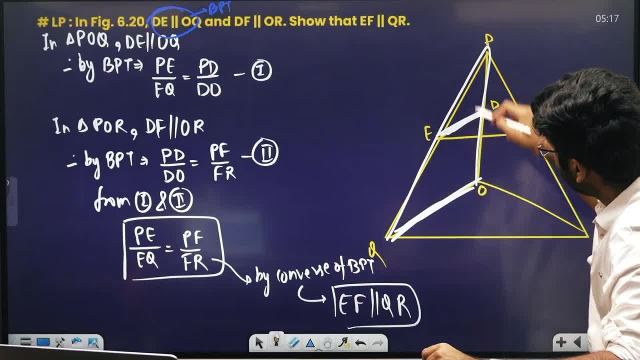 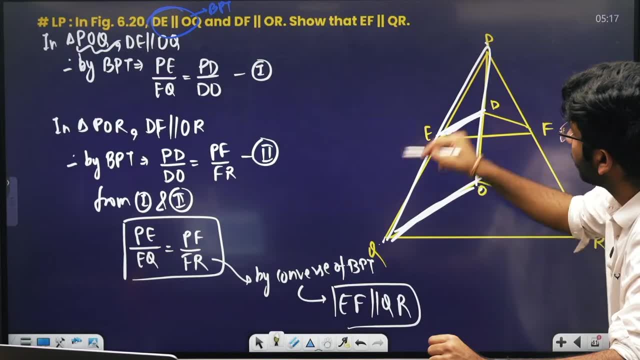 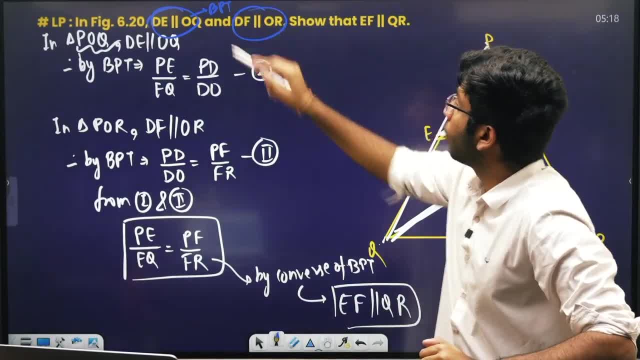 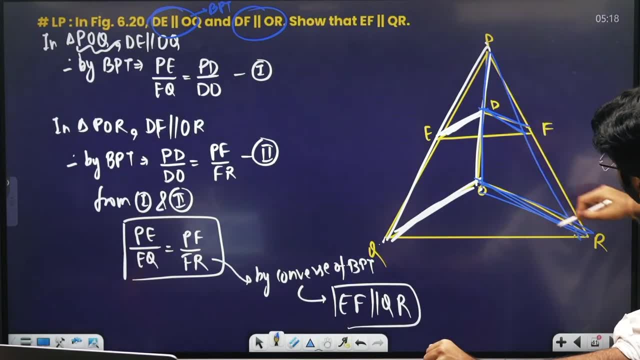 POR, POR, POR, POR. EVEN. directly TUE for DO, We will say POR. Okay, See you, That's same In this happens. So then I will put PPT: mettokam Now. Now I will put PPT. 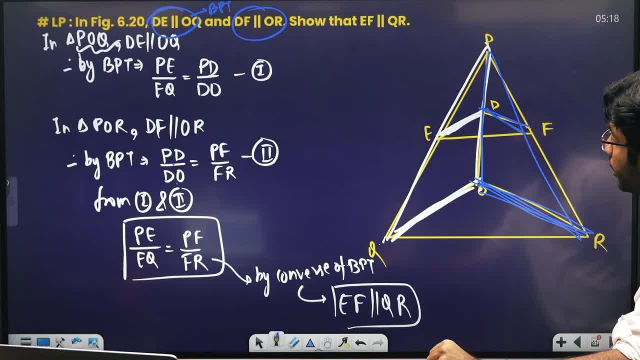 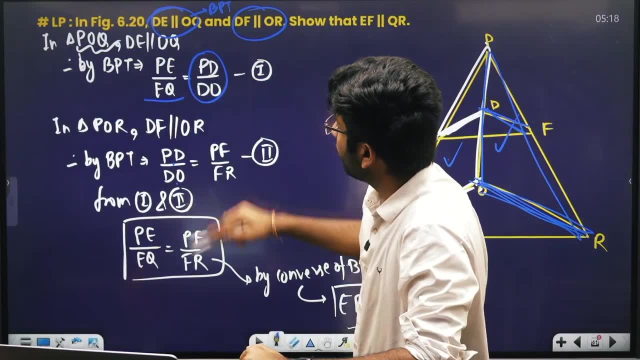 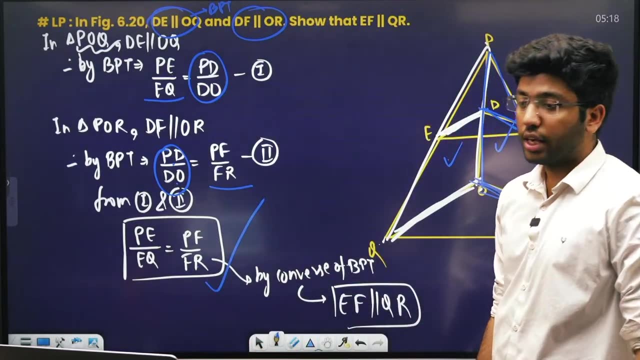 missions done at this triangle. Di, you are never giving money. I only give to you Dev OOaxay, All I give. Yeah, In this triangle He put four dollars. Yeah, Why No? Now Look What is this? This is the answer. This is the answer I had to prove: the parallel EF, parallel to QR. 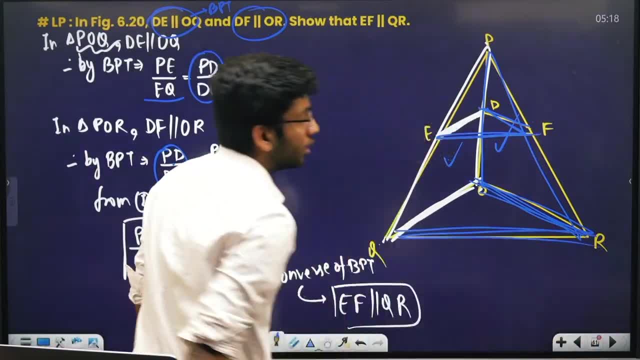 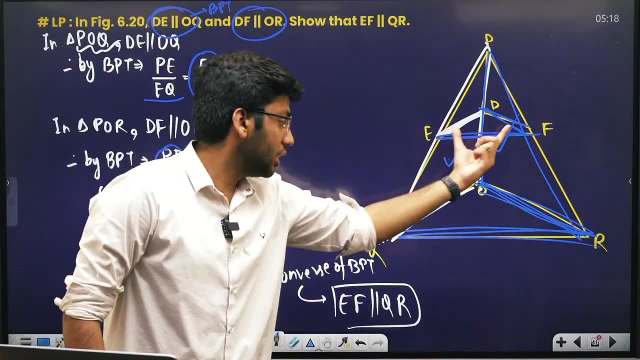 I had to do EF parallel to QR. So see, if I had given the parallel, then I applied BPT. If I want to prove the parallel, then I will apply the converse of BPT. So if I want to do the parallel of EF- QR, then I have to do PE upon EQ equal to PF upon FR. 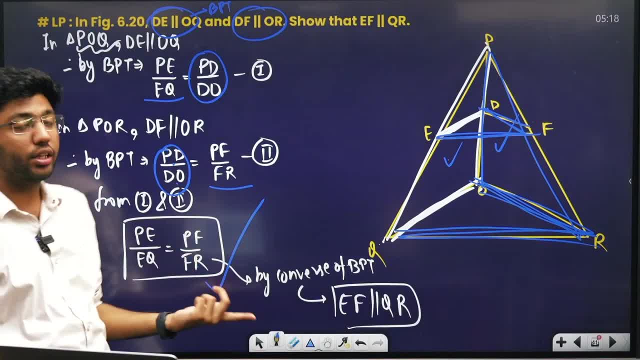 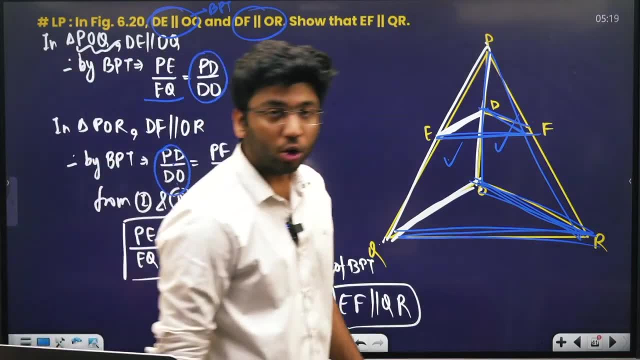 I have done the same: PE upon EQ equal to PF upon FR. So if I do this, then by converse of BPT, EF is parallel to QR. This is a very nice question. CBC asks this. This is a very nice question. CBC asks this. 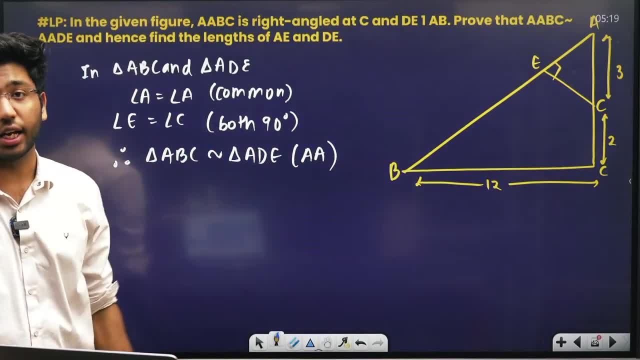 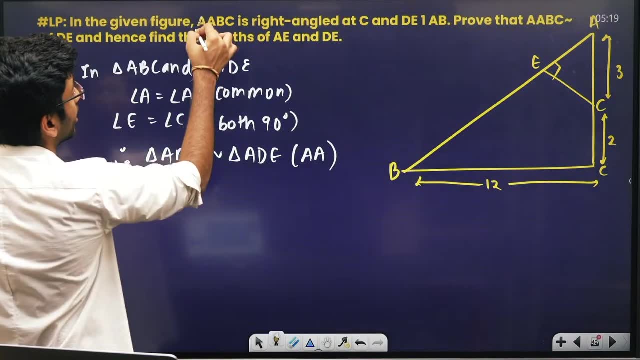 I am going fast, We don't have much time, So I have already written all the questions for you, See. See, It is written in the given figure. Triangle ABC is right triangle. This triangle is written. Triangle ABC is a right angle. triangle ABC is ABC. This is right angle triangle. Okay, 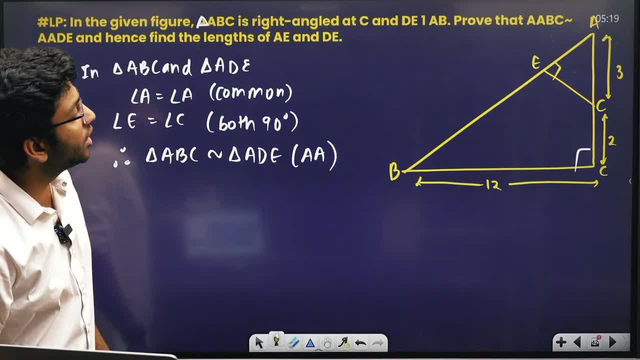 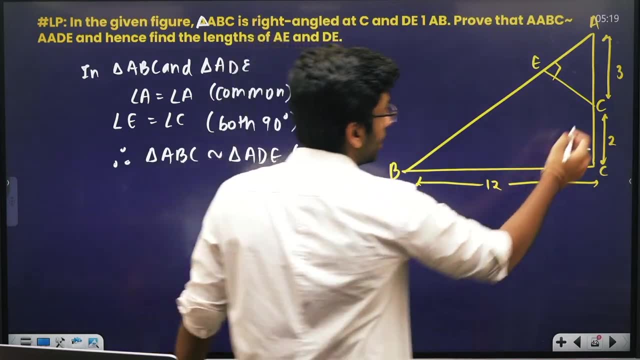 Right angle at C. Okay, DE is perpendicular to AB. Where is DE? DE? Not DE, This will be CE. Yes, This is D. This point is D. So DE is perpendicular to AB. It is written perpendicular, Perpendicular to AB. 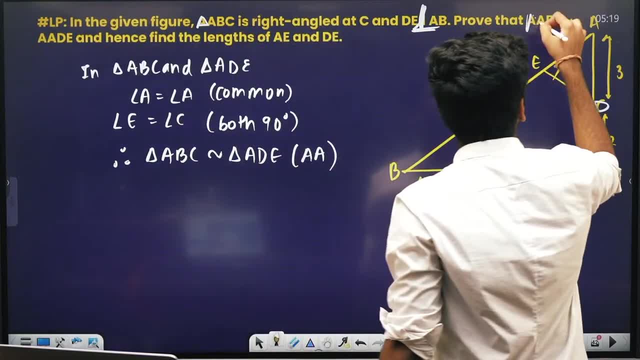 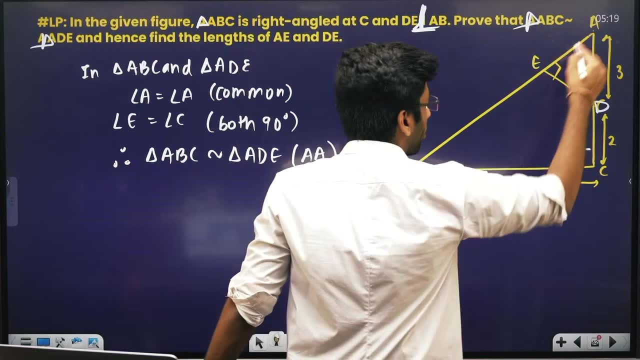 This DE is perpendicular to AB, Proof that triangle ABC, Proof that triangle ABC. So ABC is a big triangle. This is similar to triangle AED. This triangle is similar to ADE, So we have to say that this triangle is similar to this small triangle. 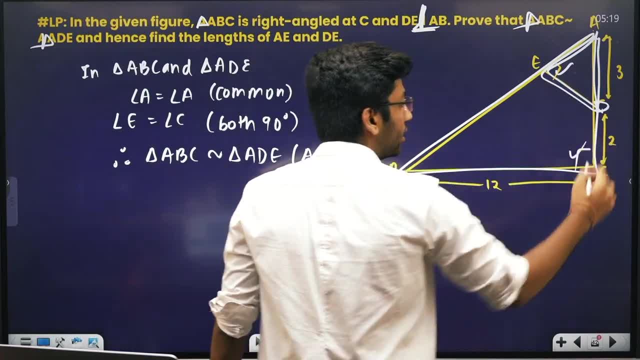 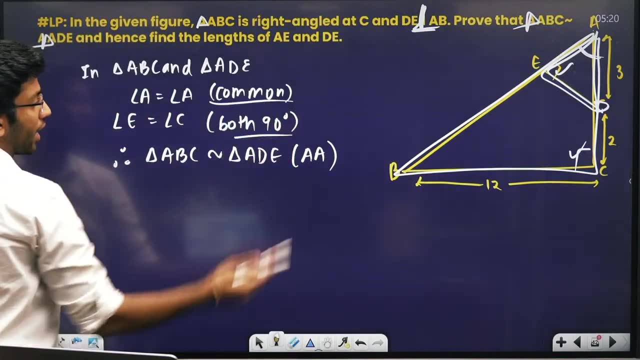 How will you prove? See, This is 90.. This is 90.. Both are 90.. And this angle is common in both, Common in small and common in big. So both are 90 and angle is common. So what happened? Both are similar in angle and angle similarity. 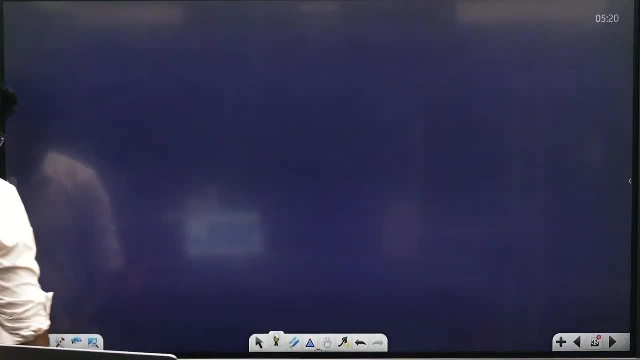 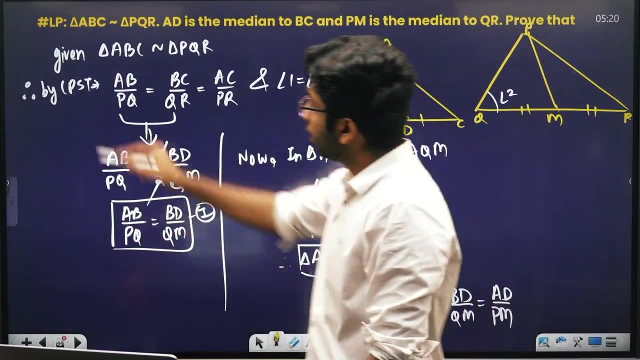 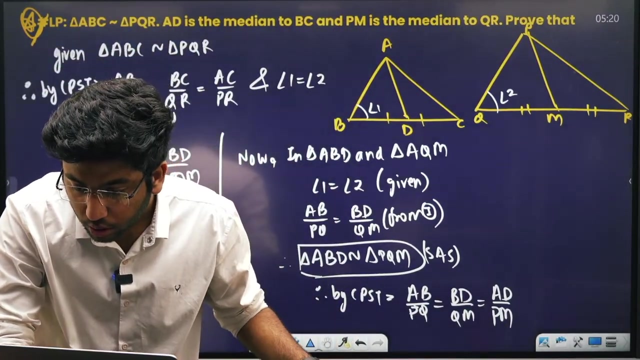 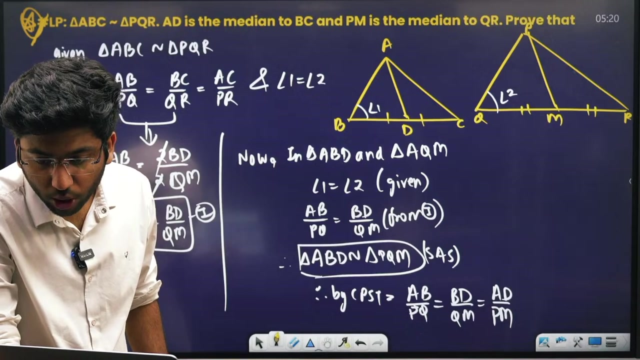 So these small questions are directly asked from you. Okay, These small questions are directly asked from you. Medium question- Medium question. I told you yesterday Medium question can be seen. Medium question can be seen. Medium question can be seen. Spam for upstream- downstream. I would have made you do upstream, downstream yesterday. 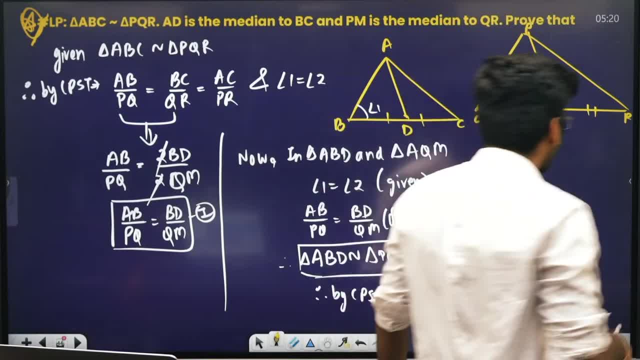 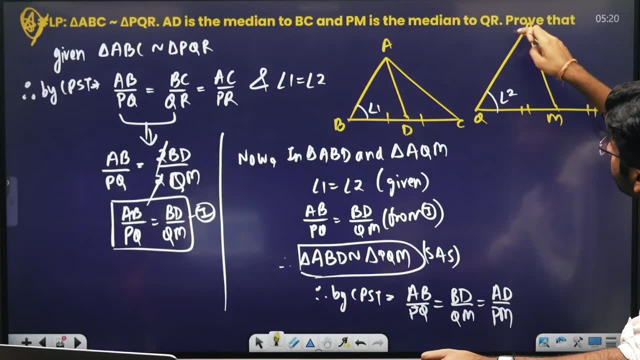 I would have made you do it the day after tomorrow. What are you talking about? See If triangle ABC is similar to PQR, This ABC triangle is similar to PQR. ABC triangle is similar to PQR. As soon as I came to know that ABC is similar to PQR. 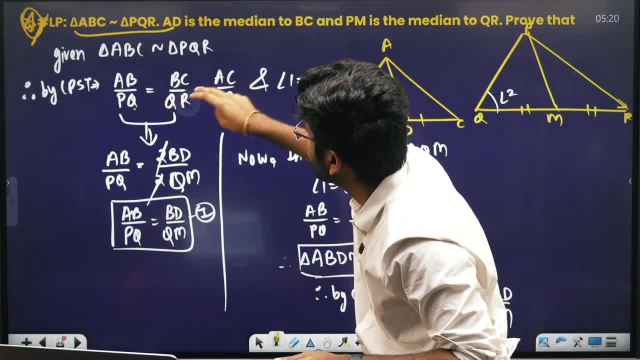 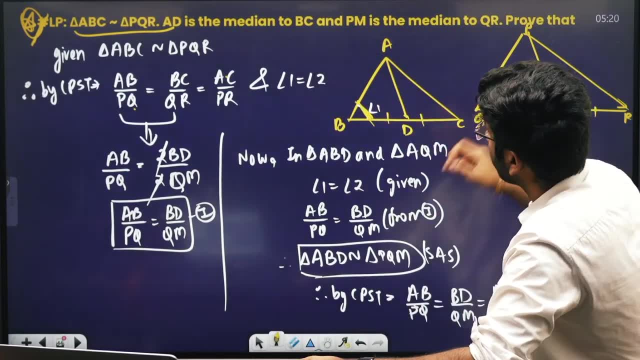 I wrote CPCT AB upon PQ, equal to BC upon QR, AC upon PR. I wrote it earlier And I wrote angle 1 equal to angle 2.. Angle 1.. Angle B equal to Q. I wrote angle B equal to Q. See, Angle B is in the middle, Q is also in the middle. 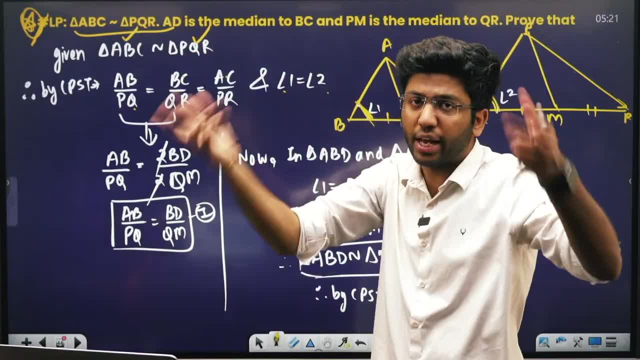 So I wrote angle 1 equal to angle 2.. So as soon as I know that it is similar, As soon as I see similar, Whenever you see similar in triangle- So assume, Start dancing- That I have given similar- I will write CPCT. 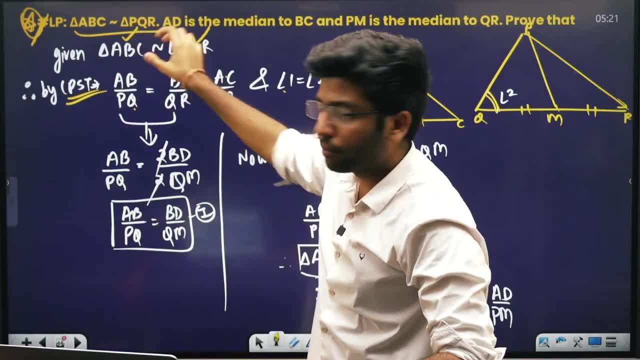 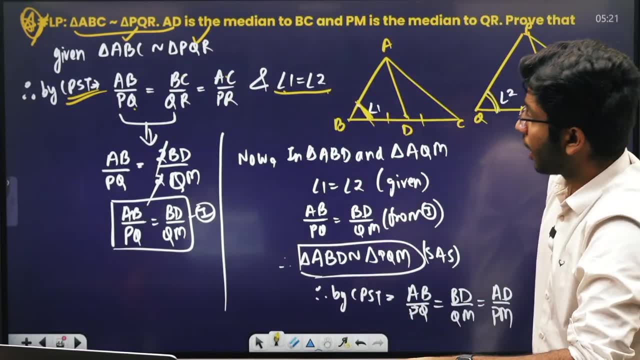 I have given similar, I will write it with CPCT. So I gave similar, I wrote this with CPCT. What AB upon PQ equal to BC upon QR. I wrote this: And angle 1 equal to angle 2.. I did this Now, see, Now it came to my mind that what I have to do 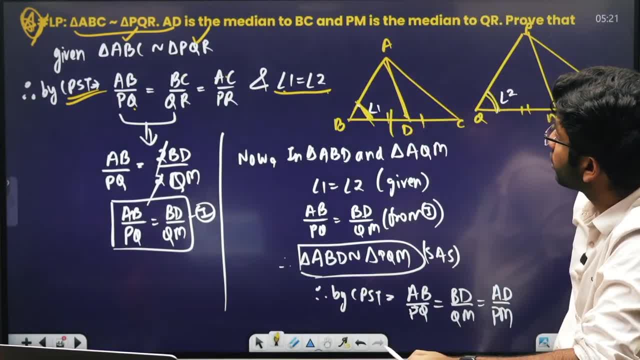 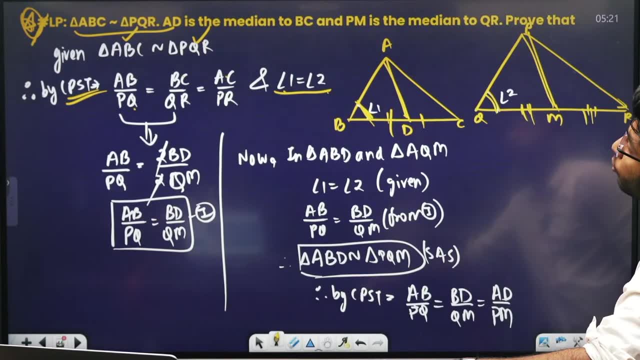 AD is median. Median means It will divide the side in the same ratio. PM is also a median Means it will divide the sides equally. Proof that. Proof that. What proof did we have to do? We had to do the proof. AB Yes. 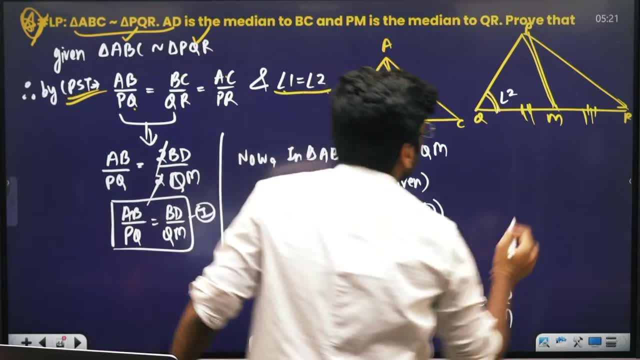 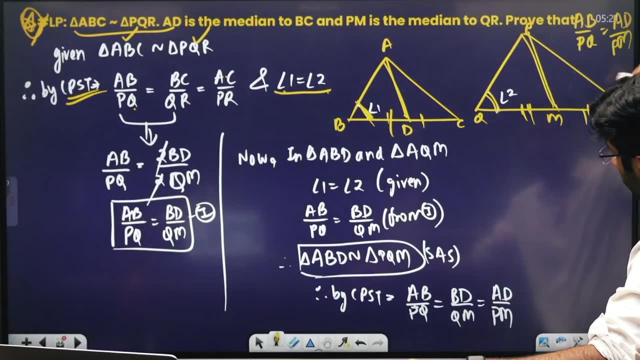 We have to do the proof, Proof that It is not written beyond, proof that Who made this slide? So proof that We have to do the proof. AB upon PQ equal to AD upon PM. We have to prove this. AB upon PQ equal to AD upon PM. What AB upon PQ equal to AD upon PM? 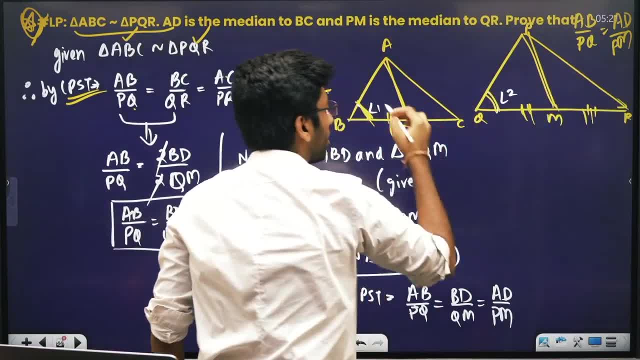 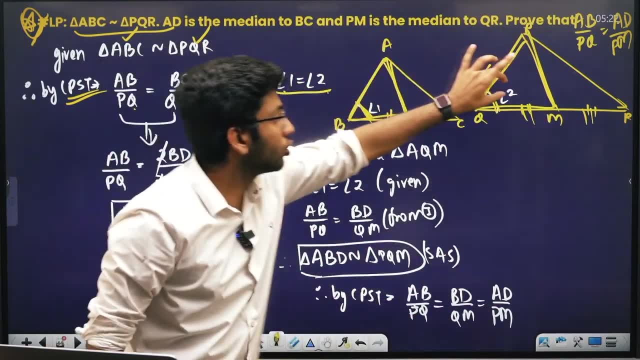 We have to prove. So means This triangle is given similar. If I somehow show this small triangle also similar, So AB upon PQ equal to AD upon PM. So I have to show this small triangle similar. So what did I do? What did I do See, See, Look carefully now. 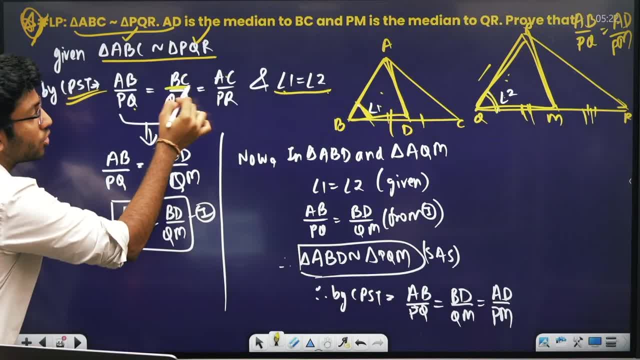 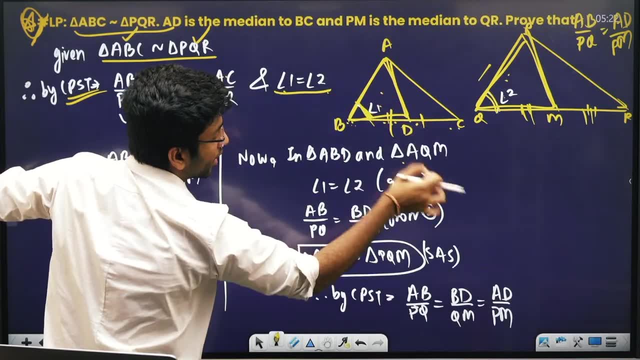 The relation I got from the given similar The BC, The BC side, BC side. I wrote this twice of BD Because BD and these two are equal. These two are equal, It is median, So these two are equal. So I wrote this whole BC twice of BD, Twice of BD. 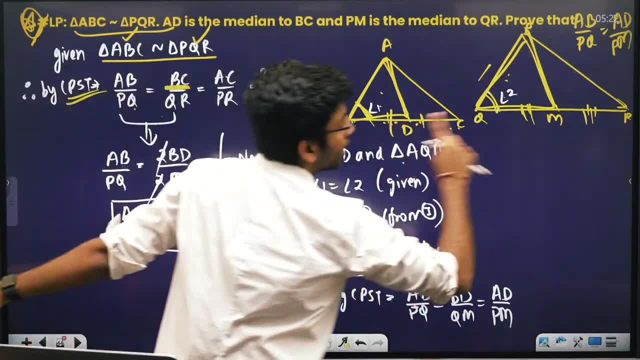 Wrote this twice of BD. Wrote this twice of BD. Wrote this whole QR. Wrote this whole QR twice of QM. Wrote this twice of QM. Cut So AB upon PQ, equal to BD upon QM. 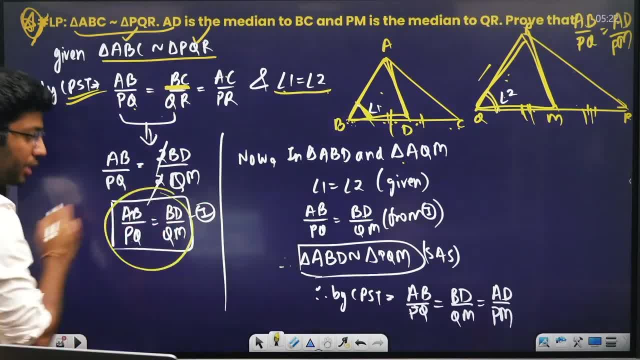 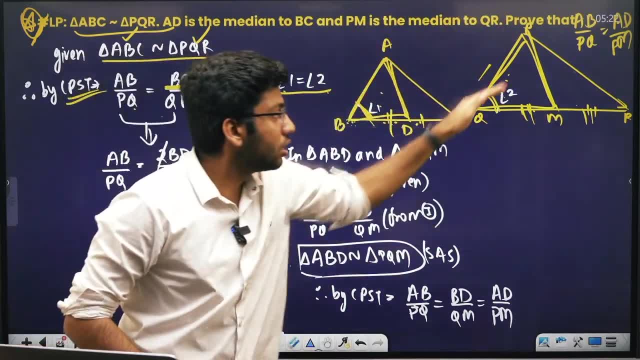 It was given similar. It was written: AB upon PQ equal to BD upon QM Means AB upon PQ equal to BD upon QM. This came. So this side, This side, And the middle angle was equal. The middle angle was equal. So with side angle, side similarity. 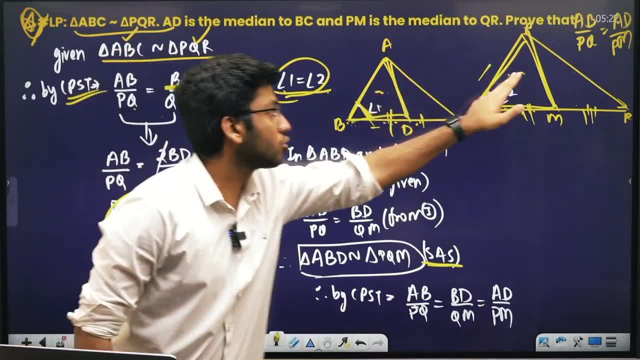 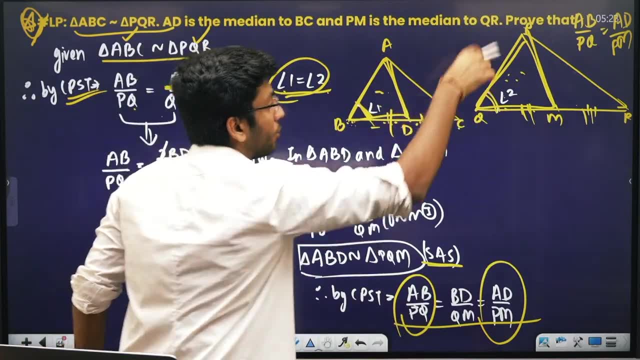 I made this triangle similar to the smaller one As soon as I made the smaller one similar to the smaller one. So I wrote CPST And from CPST I got AB upon PQ equal to AD upon QM. AB upon PQ equal to AD upon QM. I got this: 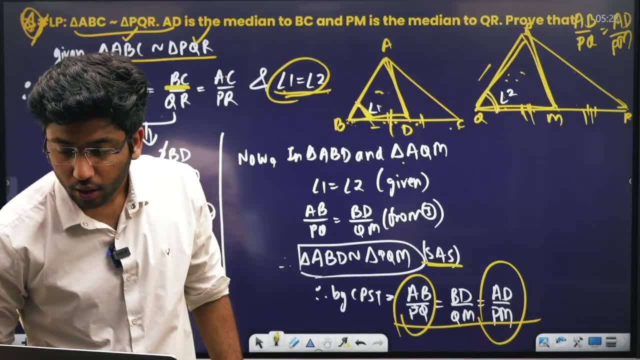 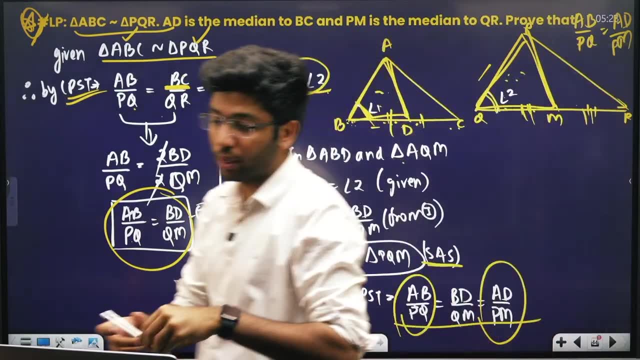 Okay, Okay, Pass it. Write the question that I am asking. Understand it. well, It will pass, Pass, Pass. You will get to see all the questions from this. Write it quickly. Write it quickly. Who wants to write? Who wants to understand? 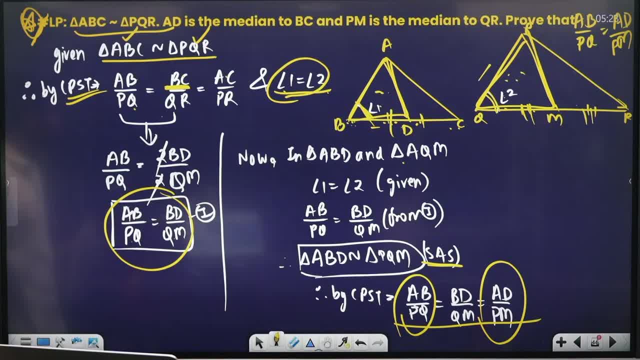 Look quickly. I didn't do anything. I had given a big triangle similar. I had given a big triangle similar. I made the smaller triangle similar to it. I got the answer. I had given a big triangle similar. I made the smaller triangle similar. I got the answer. 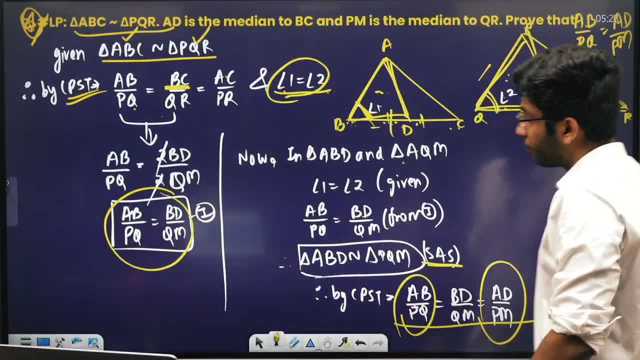 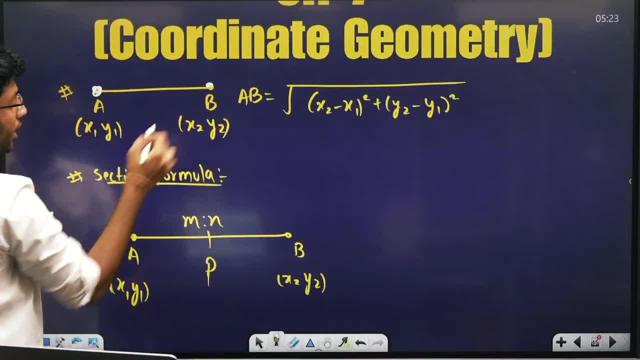 Okay, Next question, Next question, Next, If we come to coordinate geometry, Coordinate geometry, Three concepts, Distance formula: What is AB distance Square root of X2 minus X1 square plus Y2 minus Y1 square? Very important, Very important. 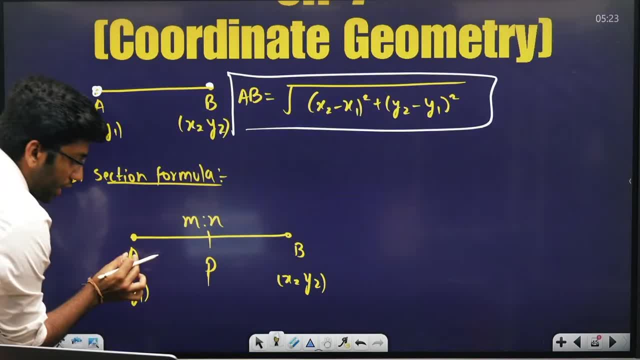 There must be a question from this Section: formula: What: There is AB point. There is AB point. If this P point is dividing it into M, ratio, N, Then how will you write P point? Tell me, how will you write. Tell me, how will you write. 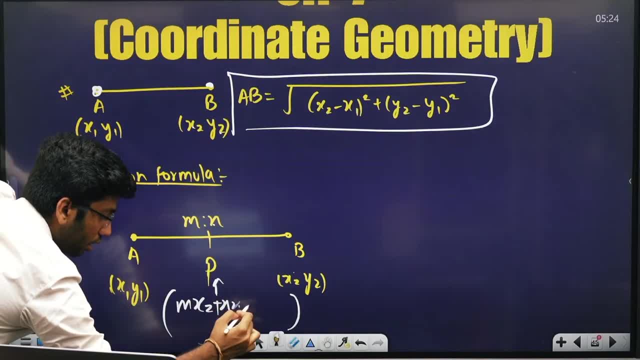 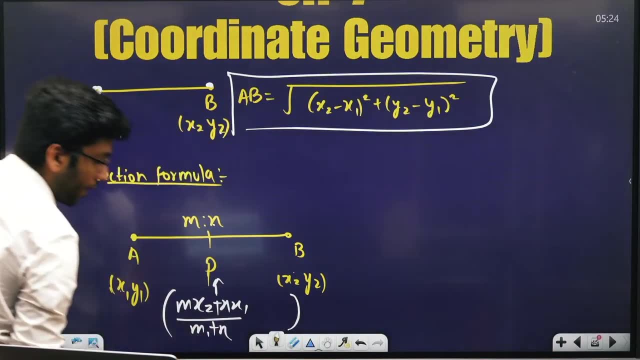 MX2 plus NX1 upon M1 plus M2.. This will happen. M1 plus M1.. M plus N, M plus N will happen. This is its Y coordinate. How will you write X coordinate? MY2.. MY2.. 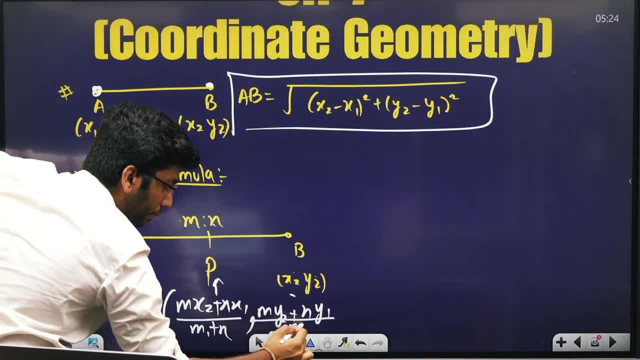 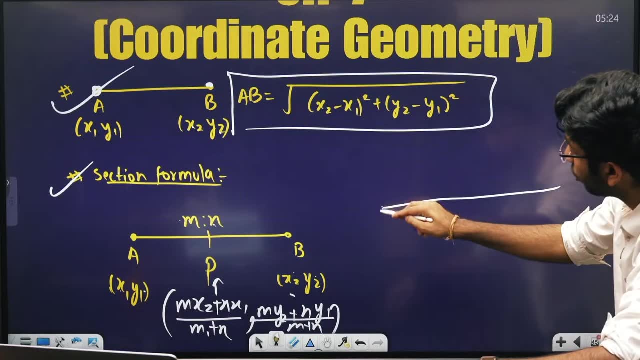 Plus NY1.. NY2.. Y1 upon M plus N. This is the section formula, Section formula And this is the distance formula. The question is asked in this way: Tell me There is AB point. There is AB point. 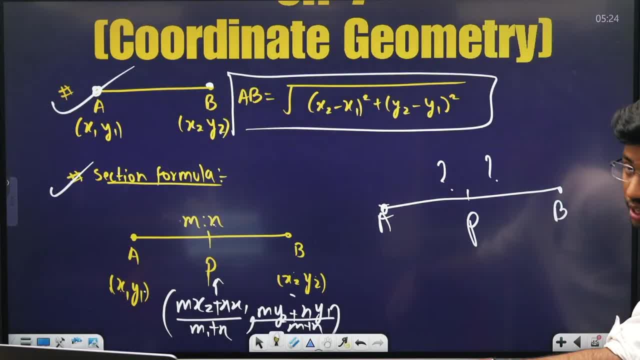 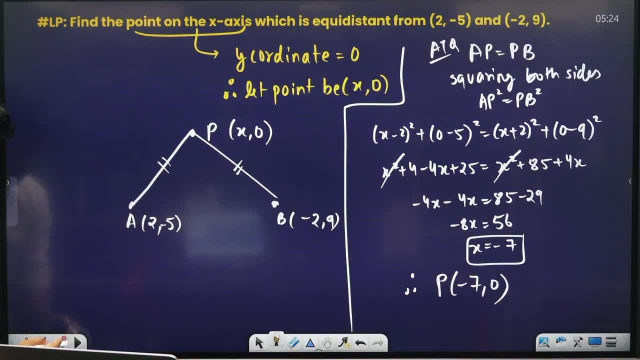 In which ratio will this P point be dividing it? In which ratio will it be dividing it? Then you will assume K ratio. Now we will ask a question. You will understand Like: see: Now we will ask this question first. First we will ask this question, See. 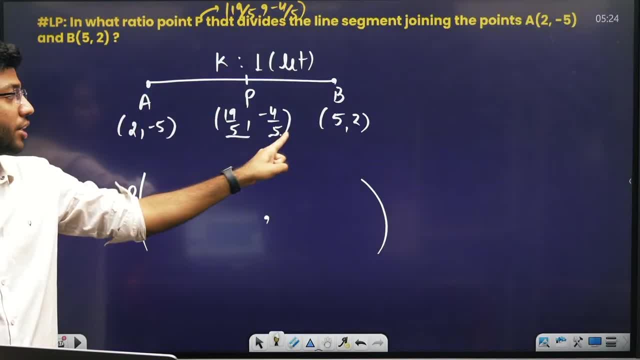 It is said that invert ratio point P Has given the value of 19 divided by 5. And minus 4 divided by 5.. In which ratio will this point P divide this line? So always assume K ratio 1.. Assume K ratio 1.. 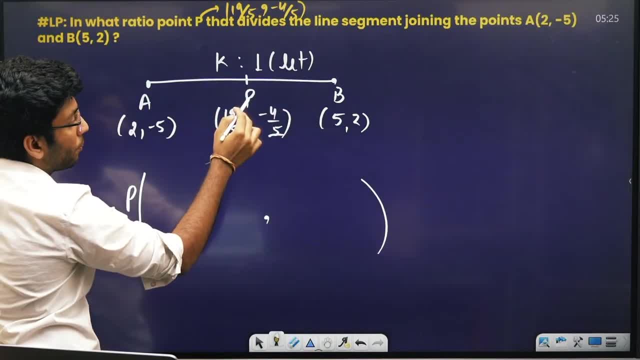 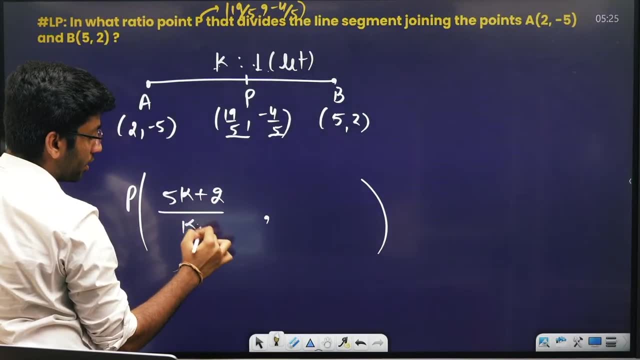 So assume K ratio 1 and write it once. Assume K ratio 1 and write the section formula once. So P point, according to our section formula, will be 5K plus 1 into 2 upon K plus 1.. And what will be the Y coordinate? 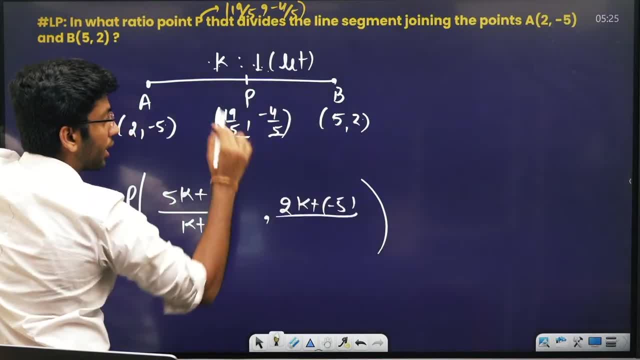 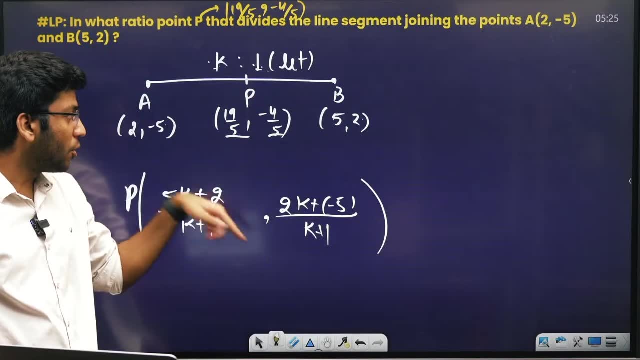 K into 2.. 2K plus 1 into 5 minus 5 upon K plus 1.. So see Assuming K plus 1. P point becomes this, And this one P point is given to us. See carefully, Assuming K ratio 1.. 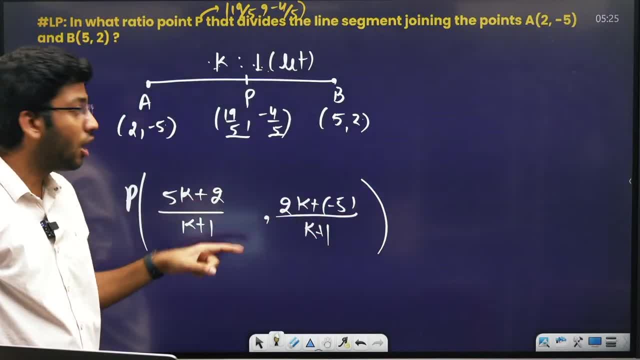 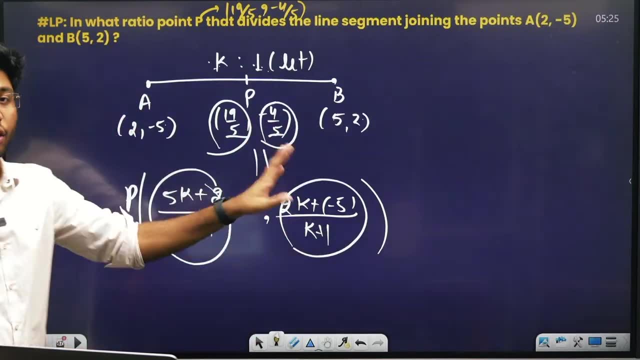 P point is given to us. This is our formula And this is already given Means. these two will be equal. So make its X equal to this And make its Y equal to this. The value of K will come out. One question is very favorite. 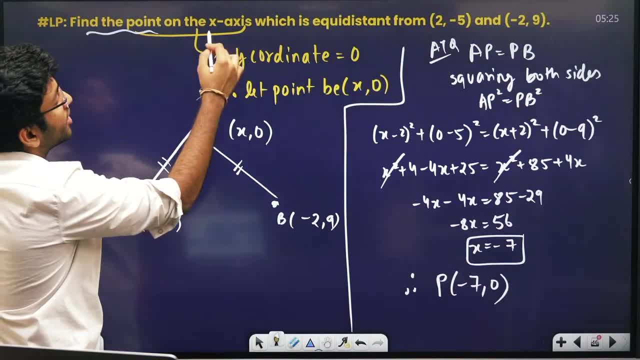 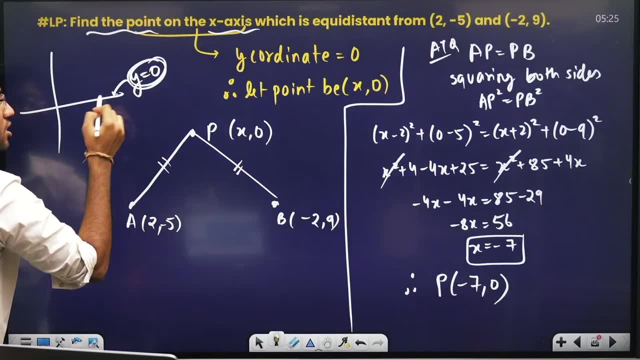 What One point is lying on X axis. What does X axis mean? X axis, This is X axis. So the equation of X axis is Y equal to 0.. Means all the Y points of X axis are 0.. All the Y coordinates of X axis are 0.. 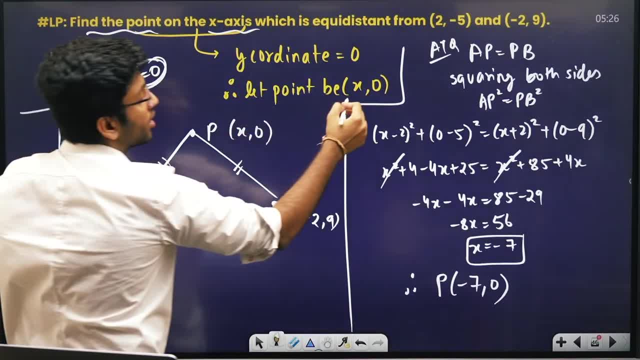 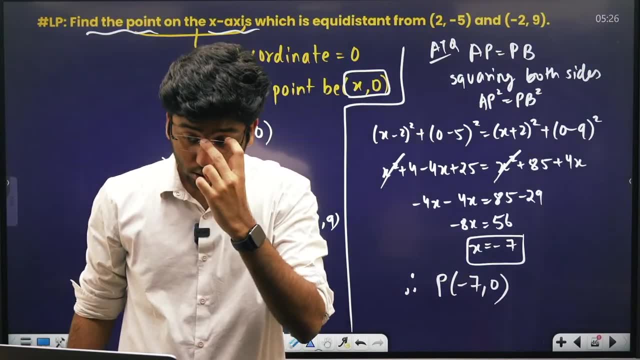 All the Y coordinates of X axis are 0. So I assumed that the point is That's it. The whole game was here in this question. The whole game was here in this question. The whole game was here in this question. What? 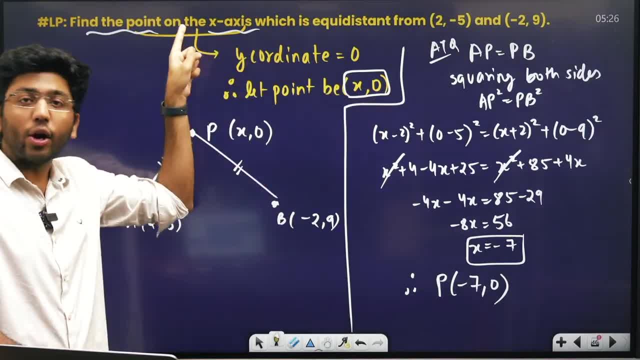 That the point is Because it is on X axis. So the equation of X axis is: Y equal to 0. bitterness, ie as much as points are at X axis, it will have 0 y. So I assume that point is. 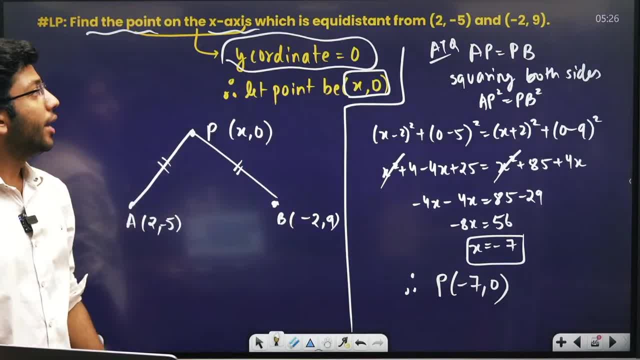 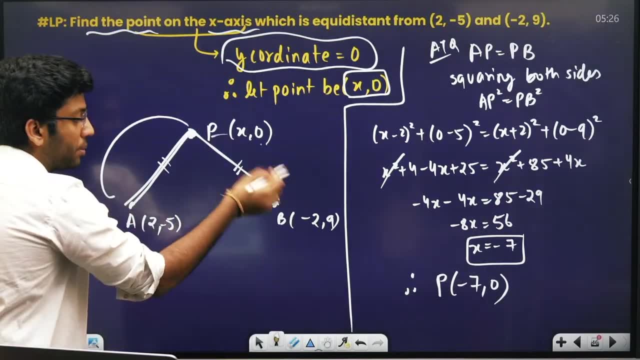 It is equidistant from these two points. It is equidistant from these two points. It is equidistant from these two points. That is meant to say that this ap and pb distance is equal. This AP distance and this PB distance are equal. 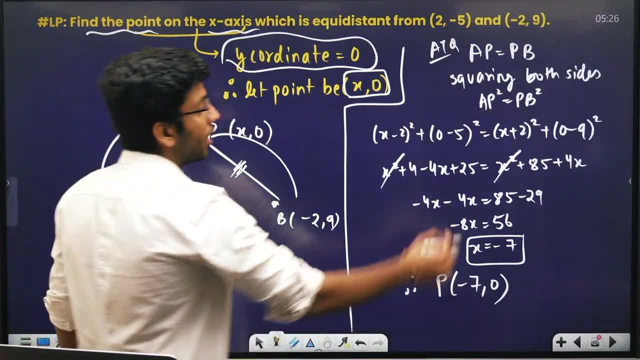 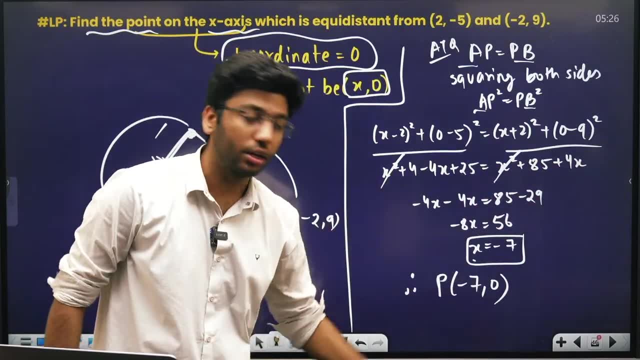 This AP distance and this PB distance are equal. I have written this, Michel, though We did the squaring and put the distance formula, put the distance formula. the value of x is minus 7, and we had to get this point P. this is minus 7 comma 0, this will be the point P. 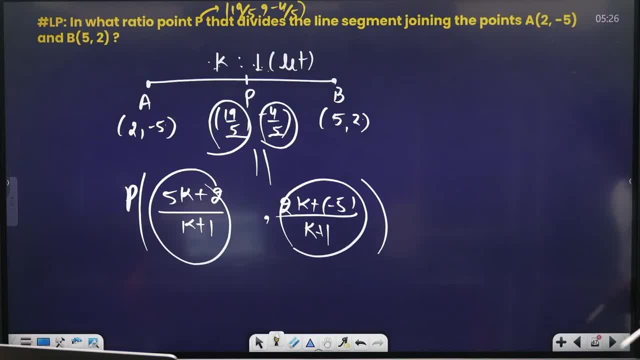 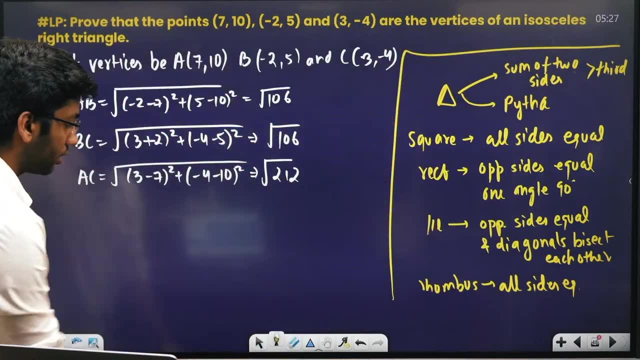 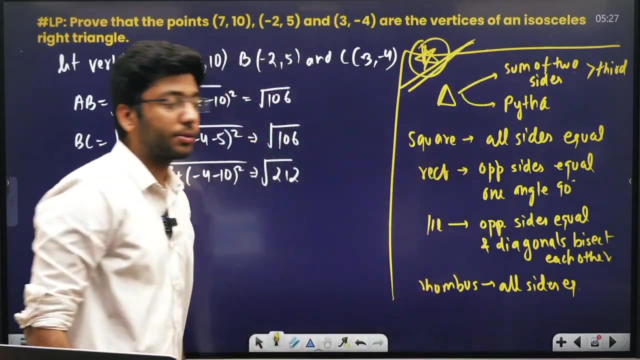 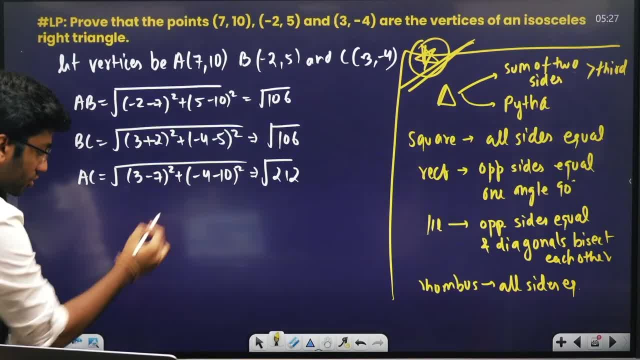 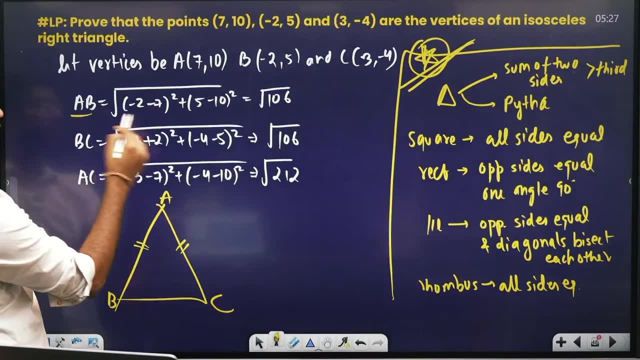 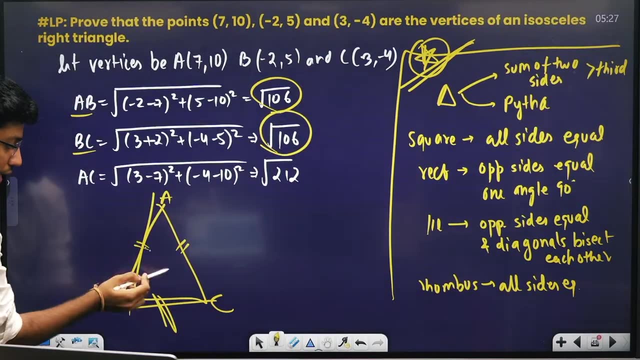 Prove that these points are vertices of isosceles triangle. isosceles triangle means: suppose one ABC is an isosceles triangle, means that any two adjacent sides will be equal. so I took AB length from the distance. formula: root 106 came, BC. length came root 106 came. so AB and BC are equal. AB and BC are equal. therefore it is an isosceles triangle. therefore it is an isosceles triangle. this is how it is proved. 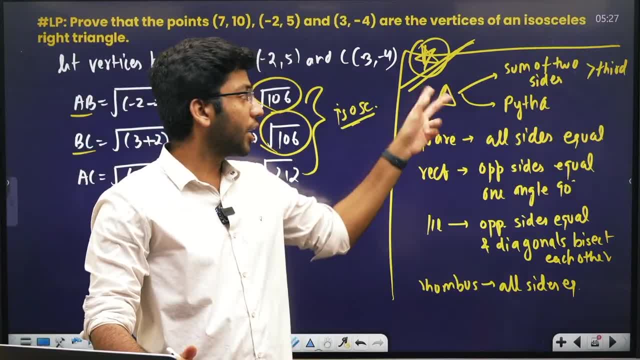 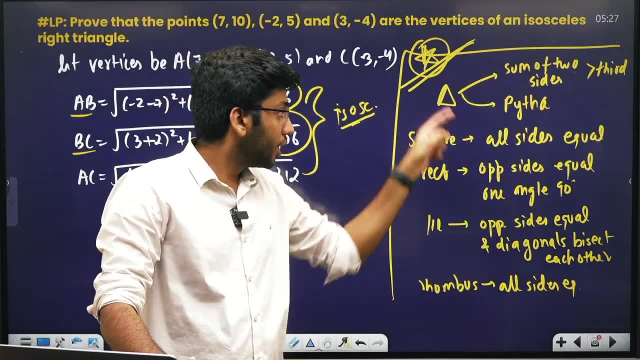 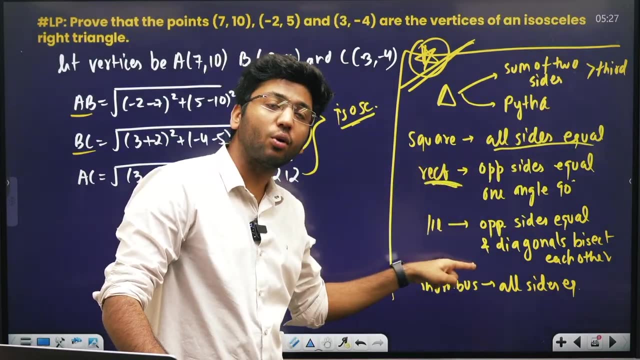 So it can tell you to prove anything. it can tell you to prove triangle. so what? to prove triangle? Either adopt Pythagoras or its sum will be greater than 1.. This is theedy triangle. if you want to prove square, all sides are equal. if you want to prove rectangle? if you want to prove rectangle, opposite sight is equal and any one angle 90.. 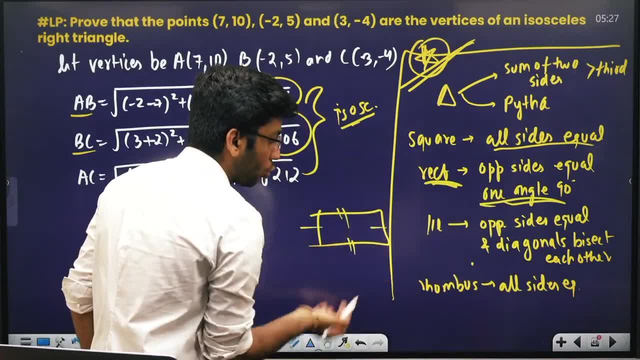 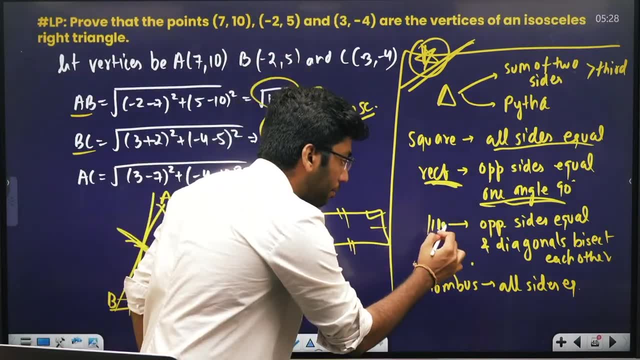 If you want to prove rectangle, do opposite side is equal- and prove any angle- 90, this is how it happens. how to prove 90 through Pythagoras: Parallel parallelogram, parallelogram, parallelogram, parallelogram. to prove parallelogram. what is parallelogram? 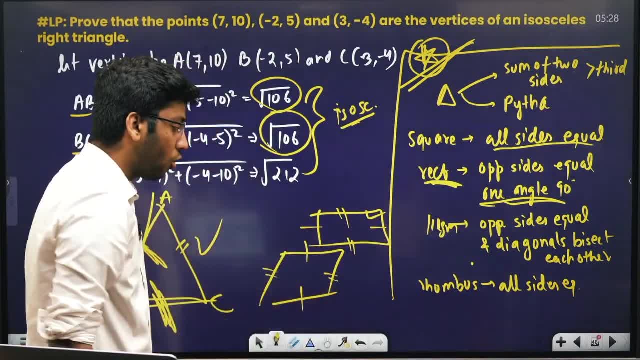 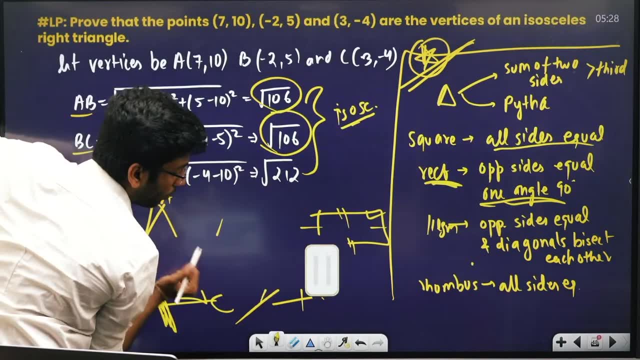 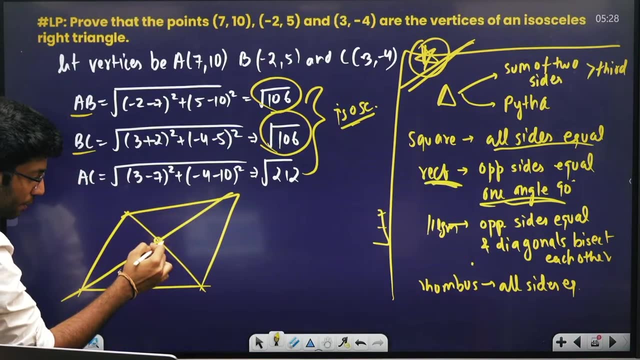 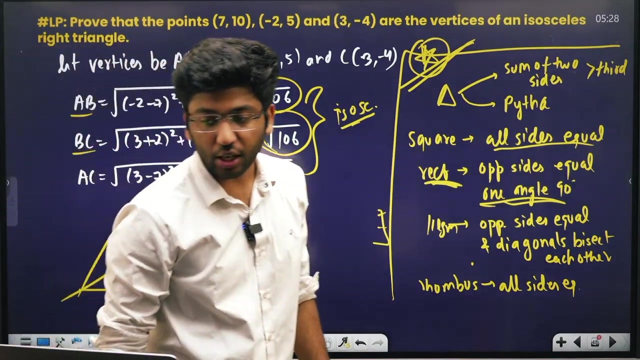 Opposite Sides are equal, opposition to opposite sides are balanced, are equal and diagonals bisect each other. Bisect means that this and this will be the midpoint, O is midpoint of this and O is midpoint of this also. This is the meaning of bisect. Write this: 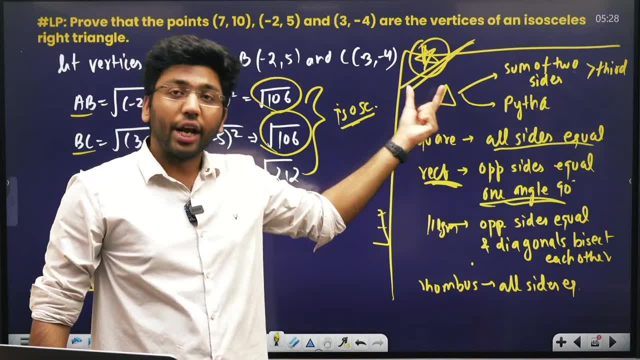 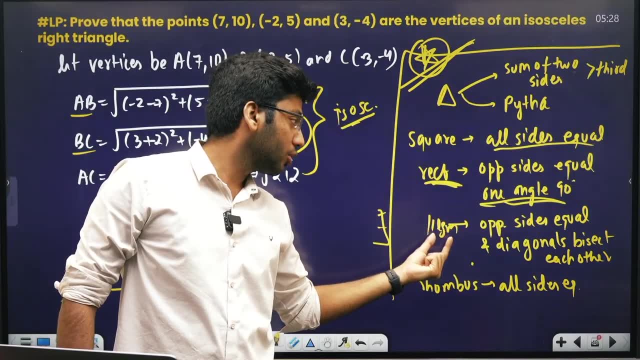 This is very important. If you want to prove triangle, prove this. If you want to prove square, prove this. If you want to prove rectangle, prove all sides equal. If you want to prove parallelogram, prove the length of opposite sides equal. 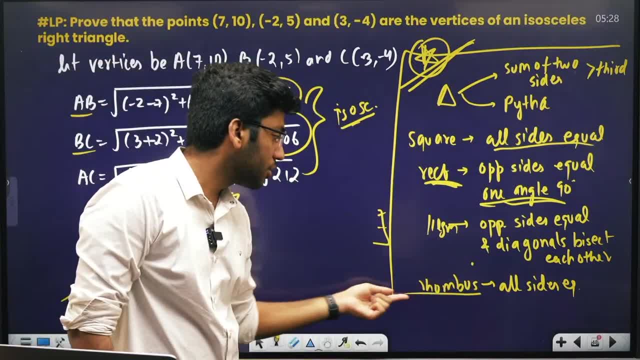 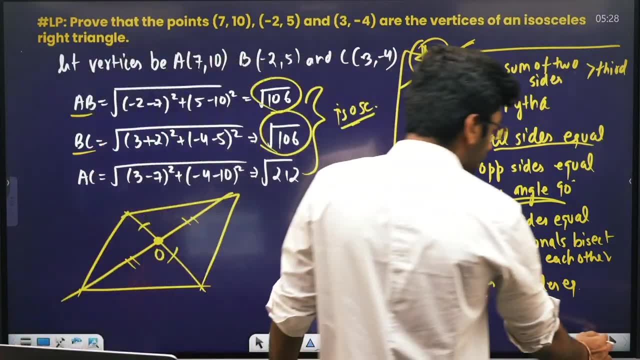 Similarly, if you want to prove rhombus, prove the length of all sides equal. This is how it is done. If this, this, this are vertices of parallelogram, We have given a parallelogram of this parallelogram. 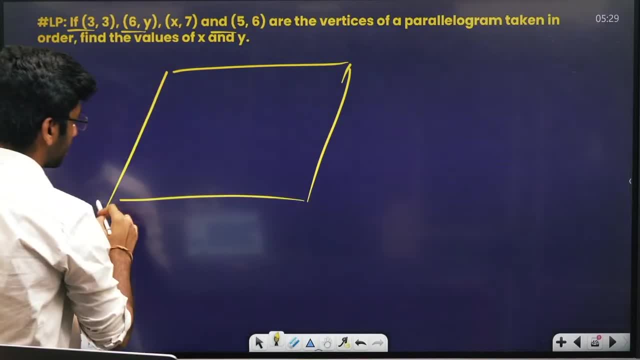 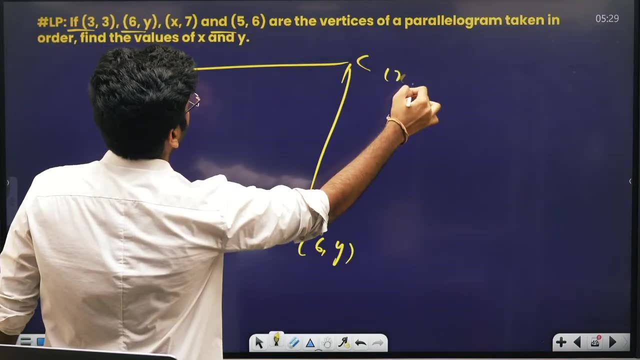 We have given a parallelogram of this parallelogram. A B C D are parallelograms. We have given A B C D as 3,, 3, 6, Y, X, 7 and 5, 6.. 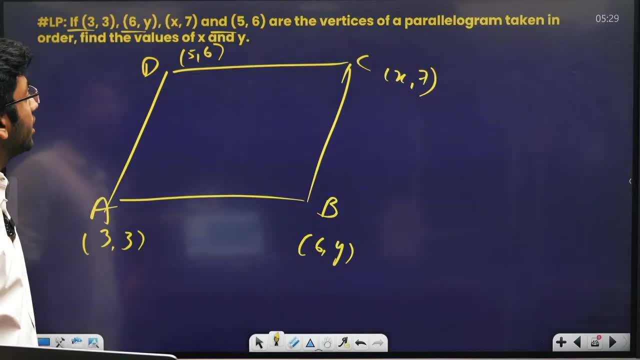 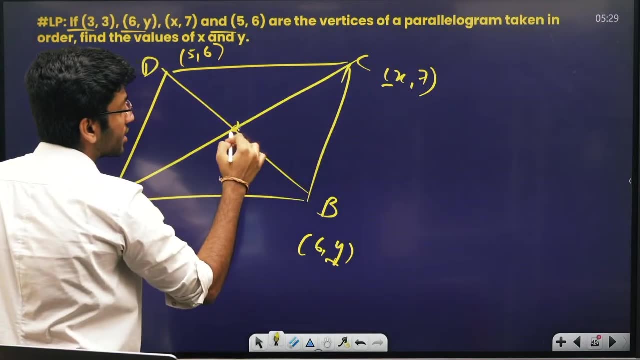 We have given these. These are vertices of parallelogram taken in order to find the value of X and Y. We have to find the value of X and Y. What is the property of parallelogram? The diagonals of this are bisect. 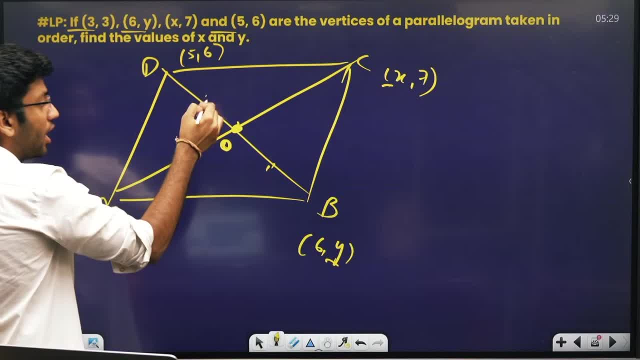 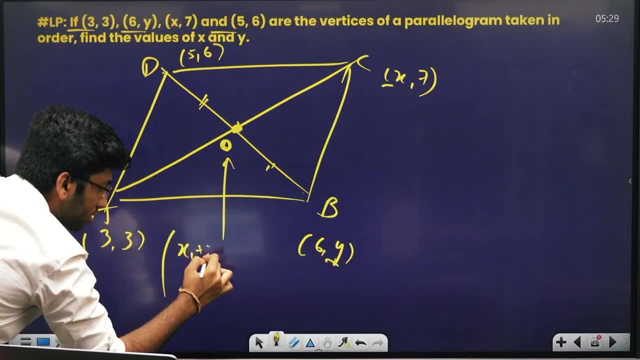 Means O will be the midpoint of this. So what should we do? Remove the midpoint of BD? What is the midpoint formula? What is the midpoint formula? X1 plus X2 by 2 comma, Y1 plus Y2 by 2.. 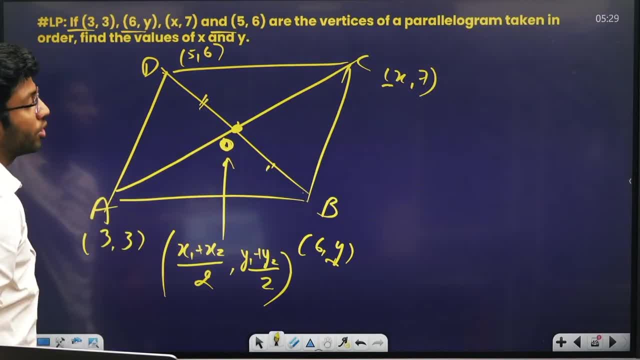 This is the midpoint formula. So what is O point? This will also be the midpoint of this And O point will also be the midpoint of this. So the coordinate of O point will be derived from this And the coordinate of O point will be derived from this. 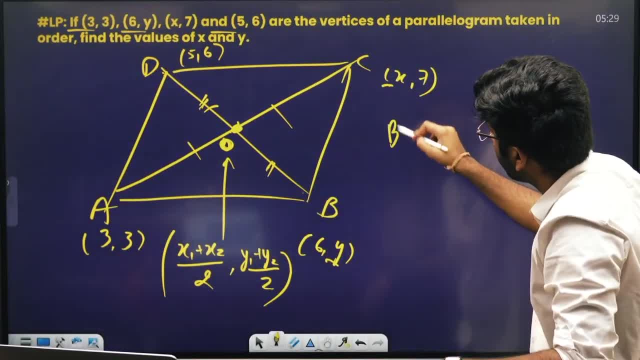 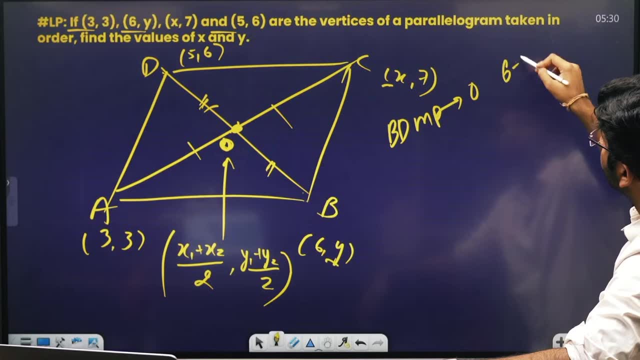 Equalize both of them. How See: remove the midpoint of BD. Who is the midpoint of BD? O? So how will we write the midpoint of BD? We will write 6 plus 5 by 2 comma, 6 plus Y by 2.. 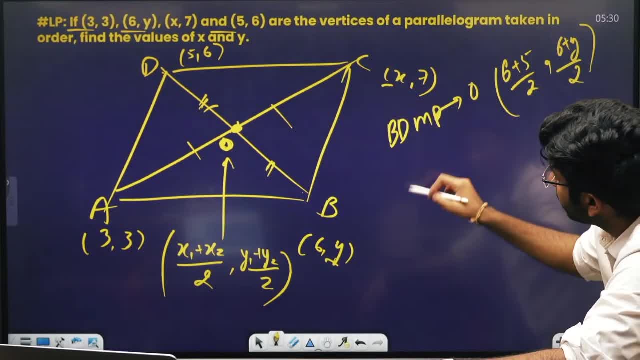 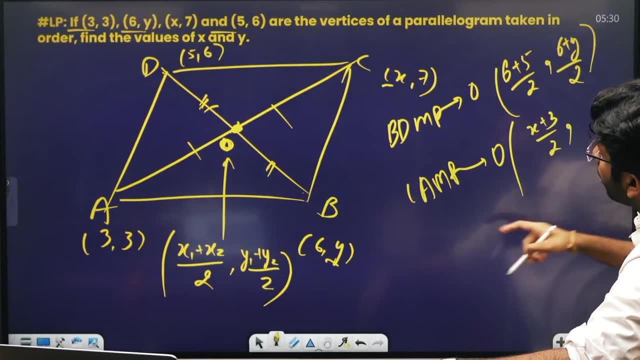 This is the midpoint of BD O. Similarly, what is the midpoint of CA? CA is also the midpoint of O. So if I write the midpoint of CA X plus 3 by 2 comma, 7 plus 3 by 2.. 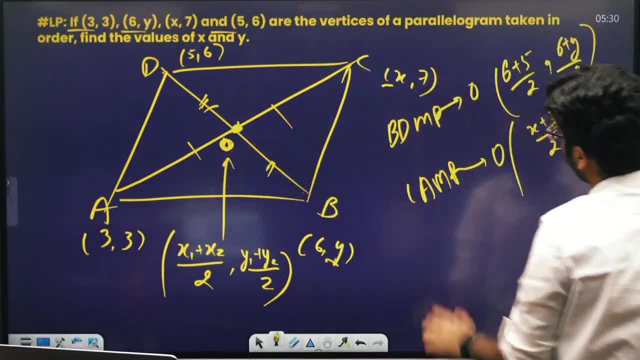 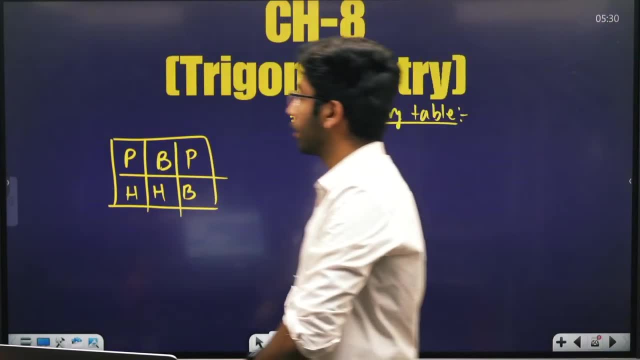 So I wrote O from this too. I wrote O from this too, And equalize both of these O's. Its X coordinate is equal to this. Its Y coordinate is equal to this. The value of X and Y will come. In this way, we will solve this question. 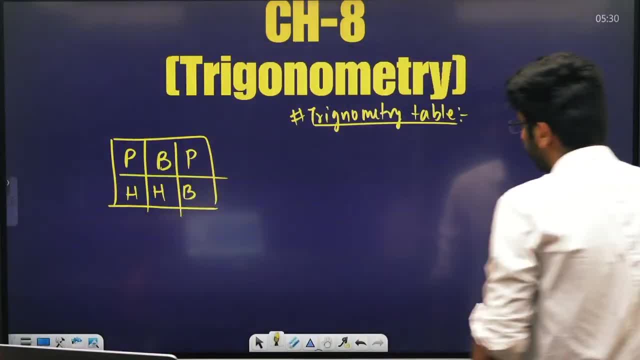 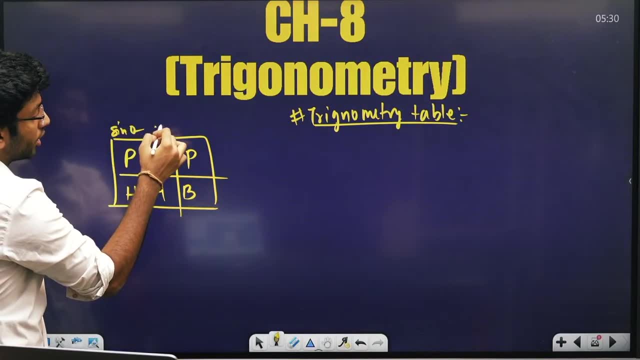 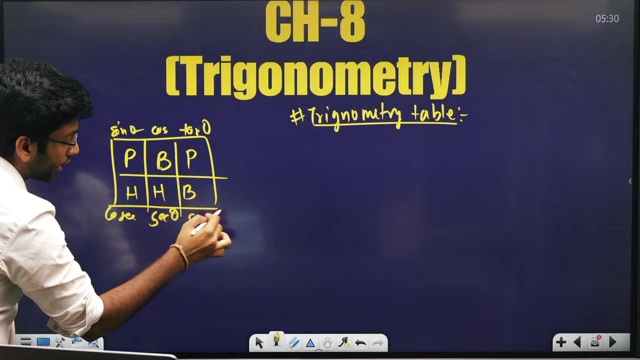 If we talk about chapter number 8.. Trigonometry, Chapter number 8: Trigonometry In Trigonometry. do you remember this? Papa PDPO said: yes, son Sin theta, cos theta, tan theta. And if we see from below, cosec theta, sec theta and cot theta. 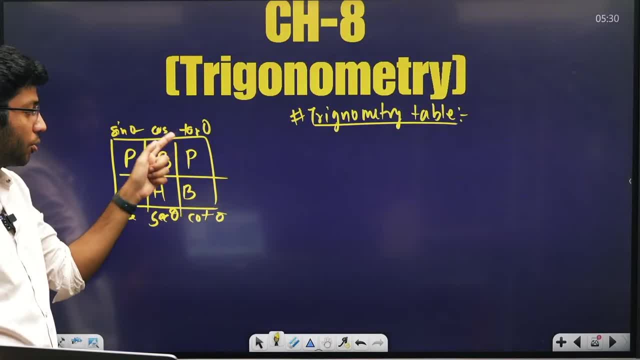 Do you remember this? So sin theta is P by H, B by H and P by B And H by P, H by B, B by P. Do you remember this? Okay, What is trigonometric table? You should remember this. 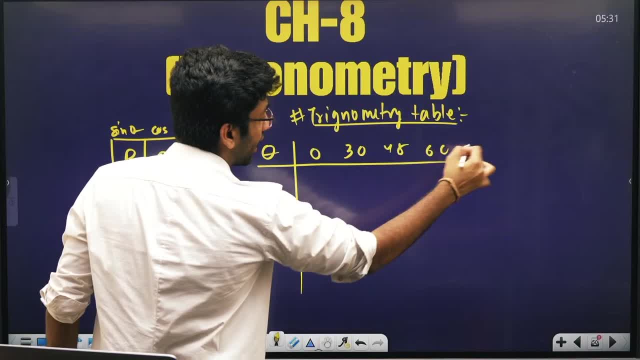 What? 0,, 30,, 45,, 60,, 90.. As soon as you go to the paper first, make a trigonometric table. As soon as you go to the paper first, make a trigonometric table. 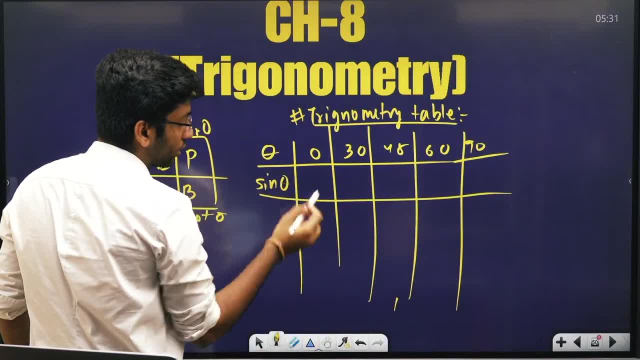 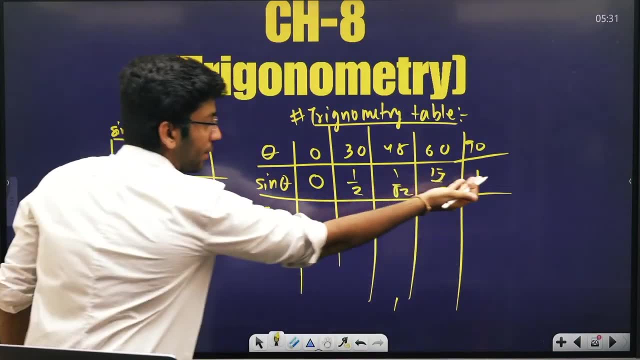 See Write. Write about sin. What is sin theta? Sin is 0.. 0, 1 by 2, 1 by root 2, root 3 by 2 and 1.. What is cos theta? Just write the opposite of this. 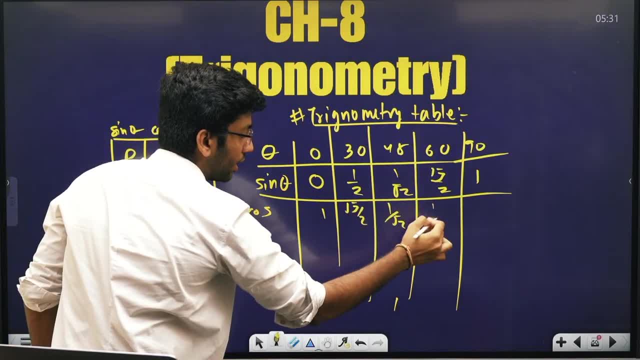 So 1 root 3 by 2, 1 by root 2, 1 by 2 and 0.. What is tan theta? We have kept tan theta. Either do sin by cos, Either do sin by cos Or write. 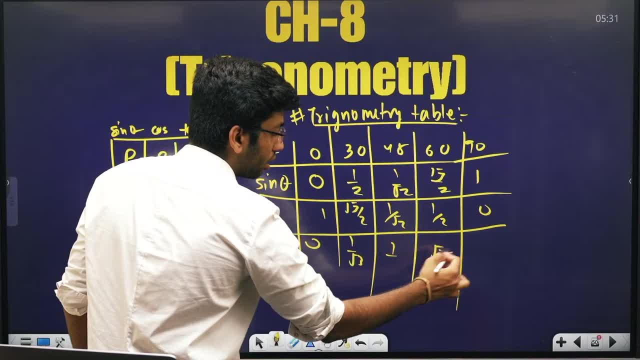 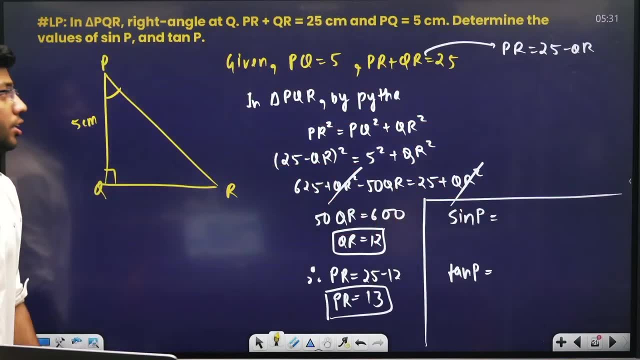 0, 1 by root 3, 1 root 3, not defined. So make your whole table like this. Make your whole table like this. Okay, This question CBC's favorite question. It is saying In triangle: PQR. 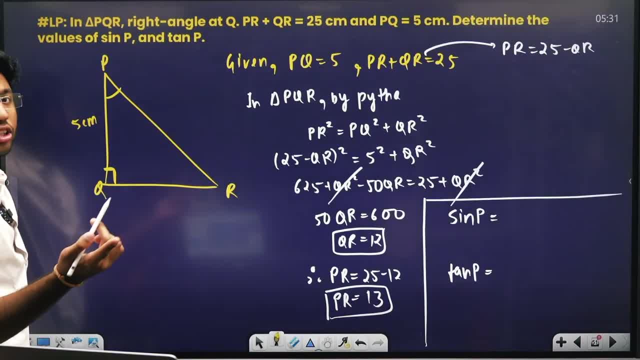 This triangle is PQR, which is right angled here. So if right angle is triangle, then it will look like Pythagoras. If right angle is triangle, then it will look like Pythagoras, for sure. PQ plus QR has given us 25 and the value of PQ is 5.. 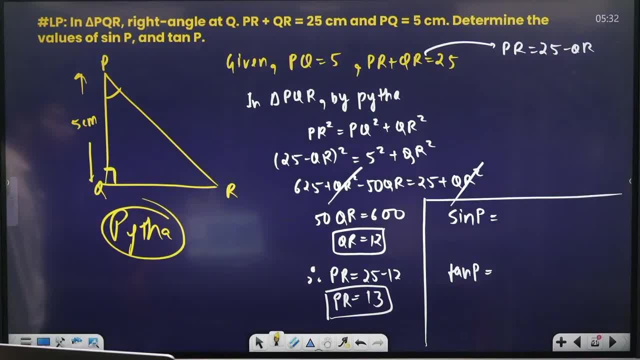 This PQ has given us 5.. Okay, Determine the value of sin P and tan P For P angle, we have to get out sin, and that Sin means perpendicular upon hypotenuse. It means need of this side and this side. 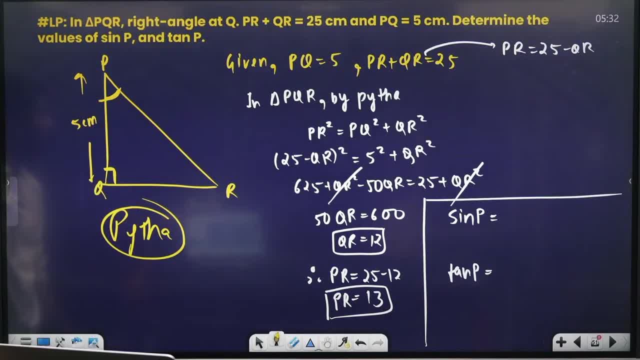 And perpendicular upon base. So it is the need of this side and this side. So, unknown side, I have taken out. Unknown side: I have taken out, I will apply Pythagoras. So what will Pythagoras? Square of PR is equal to square of PQ plus square of QR. 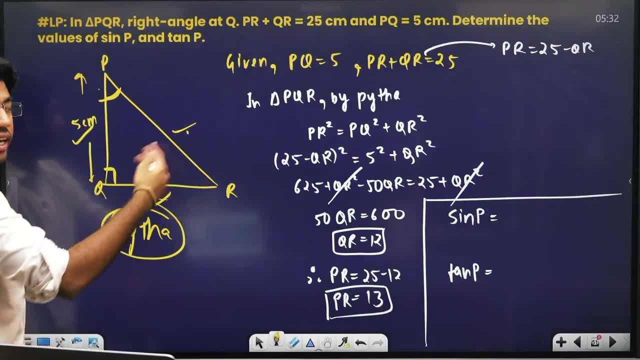 Square of PQ plus square of QR. So PR square is equal to PQ plus QR. PQ is given as 5.. So PQ is given as 5.. So PQ is given as 4.. So PQ is given as 5.. So PQ is given as 4.. 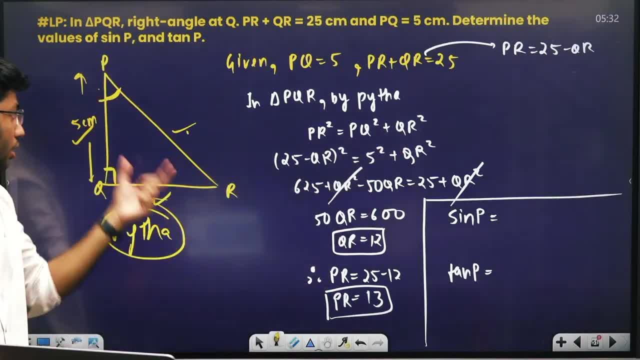 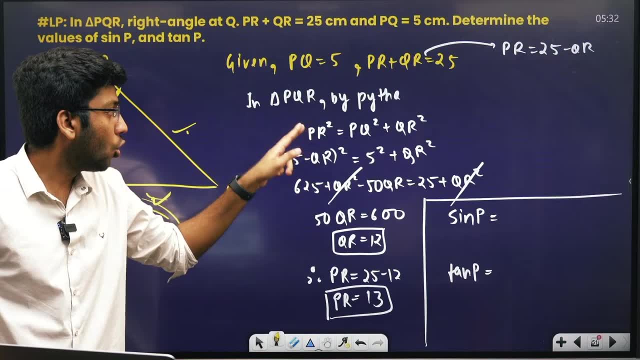 PR square is equal to PQ square plus QR square. PQ square plus QR square, PR square is equal to PQ plus QR. PQ is given as 5.. QR is written as QR And PR is from here. PR plus QR is 25.. 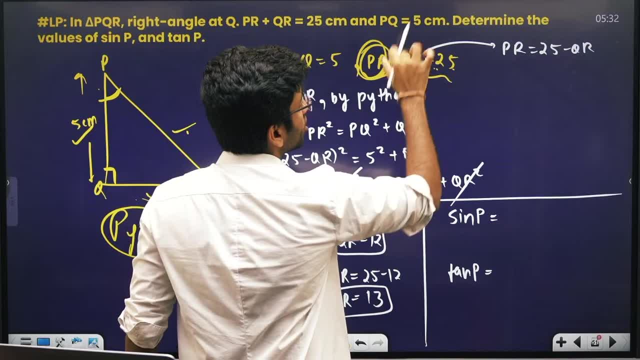 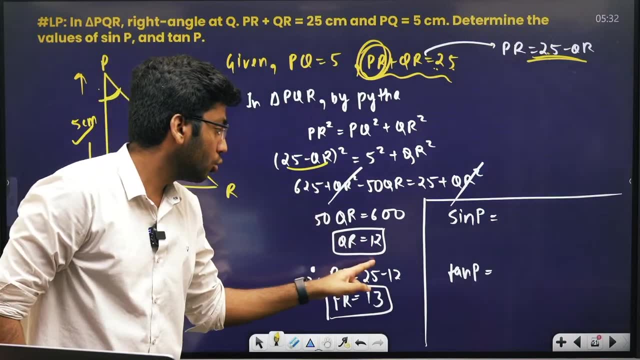 So what will be the value of PR? PR value will be 25 minus QR. 25 minus QR. I will keep 25 minus QR here. Open the whole square of A minus B, Cut the square from QR. So the value of QR is 12.. 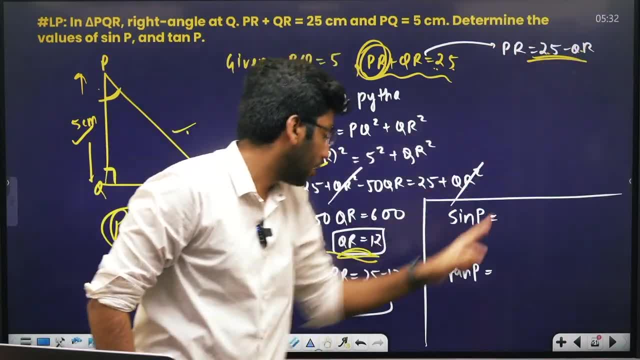 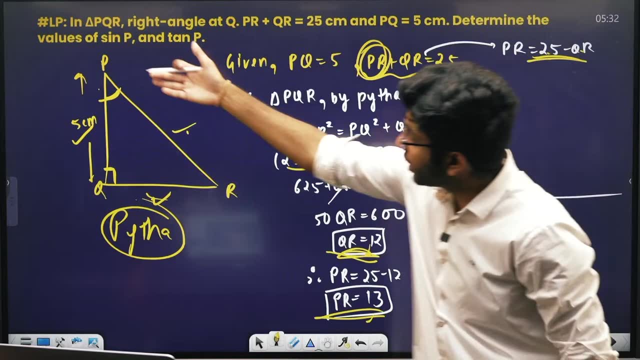 QR is 12.. So what is PR? 25 minus 12.. It is 13.. So QR is known, PR is known. What will be the sign Perpendicular upon hypotenuse? This is perpendicular to P. 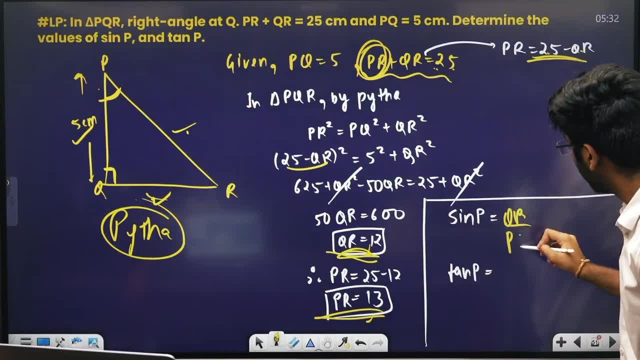 So the sign will be QR upon PR. QR upon PR. So what is QR? The value of QR is 12.. What is PR? 13. What will be 10? Perpendicular, What is base of QR upon? 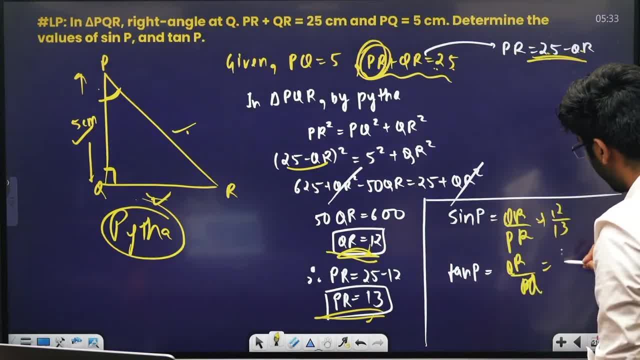 Base is PQ. Base is PQ, So the value of QR is 12.. What is base? Base is 5.. So 12 divided by 5.. This will be our answer: 10 and the sign will be P. 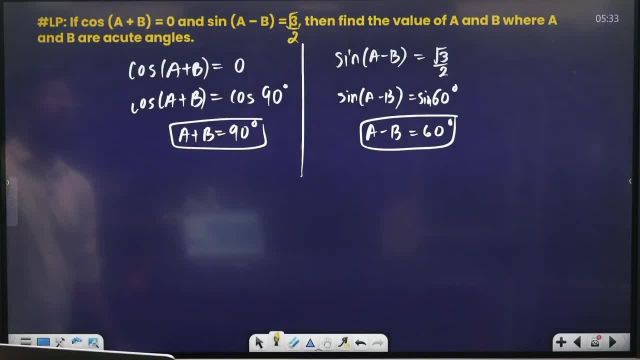 Okay, After that this trigonometric table will ask you that if cos of A plus B is given as 0 and sin of A minus B is given as root, 3 by 2. So take out the value of A and B. 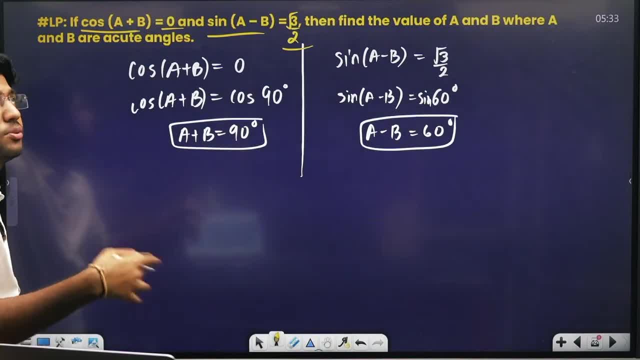 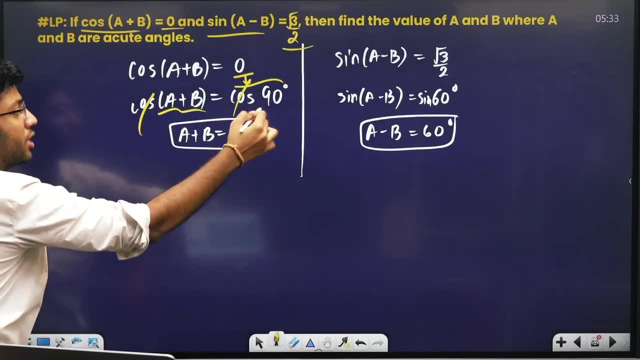 So you have to see when cos is 0.. When cos is 0. When cos is 0 on 90. So instead of 0, I wrote cos 90. So I cut the cos from the cos, So the value of A plus B is 90.. 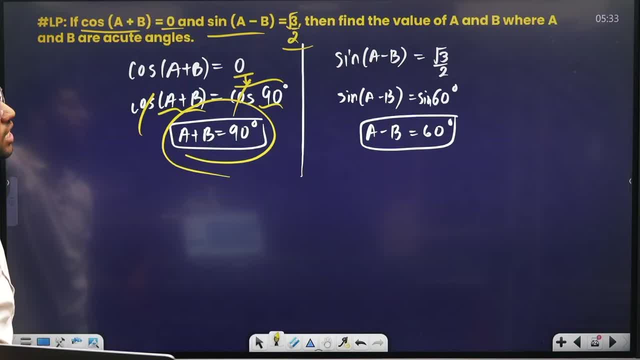 This equation became A, Then it is said that sin A minus B is root 3 by 2.. When is sin root 3 by 2?? It is instead of root 3 by 2.. I wrote sin 60.. I wrote sin 60.. 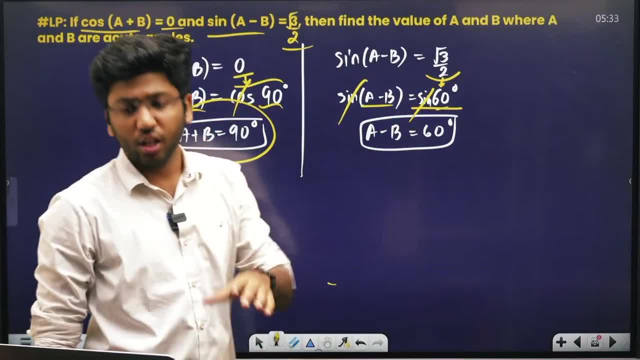 When sin is cut, A minus B equals 60. This way sin is not cut. I have cut this to make you understand. A minus B equals 60.. A minus B equals 60. So A plus B is 90.. 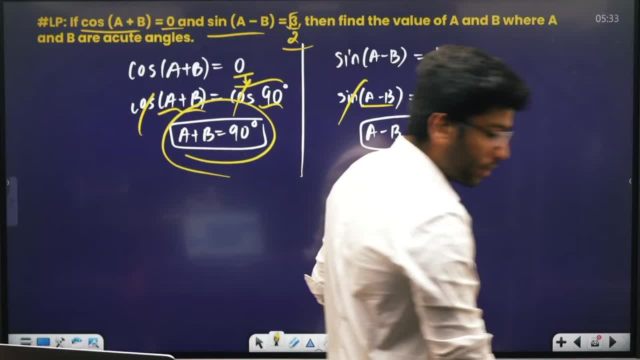 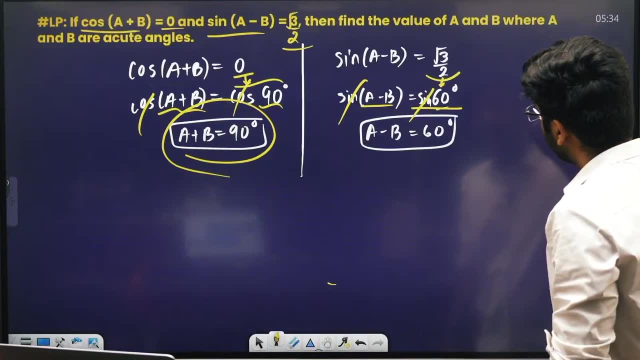 A minus B is 60.. Take out the value of A and B. Take out the value of A and B. Okay, Now see, Now see. Now see Three formulas, Three formulas, Three formulas. What sin square theta plus cos square theta equal to 1.. 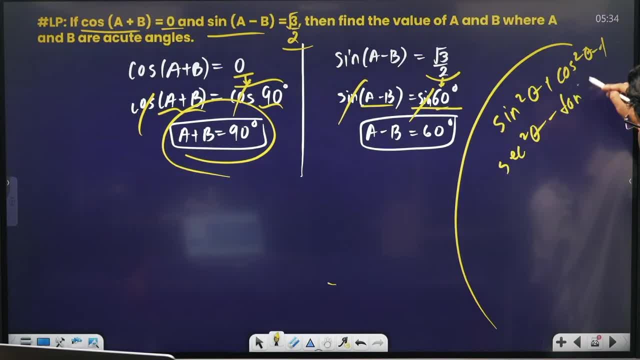 Sec square theta minus tan, square theta equal to 1.. Cosec square theta minus cot, square theta equal to 1. These three formulas, all the questions are made on them. All the questions are made on them Whenever, whenever, any question Now see trigonometry. 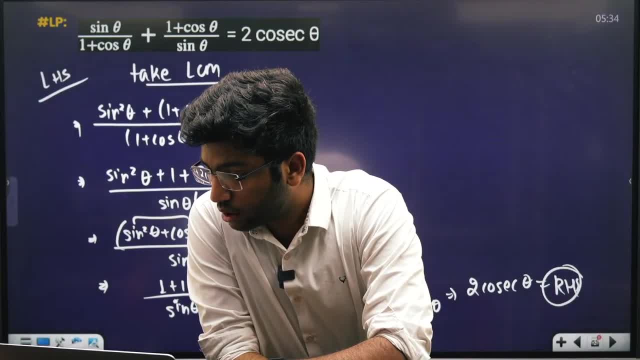 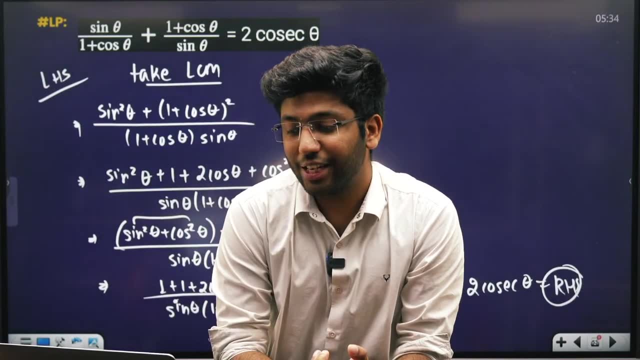 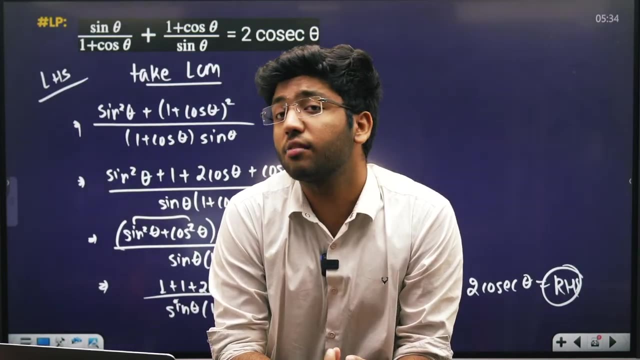 Trigonometry. What is written, Scripted? What is this Scripted? What is scripted? See, I can only tell you the methods of trigonometry. It is very difficult to predict in trigonometry what kind of question will be asked. 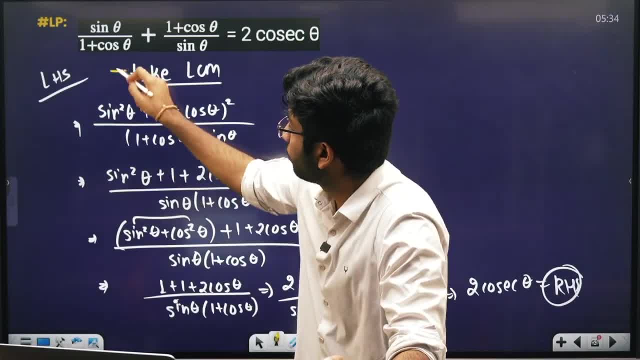 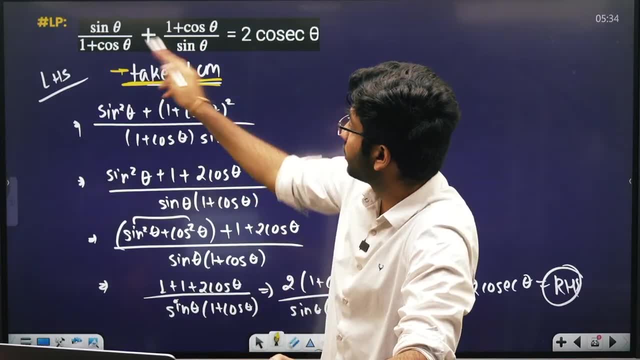 I am telling you the methods. whenever you get stuck, take LCM First thing. Whenever you get stuck, take LCM. Whenever you have to use this, Whenever you get stuck, take LCM. So what I did, took LCM, took LCM and this became: 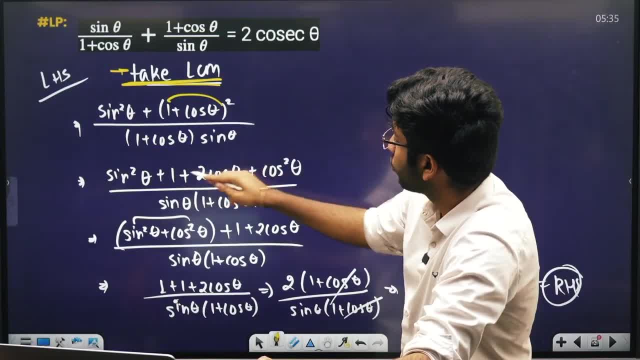 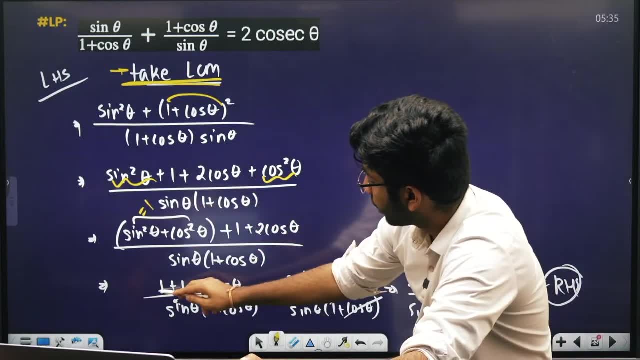 Took LCM and this became opened whole square of 1 plus cos theta, a square plus b square plus 2ab. Now see sin square plus cos square, This is 1, sin square theta plus cos square, theta is 1, So this became 1 plus 1. 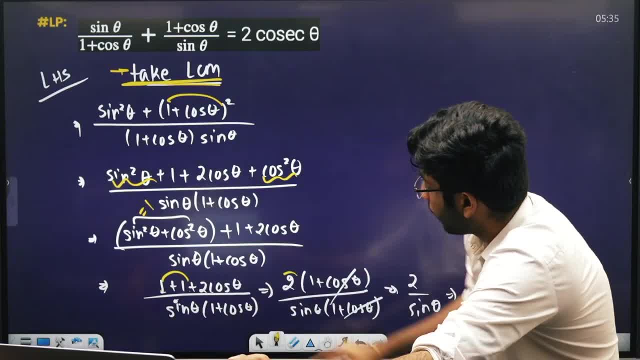 And this was going on in upon Here: 1 plus cos square plus cos square plus 2ab. Now see sin: square plus cos square plus cos square plus 2ab, And this became 2, And this became 2. Took 2 and it became 2 into 1 plus cos theta. 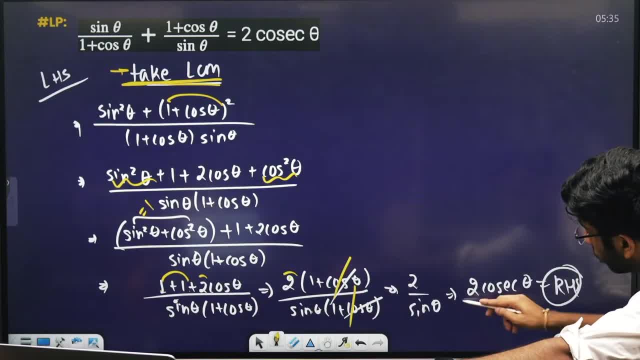 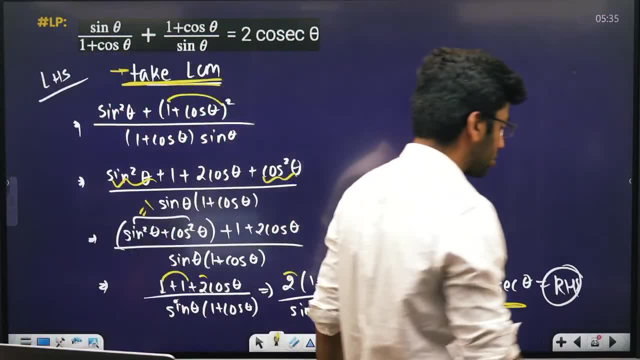 1 plus cos theta. 1 plus cos theta is 4, So 2 by sin theta is left, Which is 2 cos. So, whenever you get stuck, whenever you get stuck, take LCM, Take LCM. whenever you get stuck, When you take LCM, take LCM square. 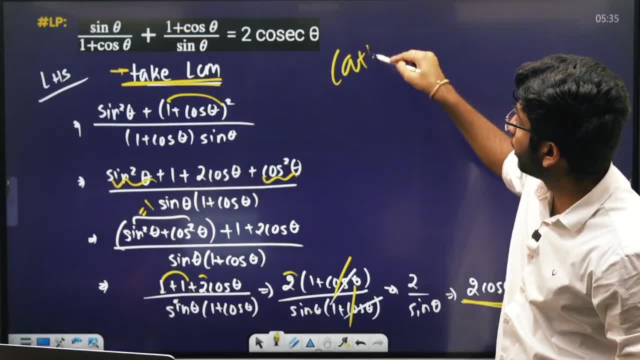 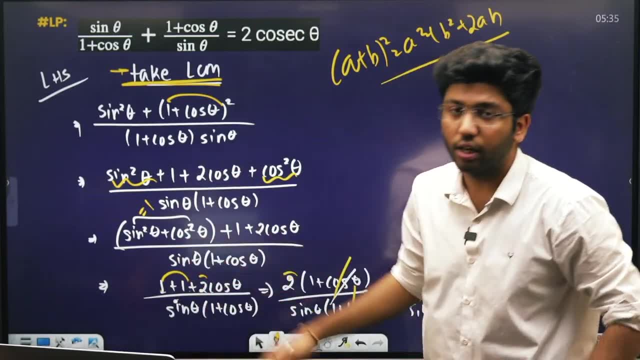 Open square, whole square of a plus b. A plus b's whole square. Do you remember what a plus b's whole square is? a plus b's whole square is a square plus 2ab. That's it. just opened it out. Open it, Sine. square plus cos square means 1. 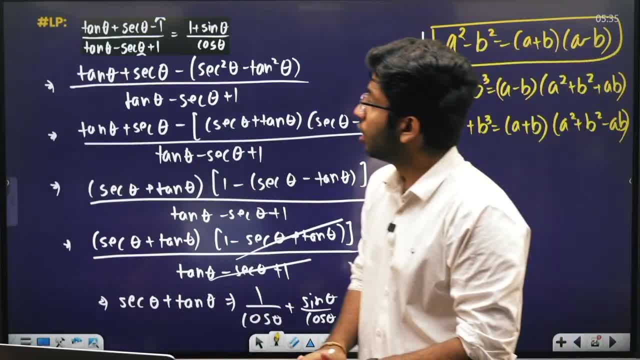 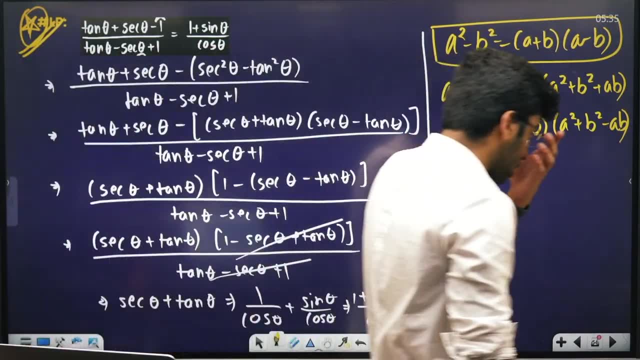 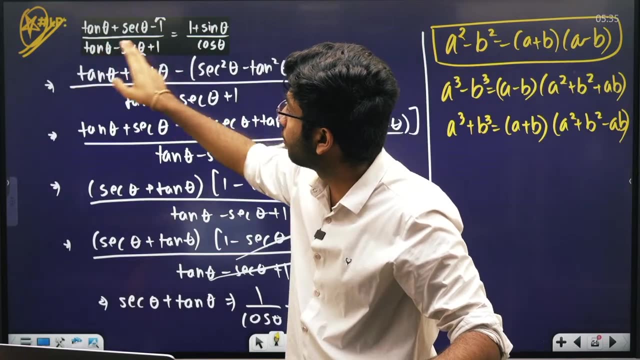 The answer is here. Okay, get stuck and take LCM. This is a very favorite question, a very favorite question of CBSE, a very favorite question. Look, understand one thing in this question: it is a question of your NCERT. I am just reminding you whenever it will be of this type: tan sec 1,. tan minus sec 1,. 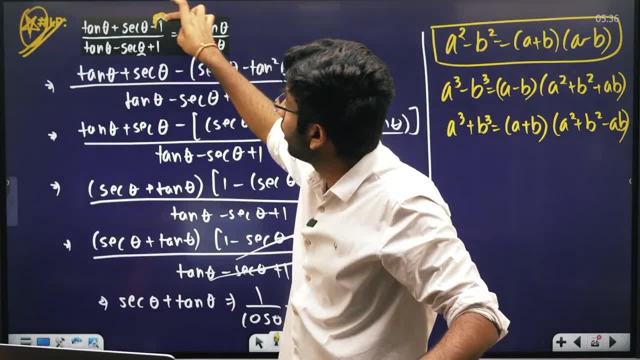 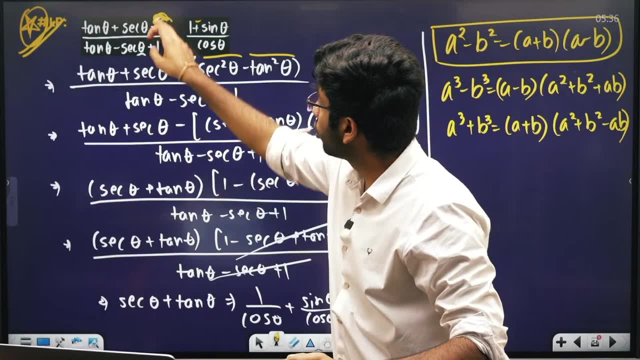 it will be of this type. so what you have to do is this upper one: write it as sec square theta minus tan square theta, because sec square theta minus tan square theta is 1, do you know this property? so this 1 is written as sec square theta minus tan square theta. this 1 is written as sec square theta minus tan square theta. 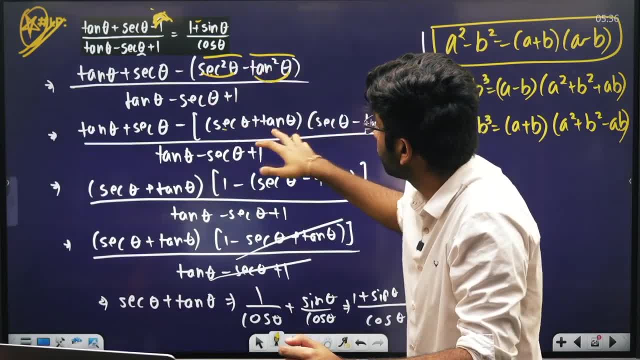 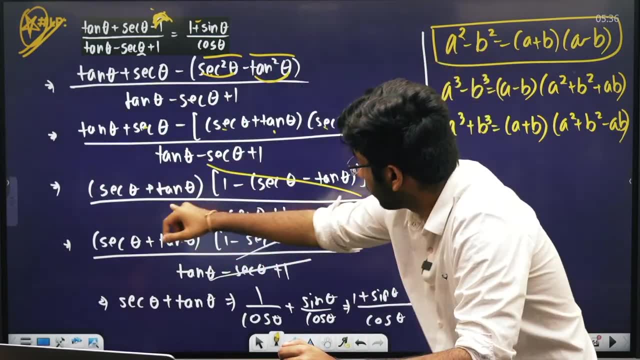 when you will write this. so look: a square minus b square. so a plus b, a minus b. now this: sec plus tan, sec plus tan. take a comma, so this becomes inside and this: this is cut from the lower one. this is cut from the lower one, so sec plus tan is left above this. is it in this question? 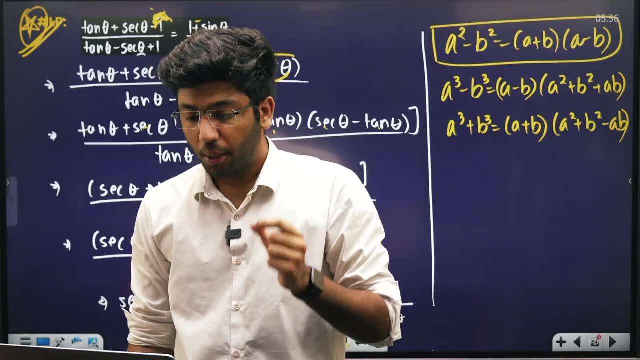 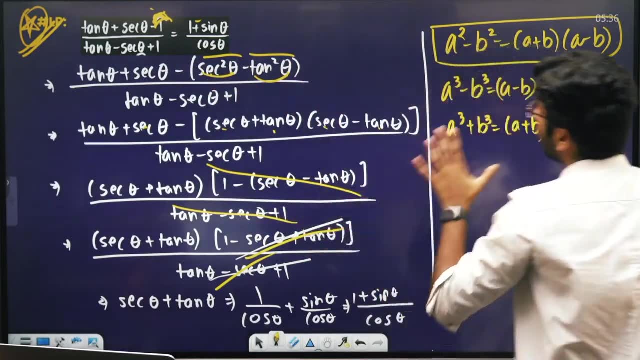 such a question, such a question. there are very big chances of such a question. so what did you do? You wrote 1 as sec square theta minus tan square theta. wrote 1 as sec square theta minus tan square theta. it is a question of NCERT. 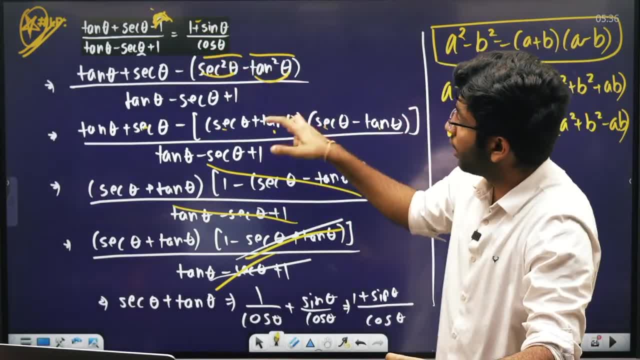 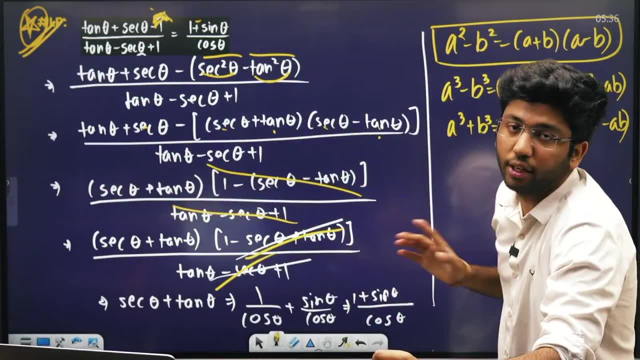 there are many chances of such coming. I have done this in my marathon also, so wrote 1 like this: A square minus b square. you opened it like this: when you opened it and took this sec plus tan, sec plus tan as a comma, then this upper one and denominator got cut. 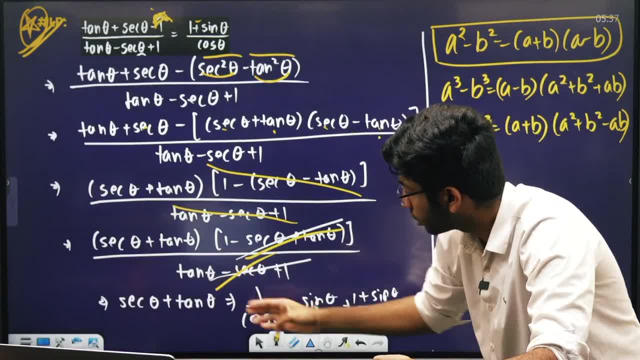 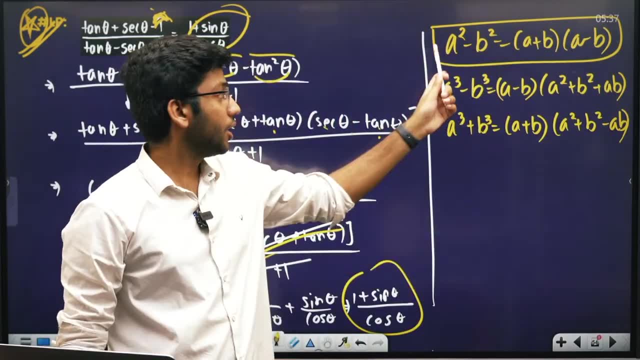 when it got cut, then sec plus tan became and sec plus tan was written as sec 1 by cos. tan was written as sin by cos took LCM. so this is RHS, this is RHS which we have to prove. remember these 3 identity: A, square minus b, square A plus b, A minus b. 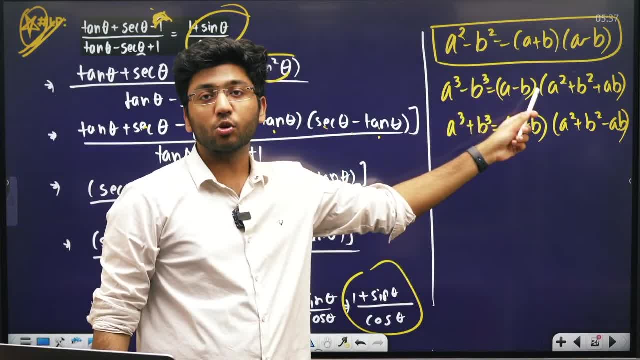 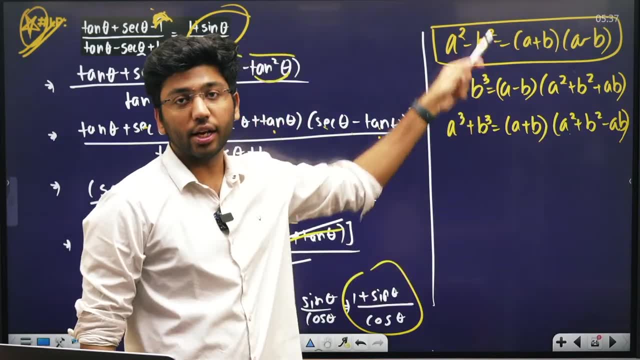 a squared plus b squared is a minus b. a cubed minus b cubed is a minus b. a squared plus b squared plus a b. a cubed plus b cubed is a plus b. a squared plus b squared minus a b. remember these three identities. 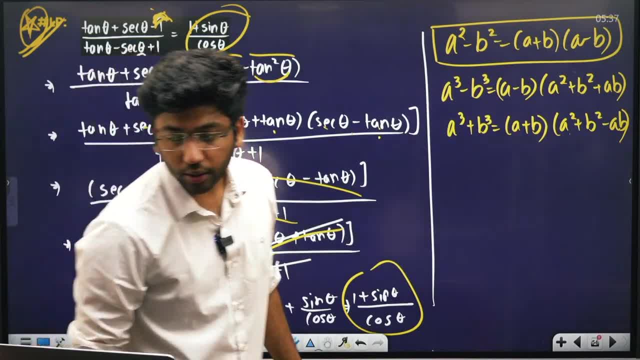 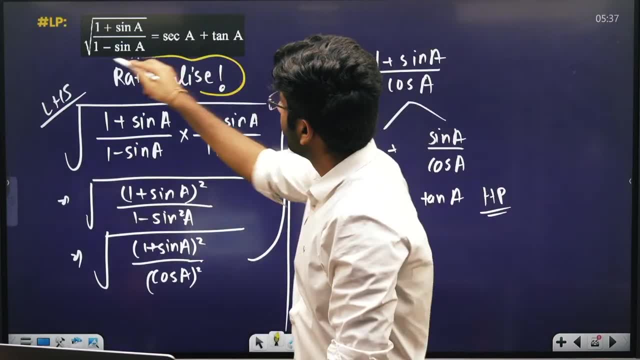 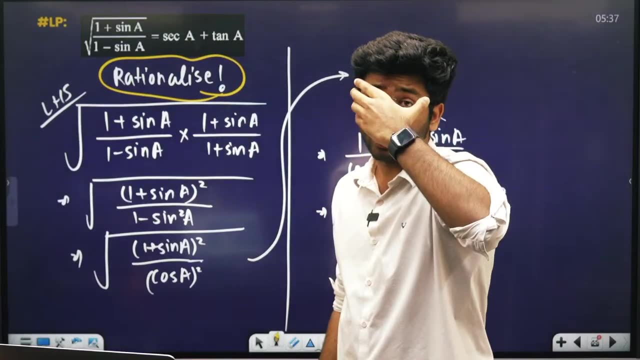 you can directly ask questions on this too. remember these three identities: ok, ok, ok, whenever you get such questions, don't do anything, just do rationalization. a question like this: one plus sign upon one minus sign, a question like this comes up right away, just personalize it. 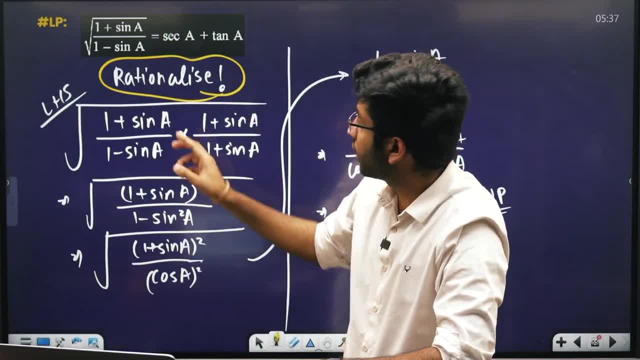 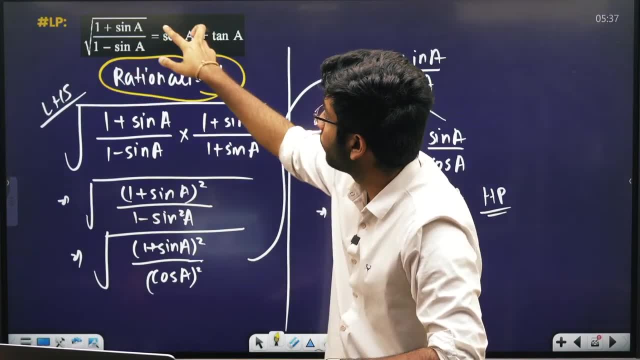 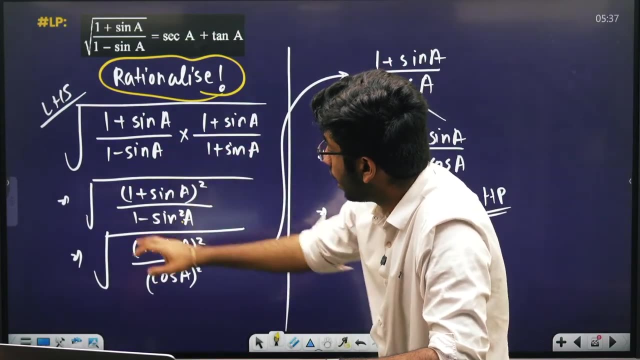 so rationalize with one plus sign upon one minus sign. so what we did change: one plus sign, toωςine. multiply and divide one plus sign. one plus sign. multiply and divide one plus sign whole squared. one plus b squared, minus b squared. now you can write: 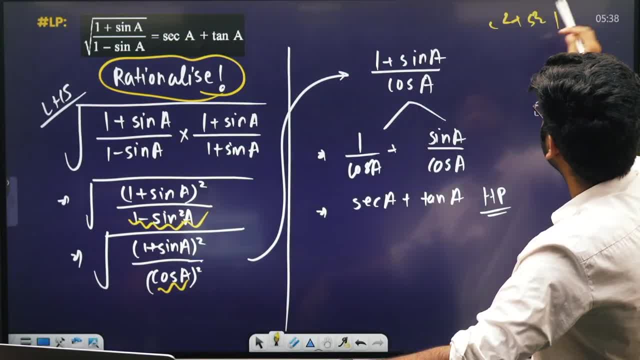 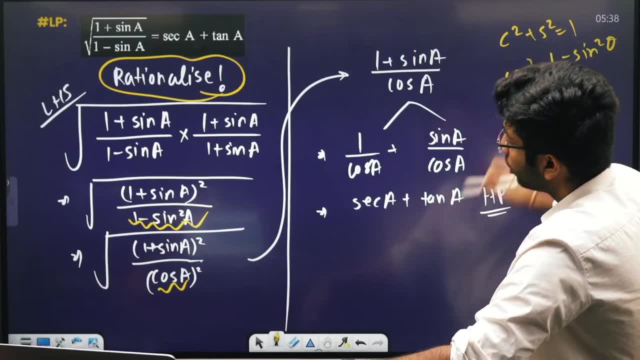 one plus sign squared theta because it equals one minus variation. yes, So 1 minus sin square theta will be cos square theta. So 1 minus sin square theta will be cos square theta. Now, this is the whole square. The root will be cut from the whole square. 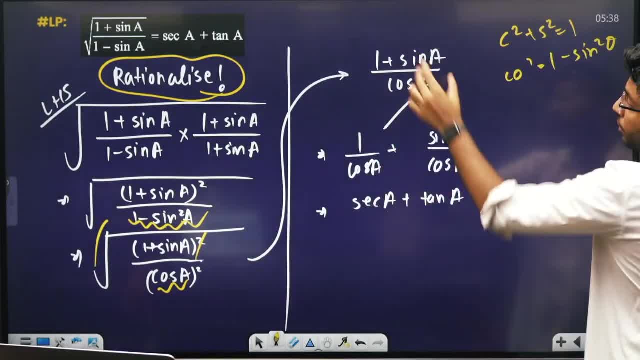 So 1 plus sin upon is cos And 1 plus sin upon is cos. We took cos separately in LCM. So 1 upon cos is sin by cos, 1 upon cos is sec, Sin by cos is tan. 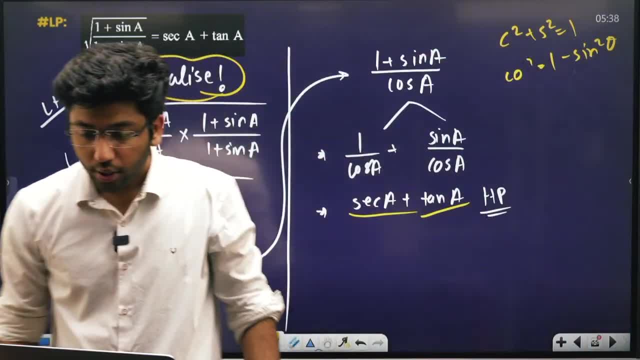 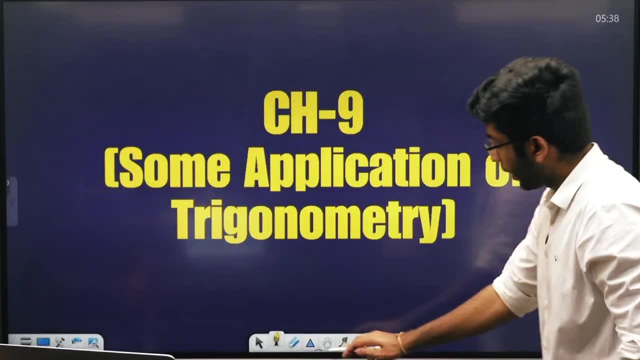 This is our answer, Okay, Okay, Hit the like button. It will be done later. It will be done later. Next, Next chapter: Some applications of trigonometry. In some applications of trigonometry, 2-3 questions which are very famous. 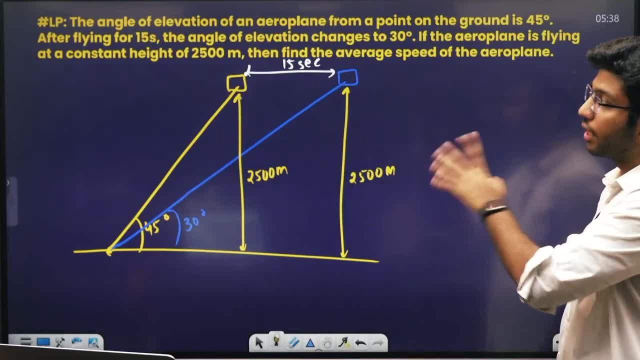 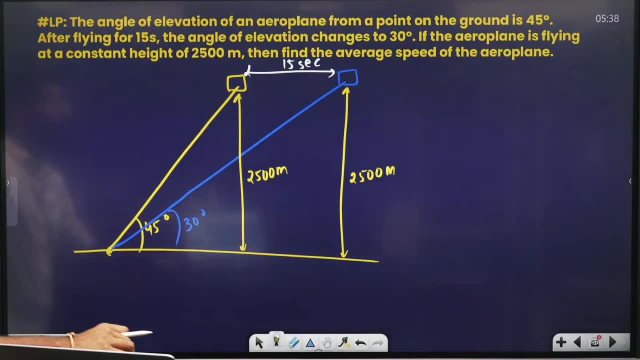 I am telling you that, See, See First of all this: The question about aeroplane which I did in marathon. The question about aeroplane which I did in marathon, See Angle of elevation of aeroplane. 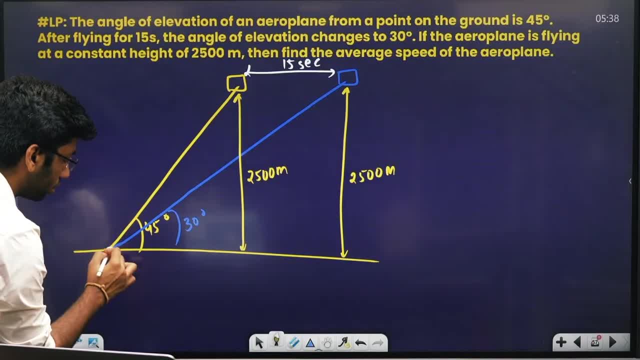 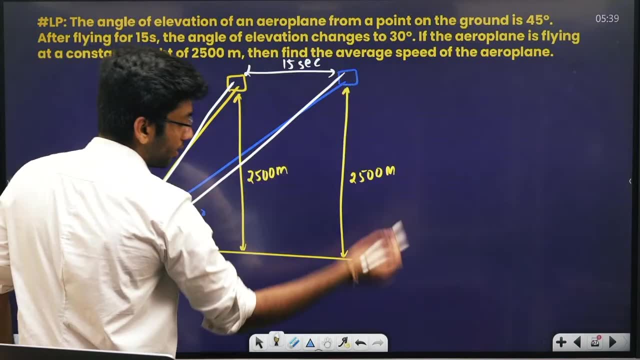 from a point on ground is 45. So if I am looking from here, then it is visible at 45 degree. After 15 seconds, after 15 seconds of walking its 30th second, it is at 30 degree. 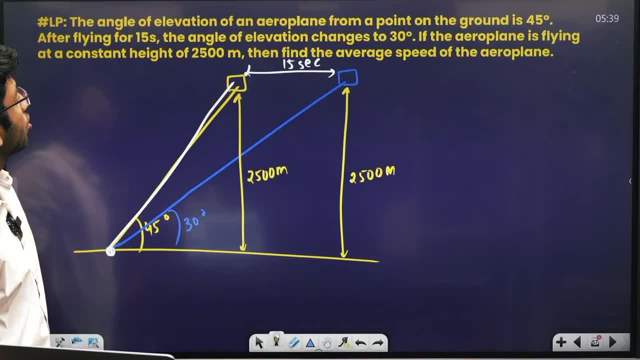 After walking for 15 seconds, it is at 30 degree. If the aeroplane is flying at constant height of 2500,, running at the height of 2500, find the average speed. So we have to tell the speed. 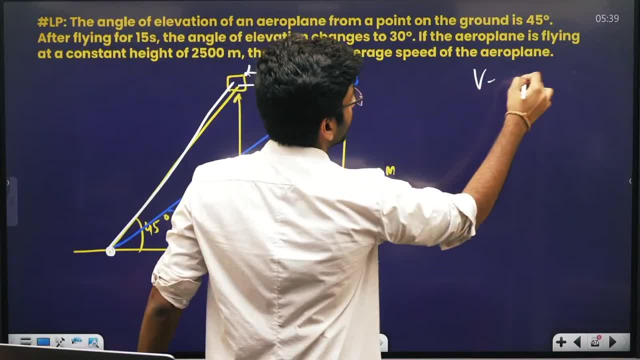 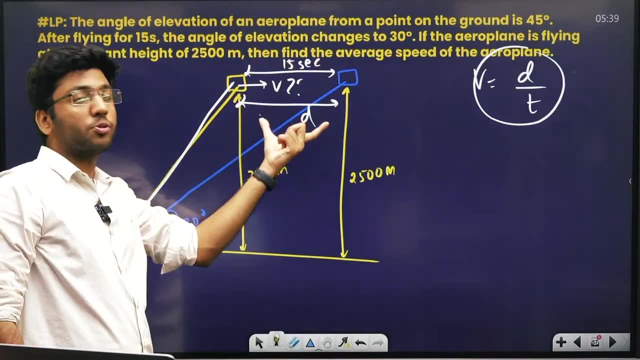 We have to tell the speed What is speed? Speed is distance upon time. So I know the time. Somehow I know this distance. If I know the distance of this much time, then I will calculate the speed by doing distance upon time. 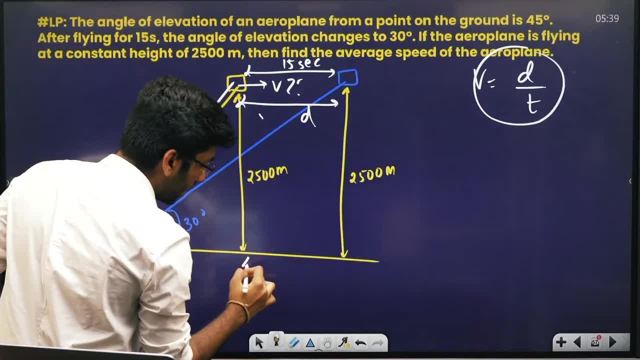 So how will we know the distance? We have to find out this d. We have to find out this d. How will you do it? So, once you will apply trigonometry in this triangle, Apply trigonometry in this yellow triangle. 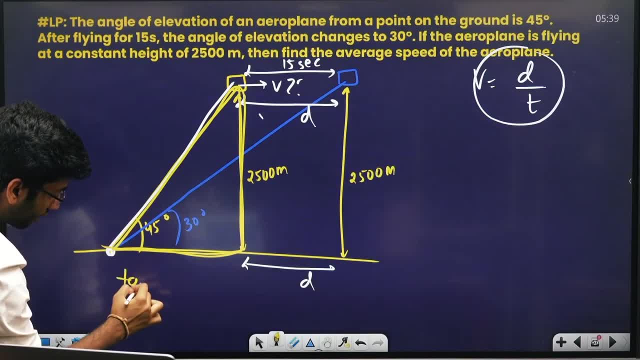 in this small triangle. So this is 2500, 10, 45,, equal to 2500 upon upon. If I consider this as x, then x is x, 45, 1 is there, So x is equal to 2500,. 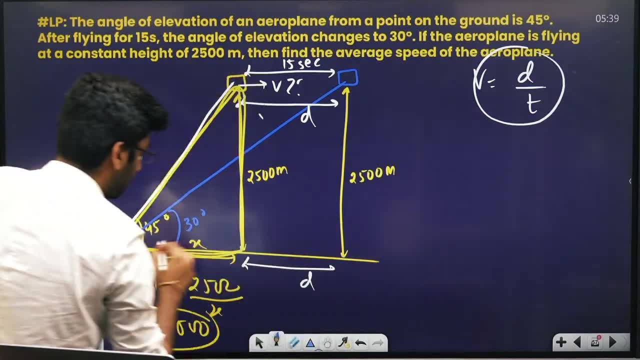 so this is equal to 2500.. Now the blue one. Now I will apply trigonometry in the blue one, I apply trigonometry in the blue one, I apply trigonometry in the blue one. so 10,, 30,. 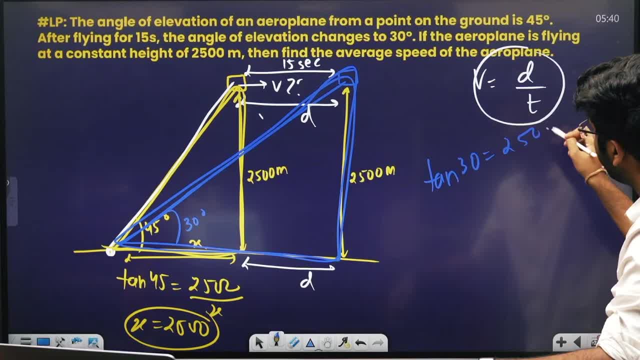 10, 30 will be. It will be 2500 upon x plus d. 0, 1 by root 3 is equal to 2500 upon x. The value of x is 2500 plus d. So if cross is multiplied, 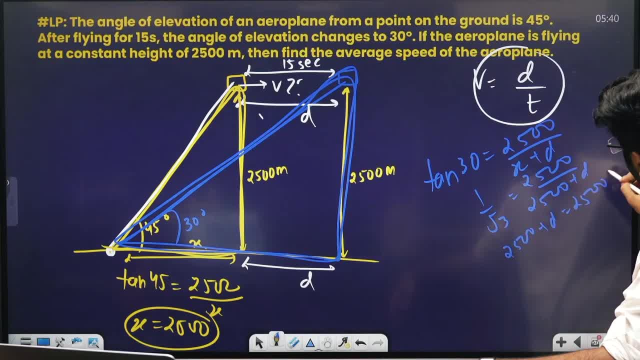 then 2500 plus d is equal to 2500 root 3.. So the value of d is 2500 into root 3 minus 1.. This is the value of d. If you know d, then divide by time. 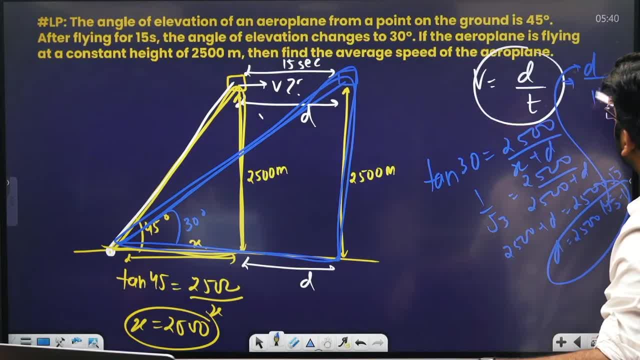 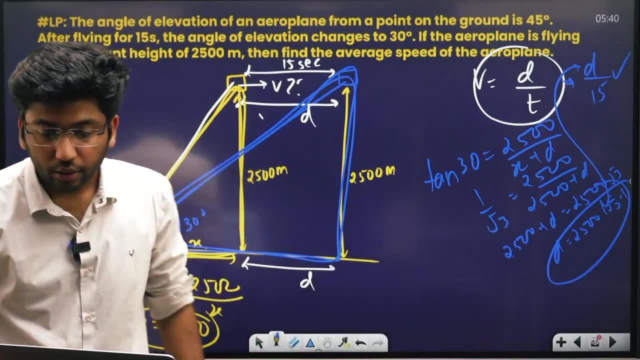 If you know d, then what is the time? 15.. This will be your answer speed. So d by 15, this is your speed. Okay, Okay, Okay, In this way you will do this question, One famous. 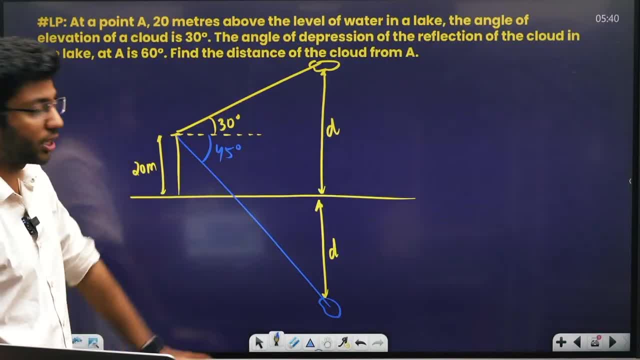 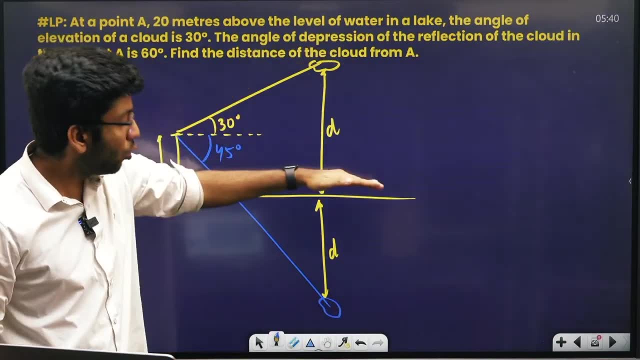 Second. second, this cloud, one Cloud, has only one concept: The higher the cloud is, the lower the shadow will be. The higher the cloud is, the lower the shadow will be. You should know this. So it is a point A. 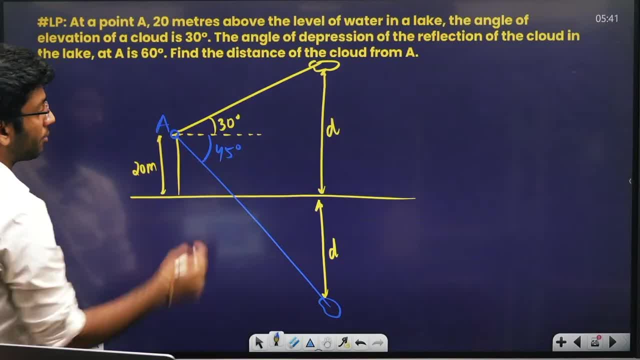 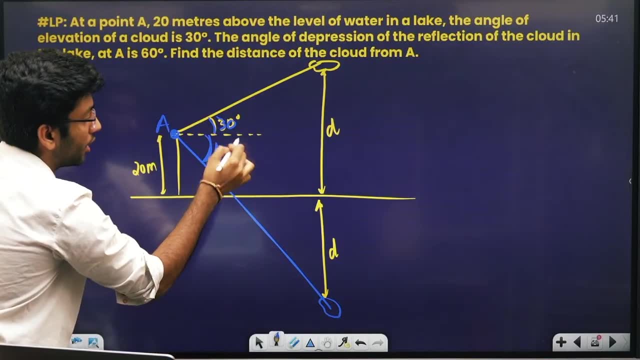 20 meters above the water level. So this is point A, which is 20 meters above. If I divide this by d, then it is 30 degrees, And if I see its shadow, then it is 45 degrees. So we can see it is 30, it is 45.. 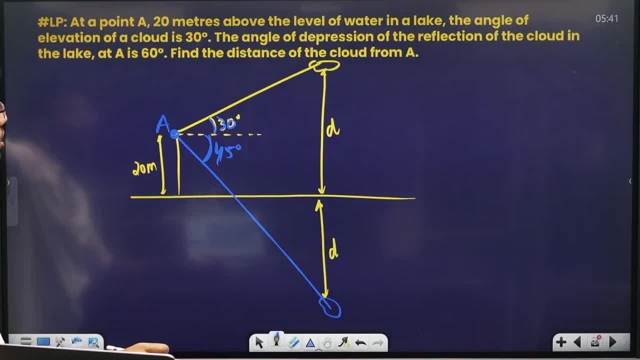 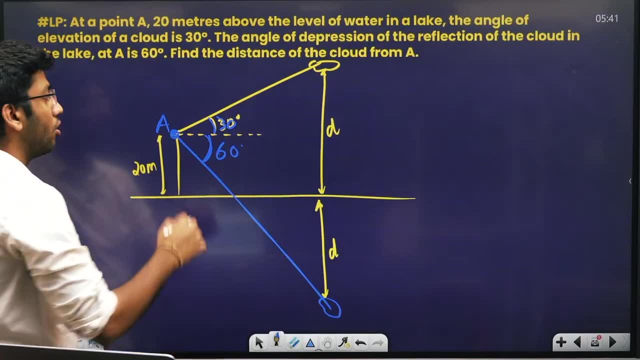 So angle of depression is this. So angle of depression is 45.. Not 45,, it is 60.. 60,, 60,, 60 is written. Angle of depression is 60.. Find the distance of cloud of A. 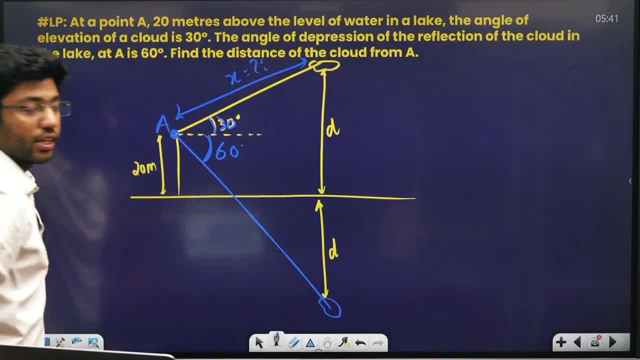 So we have to find the distance of cloud x from A. How will you find it, Look? the question of applications of trigonometry is: you don't have to do anything, just make triangles and play. So look, one is this triangle. 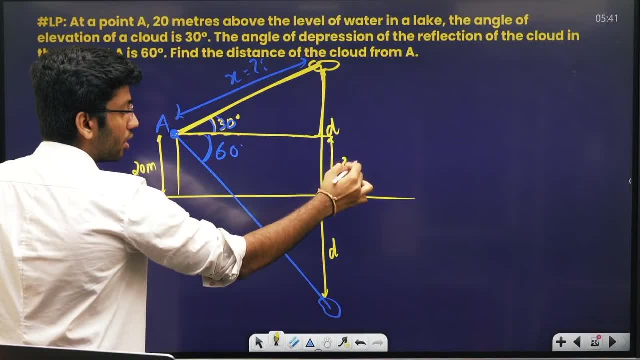 One is this triangle: If this is 20,, then this is also 20.. If this is 20,, then this is also 20.. So let's see the upper triangle once. So if the total is d, then this is d minus 20.. 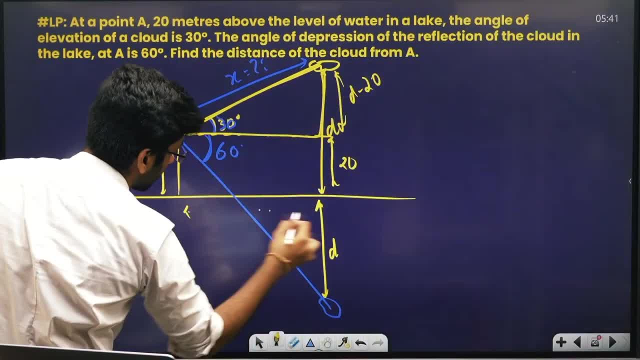 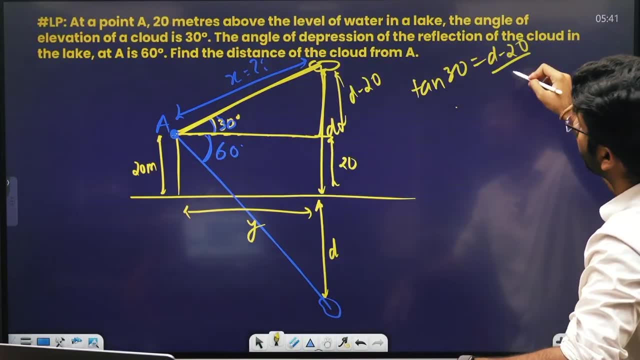 Okay, And if the distance from here to here is y, So if I put it in the upper triangle, then tan 30 equals d minus 20 upon y. So 0,, 1 by root 3 equals d minus 20 upon y. 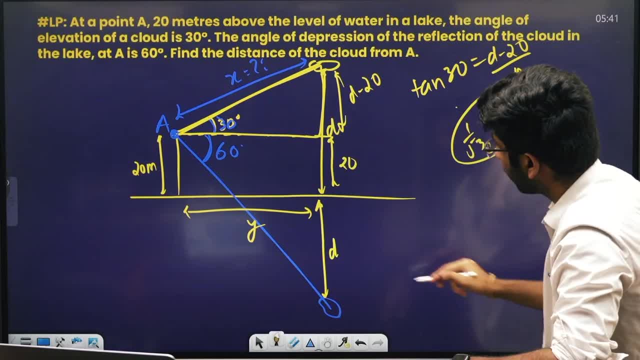 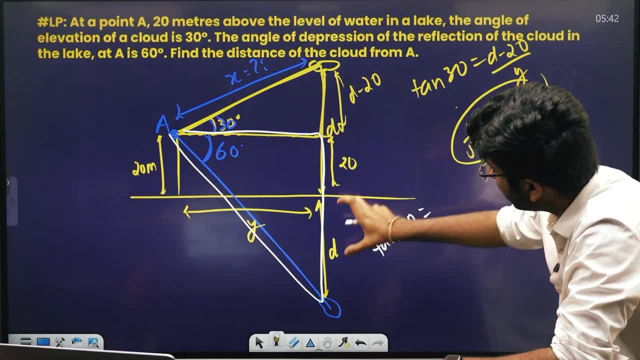 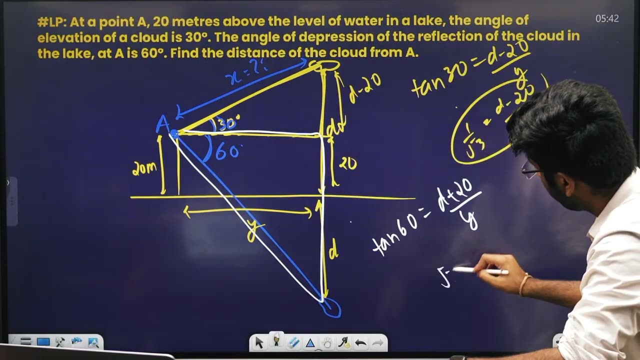 This is done in the upper triangle. Now if I put it in the lower triangle, if I put the trigonometry in this lower triangle, then look, tan 60 will be equal to d plus 20 upon y 0, 1 by root 3 equals root 3.. 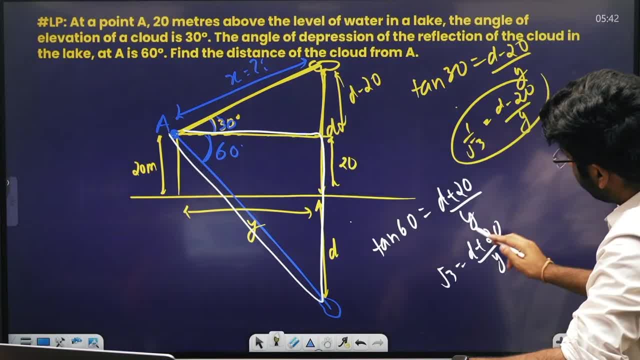 d plus 20 is equal to d plus 20 upon y. So from here two equations have been made in d and y. d minus 20 upon y is 1 by root 3.. d plus 20 upon y is root 3.. 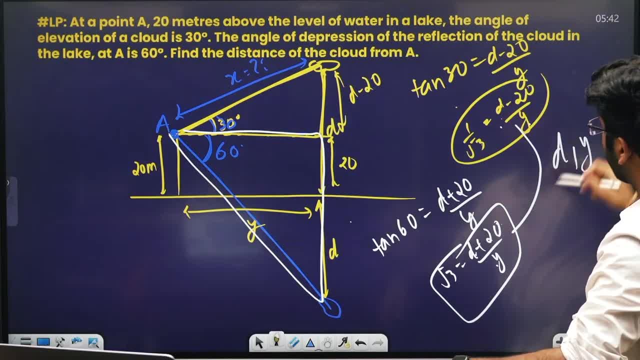 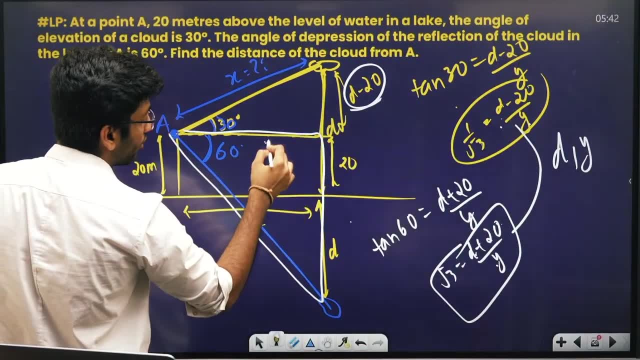 So these two equations have been found. What have you got from this? You will find d and y. You will find d and y from two equations. You will find d and y from two equations. What You will find d and y from two equations. 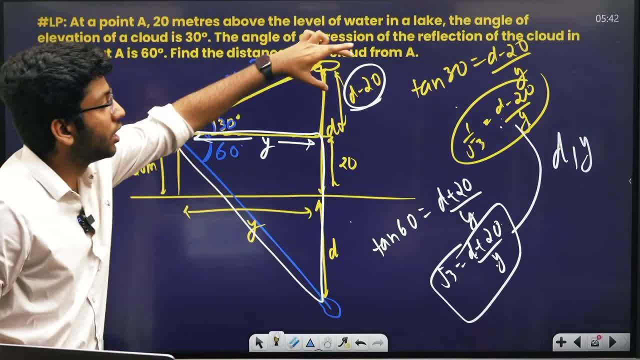 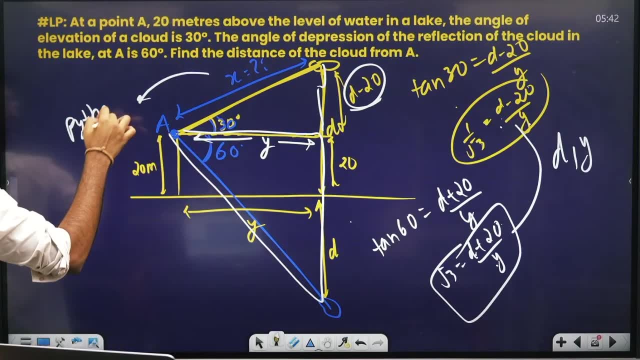 You will find y from here to here. So in this triangle you will find this length and this length. So how will you make this unknown length? You will subtract this unknown length from pi. You will subtract this unknown length from pi. 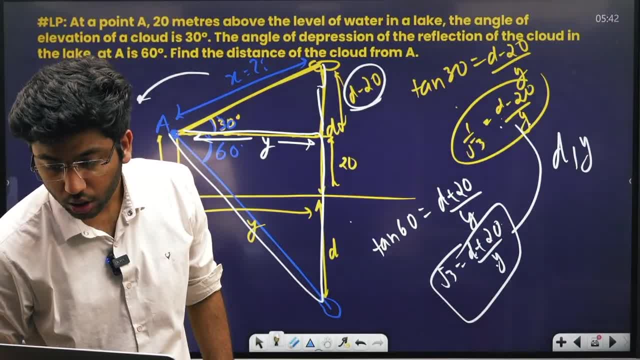 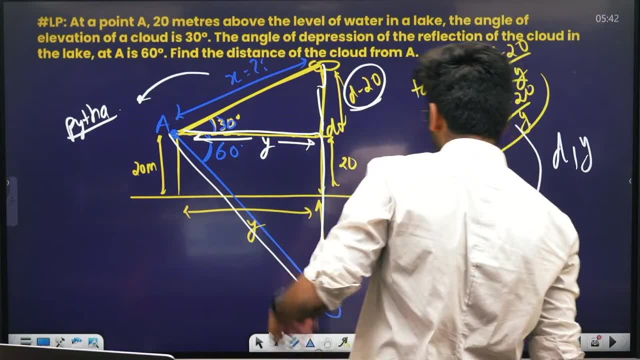 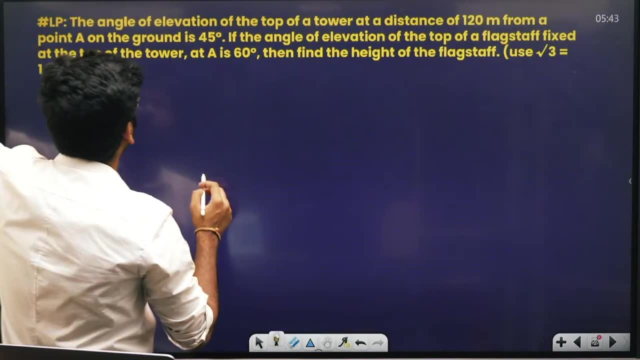 Okay, Okay, I am feeling sleepy. Okay, The angle of elevation of top of the tower from a point A, This flag question is very important. The angle of elevation of top of the tower. There is a tower. I will make a diagram for you. 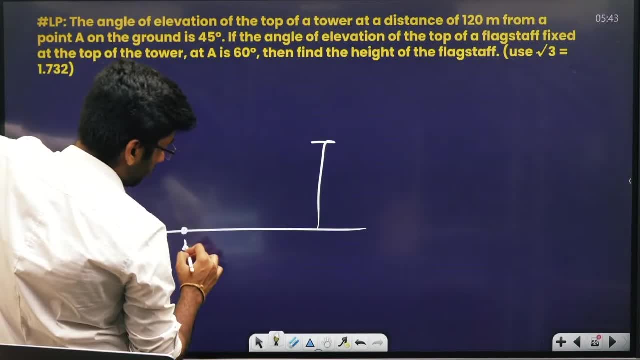 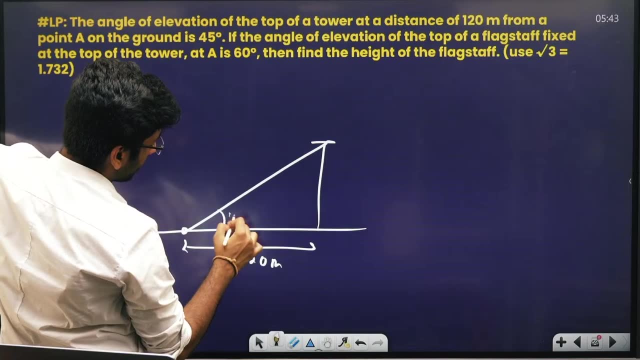 You will do it later. The angle of elevation of top of tower is 120 meters away. The angle of elevation of top of tower is 45. If the angle of elevation of top of flagstaff Flagstaff means there is a flag on top of it. 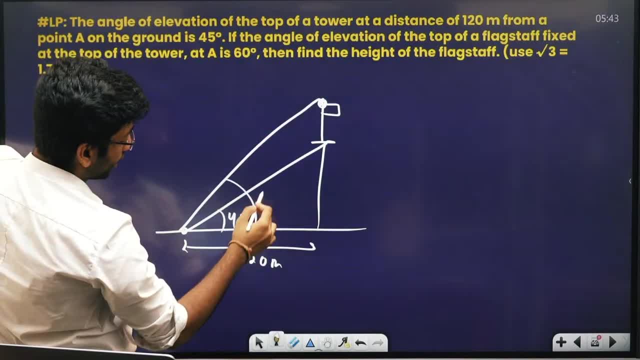 If I look at the top of it, then how much is the angle of elevation? It is 60 degrees. Then find the height of flagstaff. We have to tell the height of flagstaff. We have to tell the height of flagstaff. 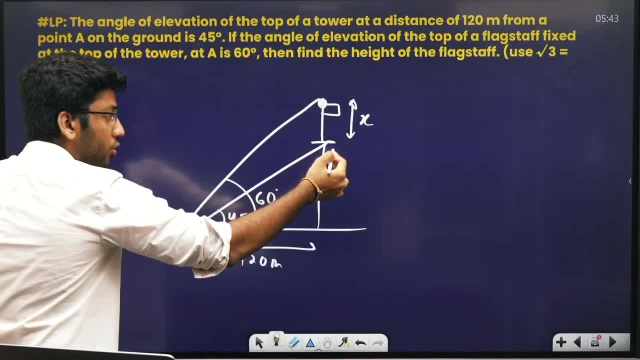 We have to tell x. So what will you do? Once you put it in this triangle, you will find this height, You will find h, And once you find it in the big triangle, you will find h plus x upon this. 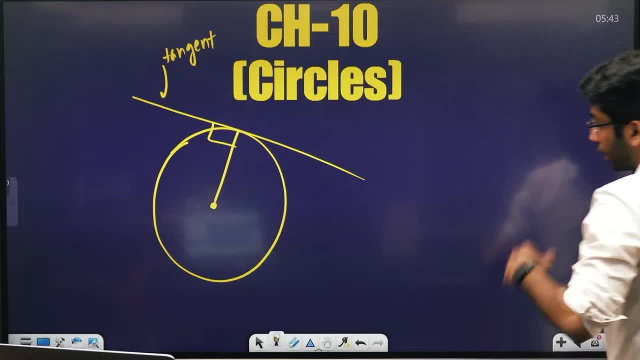 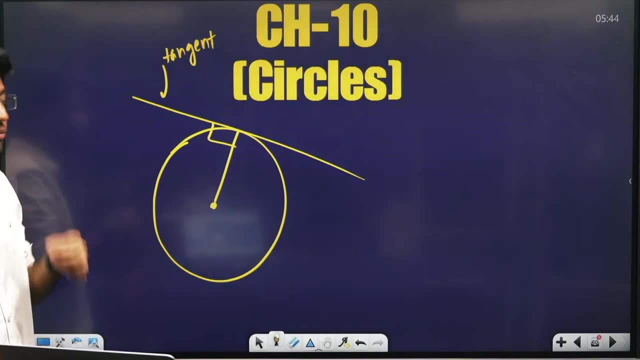 You will find this: x. Okay, So in big and small triangles there will be two trigonometry. You will get the answer: Circle, Circle, Circle, Circle, Circle Circle. See the circle, The tangent, that is the circle. 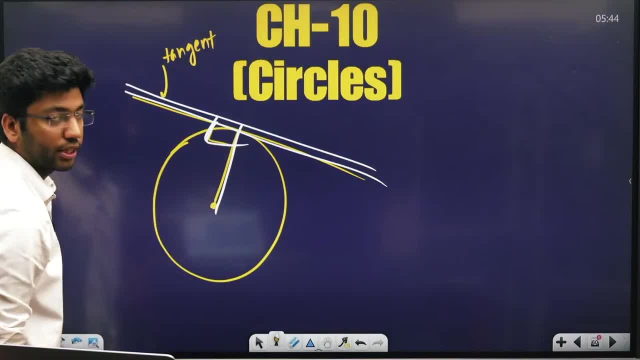 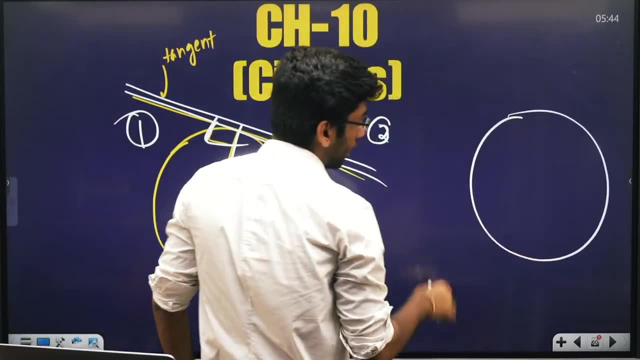 it gets perpendicular to the center. The tangent这个 circle, it get perpendicular to the center. The first theorem of the circle is very important. The second theorem, The second theorem of the circle, is that that if I take two tangents, form exanlterna point. 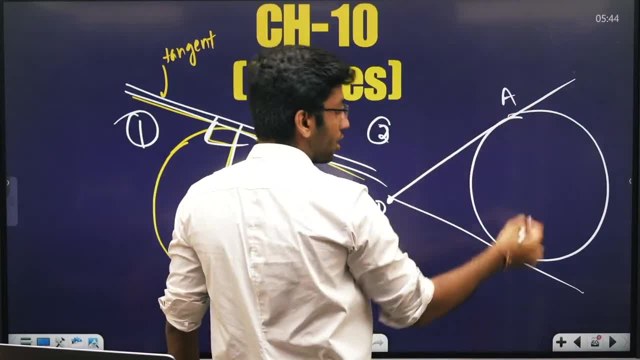 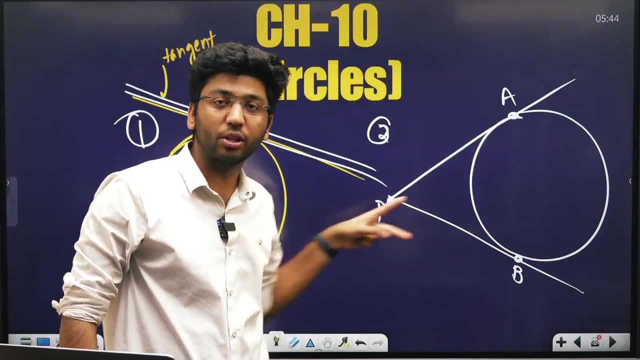 This is point p, so it is a and this is b. So this is a and this is b. So if I take two tangents from an external point of a circle, So this time the length will be equal. 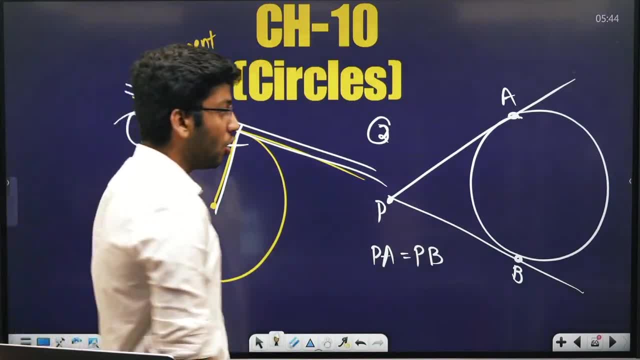 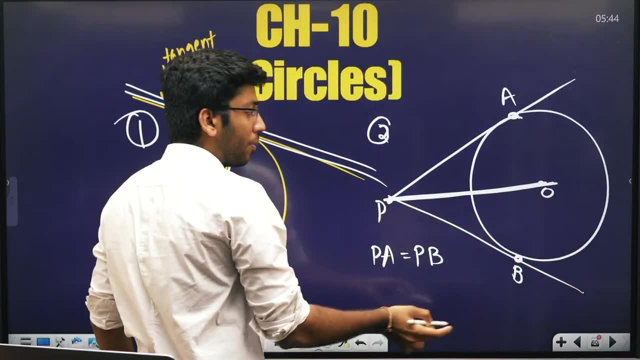 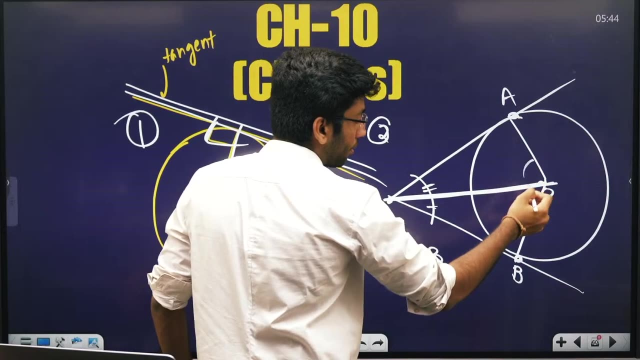 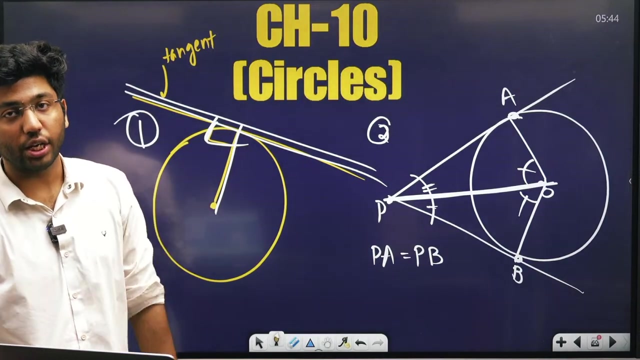 P is equal to Pb. first thing- and suppose I join this point from the center- then the line that is formed, the line that is formed PO, this is the angle bisector of this ie. this is equal to this, and the angle bisector is of this ie. this is equal to this, this is equal to this. this is important. there are four theorems. there are four theorems that you should understand. one is tangent, perpendicular. the tangent is perpendicular to the center. 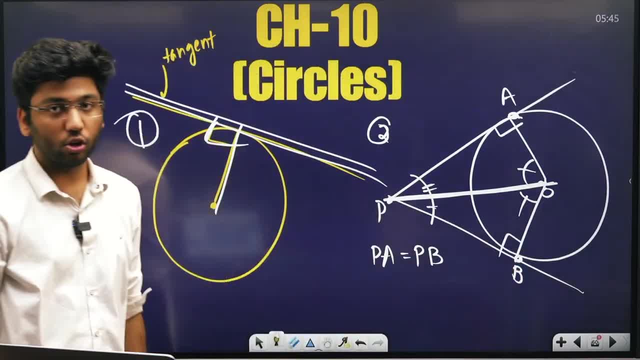 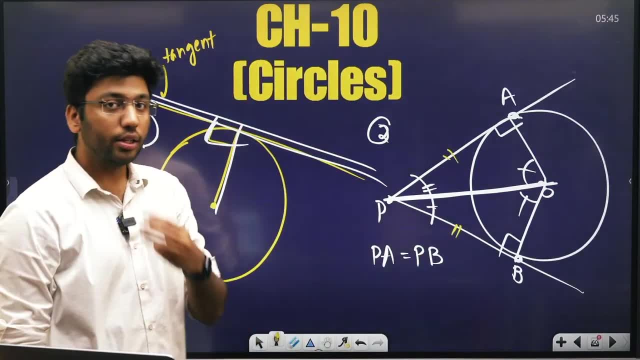 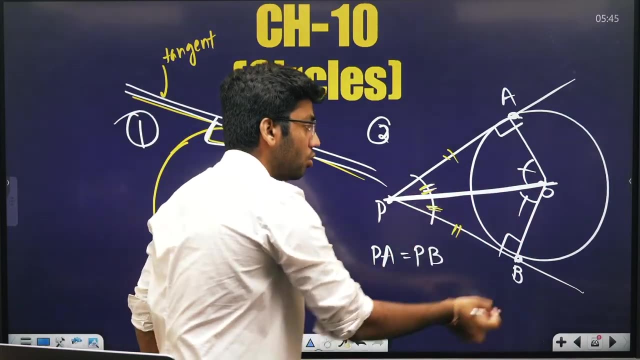 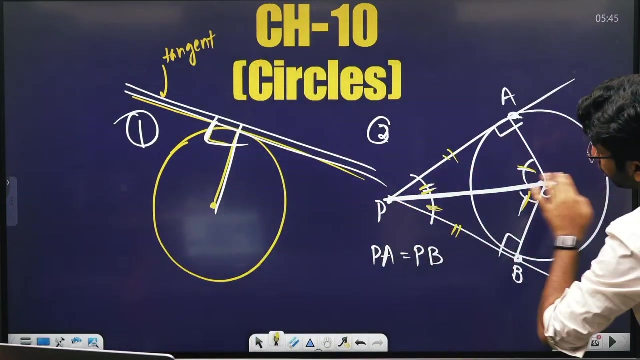 the tangent is perpendicular to the center. the second: the length of tangents is equal to this length. the third thing: this line joining center and this. they both bisect this and this angle. this is bisecting this angle and this is bisecting this angle. this is bisecting this angle. this is bisecting this angle. so it is like this. 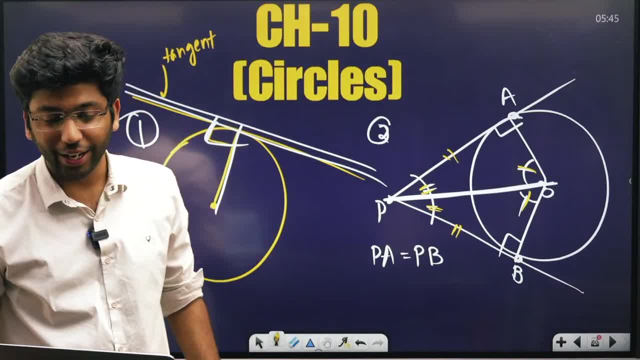 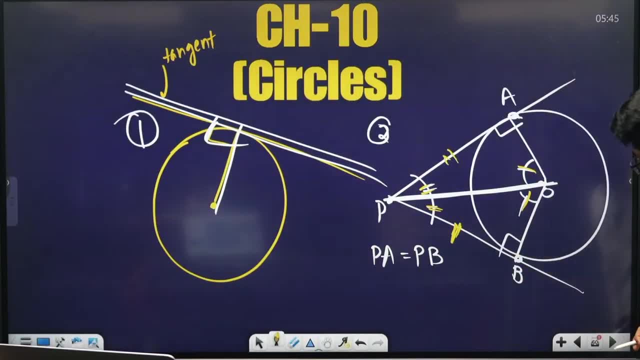 Sir, not yesterday. today is the paper, So we should know these four things. The proof of this PA is equal to PB is asked from you that prove this length of tangent. Prove this length of tangent PA and this length of tangent PB equally. 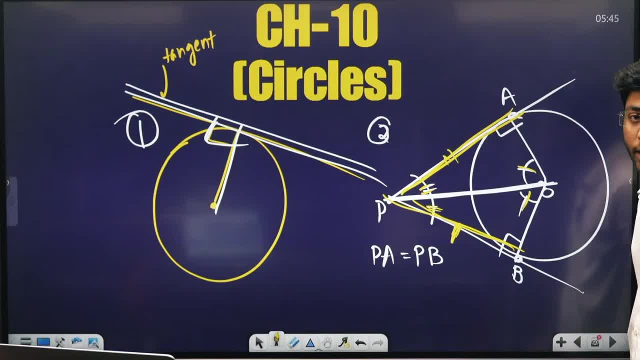 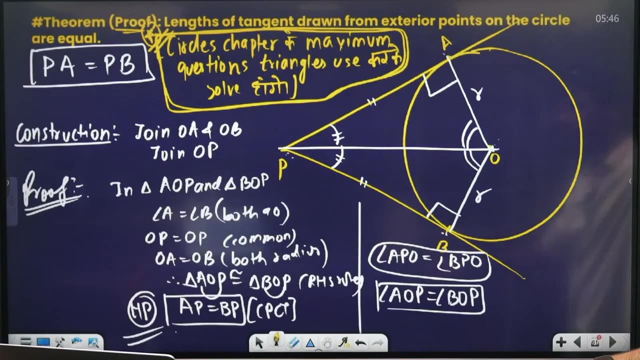 So this PA is said to prove equal to PB. How will you do it? This triangle and this triangle will be proven to be congruent. This triangle and this triangle will be proven to be congruent. How will you prove it? See, this is your theorem. 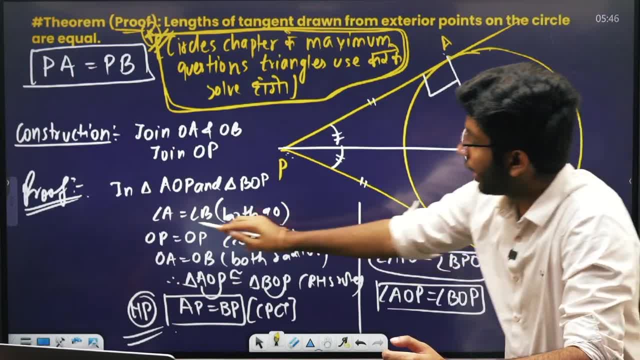 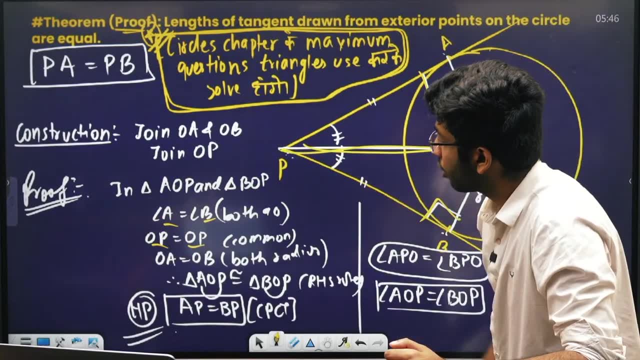 You will prove it to be congruent. So how will you prove it? See, A will be equal to B. This angle A, This angle B, is equal to both. 90.. OP will be equal to OP. Common OP will be equal to OP. 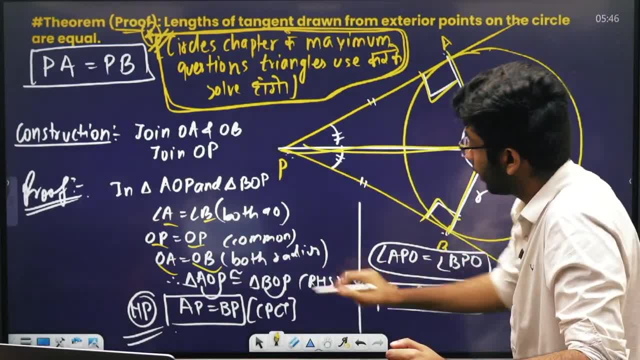 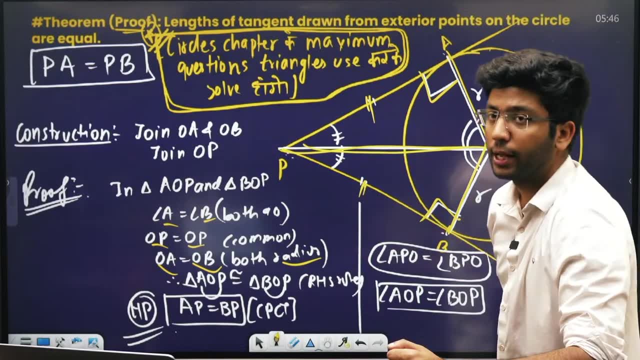 Common And OA will be equal to OB, OA will be equal to OB, Both radius, Both radius. So this triangle and this triangle are congruent by RHS rule. As soon as it is congruent, I will say PA is equal to PB. 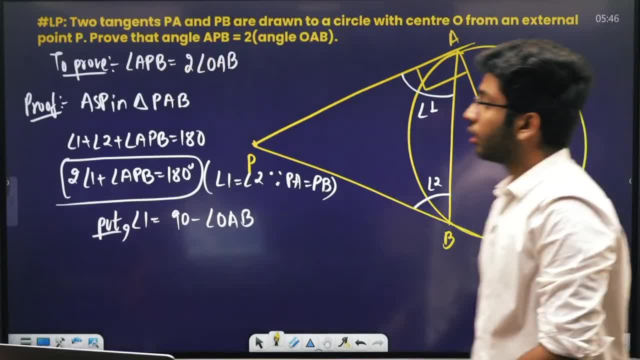 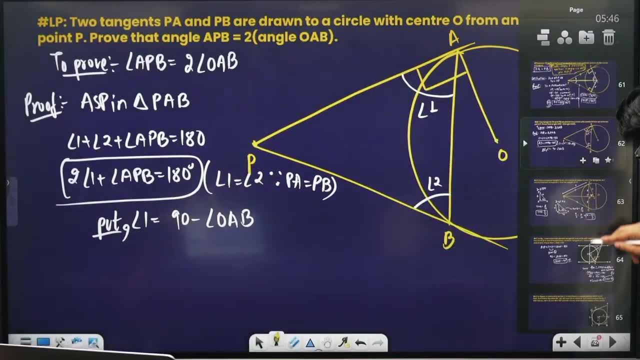 This theorem can come to you. This is for proof. Okay, Next, Three, Three, four. Three questions: One, two, three, The four questions of circle, which is very important, The four questions of circle, which is very important. I am going to tell you that. 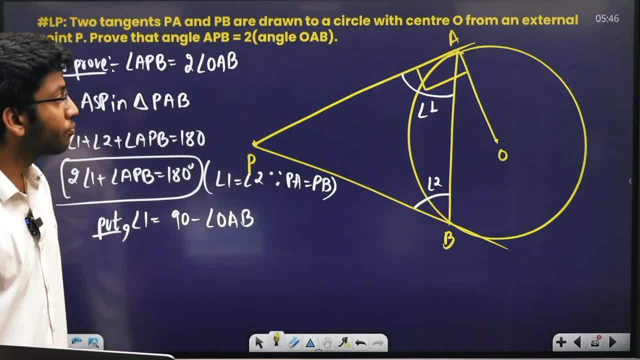 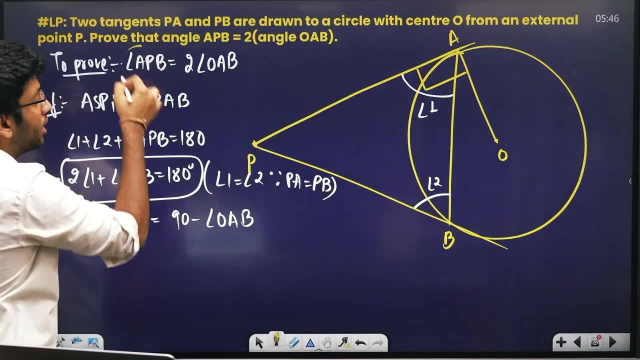 The four questions of circle, which is very important. I am going to tell you that See, See carefully. This kind of diagram will come. You have to prove. You have to prove What That APB is equal to twice of AOB. 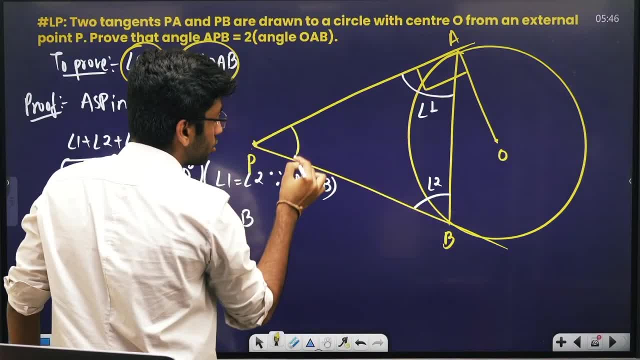 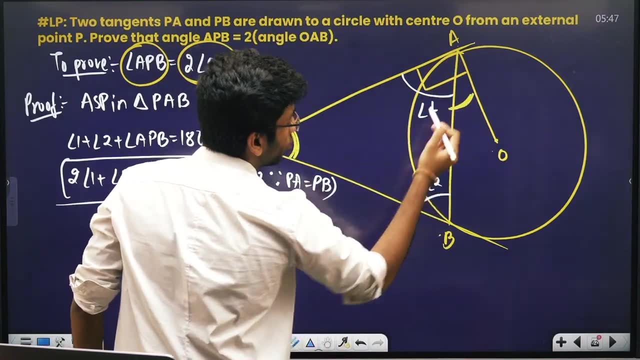 What? This APB angle, This APB angle. This is the angle. You have to prove twice of OAB. OAB Have to prove twice of this angle. Okay, You have to prove this. To prove this, the best way is to put angle sum property first. 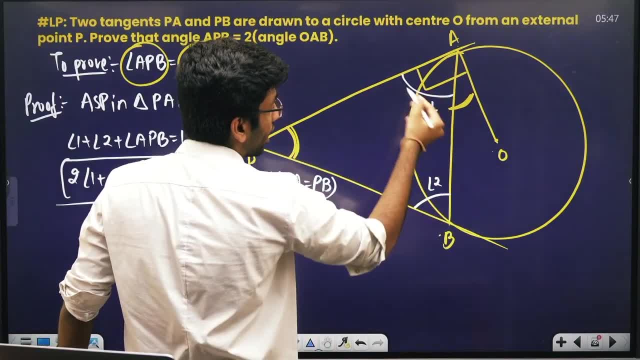 In what In this triangle? Start putting an angle sum property in this triangle. So angle 1 plus angle 2 plus this angle, Angle 1 plus angle 2 plus APB, This will be 180.. Now angles 1 and 2 are equal. 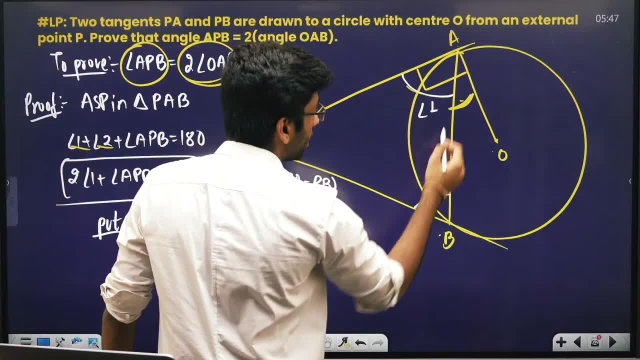 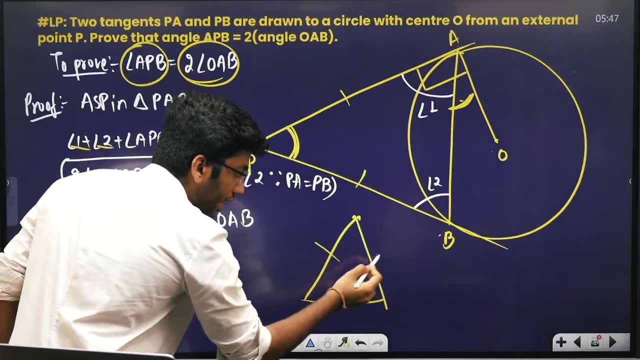 Why are angle 1 and 2? This angle 1 is equal and angle 2 is equal. Why is it equal? Because this is the length of tangent Is equal. If there are two sides equal in any triangle, then the angles in front of it are also equal. 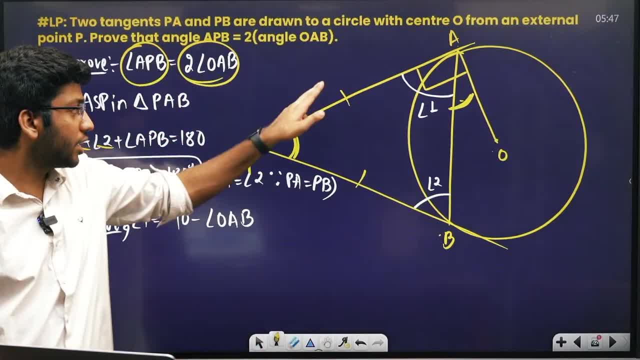 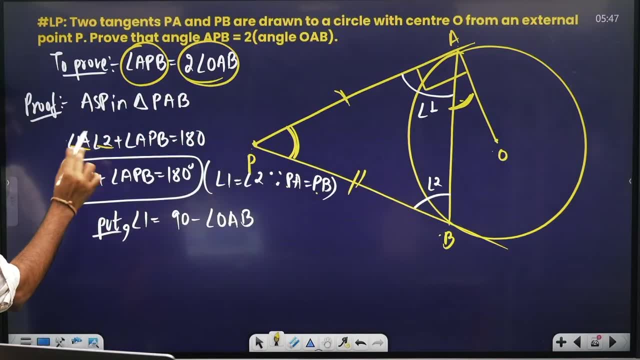 So what did we do? We said that the length of tangent is equal because PA is equal to PB, So angle 1 and angle 2 are equal, So I called it twice of angle 1.. Angle 1 plus angle 2 is called twice of angle 1.. 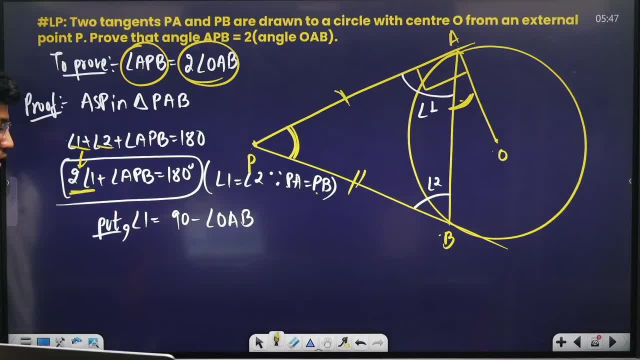 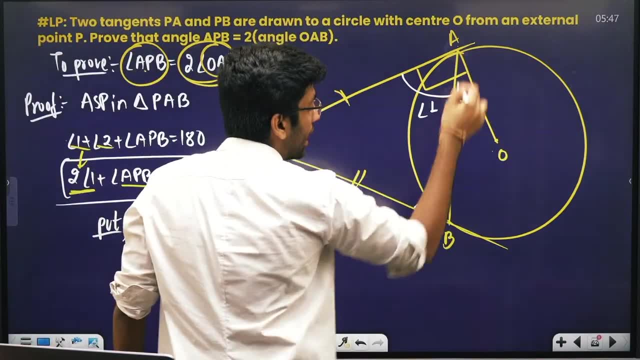 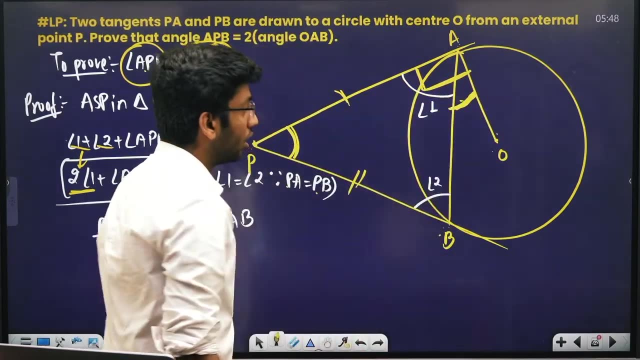 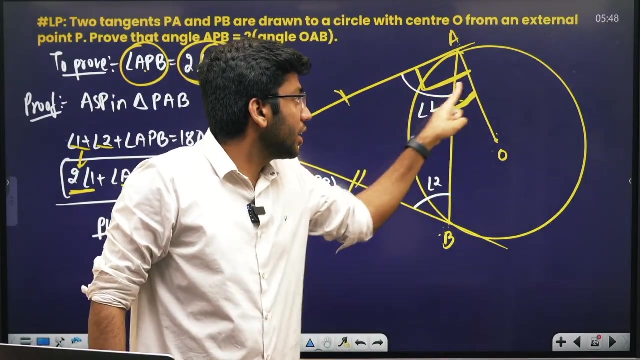 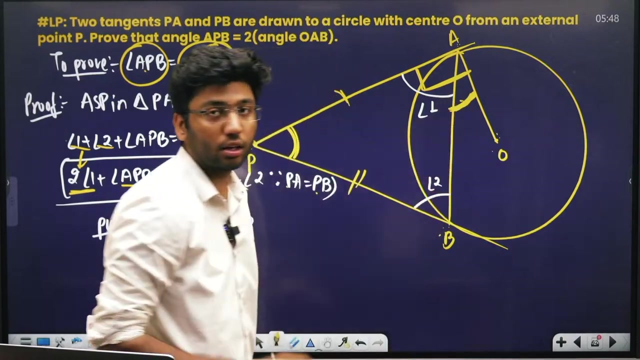 So twice of angle 1 plus AP is also equal to 180.. I got AP also, which I had to prove. I am not getting OAB. Should I remove angle 1 from 90 from OAB? Look carefully, If I remove angle 1 from this 90 degree angle, then I will get OAB. 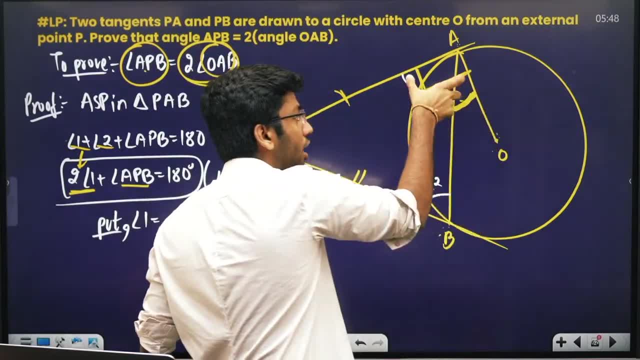 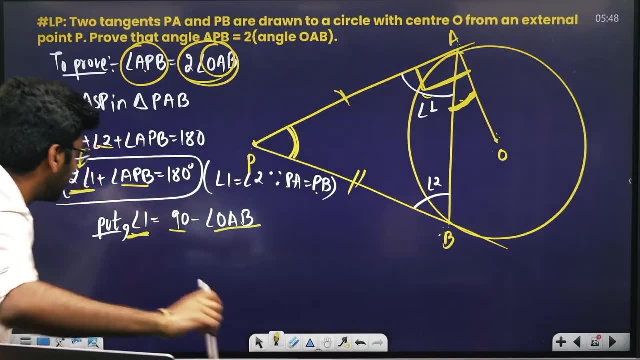 Look carefully. If I remove angle 1 from this 90 degree angle, then I will get OAB. So what did I do? I wrote angle 1 as 90 minus OAB, So I will put angle 1 here as 90 minus OAB. 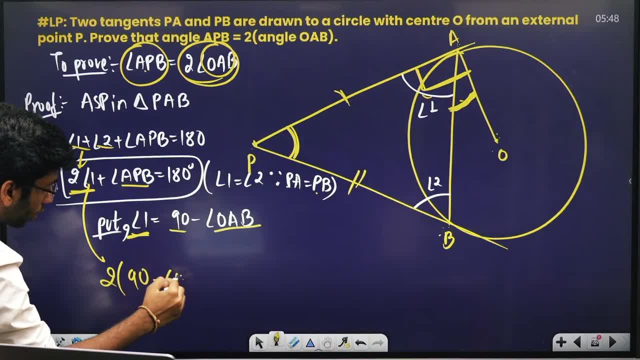 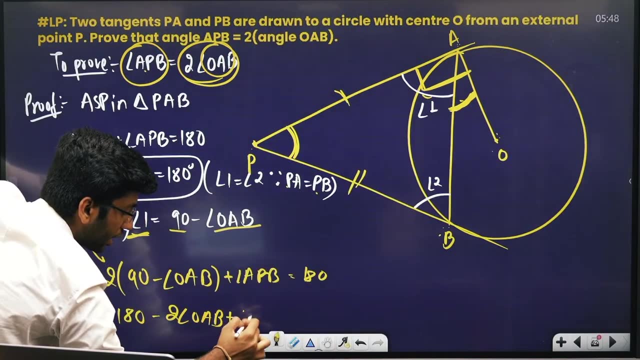 I will put angle 1 here as 90 minus angle OAB, equal to 180.. So this is 180 minus twice of angle OAB, plus angle APB is also equal to 180.. So 180 minus 180 is equal to 180.. 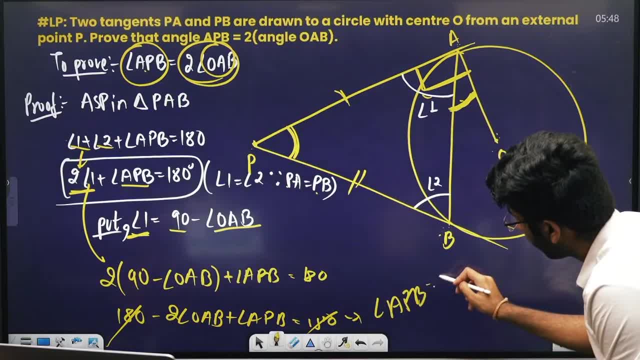 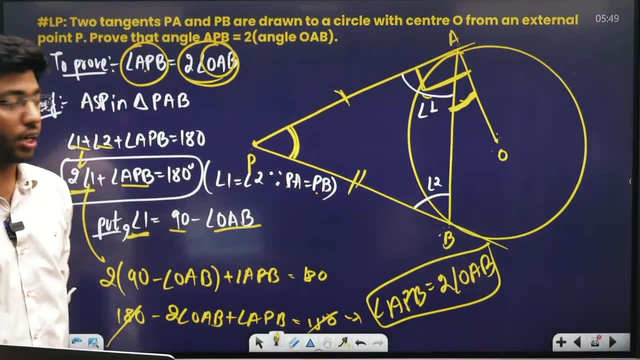 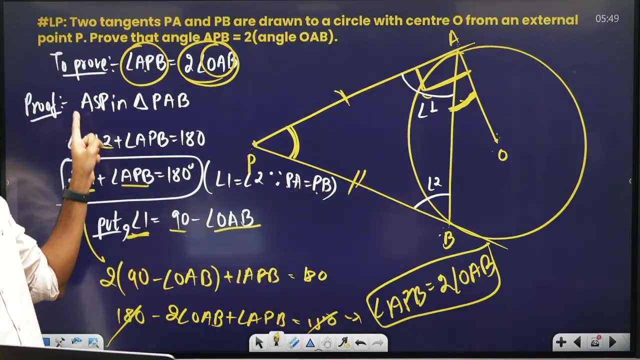 So from here, angle APB is also equal to twice of angle OAB. This is our proof. So we have to do three things. What We have to do? three things: One is to put angle sum property in triangle. So I put angle sum property in triangle. 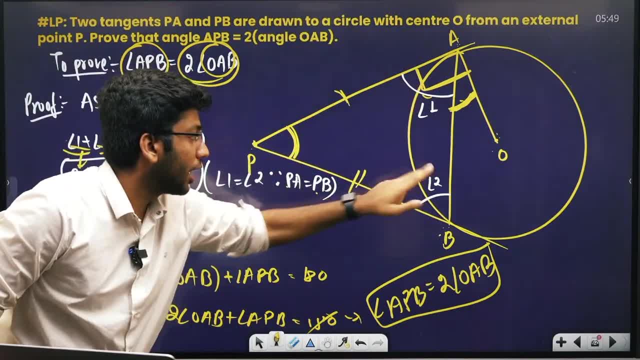 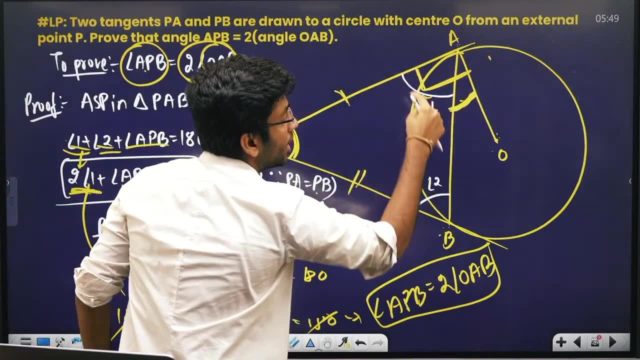 Angle 1 plus 2 plus APB is also equal to 180.. Then I said angle 1 and 2 are equal, So I wrote twice of angle 1.. Then I wrote angle 1.. I wrote angle 1.. From this 90 degree angle I removed OAB. 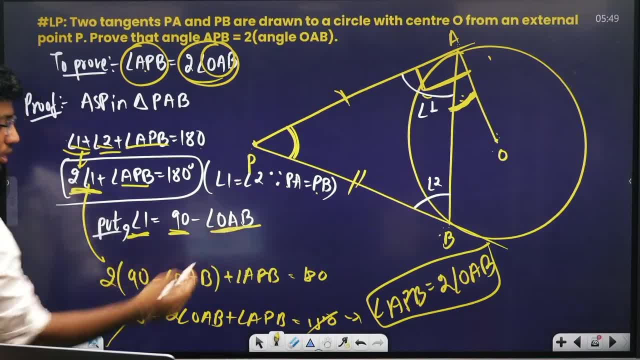 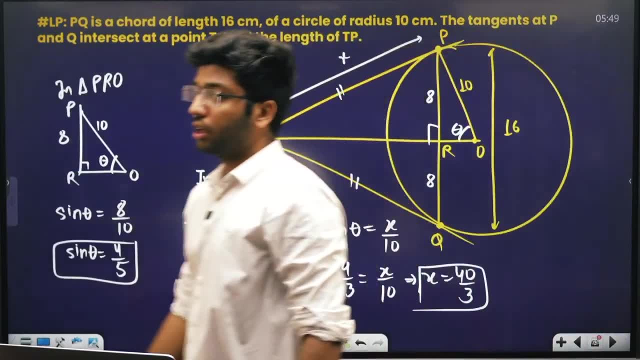 I wrote angle 1.. So I wrote angle 1 as 90 minus OAB. I wrote angle 1 as 90 minus OAB. I got the answer. I wrote 90 minus OAB. I got the answer. Second question, like this will be asked: 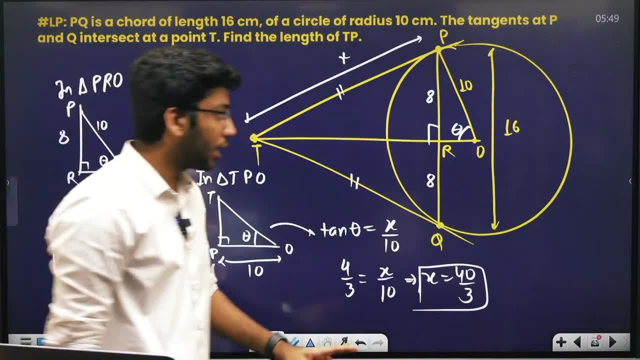 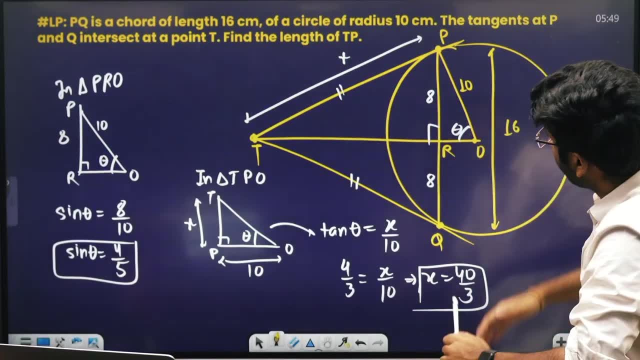 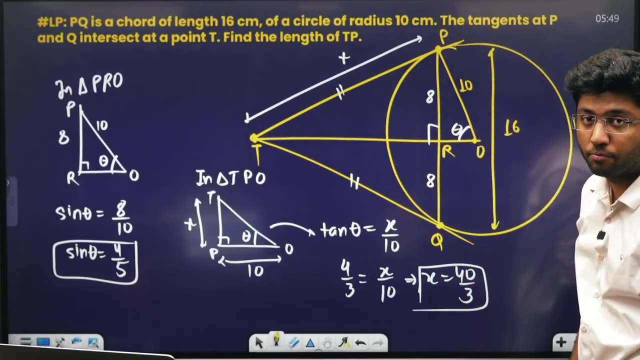 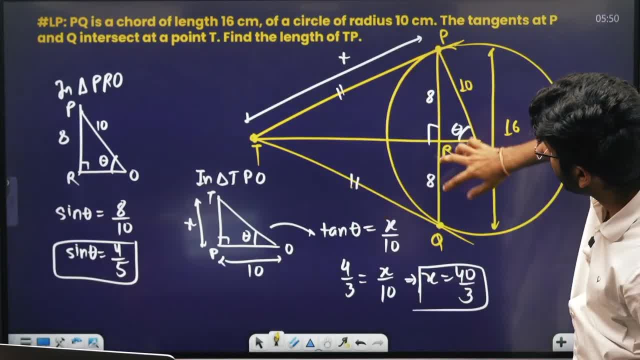 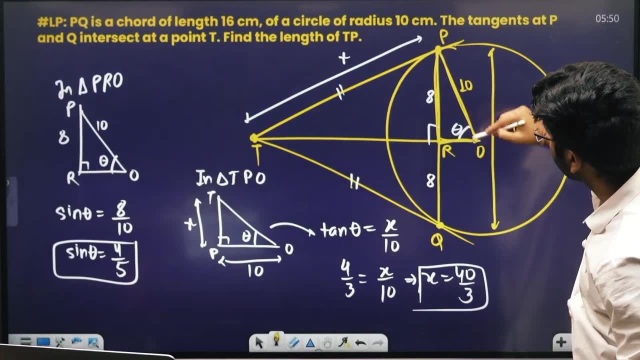 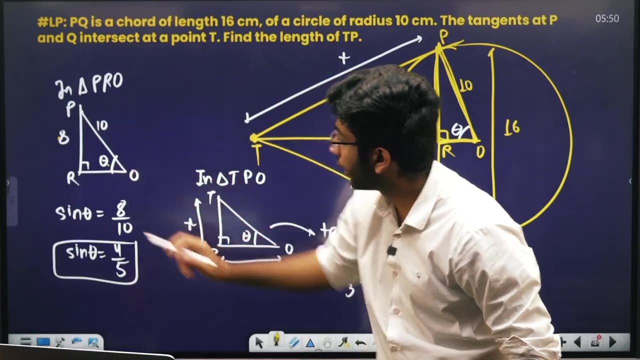 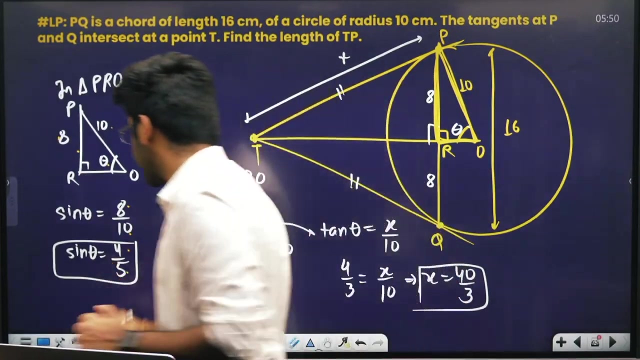 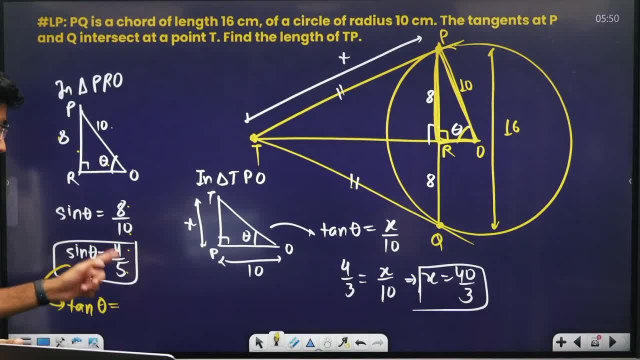 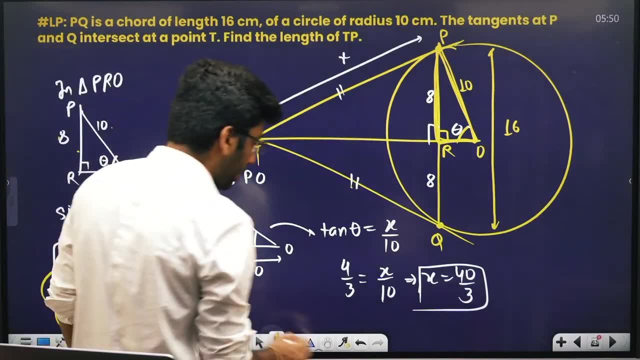 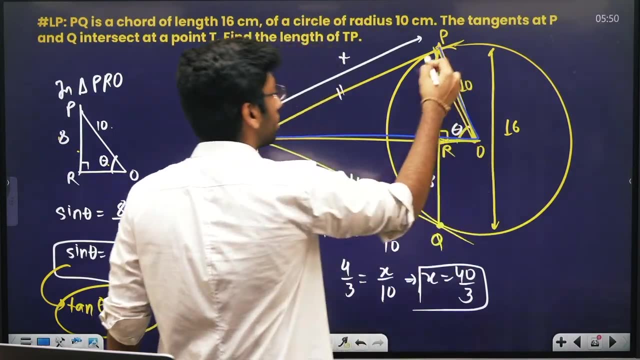 See, See, See, See, See. Okay, See What I made you do, right? Why do I write blind? Yes, Yeah, See, See, See, See, See. I will take this big triangle because this is also 90 degree. 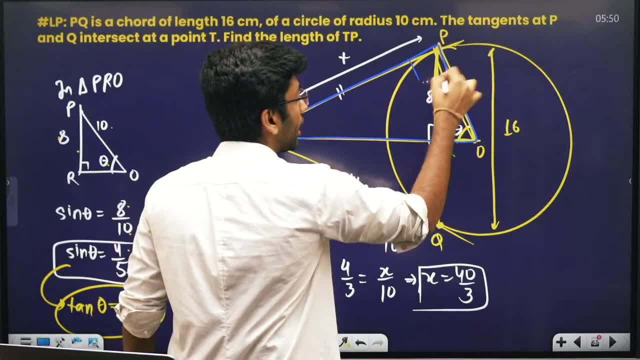 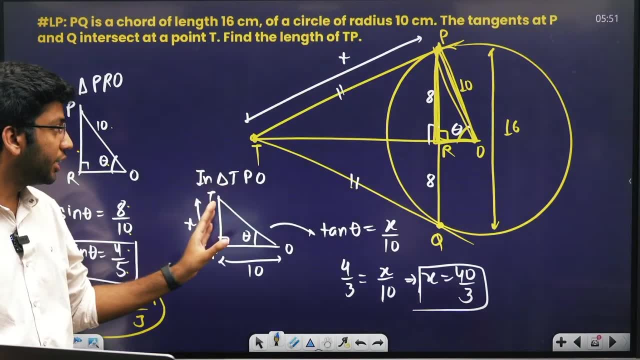 So what I have to do is take this small triangle and this big triangle. This is also 90 degree, So I took both of them. So once I took the small one, I got tan, theta. Now I will take the big one. TPO I have made it here, so I have to take out x and tan is given. 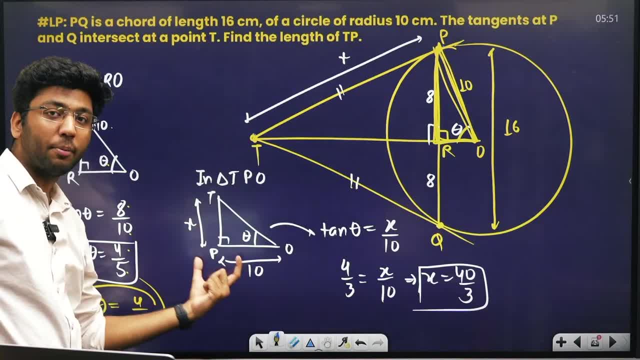 So x has to be taken out and tan is given. Perpendicular has to be taken out and base is given. Perpendicular has to be taken out and base is given. So what I will do is I will do tan theta equal to x by 10. I will keep tan theta equal to 4 by 3. 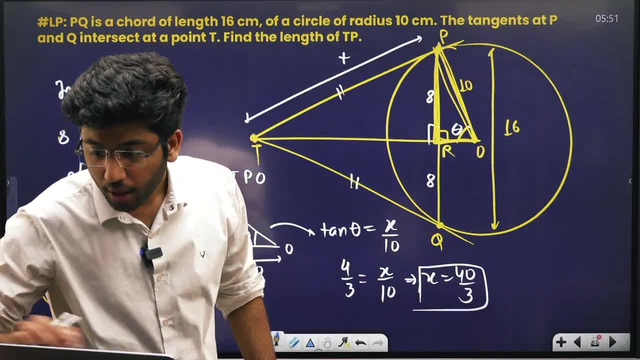 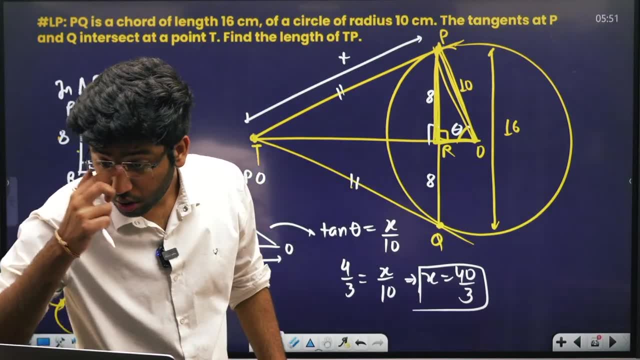 So, from x by 10, the value of x will be 40 by 3. Okay, Okay, Did you understand. Did you understand? So in this way, these are our two favorite questions. There is a chance that one of these two questions will come. 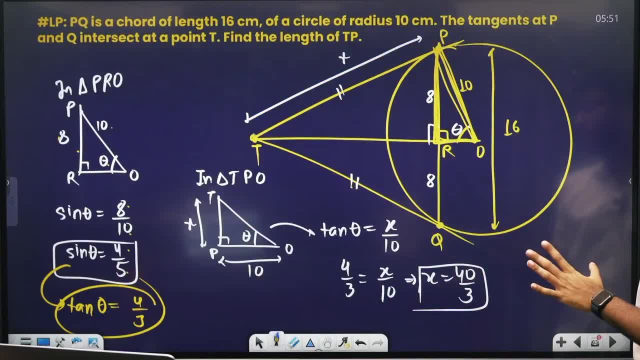 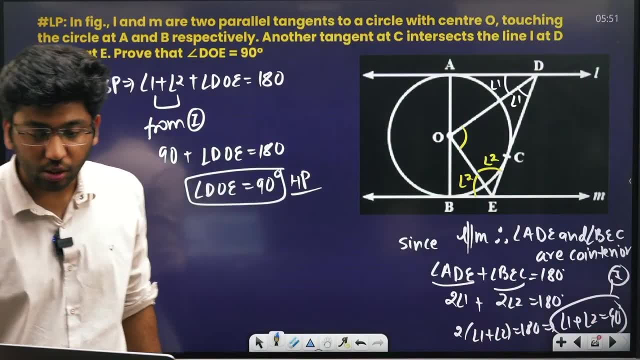 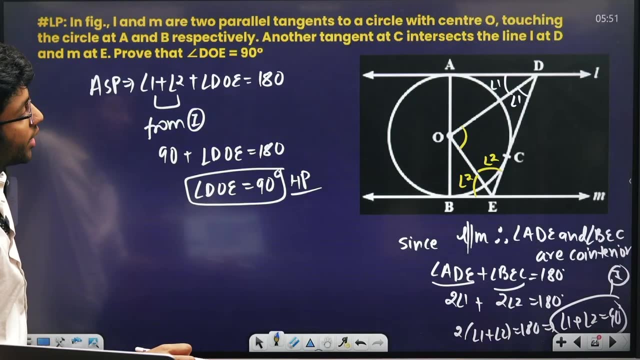 Either this will come or this will come. There is a chance that one of these two will come, Okay. Third, this is a very important question, Very important question. CBC has a very favorite question. See: L and M are two parallel tangents. There are two parallel tangents. 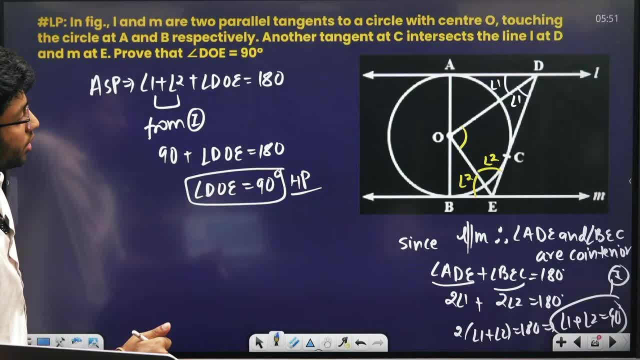 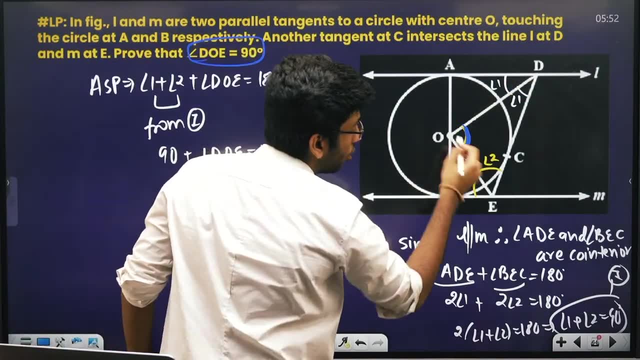 Circle is O. touching the circle at A is also okay. Another tangent C is like this: See, I have to prove DOE equal to 90. This angle is DOE. We have to prove this 90. So if we have to prove the angle of any triangle, 90. 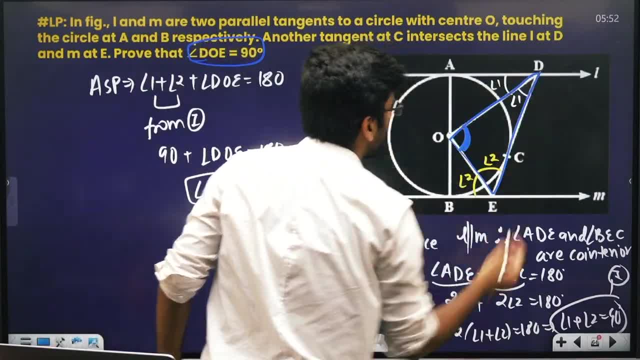 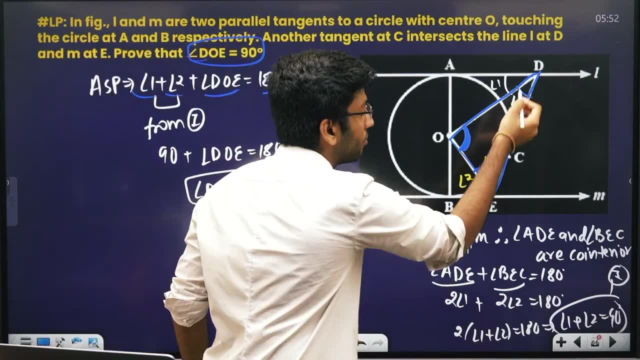 Then we will apply the angle sum property. So I applied the angle sum property in this triangle. So angle sum property means 1 plus 2 DOE equal to 180. I said this is angle 1, this is angle 2, So 1 plus 2 plus DOE. 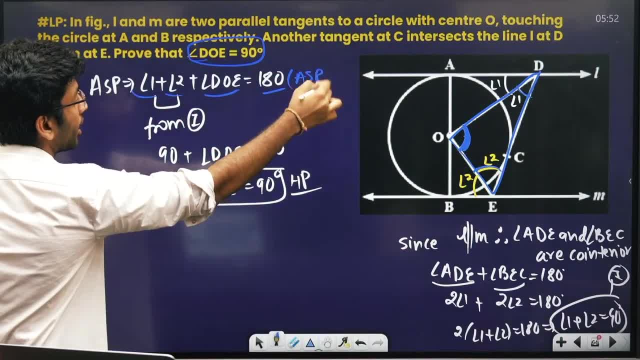 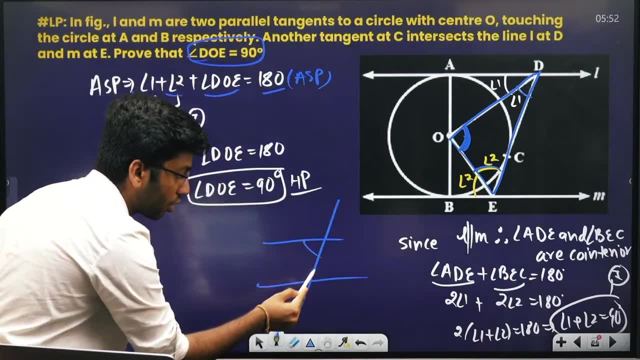 This is done. I applied the angle sum property equal to 180. Now see, now see, my dear, Look carefully, look carefully. This is the most important: If there are two parallel lines. If there are two parallel lines, Then what is the sum of these two? 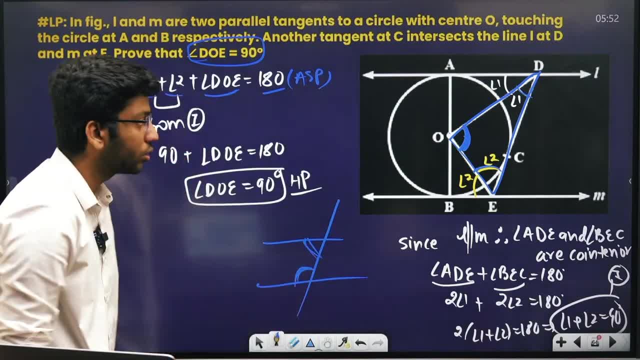 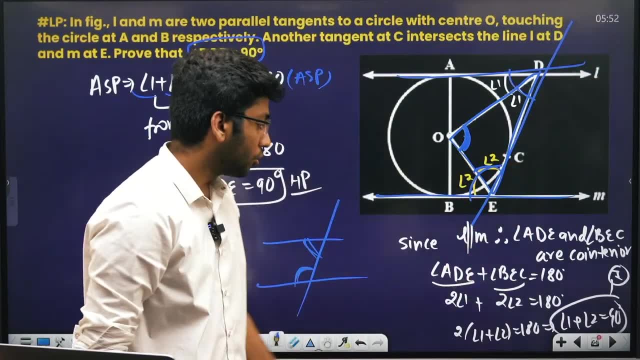 180 is there. If there are two parallel lines, Then what is the sum of these two? 180 is there. So see, these two lines are parallel And this is a transversal. So the sum of this and this will be 180. So it means ADE plus BEC. 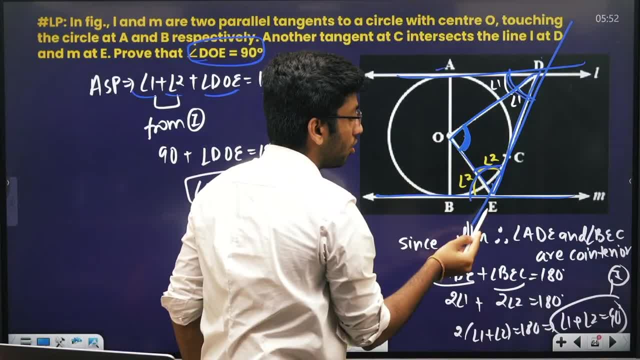 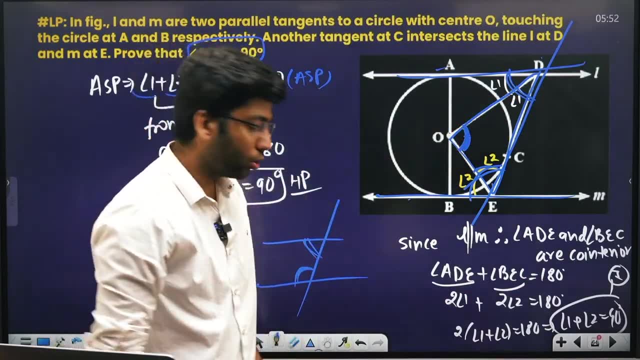 The sum of this will be 180. ADE this angle And BEC The sum of this angle will be 180. The sum of both will be 180. Now I have written 1 equal to 1. Why? Because if I draw a tangent from any triangle, 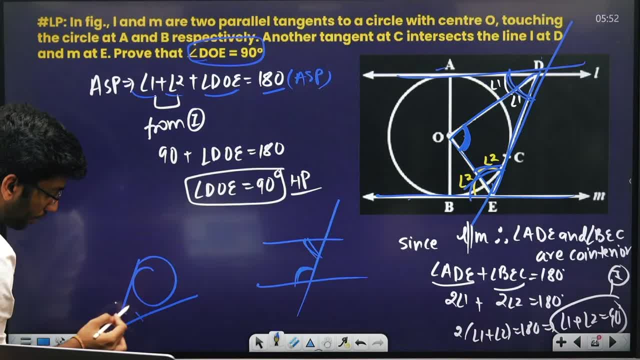 From any distant point of any circle, Then the length is equal. So see, There are two tangents from D point, So the length is equal And the angle between it is equal. So if this is angle 1, Then this is also angle 1, So I have. 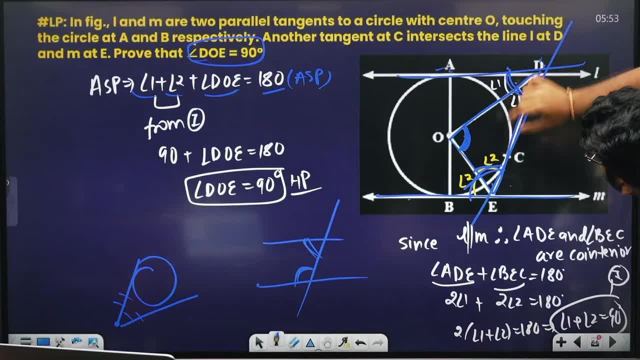 ADE, ADE. I have written twice of angle 1. Similarly, BEC This big angle, I have written twice of angle 2. I have written twice of angle 2. I have taken 2 commas. So angle 1 plus angle 2, Angle 1 plus angle 2 is 90. 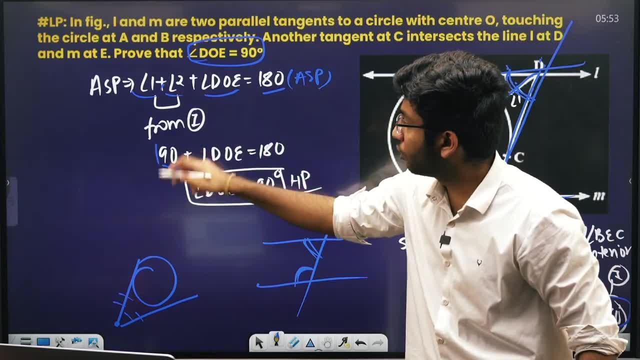 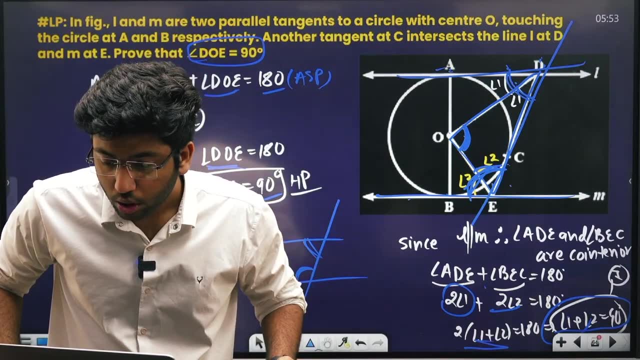 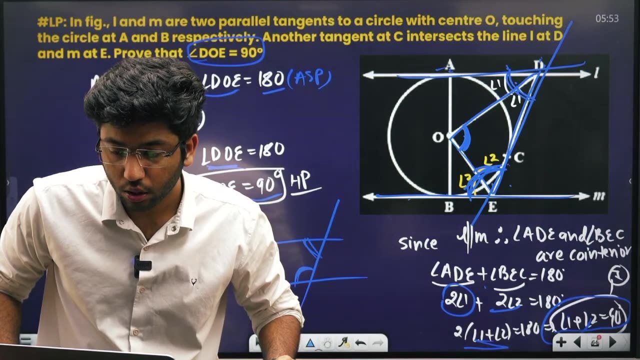 That angle 1 plus angle 2. I have put here Angle 1 plus angle 2. I have put the value of 90, So DOE is equal to 90. DOE is equal to 90, Understood, Understood. Okay, Okay, Got it. 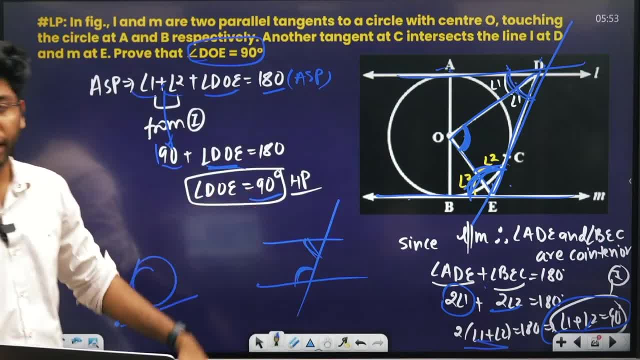 This kind of ohm's problems Are real, Got it? Then these type of this kind of questions Have chances to come. I have told you four questions. Which four questions? One is this kind of question, One is this kind of question And one is this last question. 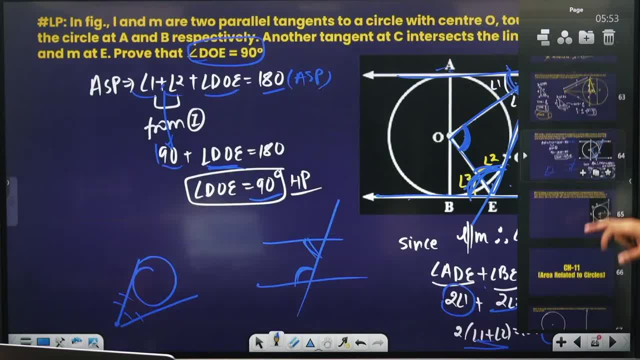 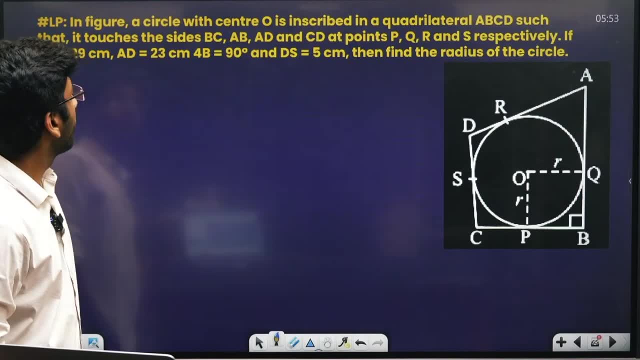 There are chances of coming up. Which them is this question And one is that last question From this chain. What does this QS say? QS says This, QS says This. QS says: QS says In figure center O The qildr ABCDR See. 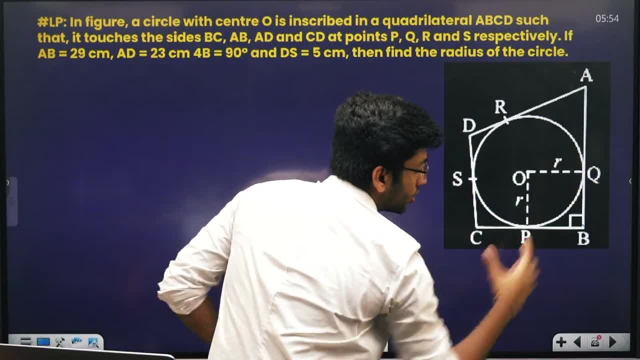 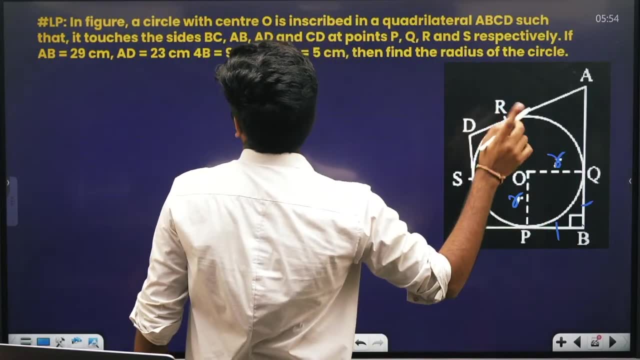 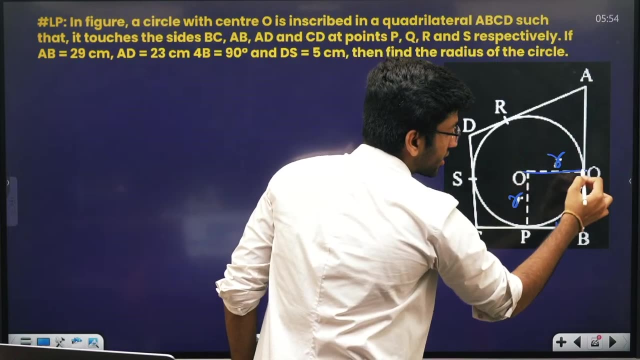 You have 2 tangents from external points, Two tangents from outside point. Means: this length is equal to this, This radius is equal to this, Okay, And it is also said that this 90 degree is 90 degree. If we draw from the center of the circle, then this is also 90. 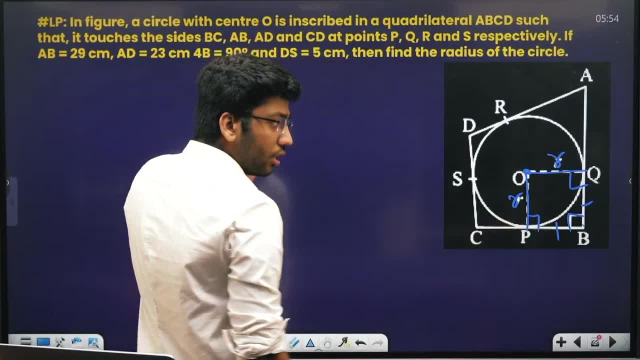 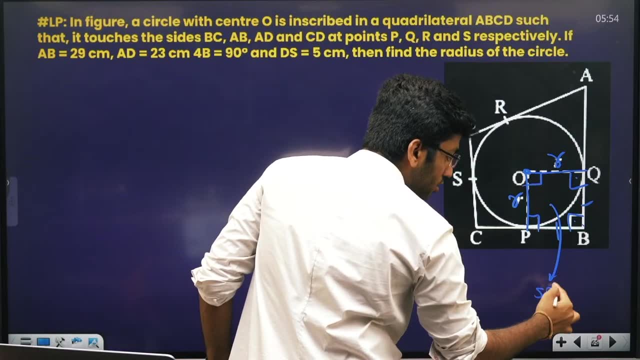 If we contact the point of tangent from the center of the circle, then this is 90, And if the sum of all four is 360, then this is 90,, this is 90, this is 90, then this is 360. Means what is this? This is one square. 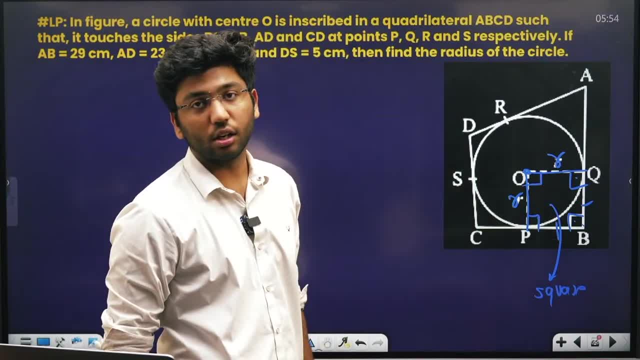 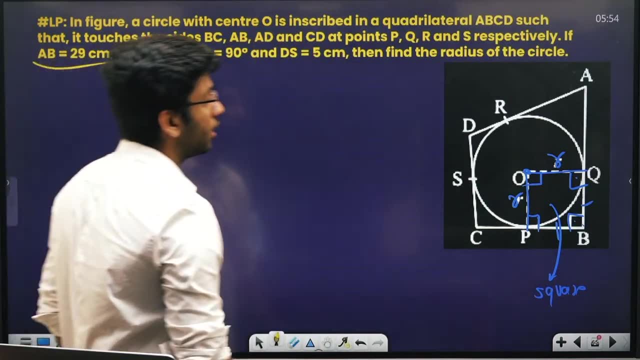 All angles are 90 and the lengths of the sides are equal, So this is a square. When this is a square, then now see. Now see what is given to us. The value of AB is 29. The value of AB is 29 AD. The value of AD is 23. 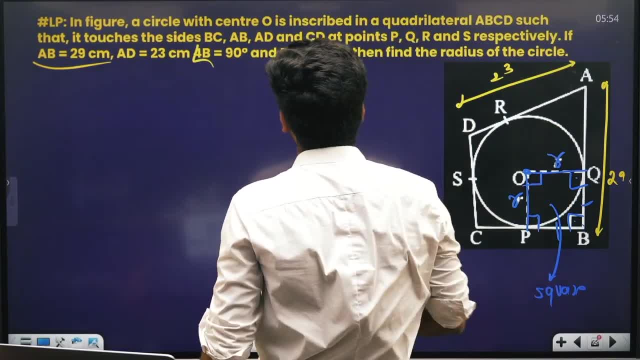 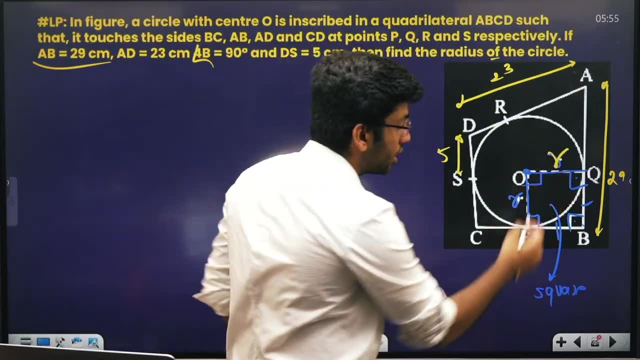 Isn't it? This angle B is equal to 90 and DS is equal to 5. This DS is equal to 5. We have asked for radius of circle. we have asked for R. See, this is the whole square. so this is R. So this will also be R from here to here. 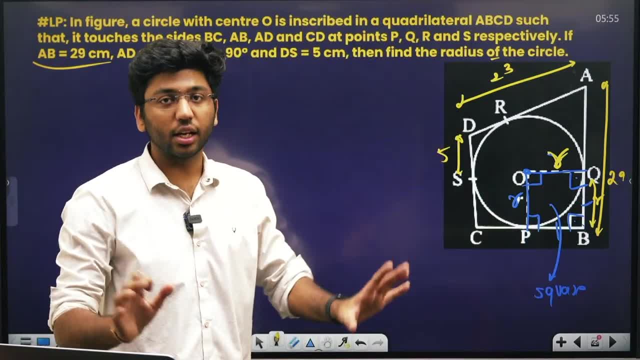 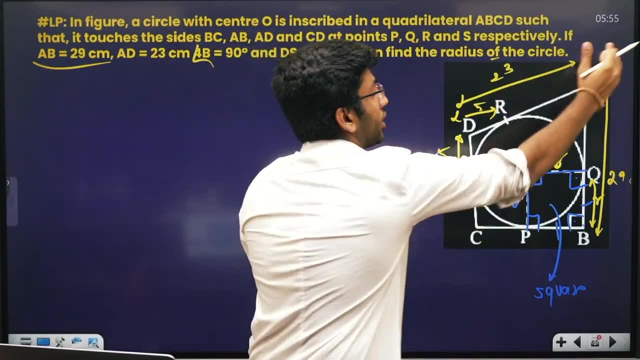 Ok, Now see, Now see, see, carefully, see carefully. From this point there are two tangents. So this is 5, so this is also 5, This is 5, this is 23, This is 5, this is 23. So what is this? 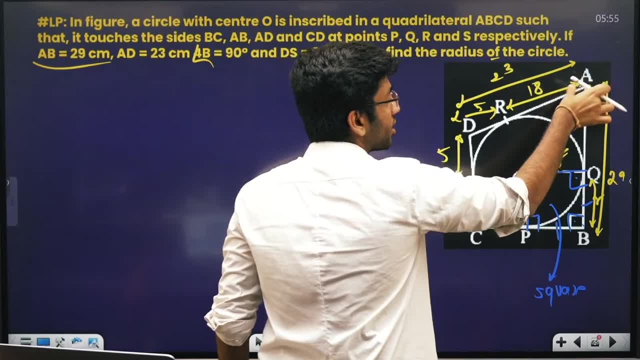 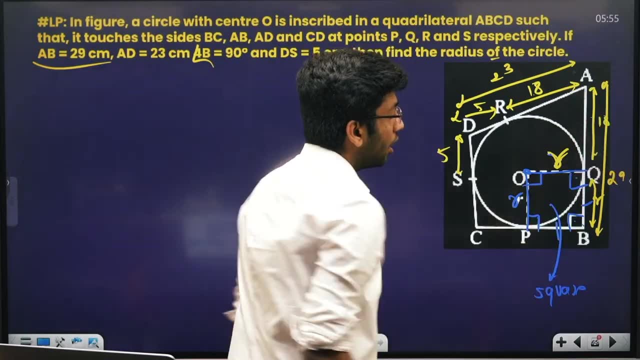 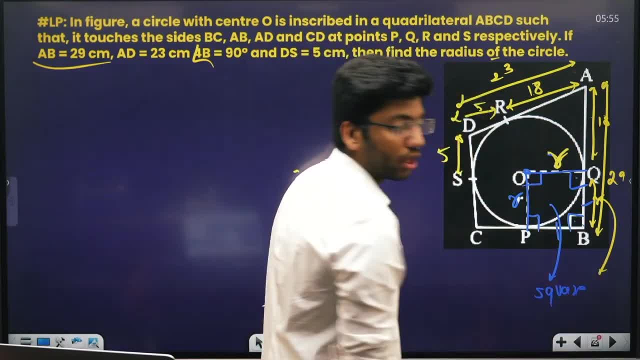 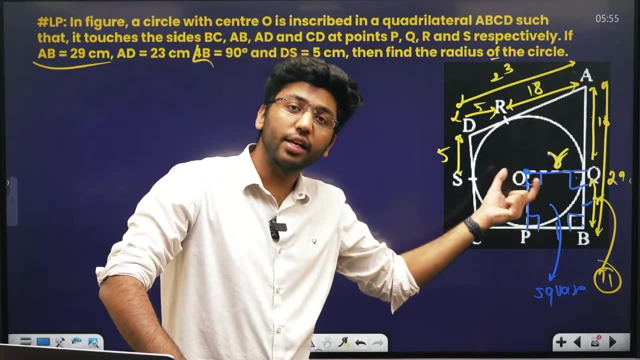 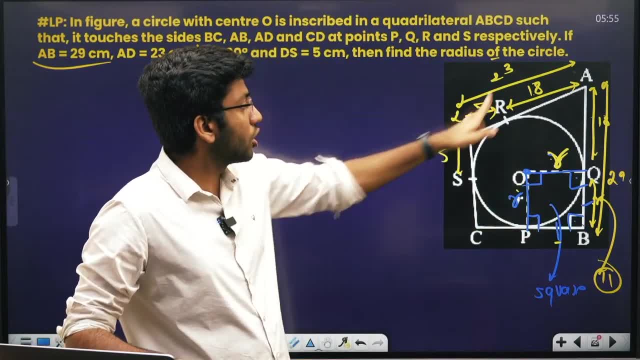 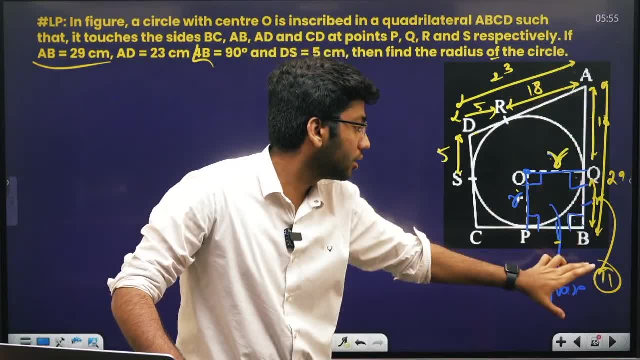 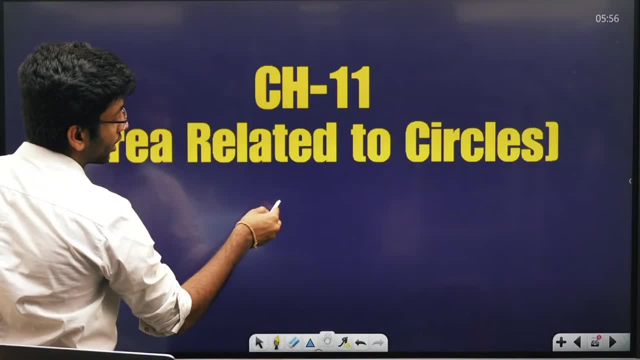 This is 23,. this is 18. So what is this? This is 11. We will do it like this. Ok, So here your circles are finished. Now comes area related to circles. Area related to circles. Area of sector. We have read this chapter today, So I will do it quickly. 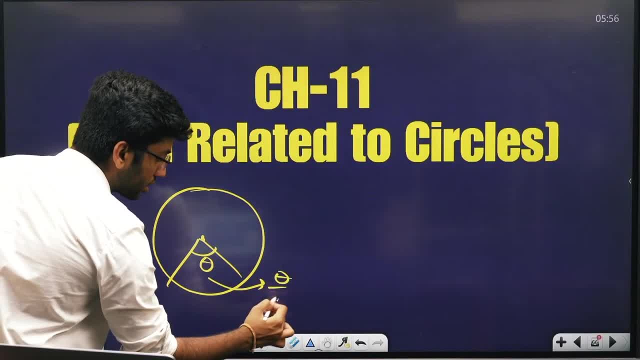 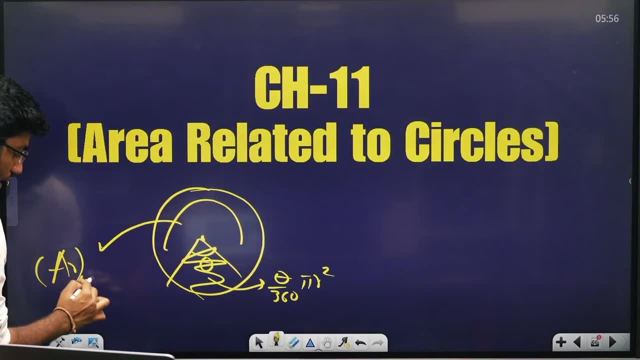 Area of sector. This is angle theta, So area of sector. theta, by 360 into Pi R square. This is area of sector. If major sector is to be taken out, So area of circle, Area of circle minus area of sector, Do it. This will be the area of sector. 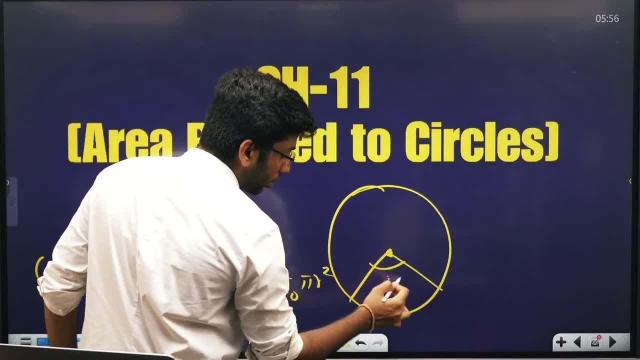 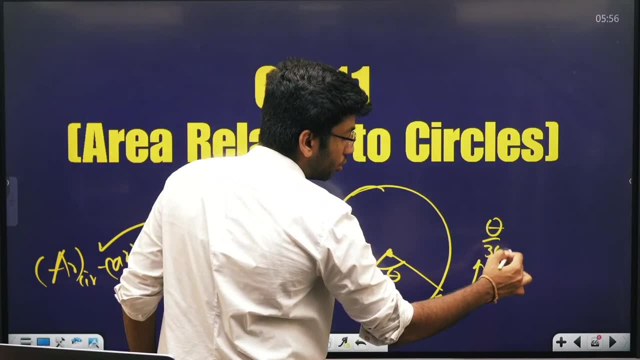 Then if I talk about the length of the arc, If I talk about the length of the arc, So angle is theta And this is length of arc L. So this is L arc. Length of arc is theta by 360 into 2 Pi R. This is the length of arc. 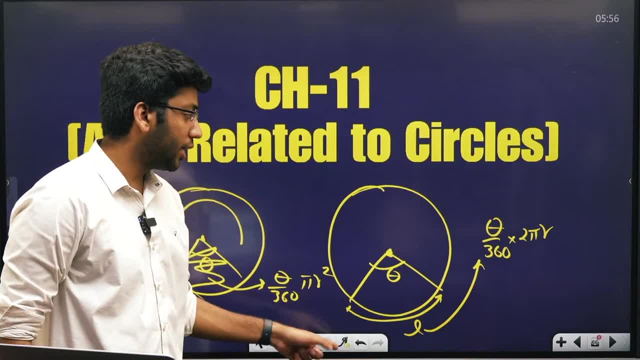 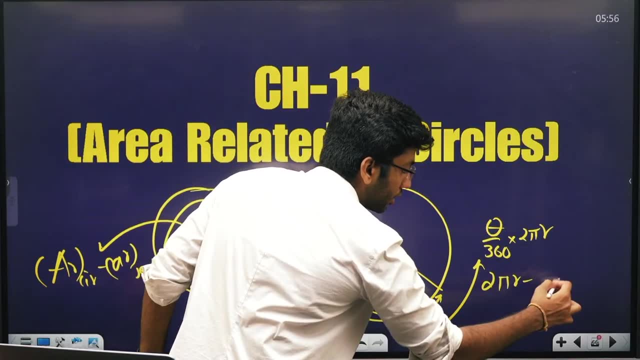 This is the length of arc. Ok, This is the length of the minor arc. So what will be the length of the major arc With the length of the whole circle Means from 2 Pi R theta by 360 into 2 Pi R Minus this. 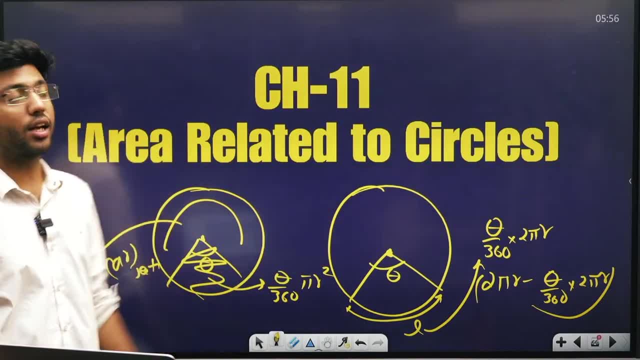 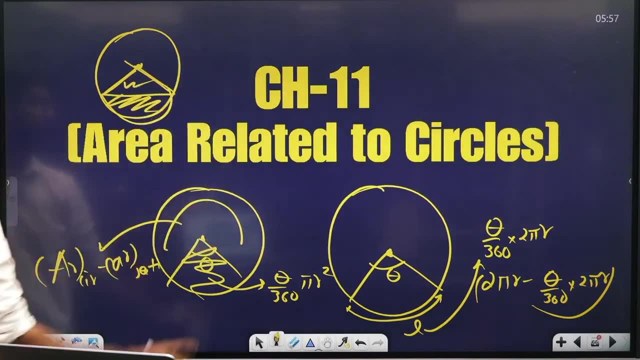 So this will be the length of the major arc. And how do we take out the segment? How do we take out the area of the segment? Means we need the area of segment. So remove the triangle area from the sector area. Remove the triangle area from the sector area. 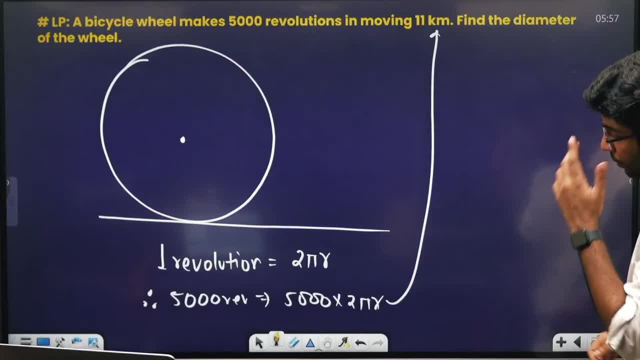 This is read today. That's why I am not revising it again and again. This is read today. That's why I am not revising it again and again. See, this is exactly the same Which we questioned today. This is exactly the same Which we questioned today. 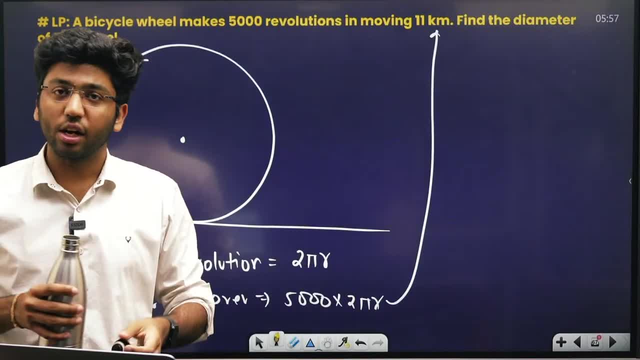 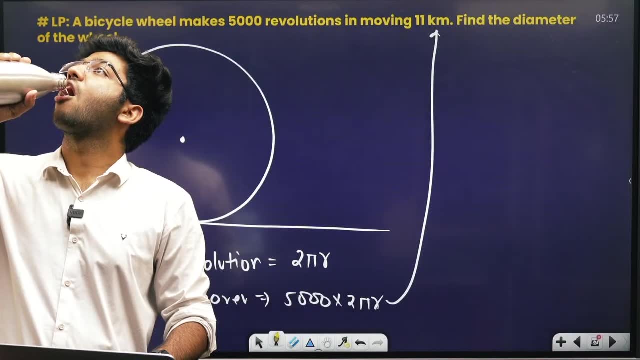 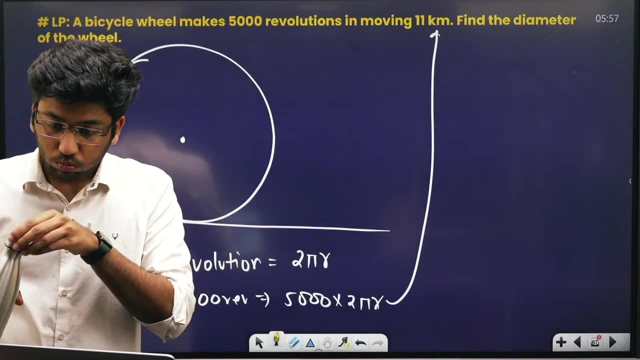 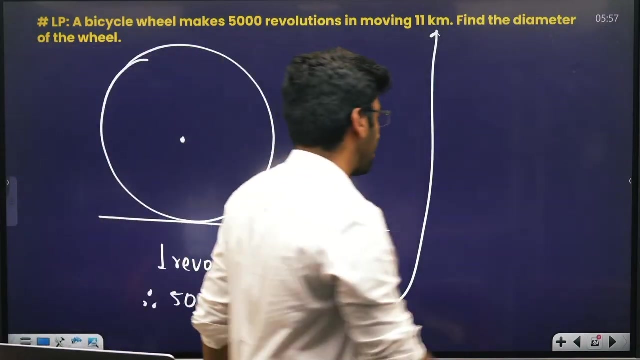 Just one second. Just one second. It will be over in 10 minutes. It will be over in 10 minutes Because these are the same things Which we have read today. All these questions, These are all questions. I will send these in the PDF If I give these to the exam center. 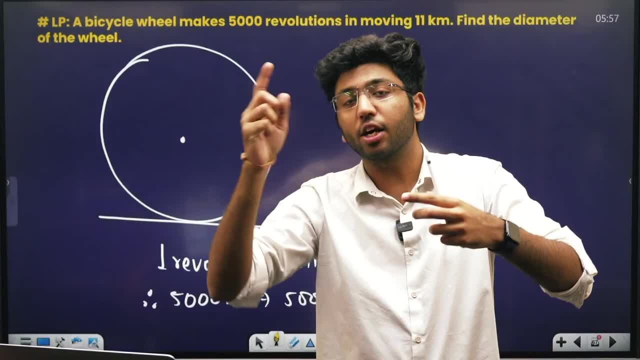 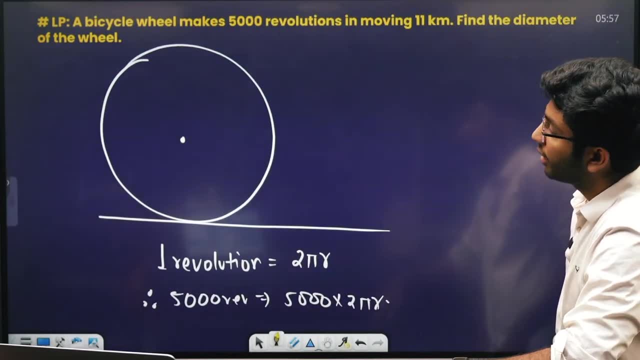 Go to the exam center. Once you go to the exam center, Take a PDF and go through the question. This is a bicycle wheel Which is doing 5000 revolutions In 11 km. Find the diameter of the wheel. See, See, this is a wheel. How long will it run in one revolution? 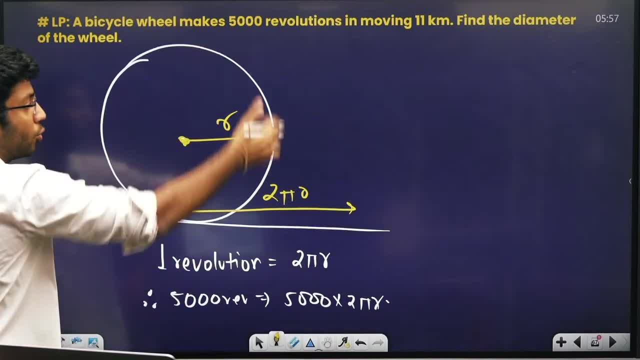 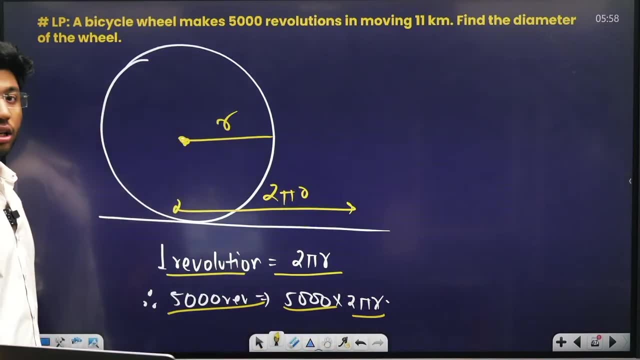 In one revolution 2 Pi R will run, Because its length is 2 Pi R. In one revolution 2 Pi R will run, See. so how much will it run in 5000 revolutions? 5000 x 2 pi r. so he said in 5000 revolutions. 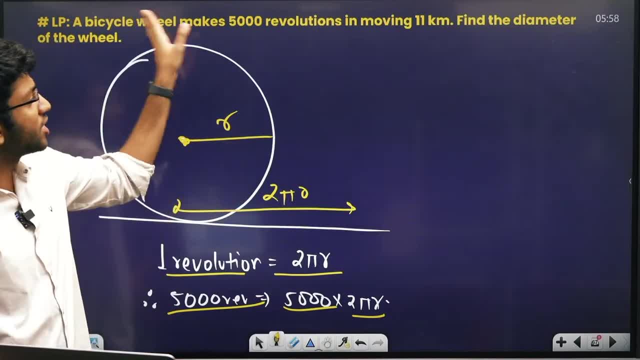 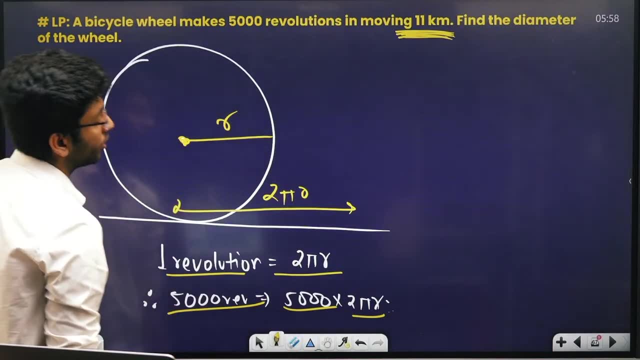 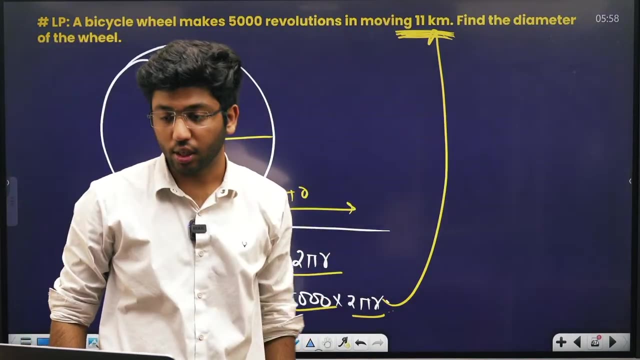 according to us, 5000 x 2 pi r will run and according to him, how much is running? in 5000 revolutions, 11 km. so this length, this length, this which we got in 5000 revolutions, make it equal to this, make it equal to this and the answer will come. 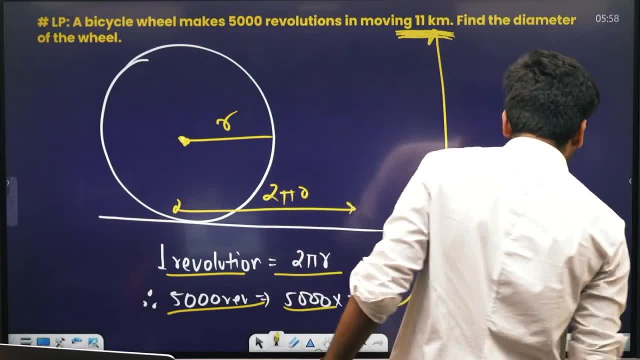 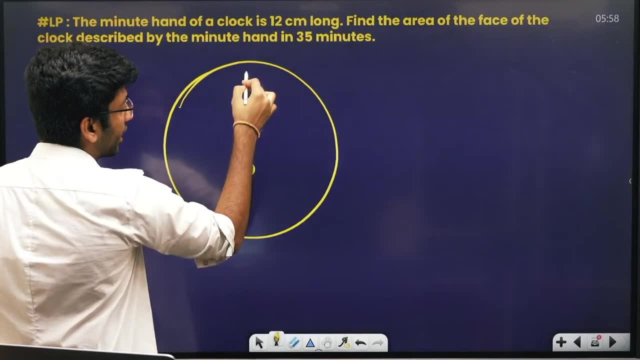 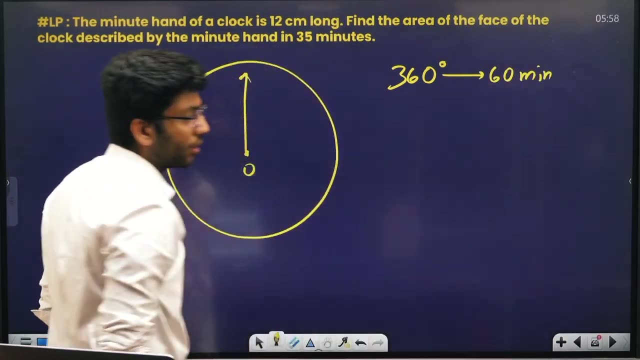 make it equal to this and the answer will come ok. so I am making it fast. minute hand of the clock. we did question today what is minute hand. minute hand means how much it rotates in 360 degree in 60 minutes. in 60 minutes it rotates 360 degree. 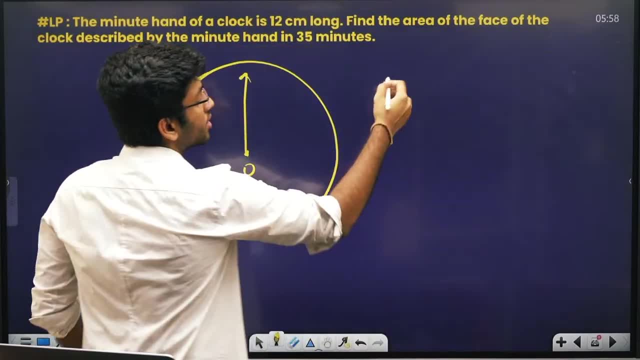 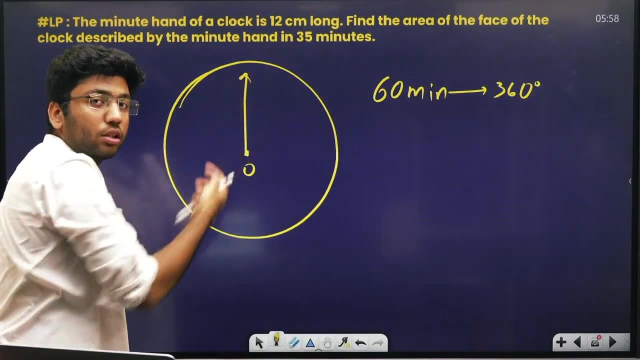 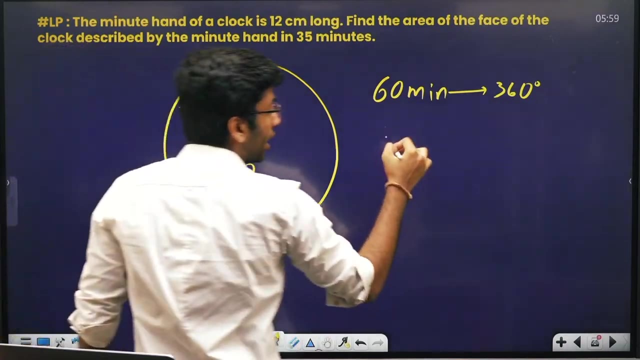 or I can say that in 60 minutes, how much it rotates? it rotates 360 degree. so this minute hand, it rotates 60 degree in 60 minutes. in 60 minutes it rotates 360 degree. so how much it rotates in 1 minute. 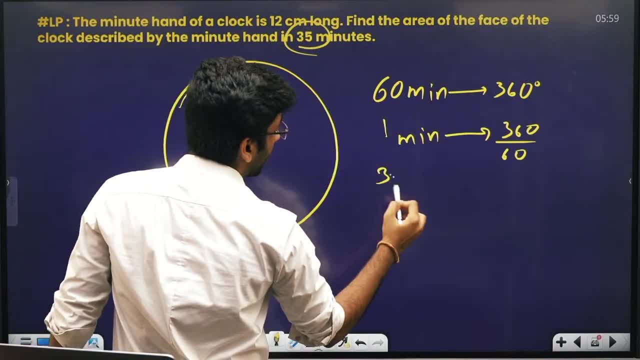 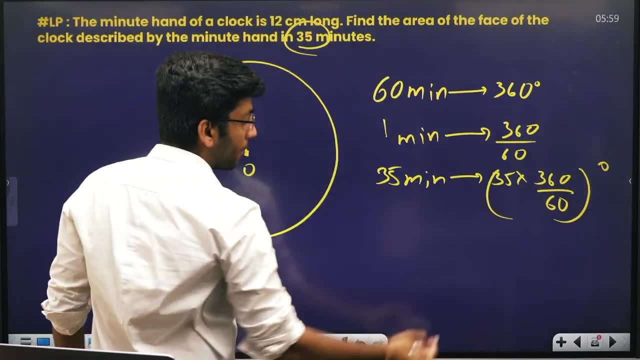 it rotates 360 by 60. so how much it rotates in 35 minutes, how much it rotates in 35 minutes: 35 into 360 by 60, this much degree, this much degree it rotates. this is theta. it goes from here to 35. 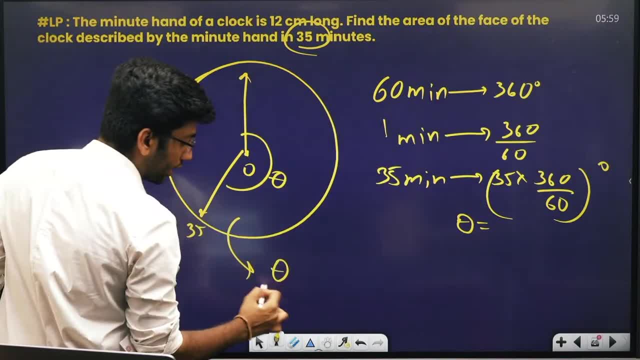 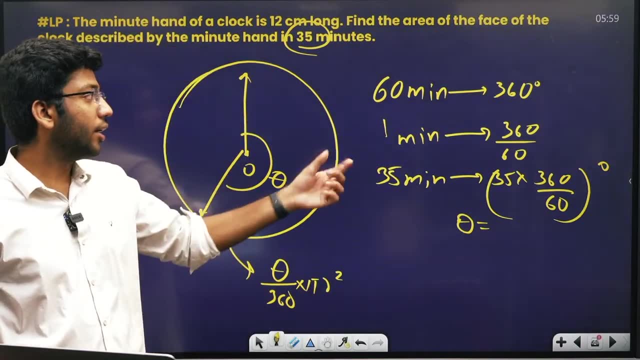 so we got this angle theta. now we have to find the area. so what will be the area? theta by 360 into pi r square. so we have to understand minute hand: 360 degree in 60 minutes, 360 upon 60 in 1 minute. 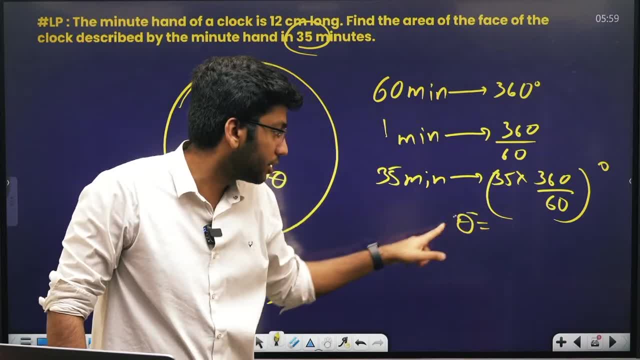 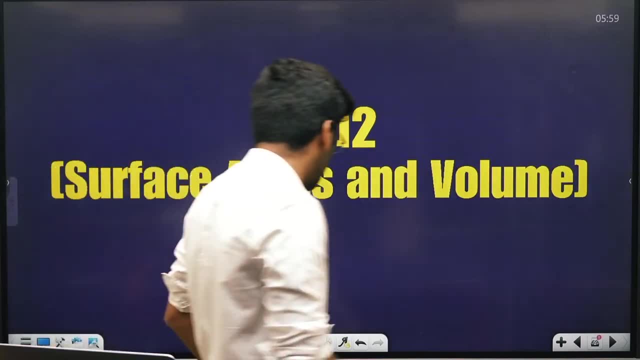 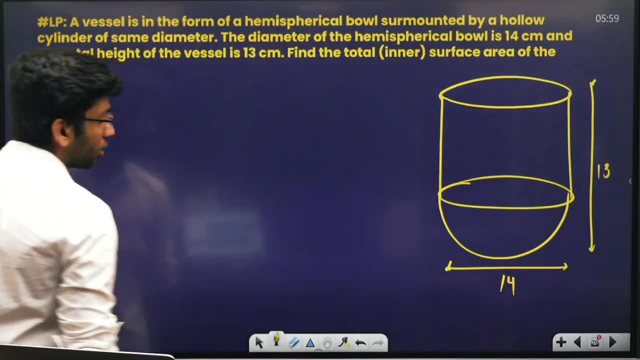 so how much? it rotates in 35 minutes theta angle 35 into 360 by 60 you will get theta angle ok. surface area volume: we have read many formulas ok from that. one important question: I am telling you: there is a vessel like this: 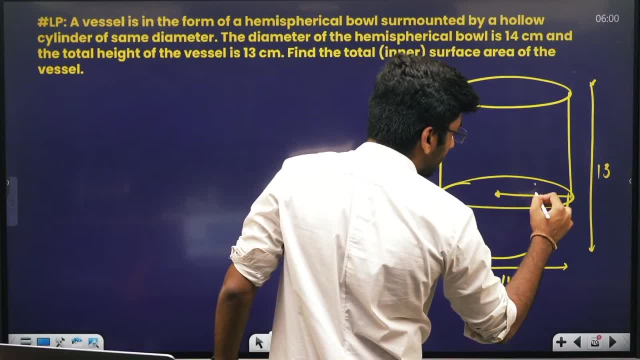 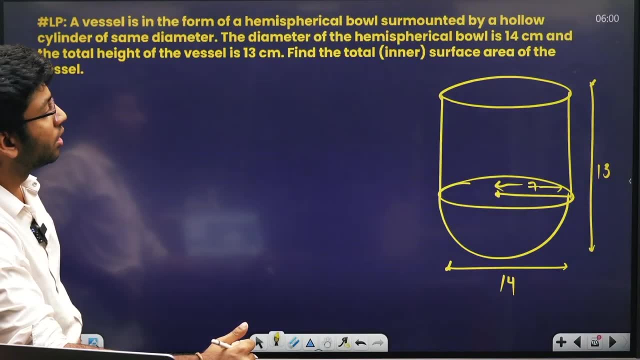 its diameter is 14. diameter: 14 means this radius is 7. diameter: 14 means this radius is 7. diameter: 14 means this radius is 7. the diameter of the hemispherical bowl is 14 and the total height of the vessel is 13. 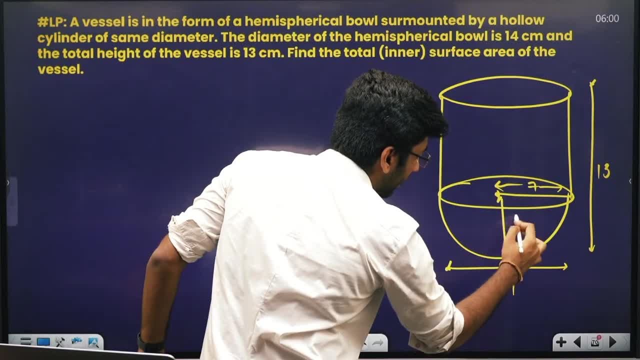 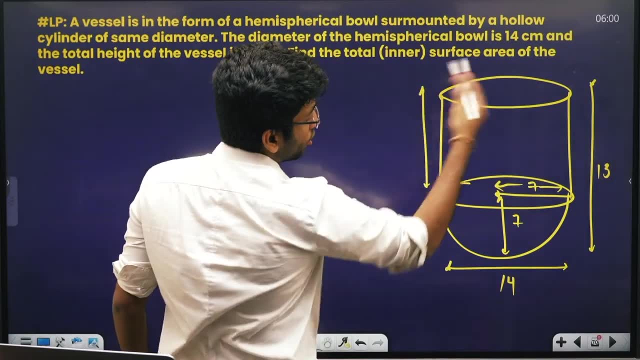 total height is 13. so if this is 7, radius is 7 and total is 13. this is 7 and total is 13. so how much height will be this? this cylinder's height is 13 minus 7. 13 out of 7 is 5. 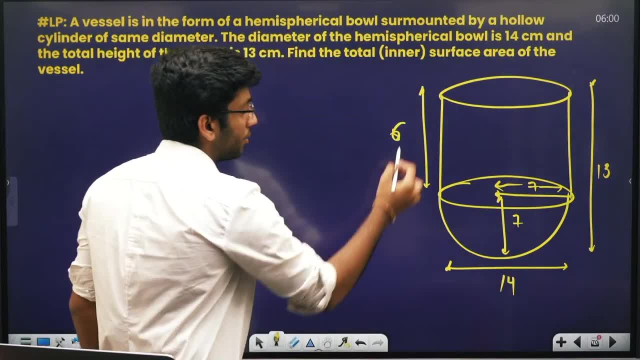 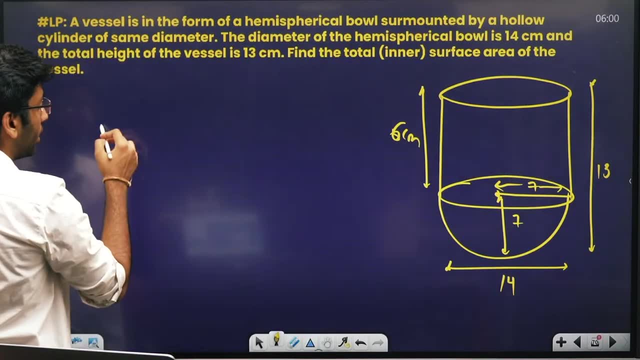 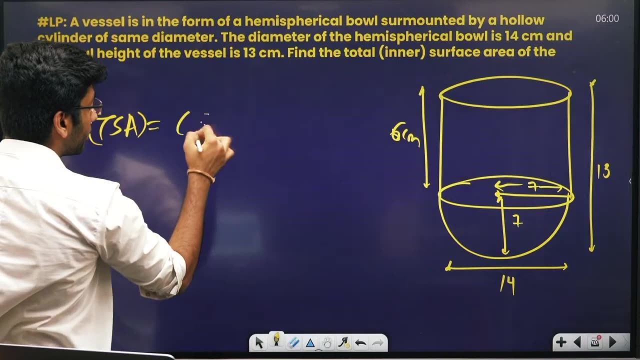 so 6, 6 poems. which is? this would be the height of a cylinder. we have been asked total surface area. what can I touch? total surface area: where can I touch? I can touch its curved surface area of cylinder. cylinder curved surface area. the surface area is: 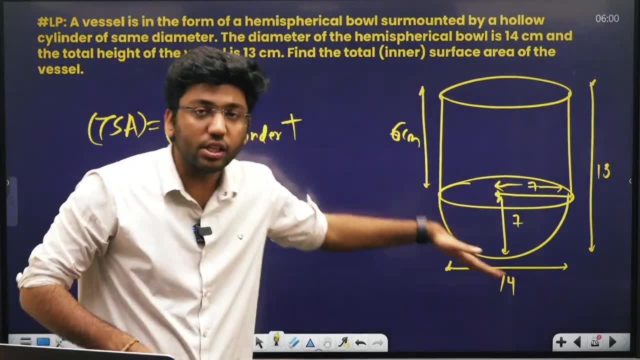 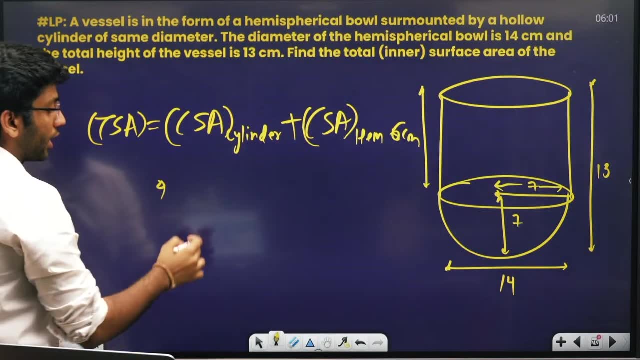 its surface area core also its surface area core 6. I can also choose the curved surface area of the hemisphere. So what is the CSA of cylinder? Curved surface area is 2πrh Plus. what is the curved surface area of the hemisphere? 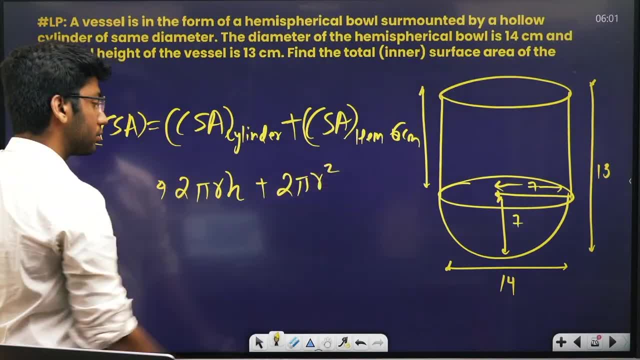 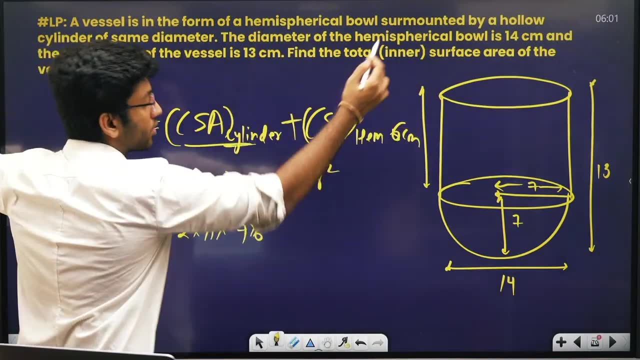 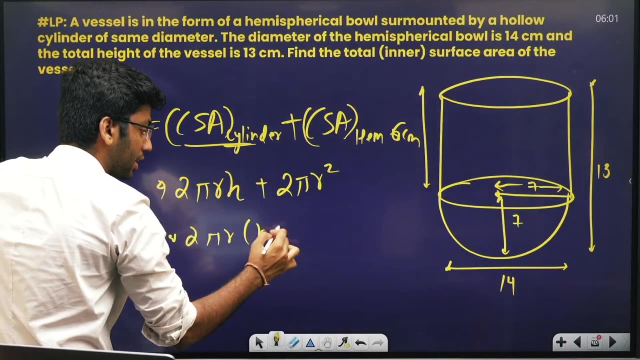 The curved surface area of the hemisphere is 2πr², So the value of 2 × π × r is 7 × h. Height of cylinder is 6 Plus 2πr. Take 2πr common first, So h plus r is left inside. 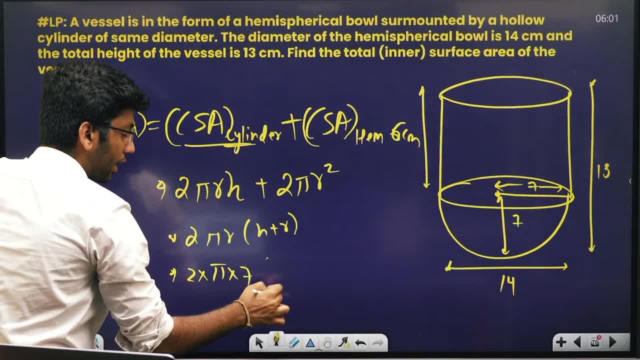 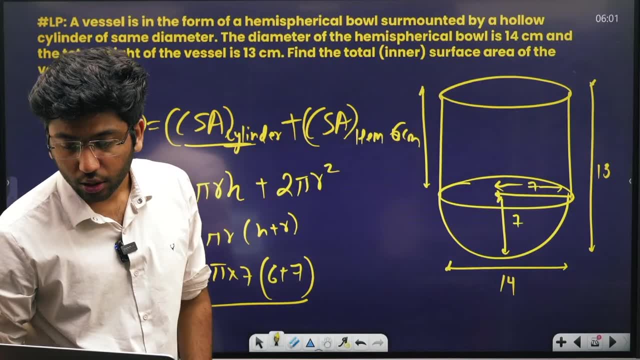 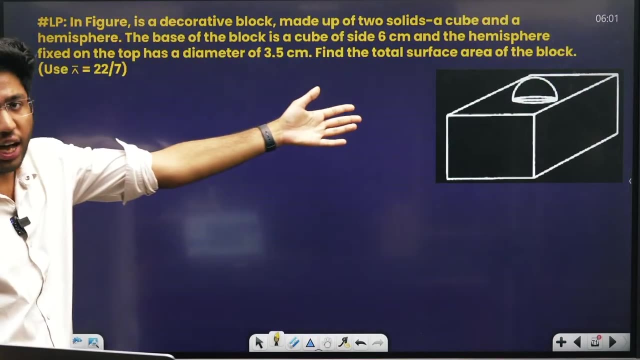 So 2 × π means π, r means 7, h means 6 plus 7. This is our answer. This is our answer, Okay, Okay, Okay. Next, In figure, it is a block like this. Today we did this question. We were asked to tell the total surface area. 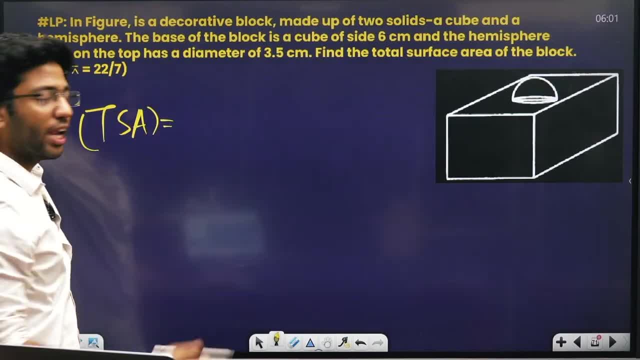 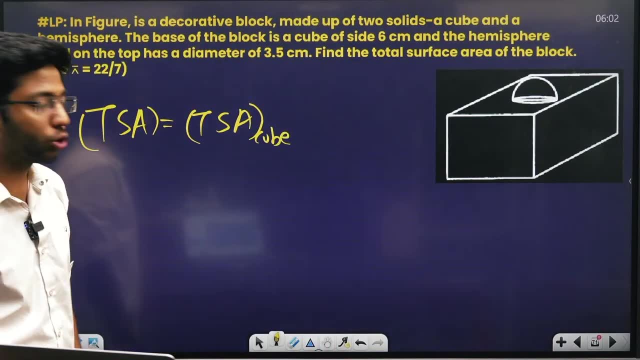 So see the total surface area Where I can touch. So first, if I assume the total surface area of cube, Take it. So what did I do? I took the total surface area of cube. So in the total surface area of cube, Where can I touch? 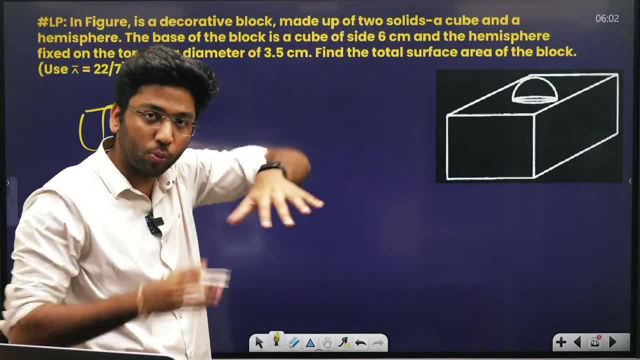 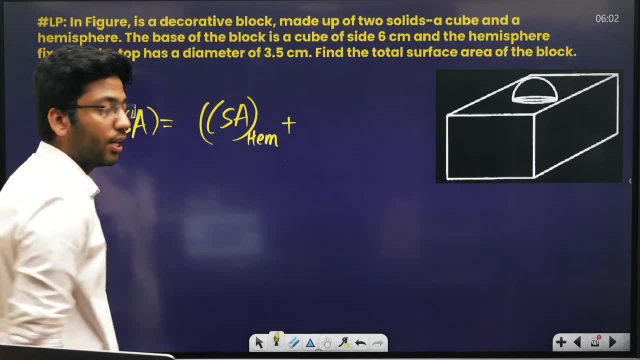 Tell me First, I can touch this hemisphere bowl from top to bottom. So I can touch the bowl from top to bottom. So I can touch the curved surface area of hemisphere Plus If I take the total surface area of cube. So did I make any mistake? 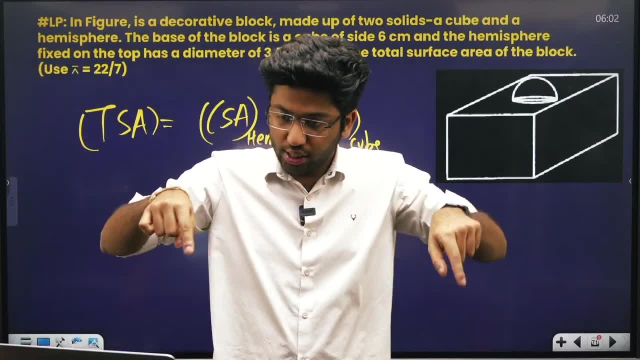 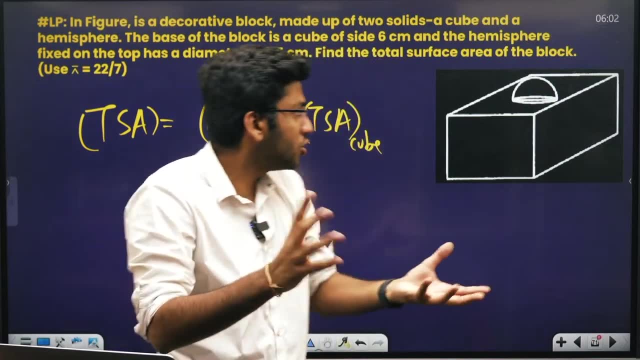 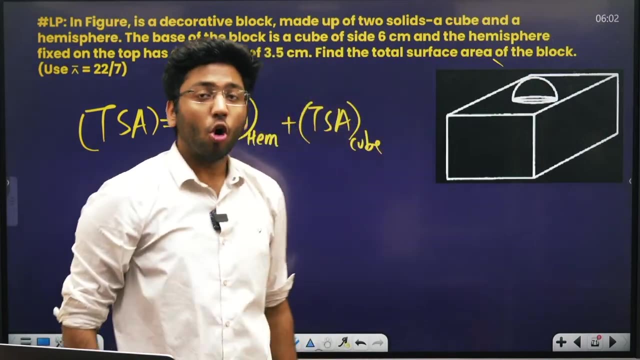 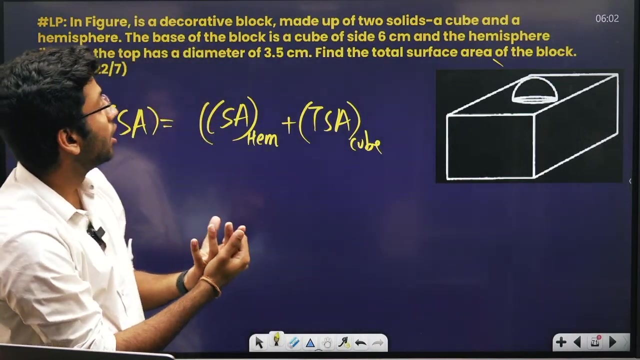 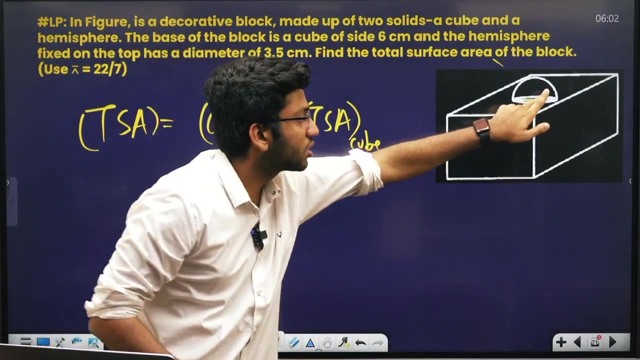 I made a mistake. See, This was a cube like this. This was a cube. This was a cube. I stuck a hemisphere on it, So the base of the hemisphere. I will not hide it. I will not hide its base. It was stuck inside. So I took one. 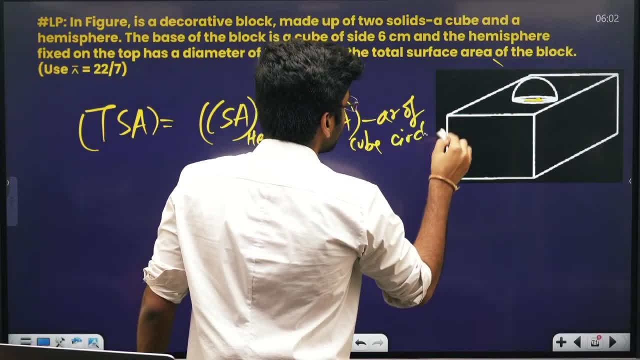 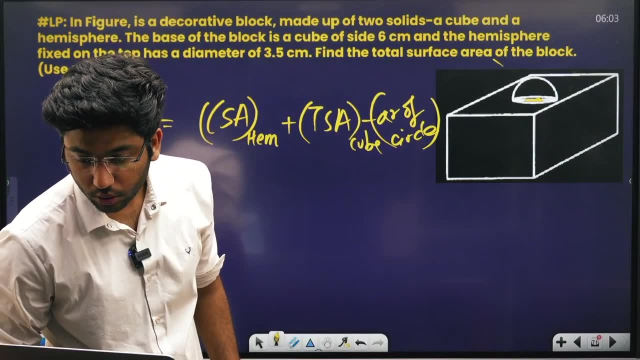 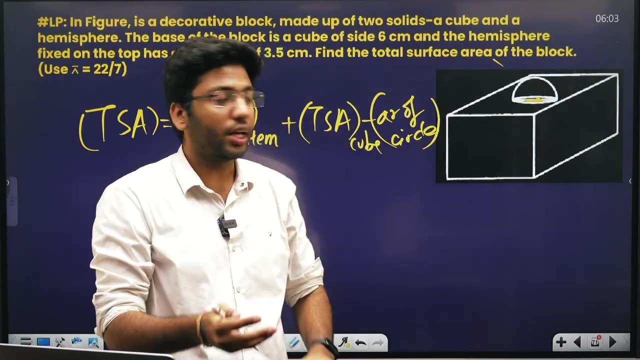 So I will subtract area of circle. I will subtract bed circle area. I will minus the area of circle. Ok, I will minus the area of circle, Ok. So what did I do? Where I can touch, What could I touch? I can touch the curved surface area. 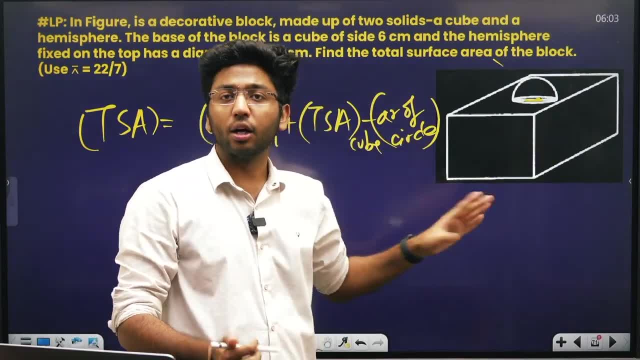 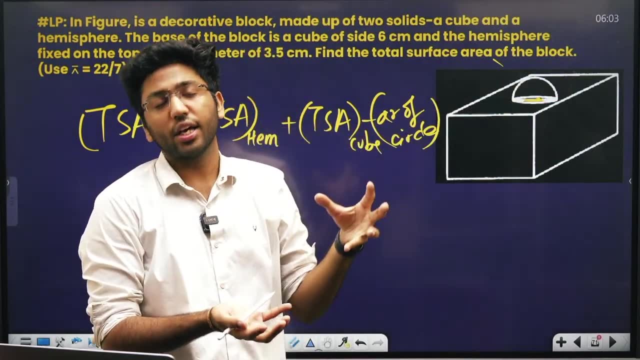 And If I took the total surface area of the cube, I can touch everywhere of the cube, But I can't touch the top of the cube Because it is hidden from the hemisphere. It is hidden from the hemisphere. So I have minused the area of circle From the total surface area of the cube. 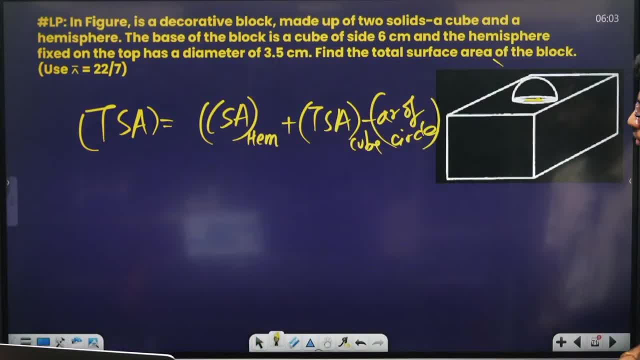 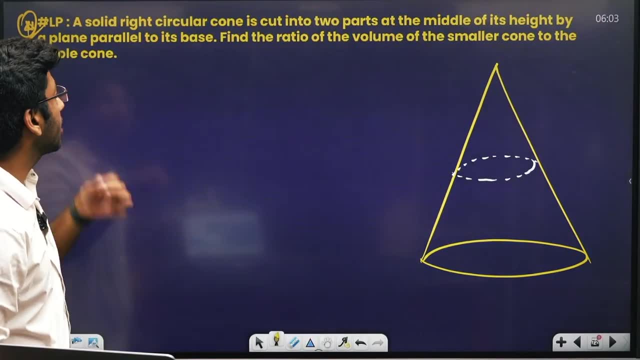 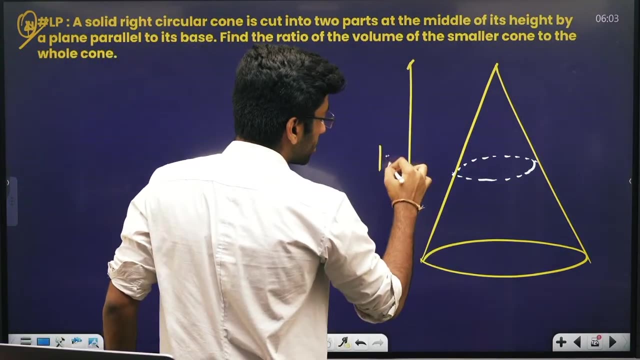 Ok, Next question. This type of question can be asked by CBS. This type of question can be asked by CBS. It is said that there is a solid right circular cone. It is cut into two parts in the middle by its height. Ok, If its height was h. If its height was h. 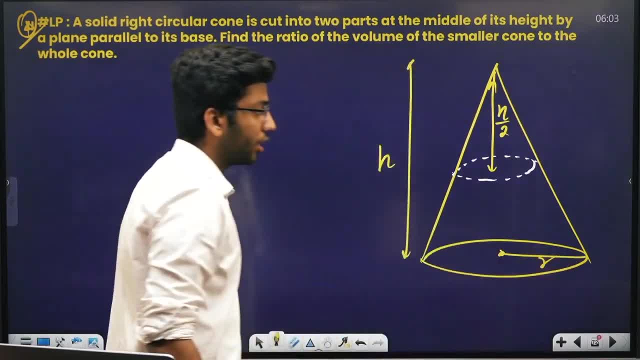 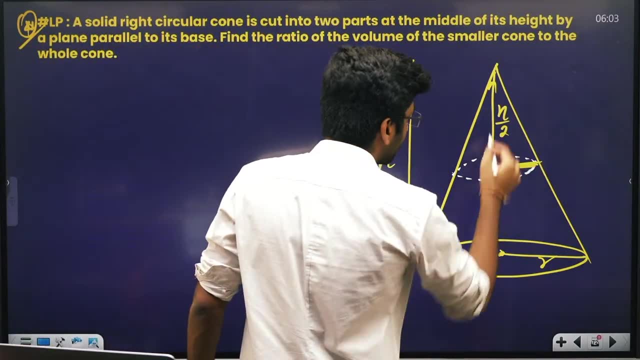 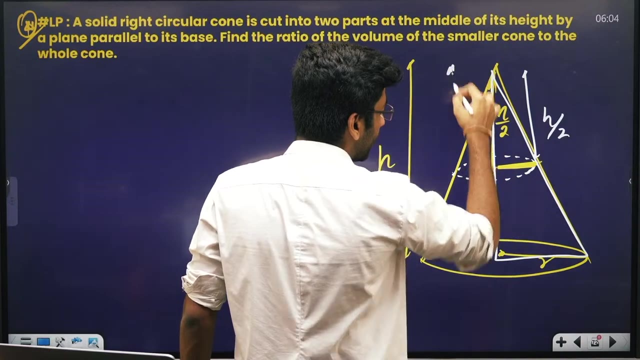 Then there is a small cone whose height is h by 2. Its radius is r. Its radius is r. First tell me How will we find its radius? Look carefully In this triangle. This is the height h by 2 And this is the complete height h. 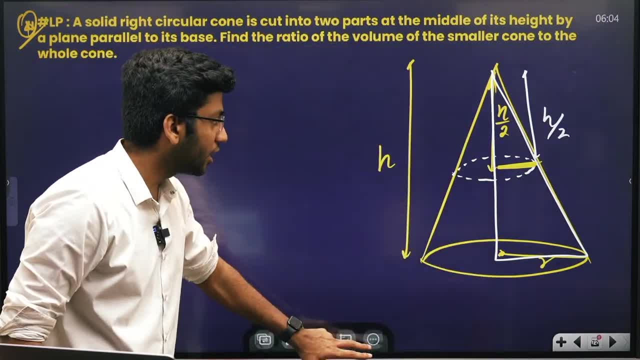 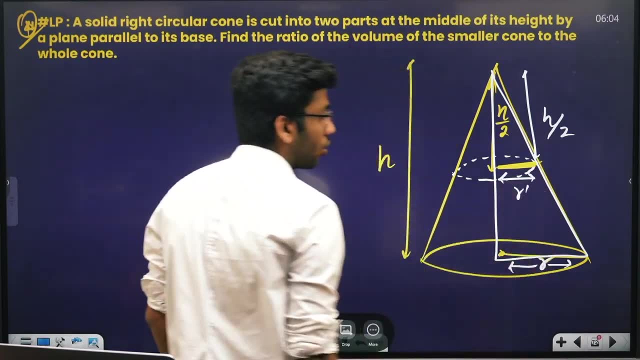 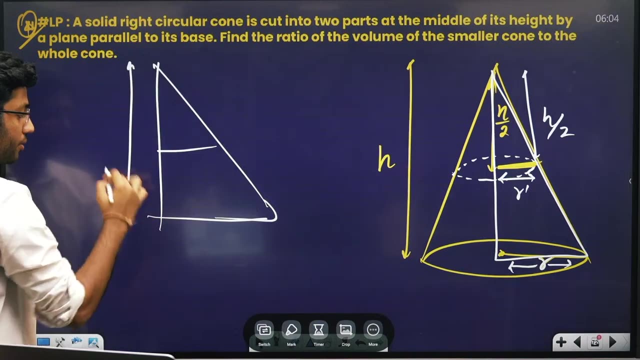 This is the complete height, h. So can I put a similarity? If this radius is r, If this radius is r, Then what will be this radius, What will be this r dash? So look in this triangle, Look in this triangle, Look carefully. And this is h by 2. 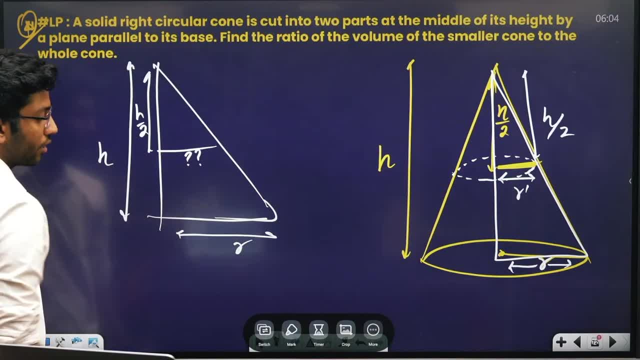 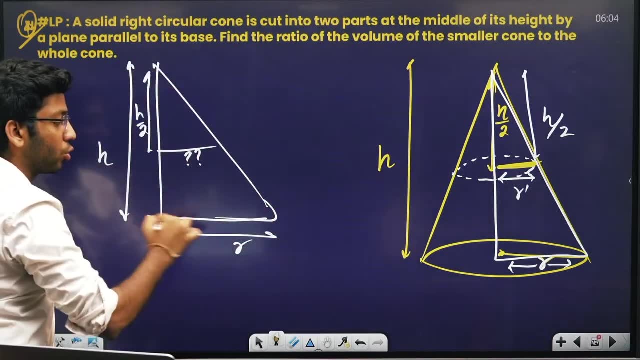 So this is r. So what will be this? Ask us this: If I put a similarity in these two triangles, In which, In the big one and in the small one, In the big one and in the small one, I have to find r dash. So if I put a similarity in the big one and in the small one, 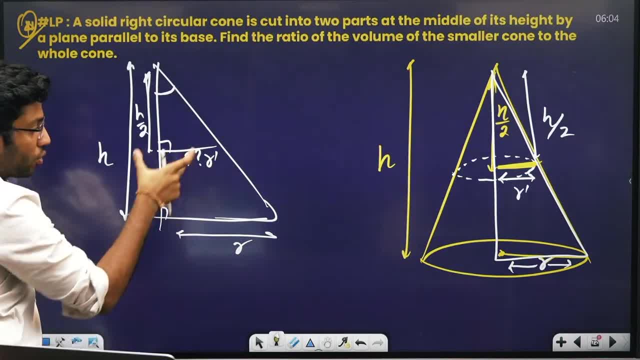 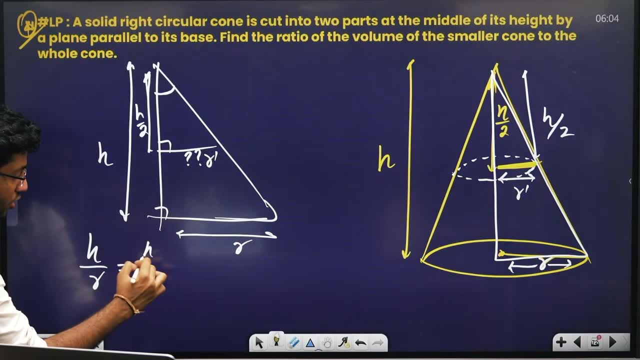 Then both will be similar. Because this angle is this angle and this is 90. I have to find r dash. So after similarity I will put CPST in this. So h by r will be equal to h by 2 Upon r dash. So from here I will know the value of r dash. 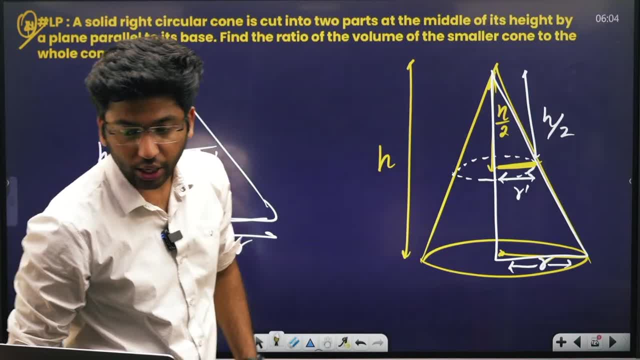 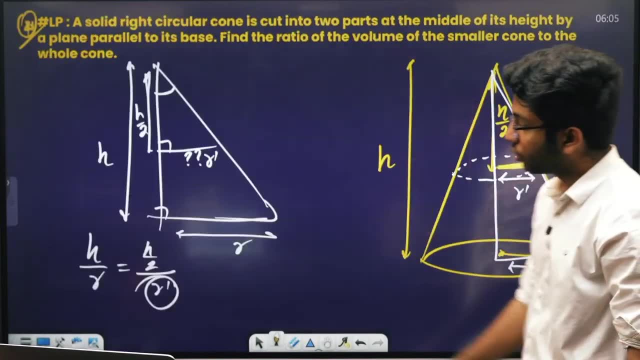 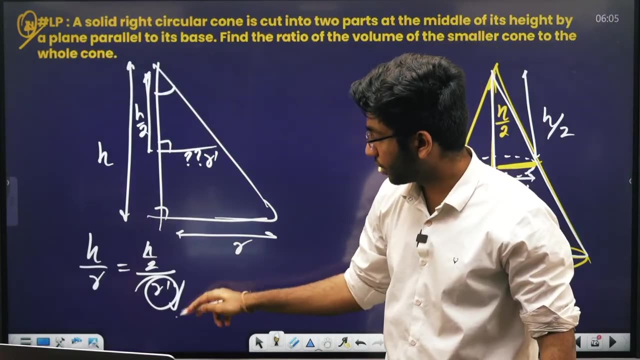 From here I will know the value of r dash. It is not coming, It is deleted. It is deleted. But if you want to find, Then find r dash. in this way, You will do similarity, You will do similarity of this and this, So you will know the value of r dash. 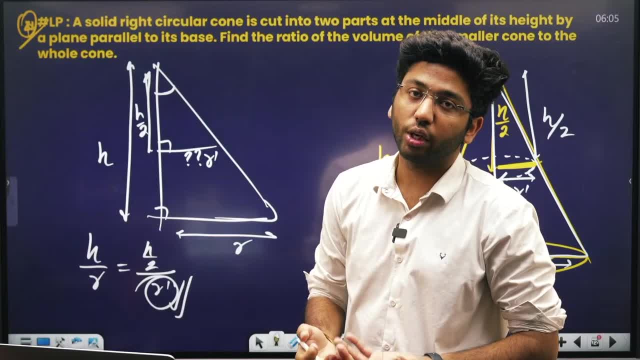 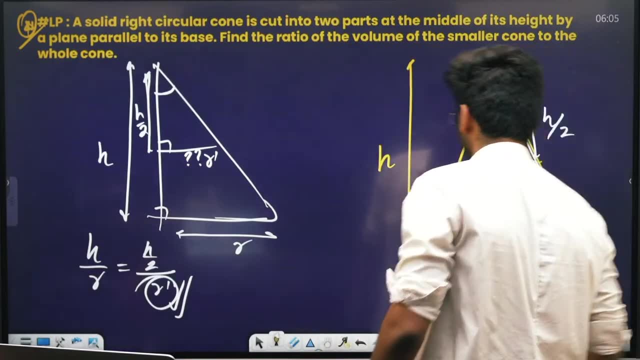 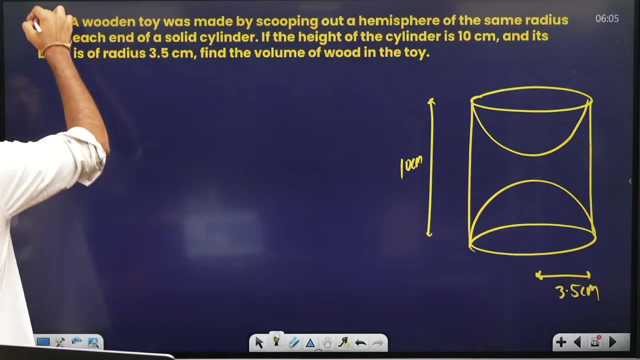 If you know the value of r dash, Then just find the volume of cone of both. So find the volume of the upper cone And the volume of the lower cone. Ok, Next question: There is a wooden toy Which is scooping the hemisphere. This is a very important question. 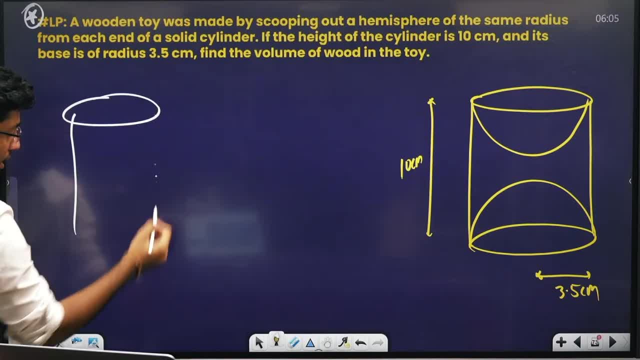 There are many questions related to scoop Like this is hemisphere. We have done it today. From this we will scoop the cone, From this we will scoop the cone. So even if we scoop the cone, Then we can do the question. So they scooped the hemisphere from the wooden toy. 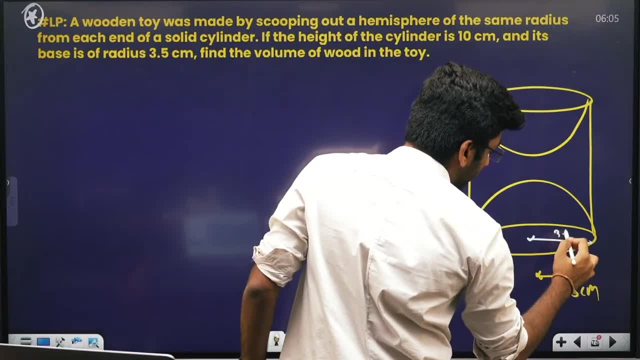 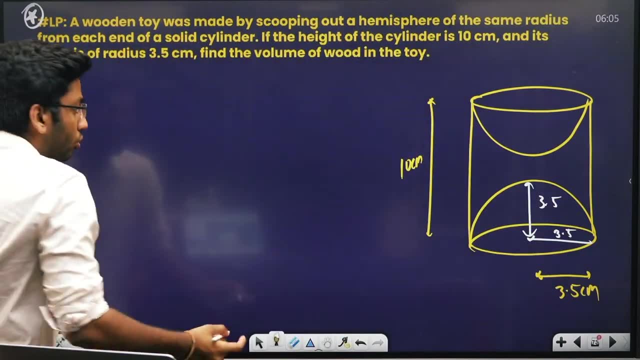 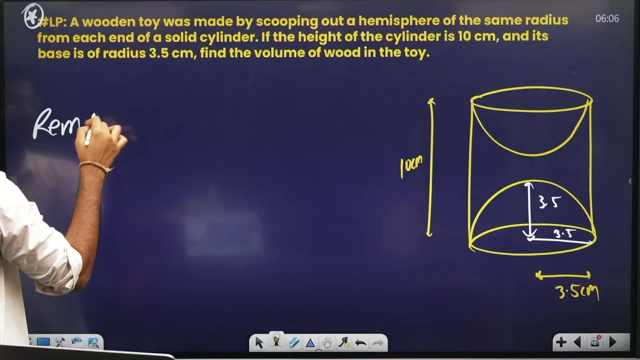 Same radius. Height of cylinder was 10, So its radius will be 3.5. So I have to tell you How much remaining wood is there. So what will be the volume? So the volume of this combination, The remaining volume, We have to tell the remaining volume. 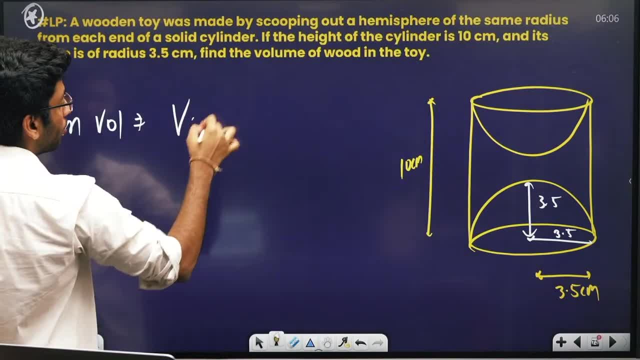 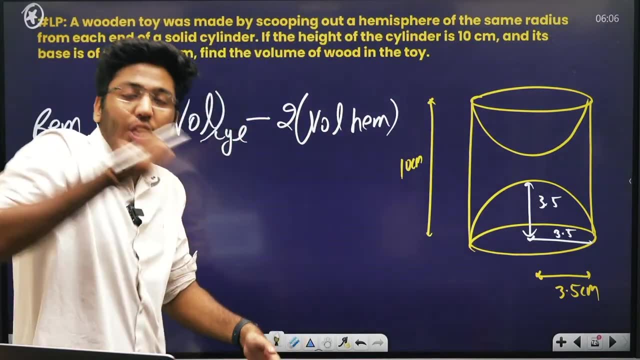 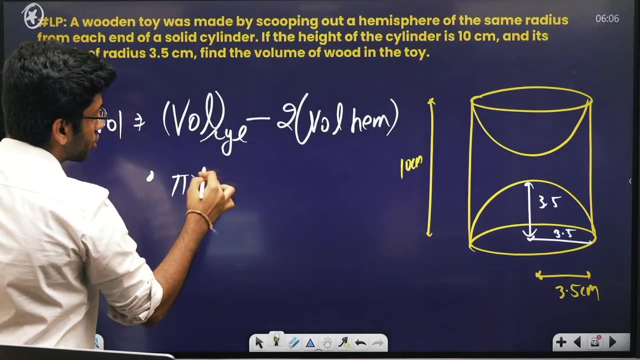 So what will be the remaining volume? So the volume of cylinder Minus 2 times Volume of hemisphere, Because I scooped 2 hemispheres Like we scoop ice cream. So I scooped 2 hemispheres. So, volume of cylinder, What will be Pi r square h? 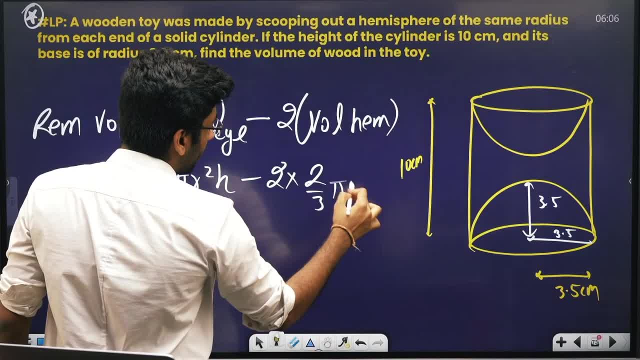 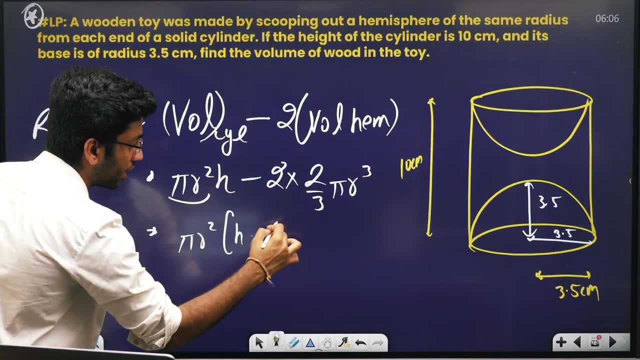 Minus 2 times volume of hemisphere. Volume of hemispheres is 2 by 3 Pi r cube. I scooped this From this. I am looking how to solve Pi r square common. Pi r square is not common. H minus 4 by 3 r. 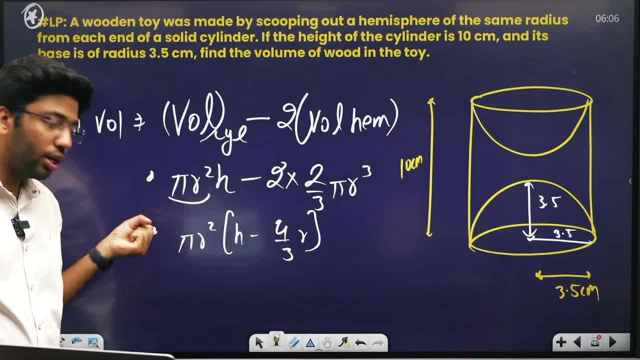 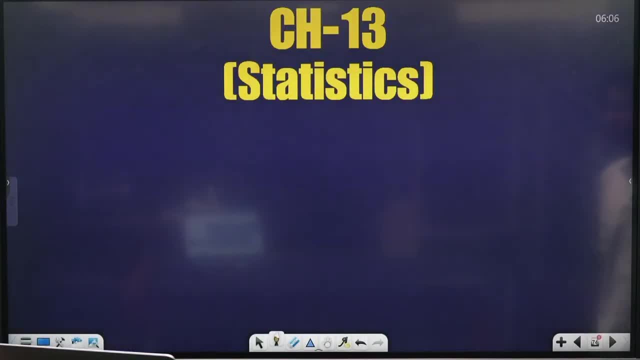 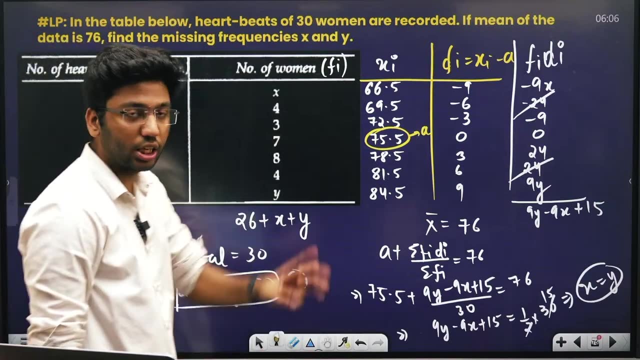 Now put the value. Don't put the value directly. Don't put the value directly. First take common, Then put the value In the statistics. This is the important question Today. we did not question this domestic. Today I am telling I have three methods. We study assumed direct method. 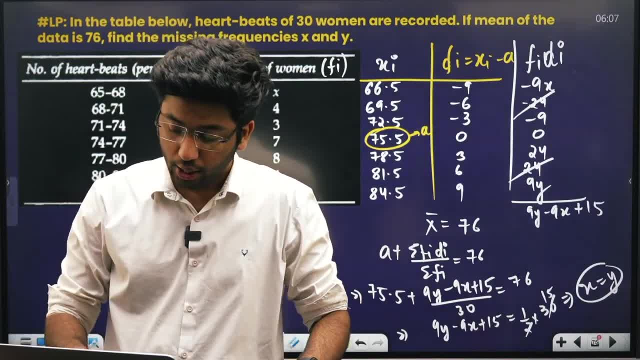 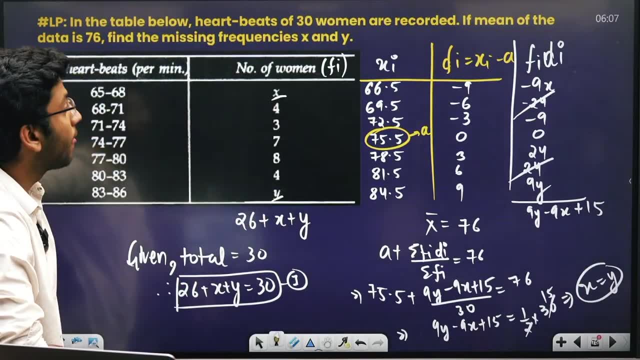 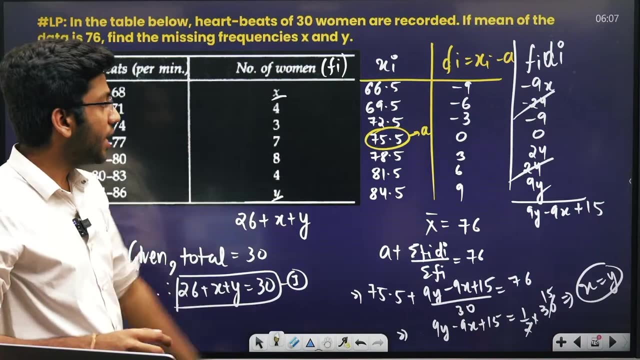 Assumed mean method And step deviation method, See tomorrow. I'm telling you The values of x and y, Of x and y We are given mean. The hypothesis was, But they were very big in xi. So how will I do summation of fi xi? It will be very big. 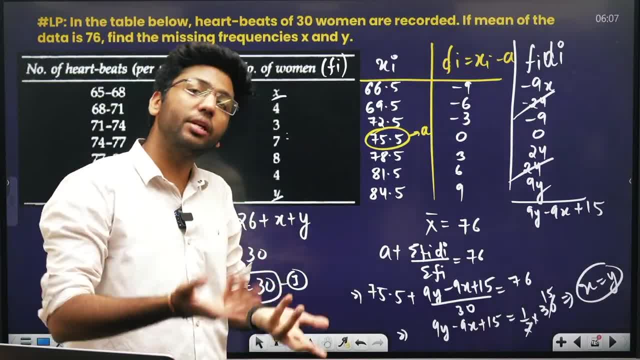 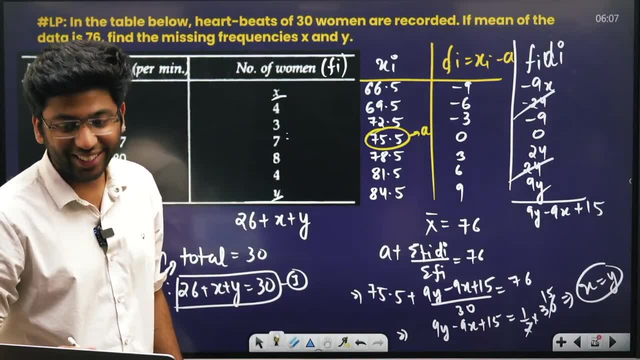 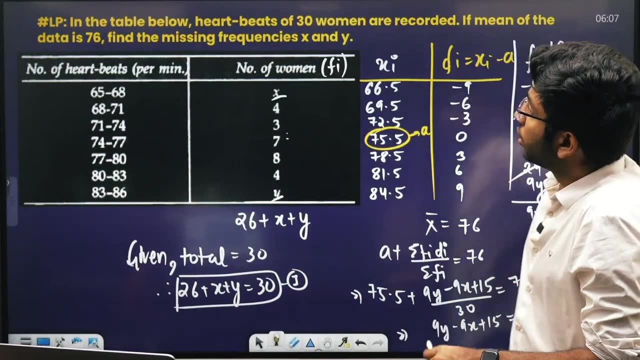 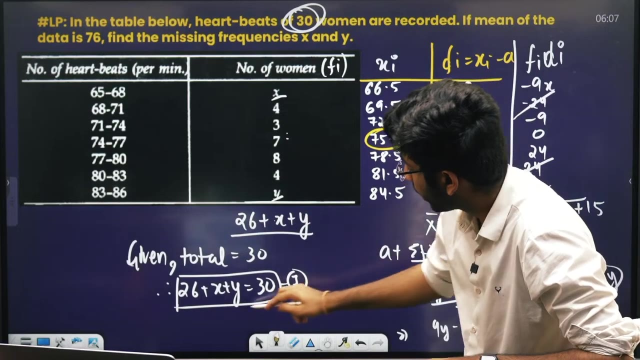 So I said Let's do it with assumed mean. Listen carefully, It is very important. One is writing: Ok, son, Step deviation is not deleted. See: Total is 30. women: Total is 30. What will be the sum of all this? It will be 30. So 26 plus x plus y is 30. 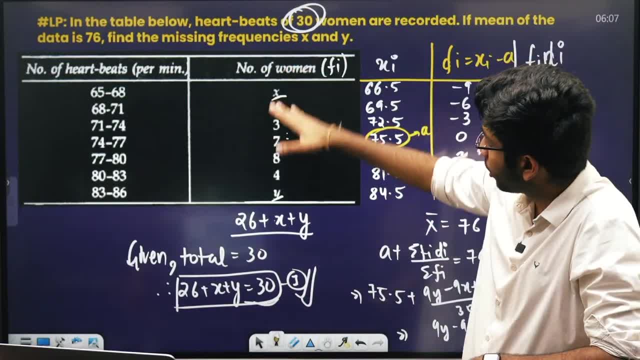 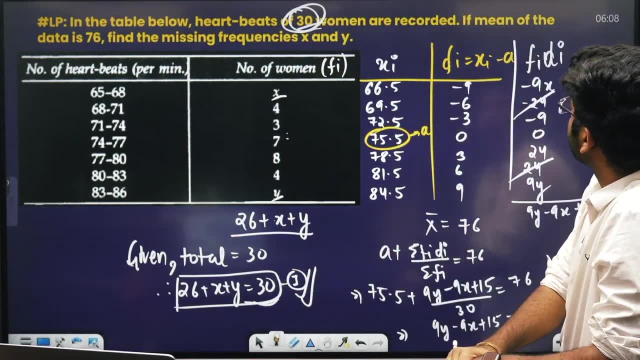 This is the first equation. This is the first equation. What is the number of women? Total number of women is 30, So the sum of all this will be 30. First equation. Second, The mean of this is told to us If mean is 76. So what did I do to get the mean? 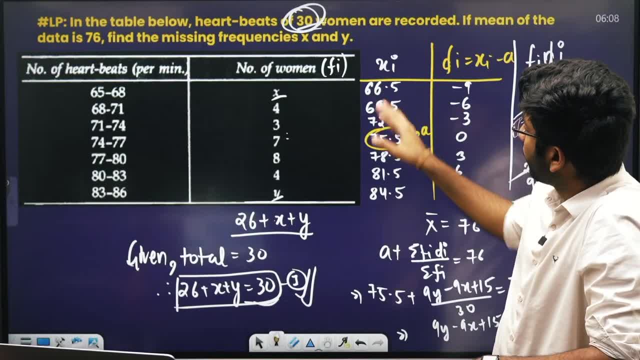 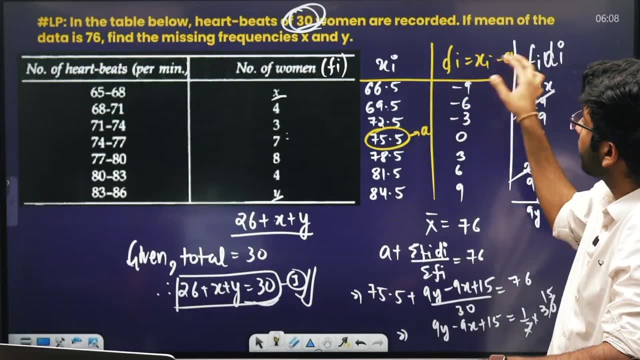 I knew fi, I took xi, But xi was increasing so much. So if I did fi xi, If I did it with direct method, Then it would have been very big. So what did I do? Assumed mean Means: I took di, Di means xi minus a, A means middle term. 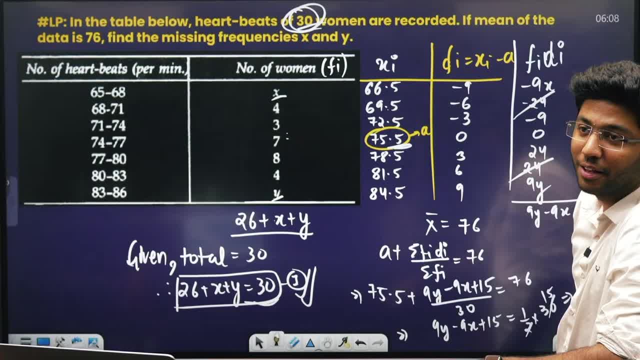 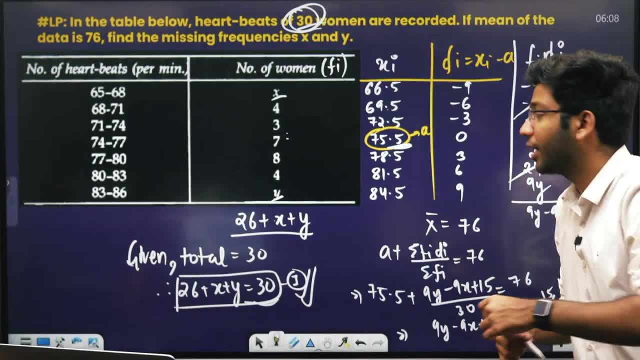 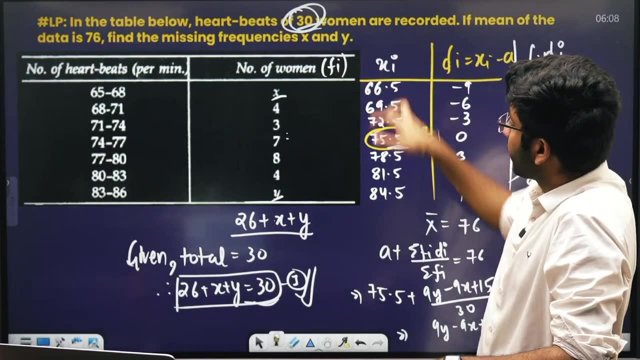 So xi minus a Minus a. I don't even know about this. Alexa heard something. She let Alexa hear. Alexa, I will close it for a second Sister. Wait, sister, Let me study first. So I knew fi, I took xi. I said I will do fi xi. It will be very big. 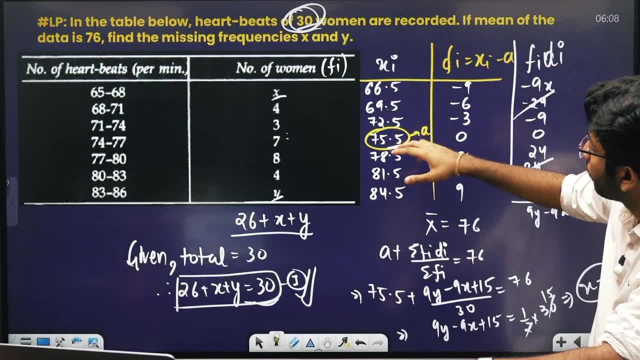 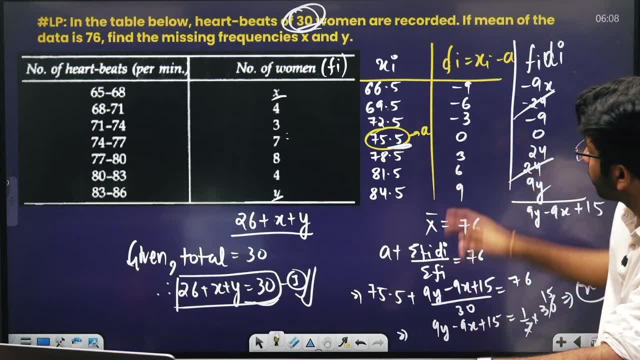 So let's take di: Di means xi minus a, So from xi Minus the middle term, So 66.5 minus this. 9 came From 69.5. Minus this: This came From 72.5 Minus 75.5, So di came. 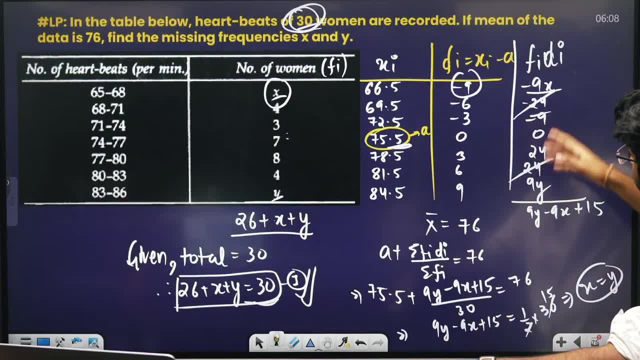 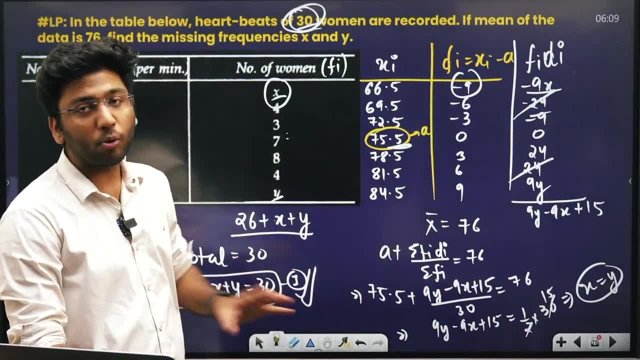 Now I did fi into di, So these came small And all these were seen cutting. So now I have, Now I have done this With assumed mean method. So, whenever you, Whenever you, Whenever you See xi very big, Xi will look very big, Xi will look very big. So do it with di. 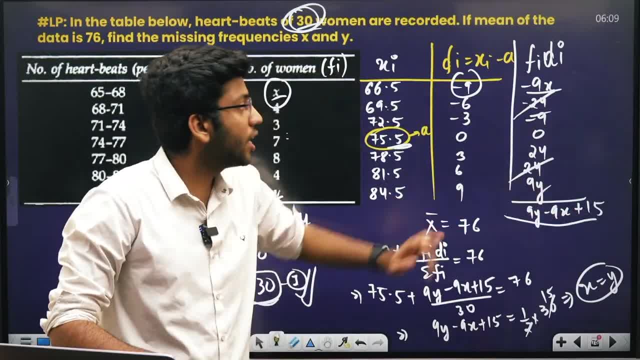 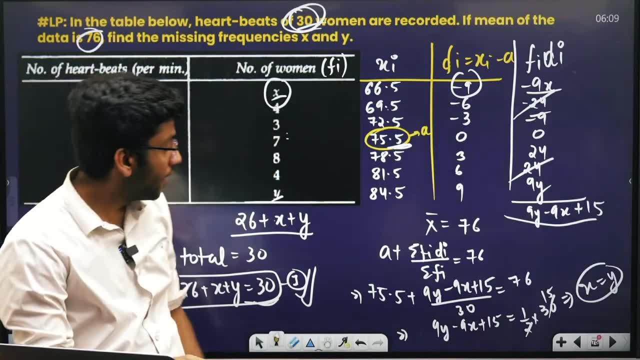 So now look at you How easy it is. in your calculation, Fi di came Ok, So a plus fi di upon Fi equal to 76, Because 76 means given, 76 means given, So a plus fi di upon Fi equal to 76. What is a This? 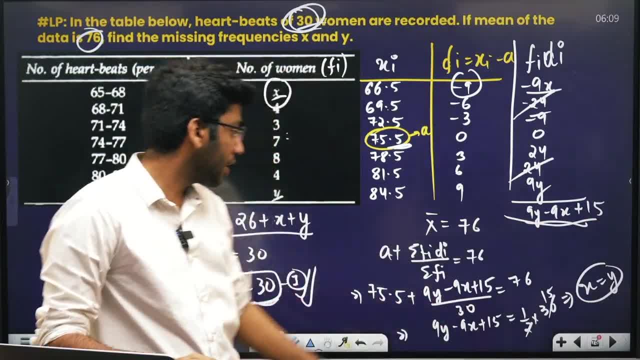 What is fi di submission? This is fi di submission. What was fi upon? What is the sum of all these? What is the sum of all these? What is the sum of all these? This is the sum of all these. It is only 30. 30 is only given. 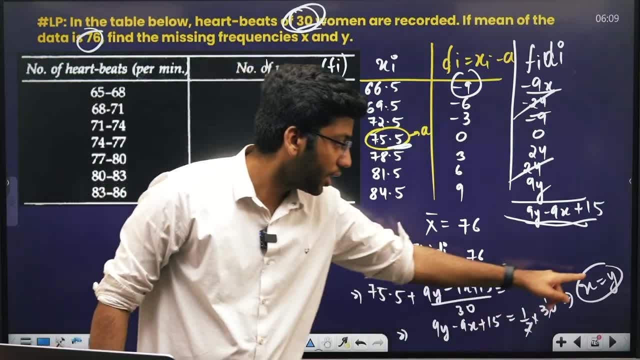 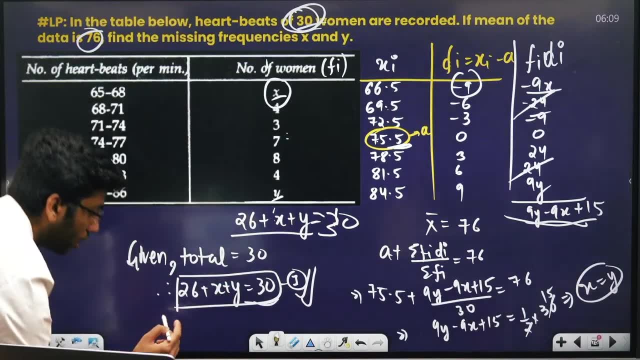 So upon, fi is 30 Equal to 76. From here I saw X and y came equal. That means, After solving this equation, X equal to y came That I put here: X equal to y. If I put here Then it will be 26 plus 2x. 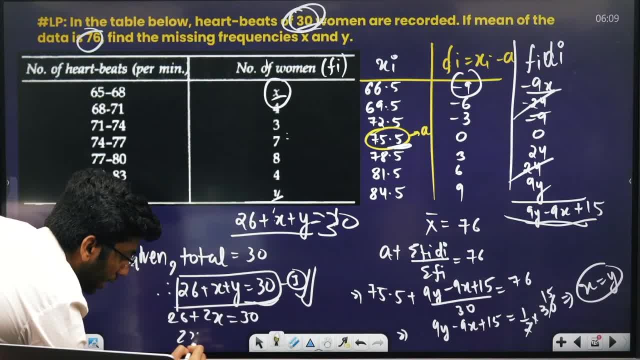 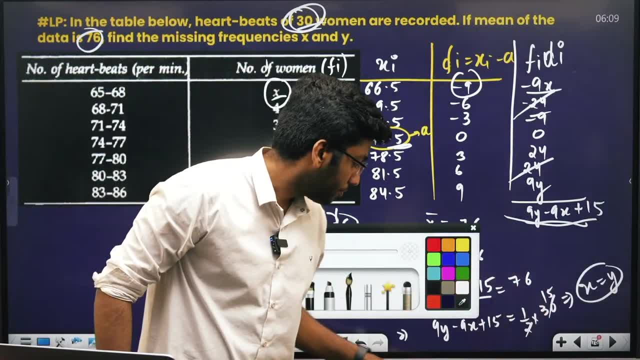 Equal to 30. So from here, 2x equal to 30 minus 26, 30 minus 26, 4. So from here, X equal to 2, X and y equal to. So if x is 2, Then y will also be 2, If x is 2. 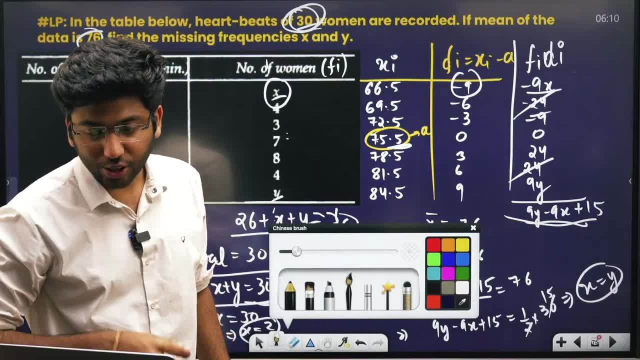 Then y will also be 2. If x is 2, Then y will also be 2. Alexa op is done. Ok, This is the question of our mean. This is the question of our mean. This is the question of our mean. One is yours, One is yours. 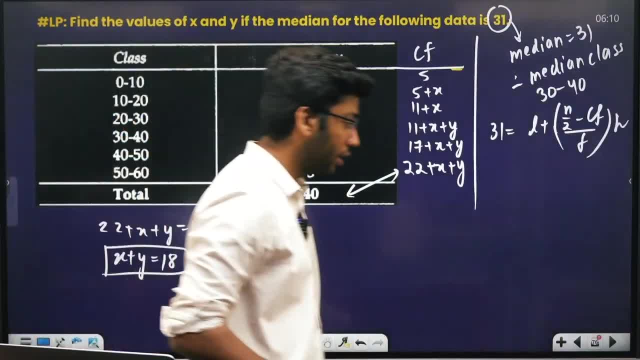 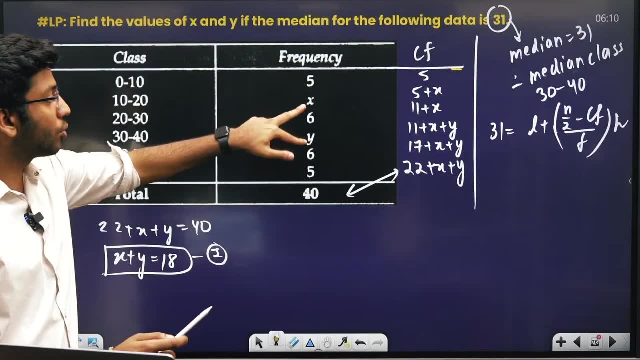 The question of median, Which we skipped today In the class Because I had to do this today. See, See carefully, See carefully, See carefully. In the median, In the median, In the median, You have to find these missing frequencies. This question can come Your question, This type of question. 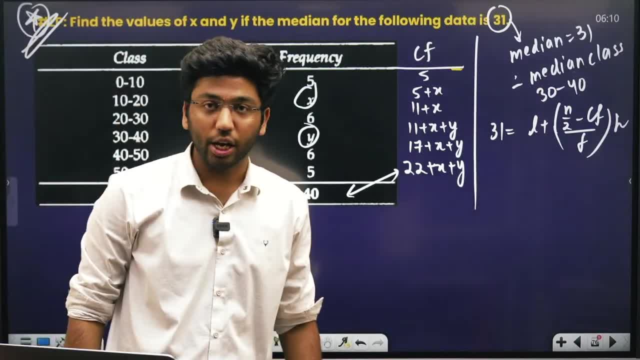 An example of missing frequency Can come in your exam. Take a careful look For 5 to 10 more minutes. Take a look carefully For 5 to 10 more minutes. Take a look carefully. So what is the走吧 formula for median, The formula of the median? 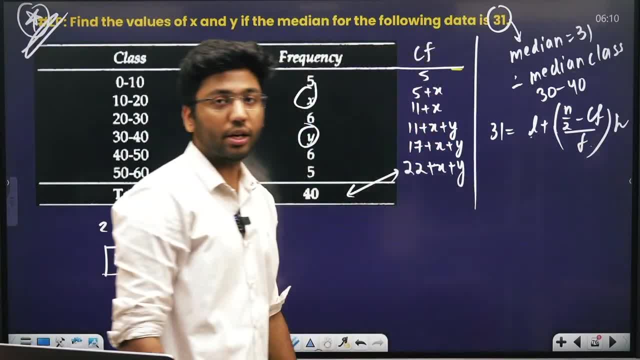 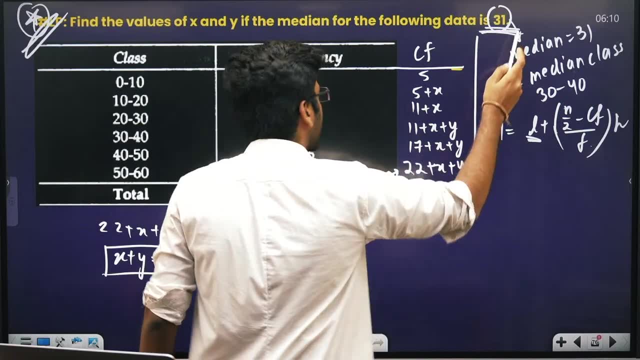 The formula is L plus n minus 1 Cf upon f into H. This is the formula of the median. This is the formula of the median. Ok, l means The lower limit of the median class. When the median is 31, The median is 31. The median is 31. 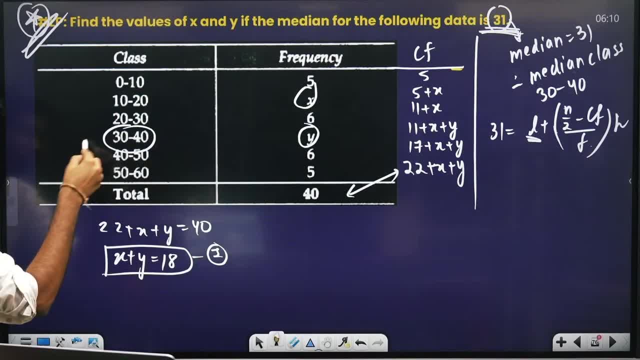 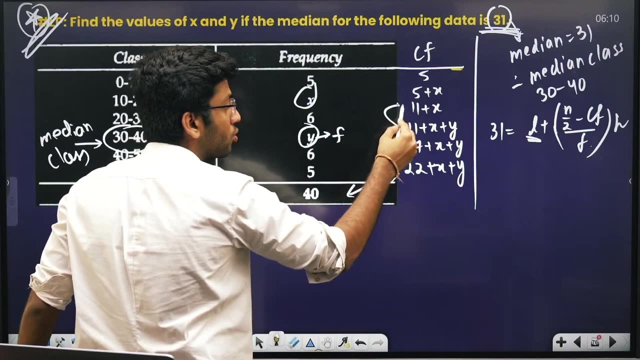 In which class is 31? Which class is 31, Which class is 31 Coming to this? So this is the median class, This is median class, This is the median class and the corresponding frequency of the median class is f and the cf above this will be cf. 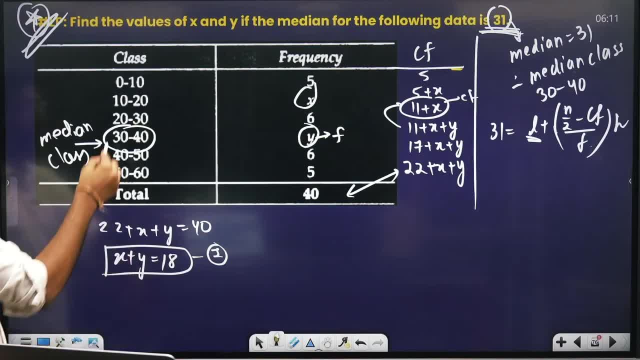 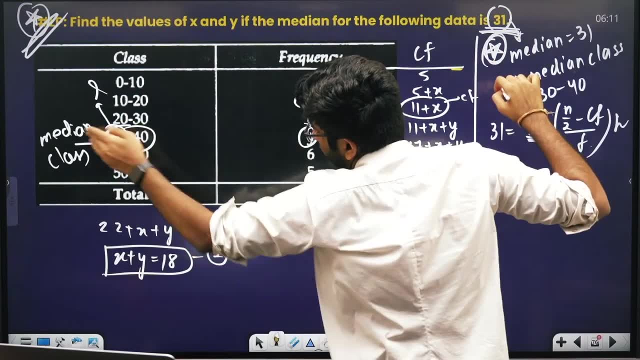 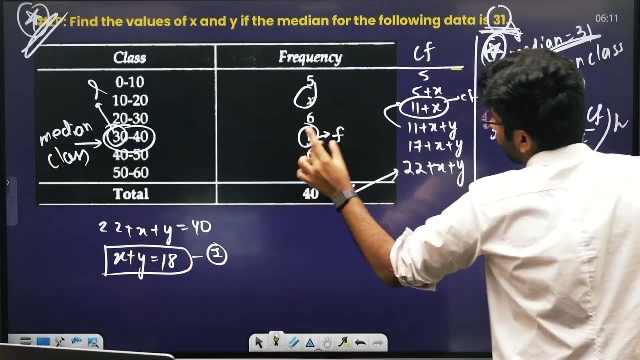 I got to know f, cf and l. This is the l of the median class. To get the median class, the most important thing was in which class is the median coming. The corresponding frequency of the median class is f and the cf above it is cf. 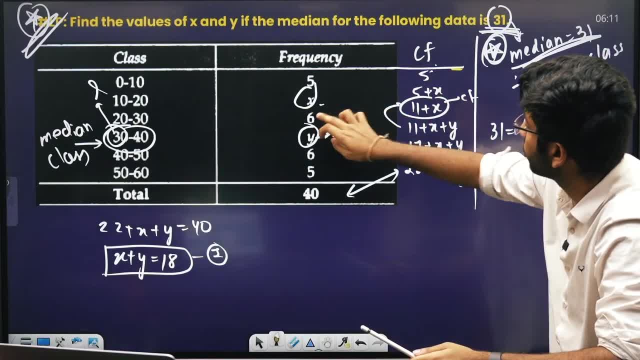 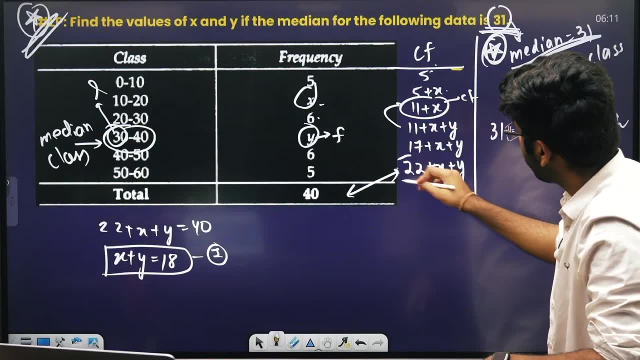 How do we get the cf: 5, 5 plus x, 5 plus x, 6, 6 plus x, 5 plus x plus 6, 11 plus x, 11 plus x plus y. This is how we got it. Then this cf is equal to 40.. 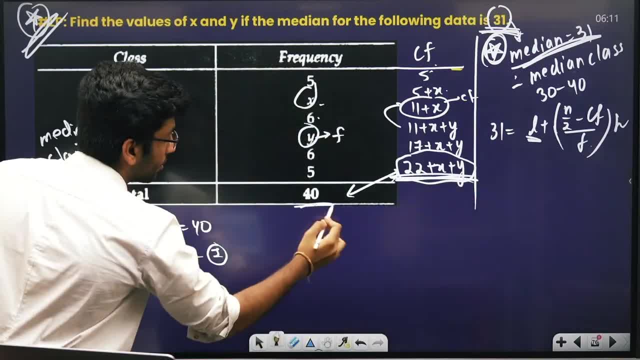 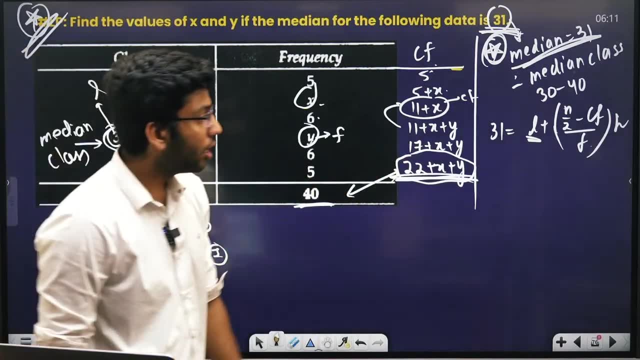 So the first equation came: that 22 plus x plus y is equal to 40. We had read this in the median, that the cf that comes at the end is equal to this. So this is the first equation equal to this, And now we will come to the second equation. 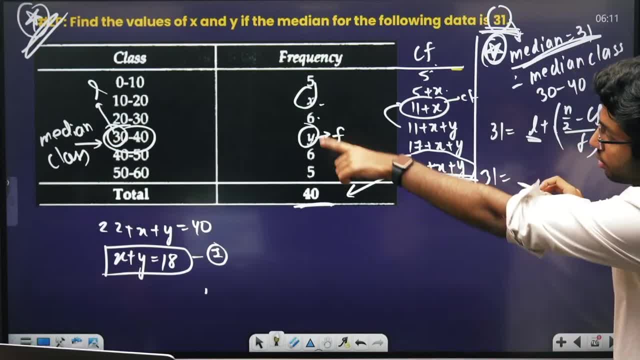 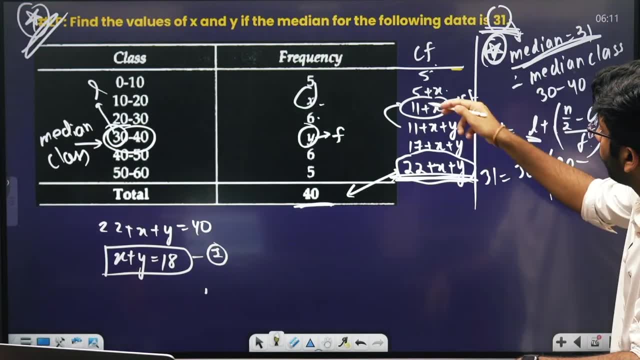 We will write it here. So here, if you see, 31 is equal to what is the value of l, 30 plus n by 2, n by 2 is 40 by 2.. 40 by 2 is 20 minus what is cf. The above, minus 11 plus f. 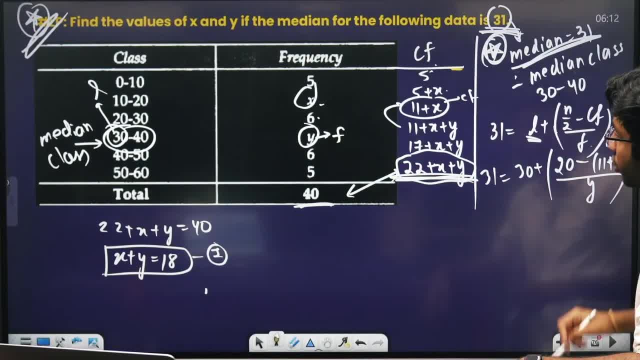 What is f in upon f is y. What is into h. h is the height class size: 10 minus 0, 10.. So into h, here we did 10.. Here, here we will do: into 10.. 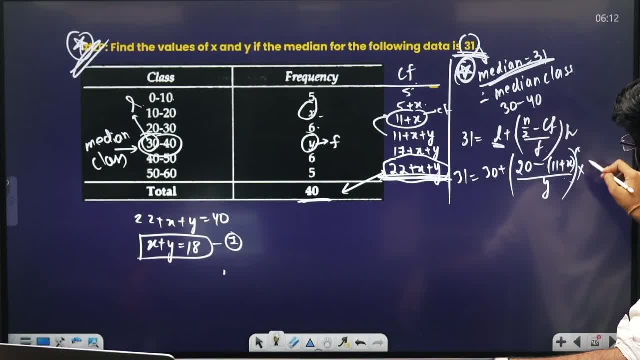 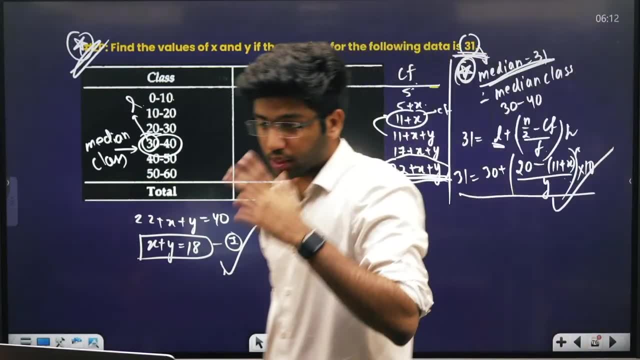 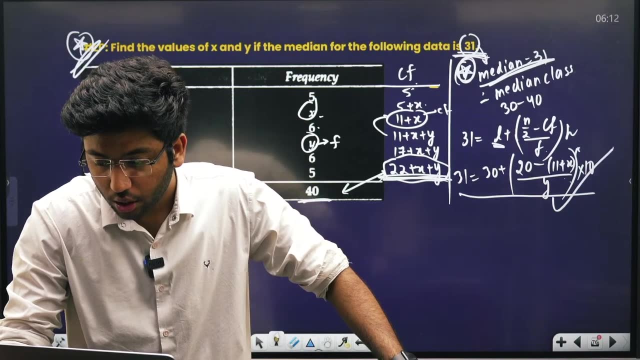 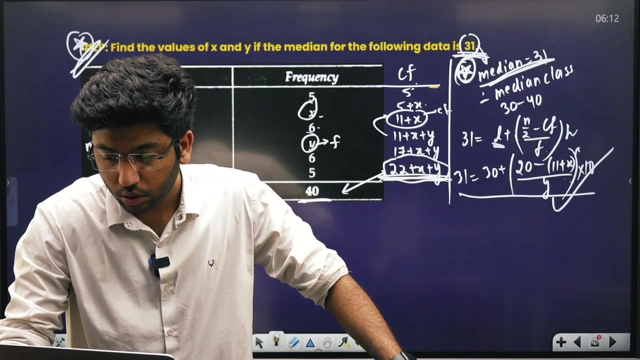 Here we will do into 10.. Look carefully here. Here we will do into 10.. So one equation became this And one equation became this in x and y. Solve this, Solve this. Okay. Okay, Understood, Brother. will the paper be easy? 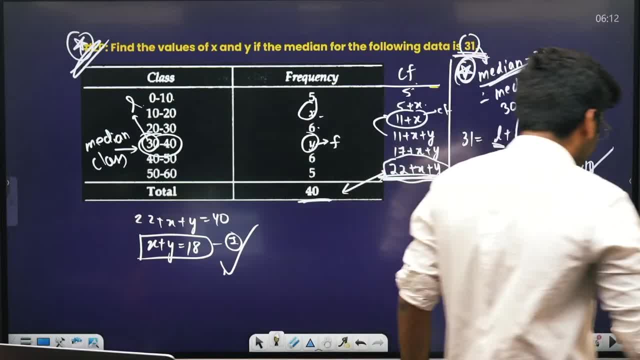 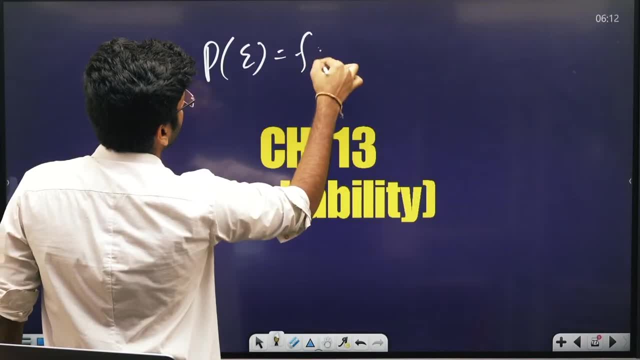 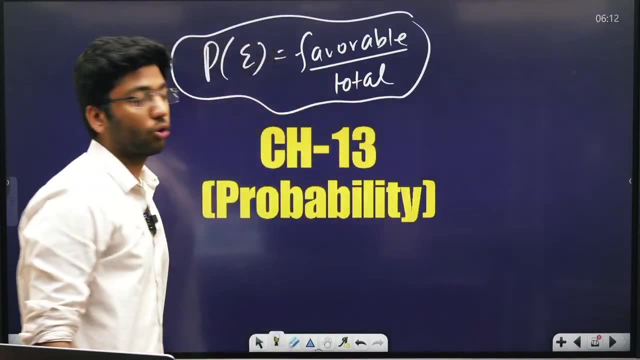 It will be absolutely easy, my love. You understood this right. Now comes the probability chapter. Priority: Priority of event. Priority of event is your favorable outcome. Total outcome in favorable upon Total outcome in favorable upon. So favorable, which is my favorable. 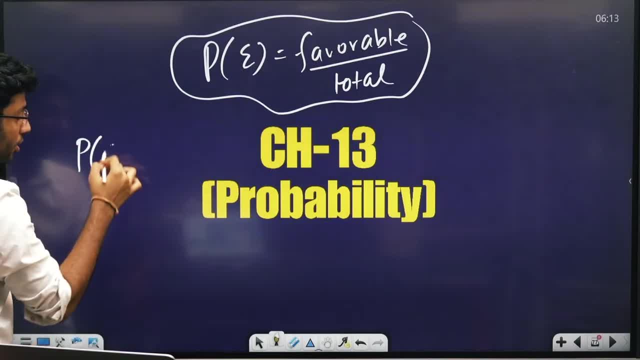 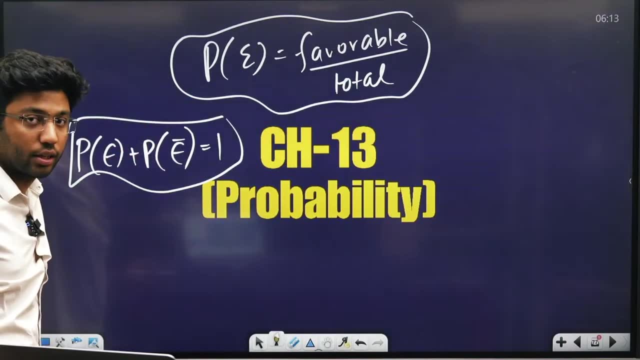 Total in upon. This is the probability. From this the question can come: Probability of e plus probability of not happening. happening of e Equal to 1. This is important. From this the question can come. So, if you have been told that the probability of having an event is x, 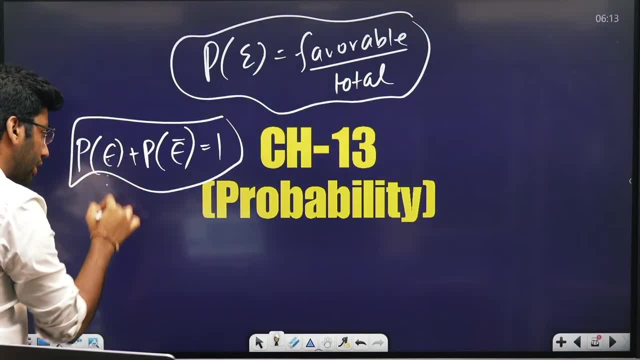 So what is the probability of not happening? So what will be the probability of not happening? So if it is x, So what will be the probability of not happening? This is equal to 1.. So the probability of not, e, Not e means e, bar. 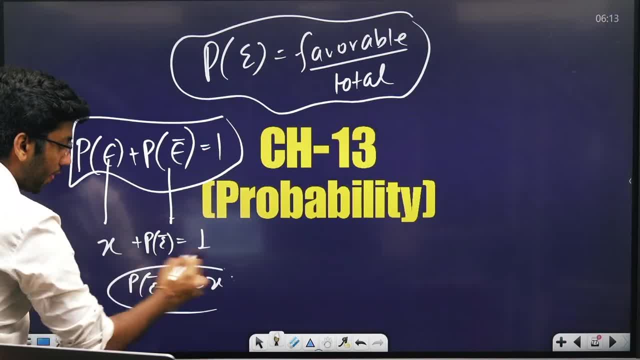 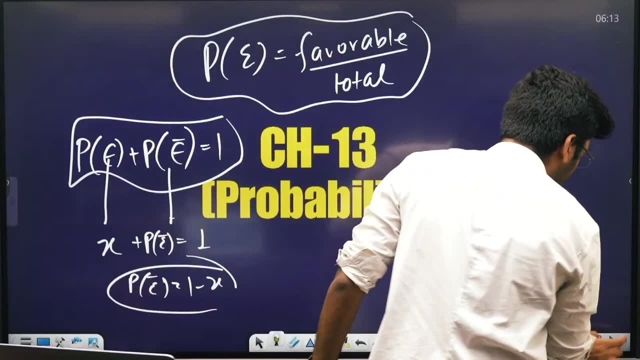 So what will happen? The probability of not e will be 1 minus x. On this, the question comes: We did it in class today. We did it in class today. We did it in class today. Okay, Find the probability of getting 43 Wednesdays in a leap year. 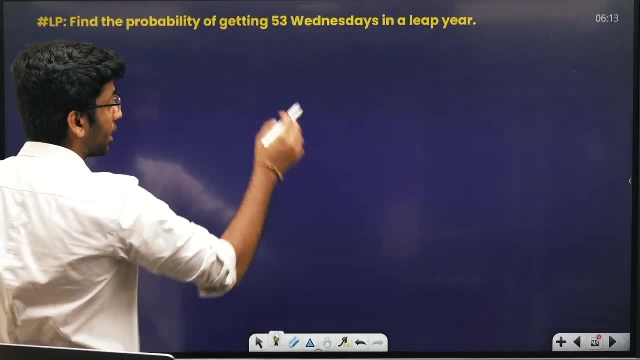 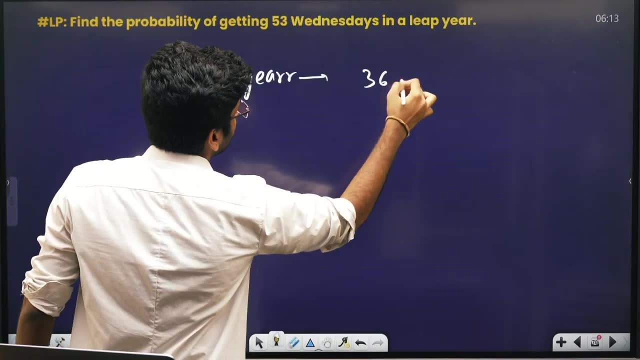 What happens in leap year? We did this question in class today, So I will tell you again carefully. The chances of getting this question are higher. What does leap year mean? Leap year means 366 days, So there are 367 days. 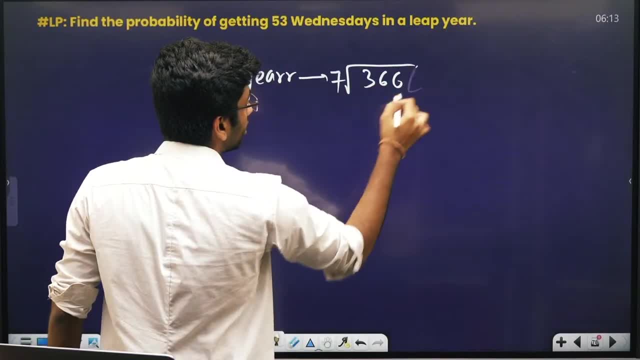 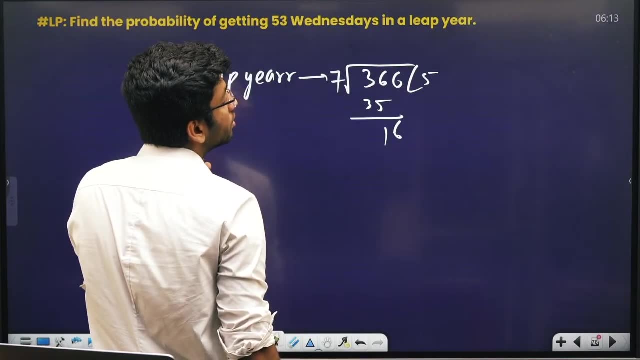 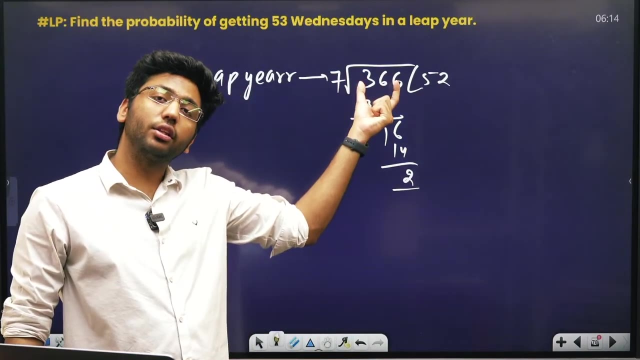 Okay, If we divide it by 7.. So 7 x 5 is 35.. 1 is 16.. 7 x 2 is 14. 2.. So see, my dear, There were 367 days If we divide it by 7.. 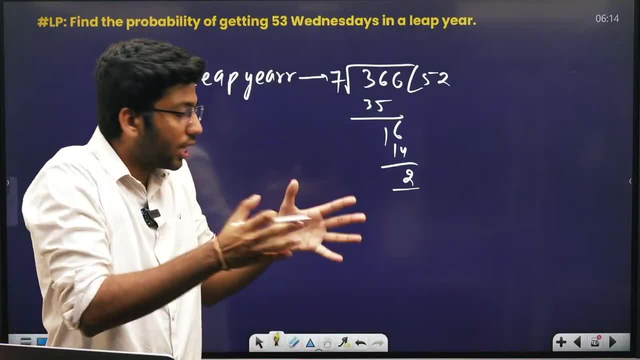 So it means There are 7 days in a week. So 7 x 7 is 7.. 7 x 7 is 7.. So then 32 weeks have come. There are 52 weeks have come. How many are 52 weeks? 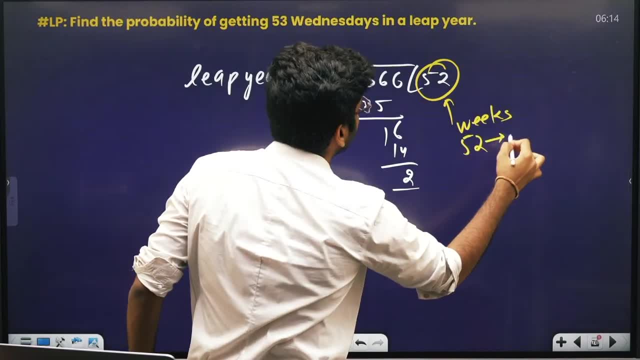 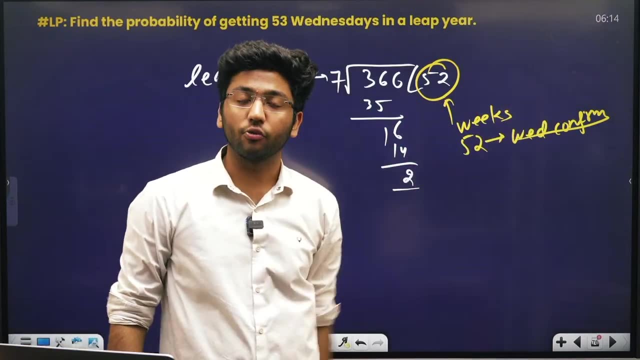 That means 52.. 52 Wednesdays are confirmed in 52 weeks. 52 Wednesdays are confirmed in 50. two Bache 2 din. bache 2 din Now, this 2 days, this 2 days. 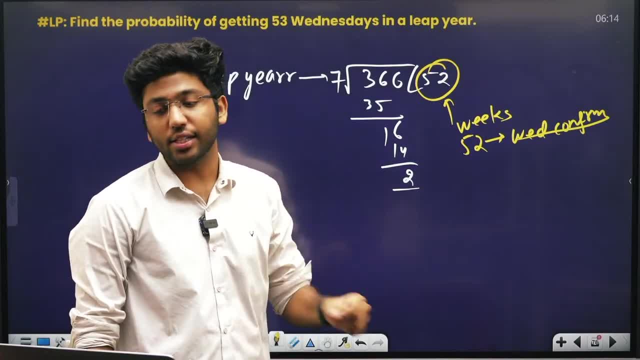 What is the� had probability of getting these 2 days Wednesday? What is the had probability of getting these 2 days Wednesday? What a probabilityあります? 2 days, this 2 days? What kind of things can be on it? 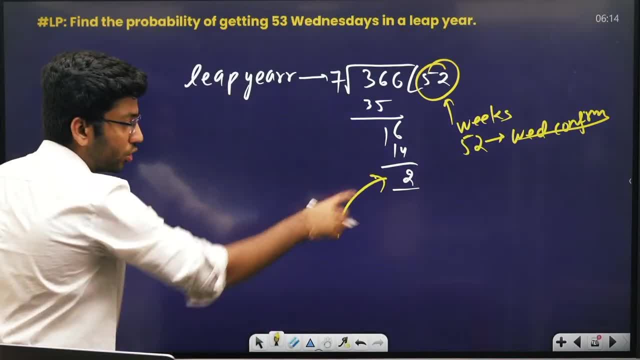 All right, I read 3 days. let me see. For how many days has it become? What is the probability of only getting these 2 days on both? Well, 52 weeks are over. Now 2 days are left. Those 2 days will be consecutive. 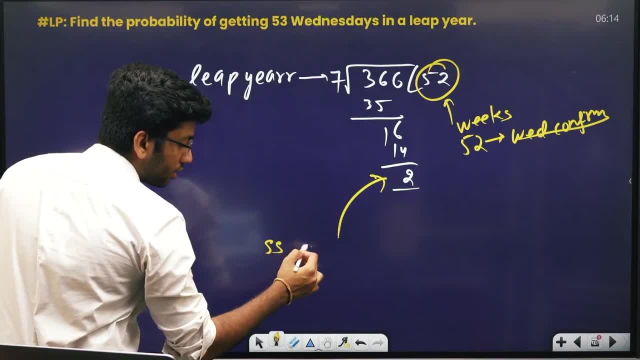 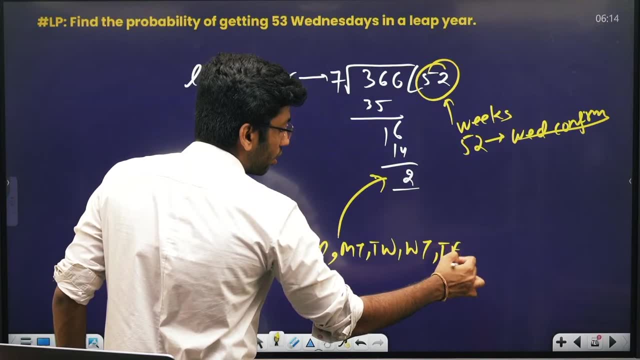 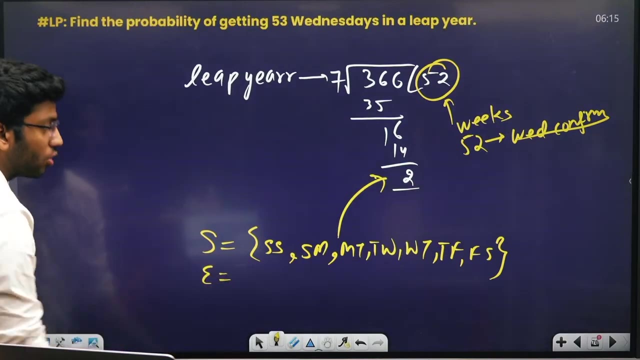 So suppose if Saturday is Sunday Or Sunday is Monday Or Monday is Tuesday Or Tuesday is Wednesday Or Wednesday is Thursday Or Thursday is Friday Or Friday is Saturday. So these are all possibilities, These are all sample space, And what is our work? 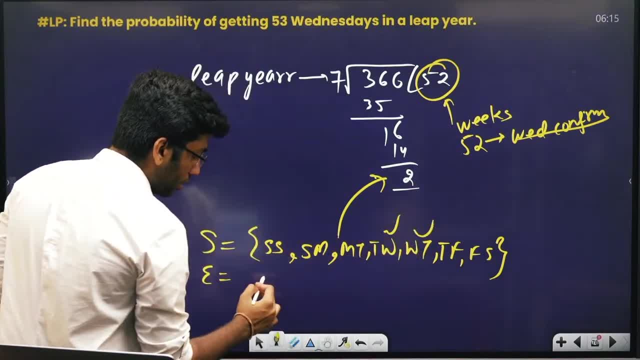 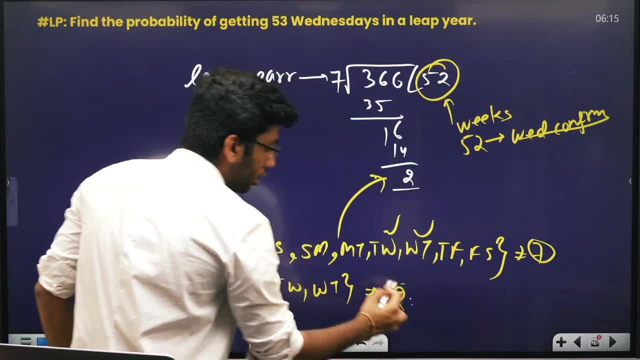 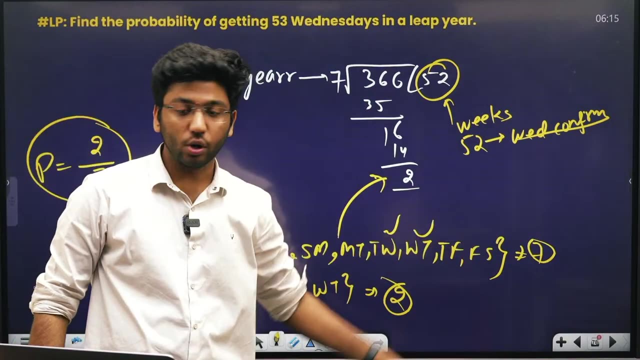 On which is Wednesday coming? On which is it coming? So our work is TW and WT, So total is 7.. And our work is 2.. So 2 by 7, it is your probability. Ok, If Wednesday is coming in 2, then 2 by 7. 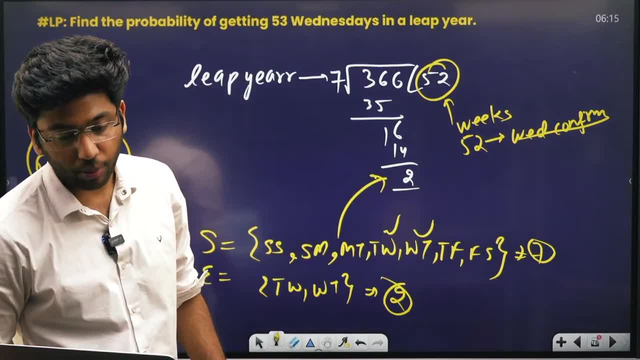 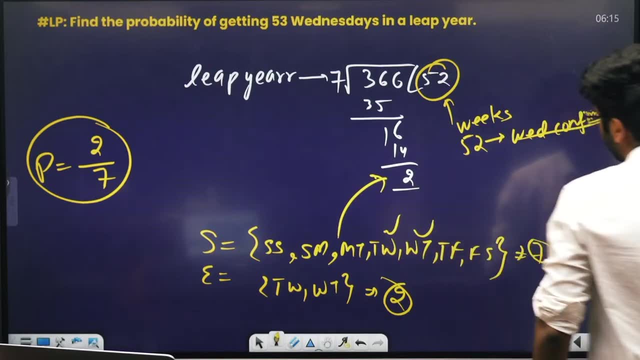 will be our probability. 2 by 7 will be our probability. 2 by 7 will be our probability. Ok, So in this way, we will ask this question when LEPR will come. 52 is confirmed, 2 is left. So what are the cases in 2?? 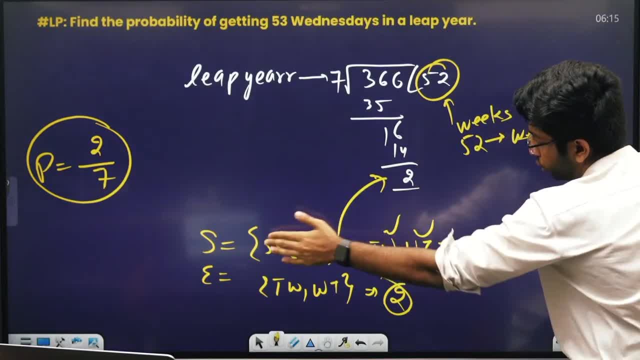 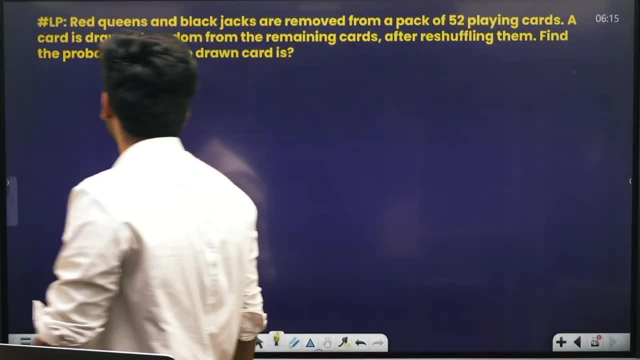 These are all cases, So total is 7 cases. 2 is our favourable. So 2 by 7, it is your answer. 2 by 7: it is your answer. 2 by 7: it is your answer. Now see: 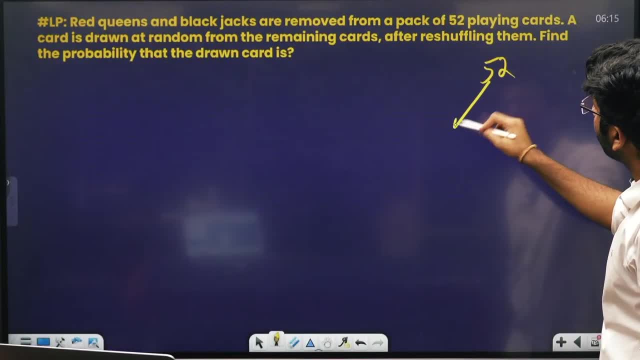 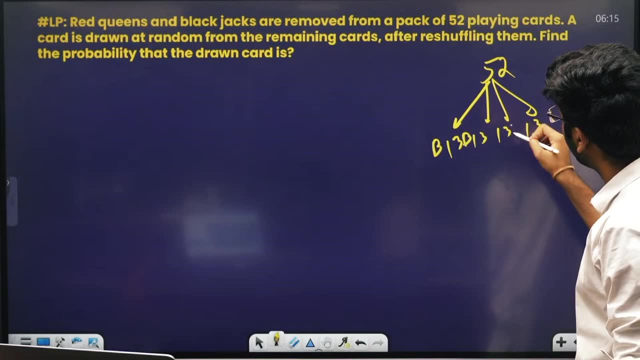 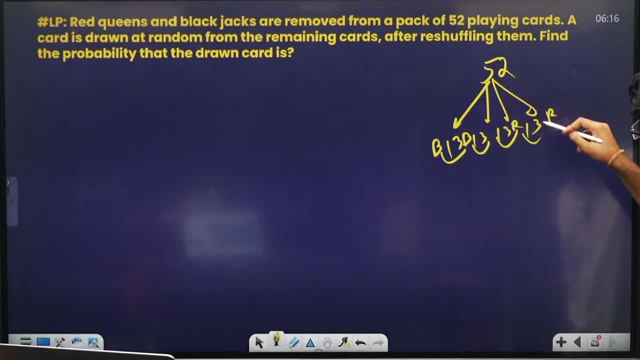 And 2 red red, 2 red red. This one is blue, This is called spade, This is club, This is heart And this is called diamond. Okay, These 13 is from 1 to 3, 10, and then it is king queen. 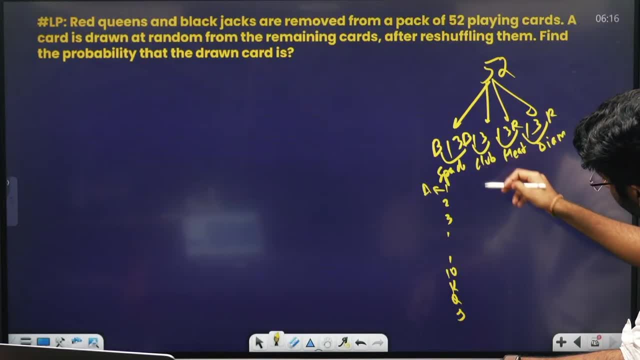 jack And 1 in ace class. Similarly, in this also, from 1 to 10 is king queen jack. In this, also, from one to 10 is king queen jack. In this, also, from 1 to 10 is king queen jack. 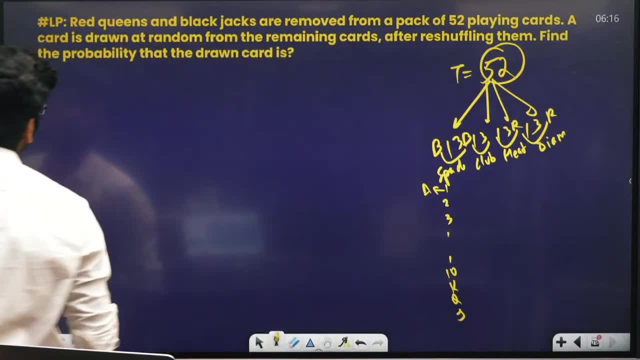 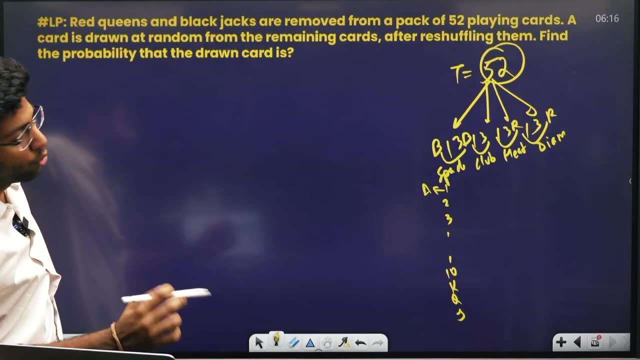 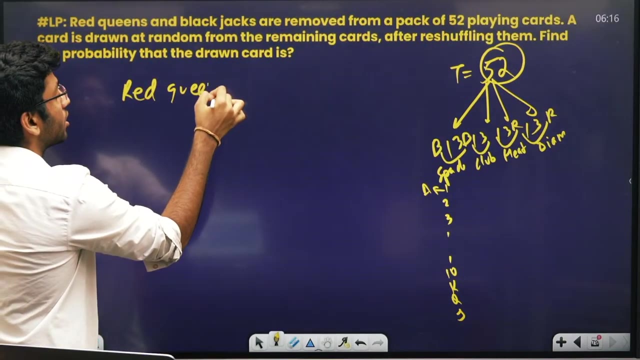 Total 52 leaves are there. We know this. So Red Queen and Black Jack removed. These are important questions. they come like this: Red Queen, how many Red Queens are there? How many Red Queens are there? Red Queens, how many are there? 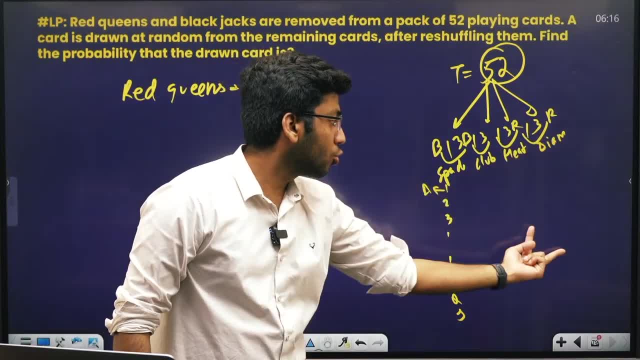 Red- how many are there? This is also red, this is also red. So we will get two Queens in this. So Red Queen is two And Black- how many Black Jacks are there? How many Black Jacks are there? 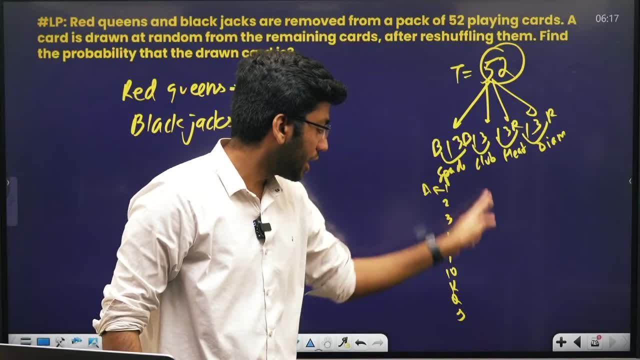 Jack Black. One is here in Jack in black And one is here in black, So there are two Black Jacks. So what did we do? Out of 52 leaves, we removed these two and two. We removed these four. 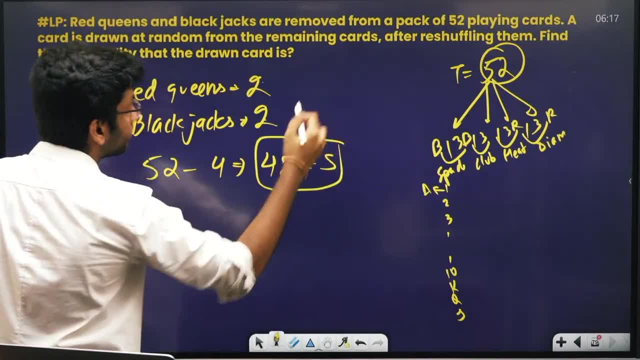 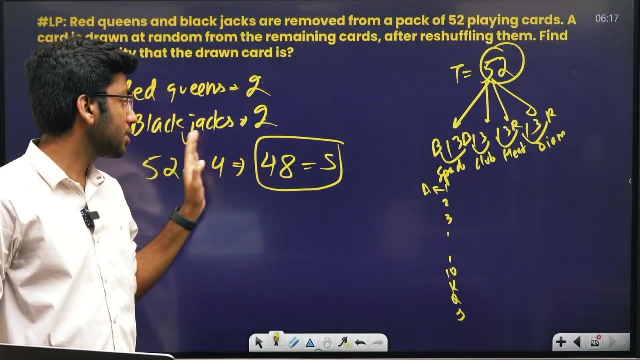 That means 48 leaves are left. So this is our sample space. What did we do? We removed two Queens, removed two Jacks Out of 52.. So, out of 52, if we remove four, if we remove these four leaves. 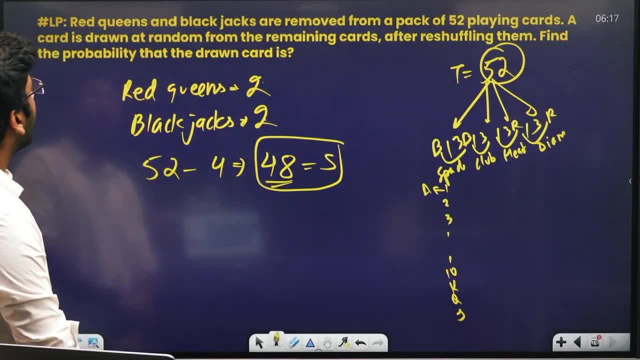 then what is our sample space? 48. Now a card is drawn at random from these remaining cards. Now, from these 48 cards, we picked up a card. Find the probability that the drawn card is Hey. Hey, This is half of the question. 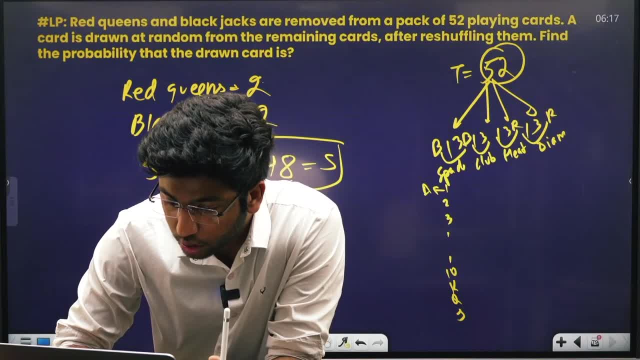 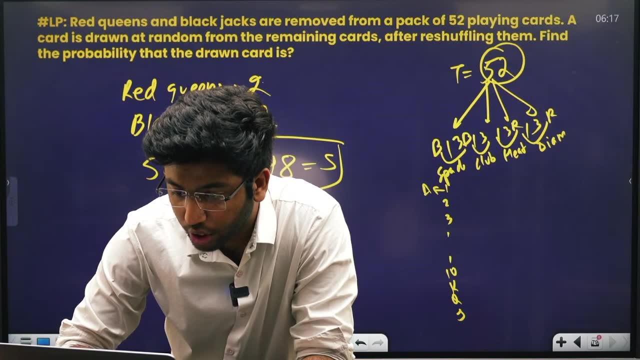 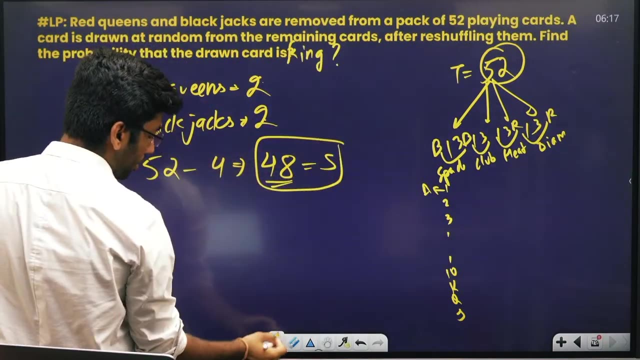 The drawn card is. The drawn card is: Hey, This is half of the question. One second: The drawn card is First King. The drawn card is King. Tell me there is a King. What is its probability? So look, my dear. 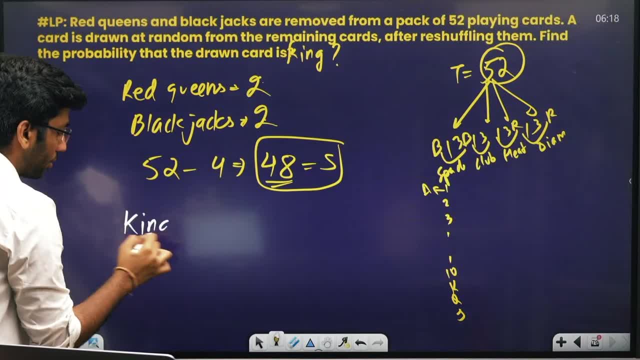 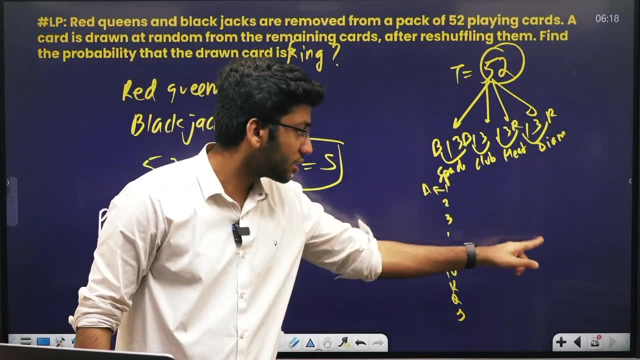 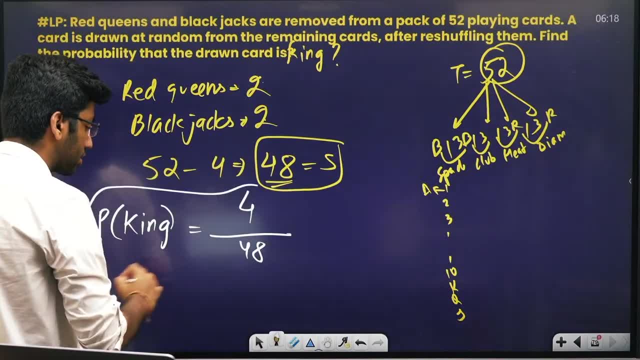 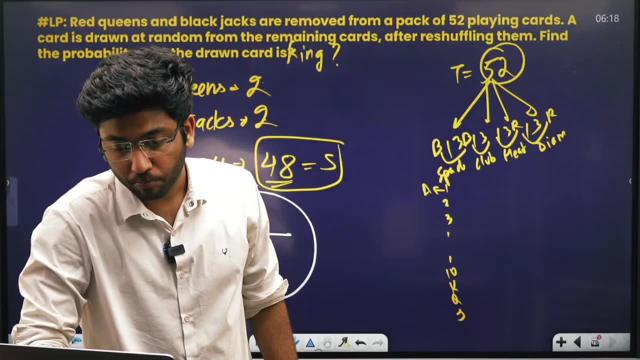 So there are 4 Kings, So 4 upon 48.. 4 upon 48.. This is your probability of the King 4 upon 48.. This is your probability of the King. Okay, 4 upon 48.. 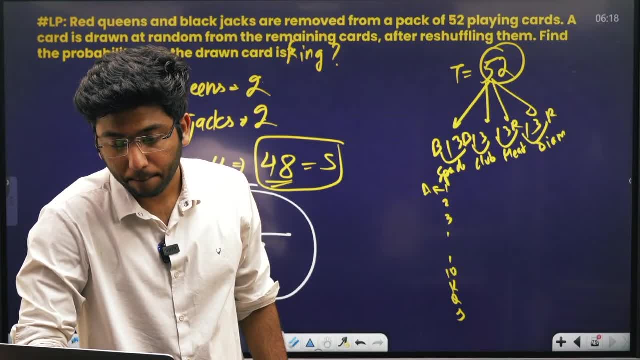 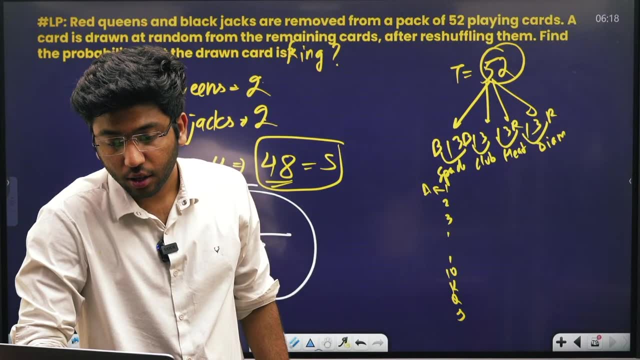 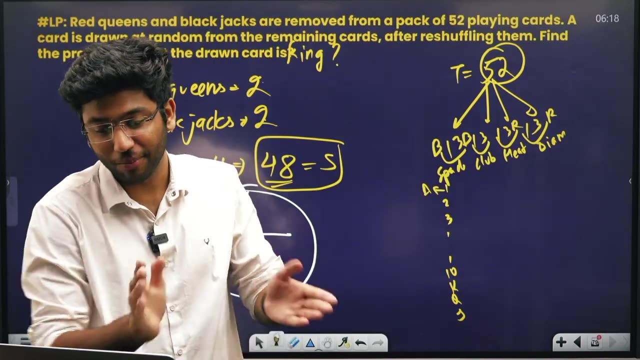 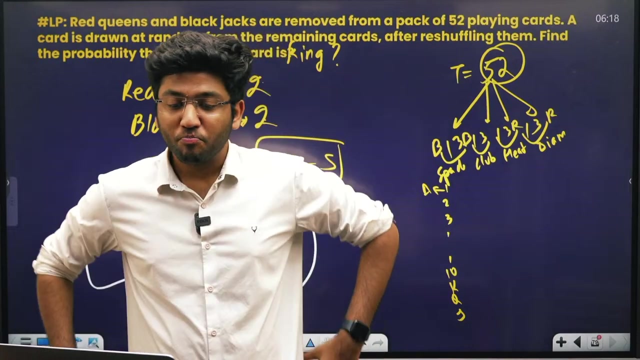 This is your probability of the King King: 174, 1174 thousand kids, Great, Great. Thank you so much. Thank you so much. So this is my answer. All right, This is my answer, So we will ask the same question. 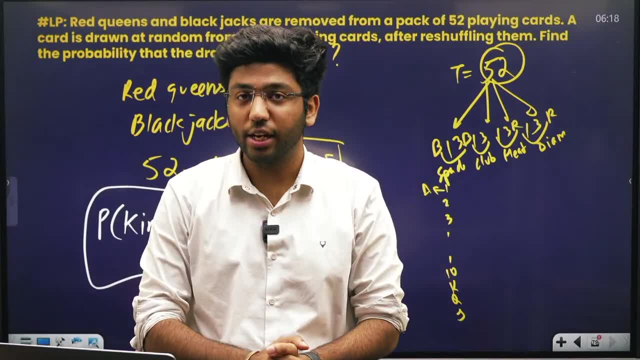 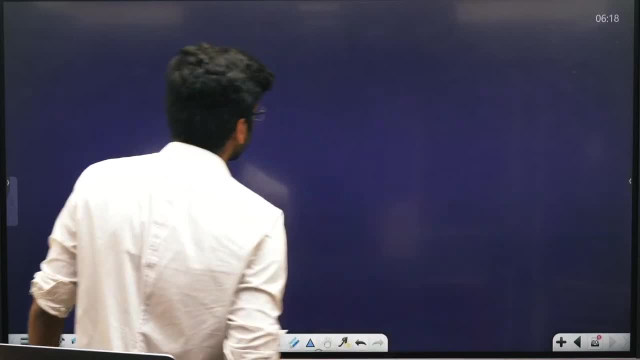 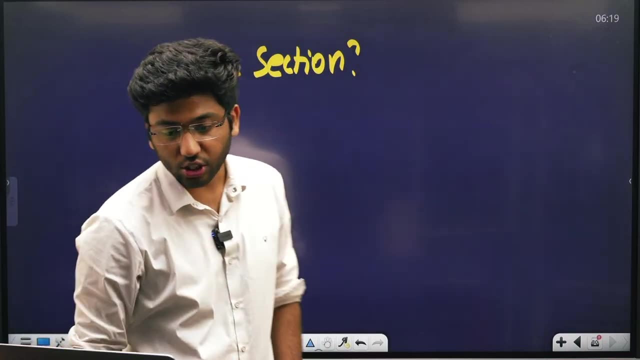 in the same manner. We have revised all the chapters. We have revised all the chapters. Let us wait for 2 minutes. I will tell you after the presentation. The main thing is: which section should we start from, Which section should we start from? Watch carefully If you start from the first section. 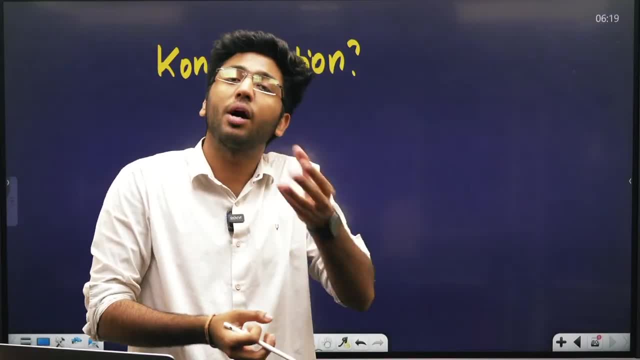 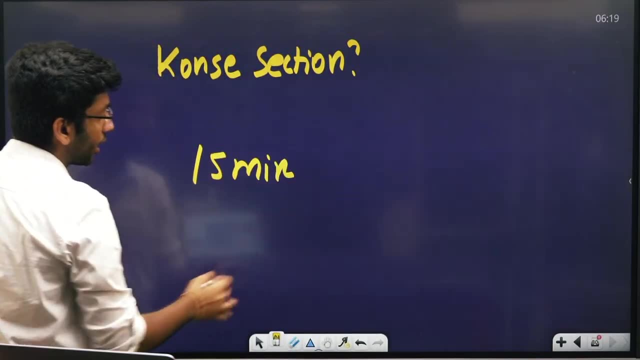 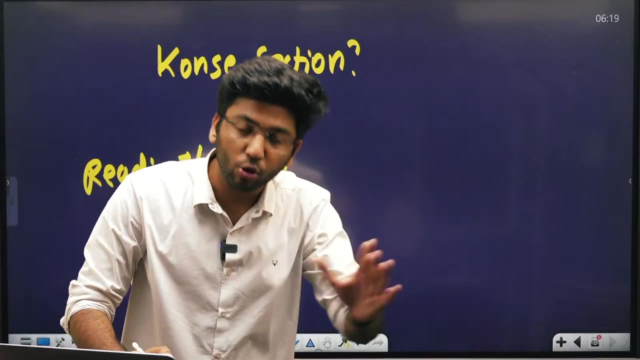 then you will start from 1st number, 2nd number, 3rd number, 5th number. According to me, the 15 minutes that you have in the beginning, this is your reading time. In this reading time, in this reading time, in this reading time, go through the whole paper once. 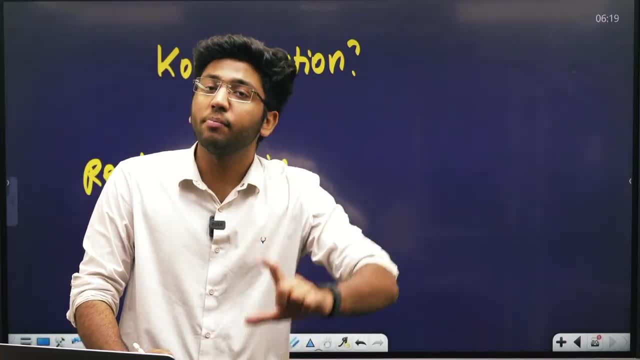 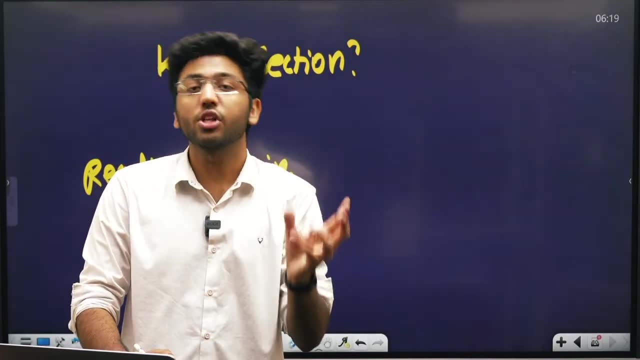 Whichever section you find that you get the maximum number of questions from, pick up that section. Whichever section you find that you get the maximum number of questions from, pick up that section. First thing, first thing. Okay, Pick up the section and complete it there. 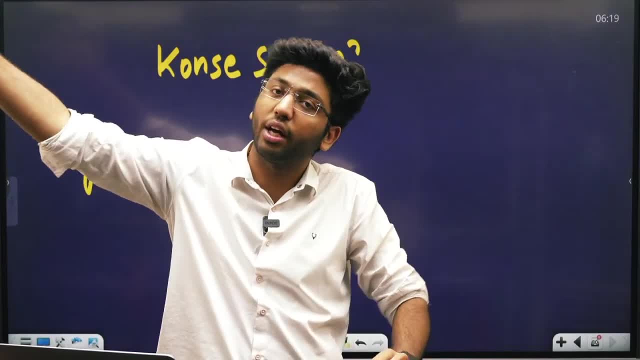 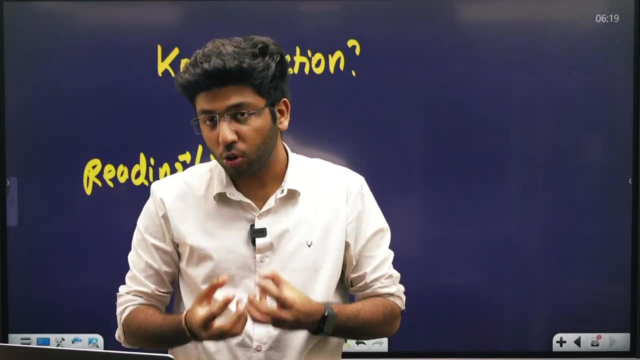 Not this. I have already done it. You are doing the 10th question at the very end. Don't do it like this: The paper that the teacher is checking your paper. That paper, that paper, the teacher who is checking your paper. 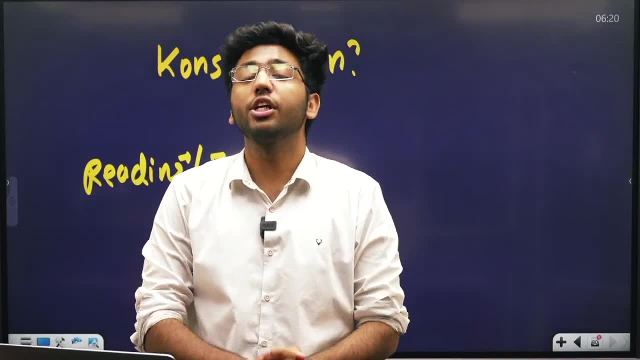 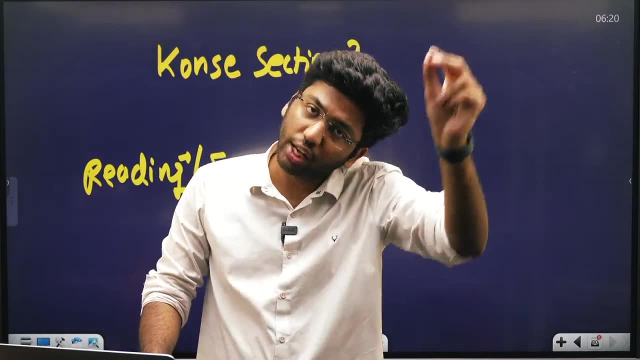 You don't have to trouble that teacher. If you trouble, then the teacher will cut your number. So let's go in a sequence. Suppose if you started from section D, then do all the questions of that D there. If you don't know, then leave the page and do it on the next page. 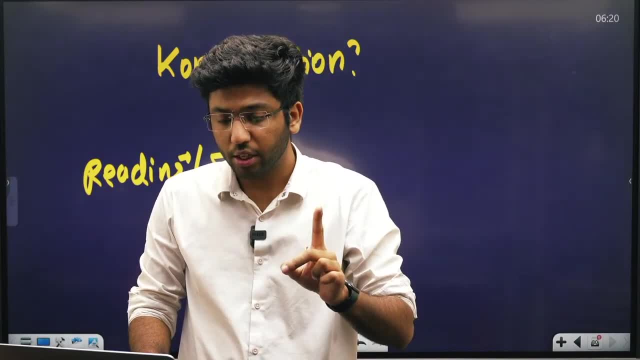 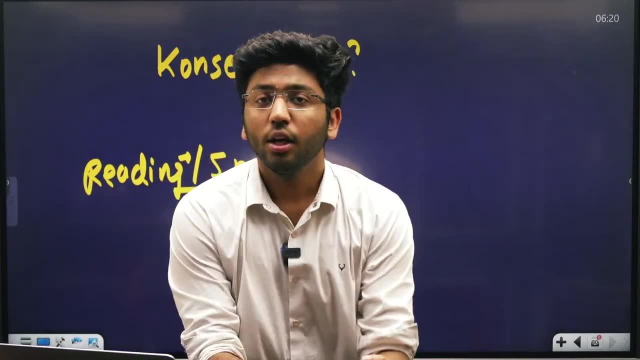 Second question: But all should be there. Do you understand what I am saying? All should be there. Listen carefully, Listen carefully. It is important. The first thing is this And the second thing: Calculate very carefully. Okay, I am telling you very nice things. 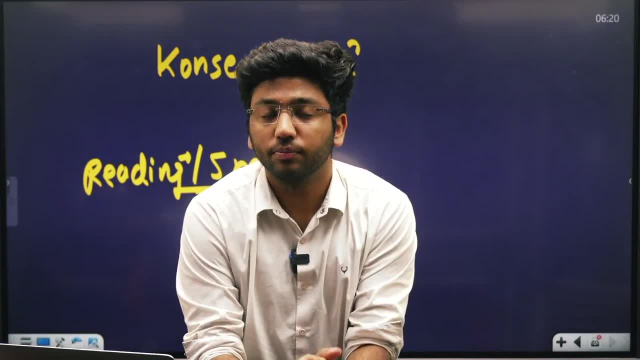 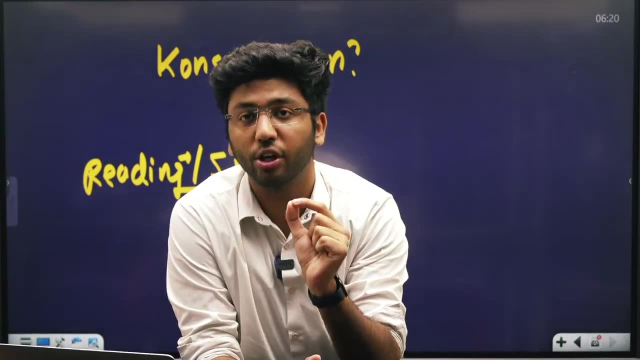 Listen carefully. I will take 10 minutes of your time. I will take 10 minutes of your time. Listen carefully. First of all, go to the exam hall Now. listen carefully with your eyes. Okay, Mr Shauyit is telling you very important thing. 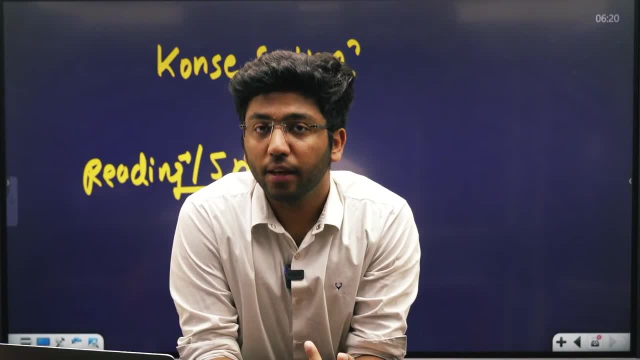 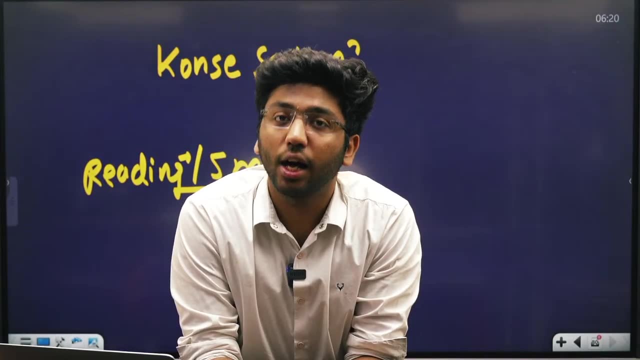 The first thing is this. The first thing is this: That that as soon as you enter the exam hall, Listen carefully, Listen carefully As soon as you enter the exam hall. So in 15 minutes you have to see which section you know the maximum questions. 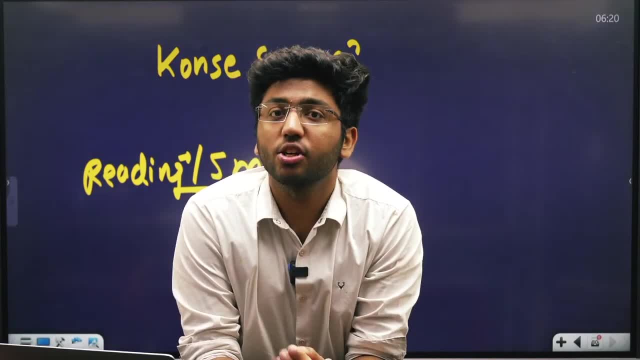 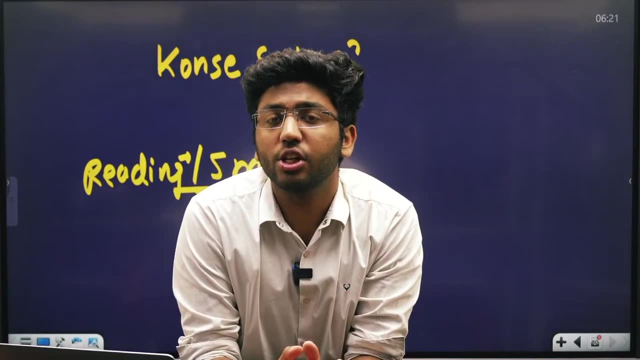 Okay, Look carefully Now I am looking at you. Which section do you know? the maximum questions. Pick up that section first. Okay, Try to pick up the section with high marks first So that you write it in very good writing. Reduce the cut-peat more. 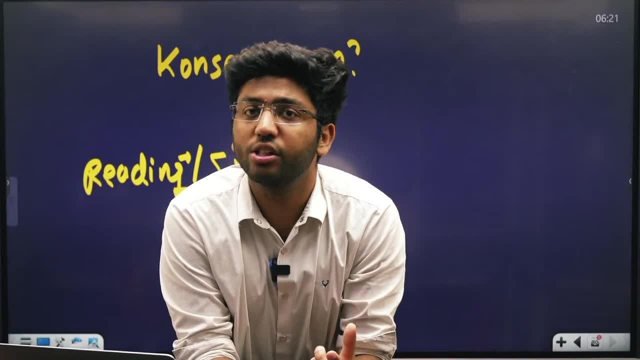 So the teacher will reduce the cut-peat. See, the teacher is that moody teacher Who is checking If he felt that there is a lot of cutting. There is a lot of cutting. Some question is done somewhere. Some question is done somewhere. 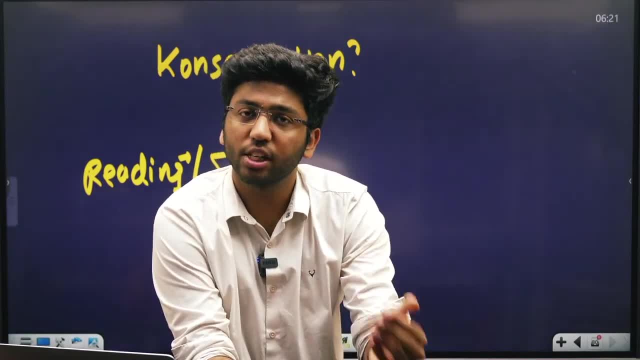 Now suppose he is checking. He saw the 10th question, Then after that you did the first after the 10th. So he will flip the question paper again and see the first question. Then you did the third after the first. 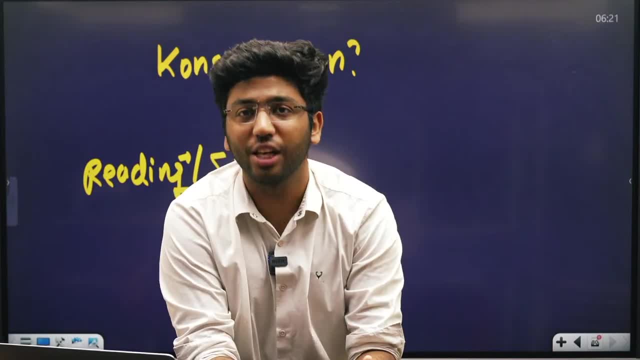 So he flipped the question paper and saw the third question. So you are giving him a lot of trouble. my dear, Don't give him so much trouble. Do all the questions of the section you are picking up there. If it is not coming, then leave the page. 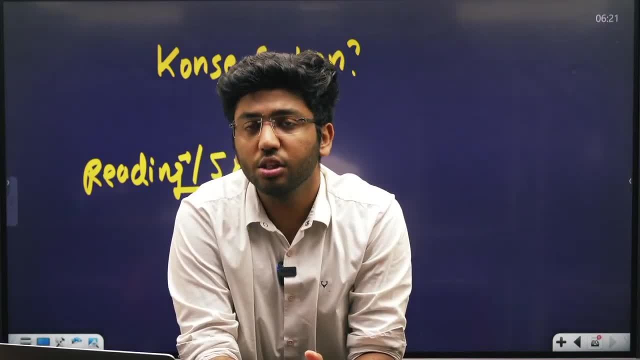 This is the first thing. This is the first thing. Second thing, Second thing, Second thing: In 15 minutes you have to see which one, And in 15 minutes You have to see all the case-based questions in the section. 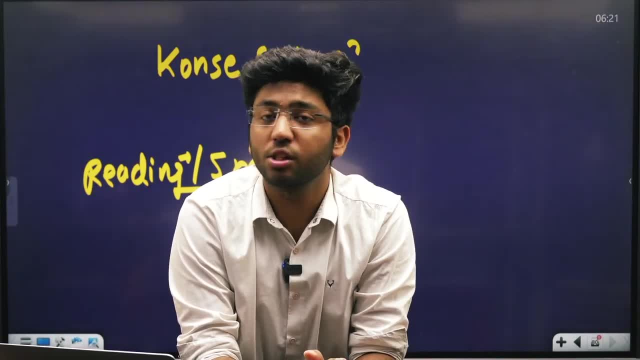 Don't pick up the case-based questions first. Okay, Don't pick up the case-based questions first. Just see the case-based questions once in the reading time, Think about how to solve it, But don't do it first. So first of all, according to me, there should be the heaviest section. 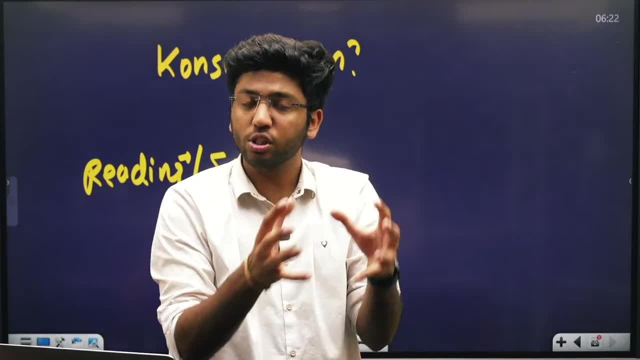 Not case-based, The one after that, Which are the questions of number 5.. So, the heaviest, Less than that, Less than that, Less than that, And then, in the end, do the case-based. Okay, Did you understand this? 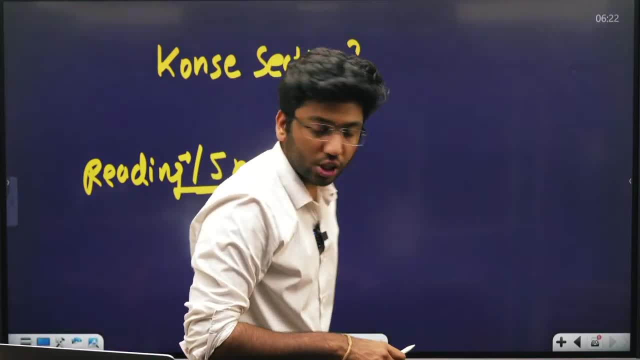 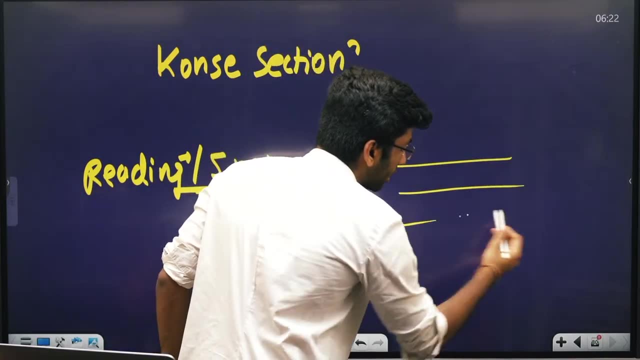 Calculation, always Calculation, always, Always double-check, Always double-check the calculation. What I mean to say? See, Assume you did one step, Then you did two steps, Then you did three steps, Then you did four steps. Now stop at four steps. 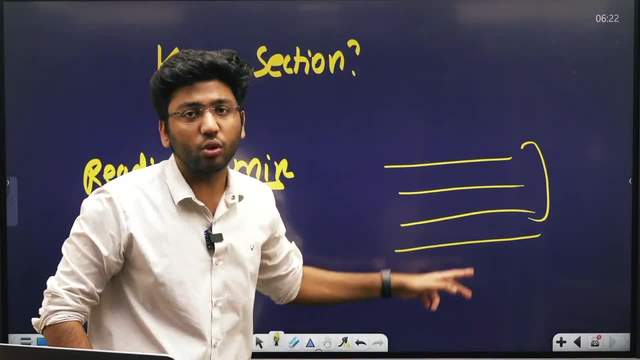 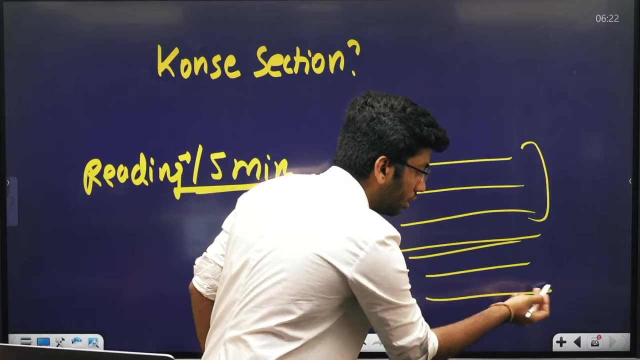 See once These three steps. Did I make any mistake here? Stop for a second. Look up again That I didn't make any mistake. If it's right, then start solving it further. Then, when there are three or four steps, 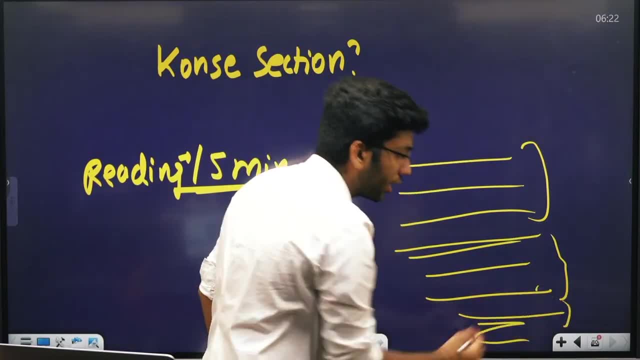 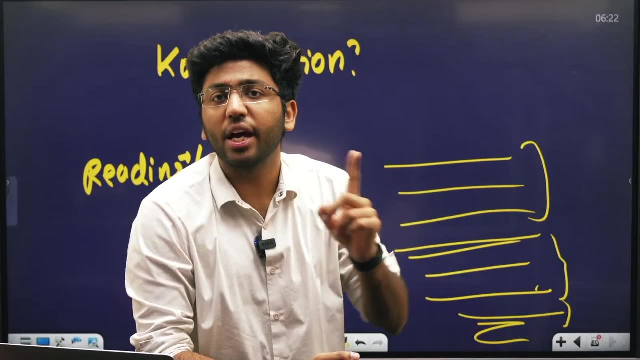 Then look up a little. Then, when there are three or four steps, Then look up a little What will happen with this If there is any mistake. I always do this. don't ever do this in your calculation- that I have to do the calculation very fast. 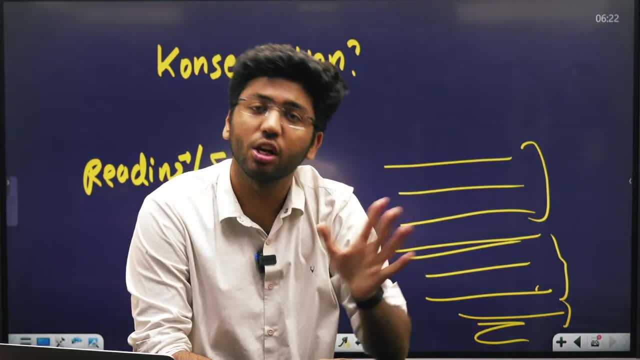 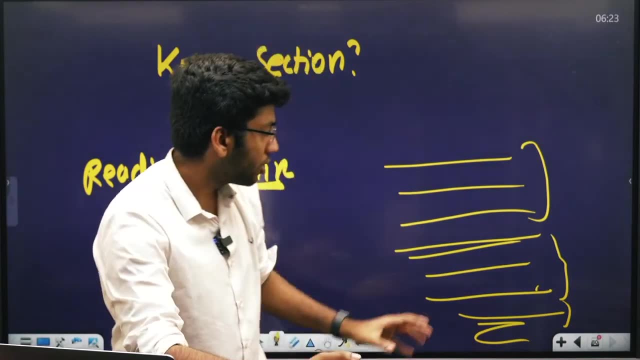 The answer should be correct as compared to the whole question being wrong. We are not racing with anyone. we are not racing with anyone in the class. We just have to see that our step should be correct. So do the calculation, like children. You must be seeing here that I do the calculation 13x9.. 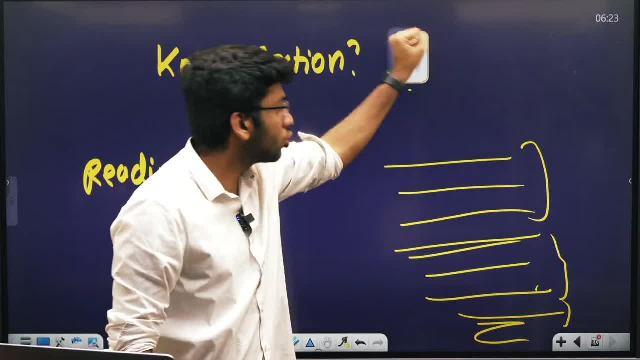 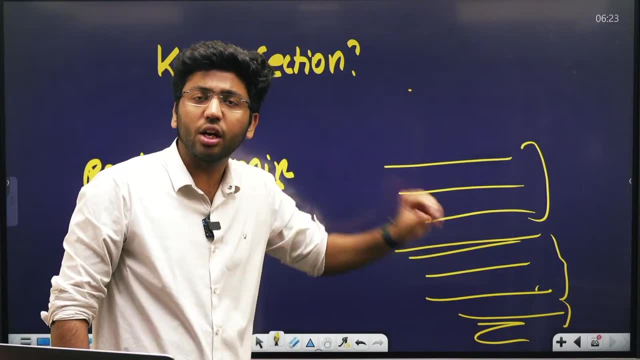 Do I not remember? Yes, I remember, But I do it like a child to make you understand, Because sometimes we do it wrong every time. So that's why do the calculation like a child. Whatever is the basic, do it in the back track. 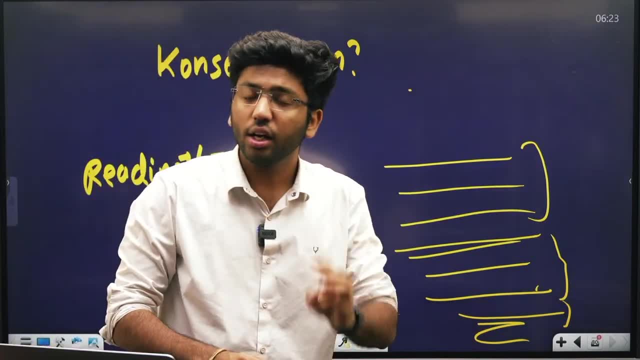 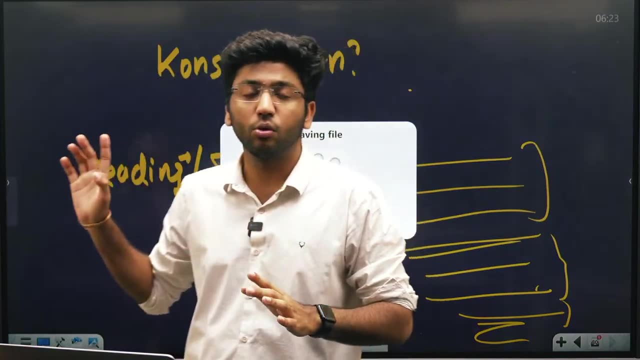 Do it while back checking. This is the second thing. The third thing: Now it is done, I am saving it. I am saving it. I will give it on the telegram, If you want. you can see the PDF. If not, no problem. 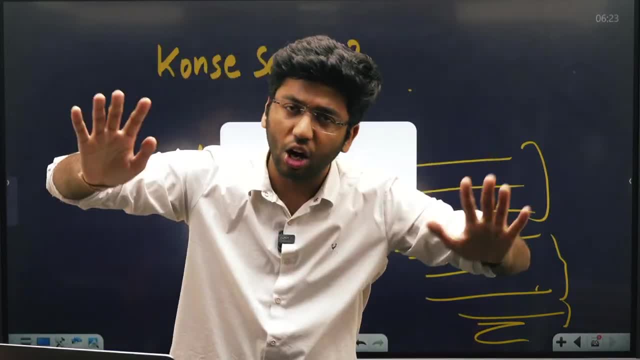 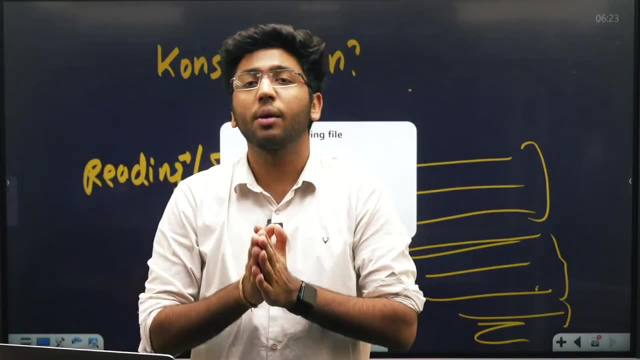 Now chill calmly. All the tension is gone. Leave it. Go and take a bath. Drink, Eat your food. After eating your food, touch the feet of your parents in the morning. Touch the feet of the elders in the house. Take blessings from them. 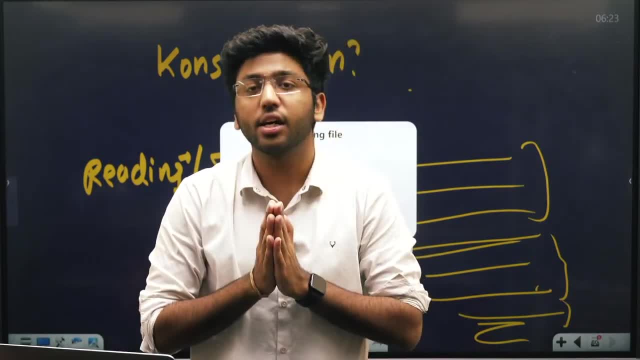 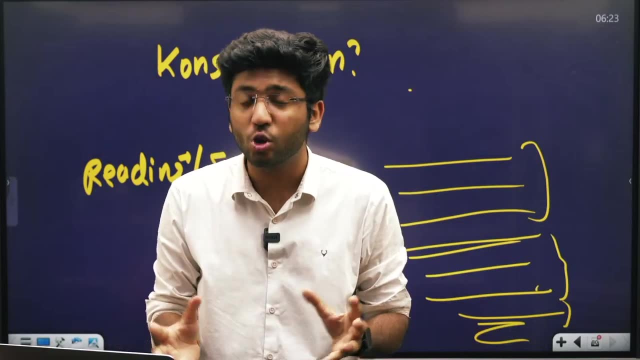 Okay, Whoever you ask for, God, you have to join your hands in front of them. once That, God, I have worked hard on my own. I have given my 110% on my own. I did not sleep the whole night. I did not sleep the whole night. 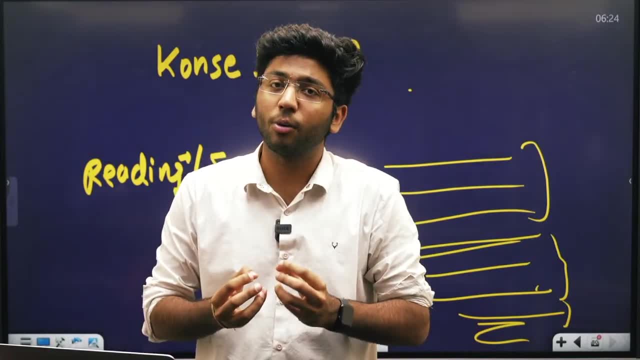 I woke up in the morning and took the session at 4 o'clock, So I am working hard on my own. God, Please give me such questions that will be done by me. Okay, Please give me such questions that I have seen. 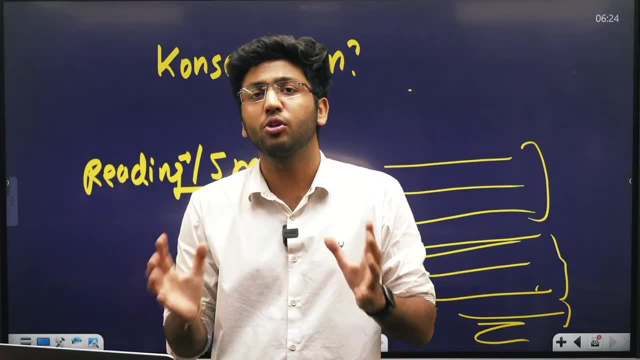 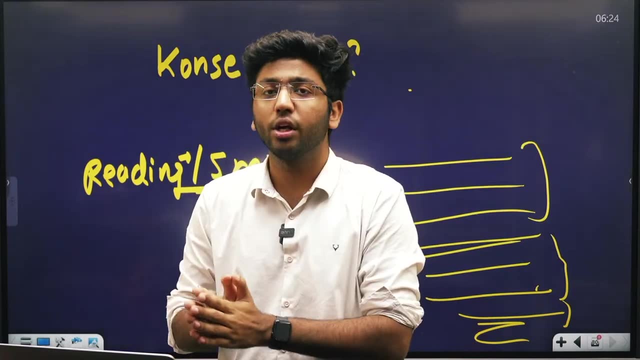 So God will help you at that time. Okay, Whoever you believe in God, you can say this thing to him Before going in the morning: touch the feet of the elders once And once. you have to go in front of them by joining hands with whoever you believe in God. 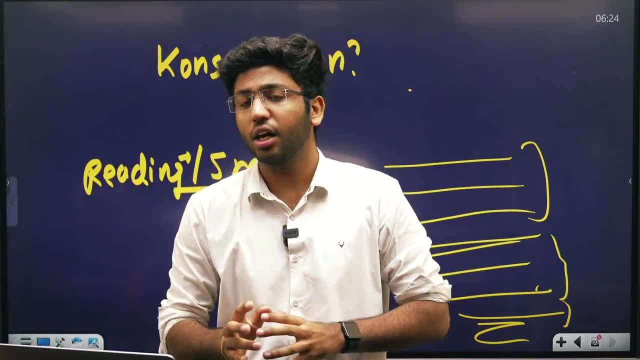 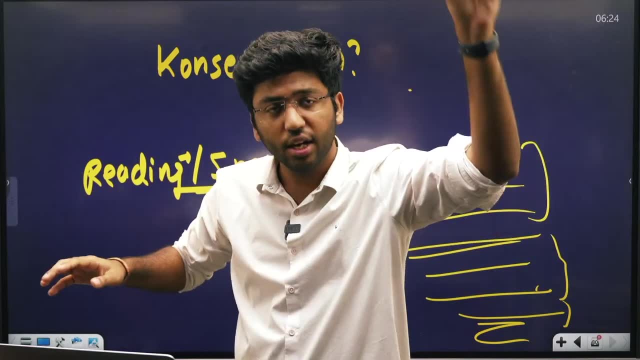 Okay, This is the second thing. Take your water with you. Enter directly into the center. Do not discuss with anyone that how much is yours and how much is mine. Everything goes to hell. You have to enter directly. You have to give the exam. 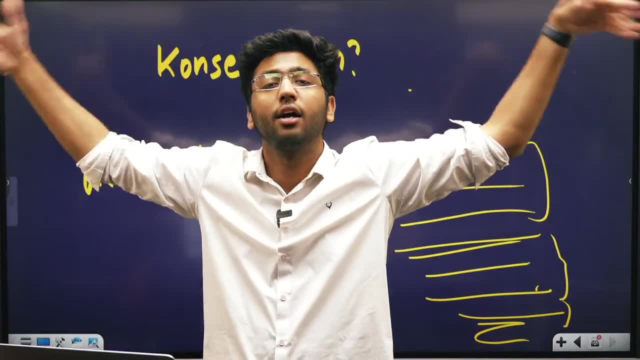 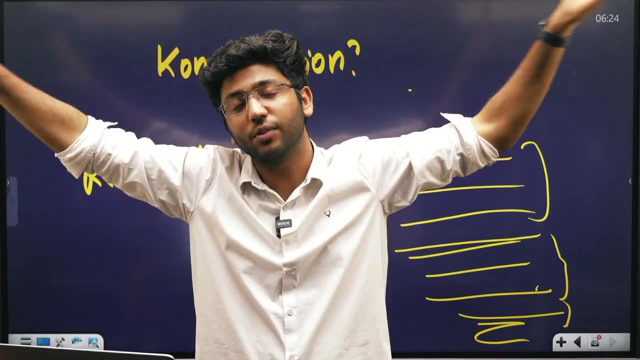 You have to come out- No discussion. You have to come home, You have to sleep, You have to chill. Okay, The exam is over. Okay, You have to chill, You have to chill. Whatever went, it went Very good. 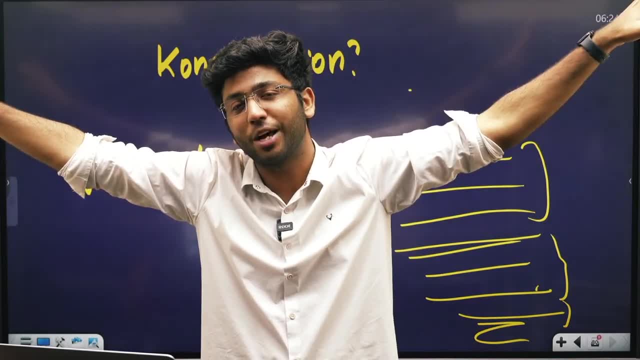 My tenth passed. Now I will do 11th and 12th. I will do very well. Shobit brother is with me in 11th and 12th. There will be no tension, Okay, Shobit brother is with me in 11th and 12th. 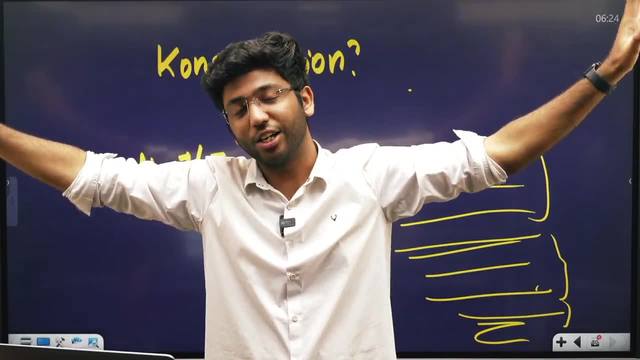 Like it. So Shobit brother is with me in 11th and 12th. There will be no tension. I am always with you. Your paper will go very well. It will go very well. I guarantee you that All these things will be done by me. 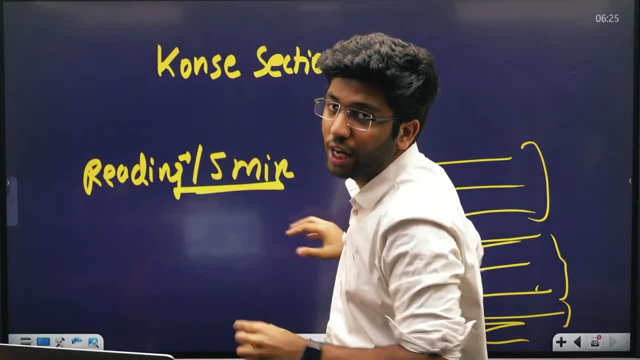 You will get to see a lot of questions from all these questions. So see this PDF once If you get the time. If you don't get it, it's okay. You just saw it. Okay, All the very best. Thank you so much. 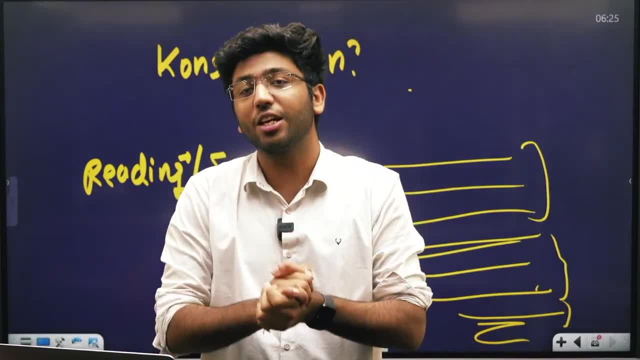 We did a marathon of four days. Okay, We did a very good marathon of four days. I am standing with you all the time, from 24 to 24.. Okay, You stand with me. Thank you so much. I love you so much. 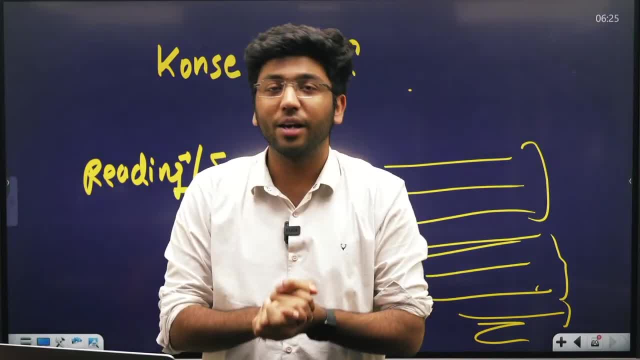 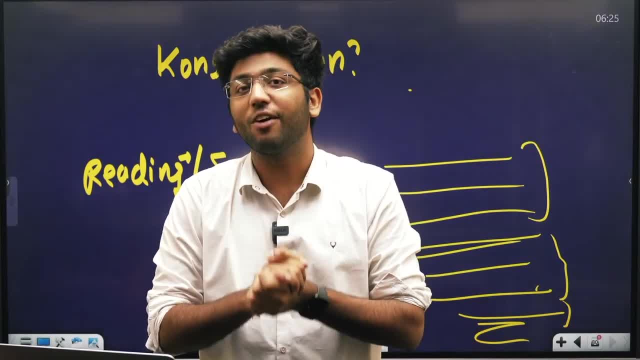 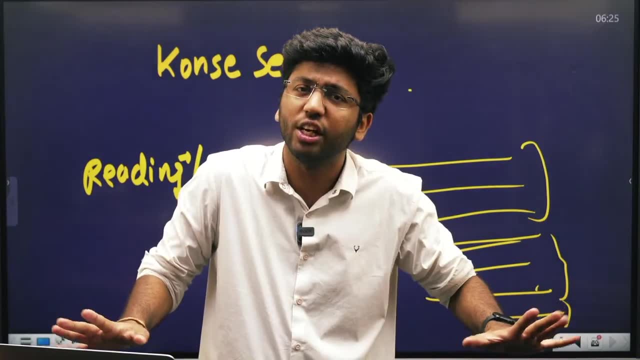 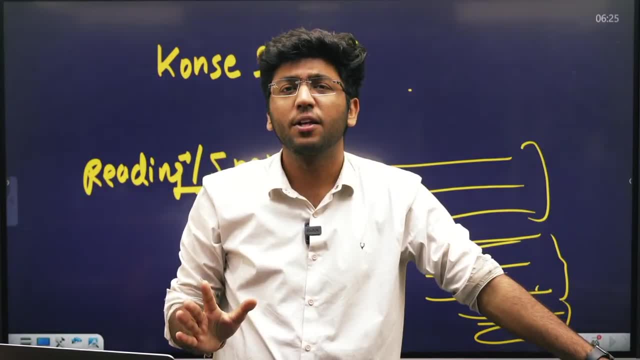 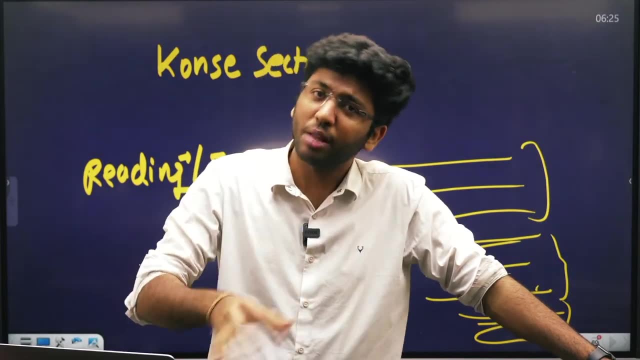 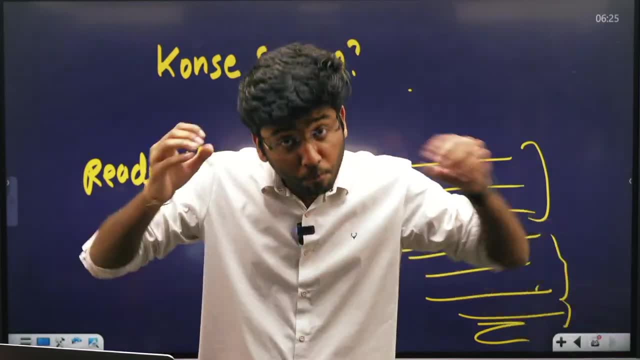 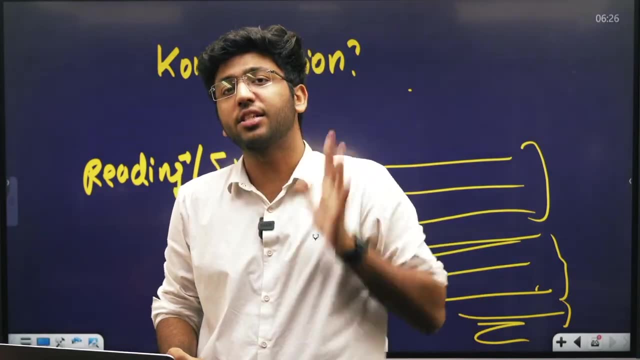 So it doesn't matter which you are in which thing and how many marks you are getting. The main thing that matters is whether you have done your hard work or not. You have done your hard work or not, It doesn't matter. I am giving my 100%. 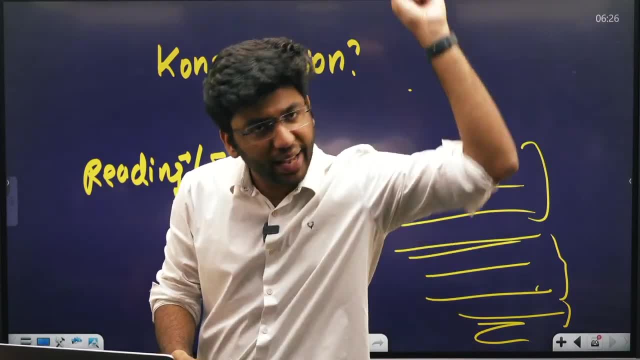 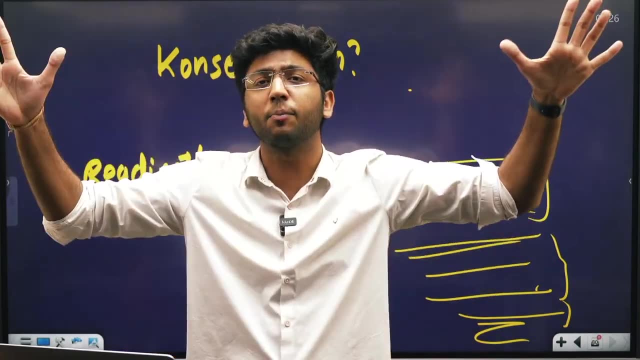 I woke up at 4 in the morning. I woke up at 4 in the morning. Until the last moment in the exam, Until the teacher didn't come to snatch the paper from me, I kept writing. till then. I gave my 100%. I gave my 100%. 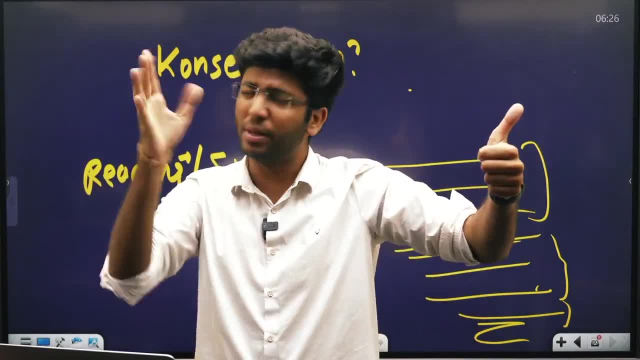 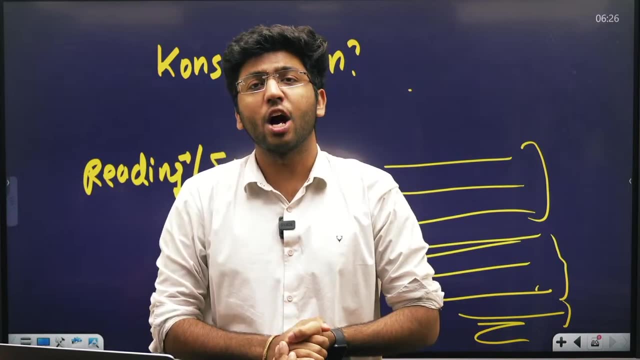 That's it. you will see what will happen. You will get the stream of your choice. All the school people give it to you. there is no problem, You will get the stream you want. Okay, showbiz is with you. Break the paper, Burn the paper. 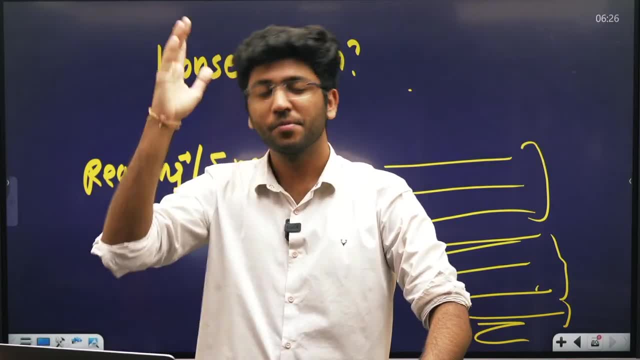 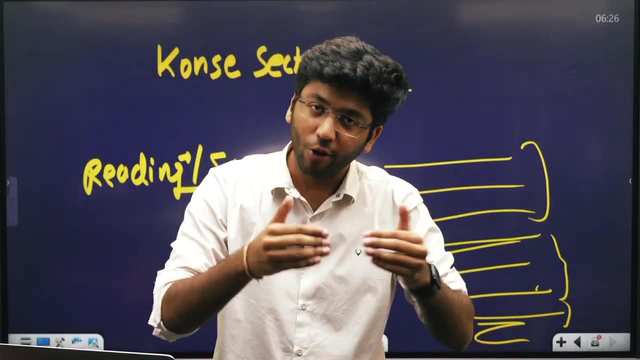 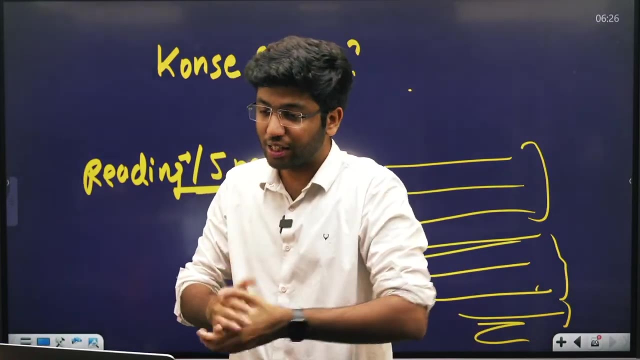 Got it And tell me how was the paper. You will like it And I will try to come to a school near Delhi. So all the students who live in Delhi Go out and see If I am standing there. meet me, Don't hide from me, Let's meet. 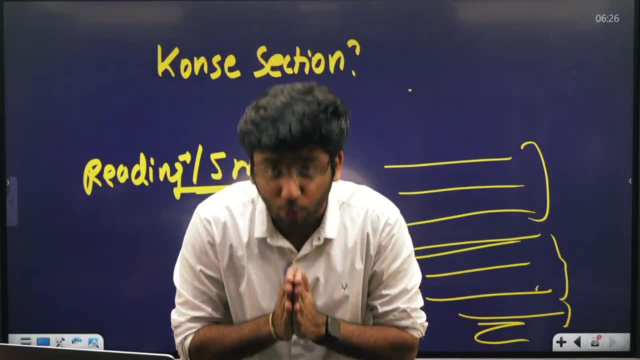 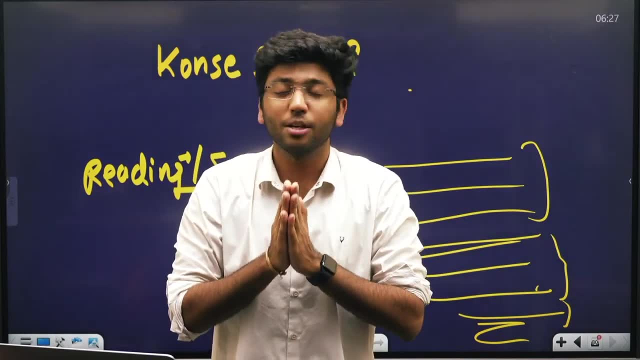 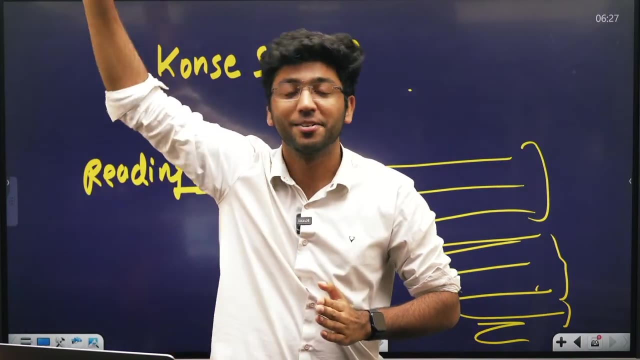 I won't take much time. Thank you so much. If I have made a mistake, I apologize. If I have said something wrong, I apologize. You all are very nice. Best of luck, Showbiz's best wishes to you. Go and break the paper. Go fast, bye, bye. 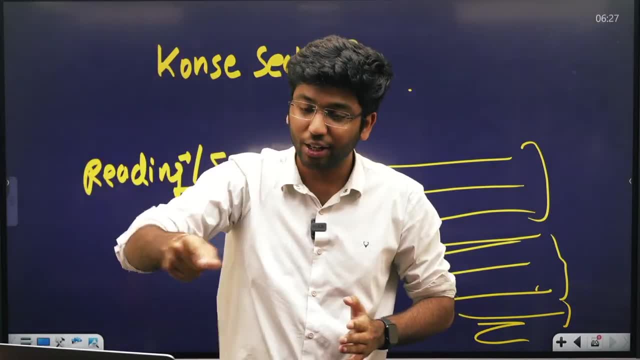 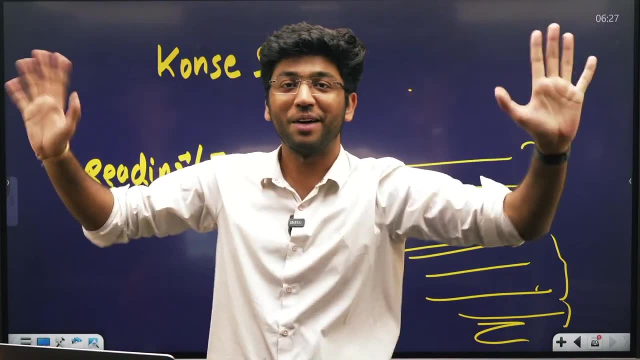 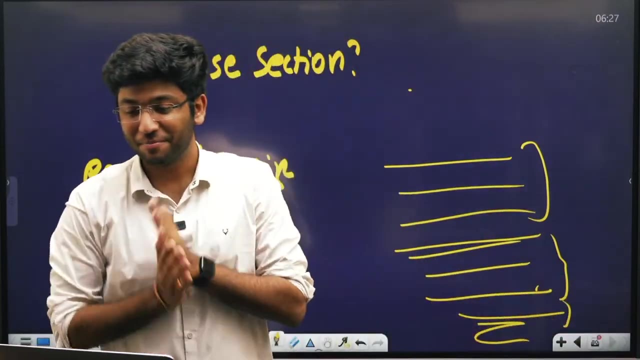 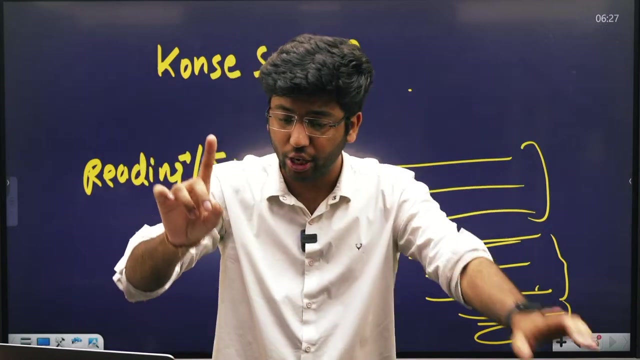 Good morning, bye, bye. Go and break the paper. Close it fast. I will give a pdf on telegram. Go and burn it. Thank you so much, Bye, bye. You are very nice, Thank you so much, Bye, bye. See you. Tell me how was the paper. And one more thing. 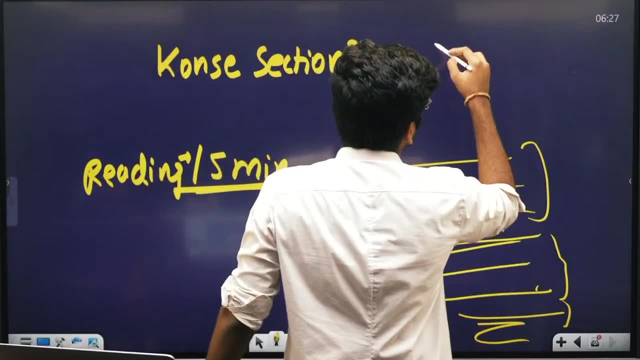 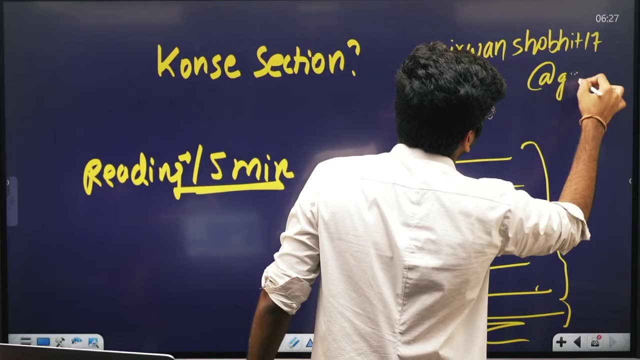 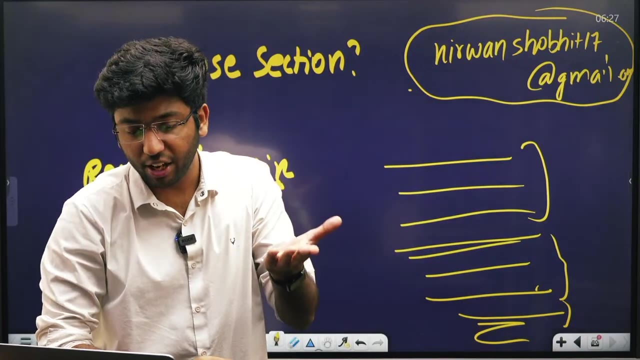 My mail id. You will get it on the channel mail id nirvanshobhitsatra at the rate gmail dot com. This is my mail id. Send me the paper On this mail id. Make a pdf And send me the paper. I will check all your sets. 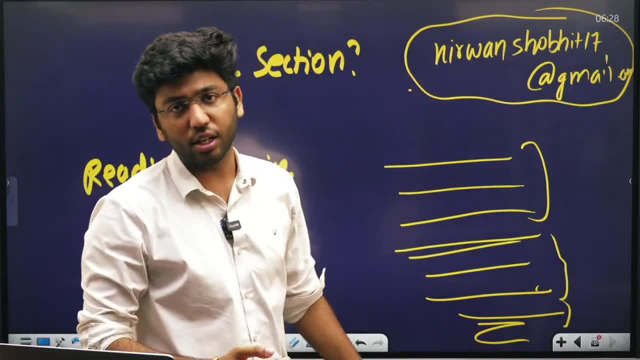 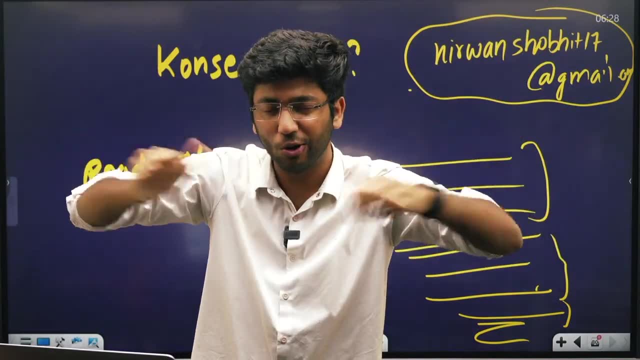 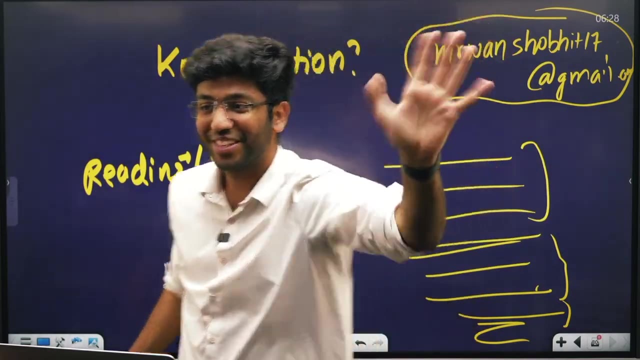 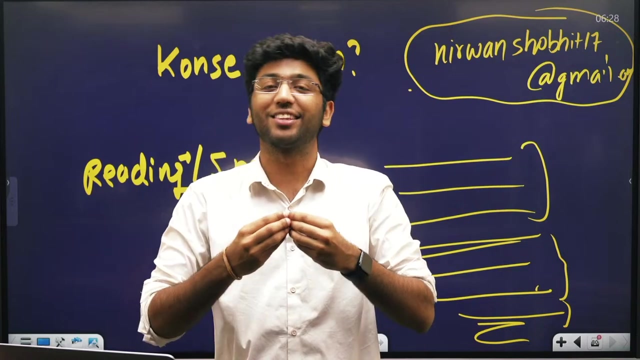 Send 2-3 kids, Send me the paper And I will come back. Bye, bye, All the best, Don't worry. Don't worry. Take the name of God, Go and break the paper. Bye, bye, See you. I don't want to go in front of you. I was very emotional. 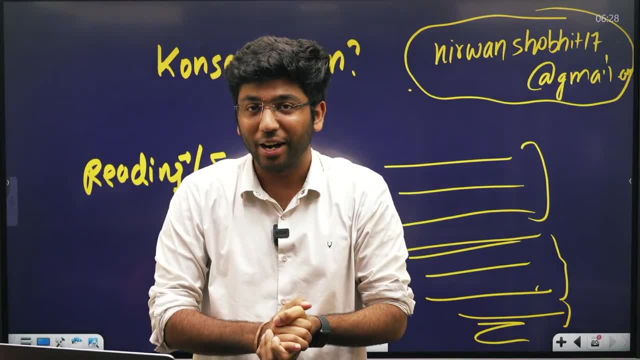 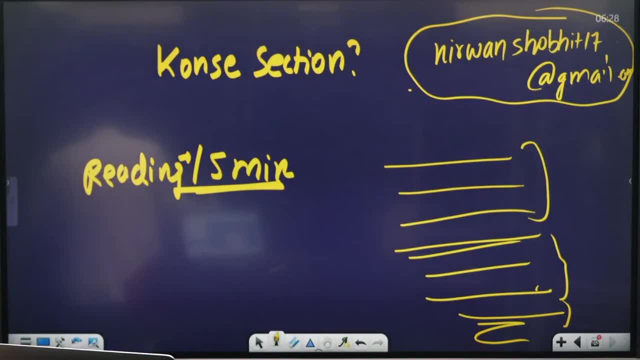 But no problem, See you, Bye, bye. Thank you so much. Bye, bye, All the best.